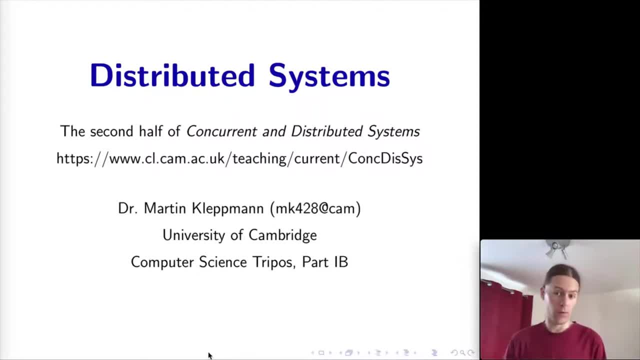 this network is part of what makes a distributed system distributed. Another aspect is also that we don't have a single shared address space anymore. So a pointer that makes sense in one process. if you send it over the network to another process running on a different computer, that pointer will. 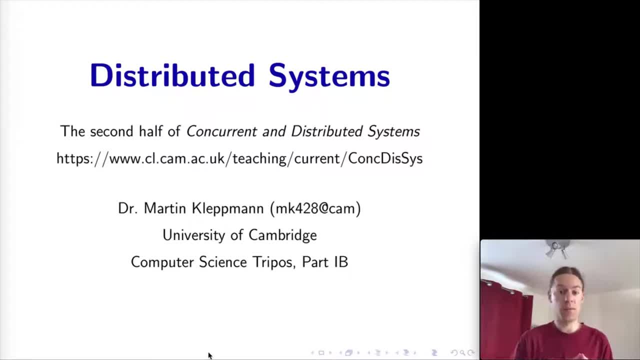 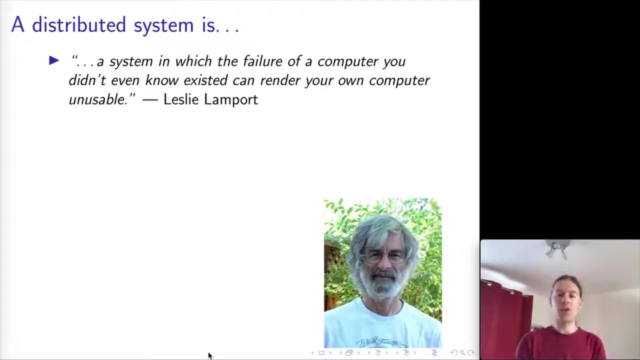 not necessarily make any sense to the recipient of that message, And so we have to think about different ways of sharing data between these concurrent entities. So a definition of a distributed system- a somewhat joking definition provided by Leslie Lamport- is that a distributed system is a system in which 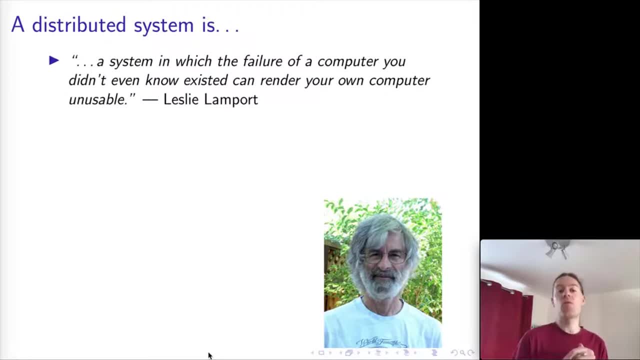 the failure of a computer you didn't even know existed can render your own computer unusable. Whether this is a good definition or not we can debate, but Leslie Lamport is a bit of a legend in the area of distributed systems and we will see various aspects of the work that he's done. 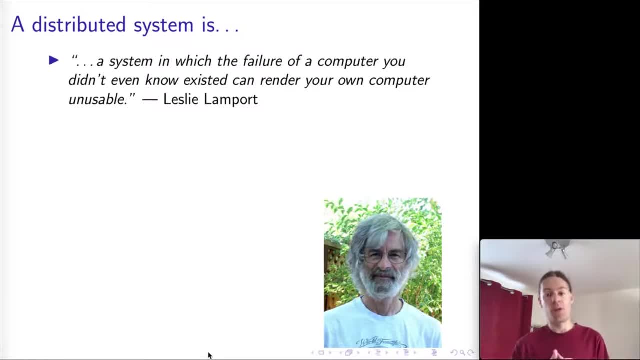 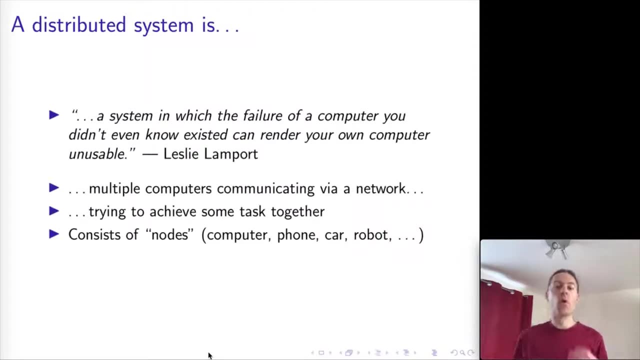 Over the decades and of course, lots of other people have done work in this area and we will see that over the course of these lectures. So more generally, I think I would define a distributed system as one in which you have got multiple computers or computing devices. These devices 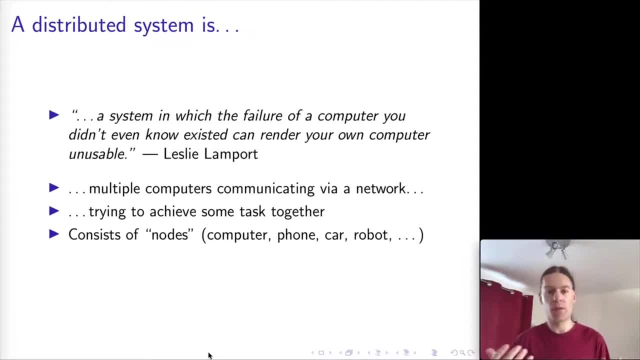 might be smartphones, they might be robots, they might be self-driving cars, they might be desktop computers, they might be servers in a data center. So any sort of computing system that you can use, any sort of computer, any sort of computer that you can use is a kind of a distributed system. 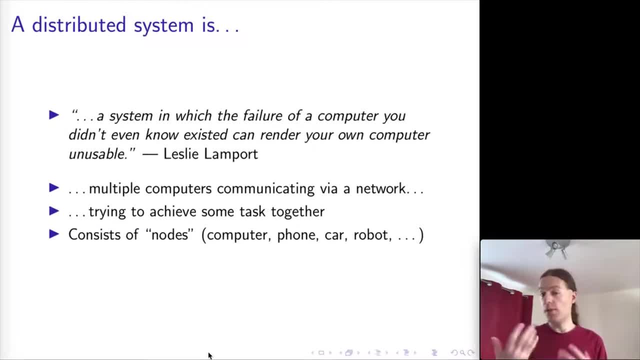 So we can say that distributed systems are a kind of computer. they are a kind of a computing device, really, and these computing devices are communicating via some kind of network, which might be the internet, and they are trying to achieve some kind of task together. And the study of 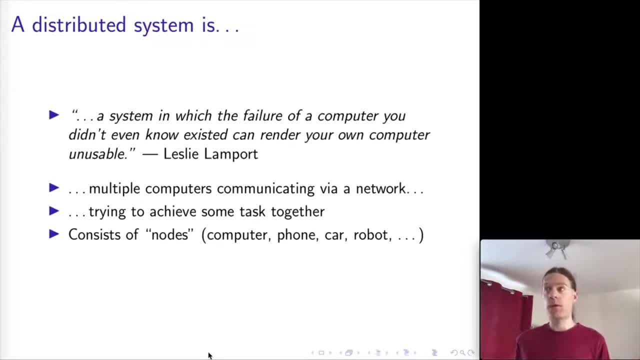 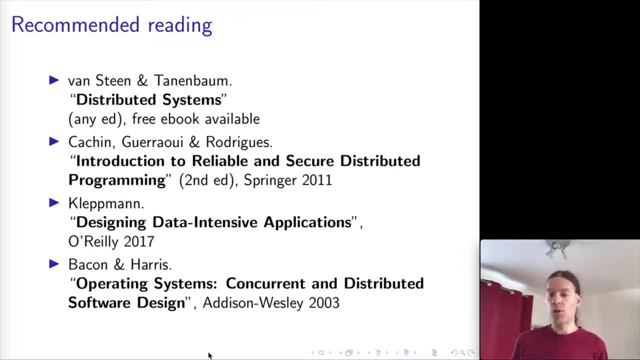 distributed systems is really the study of how do we coordinate the activities of these different devices in such a way that they achieve together the tasks that they are trying to achieve. So that's what we have done. So, first of all, if you want any further background reading, 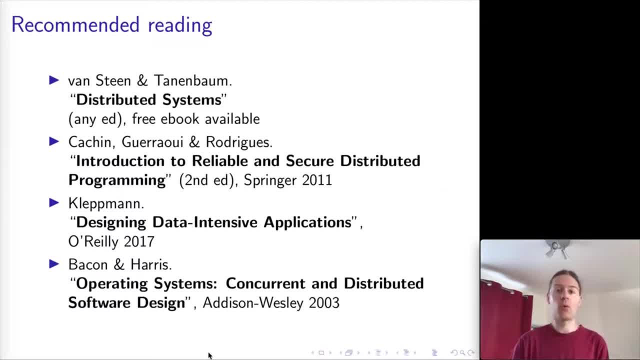 on this course. hopefully the lecture notes will be reasonably self-contained, but of course further detail is available in books if you are interested. There are several different styles of books that I've put here on the list, So the textbook by Van Steen and Tannenbaum. 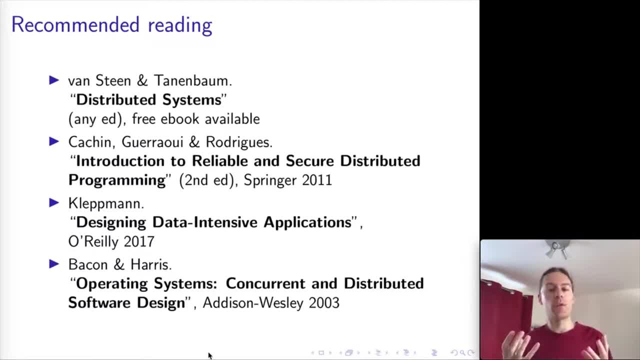 is a sort of systems level overview. So this comes at distributed systems from quite an applied angle to the application that real people use and discusses how these work and discusses the various implementation details of it. It doesn't go as far into the theory as some of the other books. 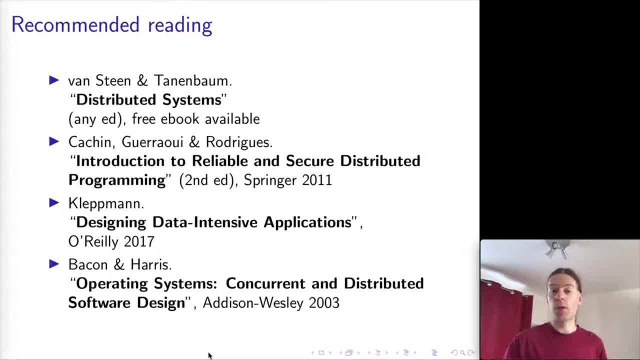 but it's more practically oriented. If you like the theory, then the second book on this list is a good choice. So the textbook by Kachin, Gherari and Rodriguez is an excellent but quite detailed overview of distributed systems theory. So it goes into a lot more depth than we have time to talk. 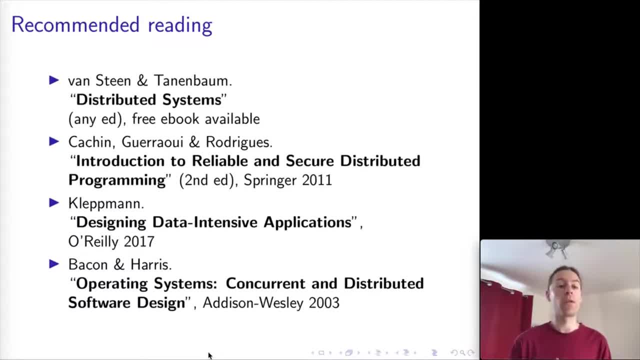 about in this course, but if you want to read more about the theory, this is an excellent book. I also wrote a book in this area called Designing Data-Intensive Applications. This book is a bit more oriented towards distributed database systems, So it's not just 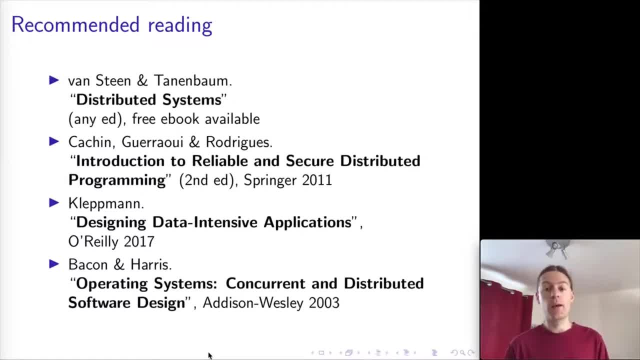 distributed systems in general. there's a lot of other databases content in there, but this book is more oriented towards industrial software engineers, So people who are working professionally with distributed databases will probably find this kind of book useful. And finally there's the Bacon and Harris textbook. 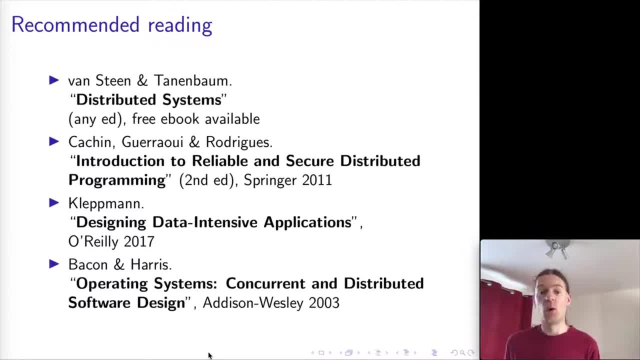 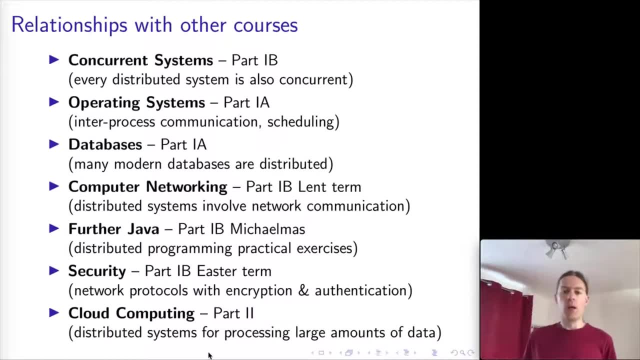 which was already recommended for the concurrent systems part of this course which really provides the link between operating systems and distributed systems. Okay, so this course is also connected to various other courses in the tripos- most obviously concurrent systems- that this course is part of. 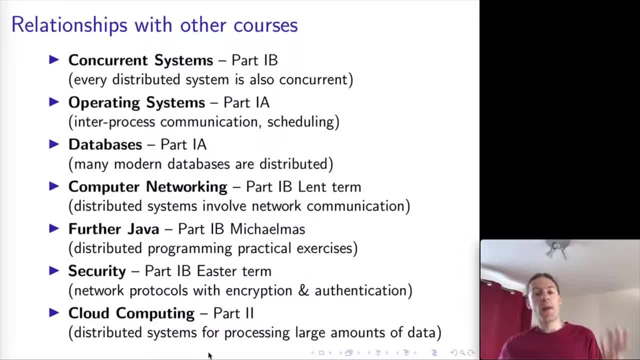 Also operating systems, which you studied last year. So all of the background that you had there- processes and inter-process communication and scheduling processes- all of that stuff is relevant for this course. Also, the databases course is connected to distributed systems because, as I mentioned just now, 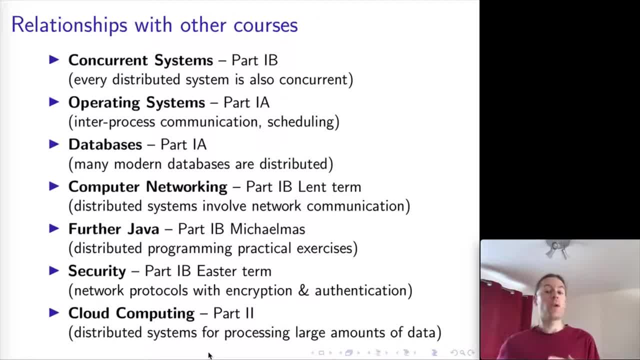 many modern databases are in fact distributed, and they use a lot of the techniques that we will talk about in this course, And so using modern databases often involves using distributed systems as well. There's a strong connection between distributed systems and computer networking because, as I say, 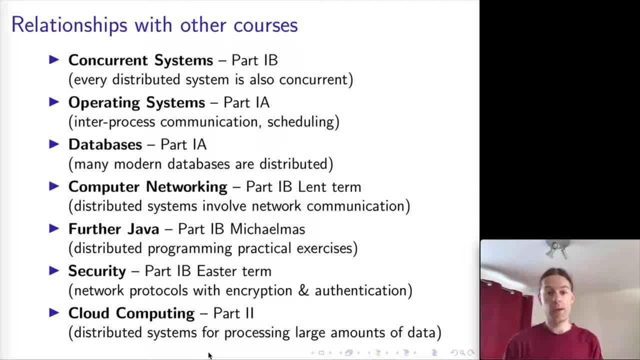 distributed systems involve network communication generally. The difference between the two courses is that the computer networking course is mostly about how do you actually get the bytes over the wire from one device to the other device. So what do the network protocols look like that enable devices to communicate? 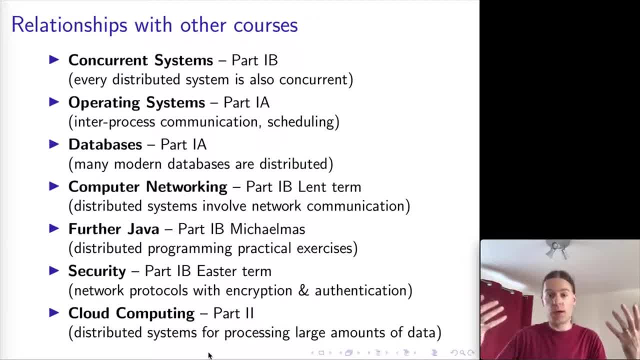 And then distributed systems builds on top of computer networking and saying: okay, assuming we now have this mechanism for devices to communicate, how can we now ensure that these devices behave in the ways that we want? There's connection to further Java, So there's programming exercises. 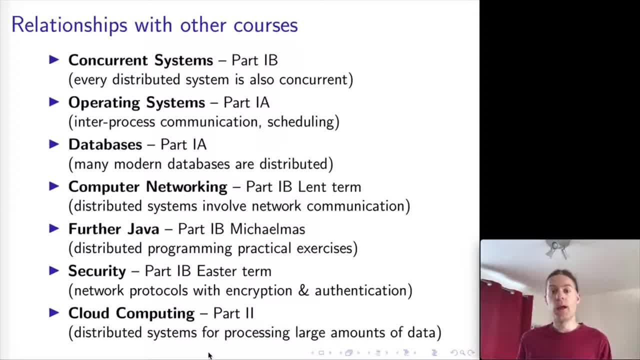 that involve a bit of distributed computing. The security aspects of distributed systems are very interesting and they are covered in a course in Easter term that's dedicated just to the topic of security. And finally, next year's cloud computing course builds upon distributed systems, because cloud computing is all about. 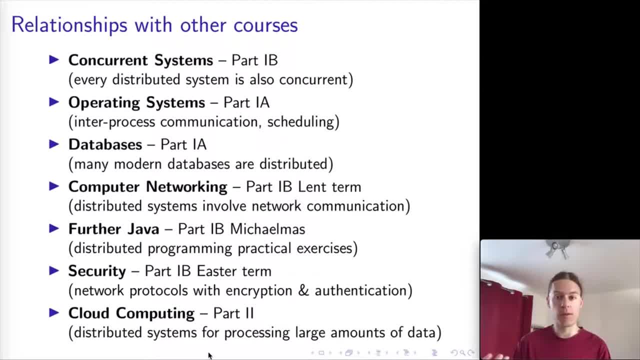 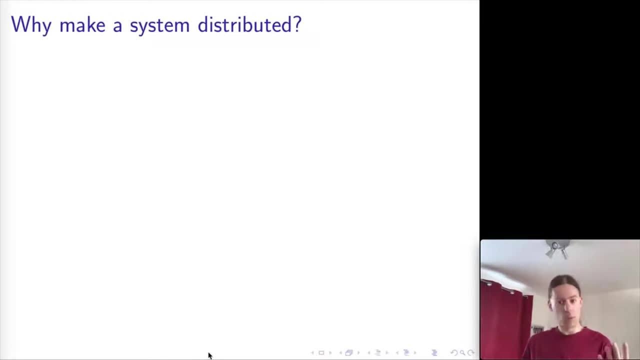 being able to flexibly process large amounts of data, And if you have sufficiently large amounts of data, you generally need a distributed system in order to process it. Okay, So I gave a brief definition of what a distributed system is. The next question is then: why, like why, should we go to all of this effort of making a system? 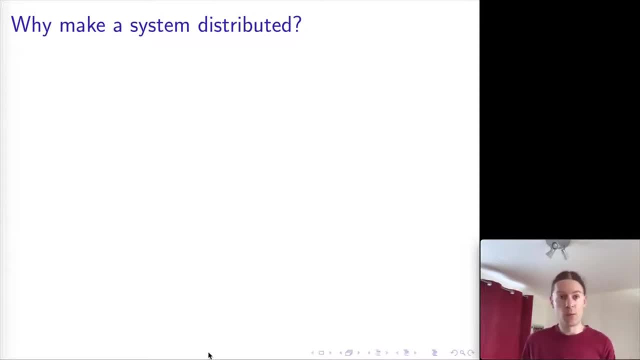 distributed. Why can't we just use a single computer and keep things simple? And well, one reason is that we don't have a single computer. We don't have a single computer. We don't have a single device. We don't have a single device. We don't have a single app. We don't have a single device. 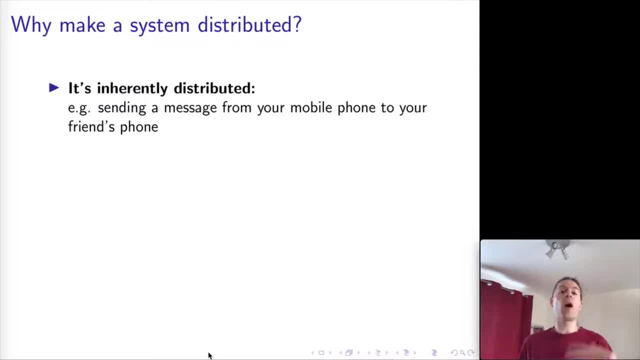 So the reason you want to go to all of these different systems is that some applications, some types of things you want to do, computers are inherently distributed. So if you want to send a message from your phone to your friend's phone, this inevitably involves two different. 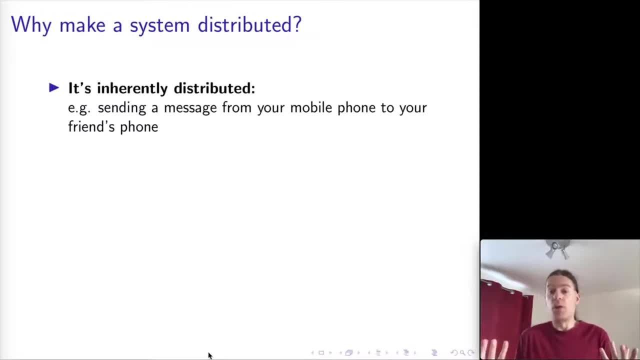 phones and a network, So this is a distributed system. There's no way around it. There's no way of building a messaging system that is not distributed If you want to be able to communicate across different devices, And so building this type of software is one reason why. 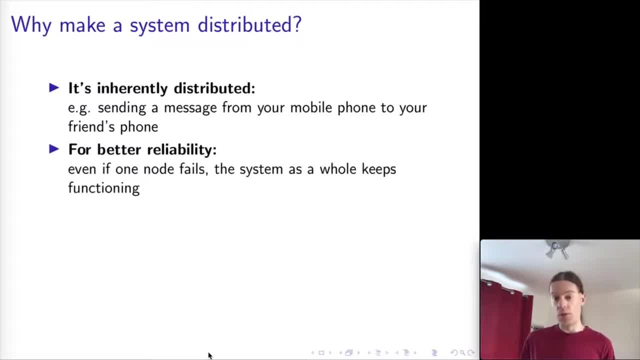 we might be interested in distributed systems, but there are many other reasons as well. So another good reason for being interested in distributed systems is that it actually allows us to make systems more reliable, And the reason for this is, say, you have multiple computers. 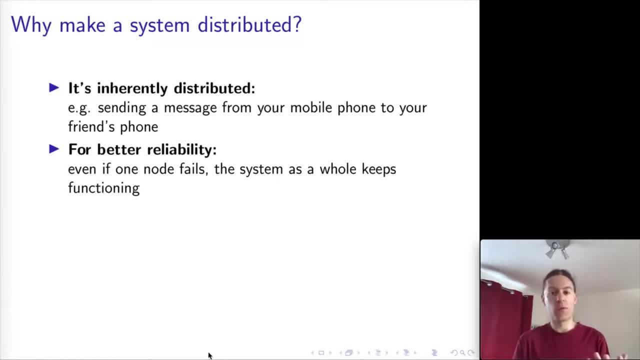 which are each performing part of some job. If one of those fails- maybe one of them has to be rebooted, for example, or one of them has a hardware failure- then maybe the remaining computers can take over the work from the failed computer, And so now this allows the system as a 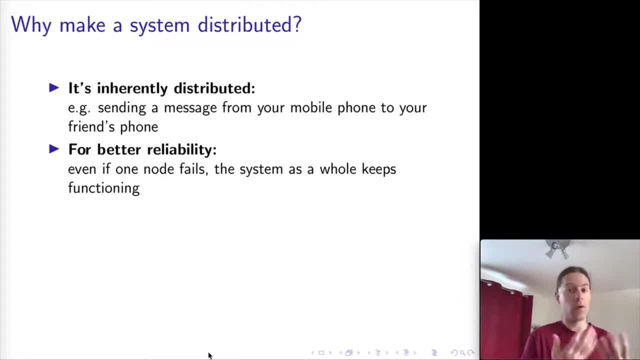 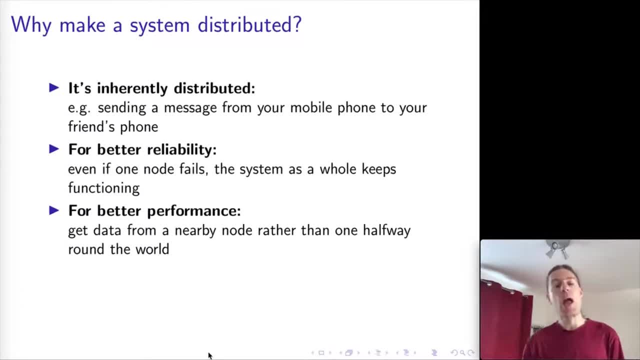 New Zealand, some users in South Africa, wherever- And there are large distances between these different places, And so network communication from one of these places to the others is always going to take a little- while You're talking- at least 100 milliseconds, simply because of the speed. 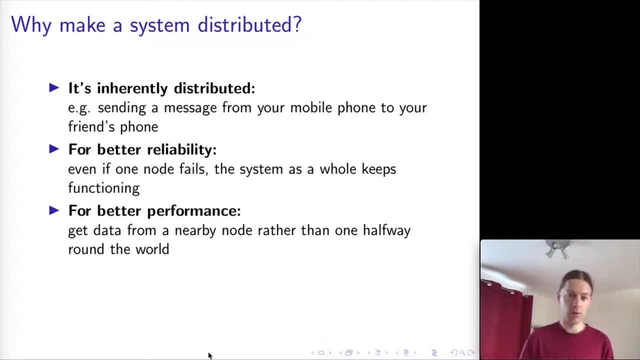 of light that it takes for communication to travel from one continent to another, And so one reason why people are interested in distributed systems is to make systems faster by putting data closer to where the people are. So if you have some users in multiple different continents, you can have 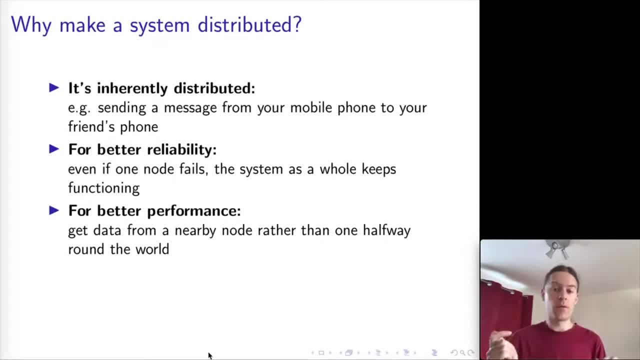 computers in multiple different continents And if you have each user communicating with the computer that is most local to them, then you avoid the long distance intercontinental communication as part of the delays that are added to their communication. So making systems distributed allows us to make them faster, potentially, And finally, another reason why people build distributed. systems is because of the speed of light. So if you have a computer that is most local to them, then you avoid the long distance intercontinental communication as part of the delays that are added to their communication. So making systems distributed is because of the speed of light. And finally, 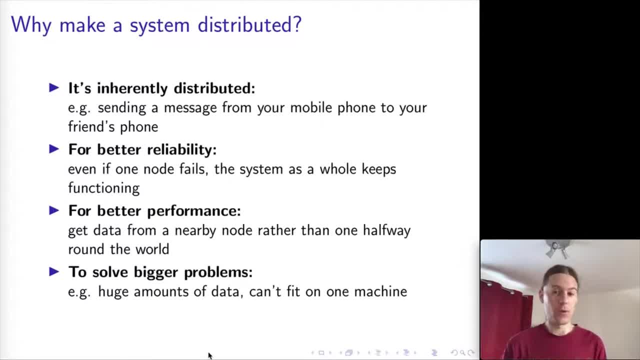 is to solve bigger problems than they could with a single computer. So some computing problems are simply very large scale. So think of scientific computing examples like, for example, the CERN, the particle accelerator in Switzerland. that includes the Large Hadron Collider They have 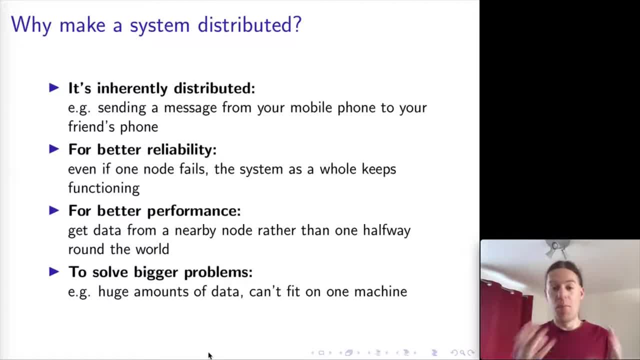 a vast computing infrastructure involving a million CPU cores and God knows how many hard disks, in order to just take all of the data that they're gathering from the computer and put it in a from the particle accelerator and process it and analyze it and try to use this to discover new. 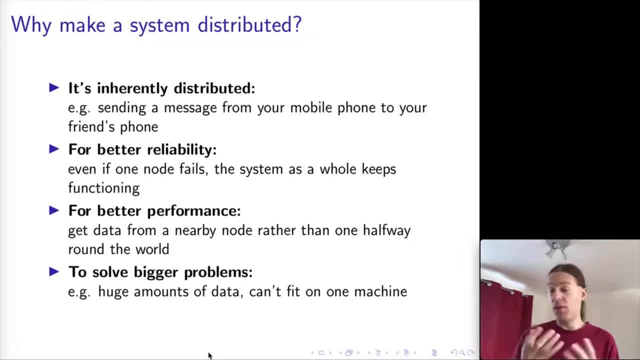 particles, for example. Now, this scale of task would simply not be possible to achieve on a single computer, because there is no supercomputer that is big enough to be able to handle these vast volumes of data. So simply solving this problem of analyzing such large volumes of data has to be 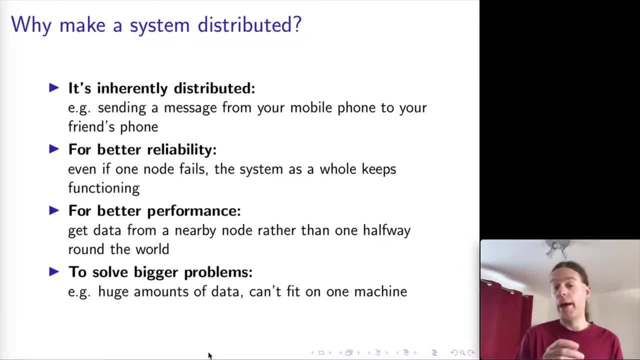 done on a network of lots of small computers. So if you have a computer that is big enough to handle large volumes of data, then you have to do a lot of work And those computers have to distribute the work amongst them and they have to work together in order to achieve the tasks that the scientists 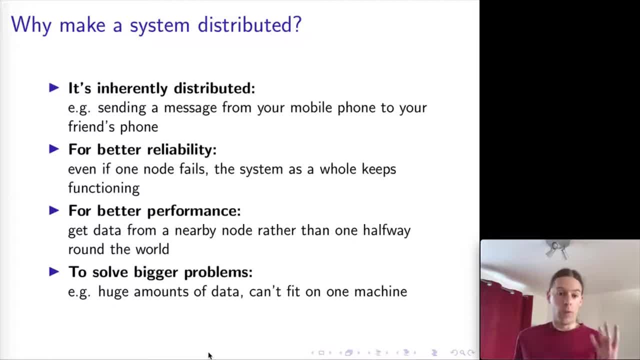 are trying to do, And so this is really one of the another key area in which we can use distributed systems is to solve bigger problems. Now, those are the advantages of making systems distributed. There are, unfortunately, some significant disadvantages as well, And the main disadvantage 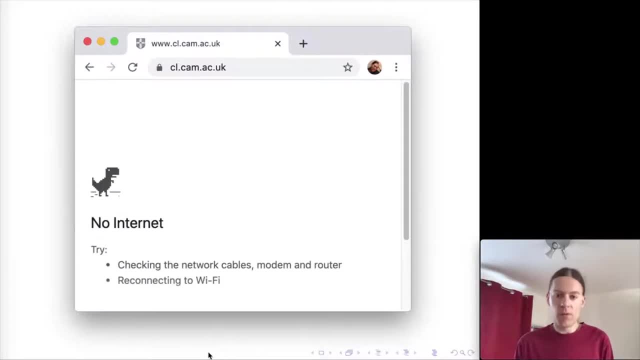 you will be well familiar with is whenever you're trying to do something over a network, that network might not be working for some reason, And so everyone has experienced what it's like for the internet to be down or for your Wi-Fi signal to be weak, or for you're in some rural part of the country. 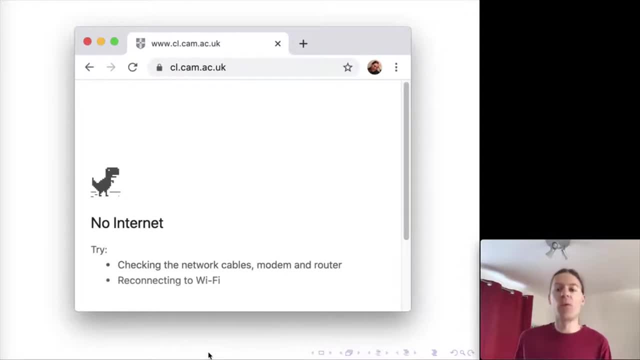 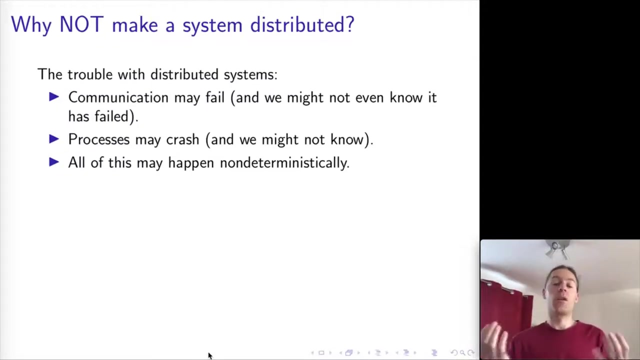 and your cellular data signal is weak and you're trying to load a map or something like that. Everyone has experienced this kind of frustration before, And, well, the study of distributed systems is all about the study of such frustrations, So we assume, whenever we are building a distributed system that involves communication over a network, that 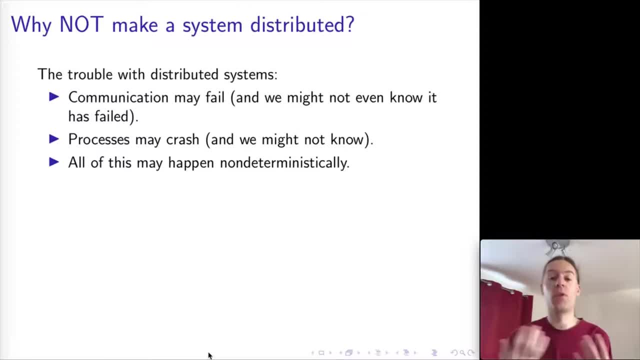 networks are not perfectly reliable, And so it is always possible for communication to fail. It is always possible that, because if it's a Wi-Fi network, you might be out of range. If it's a wired network, somebody might have unplugged the wrong cable. If it's any type of network, it might just be temporarily. 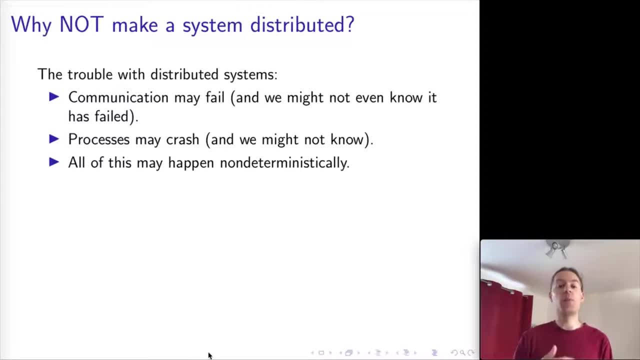 overloaded, dropping messages. Maybe even somebody might be maliciously trying to interfere with the network and cause it to drop packets, maybe causing a denial of service attack, for example. There are many reasons why communication might not work from time to time, And so we have to. 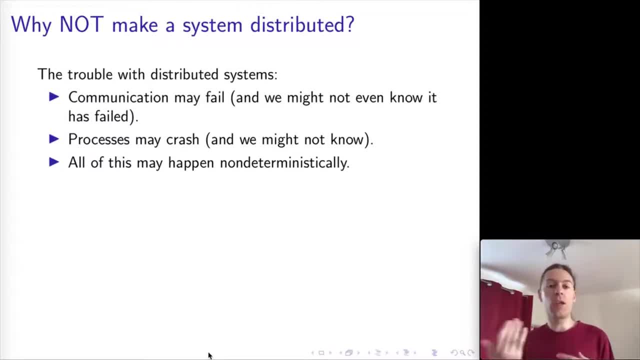 build systems that are robust so that, even if communication is interrupted from time to time, the system as a whole still functions in some correct way, where, of course, we can define what we mean with correct, but we want it to continue functioning. Another thing that can go wrong in: 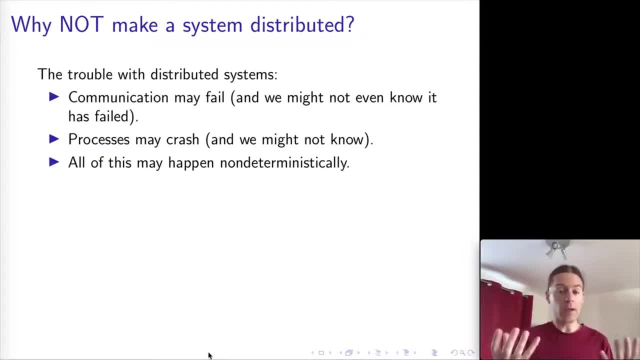 distributed systems is that some of the processes that are running the code might crash And, for example, if you have a system consisting of multiple computers and you reboot one of them, you probably want the remaining computers to carry on the task of serving user requests. 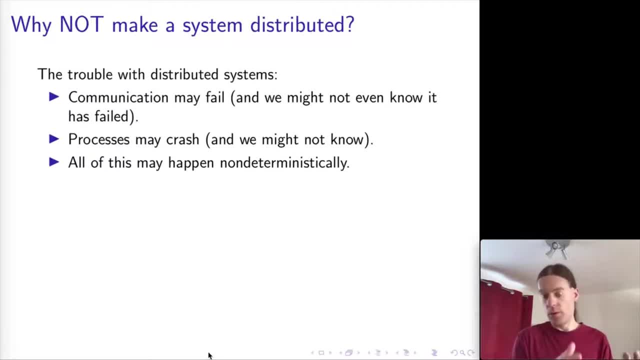 And so what we want here is that one of the processes is temporary, And so we want the system as a whole to still continue. nevertheless, And finally, all of these failures can happen non-deterministically, That is, we simply don't know when they happen. They. 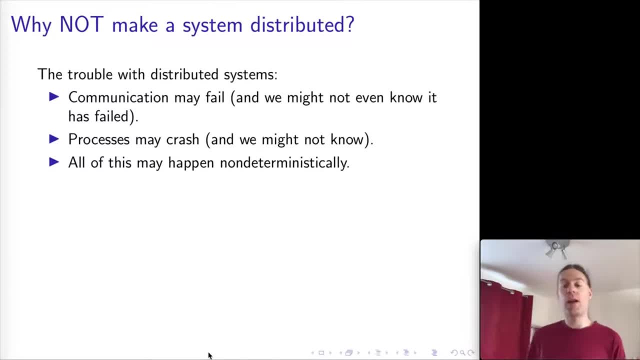 could happen at any moment, unpredictably, and we still have to ensure that the software works nevertheless. So what we often strive for in distributed systems is what is known as fault tolerance, which means that even if some part of the system is faulty, some part of the system is. 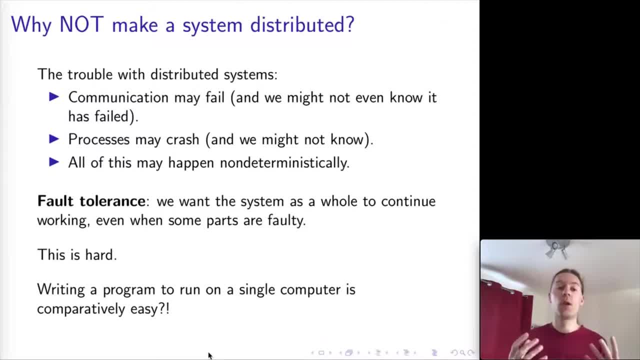 not working, the system as a whole still continues providing the service to the users, And so this is one of the main challenges in distributed systems — how do we make things in such a way that they can tolerate faults. In fact, making things distributed and fault tolerant is so. 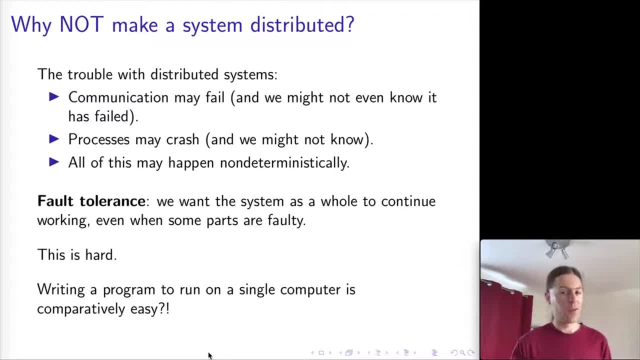 difficult that a lot of people who work professionally on distributed systems think that well, if you can solve a problem on a single computer, it's basically easy. So if you can solve a problem on a single computer, you'll probably have a much better time just keeping it on one computer, not overcomplicating. 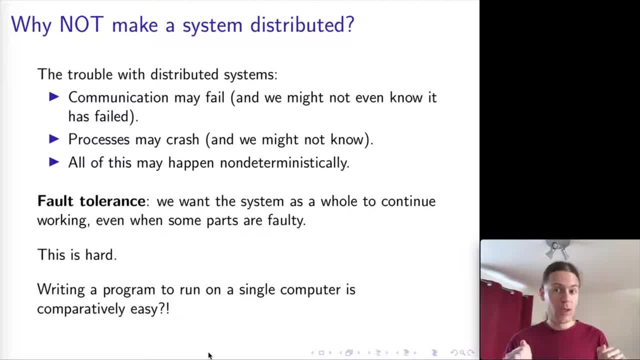 things not going into a distributed system setting, And so all of the problems, this Pandora's box of problems that arise with distributed systems. well, we should try and open that only if we actually have to. But, as we said earlier, there are lots of good reasons why you might. 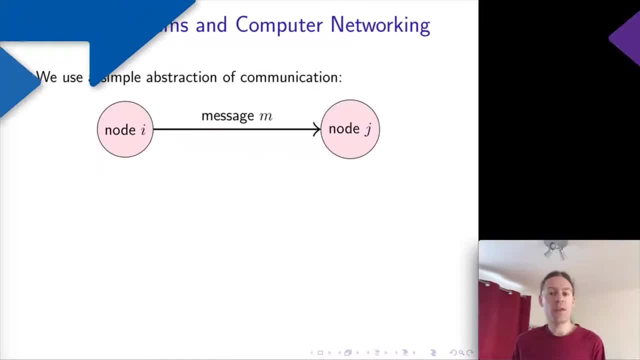 have to open that box. In this section I will talk a bit more about the relationship between distributed systems and computer networking. So in distributed systems generally, any computing device that is involved in the system we call a node. So a node could be a phone or a laptop. 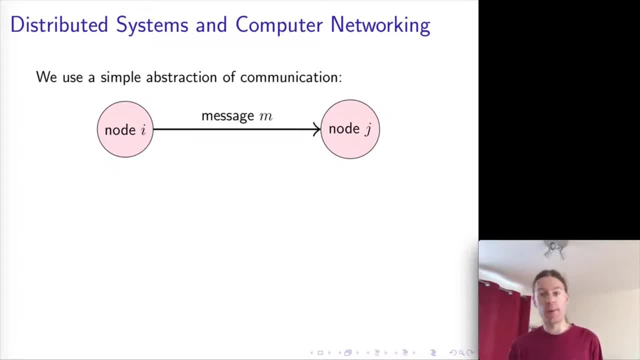 or a server in a data center or any of the other things we talked about earlier. And the fundamental abstraction of distributed systems, the communication abstraction, is that one node can send a message to another node. That's it. That's the entire basis of 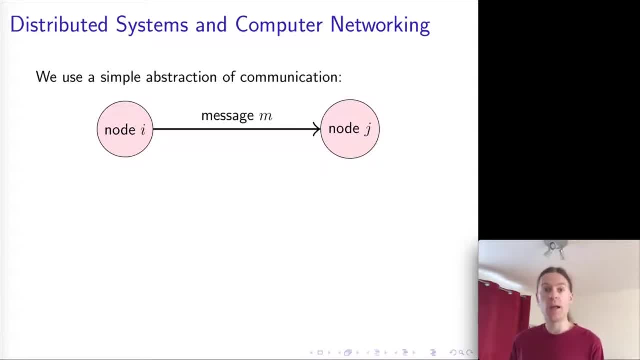 distributed system. One node sends a message, One node sends a message to another node, And this captures all of the possible modes of communication that can happen. Now, in practice, of course, there are lots of different types of network and different ways of getting a message from one node to another. So examples of that: 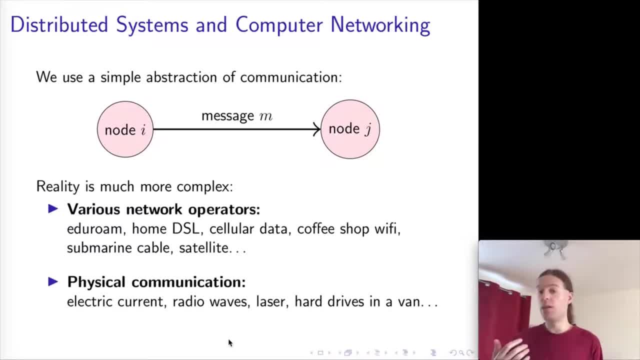 would be. if you're at the university, you will be probably using university-provided Wi-Fi or college-provided Wi-Fi. If you're at home, you probably have a home internet connection. If you're sitting in a coffee shop, you will probably be using the Wi-Fi there. If you're out and about in town, you will probably. 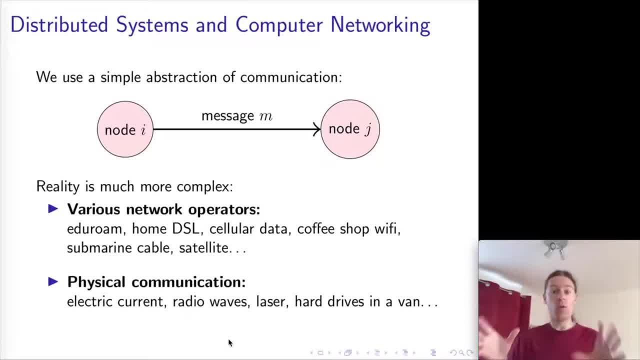 be using some cellular data on your phone, And that's only like the network that you connect to directly. On top of those, there are the backbone networks that form the internet, And there are lots of different types of network operated by all sorts of different companies. Some of those 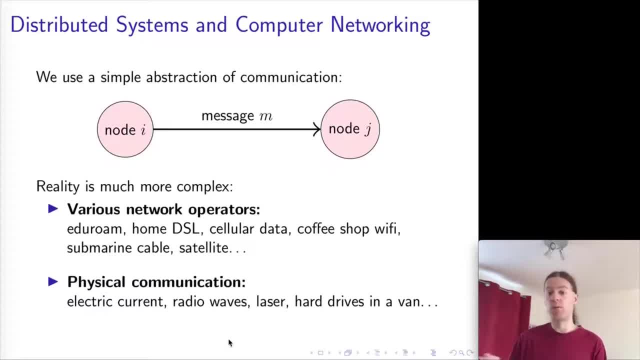 go via cables, copper cables, Some of them are fiber optic cables, Some of them go underneath the sea, Some of them go by the sea, Some of them go by the sea. Some of them go by the sea, Some of them go via satellite, and so on. All sorts of ways of getting messages from A to B. 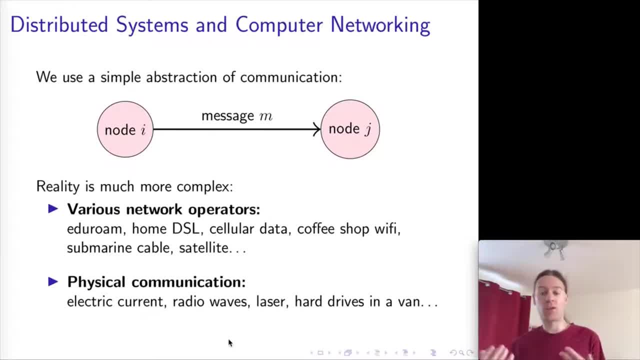 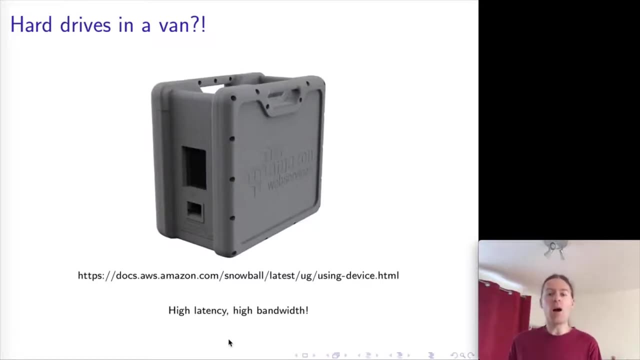 In addition, there are all sorts of physical communication mechanisms, such as electrical pulses on a wire, radio waves or lasers going down, fiber optic cables or even hard drives in a van. What Hard drives in a van? That's not a network connection. Well, I will argue that this is also. 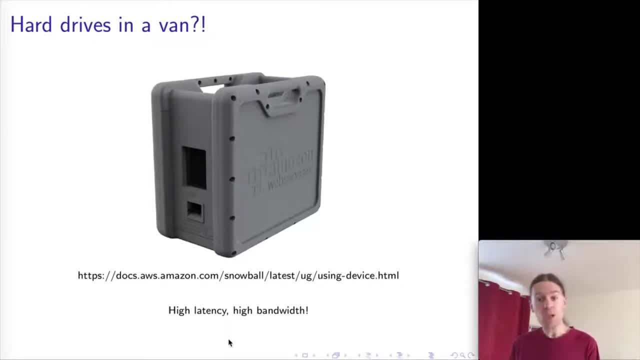 a mechanism from getting messages from A to B. So if what you have is a very large amount of data that you want to send to somebody else, maybe to transfer it to a different data center, then actually sending all of that data over the internet can be kind of slow and expensive. 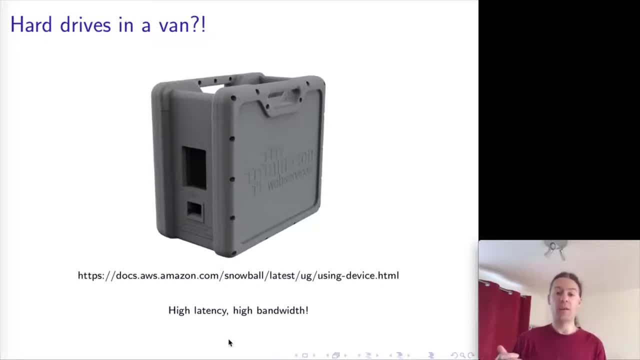 And it can actually make more sense to load all of the data onto a bunch of hard drives. load the box of hard drives into a van, drive the van to the destination And when it gets to the destination you can then download all of the data back off the hard drives and store them in. 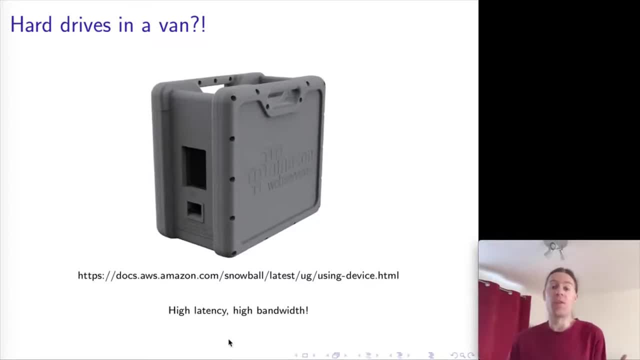 whatever system they need to be stored in- And people do this in practice, actually- And Amazon Web Services, for example, which is a big provider of data center services. they actually have this service where you can rent a box of hard drives from them and it will come as a career service And you can load all of your. 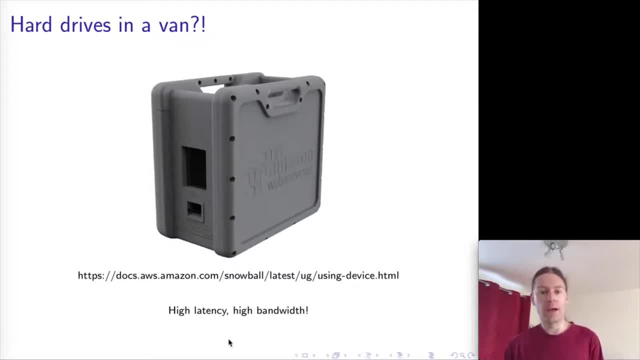 data onto it- It takes about 50 terabytes or so on one of these boxes- and send it back, And so of course this is a very slow form of networking because it might take a day or a couple of days, But it is also quite a high bandwidth form of networking, That is, you can transfer large 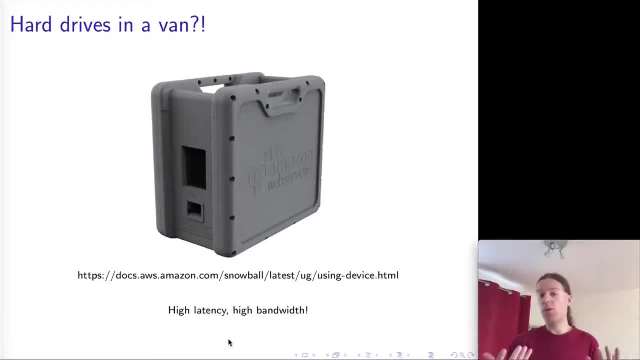 quantities of data, And I would argue that from a distributed systems point of view, this is just another messaging channel. It's another way of getting a message from A to B. The distinction is just latency and the bandwidth of those different networking channels. So latency varies hugely. depending on what sort of network you're looking at- Within the devices on your home Wi-Fi, for example, or within servers in the same data center- you probably get like a millisecond, maybe less than a millisecond, depending on how congested the network is. Latency- that is the. 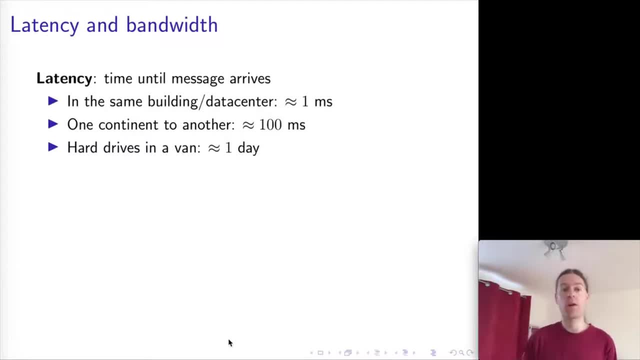 time that it takes to communicate from one device to another. If you're going over the internet and you're talking to a server that is located on a different continent, then it's probably more like on the order of 100 milliseconds. Of course, hard drives in a van will probably take a day or a. 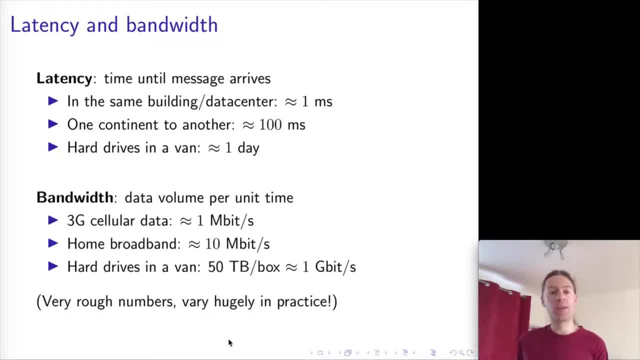 couple of days, But still, you know, it's just another networking channel. In terms of bandwidth, this varies hugely. Like a 3G phone might have like a megabit per second if you've got a good signal. It might be more like 100 kilobits per second if you've got a poor signal. Home broadband might be like 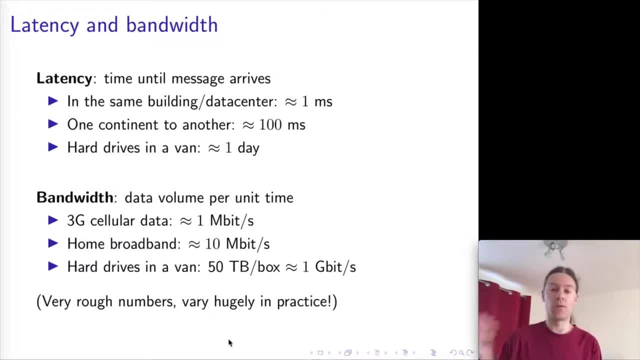 10 megabits. Of course it varies very much how close you are to the next provider, whether you have fiber and so on. Roughly estimating the bandwidth of a 3G phone, it's just another networking channel. Hard drives in a van. well, if you take one of these boxes and it takes a couple of days to do, 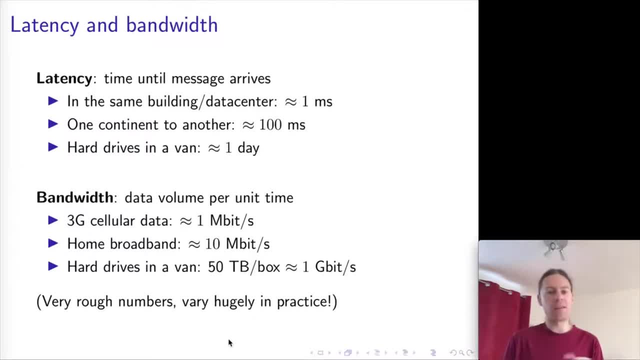 the whole loading data onto it, getting it to the other place, getting the data back off it again. you can probably estimate it as roughly being a gigabit per second or something like that. If you use one box, of course, you can send multiple boxes, in which case you can increase. 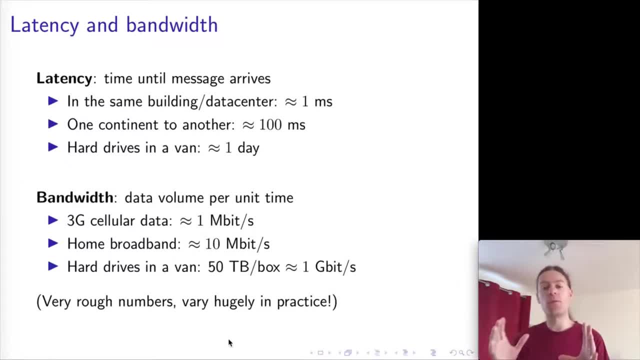 that number. Those are just very rough numbers, but just sort of to give you an idea of the order of magnitude that we're talking about with these. Now I'd like to show you an example of one concrete distributed system, which is a system: 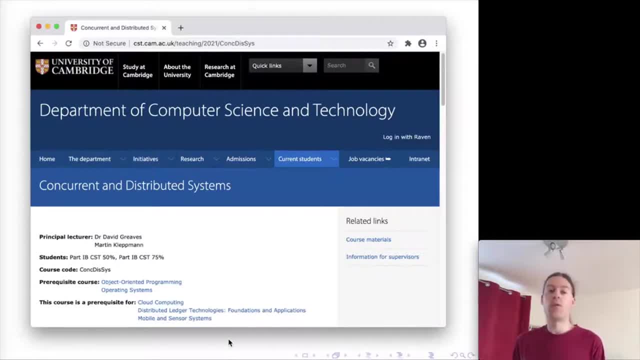 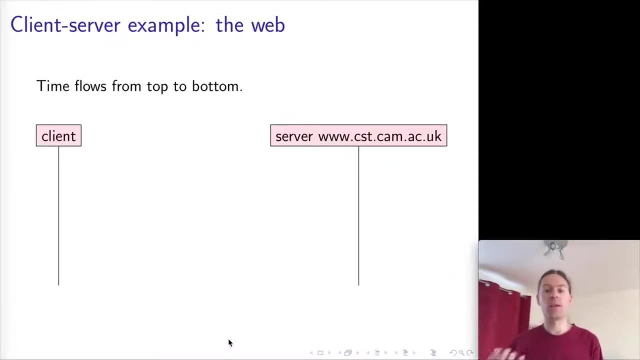 that you use every day, and that system is the web: The web we can now analyze through a distributed systems lens and see what actually happens when you load a website in a web browser. What happens there is that we have two communicating entities. First of all, 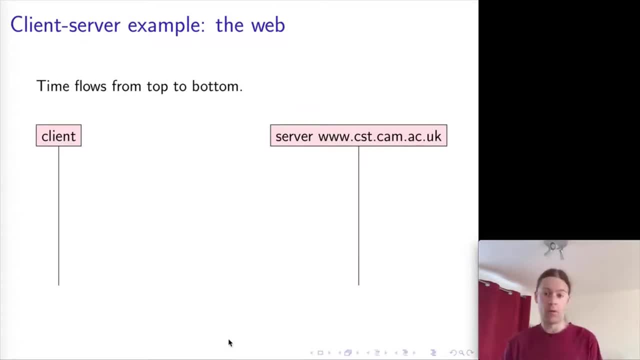 you've got the client, which is the web browser running on your computer or your phone, and then you've got the server, which is usually located somewhere in a data center, And when the client wants to display a web page, it makes a request, And so a request is just a. 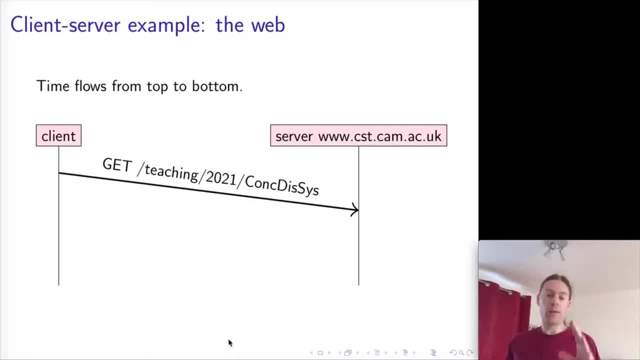 message that gets sent over the network and that request is targeted at a particular server and it contains the path of the URL that you're trying to load. So you notice in the URL you have the HTTP, maybe S, double slash. then comes the server name and then from the single, 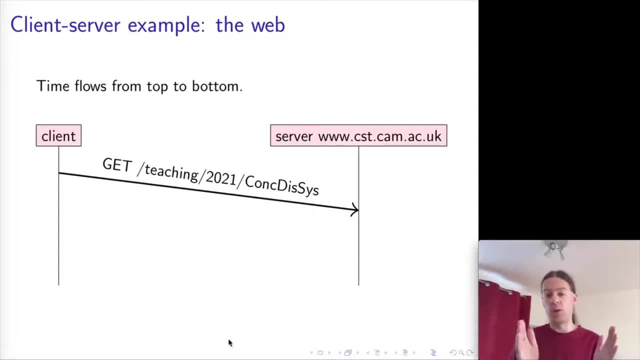 slash onwards is the path, And so the bit before that first slash is the server name, which is going to be the destination where we send the message to, and what follows after that is the path, which is then contained within the message that we send to that destination, And so that message. 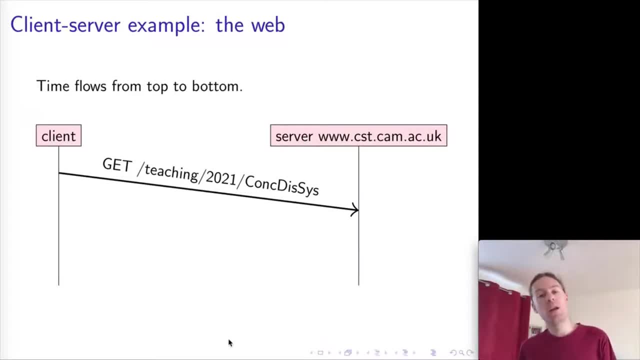 if you want to load a web page, we call that a get request, and it contains the path, and the server then will respond with the contents of that web page, And so that is probably an HTML page, if it's just a plain web page, but it could also be an image or it could be a video. 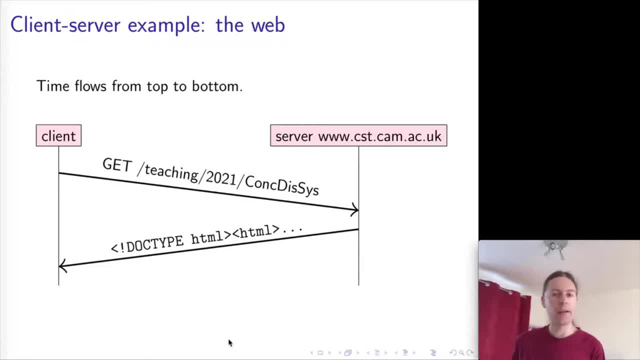 file, or it could be a PDF document or anything like that, And so what we have here is a simple protocol consisting of two messages: a request from the client to the server and a response from the server back to the client containing the data that the client asked for. So I'd like to now 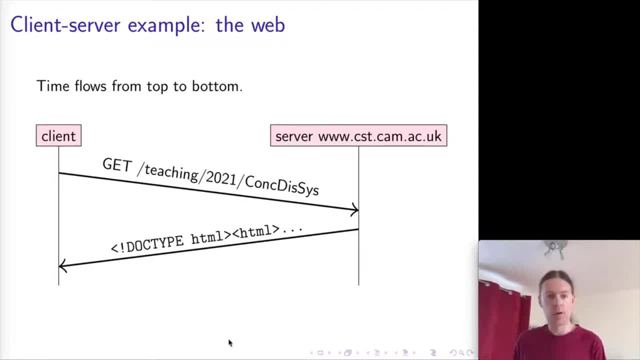 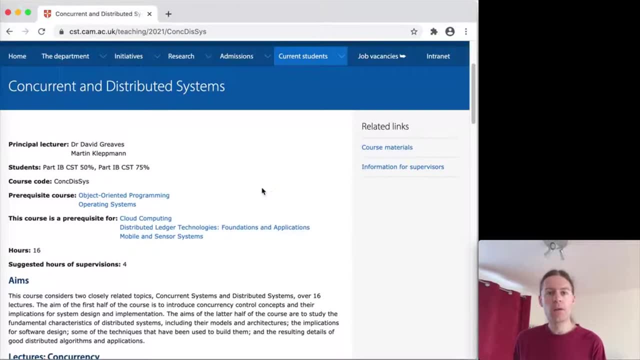 give you a little demo of what this actually looks like. And so, of course, you know what a web browser looks like. You know what a web browser looks like. You know what a web browser looks like Here I've loaded the course web page and I can scroll up and down and I can now record the. 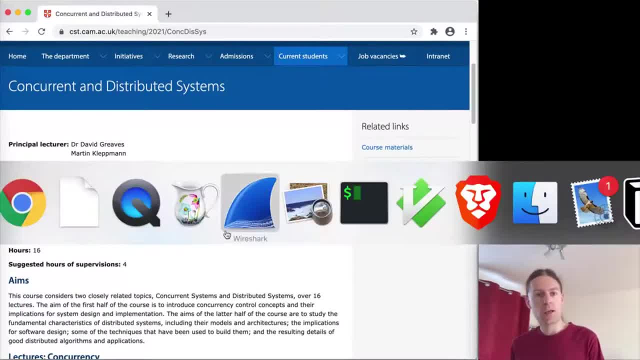 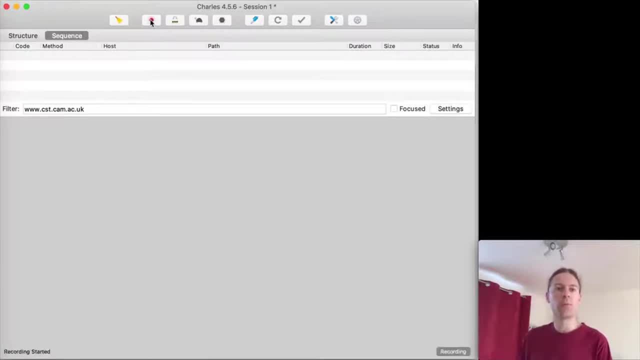 messages that are sent and received over the network using a network capture tool. So here I'm going to use a tool that's called Charles and I'm going to put it into recording mode. It's going to start recording and then I'm going to go here and just hit reload. 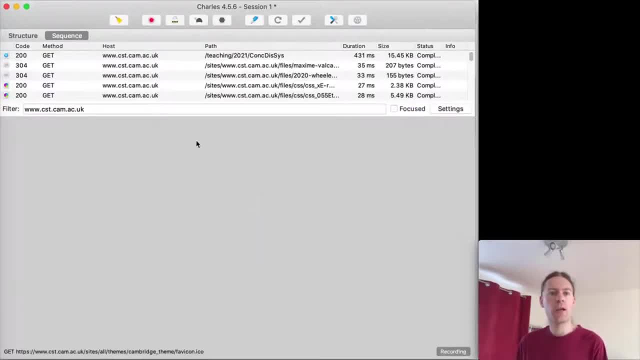 on the website. And so here we go. We've loaded the page again, and now I go back to Charles and we can see that we've now accumulated a whole bunch of requests. So each line here is one request message that was made from the web browser to the server. 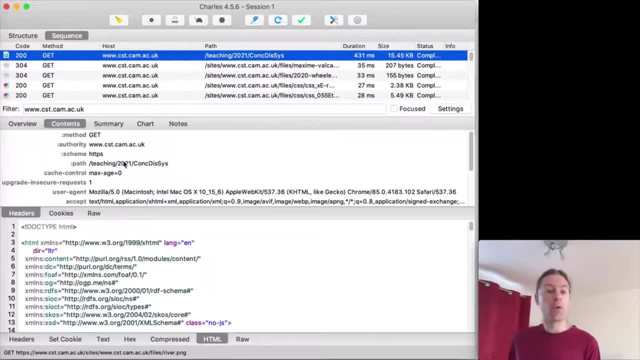 and it also contains the response that was sent back from the server to the client, And so here we can see. for example, this first request here was for this path here, which is the, the path on the web browser. You can see here in the URL that matches up with this path. 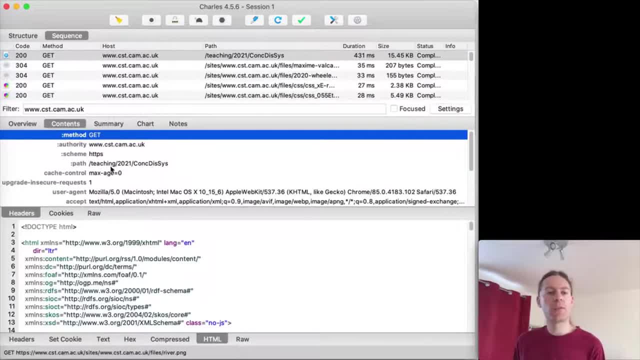 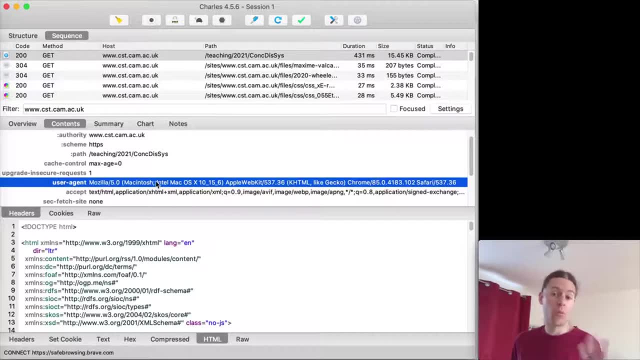 You can see, it's a GET request to load a particular website. You can see a bunch of information like this here. You can see here that this is the web browser that I'm using, So this is the agent here, for example, It's essentially the version of the web browser that I'm using. 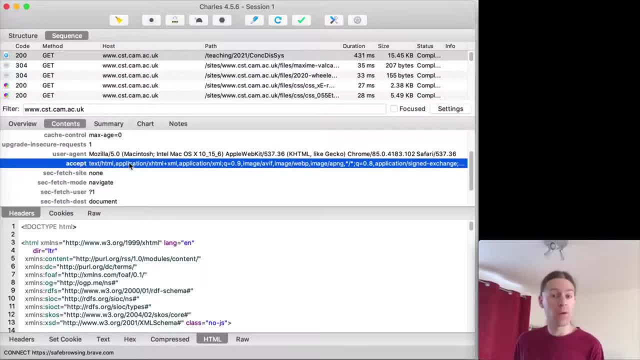 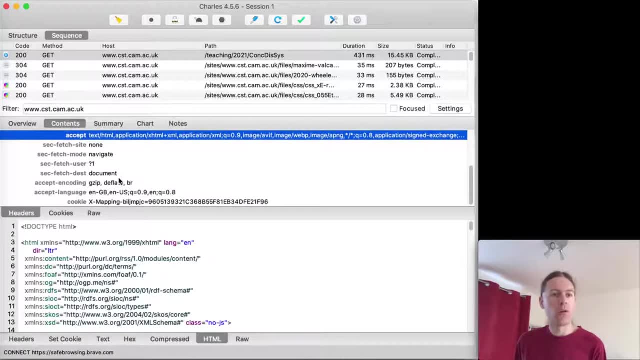 so it identifies the client software version Here this ACCEPT header. this indicates what file types the web browser understands. So it understands HTML and various other image formats and stuff like that. Then there's a whole bunch of other stuff here, like: what sort? 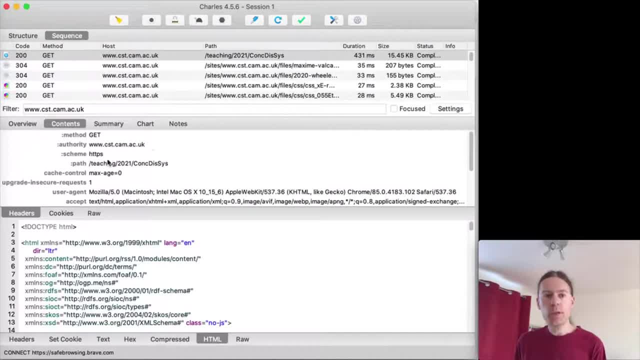 of compression, it accepts what sort of language I speak, and so on, So all sorts of stuff here. Here is the request message And then in the lower panel here you see the response message, And here the response message to this here contains some HTML And you can see the whole. 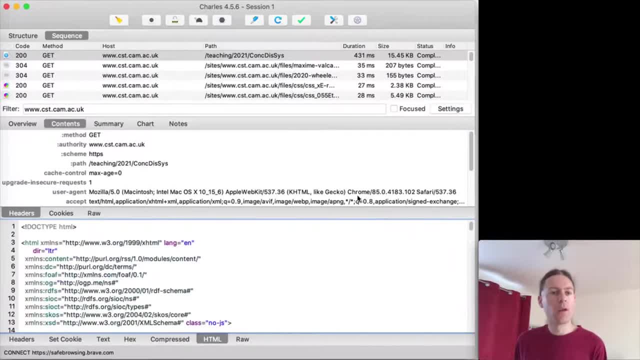 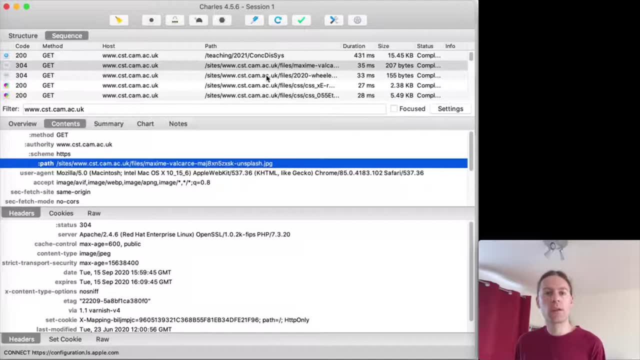 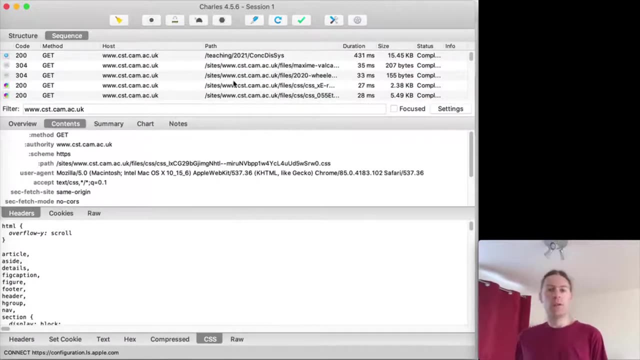 content of the HTML page. I can scroll down. It's a bit boring, Okay, And we can have a look at other requests here as well. So you can see this here. This looks like it's a picture that it's downloading, and et cetera. Here's some CSS, some style files and so on, So what we have is this. 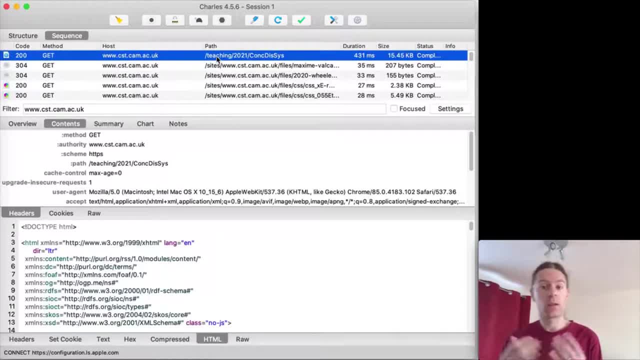 simple request response messaging protocol at the conceptual level. So at the conceptual level, here, at the distributed systems level, we're just talking about one message, one response. Now what happens at the underlying physical network level is a little bit more complicated. 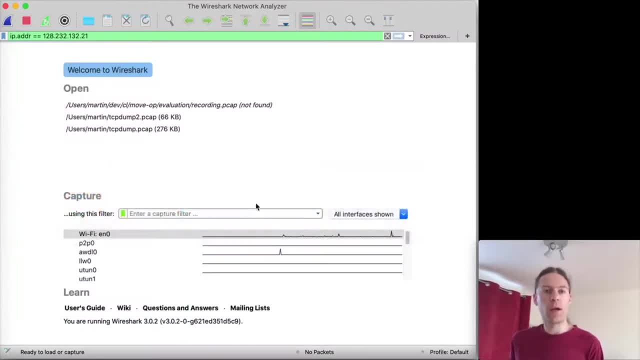 And so we can look at what happens on the physical level by using a different network capture tool. So I'm going to use a tool here that's called Wireshark, And this will actually capture, rather than capturing at the HTTP level, capturing the request and response. it's going to capture the individual network packets. 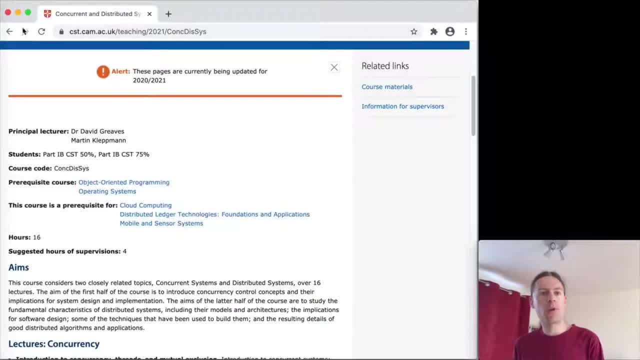 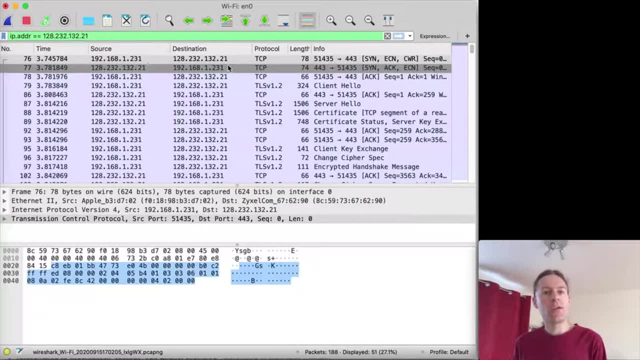 So let's see what happens here. I'll start recording and then I'll go back to the web browser and I'll reload again and go back here and hit, stop And here we now see, oh, a lot of activity again. And so here in Wireshark, every line in this table is a single network packet. 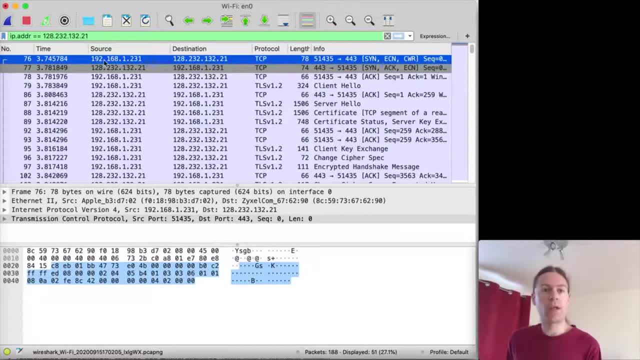 And so here you can see that there's a packet sent from one IP address to another IP address. So the 192.168,, that is the device, that is the IP address of my laptop on which I'm recording this right now, This 128.232, et cetera, that is the server, that is the name of the web server. 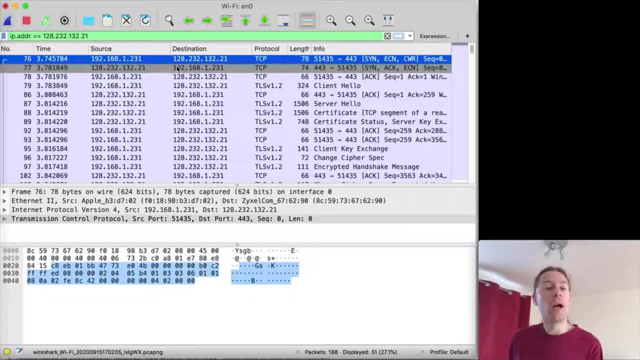 of the computer lab website that I'm connecting to, And so here you can see it's connecting using the TCP protocol. Don't worry too much about that. You'll learn a lot more about that in the future. So let's go back to the web browser and let's see. 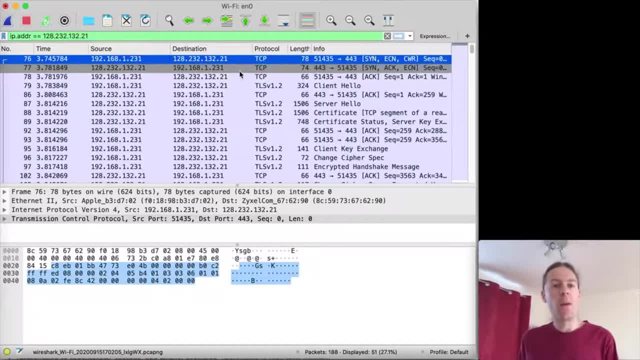 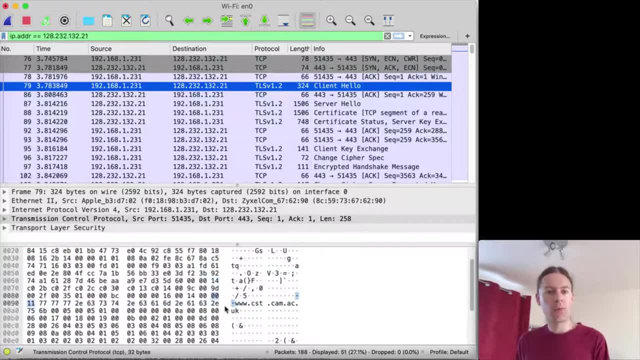 if we can learn a lot more about TCP in the computer networking course. But the bottom line of this is there's a lot of back and forth, You can see, and then here there's some encryption that happens because it's an HTTPS connection. 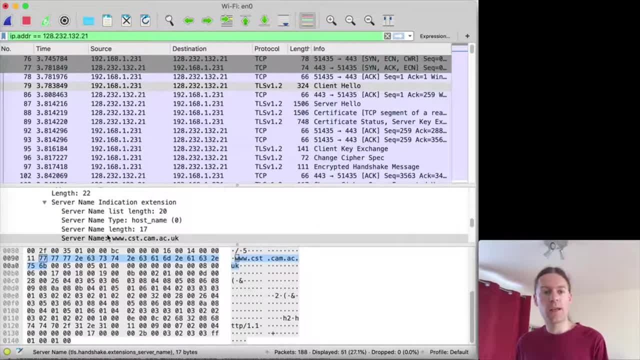 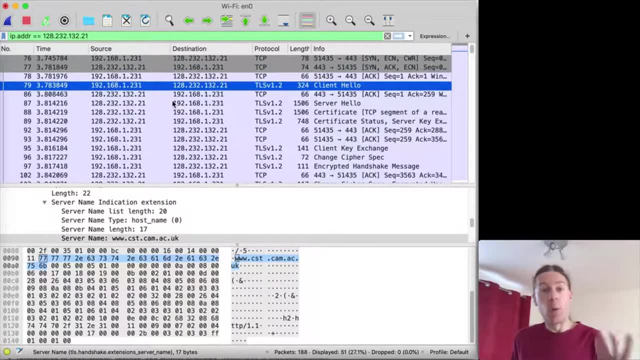 And you can see that here's the name of the website that I'm connecting to, the server name that I'm connecting to, and so on, And so, on the physical level, what's happening here on the network is that we have all of these network packets going back and forth And the 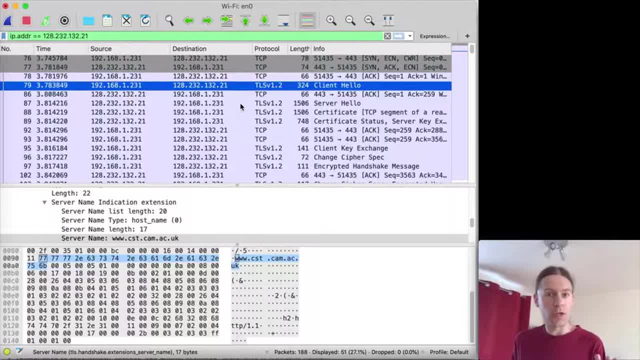 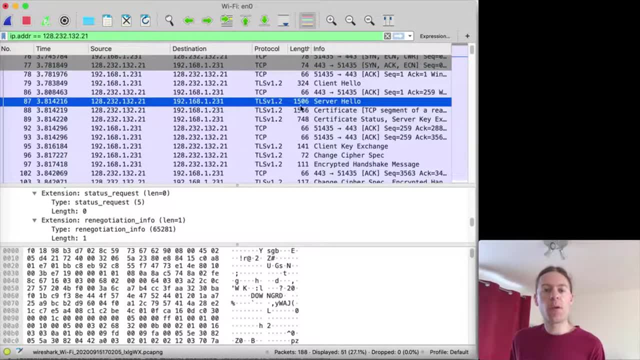 reason that we have lots of packets is that there's a maximum size of each packet And you can see here in this column it has the size, the length in bytes of each packet, And you can see the length- only goes up to about 1,500 bytes. Here another with 1,500 bytes. 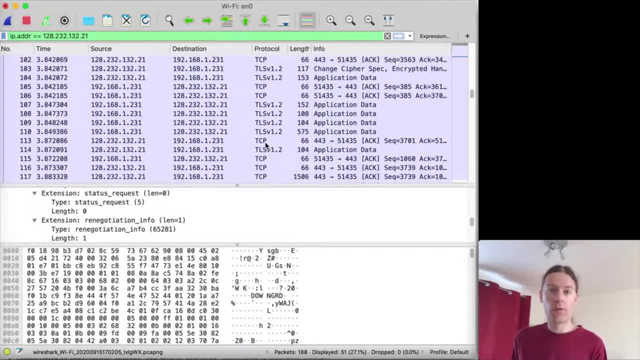 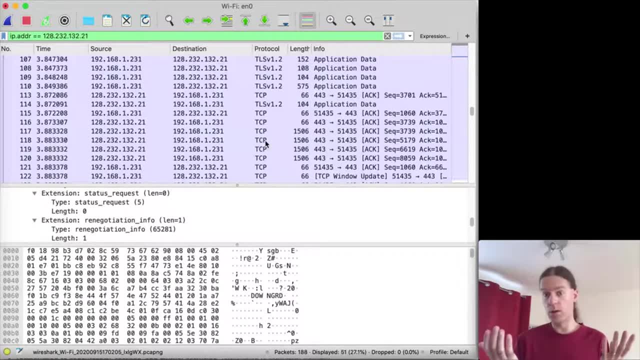 but there are none that are bigger than that, And that's because networks have this maximum size of a packet, And so if you want to send a message that is greater than the size of a single packet, you have to split it up into multiple packets, And this is what we're going. 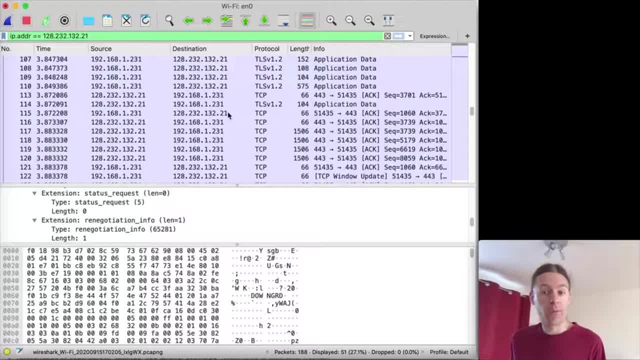 to do next. So now I'm going to throw in a look at this. I'm going to try and see if I can get. And this is exactly what the TCP protocol does. So the HTTP runs on top of TCP. So HTTP has this request message response message paradigm. 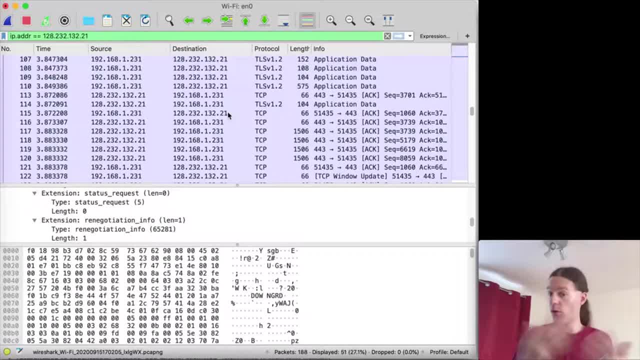 But the request might be bigger than a single network packet And the response is quite likely bigger than a single network packet as well. So then, HTTP uses TCP underneath And TCP breaks down these big messages into small network packets that are small enough that the network can deliver them. 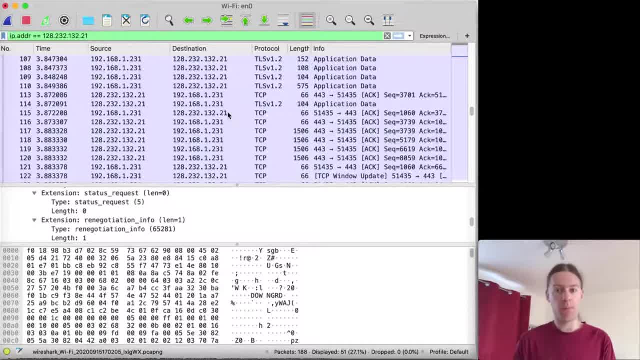 And then on the recipient side, TCP puts all of the network packets back together again to give us one large chunk of bytes, And so this is now like an important thing to keep in mind in distributed systems When we're talking about messages being sent and received. 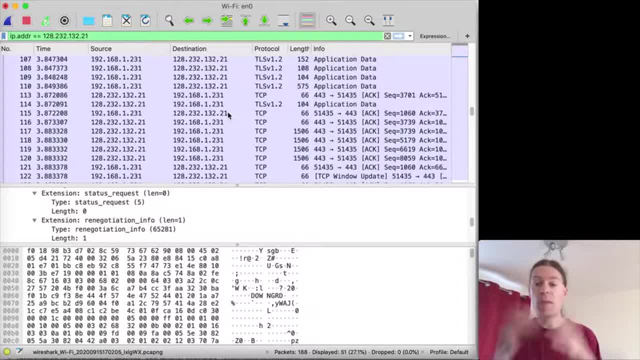 we're not talking about individual packets, Because a message may well be bigger than a single network packet, And so that message then has to be broken down into small network packets. So the message is really a higher level conceptual object that gets sent back and forth between two nodes. 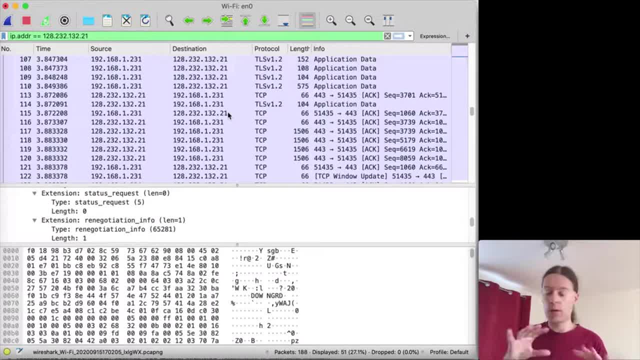 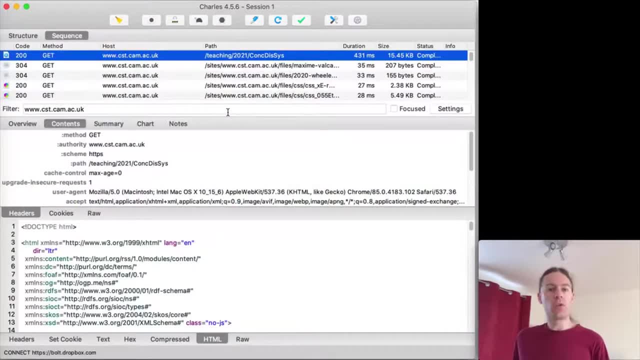 And how exactly this gets broken down on the packet level. that's something that we leave to the computer networking people. So for distributed systems point of view, we can just assume that we have this mechanism through which we can send these requests and these responses here. 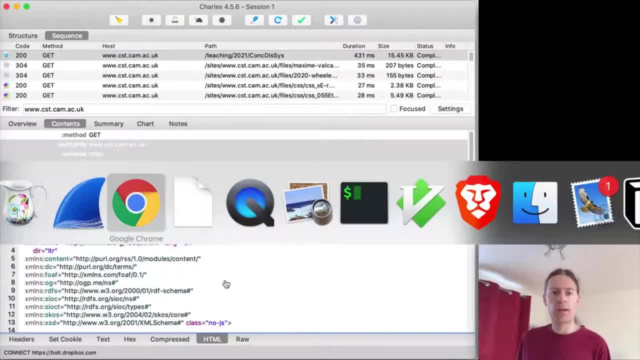 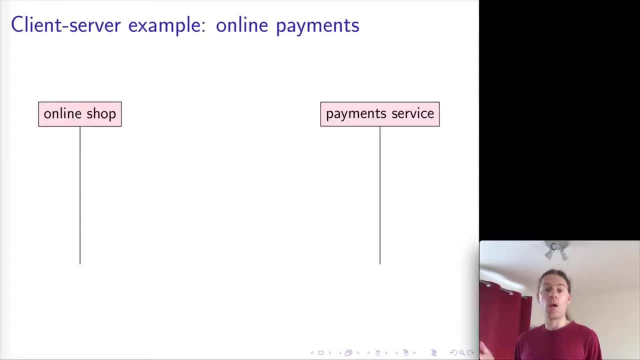 And we don't care too much about the details of how this is actually physically delivered. It's basically represented in terms of network packets. We just assume that we have this communication mechanism. So we saw the web as one example of a distributed system consisting of a client and a server. 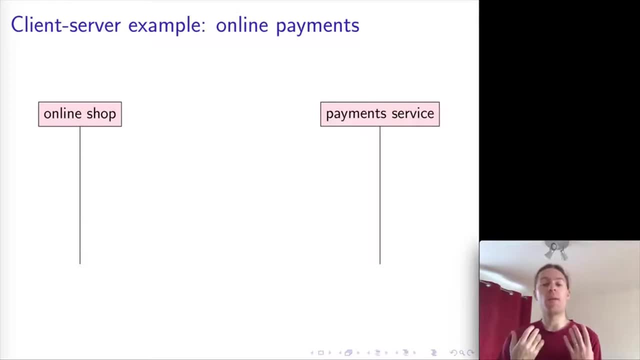 Let's look at another practical example, which is: imagine you're using some online shop to buy something, And so what you want to do is you want to enter your credit card number on this shop after you've chosen the stuff you want to buy. 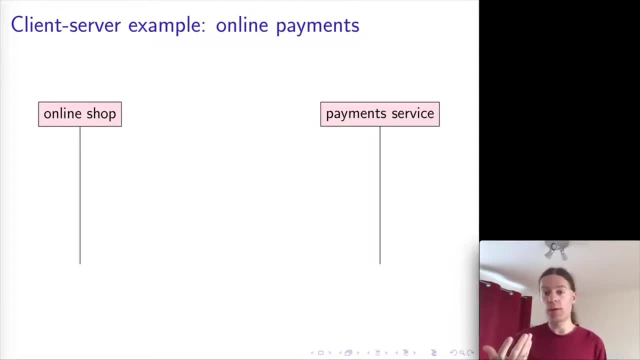 And then you check out And you pay, And then you pay with your credit card and then you get the goods shipped to you. So what happens here is that the payment service that actually processes this credit card payment is usually provided by a different company. 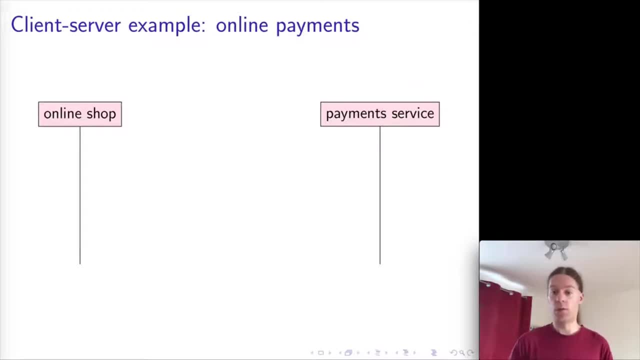 from the company that is running the online shop, because processing credit card payments is a very specialized activity. So it makes sense that there are companies that specialize in just doing credit card payments And another company specializes in actually providing the shop and the goods. 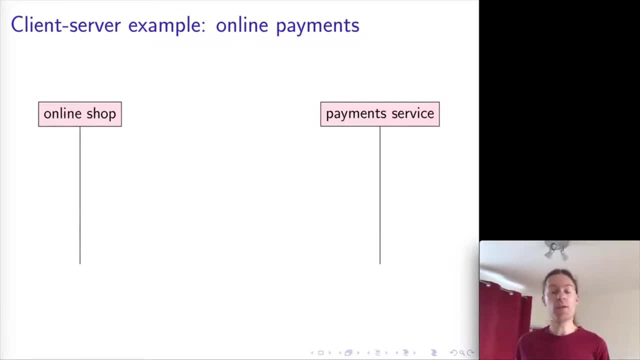 And so what happens when you enter your credit card number on some online shop is that the online shop will send a message to this payment service, which is running on a different node, provided by a different company, And this message will contain the details of your card number. 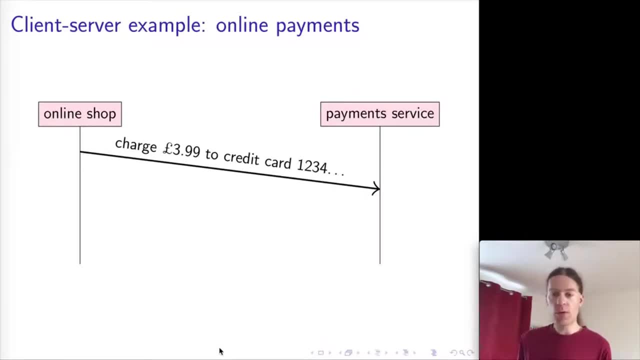 and how much they want to charge to that card and various other information, maybe your billing address and so on. This will get sent to the payment service. The payment service then does a whole lot of complicated stuff. They talk to the card payment network, such as Visa or MasterCard. 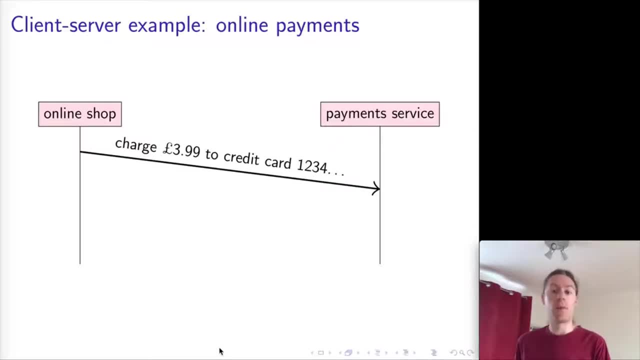 The card payment network then talks to the bank that issued your card, They make sure that you actually have money in your account And then they make sure that the payment can be taken, And if it's successful, then they go through all of this in reverse. 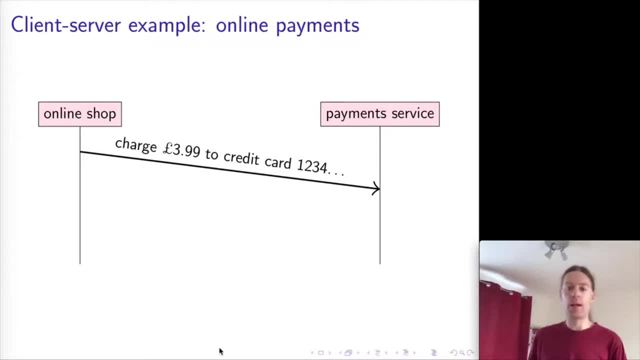 And you know, maybe they do extra checks to like make you enter a password or send you a text message or whatever it might be, And eventually, hopefully, the payment service then sends a message back to the payment service, to the online shop, indicating whether the payment was successful or not. 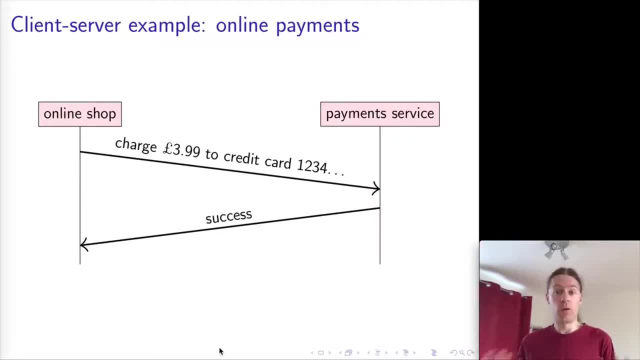 And so this is a very concrete example of a distributed system that is really used like this every single day. Now let's have a look a bit at what the code might look like. So imagine you are one of the programmers working on the side of the online shop. 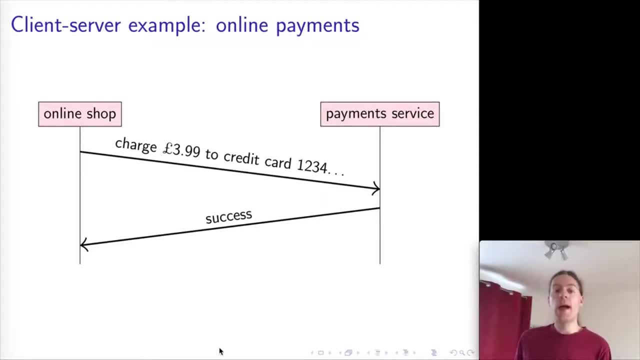 So you're developing the software that runs the online shop and you're writing the code that is supposed to handle the credit card payments and talk to the payment service, And so the code you're going to use is called the credit card payment service. 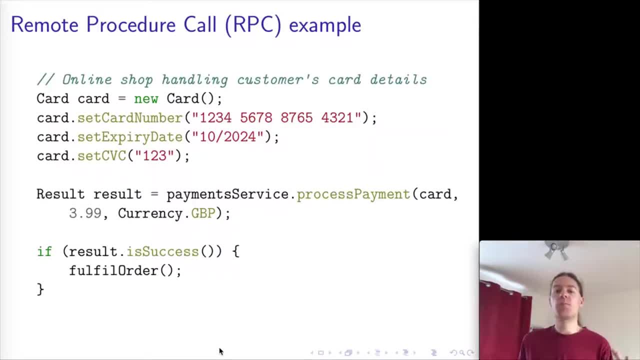 And what you write might look something like this here. So let's assume that there's a card object in your, in your code base, and you can create a new instance of this card object and you can give it the credit card number and the expiry date and the three digits on the back. 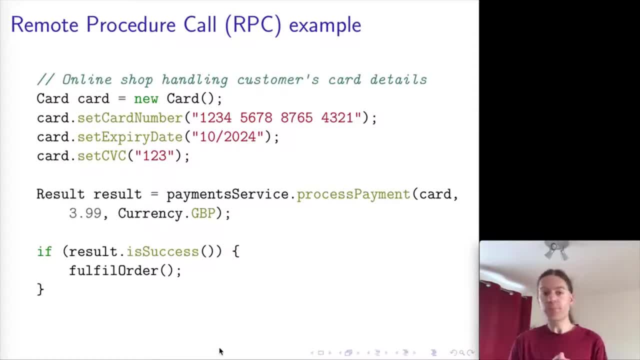 And you can package all of this up as a card object And then you call this function. So you have some object that has this payment service and you call the process payment method on this function and you give it the card that you want to charge and you give it the amount that you want to charge it and 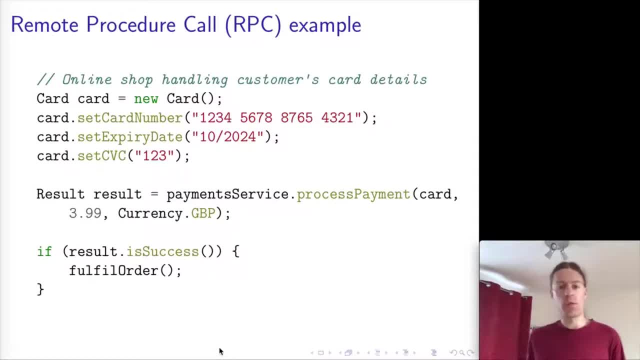 the currency in which you want to charge it And then, depending on whether this is successful or not, you then fulfill the order. So this is quite interesting what is happening here, because, if you think about it, the payment service is running on a different mode, run by a different company. 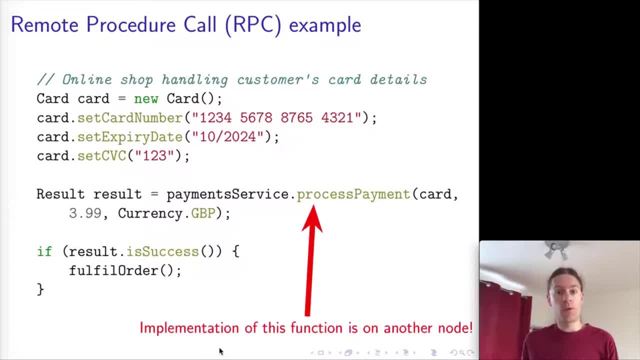 It's not part of the code base of the online shop. So what is happening here is, when you call this process payment function, the implementation of that function is not. it's not within your program. The implementation is somewhere on another node, at the other end of an internet. 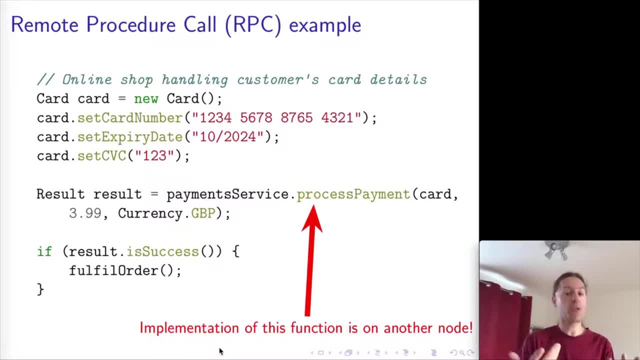 connection And what is actually happening here is what looks like a function call or a method call is actually underneath, being translated into some kind of network communication, And this is called a remote procedure call. Maybe a remote function call would be a better name. 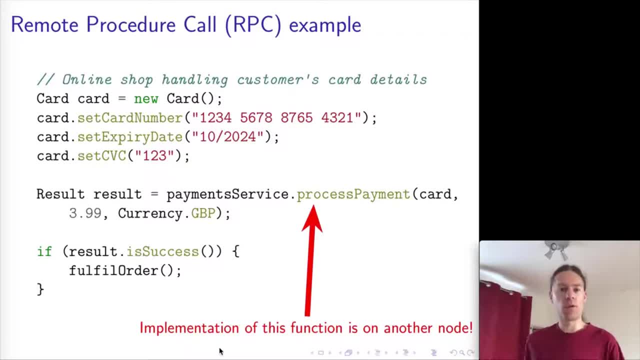 but remote procedure call is what this thing is typically called, And so we're just going to stick with that name. Java calls the same thing: remote method invocation- Again just a different word for essentially the same idea. And so let's have a look at how a RPC 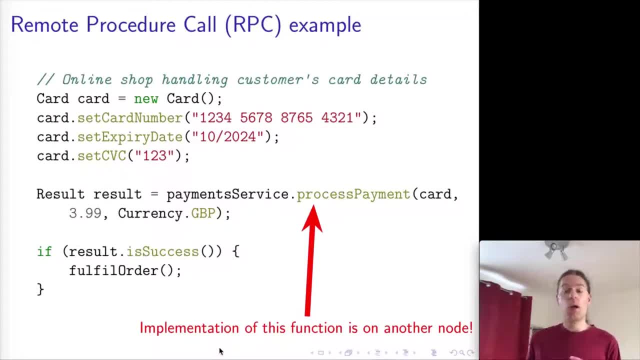 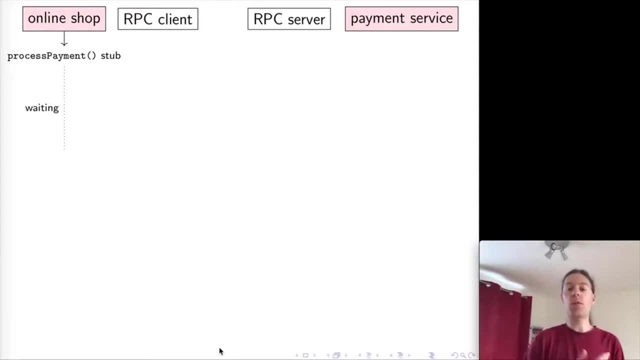 a remote procedure call works, So RPC is typically implemented with something called an RPC framework, or it's called middleware sometimes. This is a piece of software that performs the translation between the function call in your programming language and this message passing over the network. 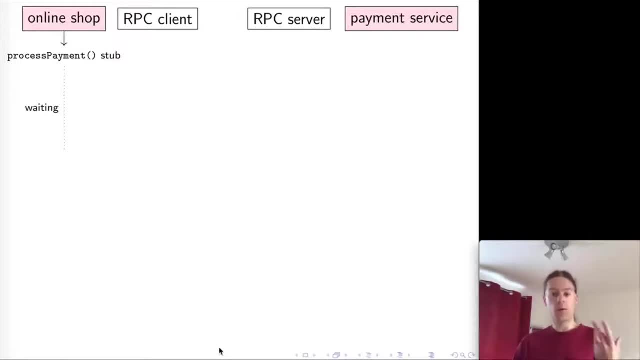 And so when the code of the online shop calls this process- call this process payment function- it can't directly call the function on a different node, because your programming language doesn't support that normally. Instead, the RPC framework provides what is called a stub. So the stub function. it has the same type signature and it looks the same as the function on the remote node that you want to call. So you want to call this process payment function And what we make is this stub function that doesn't actually process the payment. 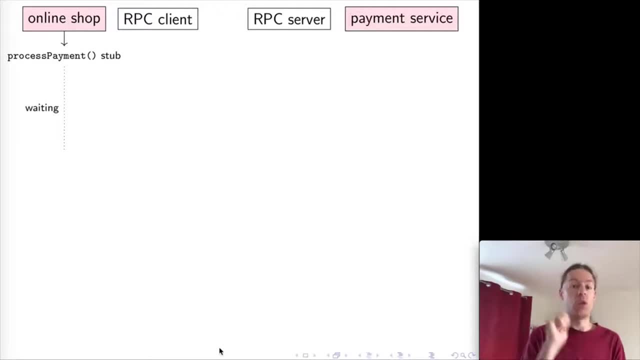 but what it does? it sends a message to the service, which then does process the payment. So the online shop calls into this stub function here and the RPC client needs to take the arguments that were passed to that function and translate them into a message that can be sent over the network. 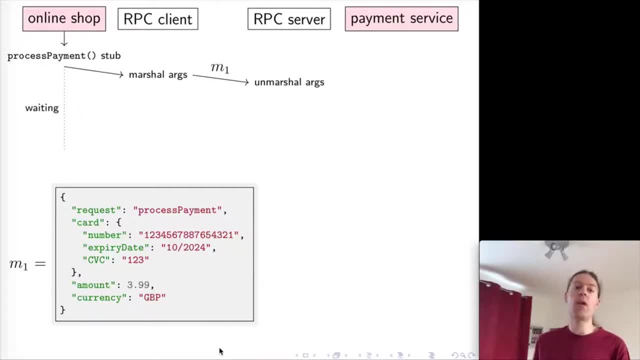 And this translation process from arguments in your programming language to message of the network is called marshalling, And so marshalling- or I call it encoding as well- takes the function arguments and encodes it in some way that can be sent over the network. 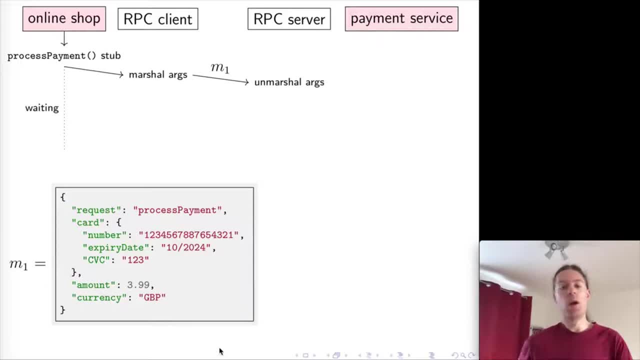 So, for example, it might use JSON or it might use JSON. in this example it uses JSON, which could use some kind of binary format. the format it doesn't really matter, but it becomes then essentially just a sequence of bytes that we can pack into a 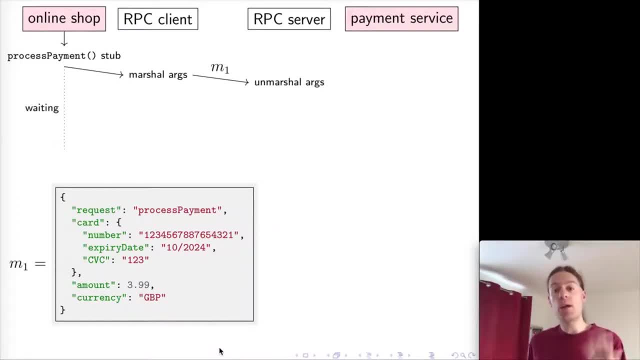 message send over the network And then, on the recipient side, the RPC server is going to receive this message and it's going to translate it back into a function call on the server side. And so here now, this is where the actual implementation of the process- payment function- lives. 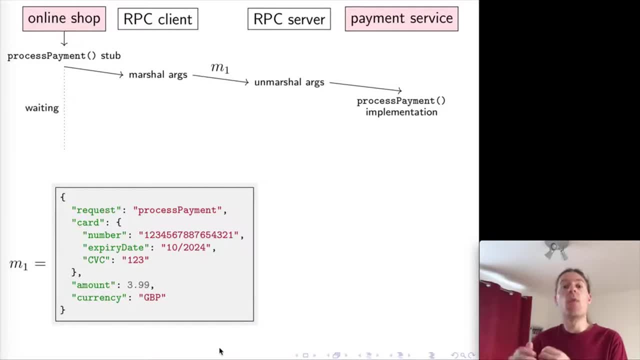 And so here on the RPC server side now this function is going to get called and it's going to do whatever is necessary in order to make this payment happen, And that will probably involve talking to the card network and the bank and updating some databases and doing a whole bunch of extra stuff. 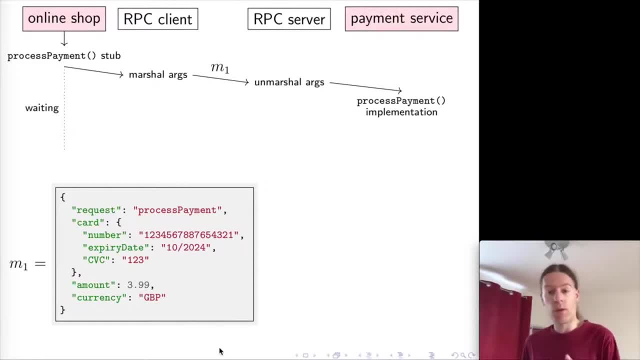 And eventually this function will return and hopefully it will tell us whether the card payment was successful or not. So the return value of this function again needs to be marshalled. We do exactly the same in reverse, So the RPC server marshalls the return value of the function. 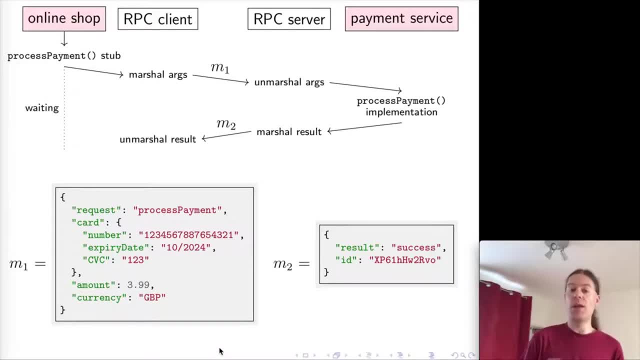 sends it back as a message M2 of the network, the RPC client unmarshalls it and turns it back into the data types of the programming language that you're using, And then eventually the function returns. And so what we've done now is to kind of pretend that this 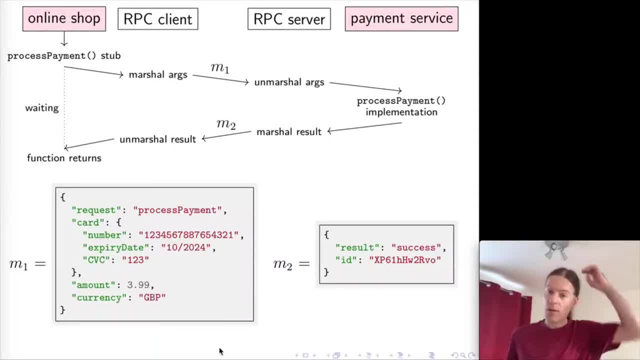 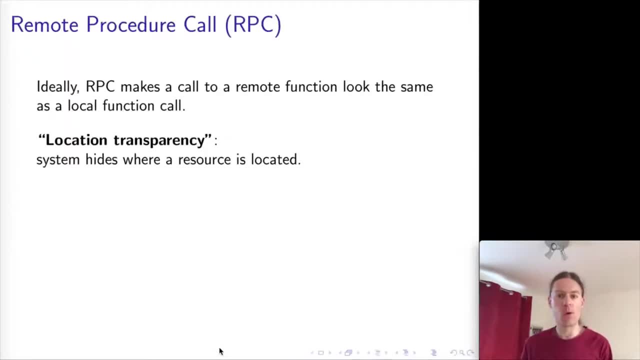 what we're doing is calling a function locally, but actually it's happening. What's happening underneath is this communication via messages to another service. So the ideal that we kind of want here is that the local function call- sorry that the function call to a different service looks just like a local function. 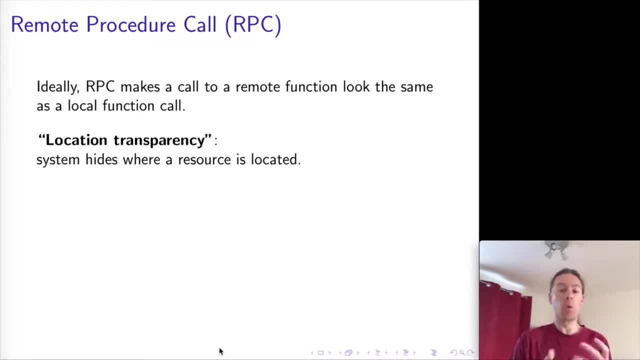 call because we know what functions in our programming language look like. We would quite like the remote RPC to look just like that, And this principle is called location transparency. So the location of where your resource is located, that is, whether the objects that you're calling your process payment on. 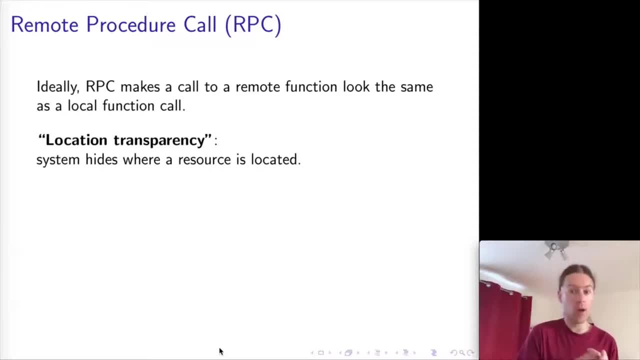 whether that's an object in your own process, in your local address space, or whether that's an object in your local address space or whether it's somewhere on the other end of an internet connection. We want that to be transparent. We want not to be able to tell the difference between the two. 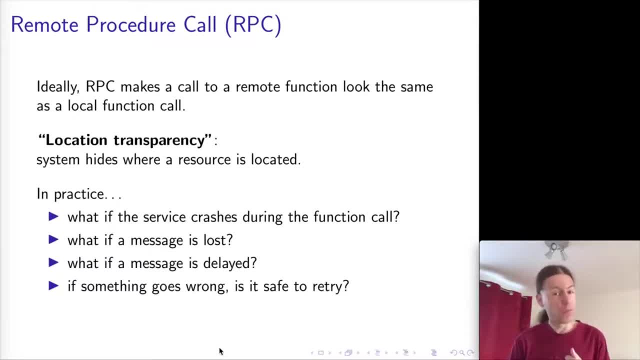 However, actually reality doesn't look that simple because, as I said in the beginning, the trouble with networks is that they can fail. So it can be that you send a message over the network and the message does not arrive. You could send it again, of course. 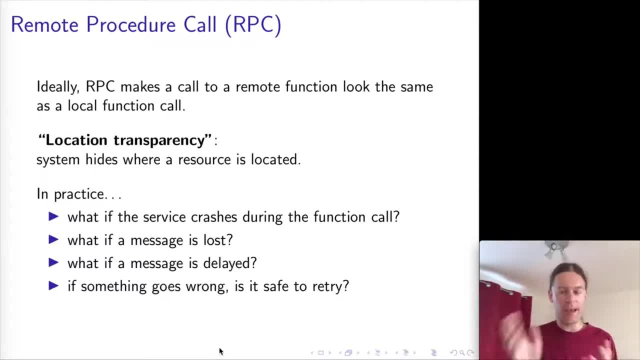 but then are you going to charge the credit card multiple times. We have to be quite careful if we're going to send messages again, right, So messages might be lost. What do we do about retries? Messages also might be delayed, So it might be that the message did actually get through. 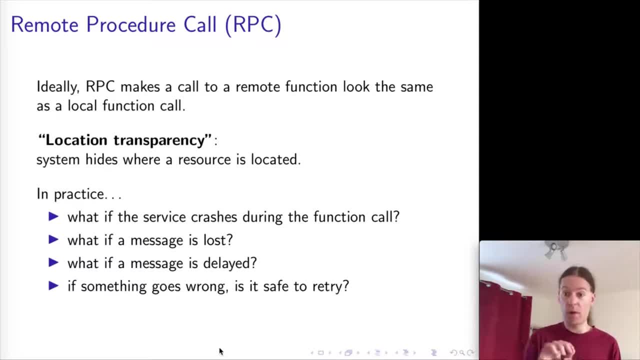 but for some reason there was some networking hiccups somewhere that caused the message to be delayed by a while. That could happen as well. It could also happen that the service that is processing this function crashed in the middle of handling, in the middle of executing our function in the way. in that case, 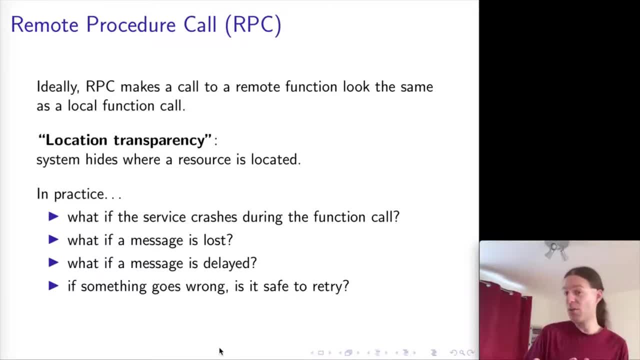 it won't be able to send us back a response, but it might have partially processed our request. I guess we can use. I guess we can use these transactions here: Acid, yes, Okay, but you can see there are a lot of open questions here. 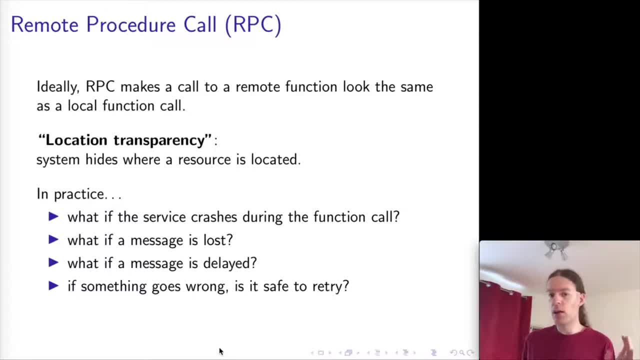 and fundamentally it seems like actually making a function call to a remote resource is something totally different from calling a local function. They're simply two different things. We can make them look somewhat similar, We can give the functions a similar type signature, but calling a remote function has all of these error cases that simply don't. 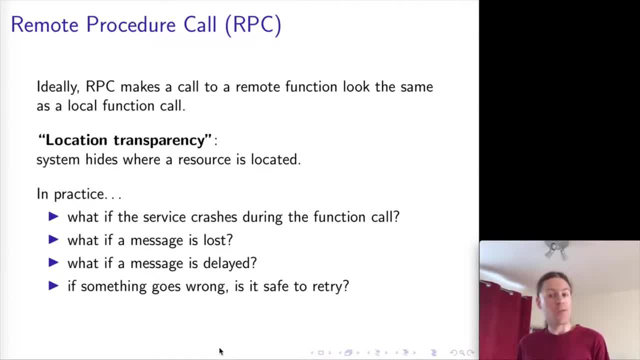 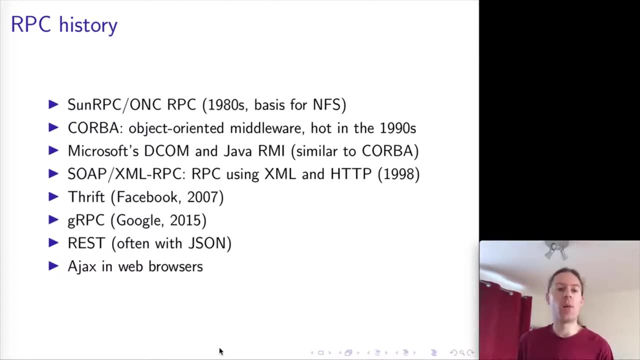 arise in local execution. but that hasn't stopped us. It hasn't stopped people from trying to build RPC frameworks over a long time to try to look like you're calling a local function even though you're calling something on another node. So it started right back in the eighties when the term RPC was first coined. 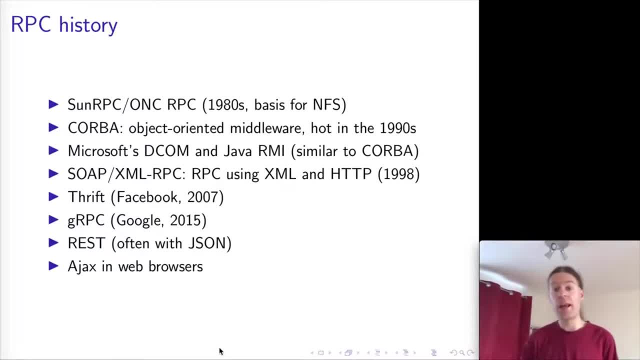 And, like some micro systems, have this thing, and it was used to build NFS, the network file system, of which we'll see more later in the course. And then in the 1990s this was a very hot topic. People then talked about object oriented middleware. 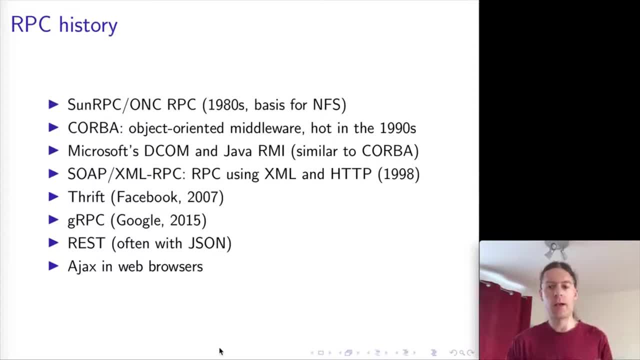 and there was this thing called core bar, which was like really hot. nowadays Nobody uses that anymore. Then there were a whole bunch of competing technologies, like Java's remote method. Invocation is kind of a similar type to core bar. We won't go into the details of all of these. 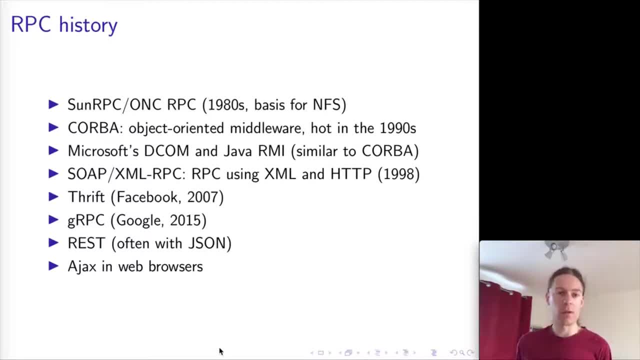 I'm just mentioning the names here because you might encounter them in your careers, And so it's good to at least have seen them before. And you know, just as as recently as 2015,, Google brought out another RPC framework. 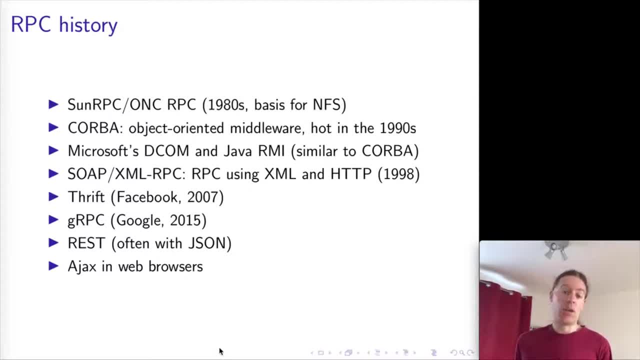 It's called GRPC for Google's RPC, And you know it's it's. it's fine. if you want to do RPC, why not? You can use it. You can do something else, It doesn't really matter. 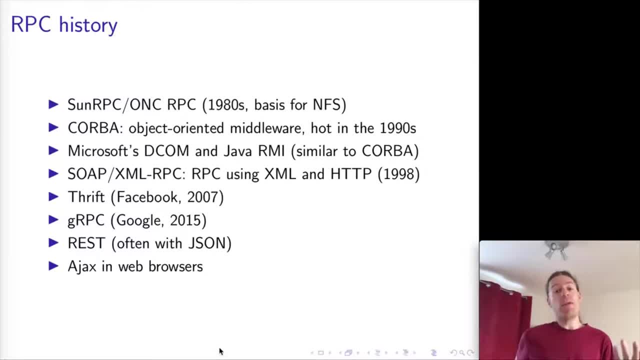 What is common, very common nowadays, is actually something called REST. This is stands for representational state transfer- a bit of a mouthful, but it's really a set of principles for how to use HTTP. People who are keen enthusiasts of RESTs don't like to think of REST as a 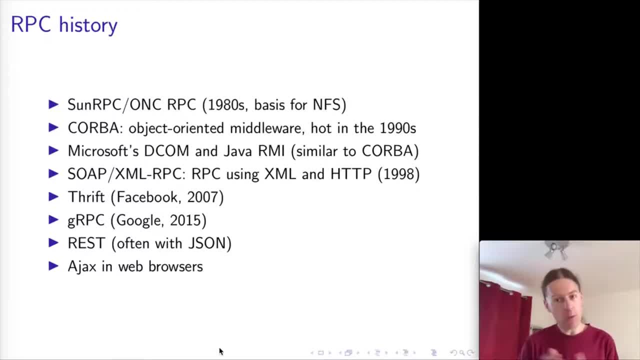 kind of a tool that can be used in a lot of different ways. And you know they like to think of REST as RPC. They like to think of REST and RPC as two different philosophies, but essentially they're the same kind of thing. 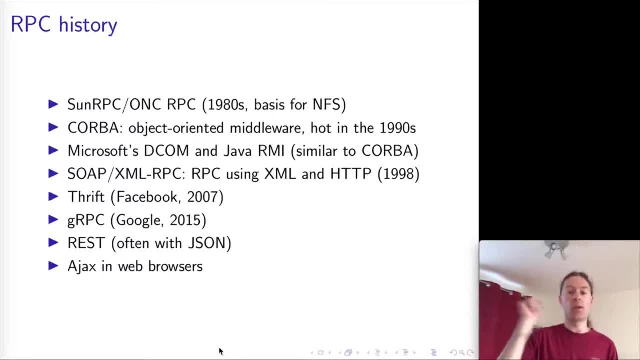 So essentially they're still about invoking code and causing something to happen in a remote service by making some network requests to it and packaging the whole thing up in some reasonably nice way in your programming language. So one reason why this RESTful approach of building RPC was 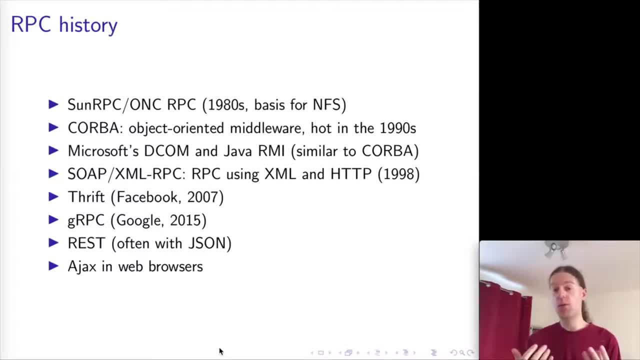 became so popular was that web browsers support making HTTP requests. So you can have some JavaScript code running within a web browser and this code can make HTTP requests to a server and it can construct whatever data it wants to send in that request send out and it can receive the response back from the server. 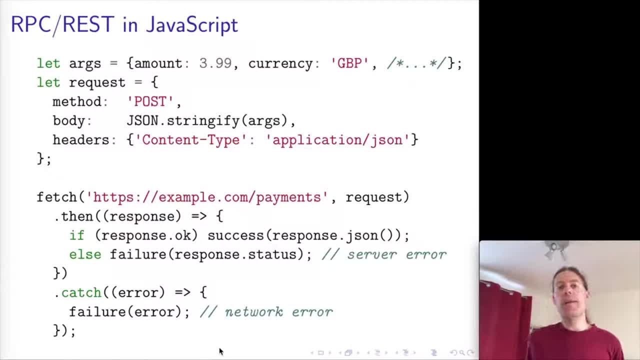 This technique is sometimes also called AJAX and it looks something like this. So if I want to implement the this credit card payment example in JavaScript, I might first of all create this object args containing the arguments to the function. call for the RPC. 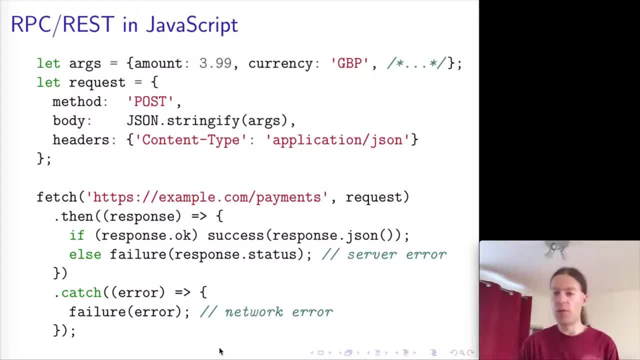 So that'll contain the amount and the currency and the card number and the billing address and so on. And then I construct this request object which says which HTTP method I want to use. So post is the method that's used for submitting forms. 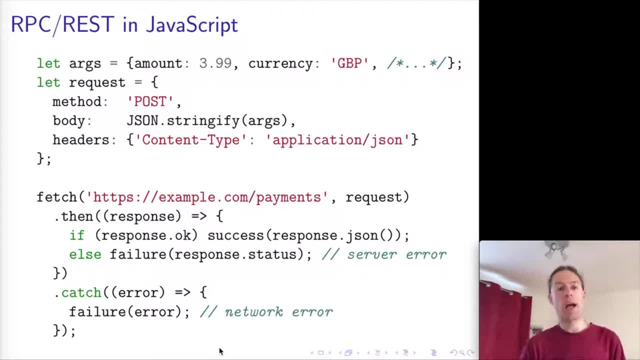 Usually when you're changing some state on the server. I'm now going to take the arguments and turn them into a JSON string using the JSONstringify function, And I can tell the server that the JSON is the type of data that I'm providing. 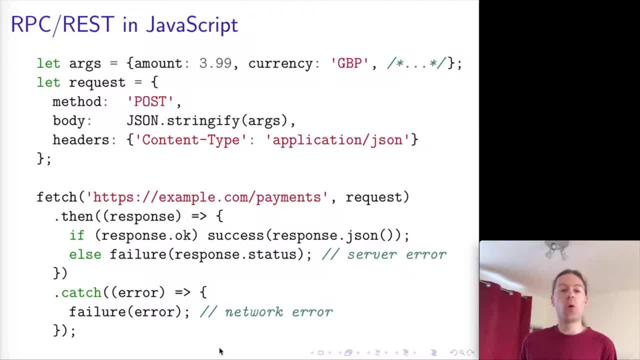 So I'm providing the file type, essentially, And then I can call this URL, which means actually sending an HTTP request to this URL: examplecom slash payments with all of the details specified above. And then we have these two, these two handlers down here. 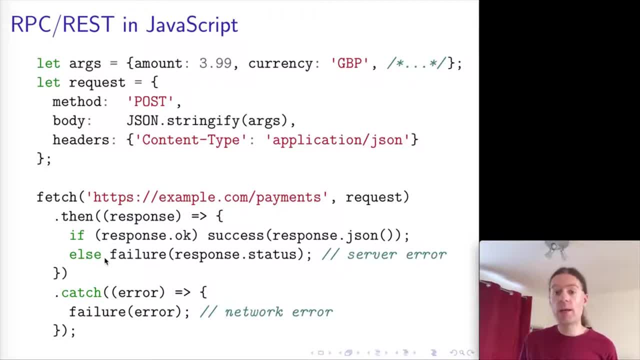 So the then case has a function call back here, which gets called. if that network requests receive resulted in a success, then it's called Successful response. So if we got a response back from the server, then this variable response here becomes that response. 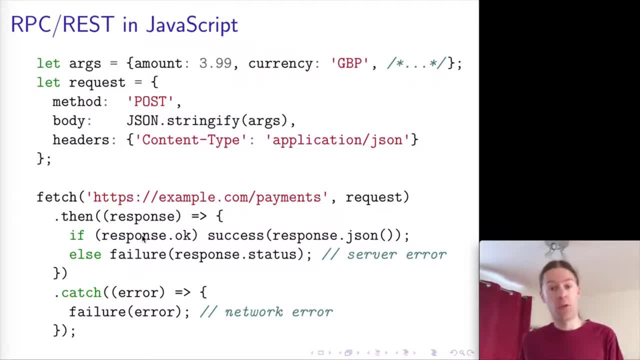 And then we execute this code here. So we can now look at the response that we got from the server and see whether the status code that it replies with indicates success or not. So if it indicates success, that means the response is probably Jason again. 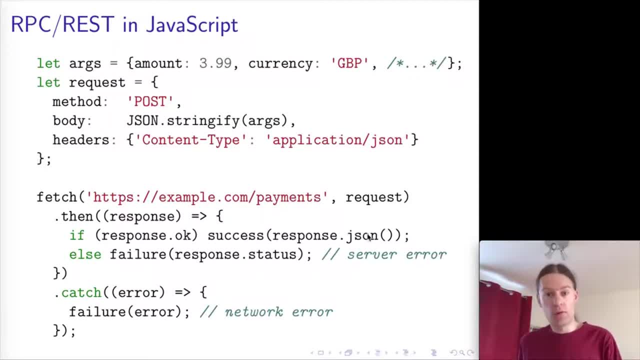 So we can unmarshall that back into objects in JavaScript by calling this Jason function and then call the success function to indicate that we got a successful status back from the server. Otherwise, if the status code was not success, then we could call a failure function with the status code. 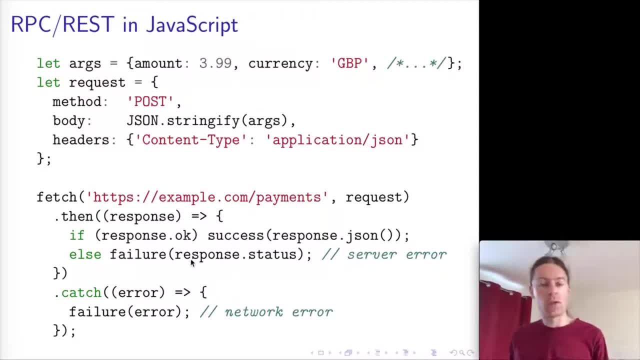 For example. of course we can do more detailed error handling, but that's just the general idea. So this is the case where we got a response back from the server. Now, of course, messages can be lost, And so it might be that we don't get a response back from the server. 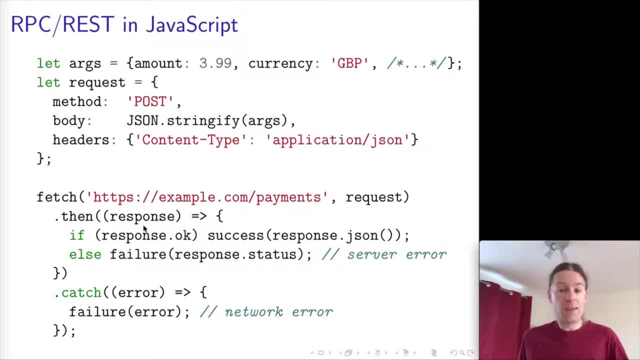 And in this case, for example, the request might just wait for 30 seconds, And if it doesn't receive anything within 30 seconds, it's going to say timeout, we give up. the message might've got through, or might not. 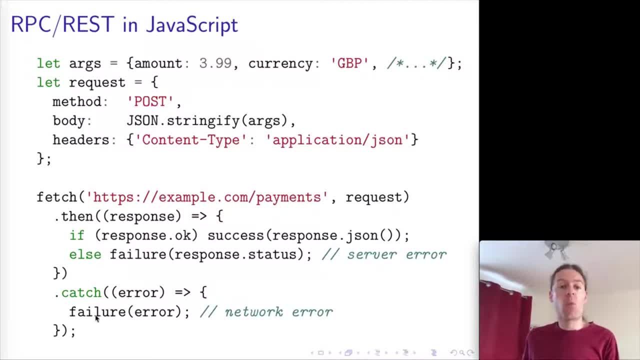 We don't really know, but we're going to give you a network error, And that's what happens here. So in this catch case, here we have another callback function which gets called if the network request did not result in a response from. 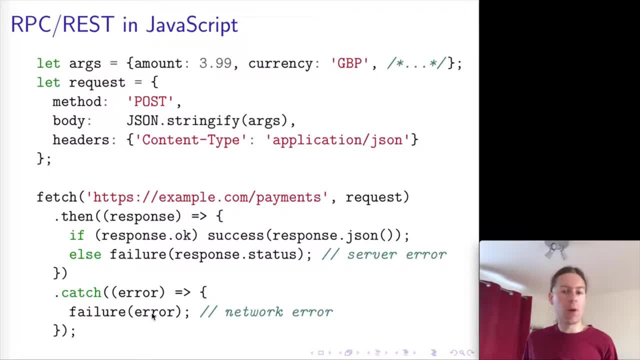 the server, And in that case I'm just going to call that failure function again and pass the error in. in practice, you would probably want to show the user message and explain that something went wrong, Anyway. So this is the basics of 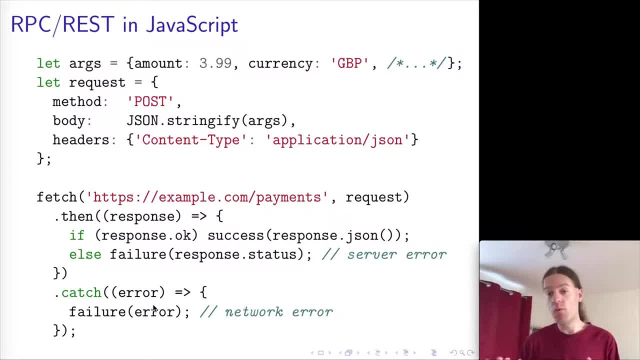 of how you would do RPC And this is how you would use a REST API over HTTP in JavaScript, And this pattern has become very popular, as I said, for web browsers, So in most websites now we'll use this kind of technique to. 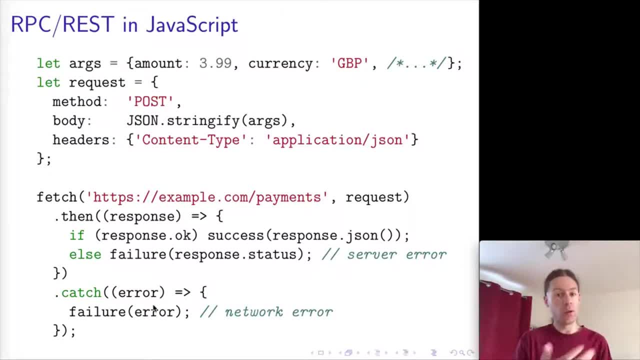 make HTTP requests to the server without reloading the whole page, And so it's just JavaScript running in your web browser that acts like a client side program which is performing these network requests, But the very similar techniques are also used for server to server communication. 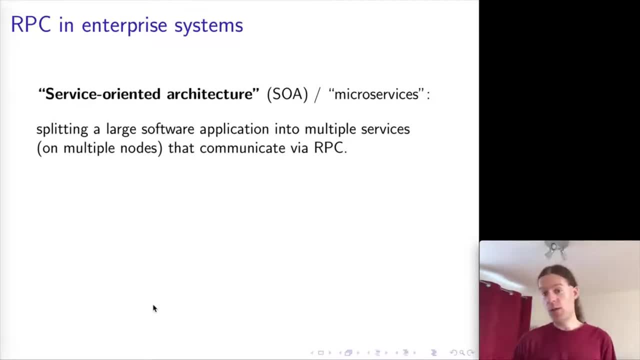 And so this technique is particularly popular in large companies. So in large enterprises you have these huge software systems which are running all of the operations of the company, And these software systems are far too big and far too complex to have just like a single program running on one computer. 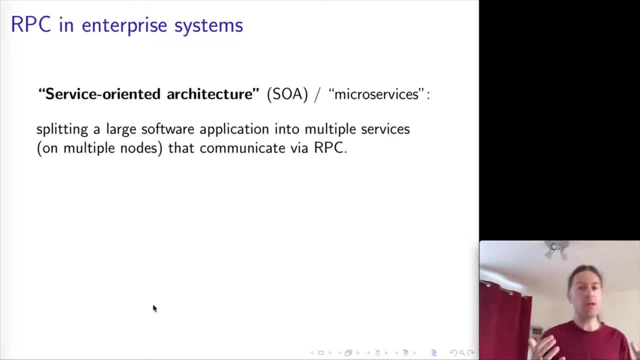 So, simply because of the sheer complexity, sometimes also because they're large, large amounts of data that these things have to process, They are distributed systems, So you have multiple nodes running on multiple computers which are all providing part of the infrastructure of this large 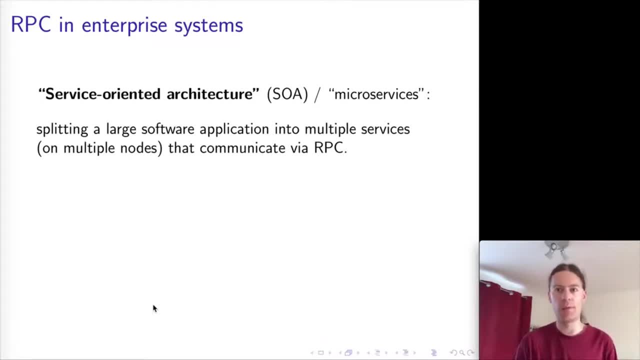 organization call it- might be a bank or a retailer or whatever- And this large bunch of software is broken up into what are called services and approach, where you break down a large piece of software into services, called a service oriented architecture or some people. now a more modern term is to call it microservices. 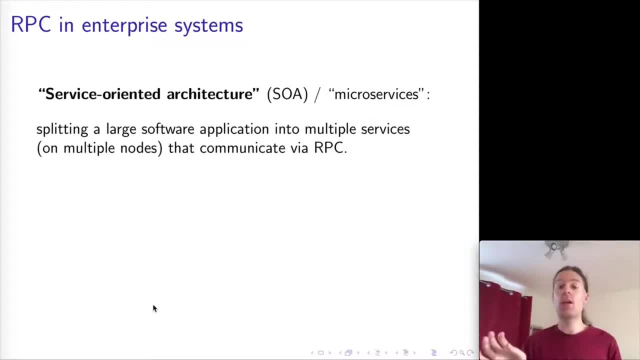 And this is just having programs running on different nodes which communicate via RPC, And so RPC here is the key mechanism that allows these, these bits of software, to interact with each other, And so I'll tell you a little bit more about RPC in these. 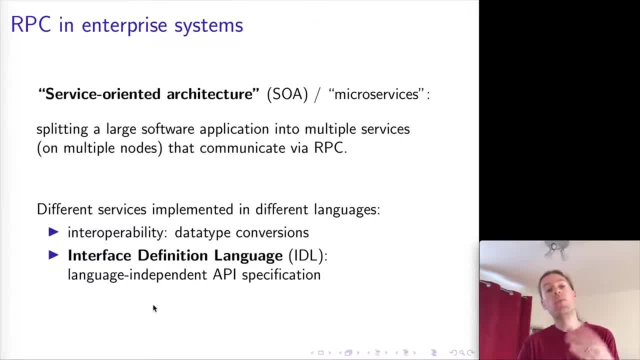 kinds of settings. So we've seen it in the web browser, but here in in in service oriented architecture, you're normally talking about services that are running within a data center, And so there might be running on multiple different servers in the same 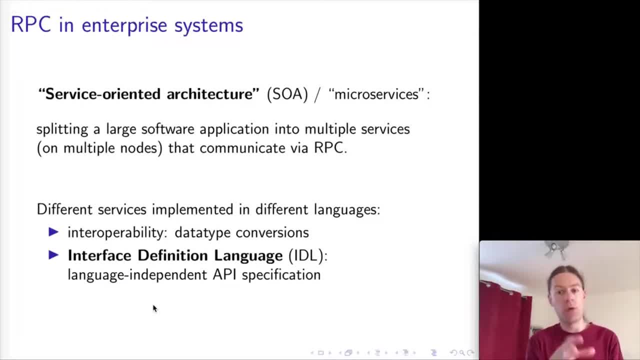 data center, but generally they're all services talking over the data center network. So these are not services running on your end user device like your phone or your laptop, but they are data center side services. but we can use RPC equally well. 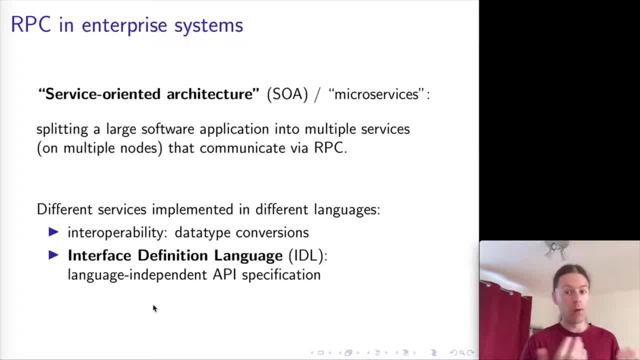 regardless of whether it's like end user devices talking to a server or servers talking to other servers. What you do get in these large scale enterprise systems is that they use a whole bunch of different programming languages because they have some old systems, You know. 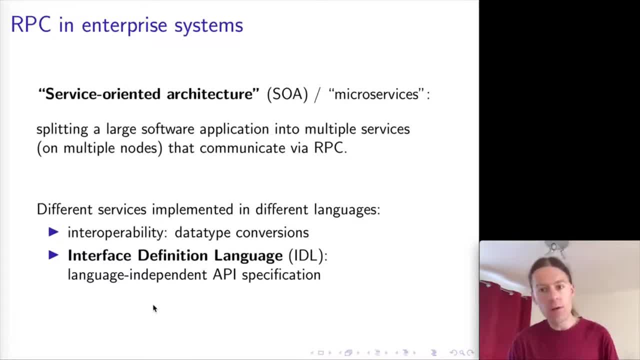 they might have some old systems written in COBOL, Then they'll have some slightly newer systems written in C++, Then they'll have a bit newer systems written in Java, And then they'll have the latest systems in whatever is the latest, most fashionable programming language right now. 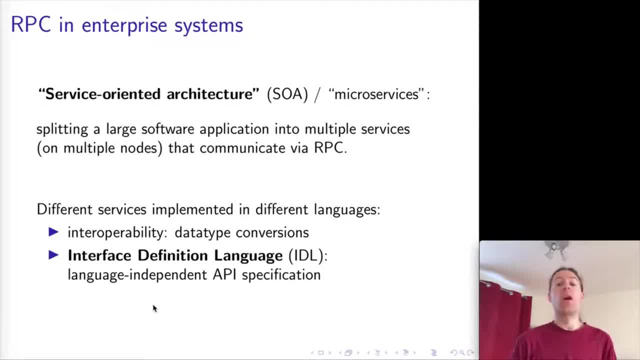 And these systems need to talk to each other, And so RPC can actually provide a mechanism for interoperability between these systems written in different programming languages. Now, this does mean that you know if the function caller and the code being called if they're written in different programming languages. 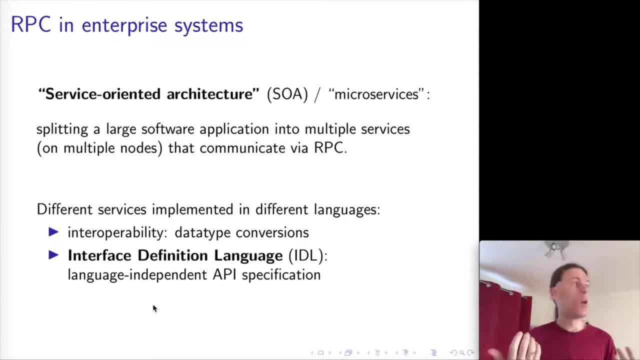 you now have to make sure that the type signatures will match up somehow, And so you have to perform some data type conversion, And so this is often implemented using something called an interface definition language on IDL, and which is essentially a language for specifying the type signature. 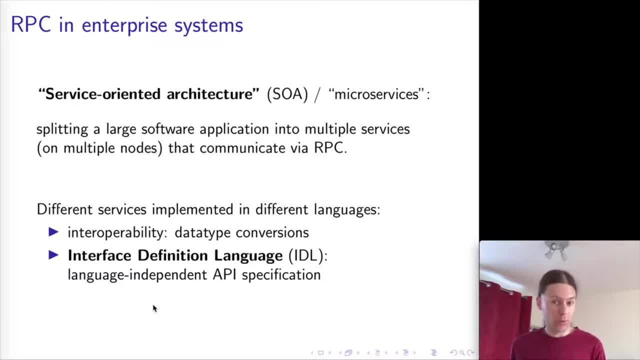 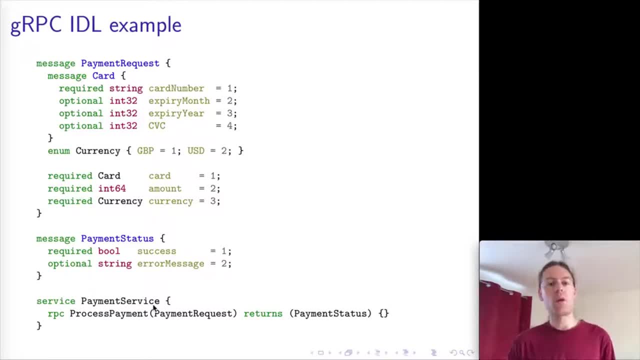 or function calls in a way that is not specific to any one programming language. So here's one example of what an IDL looks like. This example is taken from gRPC, the Google RPC framework. It uses an IDL called protocol buffers. 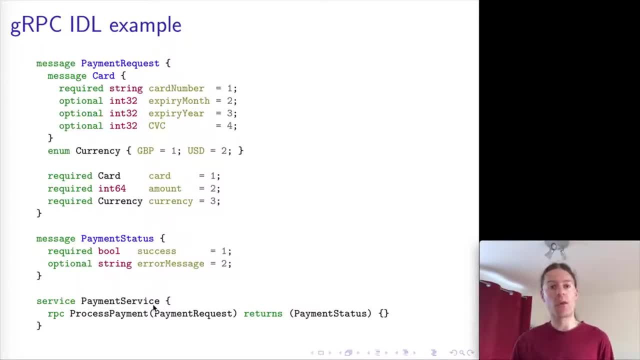 The details are not important. I just want to give you a bit of a flavor for what this looks like, And so what you have here is you can have a specification of a message type, And so we can have a payment request message and a payment status message. 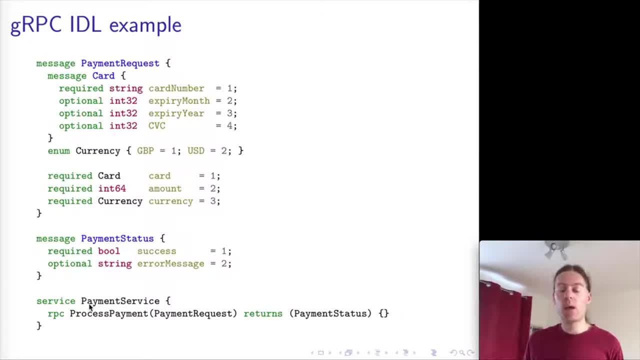 Those are two different messages type. And then down here we have the specification of a service. So the payment service has an RPC, offers an RPC function call which is called process payment. It takes as argument a payment request and it returns as its return value of payment status. 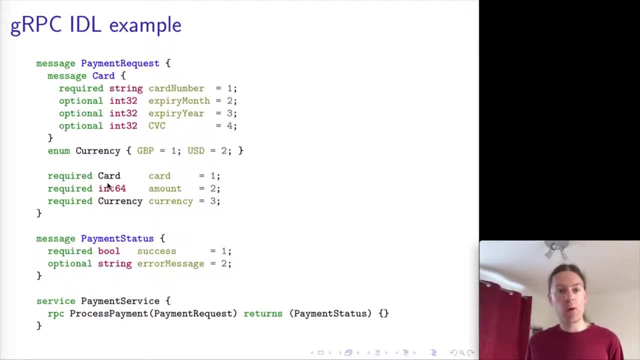 And then up here we can say: what does a payment request consist of? Well, a payment request consists of a card and amount and the currency, and the card in turn consists of a card number and expiry dates and the three digits on the back. 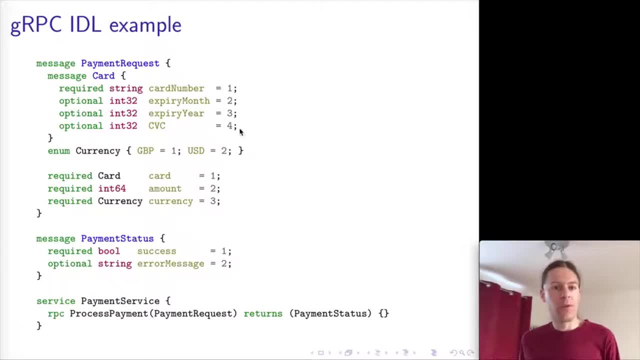 And the currency might be an enum indicating the possible values. ignore those one, two, three, four values here. The details of that are not important for the purposes of this course, But you can see here I'm using data types like in 32 to indicate this is a 32 bits signed integer. 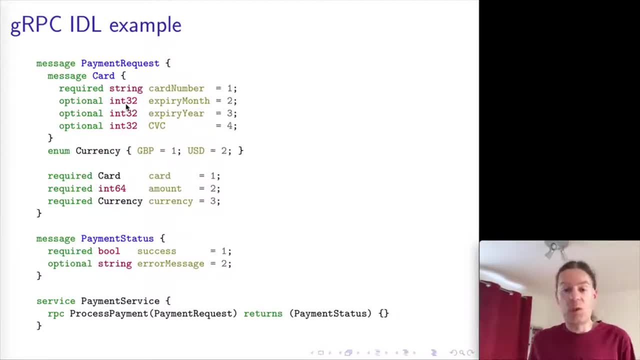 And you can. that is like a fairly generic data type that you would expect most programming languages to support that kind of thing. Likewise here, string data type is very common, An enum, you know. if the language doesn't support enums, you could translate it into just an integer or something like that. 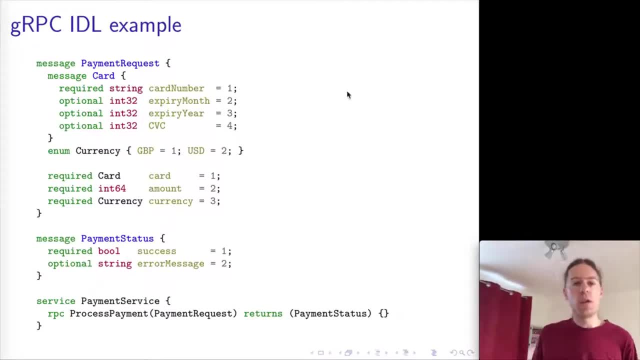 Boolean, again, is a common data type. So you can argue, you know, should the card number be a string or should it be an integer, with sufficient digits that you can have 16 digits. whatever we can argue about that, But you get the general principle. 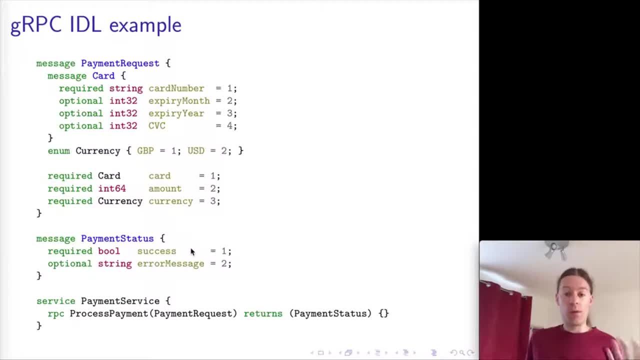 This is a language independent specification of what the RPC can look like And the RPC framework can take this IDL can take the specification and generate code in all of the, in all of your favorite programming languages, And so that's way, that way. 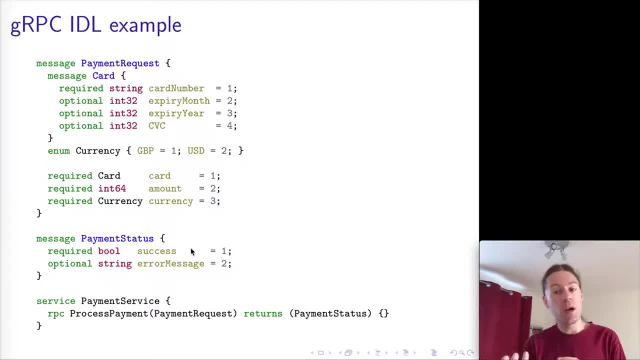 then it can generate the stubs for both the RPC client and the RPC server that make it easy to write code that performs the RPC on both the caller side and the side of the service that's being called. So that's, that's RPC. 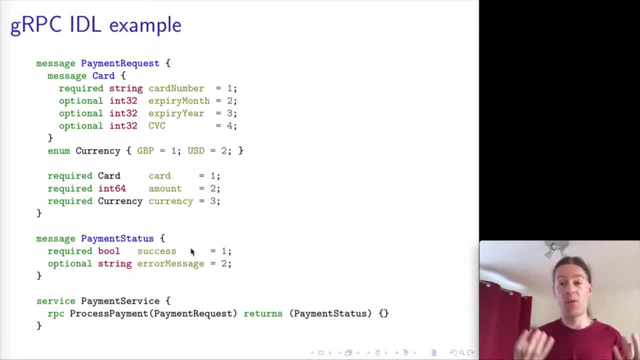 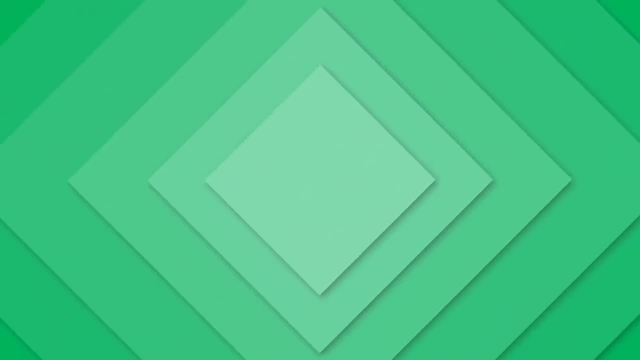 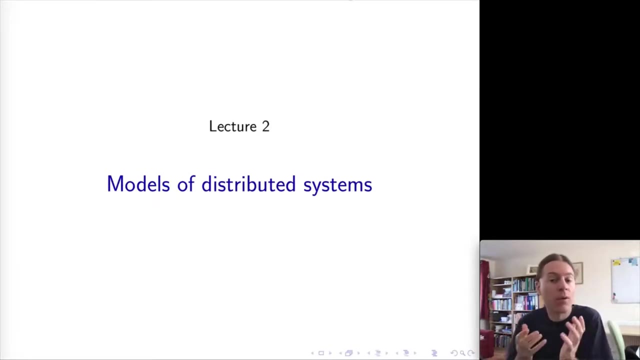 Next time we will talk about a bit more about the fundamental issues of actually making reliable distributed systems. Hello everybody, Welcome back. in the last lecture we introduced distributed systems by looking at some concrete examples such as the web and RPC, which are examples of client server systems. 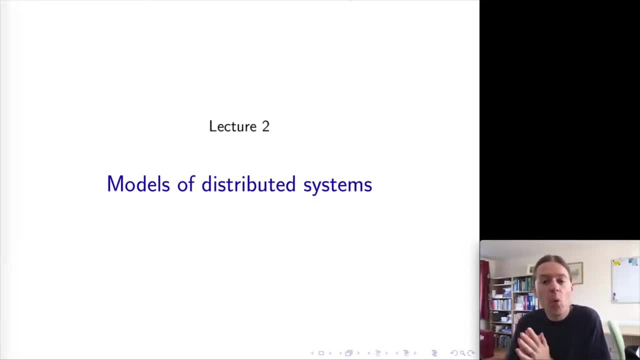 In this lecture we're going to move things to a little bit more abstract and a little more general model And we're going to talk about system models for distributed systems, which are descriptions of the assumptions that we make when we're designing, you know. 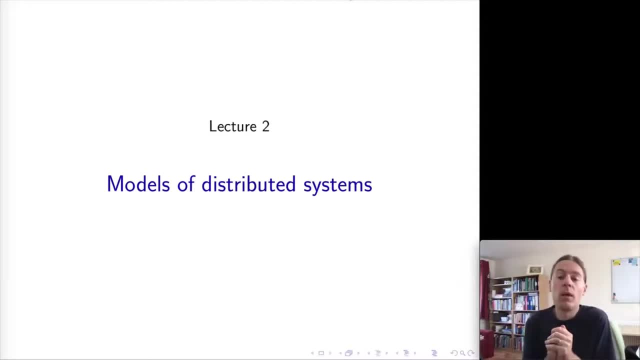 designing an algorithm to run in a distributed systems. So a system model is very important because, as we discussed, things can go wrong in the distributed systems- Nodes can crash, networks can fail and so on, And we have to be precise about what failures we are assuming are possible and what failures we are assuming are not possible. 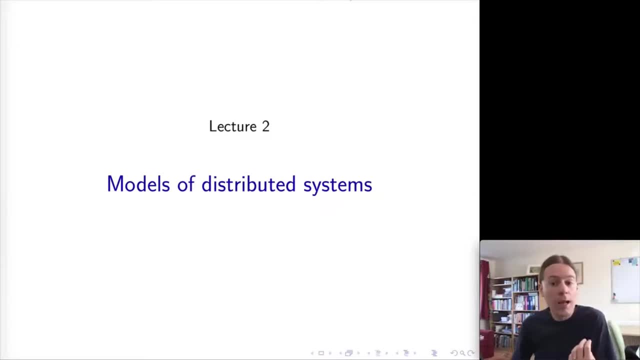 So we're going to start this by looking at two classic thought experiments from distributed systems: the two generals problem and the RPC And the Byzantine generals problem, And we're going to start now with the two generals problem. So this is. 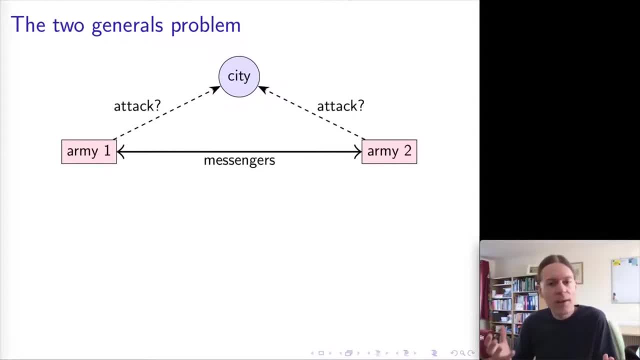 it's kind of like a military analogy, So I'm sorry about that. I'm not really a big fan of that, but it's widely known as the two generals problem, So I'm just going to stick with the convention here, And so the setting of this thought experiment is that we have two armies. 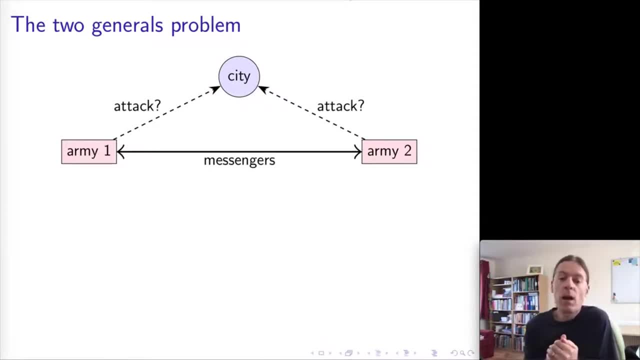 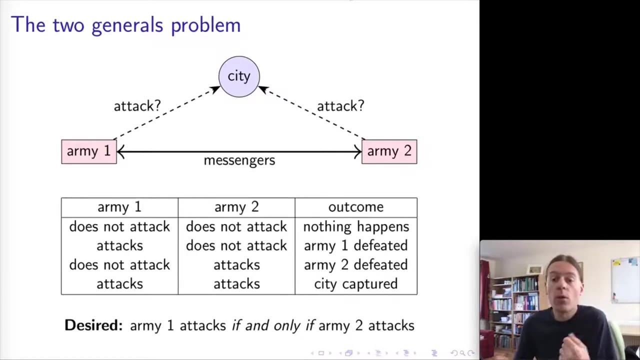 Each army is controlled by one general, and these armies are wanting to attack and capture a city. Now, the city is well defended, and so if only one of the armies attacks at one time, that army will get defeated. And so it's very important that if the two generals are going to attack, they attack at the same time, because then if both armies attack at the same time, they know that they are going to win. 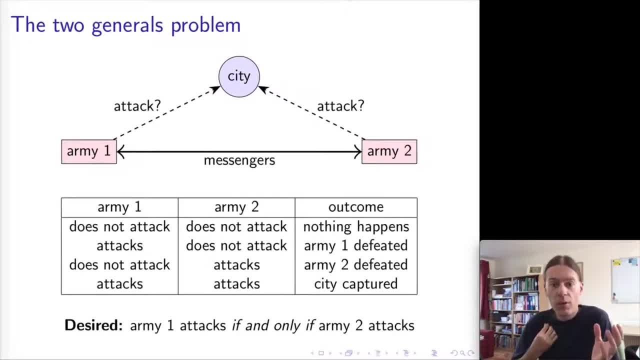 So you can see from this truth table here, what happens is okay, it's, it's all right if neither of the two armies attacks, but if only one of the two armies attacks, then it's not going to happen. It's not going to happen, It's not going to happen. 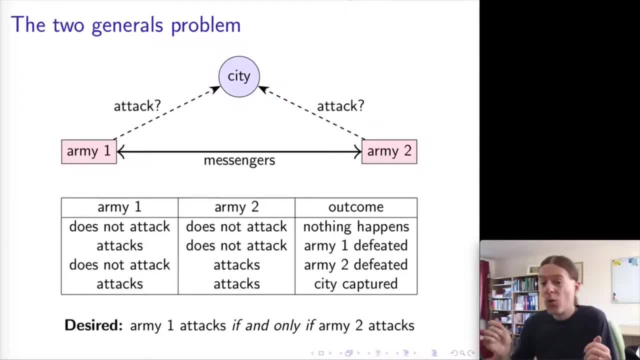 It's, it's all going to go terribly wrong. So what we really want is that one army attacks if, and only if, the other army attacks, so both armies attack together. Now what makes this difficult is that the two generals can't just talk to each other and agree on their plan of when to attack, but they can only communicate via messengers. 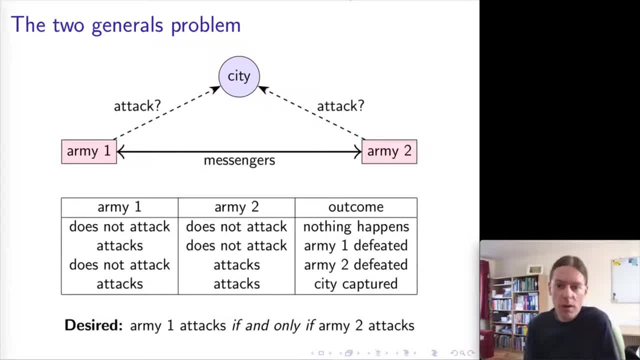 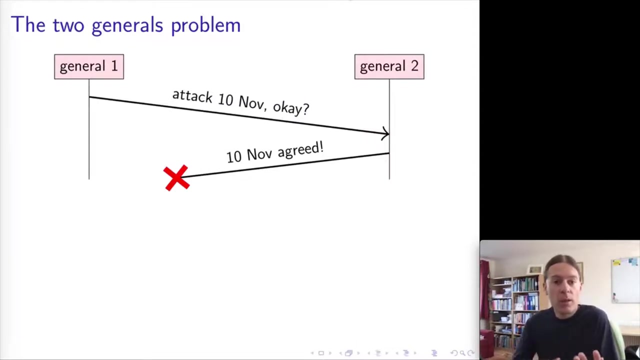 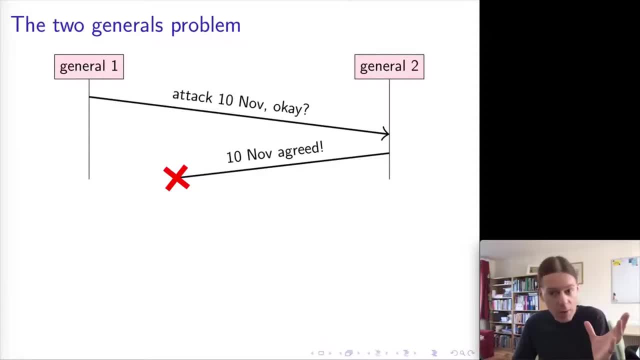 And so the problem here is now this. so imagine, for example, general one has decided to attack on the 10th of November, saying: we're going to attack on the 10th of November, Are you okay with that? And General 2: 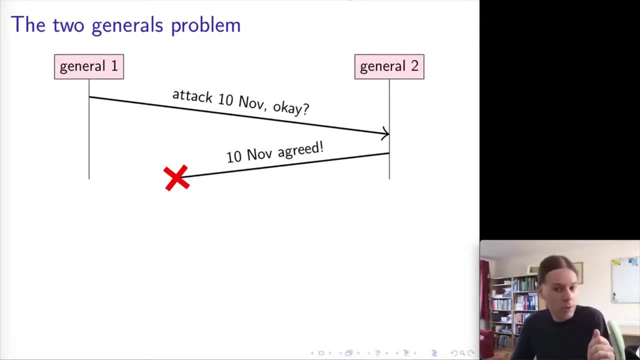 receives the message and says, yes, I'm on board, We're going to attack together on the 10th of November, sends that response back. But unfortunately the response message is captured. So the initial message, the request, gets through, but the response is lost. And so now General 1. 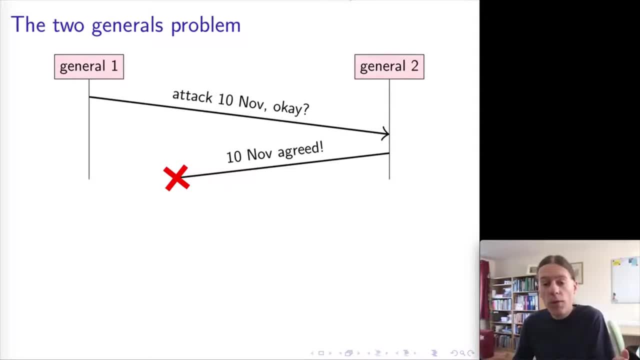 does not receive a response. Now, this is one scenario of what could happen. Here's another scenario of what could happen. It could also happen that General 1 sends the message attack on the 10th of November to General 2, but that initial message is lost and never gets through. 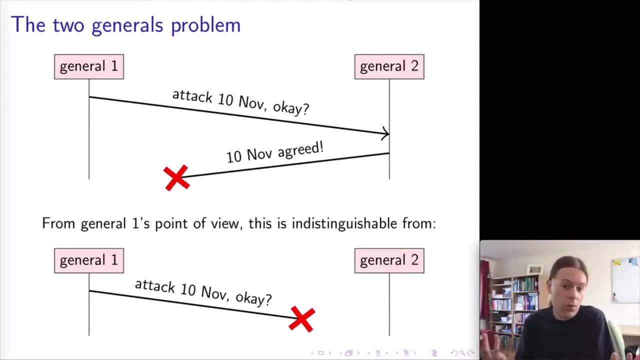 to General 2.. And now General 2 doesn't receive any message, so he's not going to respond either, And the end result is also that General 1 does not receive a response. So in both of these two cases, the only thing that General 1 observes is no response, But General 1,. 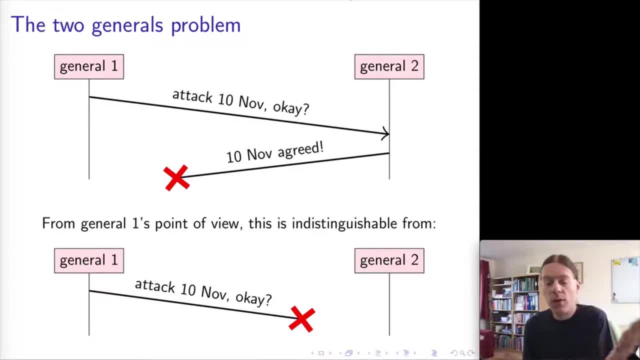 does not know whether there's no response because the initial message didn't get through or whether the response was lost. But there's a big difference between the two of these because, from General 2's point of view, in the first case General 2 has agreed to attack. In the second case, General 2 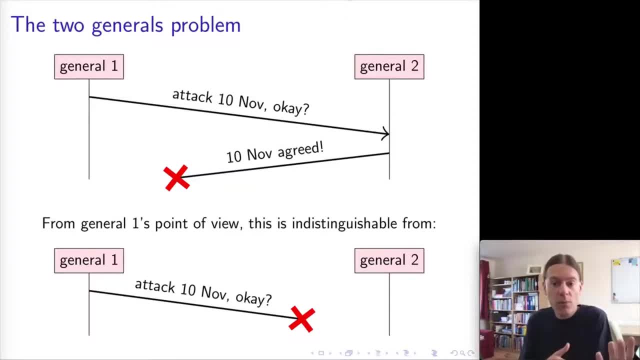 doesn't even know about the attack. So they look the same from General 2's point of view, but they look very different from General. sorry, they look the same from General 1's point of view, but they look very different from General 2's point of view. So let's try to design an. 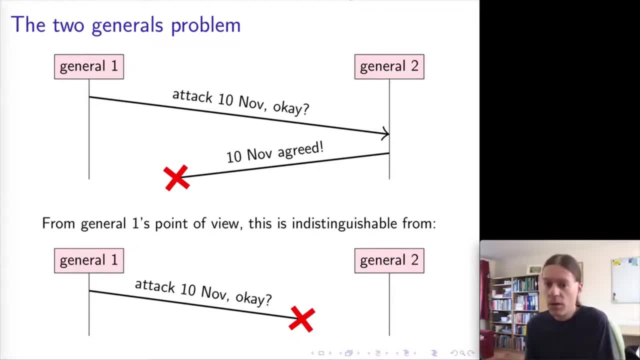 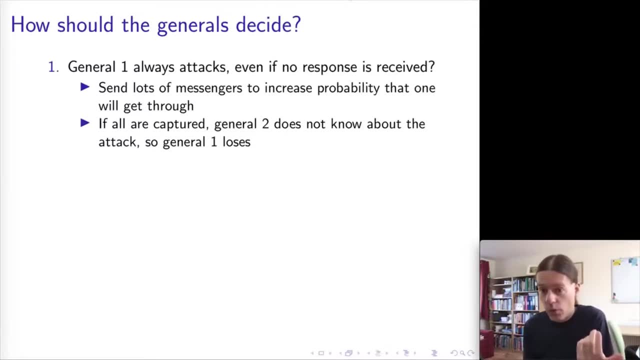 algorithm which will nevertheless get the two generals into agreement. And so let's think about it first of all from the point of view of General 1.. General 1 basically has two choices: Either General 1 is going to always attack, no matter whether any response is received, or General 1. 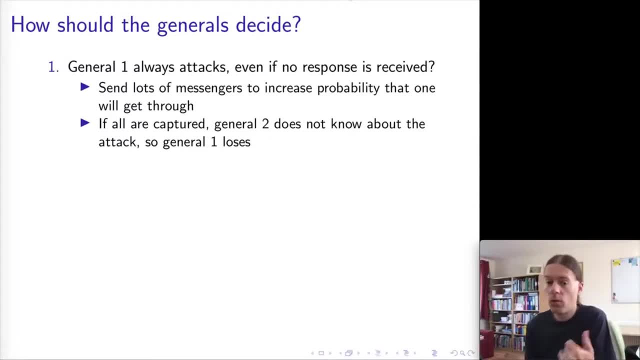 is going to wait and only attack if it receives a response from General 2.. So let's start with the first case. So General 1 always attacks even if no response is received. So in this case, General 1 wants to make sure that General 2 is also going to attack. because, also because, 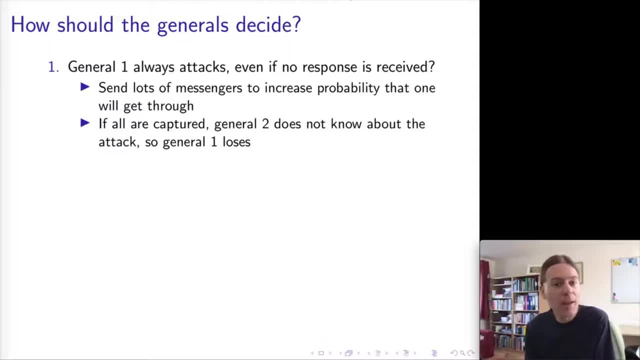 otherwise General 1 is going to be in a problem, problematic situation. So we could say that General 1 is going to send lots and lots and lots of messengers over to General 2, all saying attack at this time, attack, attack. And if one of those gets through, then things are probably okay. 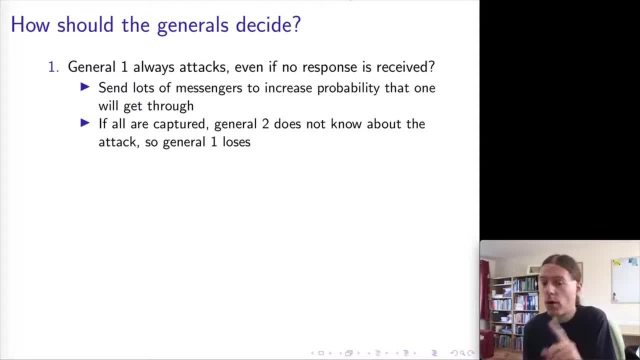 because General 2 knows that General 1 is always going to attack. So General 2 knows that it's safe for General 2 to also go into battle even without responding to General 1, because, after all, General 1 has promised that General 1 is always going to attack. However it could happen. 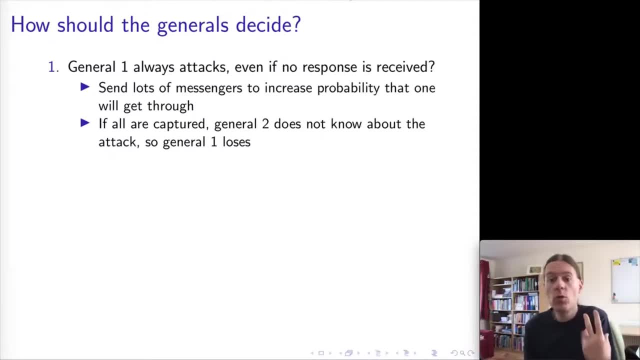 that all of the messengers are lost, And so in this case General 2 does not know about the attack. So General 1 ends up going into battle alone and loses. So that means this first option of General 1 always attacking is not really great. 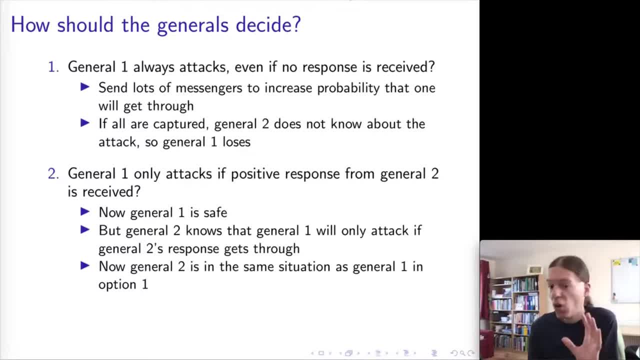 And so we consider the alternative, which is that General 1 does not promise to always attack, but General 1 will only attack if it receives a positive response from General 2.. And in this case General 1 is safe because General 1 knows that it will only go into battle if General 2 is going. 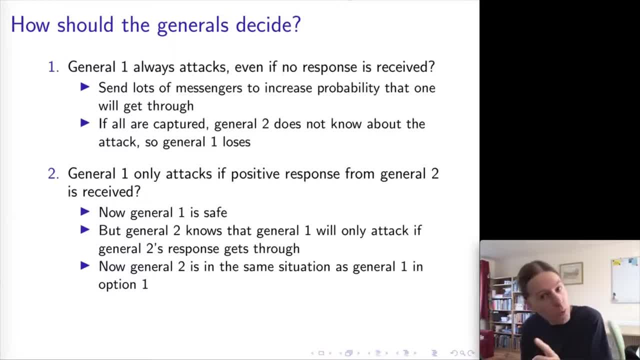 into battle. But now, if you think about it from General 2's point of view, now General 2 knows that General 1 will only go into attack if the response from General 2 to General 1 gets through, because, after all, General 1 is waiting. 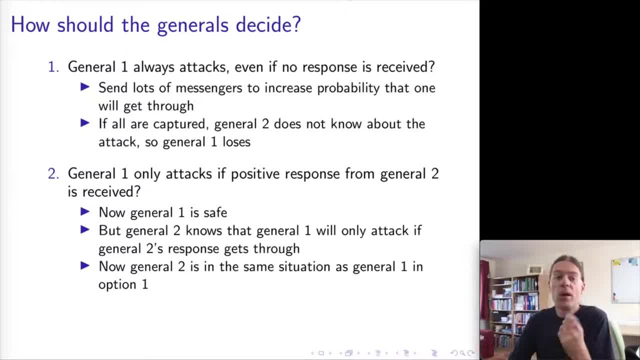 for that response from Number 2.. And so now the General 2 is in exactly the same situation as General 1 was in the first option, And that is, either General 2 must commit to always attack, in which case he risks being alone in the battle, or General 2 will wait for a response from General. 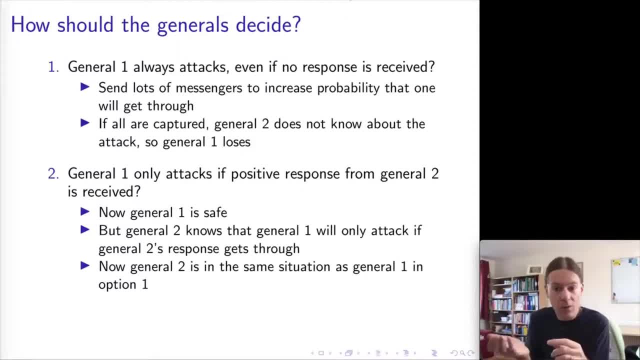 1. But now you know, General 1 has to respond to General 2.. And so now General 2 is in, exactly the one has to reply. and so you end up with these potentially infinite chains of yes, yes, i'm going to attack. okay, i'm going to attack if you attack. yes, okay, i will attack, but only if you also attack. 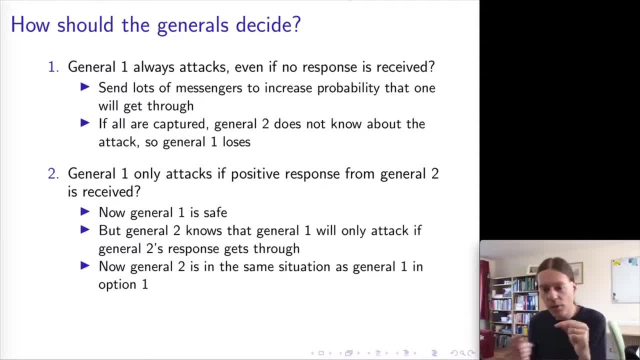 yes, yes, already said i'm going to attack, and so on, and so they have to send each other back and forth these messages. you get actually an infinite chain before there's any certainty that they're actually both going to attack together. and so what is this is called in distributed systems. 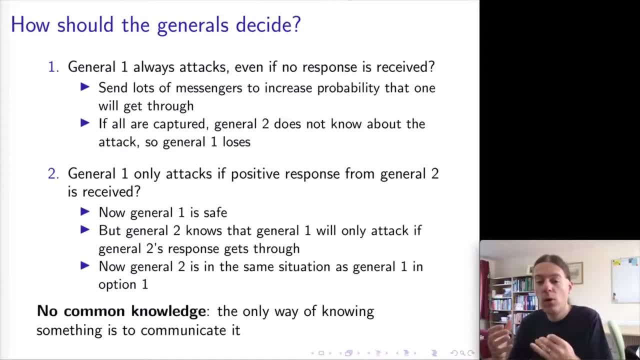 the problem of having no common knowledge. so there's no knowledge in the system that one node knows and the other node knows that the first node knows it, and the second- the first node- knows that, the second node knows that the first node knows it, and so on. so you can construct these. 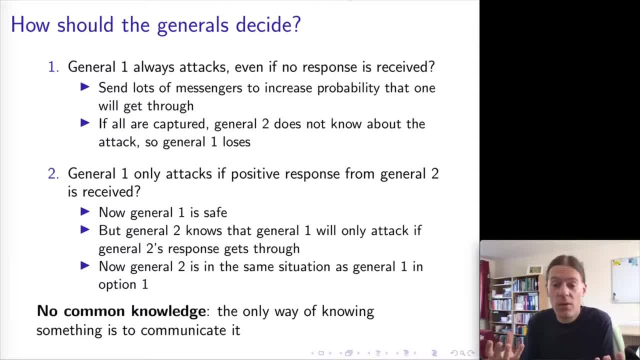 arbitrary chains and the end result is just that, no matter how many finite sequences of messages we send back and forth, we never actually have absolute certainty that general one is going to attack if, and only if, general two is going to attack. so you can build up gradually increasing like probabilistic certainty, maybe. 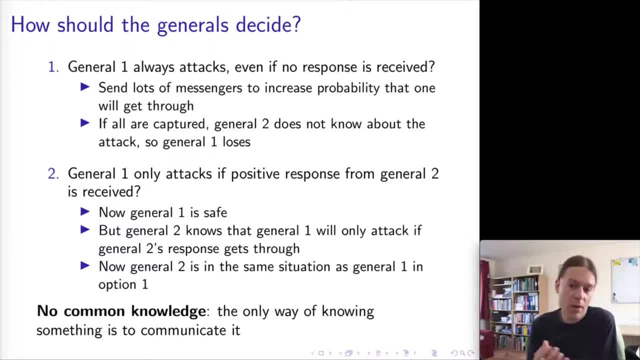 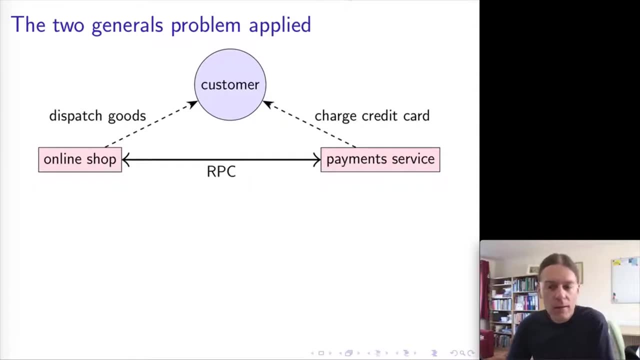 depending on your assumptions of whether messengers get captured or not, but it's actually impossible to reach complete certainty here. now let's take this abstract thought experiment and apply it to a concrete example. so we had in the last lecture this example of an online shop making an RPC request to a payment service in order to 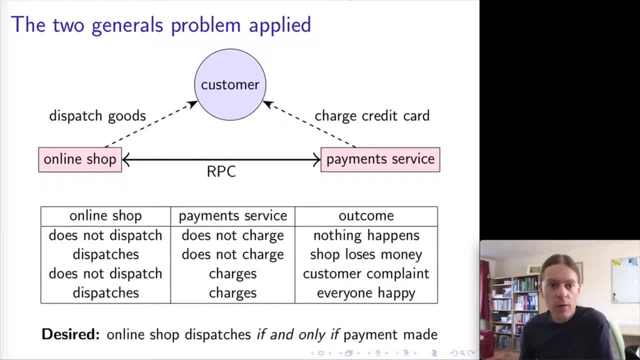 charge a credit card, and really what we want here is that the online shop dispatches the goods if, and only if, the customer pays for the goods. because you can imagine, you know, if the online shop dispatches the goods but the payment service does not charge the credit card, then the shop 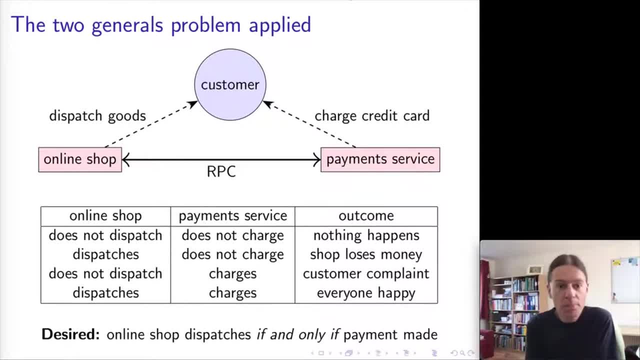 is unhappy because the shop has just given away some goods for free. if the if the online shop does not dispatch the goods but the payment service does charge the credit card, then the customer is unhappy because the customer got charged without receiving any goods. so really what we want is something that looks extremely similar to the two generals problem here. 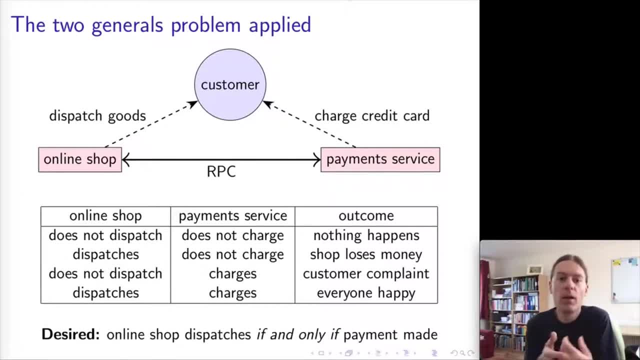 that the online shop dispatches the goods if, and only if, the payment service charges the card and, as you can imagine, the RPC between the online shop and the payment service looks very much like the two generals running through the forest in the two generals problem, which is to say that the messages 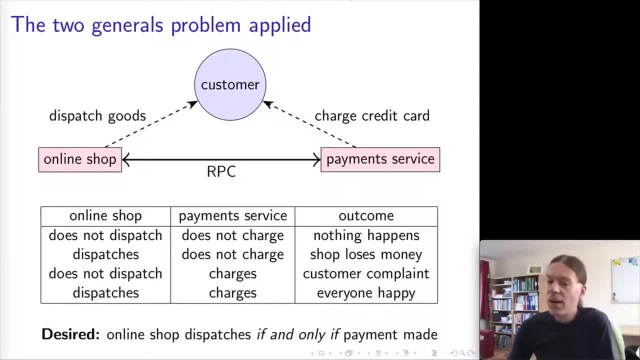 might get lost. either one or the other might get lost, and so it is actually not possible for the online shop and the payment service to achieve this certainty that one action will happen if, and only if, the other other action happens. now, in practice. actually, of course, online shops do work. 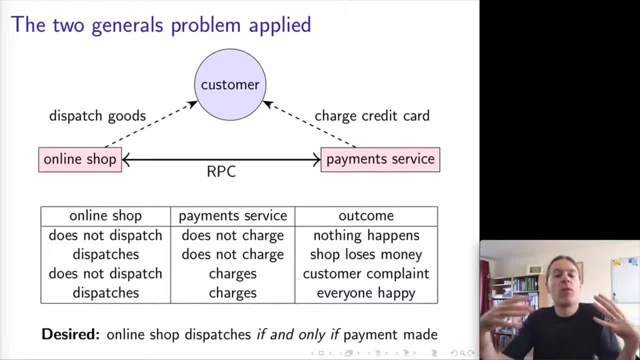 but the reason they work is because there are a bunch of second level safeguards. safeguards, then, which ensure a reasonable outcome. so, for example, if it turns out that the payment, the card, got charged but the online shop doesn't actually have the goods in stock anymore, then the online shop will just send an apology email saying: oh sorry, actually we're out. 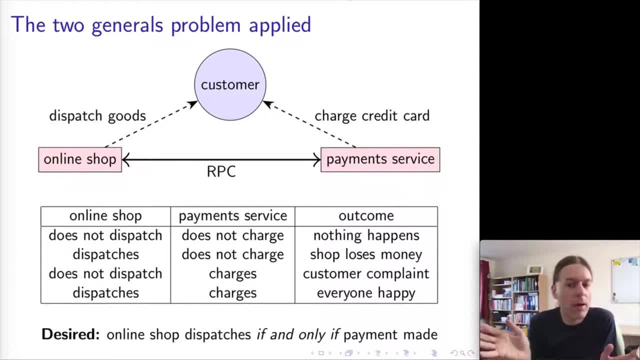 of stock. we've refunded your card and so that way it's fine. and so this: it's possible to get out of the situation because the the charge is actually a revocable action. it's possible to refund the charge and therefore it's possible to get back into a safe state where neither the goods 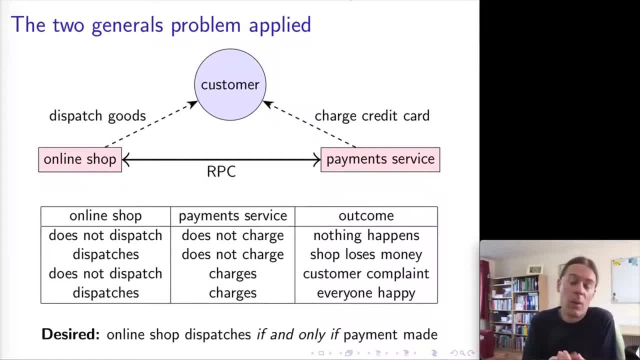 dispatched, nor the payment has effectively happened. or another option is: you know that the payment service may or may not have charged a card, and so the online shop. then, when the network is repaired and the messages can get through again, then the online shop checks with the payment service saying now, did you actually charge that card or not? because i never. 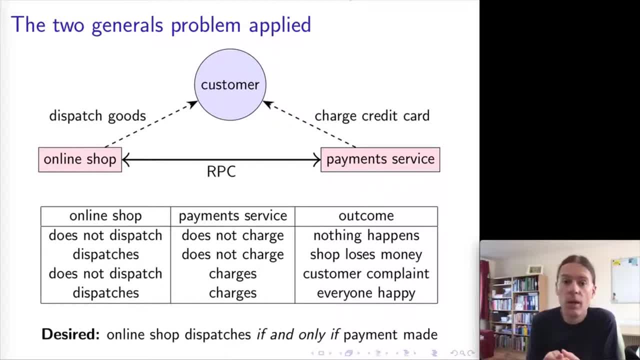 heard back from you, whether you charge it or not, and so what will probably happen is that the payment service will always go ahead and charge the card because if, even if it's not certain that the online shop is going to dispatch the goods, because in this case it's fine, because the payment 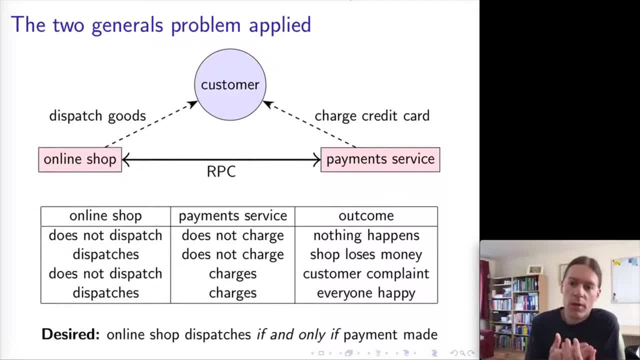 could get refunded if necessary. so that is the way in which this online shopping problem is not actually exactly the same as the as the two generals problem, but nevertheless, the two generals problem does illustrate this problem, and that's why it's so important that the payment service is. 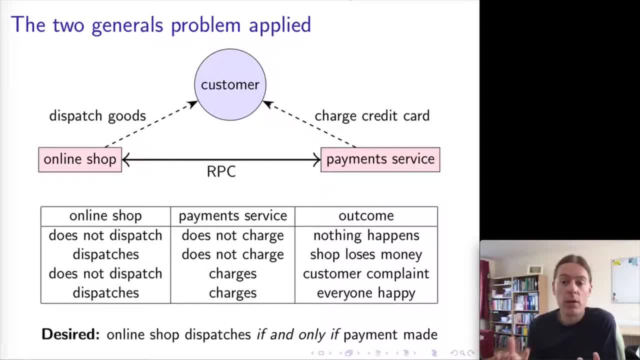 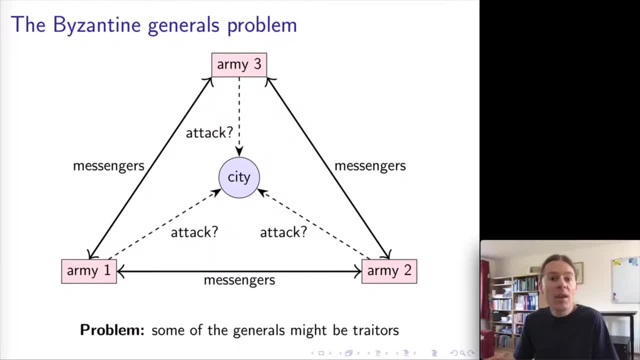 actually the best way to deal with this issue of uncertainty that we have in a distributed system, when we're not sure if the messages got through or not. the second thought experiment that i want to discuss is called the byzantine generals problem. before i get into the details, a question of 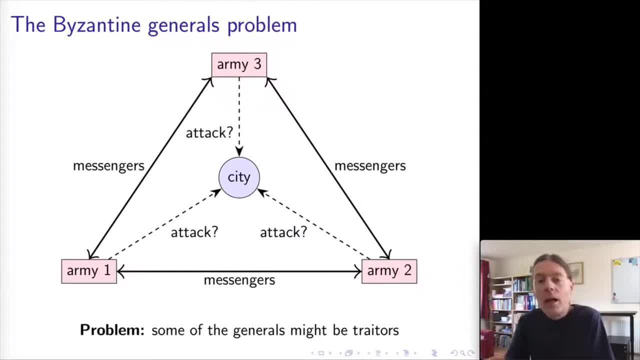 pronunciation. is it byzantine or byzantine generals? well, so as far as i know, the standard british pronunciation of this word is actually byzantine, and byzantine is the american pronunciation. However, in computing it seems to be most common to use Byzantine, and so I'm just going to stick. 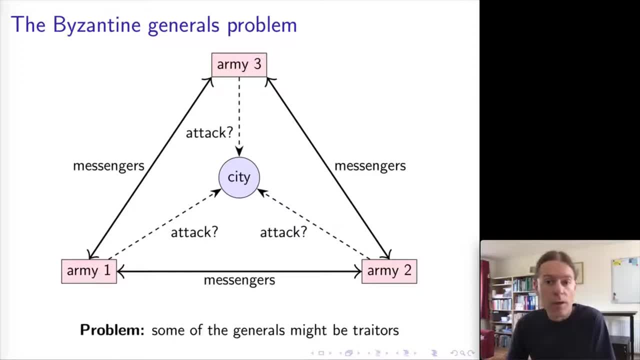 with the pronunciation Byzantine, because that's what everyone else in computing seems to do. So the Byzantine generals problem is similar at first glance, to the two generals problem. That is, again we've got generals leading armies. Again the armies want to attack a city. 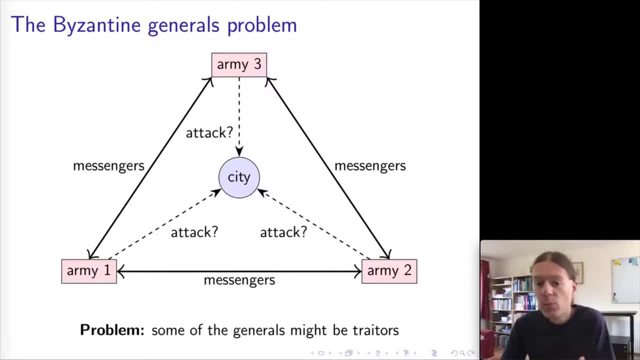 In this case, we might have three or more armies, We might have any number of armies. As before, the generals communicate by messenger And, as before, the armies want to agree on the date of attack so that to ensure that they attack at the same time. 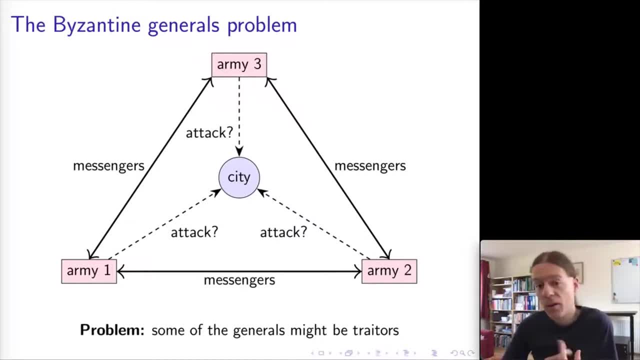 Now we make the problem easier in one way and harder in another way. So easier, first of all, is we assume that messaging is reliable. So in this case we're going to assume messengers don't get captured, but any message that gets sent will actually be received by the appropriate. 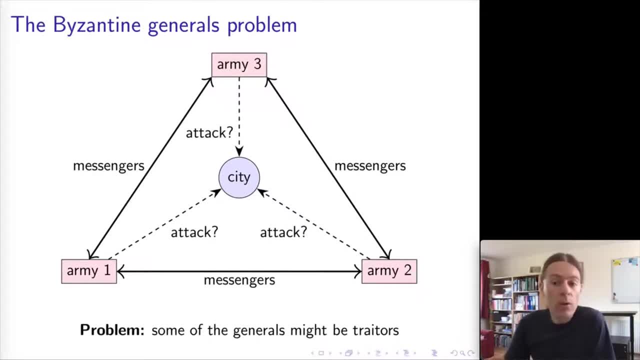 recipient. To make the problem harder, we are now going to assume that some of the generals are actually not loyal. They are traitors, They are malicious, They are going to try to actively undermine the other generals, So they are going to lie and deceive and generally misbehave in any sort of 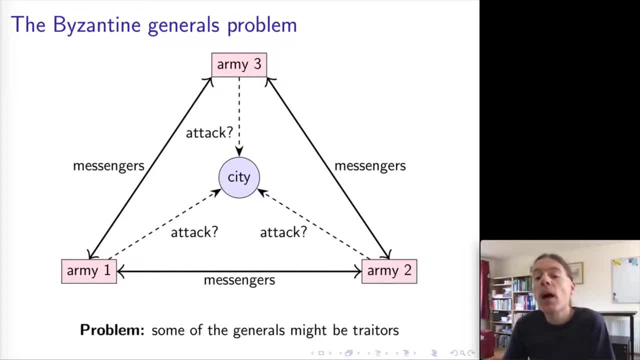 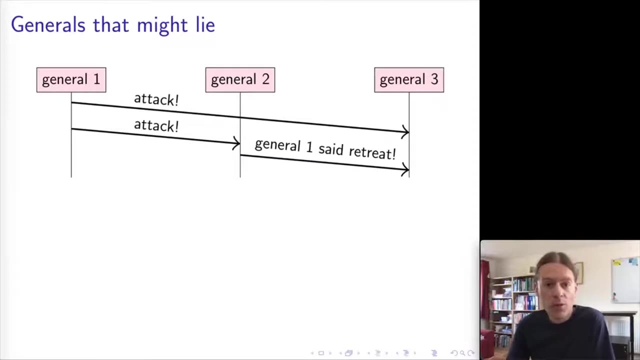 way as they wish. They might even work together, And nevertheless we want the honest generals to come to an agreement about the attack of the city. So let me give an example of the problem that might arise due to some generals being malicious. So here in this example, General 1: 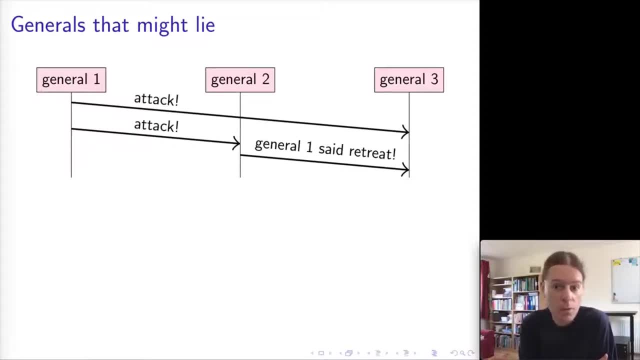 sends a message to attack to Generals 2 and 3.. The same message attack And General 3 receives that message. as expected, General 2 receives the attack message and then sends a message to General 3 saying retreat. So what General 3 does is he sends a message to General 3 saying retreat. So what? 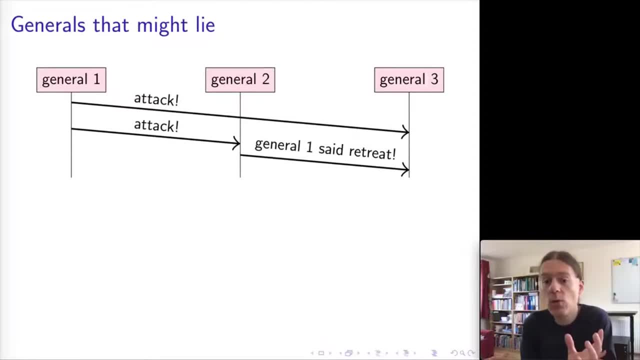 General 2 here is doing is lying. General 2 claims that General 1 sent a retreat message when in fact General 1 sent an attack message. So in this case here General 2 is the one who is being malicious. Unfortunately, from the point of General 3, it's not easy to tell what is actually. 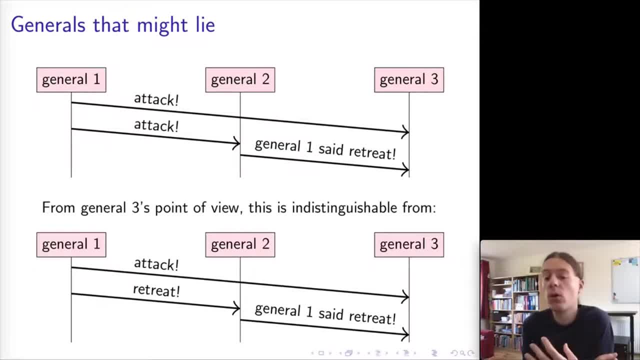 happening Because, from the point of General 3, what could have just as equally well happened is this one. So it could be that General 1 sent an attack message to General 3 saying retreat. So in this case, General 2 is the one who is being malicious And in this 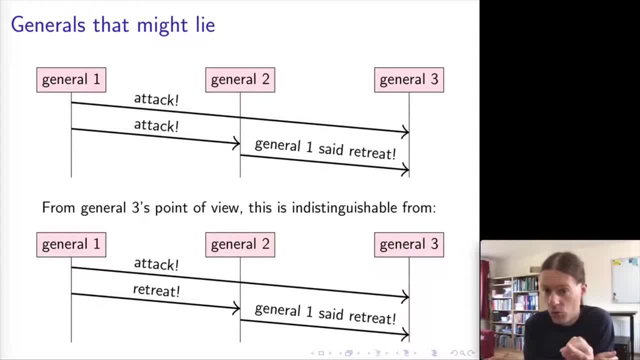 case, General 1 sent an attack message to General 3 and General 1 sent a retreat message to 2.. And General 2 is actually faithfully repeating that retreat message that it got from General 1.. So in this case, in the lower case here, General 2 is being honest because General 2 is just reporting. 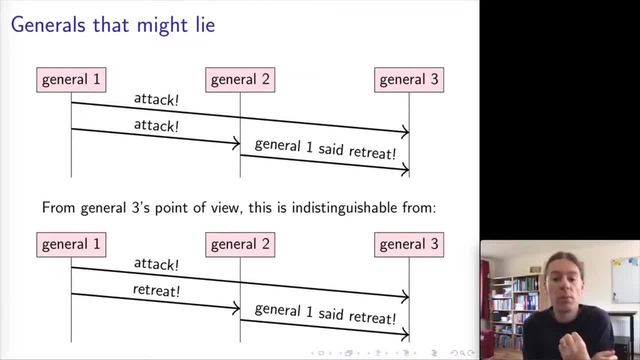 honestly what General 1 said, And it's General 1 who is being malicious by sending contradictory commands to Generals 2 and 3.. So this is the core of the problem. here, For example, General 2 is being malicious And from the point of view of General 3, it's impossible to tell the difference. 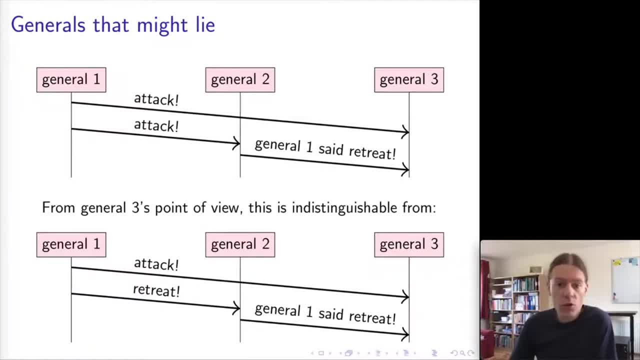 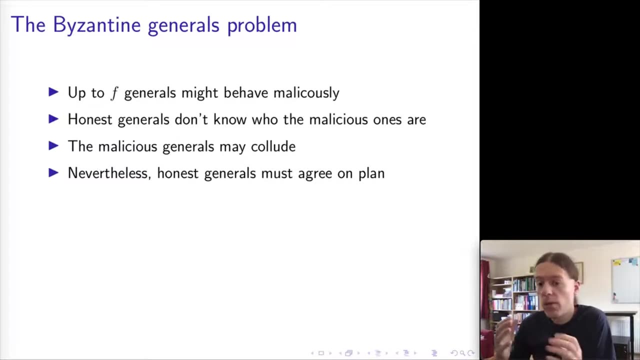 between these two scenarios, And so it's impossible for General 3 to tell whether General 1 is being malicious or whether General 2 is Now, given this scenario, where nodes might lie. the Byzantine Generals problem is, as I said, the desire that is. the problem is that we want all of the honest. 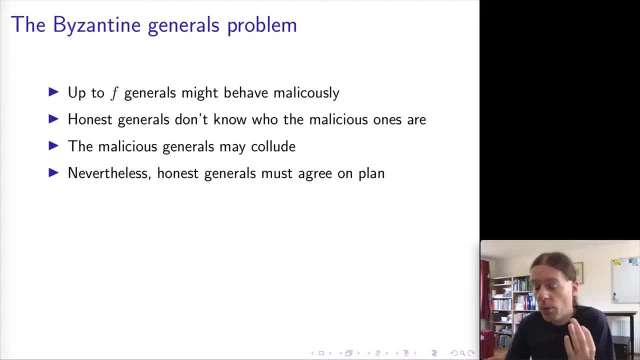 Generals to come to an agreement. So now the problem is that the Byzantine Generals are not malicious. The problem is that the honest Generals don't know who the malicious Generals are. But we are going to assume some maximum number of Generals being malicious. So let's say that up to 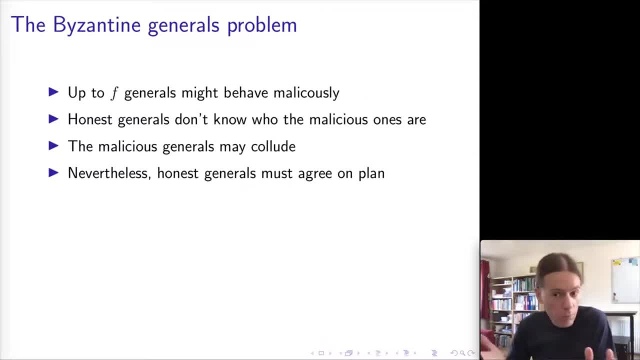 F Generals are malicious out of N Generals in total. The honest Generals don't know who the malicious ones are, But the malicious Generals may know who the other malicious Generals are, And so they might actually even work together in some coordinated fashion to try to deceive and 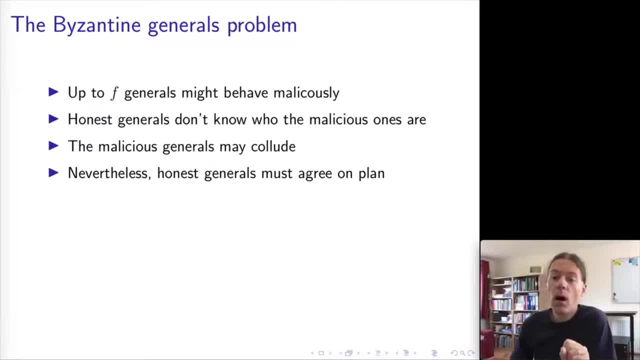 trick General 1 and General 2.. So that's the problem here. But the problem is that the honest Generals have a more direct relationship with the honest Generals And nevertheless, our requirement is that the honest Generals agree on a plan. So we can't claim we can't get the malicious Generals to 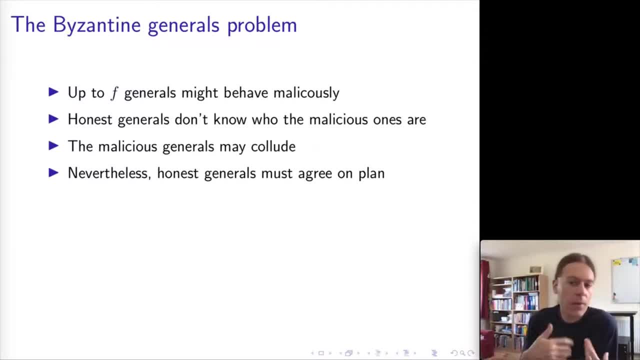 agree on any part of the plan, because we're assuming that they might misbehave in arbitrary ways, And so it's impossible for us to make any statement about what they are going to do. But we can make a statement about what the honest Generals are going to do, And that is they will. 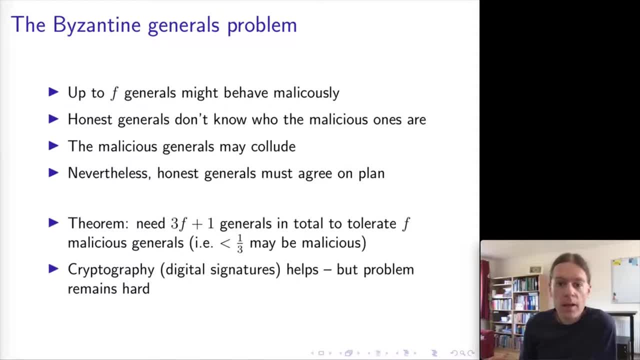 what we want them to do is to all attack on the same day. Now there are several different variants of the byzantine generals problem that vary in the details of how exactly it's set up, but a typical result that we can prove about some of these variants is that if we have a maximum of 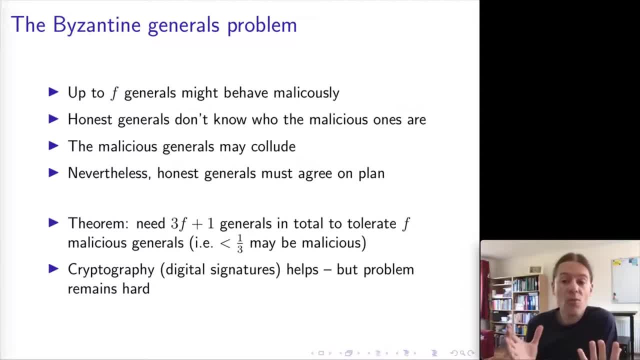 f malicious generals, then we need three f plus one, at least three f plus one generals in total in order to tolerate those f generals being malicious. that is, less than one third of the total number of generals can be malicious. so if we have three generals and one is malicious, 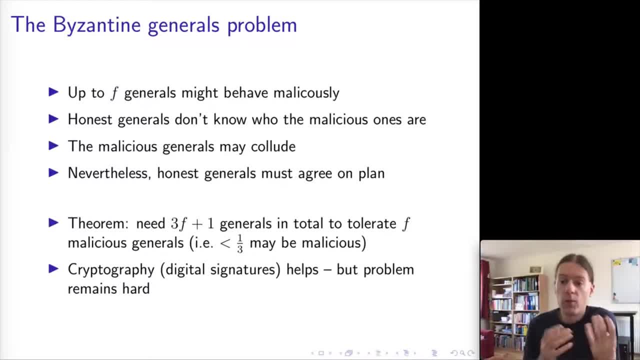 the problem is unsolvable. in order to tolerate a system with uh, with one malicious general, we need at least four, and it's f equals one. we need at least four generals in total, so three honest ones and one malicious, if we want a system which two generals might be malicious. 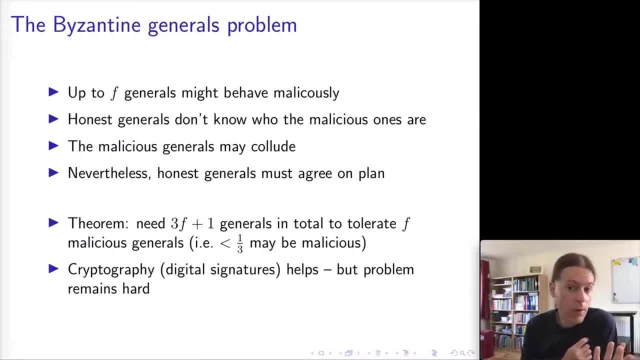 we actually need seven, so five honest and two malicious generals. now the problem becomes somewhat easier if we assume that we can use cryptography, and so i won't go into the details of that in this course. there's more detail on this, uh, in the security course and in the cryptography course that you will have next year, and but what we can do here is: 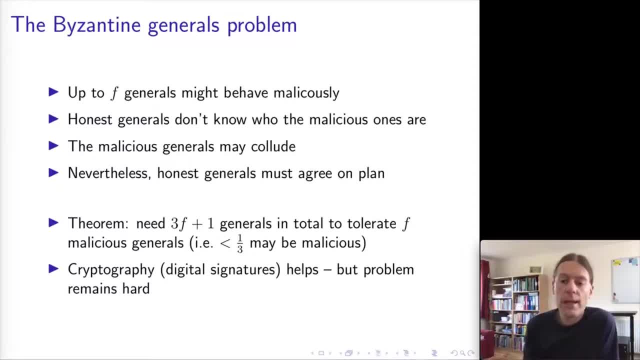 use something called a digital signature, which is a form of message in which it can be proved that a certain party sent a certain message, and so in this case, for example, it would allow just a certain party to send a certain message, and so in this case, for example, it would allow just 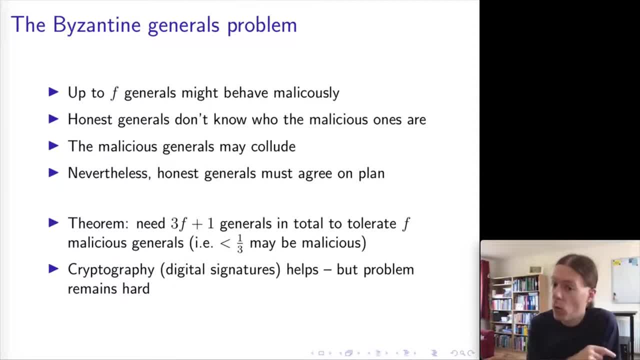 general 2 to prove what command general 1 sent to general 2 and prove that to general 3 in a way that general 3 would be convinced that general 2 really is honest. so cryptography does help, but it doesn't make the problem representing general problems magically simple. so even if we do assume, 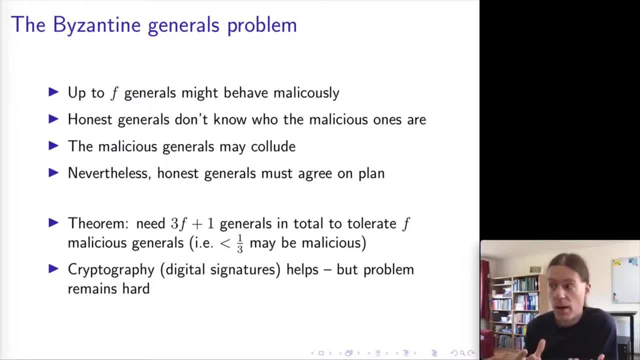 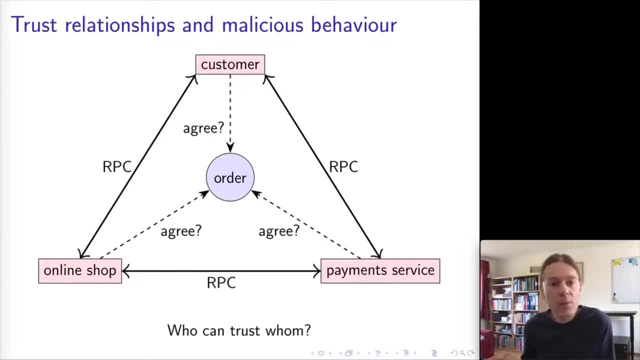 that we can use cryptography, the problem remains difficult. so is this at all of practical relevance, you might ask. so let's adapt this earlier example that we've had a few times now of the online shop and the payment service, and let's take, in this case, the customer as a third party in this. so we have this. 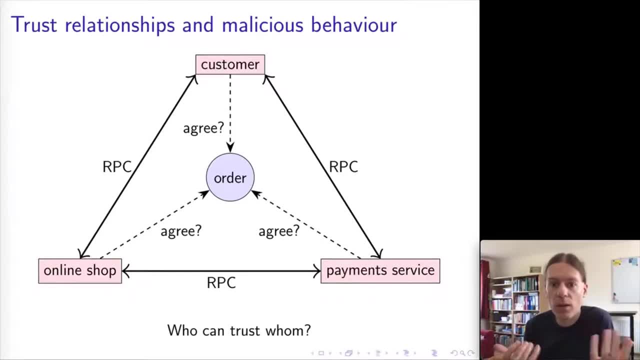 kind of three-way relationship between the shop, the payment service and the customer, and we want all three of these parties to agree on the status of a transaction or status of an order. so we want the online shop to ship the the goods only if it agrees with the payment service that the payment 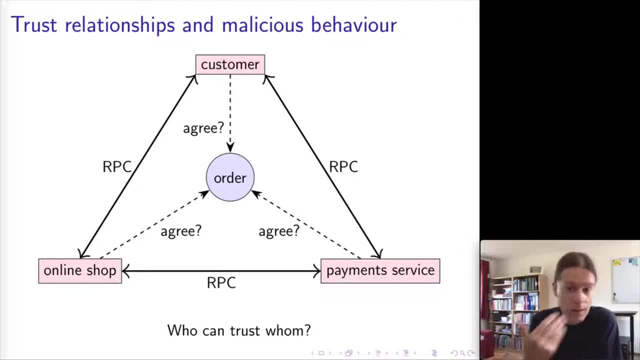 actually happened and if the customer actually agreed that they did actually order this thing. and the customer agrees on the quant, on the amount that was charged, the card and so on. so all of these parties need to agree and in real life the trust relationships between these three parties might be quite complicated. so if you think about it from the perspective, 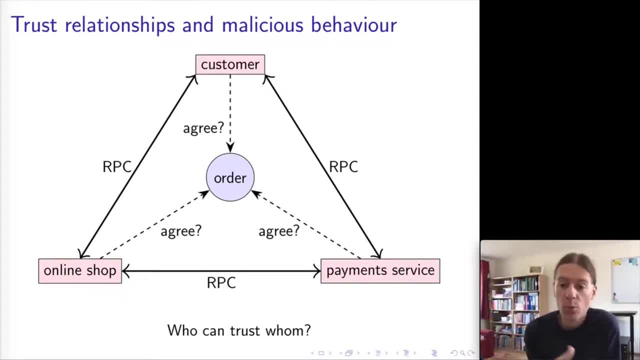 of the online shop. if there was some way how people could order goods from an online shop without paying for them, you can imagine that fraudsters would be using that pretty quickly and they would be ordering all sorts of expensive things without paying for them, and so the online 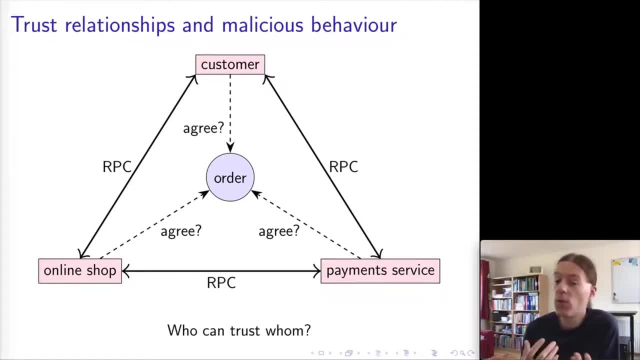 shop would not be happy then. so from the point of view of the online shop, the customer needs to be treated as potentially malicious, because if the customer was just blindly trusted, then they might start doing fraudulent activity like that, and so in that case we do have this kind of untrusting. 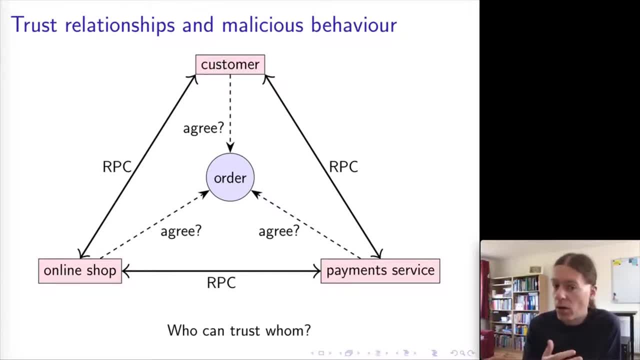 relationship? what about the online shop and the payment service? the relationship? well, you can see, imagine, maybe the payment service doesn't quite trust the online shop because otherwise someone might set up a fraudulent online shop and use, say, stolen credit card numbers to try and process transactions and get money without actually shipping any real goods. so in that case, probably, 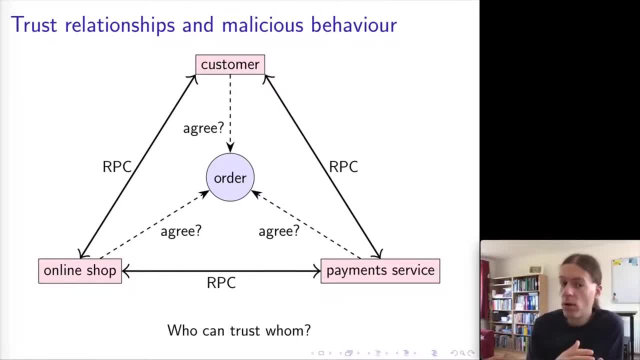 the online shop doesn't, sorry. the payment service doesn't fully trust the online shop, but maybe the shop does trust the payment service, so it might be this kind of asymmetric relationship. so, as you can see here, the trust relationships in real life get rather complicated. you do end up in 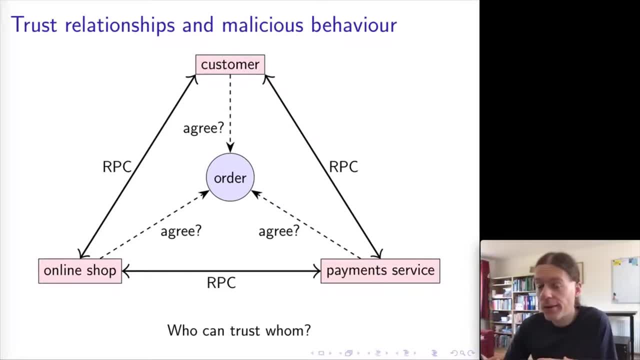 these situations where one party does not trust another party and they nevertheless want to get something done, and so, in that sense, Byzantine behavior is real and practical. the Byzantine generals problem is, of course, a simplification of this kind of scenario, because it's treating all of the generals as symmetric, for example. but nevertheless, the Byzantine generals problem. 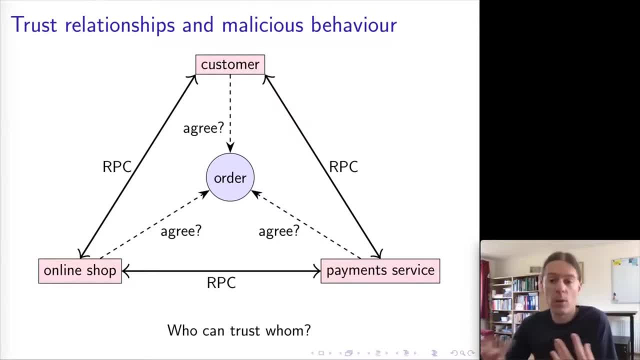 is a simplification of the scenario, and so, in that sense, the Byzantine generals problem is a simplification, is a useful starting point for studying these kind of situations in which the participants don't fully trust each other. So, before I wrap up about the Byzantine generals problem, 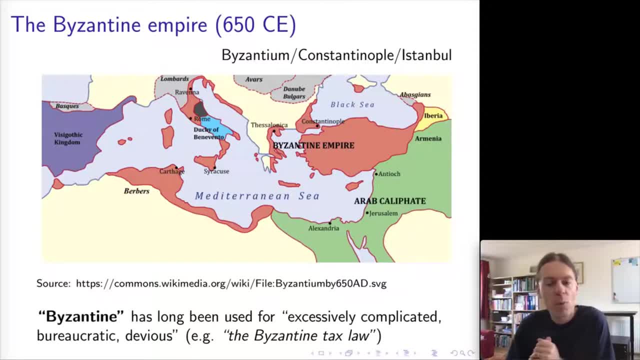 one more little historical digression. You might be wondering where the name Byzantine comes from. So this comes from the Byzantine Empire, which are also known as Byzantium, the former East Roman Empire, which, after the collapse of the Roman Empire, this was the eastern part of it, And 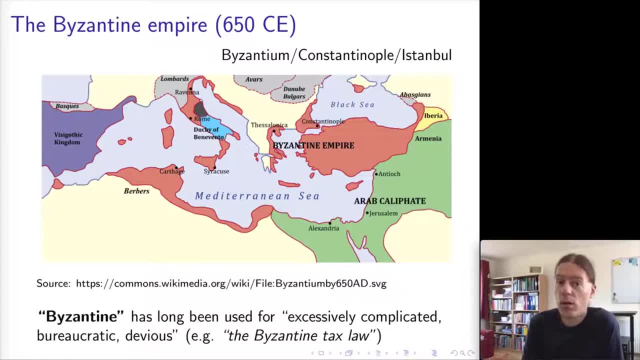 its capital city was Constantinople, which was formerly known as Byzantium, which is now where Istanbul is located, in Turkey, And so for some reason in the 20th century- early 20th century, I think- the term Byzantine became used in order to describe. 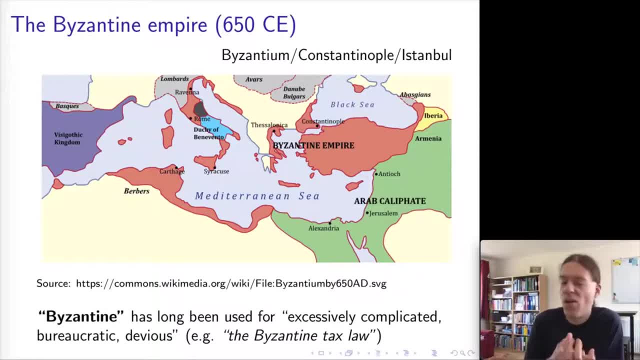 scenarios where things are excessively complicated or incredibly bureaucratic or potentially even devious, for example tax legislation or these kind of thing. Not entirely sure why that meaning of Byzantine occurred, because there's no historical evidence really that the Byzantine Empire was. 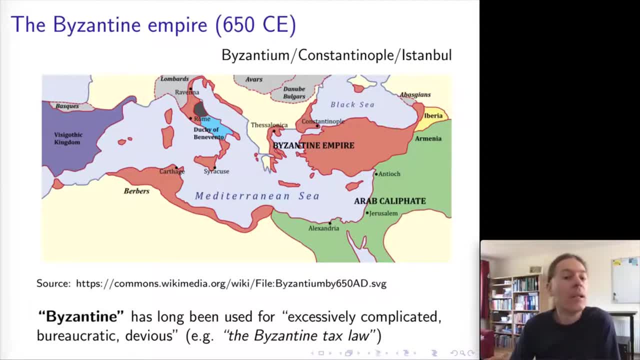 any more or less malicious than any other empire, But anyway, that's where it came from. So the term Byzantine had this meaning long before it was used in the context of computing. So it outside of computing. it has had that meaning for a long time. So that's all on the Byzantine. 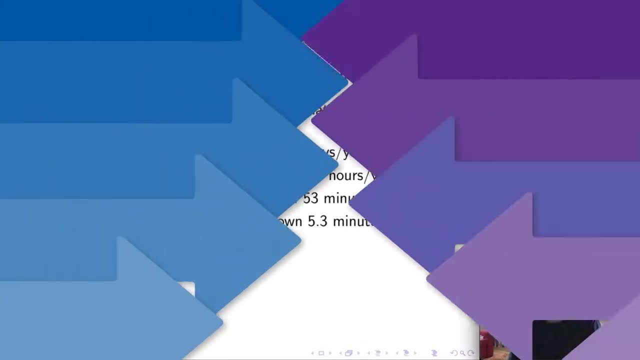 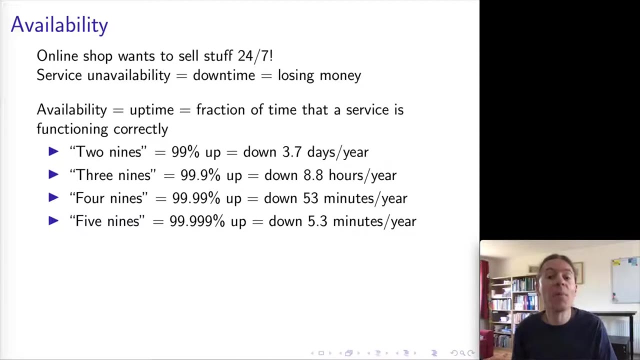 generals problem for now. In the last bit of this lecture, I want to talk a little bit about a practical, real life context for faults, handling faults and making highly available services. So imagine you are running an online shop, for example. you probably want that shop to be. 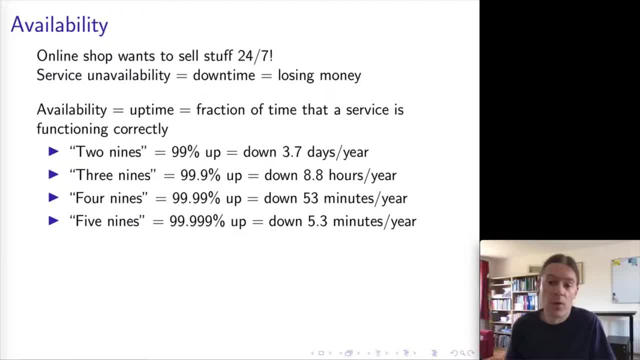 available 24 hours a day, seven days a week, because who knows what time of day or night somebody might decide that they want to go and look at your shop and maybe buy something, And so any time during which your shop, your service is not available actually means losing money In other cases you might imagine. 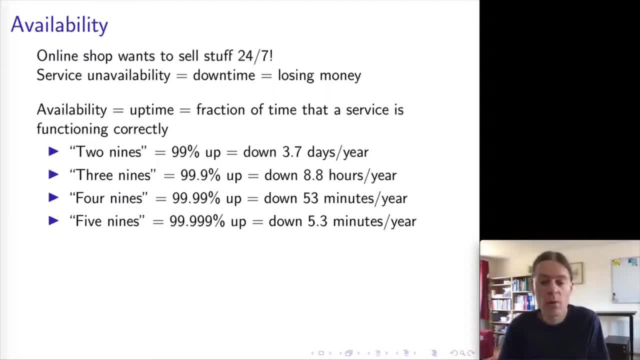 that a service may even have contractual relationships with its customers, specifying what percentage of time a service needs to be available, And so a typical model for how we usually talk about availability is the fraction of time during which a service is functioning correctly. So if a service is functioning correctly 99% of the time, for example, that means that 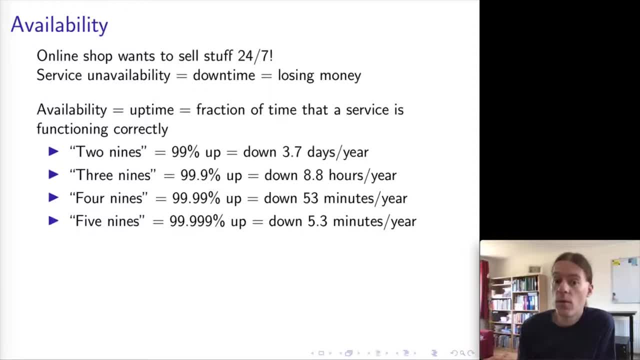 there might be three to four days a year during which the service is not available. in total, Of course, this might be several smaller outages, Or if you go up to 99.9% of the time, you're allowed a maximum of nine hours per year of outage, And you can increase this. 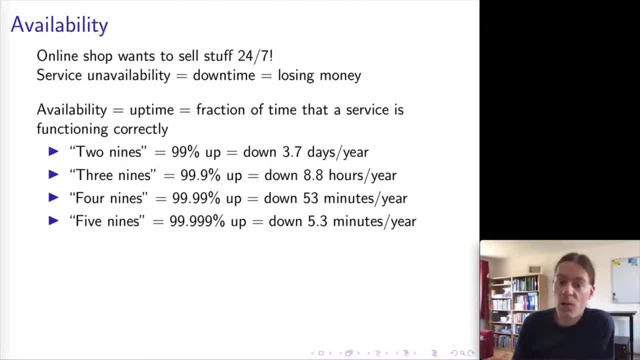 further to as many nines as you like. So the telephone network, for example, is apparently designed for five nines. And so this is the, the old fashioned fixed line telephone network, not mobile networks, certainly not the internet. they don't have this sort of availability. 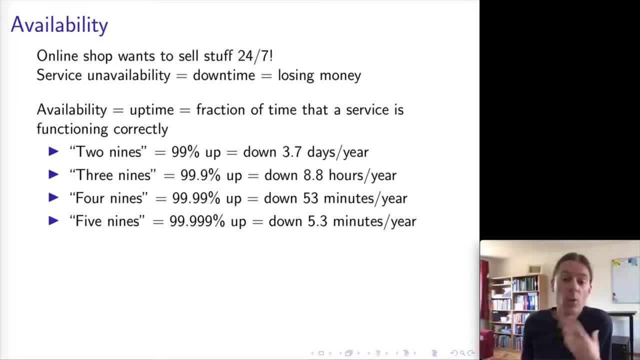 The telephone network is designed in a very conservative way in order to achieve this, this very high reliability. but it is possible, And typically terms that you get in the context of availability is SLO and SLA, So an SLO a service. 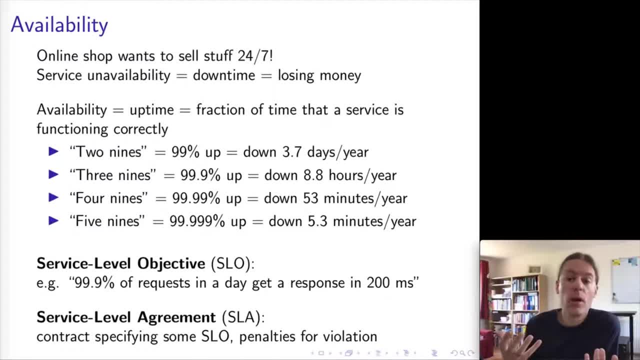 level objective is the goal that you are setting yourself in terms of the availability of a service. So this might specify the percentage of requests that need to get a correct response, where the maximum time that it's allowed to take for that response, say, 200 milliseconds or. 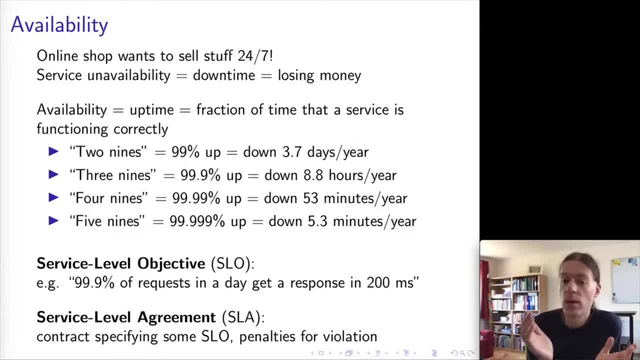 whatever, and the period of time over which you're going to measure it. So you're going to take that 99.9% over the course of all of the requests made in one day, for example, And then, at the end of the day, you're going to take that 99.9% over the course of all of the requests made in one day. 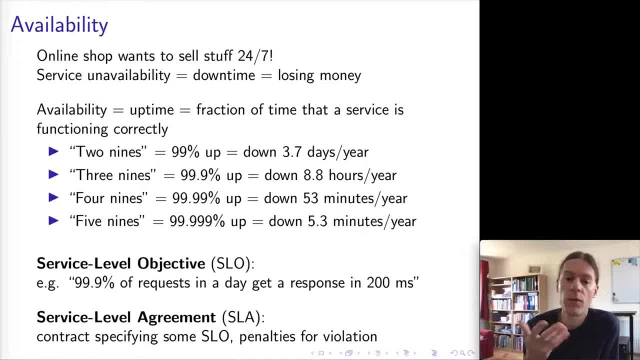 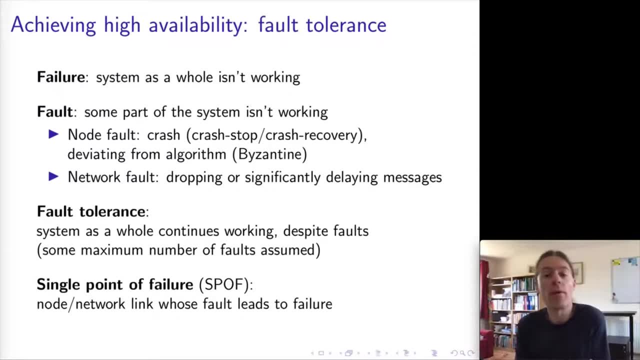 for example. So SLA is basically a contract between a service and its customers or its consumers, specifying what the expected service level is Now in order to achieve that sort of very high availability. the way we typically do that is in distributed systems, is by fault tolerance. 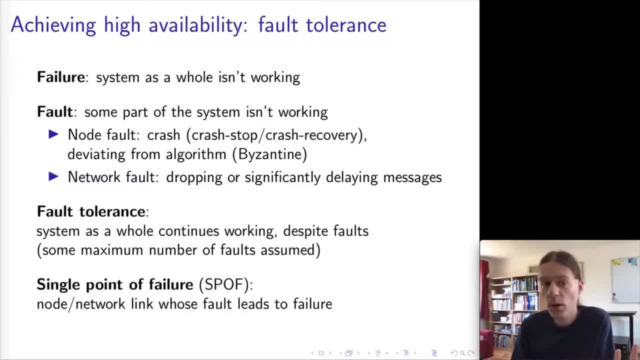 So a fault is when some part of the system isn't working. We talked about node faults, which might be a crash, for example, or network faults, which might be a network partition, And what we want is the system to tolerate some number of faults. So it doesn't make sense to say: 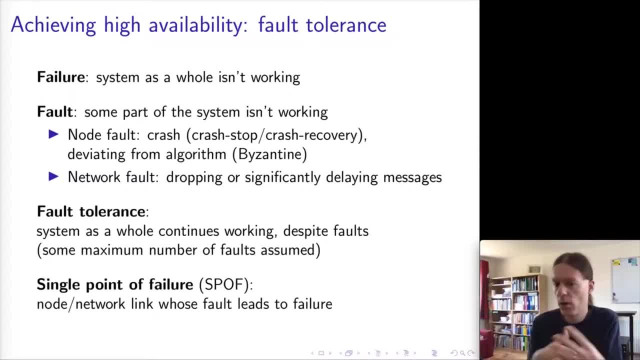 that the system will tolerate all faults, because if all of your nodes crash at the same time and all of your network links go down at the same time, the system is not going to be able to do anything. obviously There's no way it can make any progress in that case. But what you might be able, 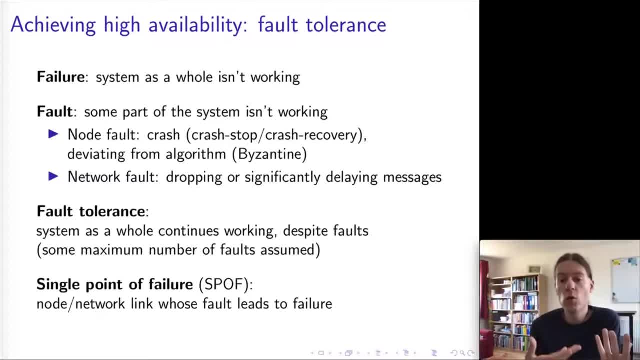 to say is that the system as a whole will continue working if fewer than half of our nodes have crashed, for example. nodes have crashed, for example, So you allow one out of three to crash, or you allow two out of five to crash, and the remaining nodes can still continue running the service. And so, in a system, 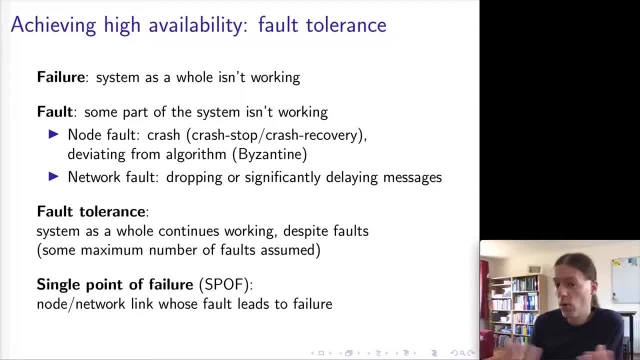 in which some parts of the, some nodes or some network links are allowed to be faulty, we avoid what is called a single point of failure. So a single point of failure would be, say, one node, that if that one node crashes then the system as a whole becomes unavailable. But if we can design 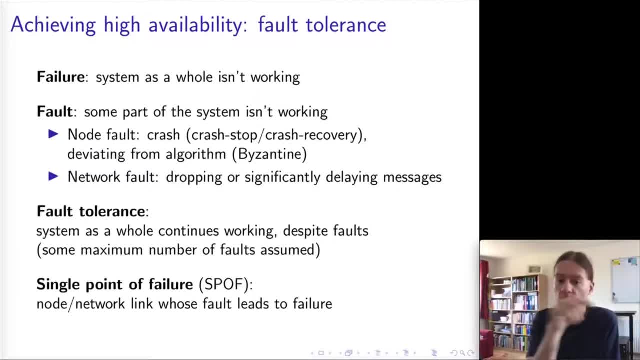 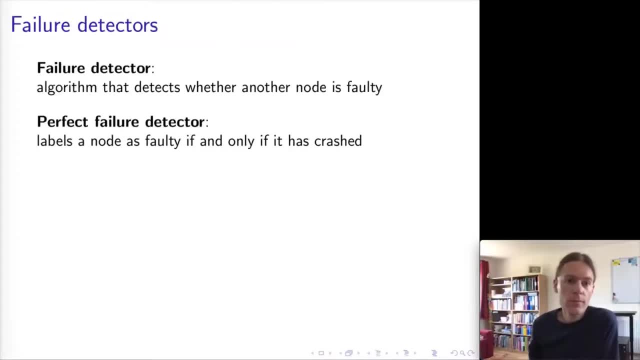 a system without a single point of failure. that means that we can take out any one component of the system and the system as a whole will hopefully still continue working In order to enable to tolerate faults. usually, the first thing we have to do is to detect a fault, and then we can handle. 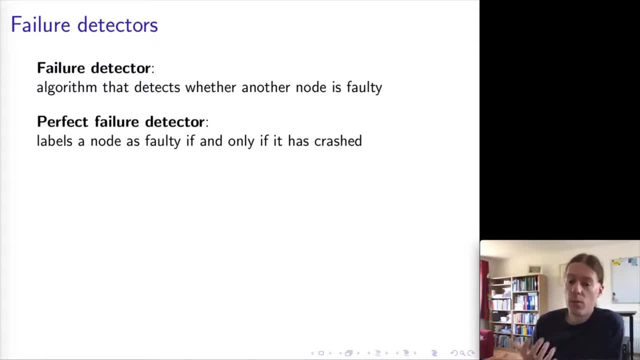 it. So the mechanism for detecting a fault is known as a failure detector. The terminology is a little bit odd. It ought to actually be called- should be called a fault detector. That would make more sense. But a failure detector is the common term that is used, so we're going to stick with that. So a failure. 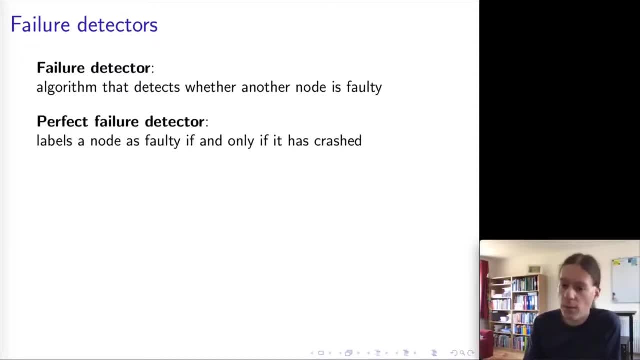 detector is. it could be like a software algorithm, or it could be a piece of hardware or something, some mechanism for detecting whether another node is faulty, And ideally what we would love to have is a perfect failure detector. That is, some mechanism that is always accurate at telling us. 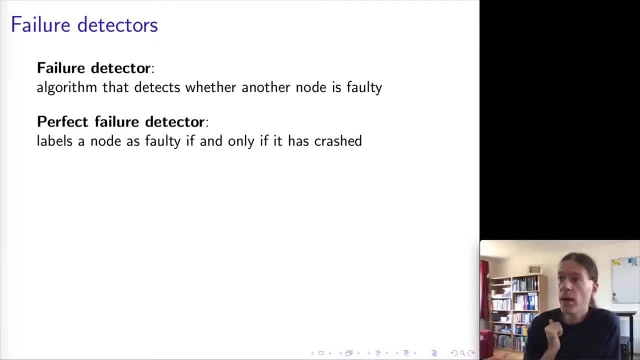 whether a node is faulty or not, And that's what we're going to do. So we're going to use a failure detector whether another node is faulty or not. Now, the way we typically implement failure detectors is we use timeouts, So we simply send a message to a node and say, hey, please respond to. 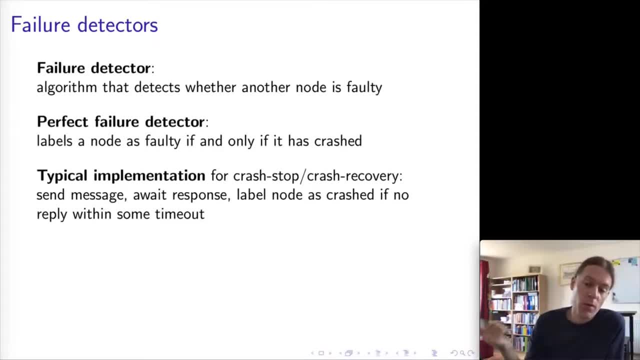 this message if you're alive, And then if we don't get a response within some amount of time, then we say, well, okay, we didn't get a response, That node must be dead, So it must have crashed, or something like that, And this is fine, This is practical, But unfortunately, as we have seen in 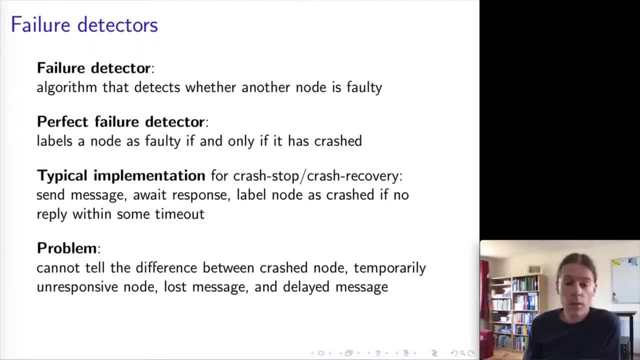 the context of our system models. if we assume a partially synchronous or even an asynchronous system, then a timeout doesn't necessarily tell us that the node has crashed, Because a timeout could also happen because we sent a message and the message was lost in the network or the response. 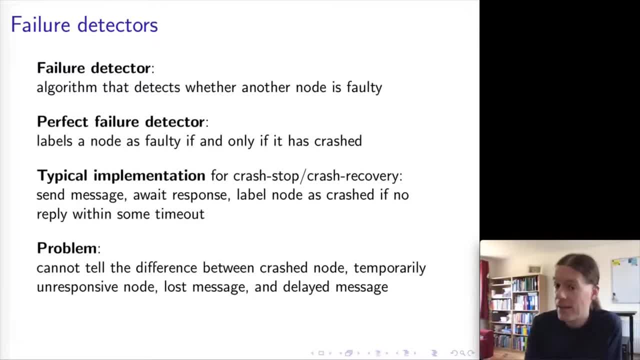 was lost in the network, or the message was delayed in the network, and it will actually still arrive. It just hasn't arrived yet. Or the response was delayed in the network, Or maybe the node is actually alive, but it's just experiencing a long garbage collection pause, And so it will. 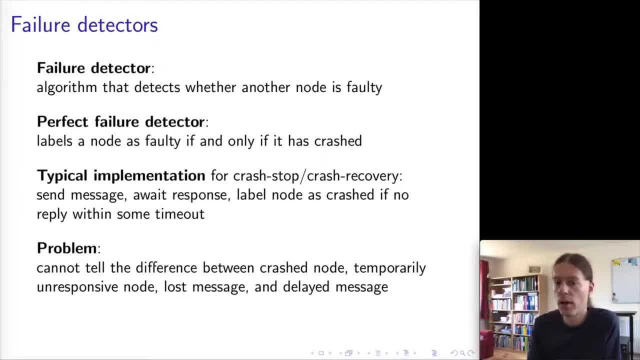 respond to your message in one minute's time. Once it's finished, it's garbage collection, Or, of course, the node might have crashed And it's impossible to tell the difference between any of these. So it's impossible for the sender of these check messages to tell whether the absence 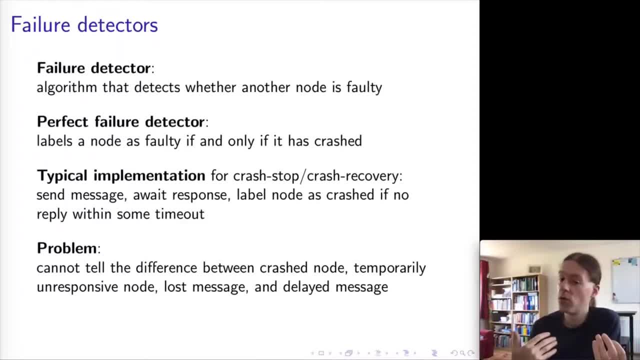 of a response is due to a network problem or due to just some kind of random delay, Or due to problems because the node has actually crashed. Now we can build a perfect failure detector if we have a synchronous system model And if we're going to assume only crash stop. 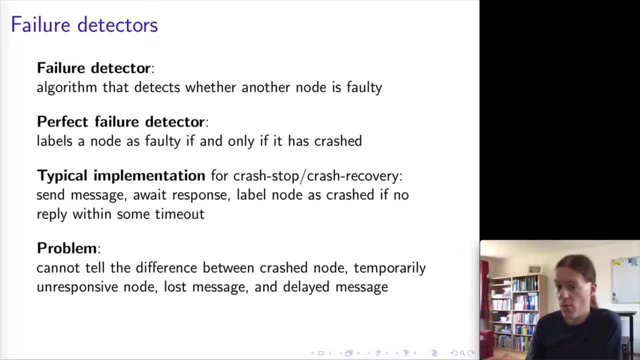 failures and certainly not going to assume any Byzantine behavior in the system. But you know, as soon as you go to a partially synchronous model, then timeouts are no longer an exact way of detecting failures. So the best we can do. 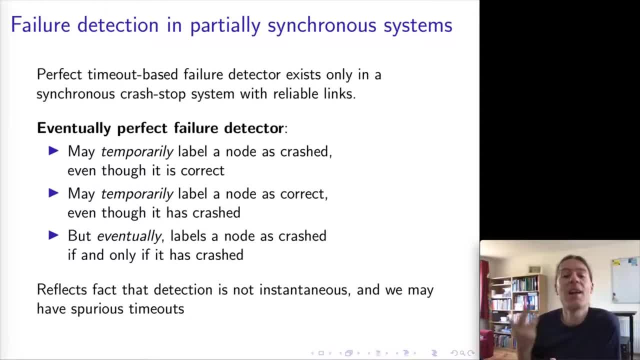 do in a partially synchronous system is what is called an eventually perfect failure detector. I love this term. You know, nobody is perfect. I like to think of myself as eventually perfect. Maybe you are also eventually perfect. And then, in the context of a failure detector, 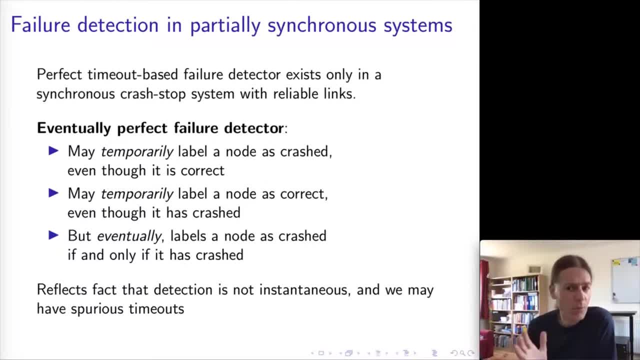 eventually perfect- means that the failure detector might be wrong from time to time. So the failure detector might detect a timeout even though the other node hasn't actually crashed yet, just because a message happened to be delayed a bit. So it means a timeout does not accurately. 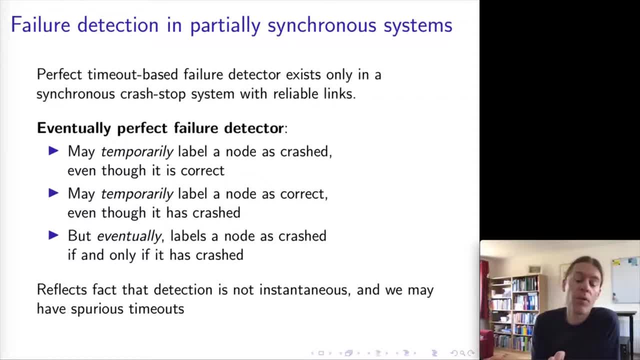 indicate that a crash has happened. Also, a failure detector is not immediate, So if a crash has happened, it might actually take a while until we detect that crash. The detection of the crash is not instantaneous, So we might be wrong. We might have both false positives and 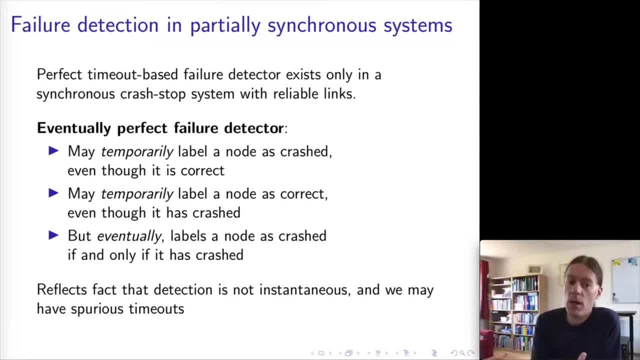 false negatives for a while, But eventually the failure detector labels a node as crashed if, and only if, it really has crashed. So that means that any temporarily suspecting another node of being failed is a failure detector. If a failure detector is failed, we'll stop and we'll go back to thinking that a node is correct. 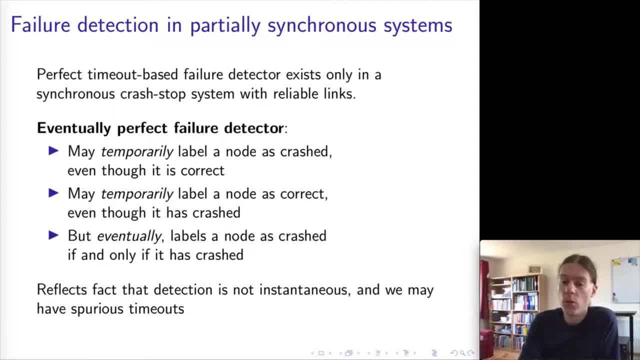 provided that the node really is still correct. And also, if a node has failed, then eventually we will detect it as failed, And so this is about the best we can do in terms of failure detection, But it's still quite useful. So, even though we might have this failure detector, 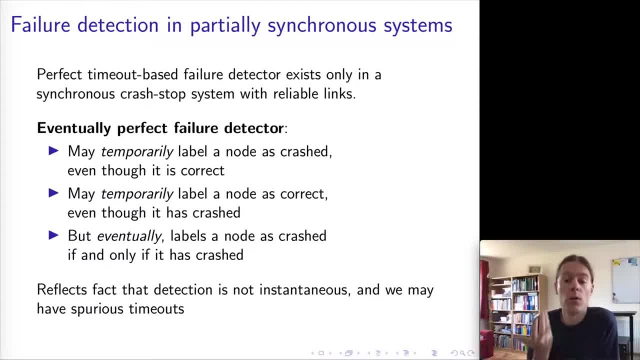 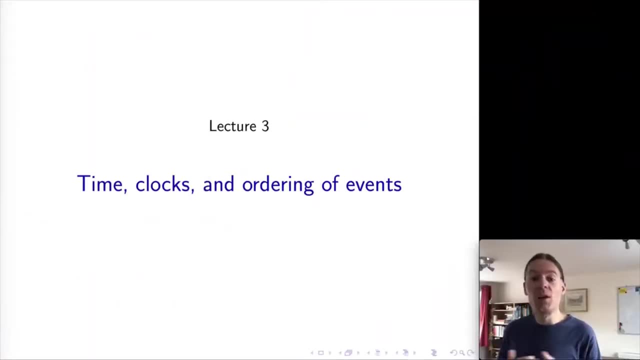 that is only eventually perfect. this is actually sufficient in order to build some useful algorithms, as we will see In some of the future lectures. So that's all for today on system models. Hello everyone, Welcome to the third lecture of distributed systems. Today we're going to have fun. 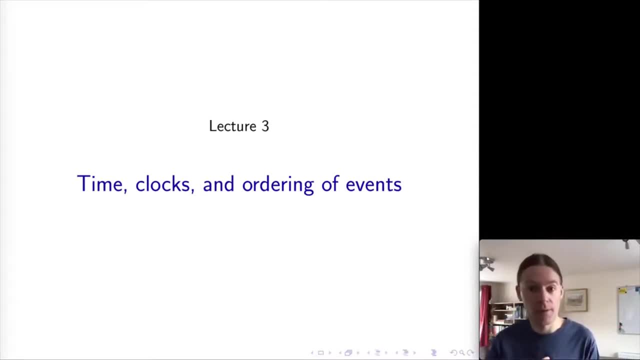 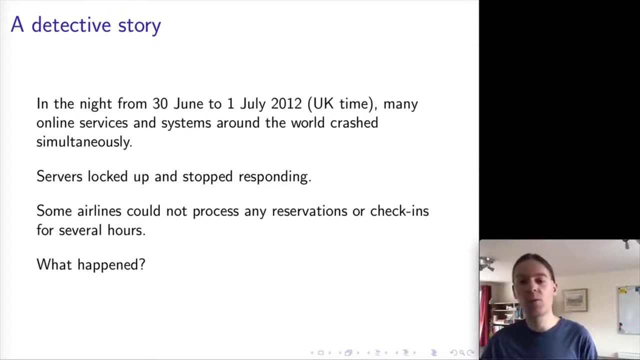 talking about time and clocks and ordering of events in a distributed system. So let me start with a little puzzle, something that you can ponder about, And I will resolve this towards the end of this video. So this is an incident, a real incident, that occurred in 2012, on the 30th of June. when system administrators at a whole bunch of different companies and services had a really bad day because for some reason, a whole lot of servers all locked up and stopped responding to requests all around the same time, sometime in the middle of the night. So what might have? 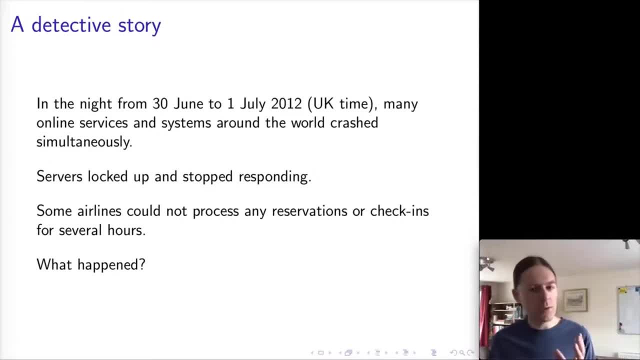 happened? Why did servers across a whole bunch of different companies all fail at the same time? We'll have a think about that and answer will come later. So I want to talk about time, And time is very useful in distributed systems, And it's very useful in distributed systems And it's very useful. 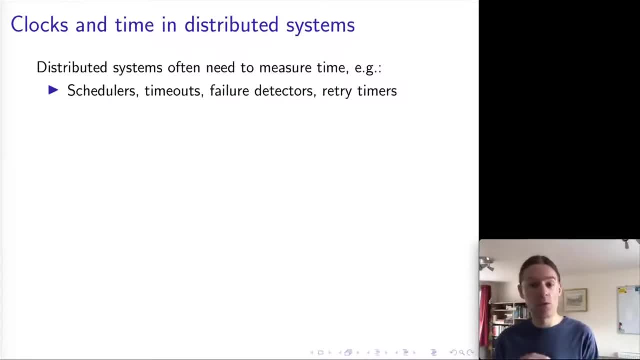 in distributed systems And in operating systems. And just to remind you of a couple of uses of time: for example, in an operating system scheduler you want to context switch after a process has been running for 10 milliseconds maybe, so you have to measure those 10 milliseconds If you want to send. 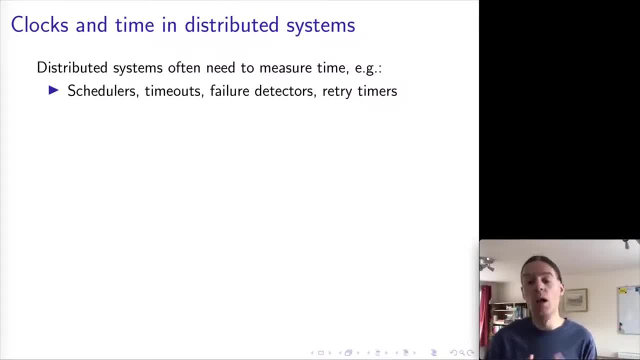 some kind of timeout, then of course you have to measure that time. Last lecture we talked about failure detectors, which again rely on measuring whether you got a response or not within a certain period of time. If you want to retry sending messages over a network again, 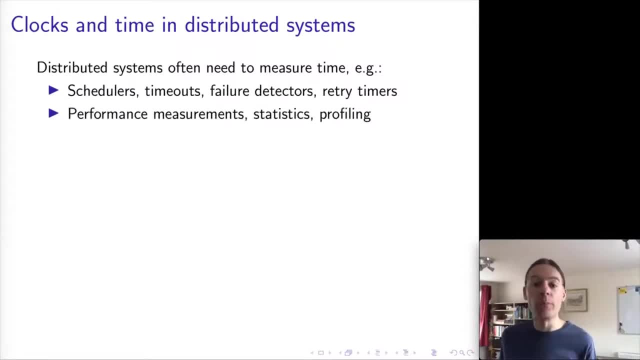 you probably want to wait for a certain time. all of those require measuring time. Other things that require measuring time are the performance measurements. So how long has the process been running? for How much CPU time has it been using? If you want to profile a system in order, 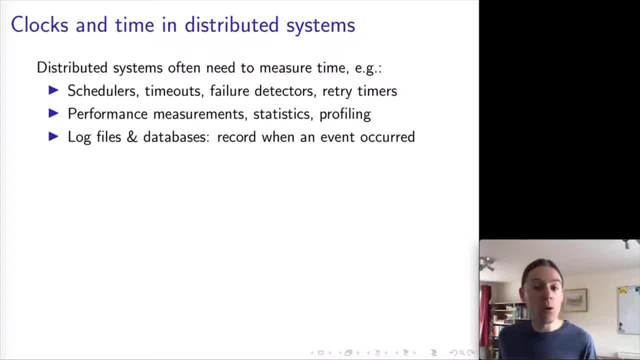 to improve its performance. that also relies on time measurement. In log files you probably want to record the date and time at which a certain event happened. So, for example, a certain user logged in at a certain date, at a certain time. you want to record that in the log. 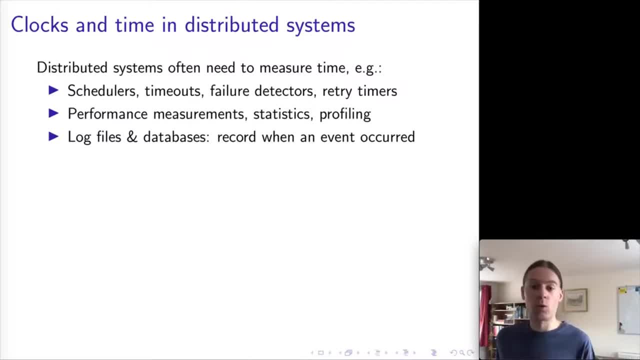 In databases you might want to record when something happened. So at which point did a user make a purchase, For example, what date, at what time did that purchase occur? An interesting one is data that is only valid for a certain period of time. So in a cache, for example, you might want. 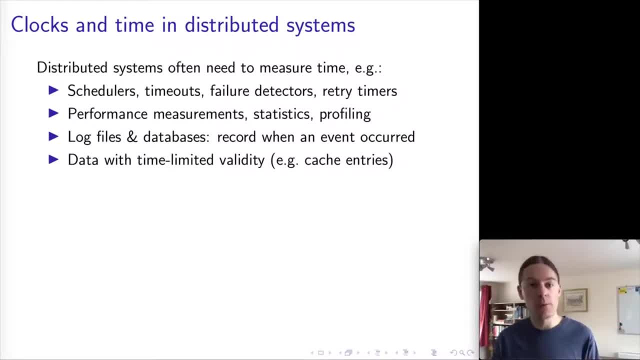 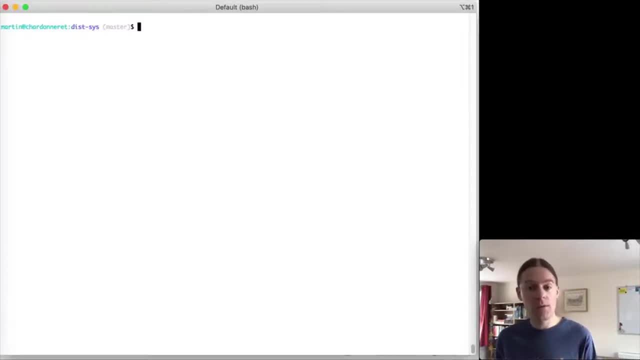 data in the cache not to live forever but to be expired from the cache after it has been there for a while. So I'll give one concrete example of this. we could use DNS, So the DNS system for resolving domain names to IP addresses we can query. So we can do something like this: I'm going to query the. 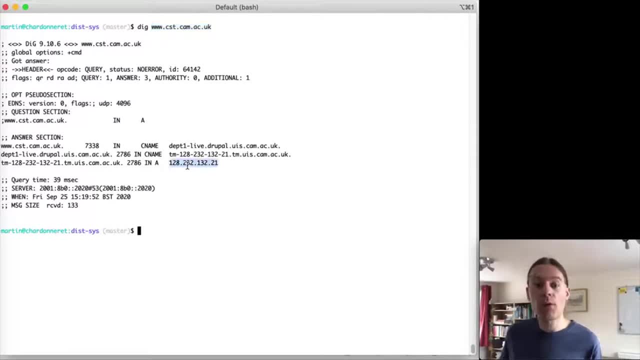 computer lab website here and it's going to give me back the IP address of that website. And if you look at this answer here, you can see in the second column there are these numbers and these numbers are the time to live in seconds of these records. So what this means is that you 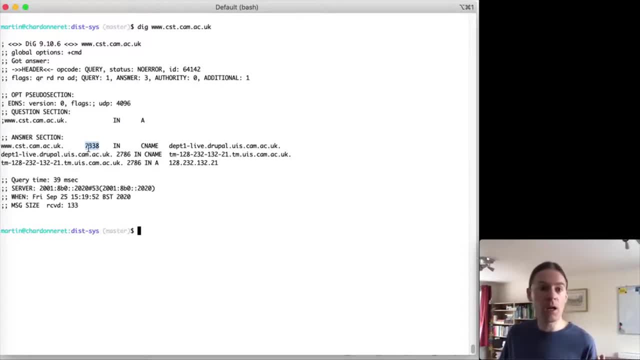 are allowed to cache the results of this DNS query for a certain period of time. Here's 7,000 seconds, so that's about two hours or something like that. The results are allowed to be cached, But then, after that time has elapsed, then we need to refresh the query. 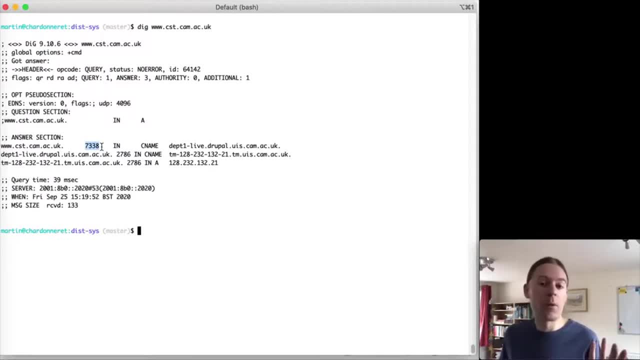 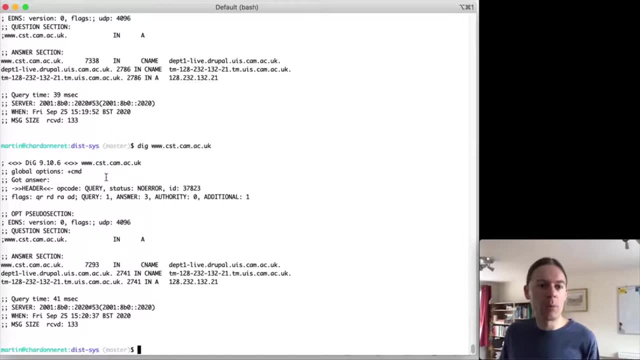 we need to re-run the query in order to get fresh data, So that if somebody wants to change the DNS record, then it will eventually propagate to everywhere. I can now actually re-run this a couple of seconds later and see that now 7,338 has gone down to 7,293, because that number of 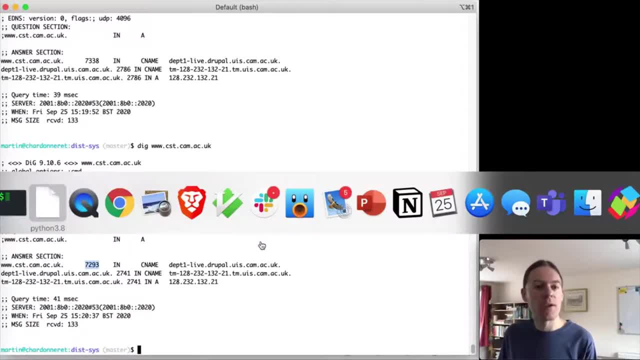 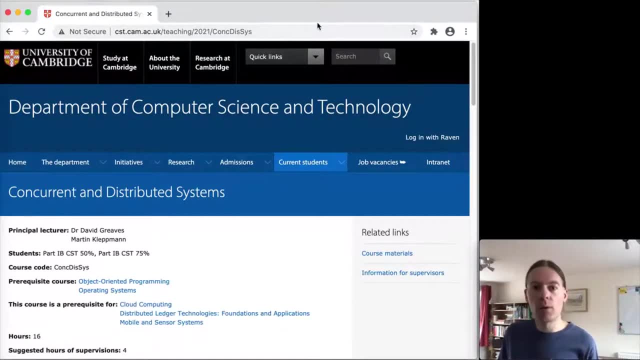 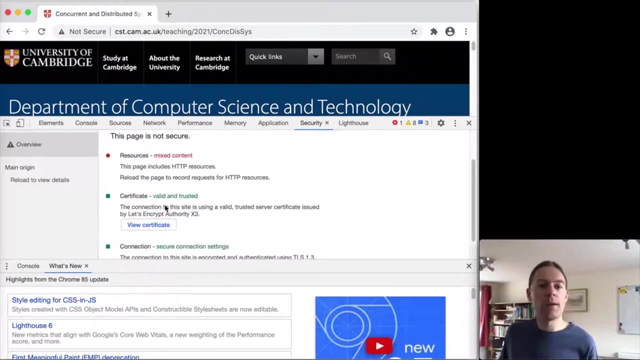 has elapsed while I was talking right now. Another interesting example of where time measurements happen is on a website. So let's say, here I have the Computer Lab website again and I'm connected to it via HTTPS, which means that it has here a certificate, so a TLS certificate. 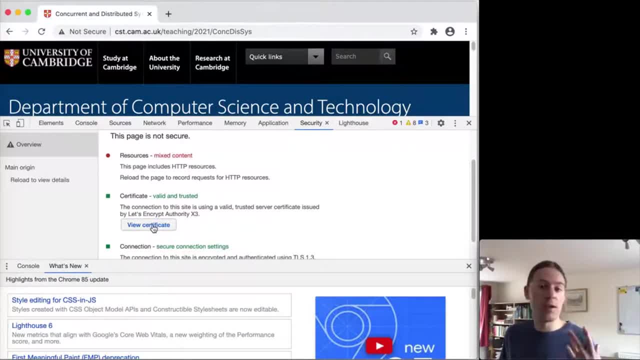 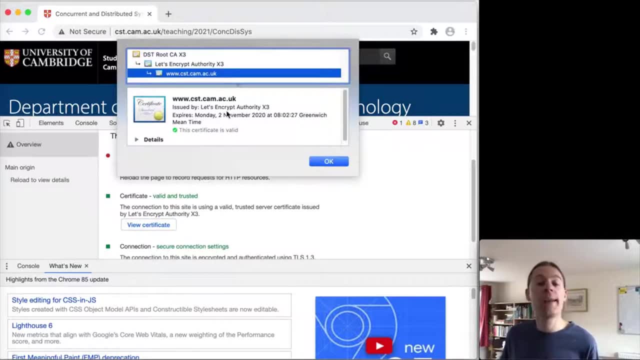 which is used as a mechanism to check that we're actually talking to the correct server, not to some fake server that is trying to impersonate this website. And if I view this certificate well again, a certificate is valid only for a certain period of time, So it has. 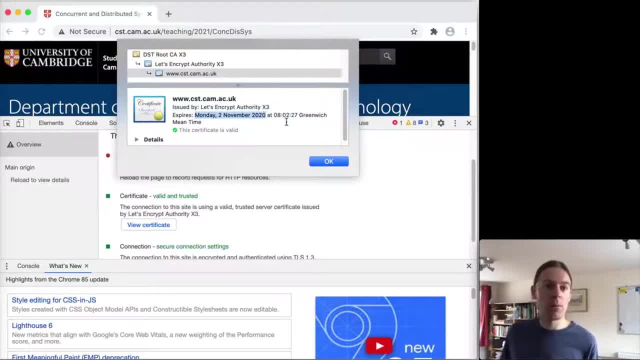 an expiry date here, So this certificate expires on the 2nd of November 2020.. I'm recording this video here at the end of September 2020.. So, at the time when I'm speaking here, the certificate has got just over a month still left before it expires, And so it will get. 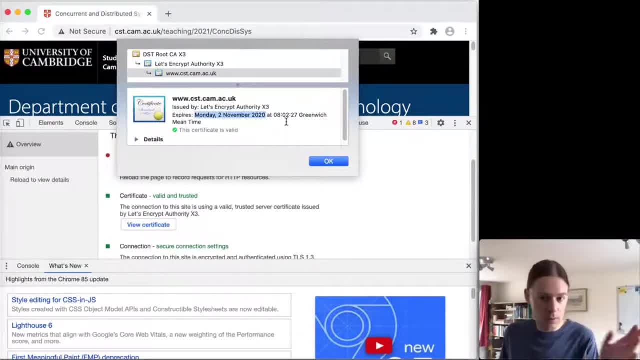 renewed from time to time, every couple of months, so that it keeps being fresh. But here again, this requires, in order for my computer to check whether the certificate is valid, my computer needs to know what the current date is, because otherwise the computer won't be able. 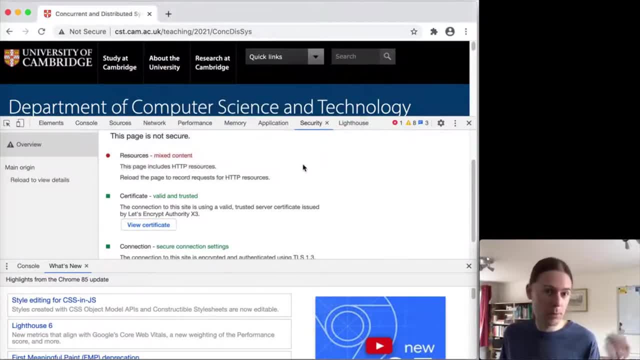 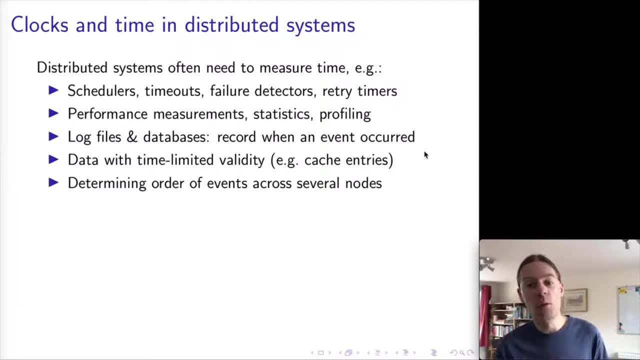 to tell are we within the validity period of this certificate or not. So that's another interesting use of time. And then, finally, we use time measurements in order to determine, in a distributed system, in which order certain events occurred, And we'll talk about that more. 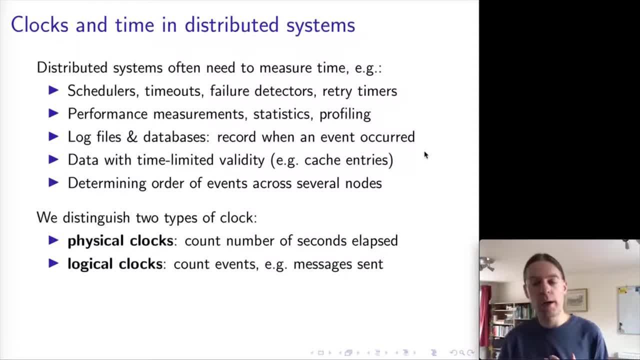 later in this lecture. So there are two types of clock we encounter in distributed systems and we distinguish them as called physical and logical clocks. Physical clocks are the type of clocks that you know from everyday usage. They count the number of seconds that have elapsed, They tell you what time of day it is and what date it is. 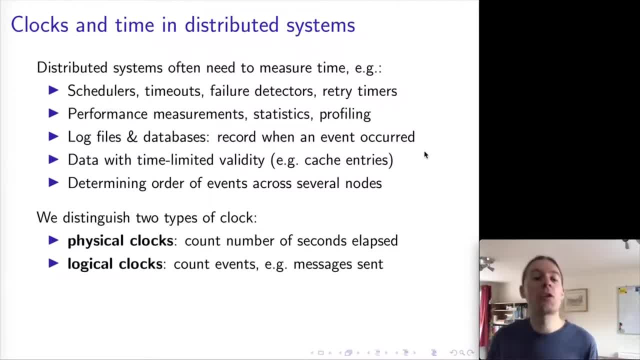 And that's the type of clock that we're talking about in this lecture. Logical clocks I will come to in the next lecture. Now just a little terminology clarification. The term clock is also used in digital electronics and you've come across it there where it means a 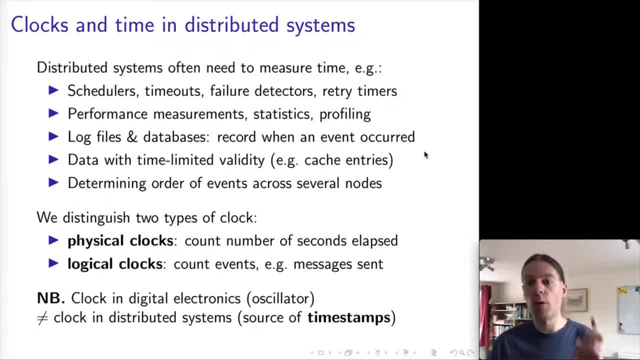 a signal which produces pulses of ones and zeros at a certain regular frequency. In distributed systems we use the word clock in a slightly different way. So the meaning in distributed systems is: a clock is something that you can ask for a timestamp, So it tells you what the 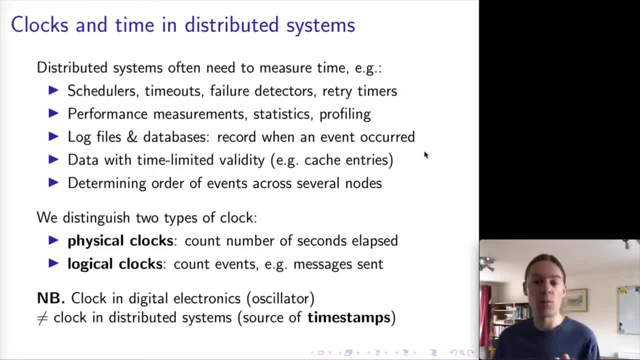 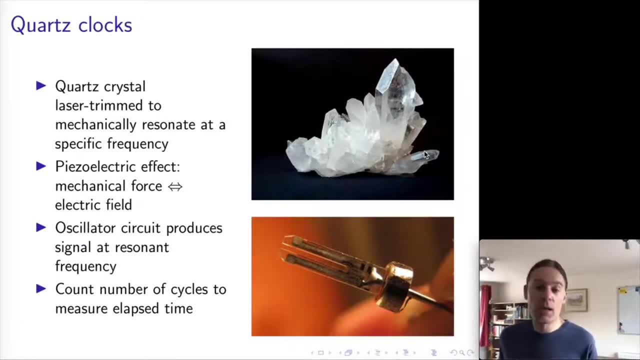 current time is, and the current time is represented as a timestamp, which might be the current date and time. So the way that most computers implement clocks nowadays is using quartz crystals. So this is literally a piece of quartz, typically not a natural quartz crystal. 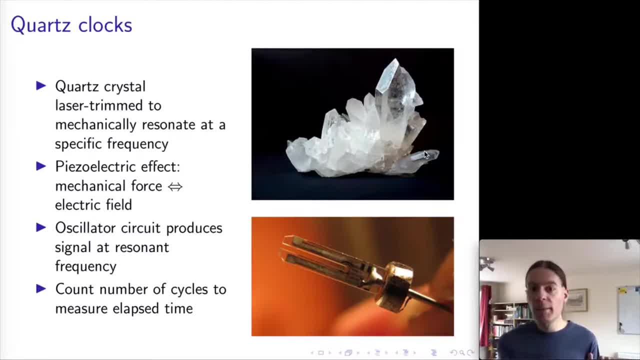 but an artificially grown one. but it's still silicon dioxide And it's cut to a certain size and into a certain shape using lasers And it then mechanically vibrates. So it mechanically resonates at a certain frequency, and the frequency at which it resonates can be tuned. 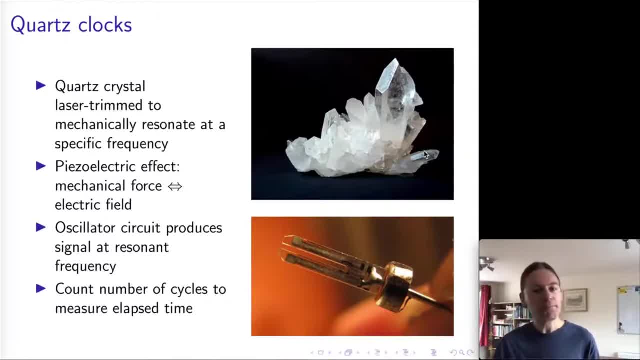 by cutting off bits of the crystal using lasers. Now, quartz is also a piezoelectric material, which means that if you apply an electric field to it, it induces a mechanical strain in the material. And also the other way: if you apply a force to it, then it creates an electric field. 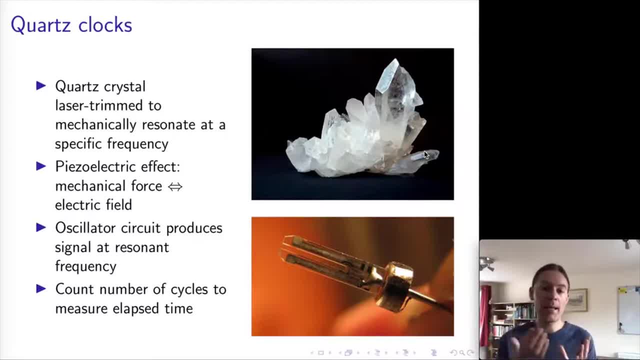 And so you can have, you can use this interplay between the mechanical motion and the electric field in order to create a fairly accurate oscillator that resonates at a fairly accurate frequency. So there's a little bit of electronics around the quartz crystal, but essentially it. 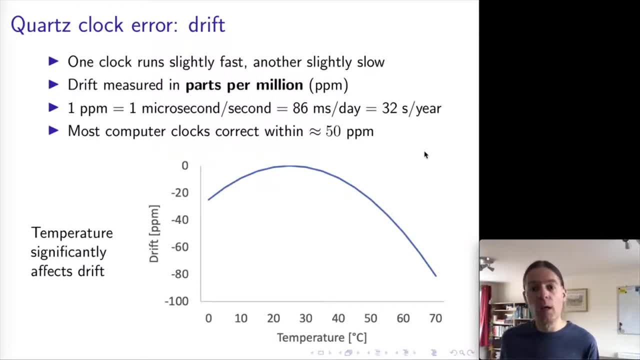 is a signal with a certain fixed frequency. Now, this frequency is quite predictable, and this makes quartz clocks quite accurate. but they're certainly not perfect, because there are always going to be certain manufacturing differences between one crystal and another. They won't oscillate at. 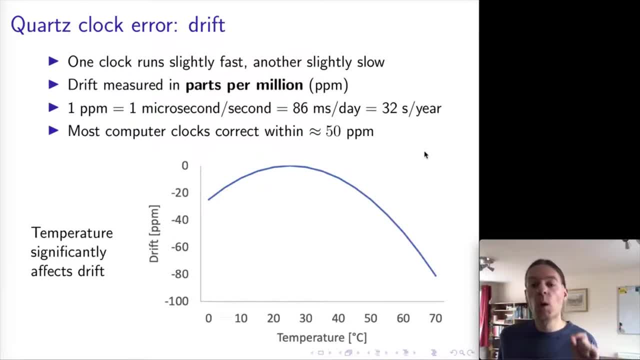 precisely the same frequency. There will be a little bit of an error. Moreover, the resonant frequency of a quartz crystal actually depends on the temperature, And so the crystals that are used for quartz oscillators are tuned, and they're selected and created in such a way that they are 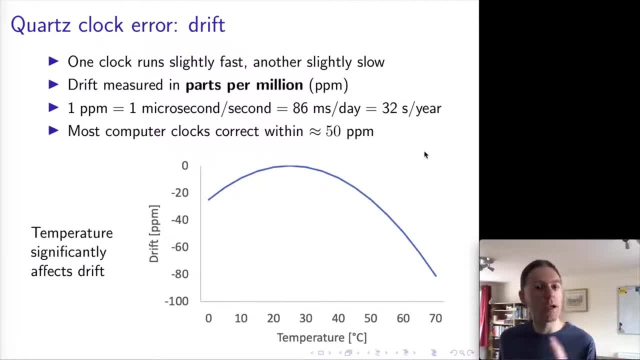 their frequency is quite stable around room temperature, around 20 to 25 degrees C. But as you deviate from this temperature significantly, there's actually a quadratic decrease in the clock speed, And so if you, if you're in a very hot server room, for example, 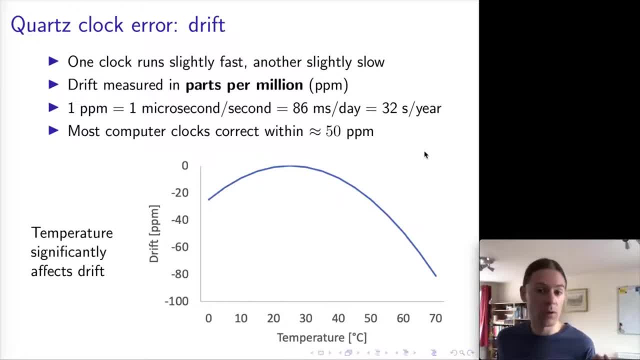 where you know you might reach significantly higher temperatures than your typical room temperature, then this actually can have a significant impact On on the frequency at which the clock is running. So the clock speed is measured in parts per million. Usually this is just like percent, but rather than dividing by a hundred, we divide. 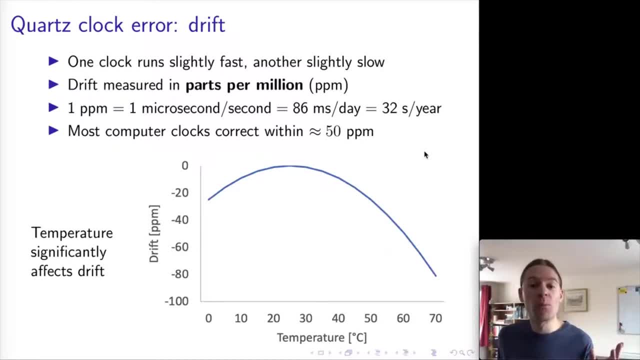 by a million, And so you can work out like if you have a one PPM error, that would mean that the clock goes wrong by about 32 seconds per year. Now most quartz clocks will be like maybe 20 PPM or something like that Order of magnitude, of course, depending on the temperature. 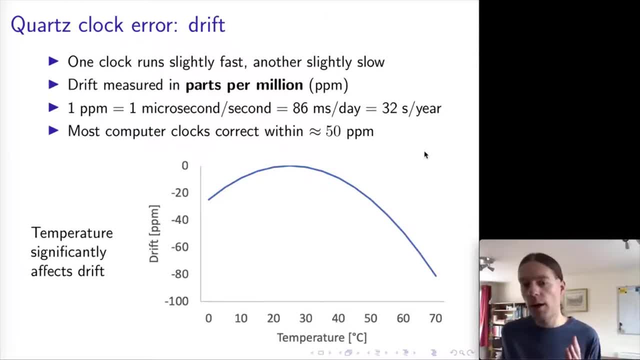 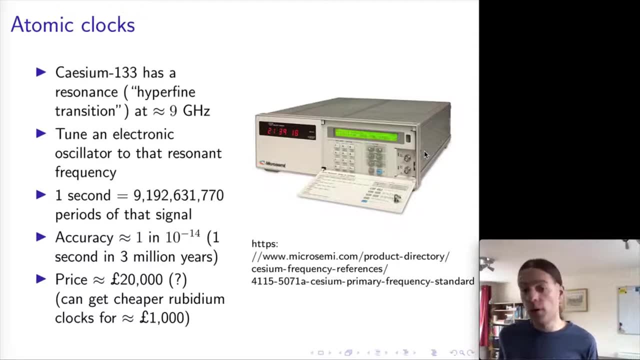 As a rule of thumb, probably most clock errors will be below 50 PPM. Now, if that is not accurate for you- not not accurate enough for you- you can use an atomic clock. Atomic clocks are much, much, much more accurate and they are based on quantum mechanical. 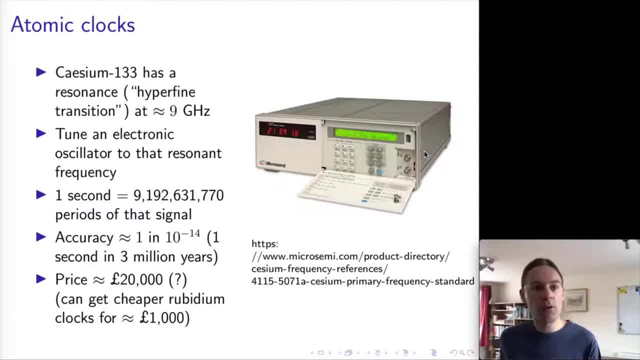 effects. So they actually use cesium atoms, of a certain isotope of cesium, And they, if you remember any quantum mechanics atoms have discrete energy levels. The difference between those energy levels corresponds to certain resistances. So if you have a quantum mechanical effect you can. 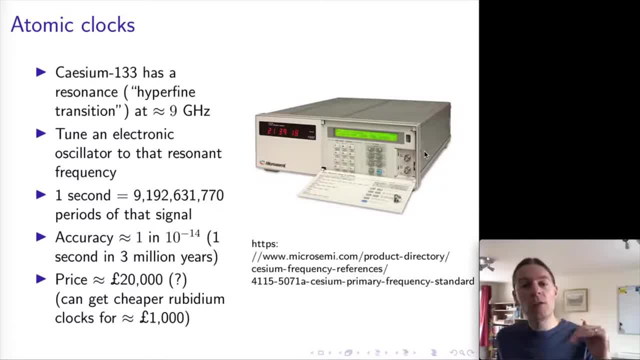 use these and you can measure the resonant frequencies of the atom. And there's one particular energy transition which is fairly friendly to measure, a frequency of about nine gigahertz. So you get about nine oscillations of this per second And this is actually how the second 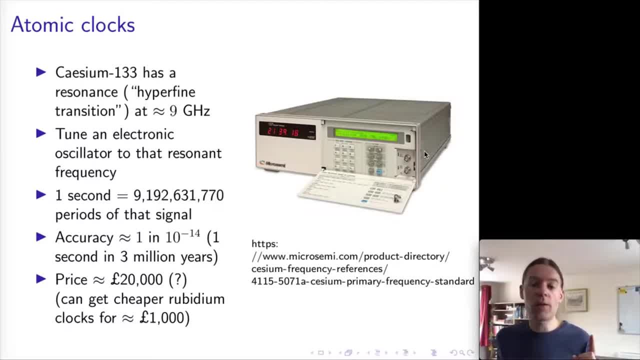 is now defined. So the SI unit of one second is defined to be exactly nine billion 192 million blah blah Periods of this particular signal generated from this particular resonant frequency of this atom. Yeah, Let's just try it. 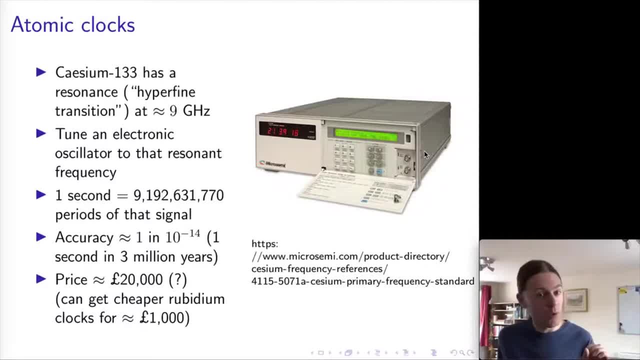 Okay, Uh okay. cesium atoms. Now this is incredibly precise. Of course, the clocks are not that cheap, but you can just buy a clock off the shelf if you have the money. I'm not entirely sure exactly how much they cost, but these were sort of the best estimates I was able to get off the internet. 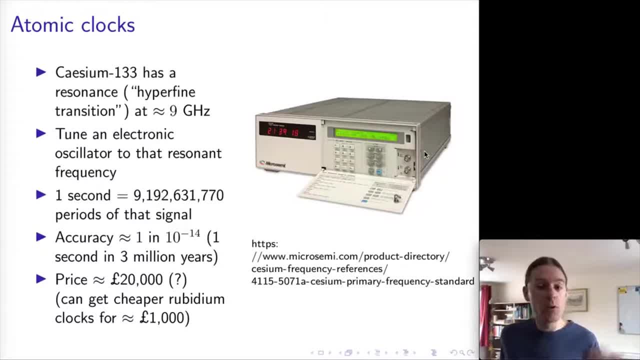 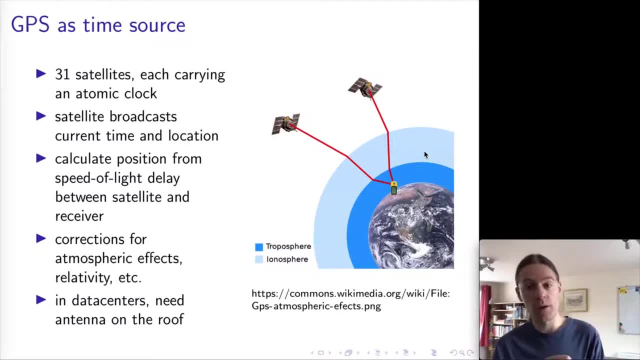 And well, if you have an atomic clock, you can do some interesting things with it, Like you can build GPS, for example. So if you want a very precise clock signal, one way of getting that clock is actually to use GPS, So the same system that you use on your smartphone to tell you where. 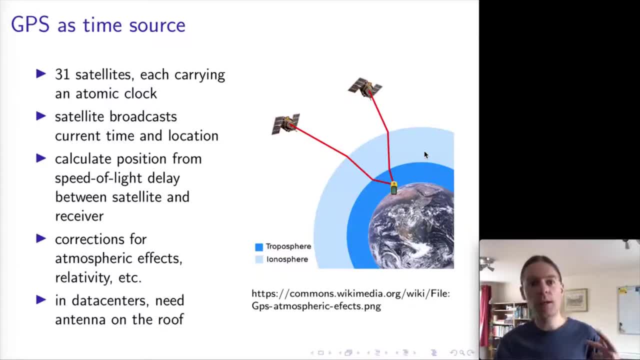 you are right now on a map. It works by having a bunch of satellites that orbit the Earth, and each satellite carries an atomic clock that broadcasts its current clock and its current location periodically, And so the GPS receiver it receives the signals from several of these. satellites. It calculates the time difference between when the signal was sent by the satellite and when the signal was received By your phone, And from that time, distance and the speed of light it can work out the actual distance in space between you and the satellite And from that it can work out where you are. 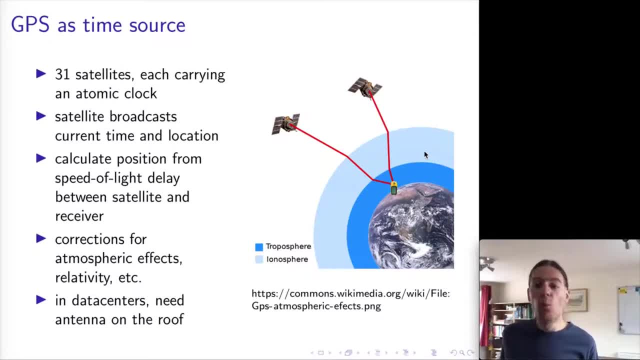 Now, there's a lot of details that go into making this accurate, but for our purposes, all we're actually interested in right now is time, not location, And you can use GPS satellites as a very accurate way of getting time and clocks. Now, this does rely on being able to actually pick. 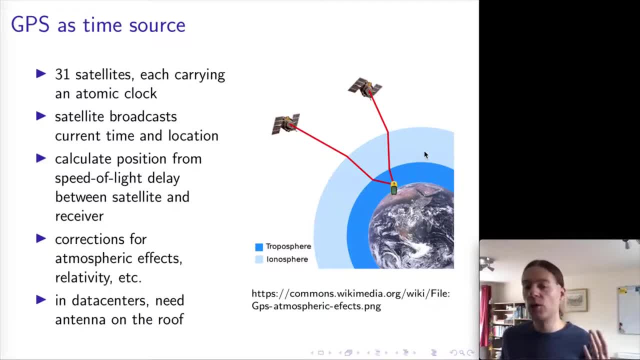 up the signal from the satellite, but it's also a very accurate way of getting time and clocks. So if you're in a data center, there's probably so much shielding and electromagnetic interference that you can't actually pick up the signal, so you have to put an antenna on the roof of the data. 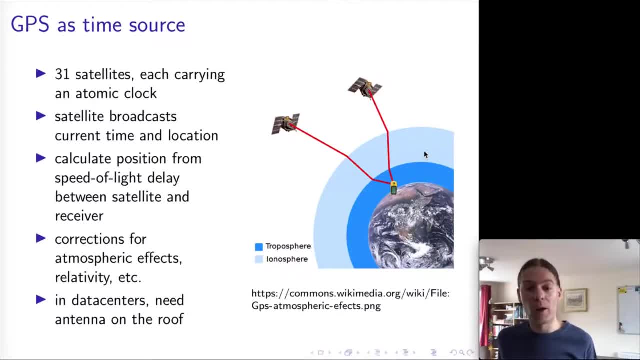 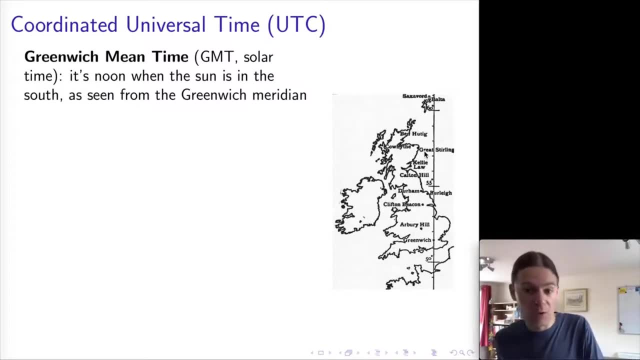 center, But this is something that people actually do as a way of getting accurate clocks. So so much about how clocks actually work. Now, how is time defined? So you might have come across the term UTC, the coordinated universal time, which is the reference time that is used for all of our time zones we use nowadays. So you might have come across the term UTC, the coordinated universal time, which is the reference time that is used for all of our time zones we use nowadays. So you might have come across the term UTC, the coordinated universal time, which is the reference time that is used for all of our time zones we use nowadays. 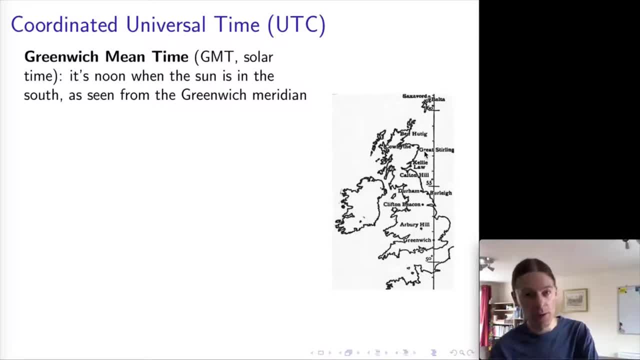 How is UTC actually defined? We have to be precise about this, And so you've probably come across the term GMT- Greenwich Mean Time, which unfortunately, the meaning of that has changed over time. Its original meaning was time based on astronomical observations, So 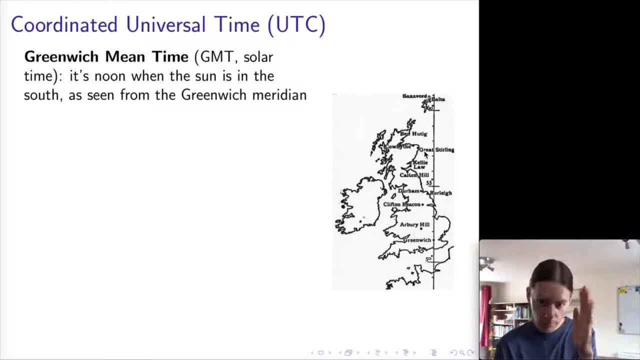 it was literally: when does the sun? when is the sun in the south, if you are looking at the sun from the Greenwich Observatory? So you can literally go to Greenwich in southeast London and visit the observatory there and see the meridian at which the sun is located. So you can literally go to Greenwich in southeast London and visit the observatory there and see the meridian at which the sun is located. So you can literally go to Greenwich in southeast London and visit the observatory there and see the meridian at which the sun is located. 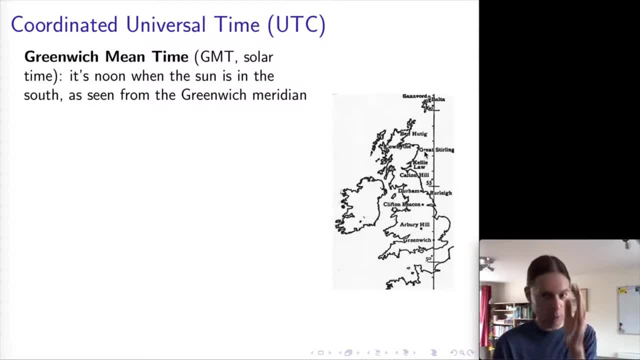 It was defined that when the sun is in the south, as seen from this particular place, then it is noon. Now the time varies a little bit over the course of the year, so that way we actually average this over the course of the year. But the idea is still. this is time based. 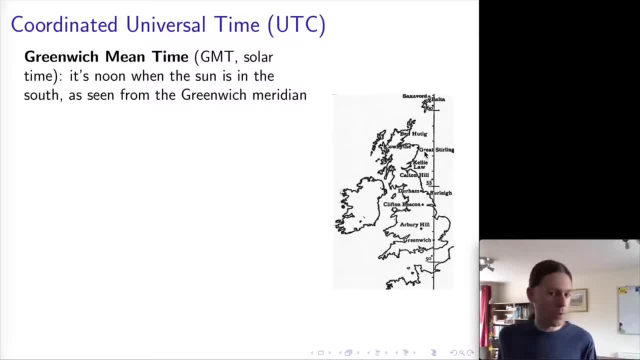 on astronomical observations. Now, I just said atomic clocks. they define time using cesium atoms, so using quantum mechanics, And so this is now actually how time is defined. The International Atomic Time is. let's take atomic clocks. we take a couple of hundred atomic clocks spread around the 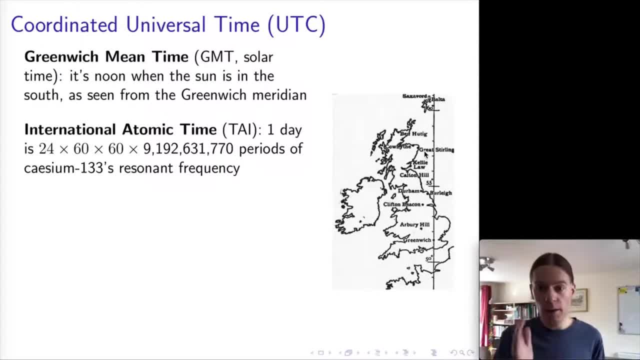 world. we synchronize those and we count exactly the number of oscillations we have from this cesium resonant frequency, and that tells us how many seconds have elapsed. Now these two things don't, unfortunately, match up exactly, So we have two different definitions of time, one based on 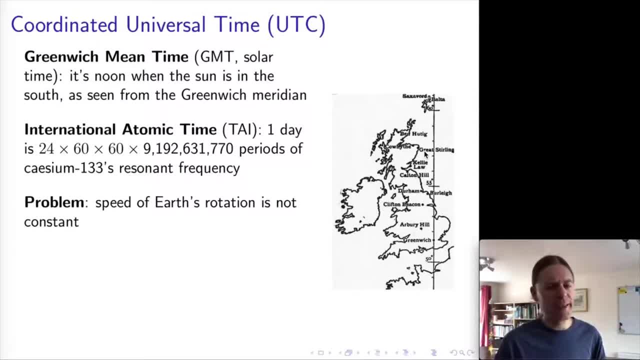 astronomy, the other based on quantum mechanics, and these two things don't exactly match up. They're pretty close. But especially the observations based on astronomy are problematic because the speed of the rotation is not actually entirely constant, Just actually the Earth wobbles a little bit and sometimes it. 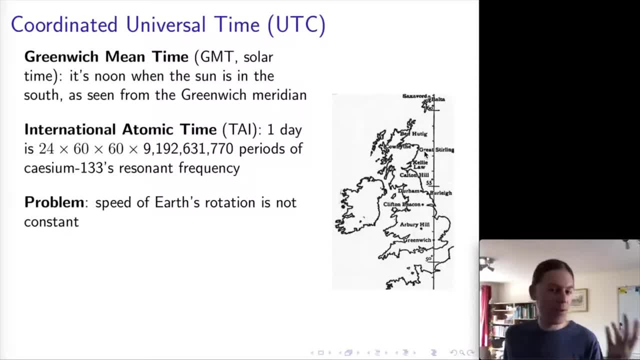 turns a little bit faster, and sometimes it turns a little bit slower, and this is affected by earthquakes and by tides and by all sorts of weird complicated effects. And so the result is that, well, we want to use atomic time, because that's much more precise. 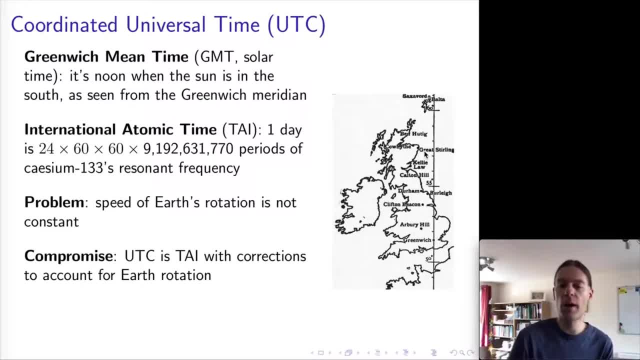 than this wobbly Earth time, But at the same time, we want our time to be consistent with how the Earth rotates around its axis, And so the compromise is UTC. The compromise is: we take atomic time, international atomic time, and we apply some corrections to it based on astronomy. 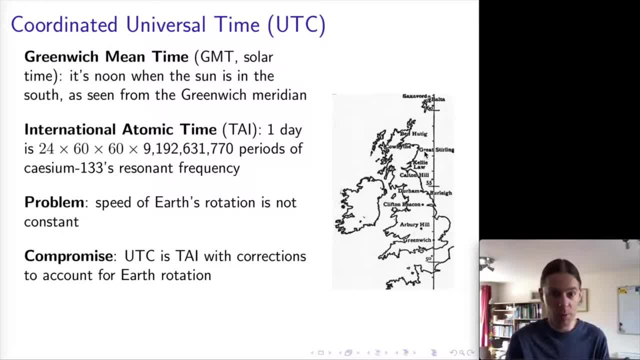 and that will give us a time that is founded on quantum mechanics but still consistent with astronomical observations. It's a bit of a complication, but that's what we've ended up with, And so this is how UTC is defined and time zones and all of. 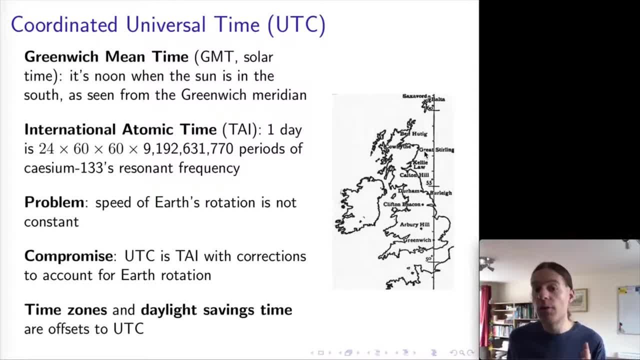 these are defined as offsets to UTC now, And so like if you're on the East Coast US, for example, you'll be in like UTC plus five, for example. Now, how does this correction from atomic time to UTC look like? The answer is: the correction takes. 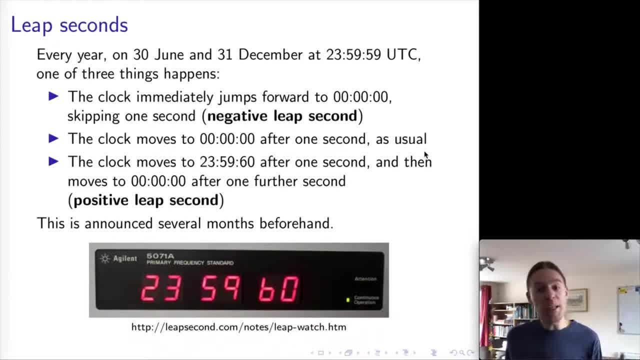 the form of leap seconds. So you've all heard of leap years before. Leap years are a very familiar thing. This is a different concept, but it's similarly weird. It's even more weird actually. And so a leap second is an extra second that can be either inserted or removed on a certain date, And 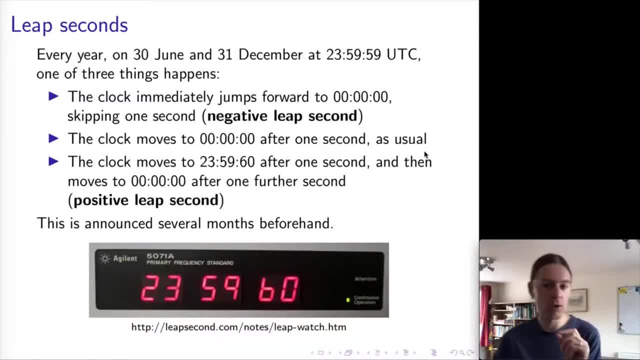 so every year, there are typically two dates on which a leap second may or may not happen, and that is the 30th of June and the 31st of December. In principle, I think it can happen at the end of every month, but these are the two months that are typically used. 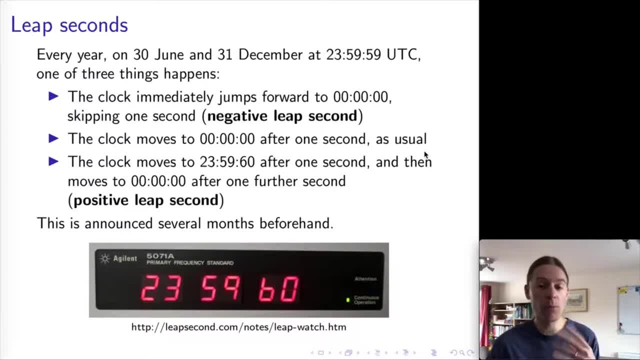 And at that point, a few months before the leap second may or may not happen, astronomers decide: okay, how fast has the earth been rotating for the last couple of months? okay, do we need to insert a second or not, to keep the UTC greatly consistent? 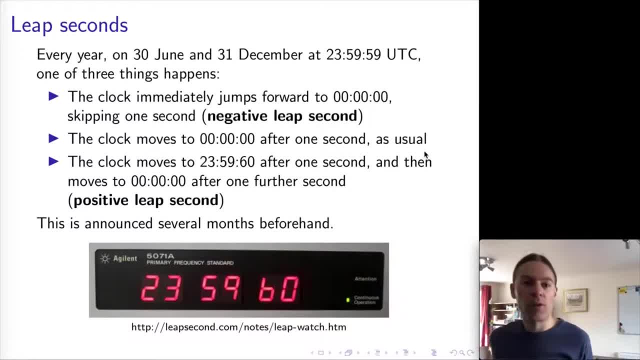 with the rotation of the Earth, And so, depending on what the astronomers decide, then the clock may or may not have an extra second, And so this means actually that if there's a second subtracted, then there is no 23,, 59,, 59 second. The clock goes 58 and then immediately jumps to 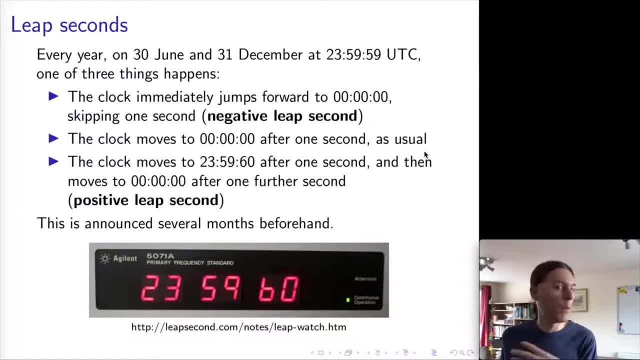 zero after one second. So the 59 second is simply skipped. Or we could have a regular second, or we can have an additional second in which the clock goes from 59, 59 to 60 and then to zero after two seconds. So we've inserted an extra second at 23,, 59 and 60. Now this sounds complicated. 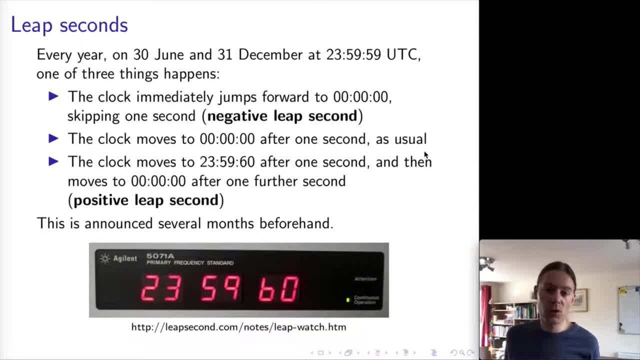 and it is, and unfortunately computers are not very good at dealing with this. So there are two typical reasons for this. One is that the clock goes from 59, 59 to 60 and then to zero after two seconds. The other is that the clock goes from 59, 59 to 60 and then to zero after two seconds. 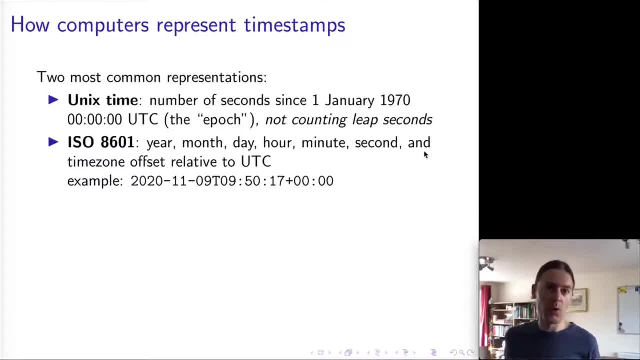 So there are two typical representations of time that are most commonly used in computer programs. Firstly, Unix time, which is simply a number, an integer that counts the number of seconds since an arbitrary point in time. The 1st of January 1970 was arbitrarily picked. 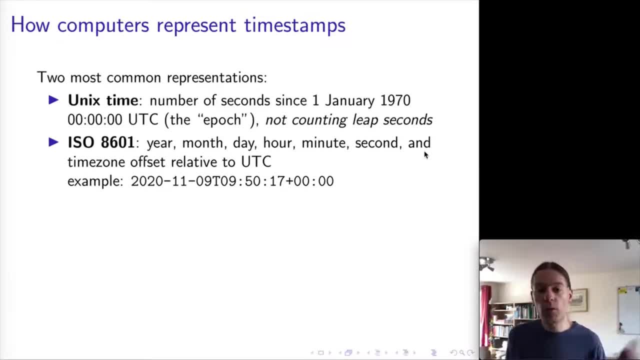 as this is called the Unix epoch, And we count the number of seconds, except that Unix time is defined as not counting the leap seconds, or rather, the standard simply doesn't say anything about leap seconds. It's simply a number of seconds, And so we can count the number of seconds. 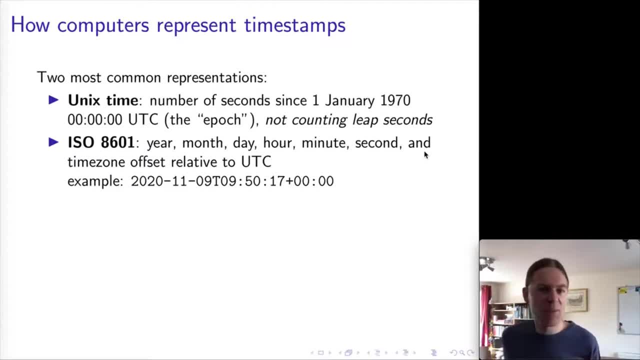 and it's implied that. well, I don't know who cares about leap seconds, whatever, But it is defined in terms of UTC, So it's not actually UTC. it's kind of international atomic time actually, rather than UTC, But everyone says it's UTC. So what is this thing? Also, then there's 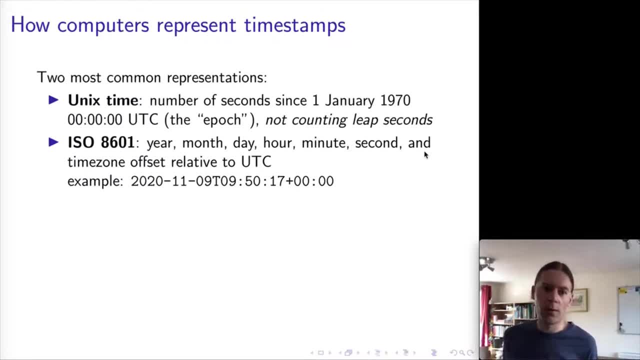 this other format of representing dates and times, which is ISO 8601,, which is based on year, month, day, hour, minute, seconds. This is convenient because it's easy for humans to read, But now it means we have to convert between these two. 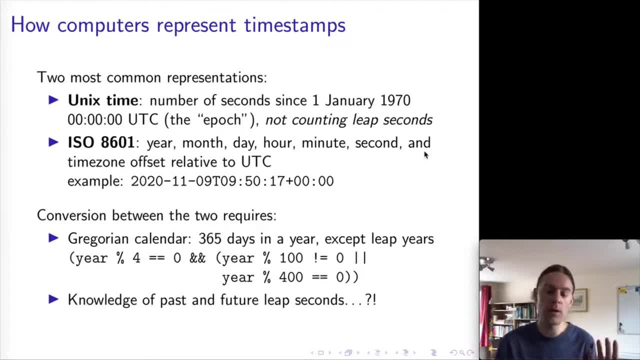 representations. And so conversion firstly needs you to know the calendar. So OK, we know how the Gregorian calendar works. We have 365 days in a year, except we add an extra 29th of February in leap years If the year is divisible by 4, but not if the year is divisible by 100., But if the 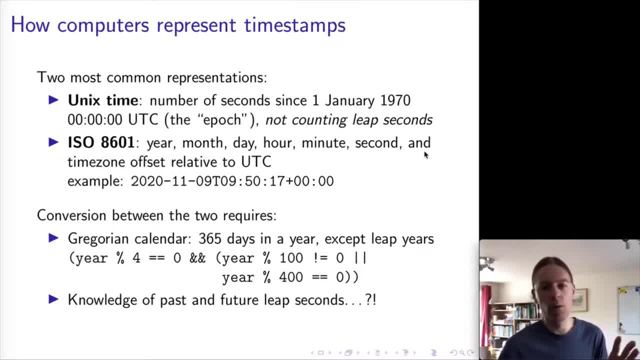 year is divisible by 400, then we do add a leap day after all. OK, fine, So that's our leap years. But then actually, in order to correctly convert these formats, we should also take leap seconds into account, because they also determine the number of seconds that have elapsed since the 1st of 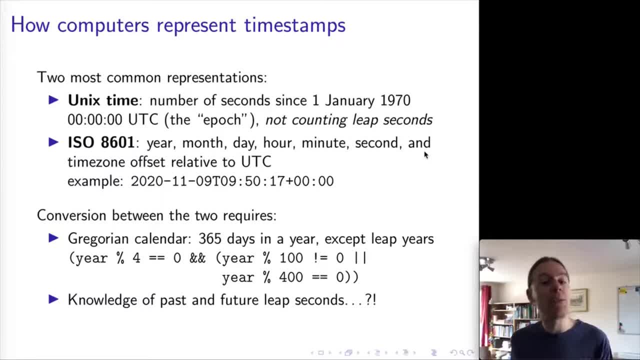 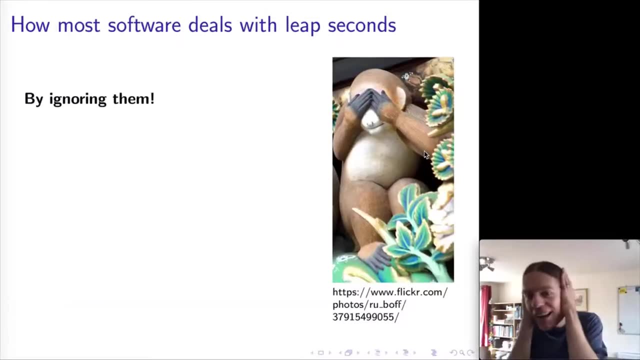 January 1970, because there have been, I think, over 20 leap seconds inserted since that point. Well, how do you think software deals with these problems of leap seconds? You guessed it. Software ignores it. Software goes: la, la, la, la la. there are no leap seconds. 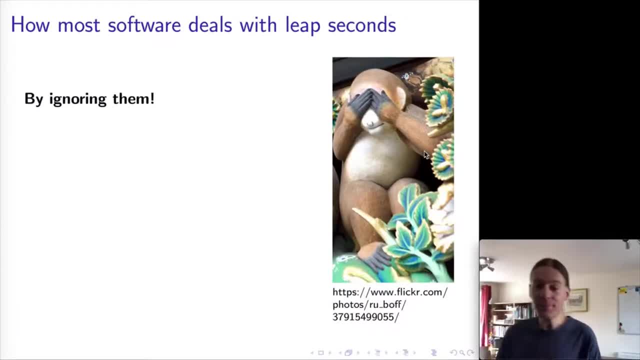 I don't care and just hopes that the problem goes away. Unfortunately, the problem does not go away. And now, of course, some applications. it doesn't really matter because you know one second here or there for many applications really doesn't, doesn't make a big deal of difference. You know, if you 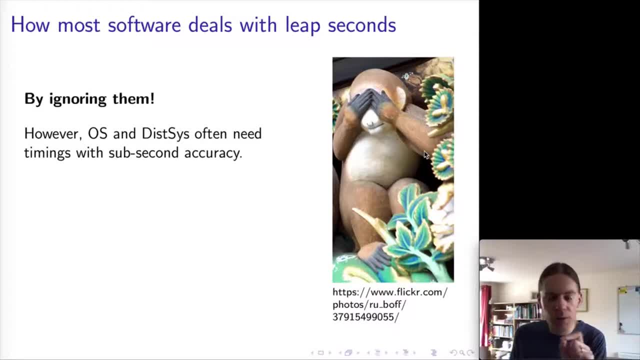 want to have on your Facebook status update at what time you posted the Facebook status update. if that's wrong by a second, nobody's going to care. But in operating systems and distributed systems often we do actually rely on quite accurate time measurements with sub-second accuracy And in 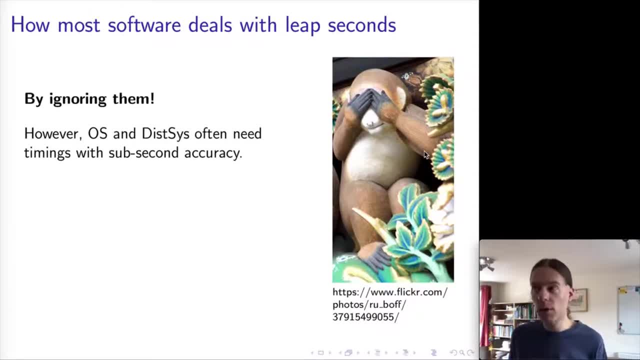 that case, actually, the difference of one second can be rather significant, And that means we do actually have to care about these leap seconds, Which brings us to the solution of the little puzzle that I presented at the beginning of this lecture, which is: what on earth happened on the? 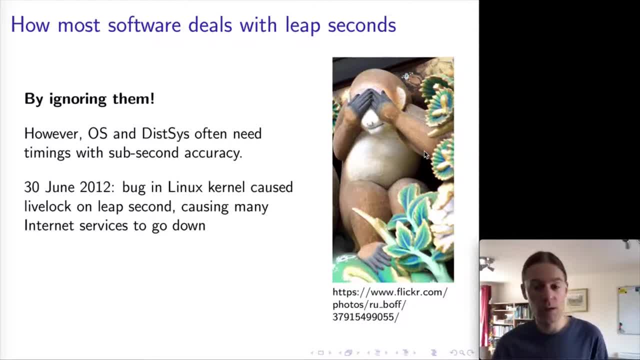 30th of June 2012, for all of these systems to go out down at the same time. Well, the answer was: a leap second happened, And there hadn't been a leap second for a couple of years before that, And so during those years, of course, the Linux kernel and all other software was updated and the 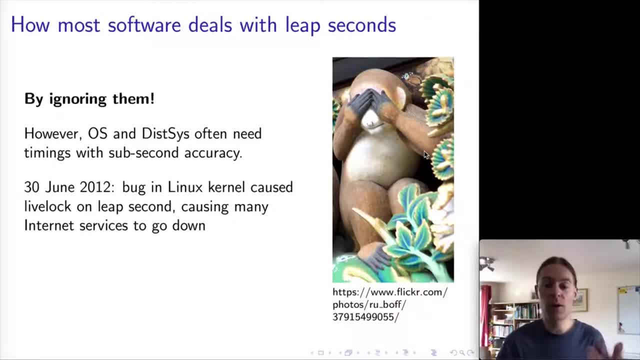 bug was introduced And as a result, there was actually a live lock condition, so that when the leap second happened, the system went into live lock, And so it was just spinning 100% CPU and not getting any useful work done, And even rebooting the computers didn't actually help. 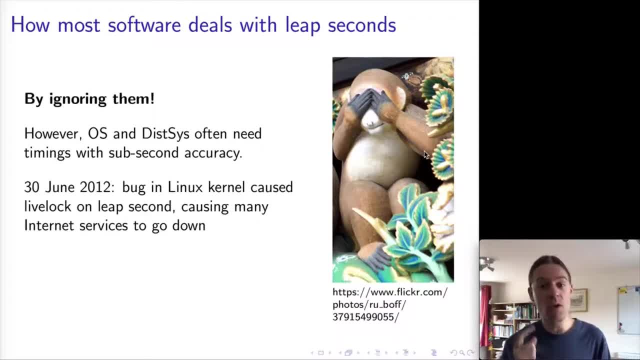 What the administrators figured out then was that you actually had to reset the system clock And that somehow cleared out the bad state in the Linux kernel and allowed us to fix those computers again. But you can imagine that that was a really bad day for administrators of these systems, who rebooted the systems and they still didn't work. 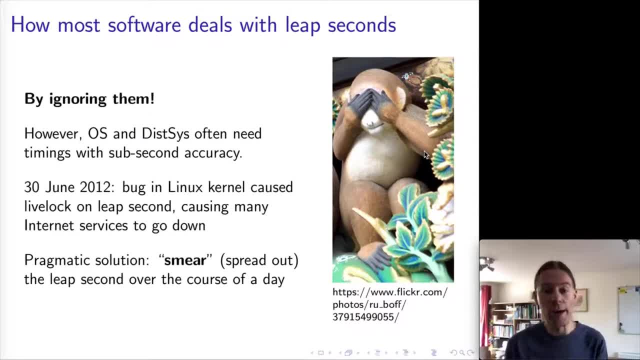 Now a solution is now more widely used which tries to get around this problem that most software does not know how to deal with leap seconds correctly, And the solution is called smearing- leap second smearing, which is rather than if we're going to insert a leap second. 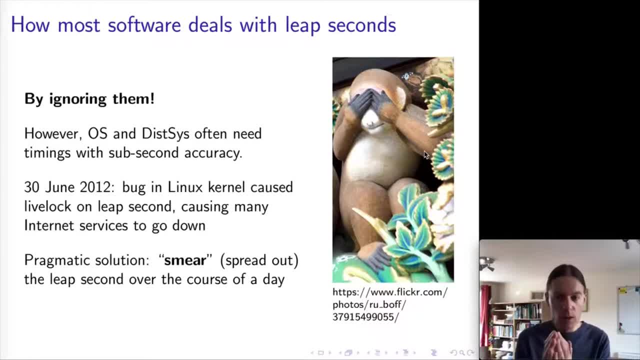 rather than inserting it at one particular moment, how about we just spread that leap second out over the course of a whole day? So let's say, for example, 12 hours before and 12 hours after the leap second is supposed to be introduced? 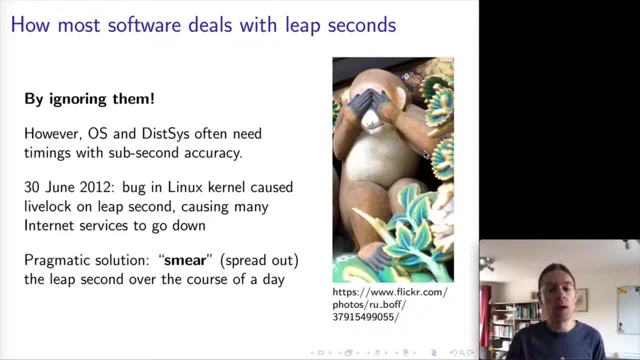 We just slow down the clocks ever so slightly enough, so that then in total, one additional second has elapsed over the course of this period, but without this discontinuity of time where we've added that extra second which confuses all of the software. 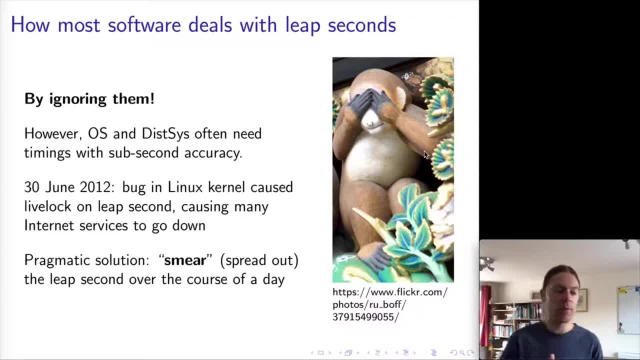 And this is kind of a hack really. It's not a very elegant solution, but it might be pragmatically the best that we can come up with, just given the problem of so much software is out there that doesn't know how to deal with leap seconds and realistically, 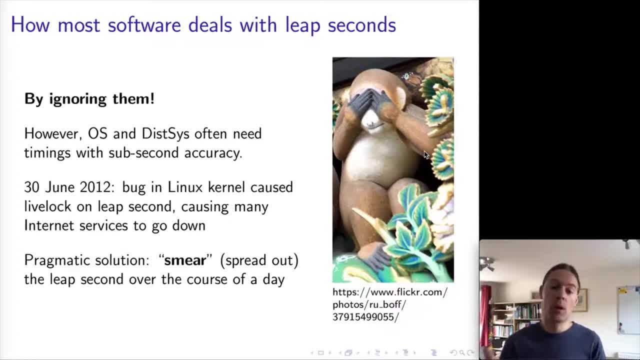 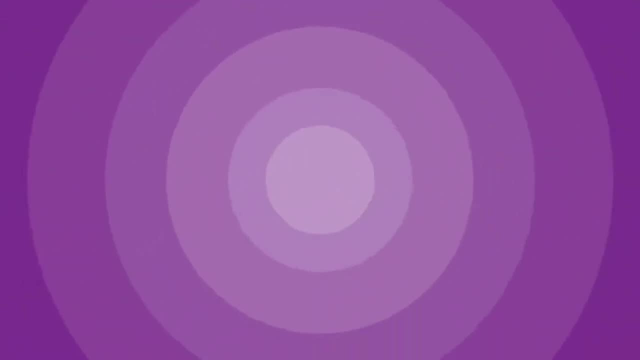 we're not going to manage to update all of that software, So probably this smearing approach is the best we have. But anyway, that is the backstory of leap seconds and why they actually have quite a significant impact on our systems. Next, we're going to talk about clock synchronization. 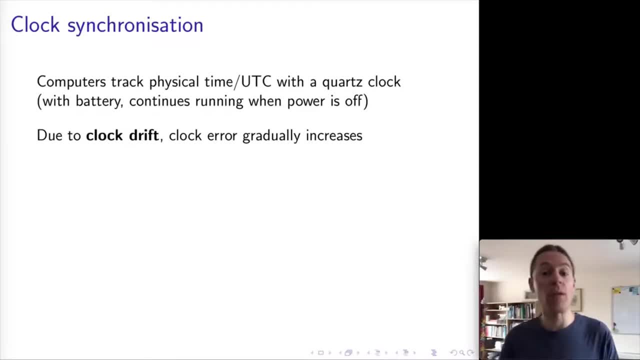 So we've established every computer pretty much contains a quartz clock, not an atomic clock, because atomic clocks are too expensive and too bulky. So what we need to do is make do with these less accurate quartz clocks, and we have to somehow try and make the clocks reasonably accurate. 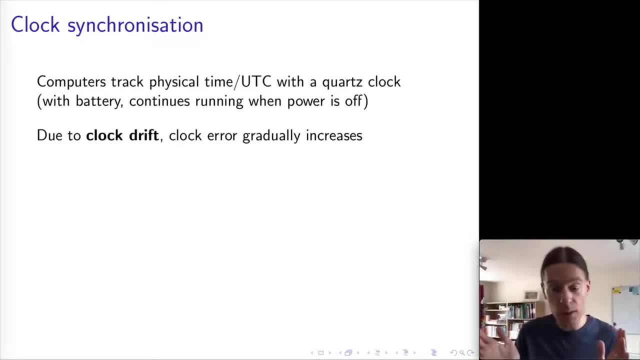 nevertheless. So these quartz clocks will drift a little bit because their rate does not match match up exactly with what the correct clock tick rate should be and we end up with clock skew. So clock skew is if we look at two different clocks at the same instant in time. 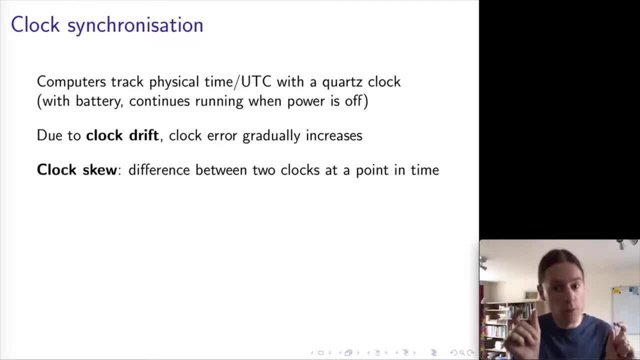 and we compare the timestamps from those clocks. clock skew is the difference between those two And what we want to do with clock synchronization is to minimize the skew as much as possible. Now, in the types of networks that we have, in asynchronous or partially synchronous networks, it is not possible to reduce the clock skew to zero. 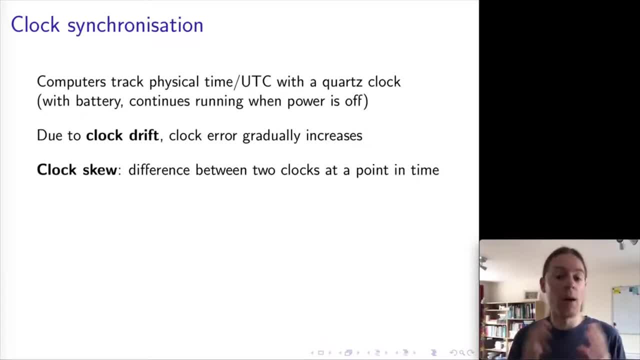 The best we can do is to reduce it as much as we can, but there's always going to be a bit of an error tolerance remaining. Now, the way that we typically do clock synchronization in practice is using a protocol called NTP, the network time protocol. 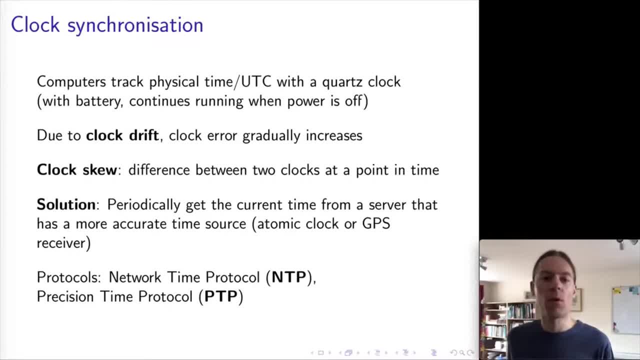 There's also another protocol called PTP, but we won't talk about that in this course, And the way NTP works is that there's a server and we assume the server has some accurate clock source, such as an atomic clock or GPS receiver. 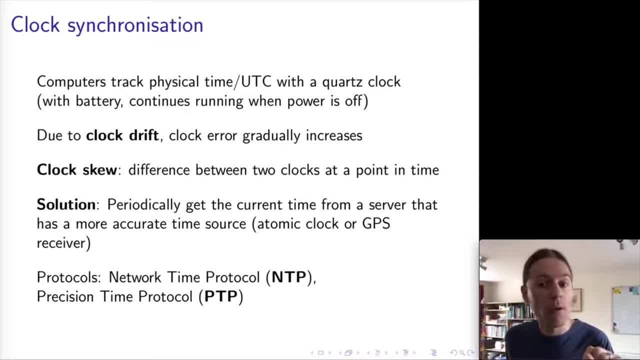 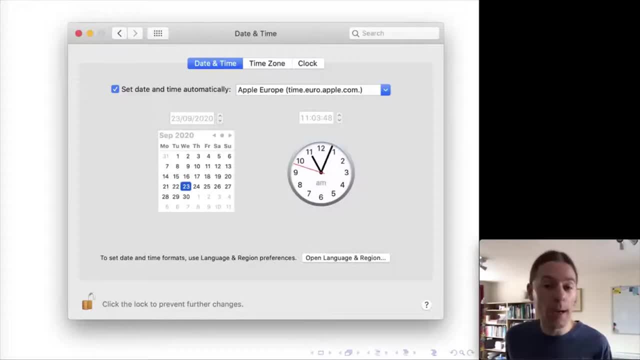 and clients can query the server and ask it for the server's current time, and then the client will adjust its own time based on the time that it got from the server. So NTP is very widely deployed. Almost all operating systems that are used nowadays have NTP built in, so for example, in macOS. 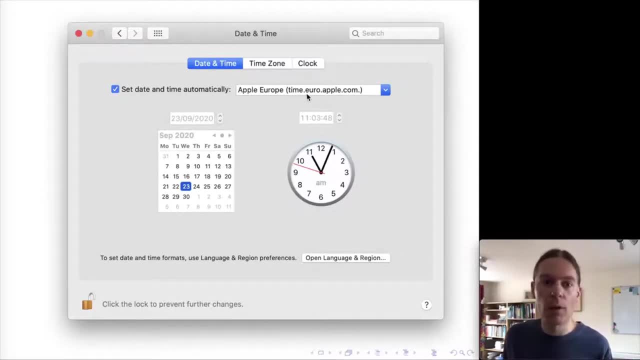 the settings dialog looks like this here. You can choose the NTP server here or type in your own. In this case I've got timeeuroapplecom as my time server, But most other operating systems will have a very similar looking dialog where also you can adjust and choose your NTP server if you want it. 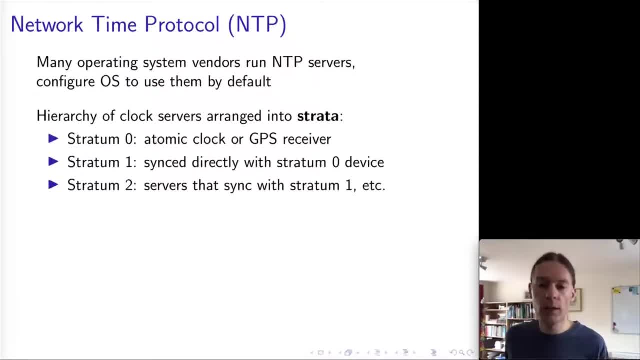 Now, the way that NTP works is that servers are arranged into what are called strata. So stratum 1 is just the accurate time sources, that is, atomic clocks or GPS receivers. Stratum 1 is a server that is connected directly to a stratum 0 time source. 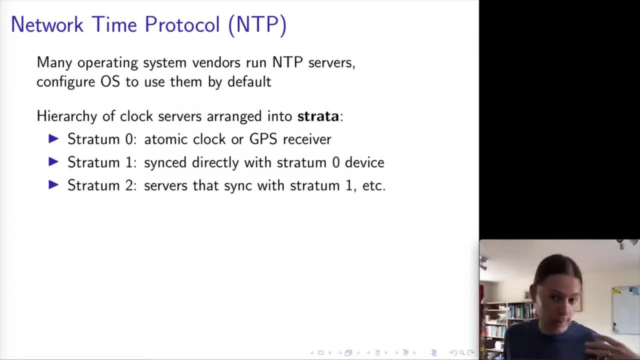 Stratum 2 is a server that is not directly connected to an accurate time source, but which gets its time from a stratum 1 server And stratum 2, stratum 3, gets its clock from a stratum 2 server, and so on. 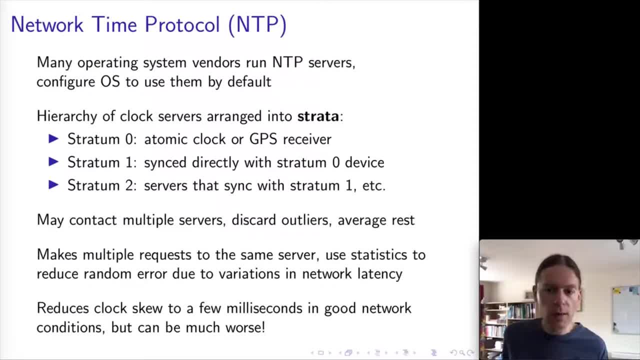 And so there are a whole bunch of statistical techniques and tricks that are used in order to try and improve the quality of our estimates of time. So one thing that NTP does is, for example, to query multiple servers, if they are available, Because it could be that one of those servers is misconfigured or it's got a fault or something. 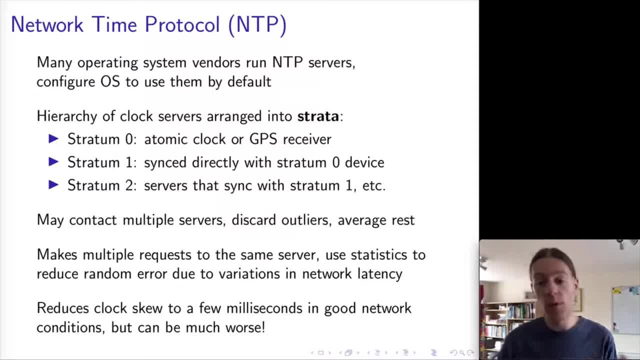 and so it's reporting a wildly inaccurate time. And so if you're querying three servers or five servers, then you can detail. if there's one of the servers which is a real outlier and the other servers are all quite close together, In that case NTP can exclude that outlier. 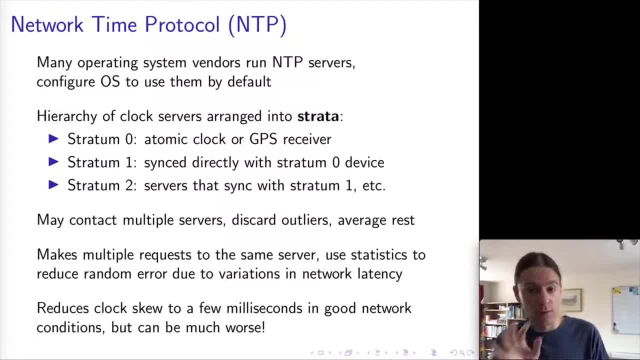 and just keep the data points from the servers that seem to be reliable. Another technique that is used is to query a server not just once, but multiple times over the course of several minutes, And so that will then ensure that at least any random variations in network delay can hopefully get filtered out. 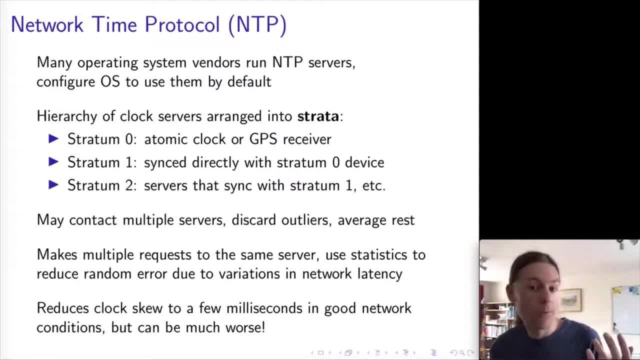 Now, if there are systematic variations in network delay, having multiple samples won't help you, But at least multiple samples will reduce the random error And with NTP, if you have a good quality network connection, it is possible to get your clock synchronized to the server within a couple of milliseconds. 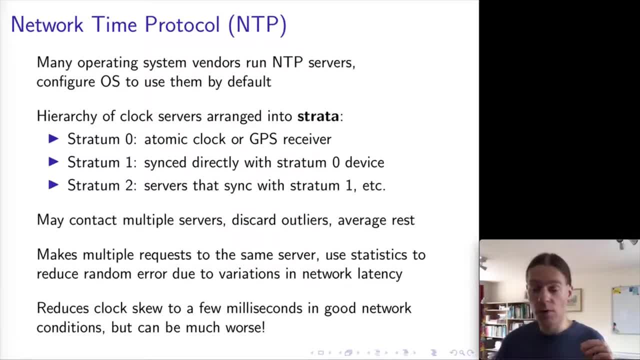 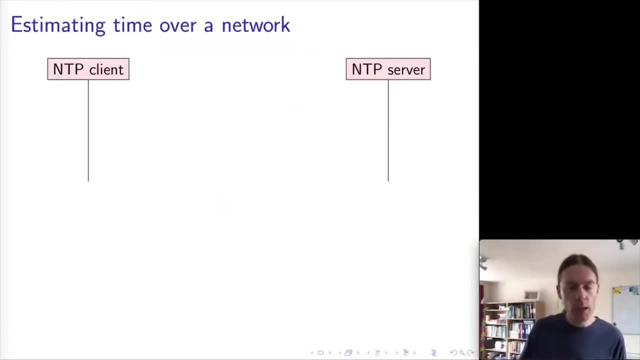 If you are on a poor quality network connection, over some kind of busy Wi-Fi, over a heavily loaded internet connection, then the accuracy could be much, much worse than that. So you always have to be careful when assuming synchronized clocks. Now let's have a look at how NTP estimates the clock skew between the client and the server. 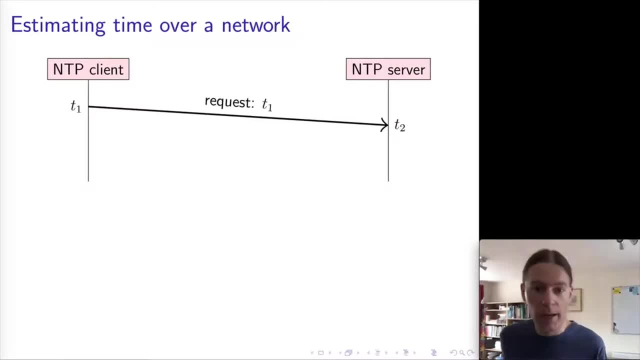 It works by sending a message over a network- again as usual. So we have a request message that gets sent from the client to the server and, as the client is sending this message, it records the clock according to the client's timestamp, the timestamp T1,, which is the timestamp at which the client sent out this message, and it copies that timestamp T1 into the request message. 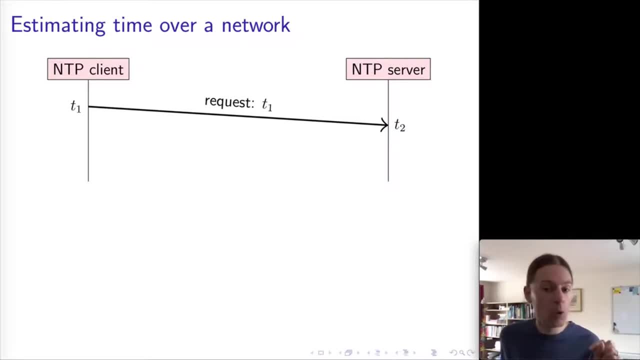 The NTP server. when it receives that message, it will also record the time according to the server's own clock, at which it received that timestamp, and we'll call that T2, at which it sorry- at which it received that message. 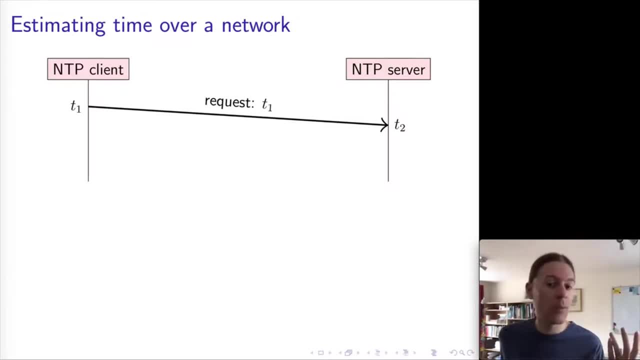 We'll call that T2.. Now the server might take a little bit of time to process the message, but eventually the server will reply. and T3 is the timestamp according to the server's clock at which the response got sent out. So now the response is going to contain all three timestamps so far. so 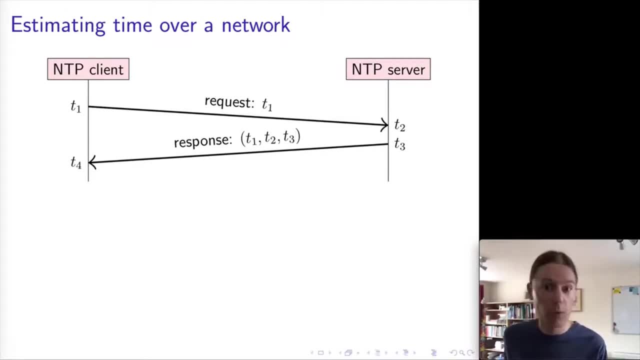 T1 simply gets copied from the request over to the response. The server doesn't do anything with T1.. T2 and T3 came from the server's clock as the arrival time and the response time respectively. And finally, when the response is received by the client, the client again records the timestamp according to the client's clock. 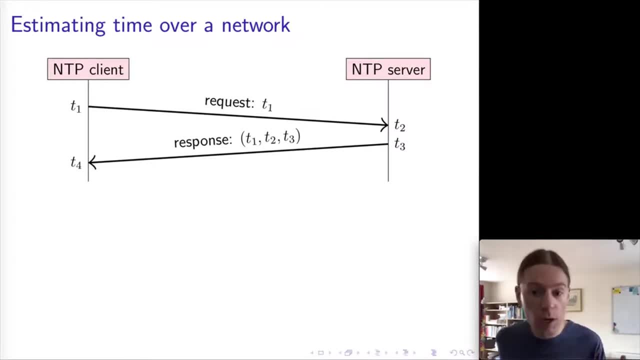 at when that response was received. And so we have now four timestamps and from those timestamps we're going to try to work out what the skew is between the two clocks. So first of all we can work out how long did the message is spent traveling through the network. 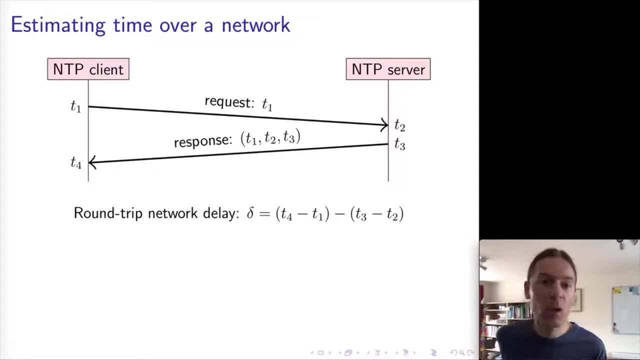 And we're going to call that the total network delay delta, and that time has got to be T4 minus T1, so that is the total time that it spent from the client's point of view, from the time it sent the request to the time it received a response. 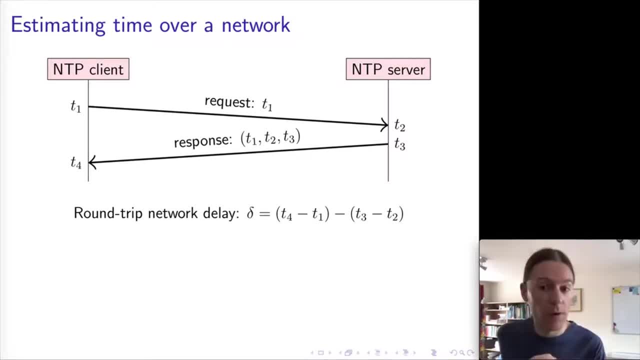 minus the time that the message was spent processing on the server. So minus T3, minus 2, which is the processing time on the server, and the remaining time has got to be then the total time that was spent in the network by the response and the request taken together. 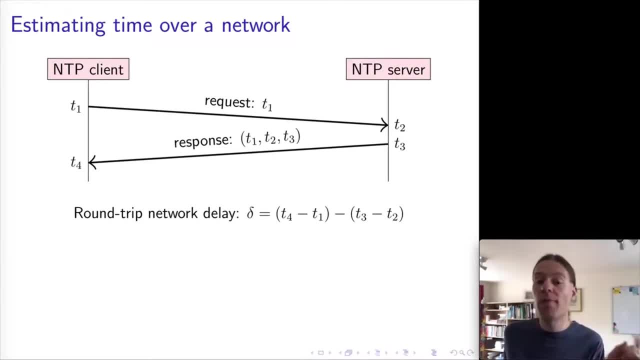 Now what we don't know is the breakdown of those two. how much time did the request spend in the network and how much time did the response spend in the network? If you want to work out that one-way network latency, you need synchronized clocks, And the whole point of this exercise here is that we don't have a synchronized clock. 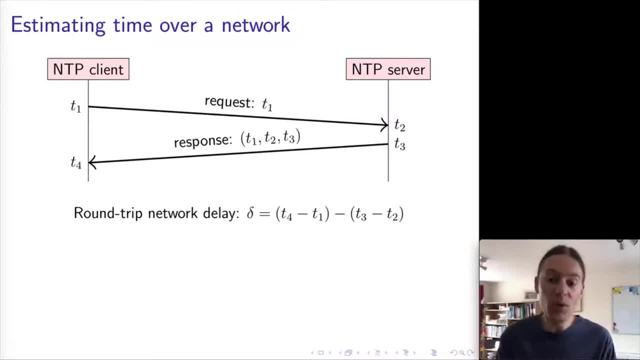 we're trying to build a synchronized clock So we don't have a way of measuring that one-way network latency. We can only measure the time that the response and the request spent in the network are taken together. We can only measure the sum of the two network latencies put together. 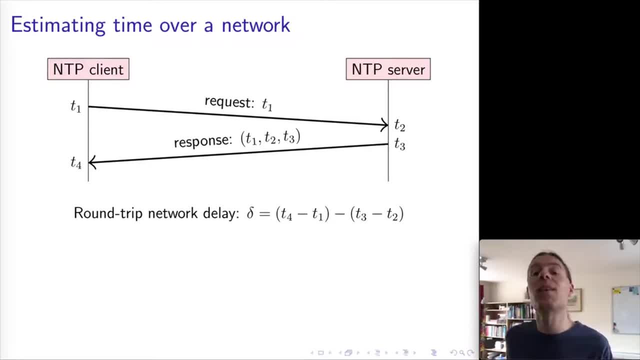 But what we can do is just make an assumption that the network latency is symmetric in both directions. So we're going to assume that the request latency is the same as the response latency, And if this is true, then the response latency will be delta over 2,. 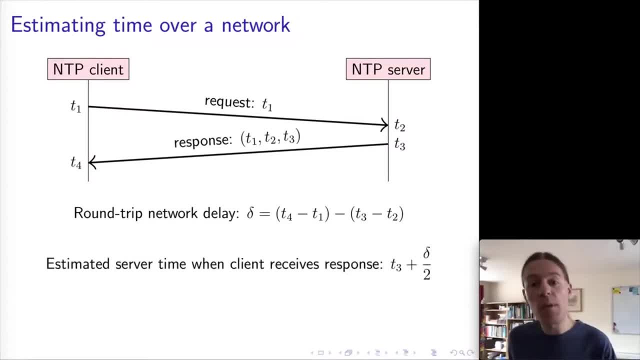 because it's just going to be half the total delay. So this means now we can estimate the timestamp that the server should have at the moment in time when the response latency is the same as the response latency. So we're going to estimate the time that the response is received by the client. 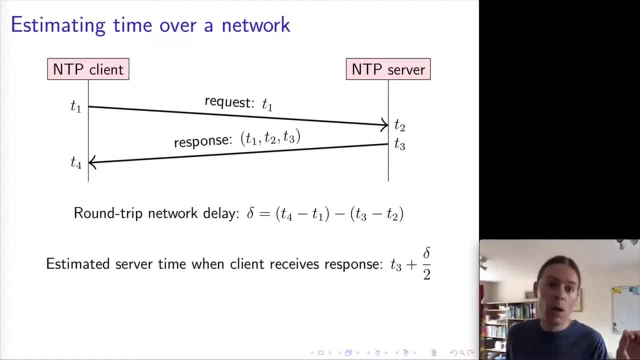 So from the client's point of view, it's time t4. But we know that the server sent its response at t3. And we're going to estimate that the response spent delta over 2 traveling through the network, And so we're going to estimate that at the time when the client receives the response. 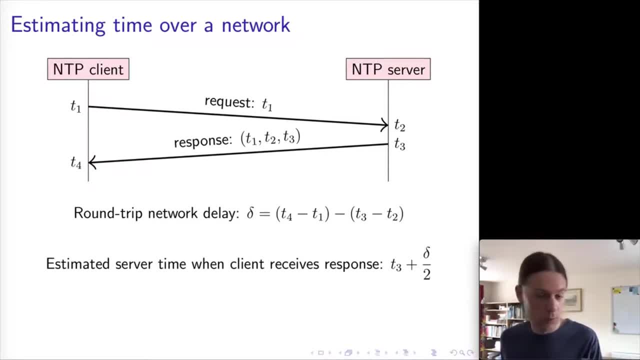 the clock on the server says t3 plus delta over 2.. That's our estimate of the server's clock. Now that we have an estimate of the server's clock, we can estimate the clock's queue, because we can just take our estimate of the clock. 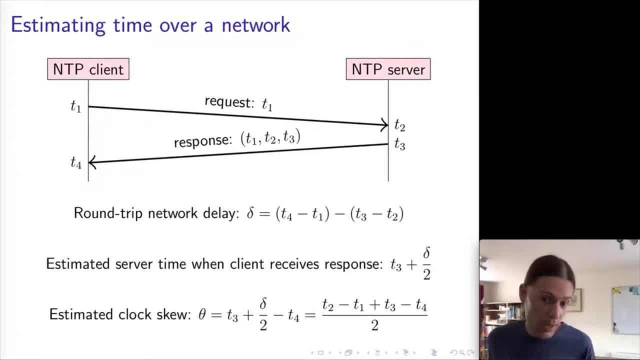 We can take our estimate of the server's clock minus t4, which is the client's clock, and that will give us the instantaneous difference in time between the two clocks at that moment. And then, if you substitute in delta and simplify the expression, you get this expression here. 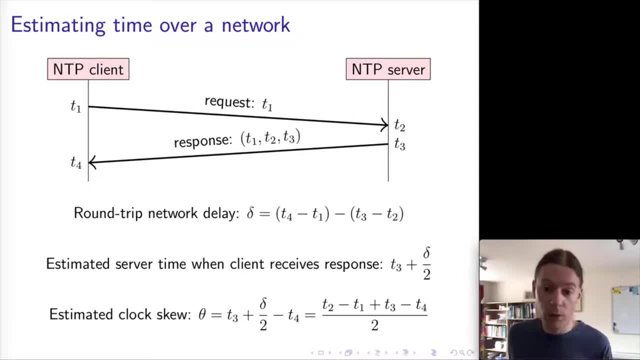 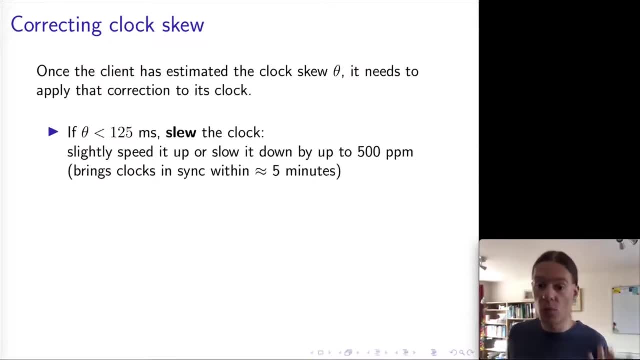 which is our best estimate we can do of what the clock's queue is. Now that we have the queue between the two clocks, the client can correct its own clock and tries to bring it in sync with the server And what the client does in that situation. 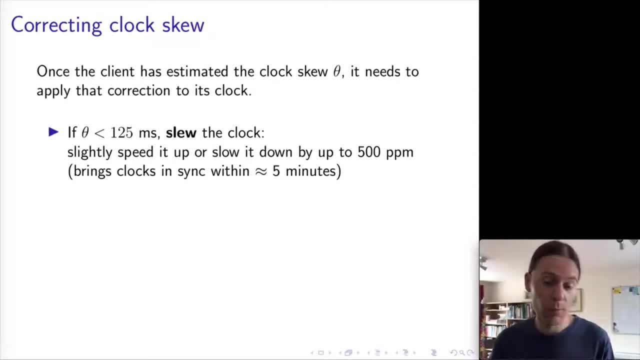 now depends on how big the clock's queue is. So, firstly, let's look at the case where the clock's queue is fairly small, So let's say theta is less than 125 milliseconds. In this case, what the client is going to do is to slightly speed up or slow down its clock as necessary. 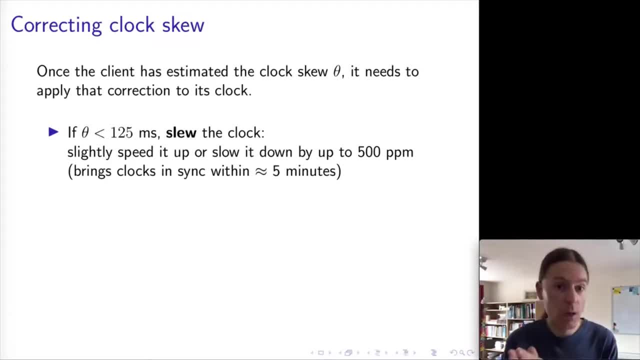 in order to bring it in line with what the server is, And so it's going to change its clock rate at most by 500 ppm, So at most by half a millisecond per second Adjustment, And so over the course of a couple of minutes this means that, hopefully, the client clock and 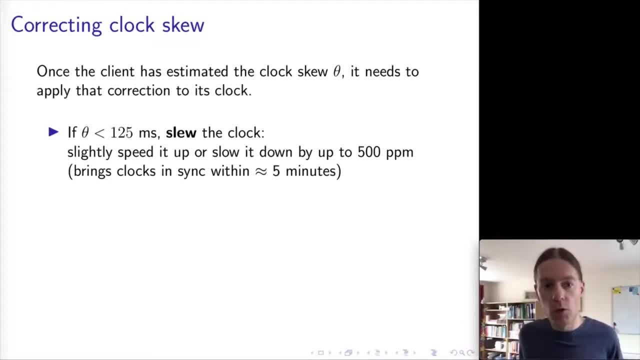 the server clock will sort of drift together and converge towards the same state, And this is called slewing the clock. That is the term that NTP uses for this. If the skew is too big between the client and the server, then NTP is going to step the clock. 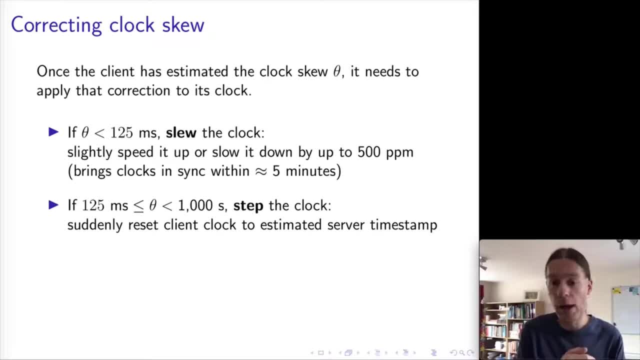 which means it's simply going to forcibly adjust the clock. So, even if this might mean moving the clock backwards or moving it forwards, but it's just going to jump right to the timestamp estimated from the server clock And from then onwards it's going to try and 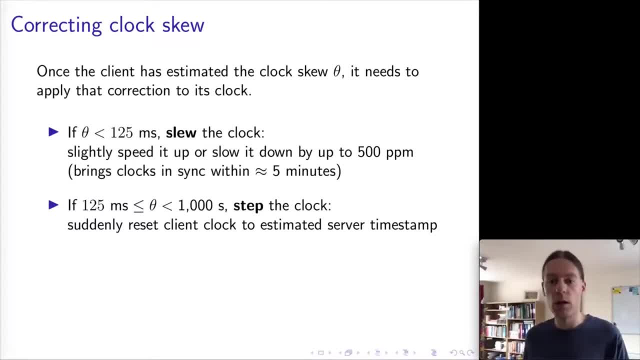 do everything smoothly. But there is this initial discontinuity of time where the client steps its clock And finally it could happen that NTP decides that the skew between the client and the server is so big that NTP refuses to adjust the clock. It just says, no, I'm not going to do. 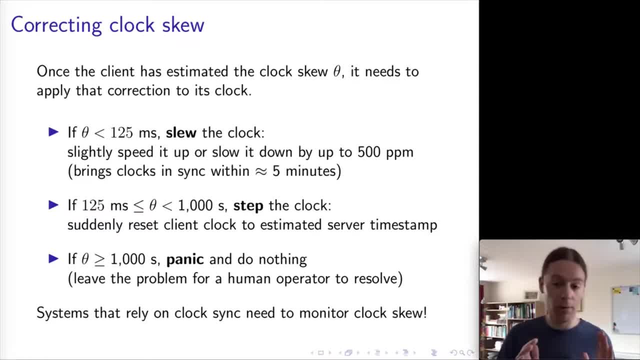 anything, I'm going to assume that something has gone very wrong. I don't know if the client's clock is very wrong or the server's clock is very wrong, But this is just so bad I'm not going to do anything here. 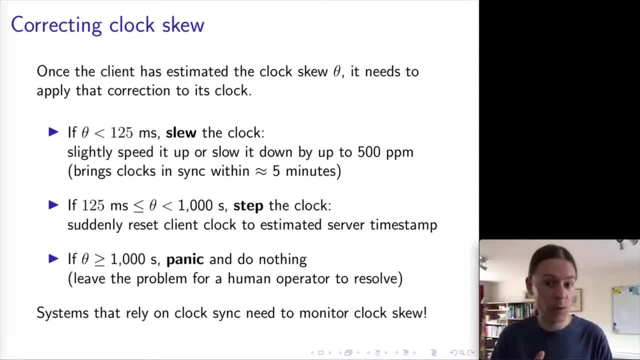 It's going to leave the adjustment for the human operator to solve. So this means now, if you do have software that is relying on clocks being synchronized, you have to be very careful to actually measure the clock skew between the clocks and make sure that it doesn't get too big, Because it could happen that an NTP client 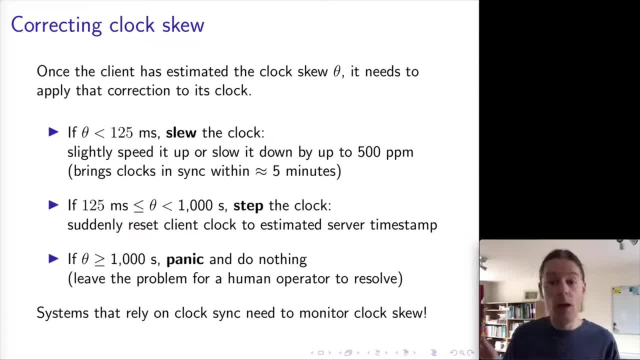 ends up in this panic state and just refuses to sync its clock with the server, And so you've got, for example, an NTP client whose clock is way off- It might be half an hour or more wrong compared to the server- and NTP is not going to correct it. So you do have to be very careful. 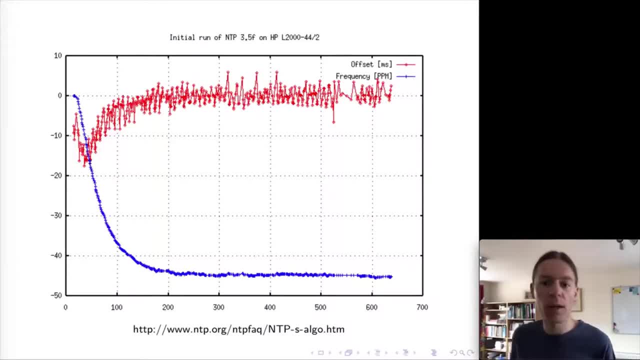 if you have software that assumes synchronized clocks. This is an example of slewing in action, So you can see here the red line, here is the skew, the offset between the two clocks, And it starts off at about 10 milliseconds offset and then the correction gets applied so that it ends. 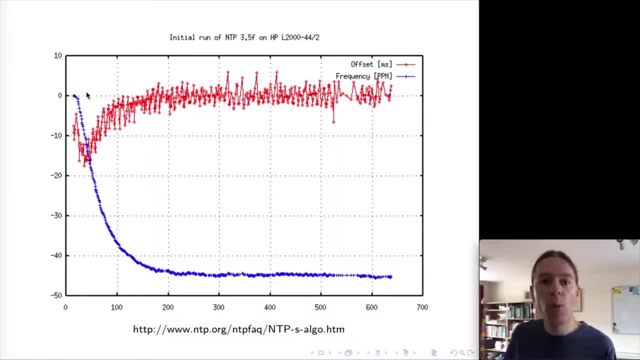 up being roundabout zero, And the blue line is the tick rate at which the client clock is running, And so the client here has applied slewing up to about minus 45 ppm. So that means that the quartz crystal in the client must have been a bit fast. It was running a bit fast, by about 45 ppm. 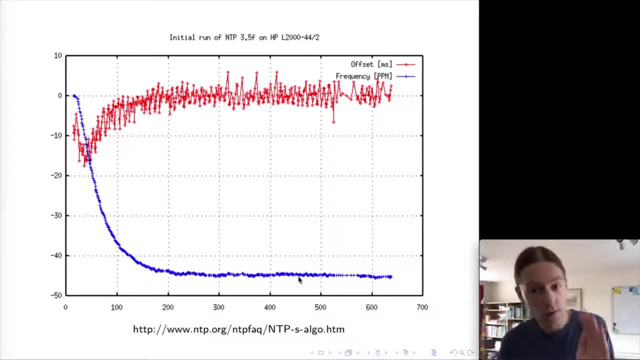 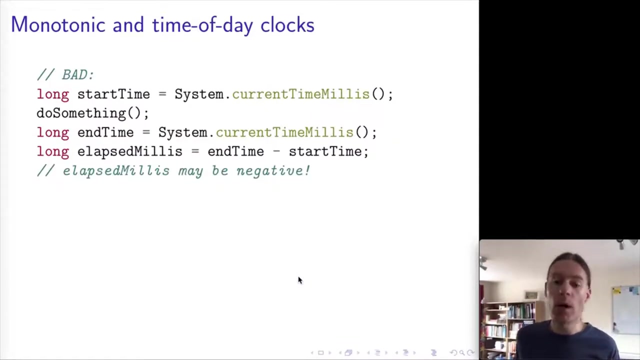 And by slowing down the quartz by 45 ppm. now the NTP client has brought the tick rate of the clock to roughly in line with the server. So now both clocks are moving ahead at about the same rate and no longer drifting apart. So this is very nice. but the consequence of NTP is that you have to be very careful when writing. 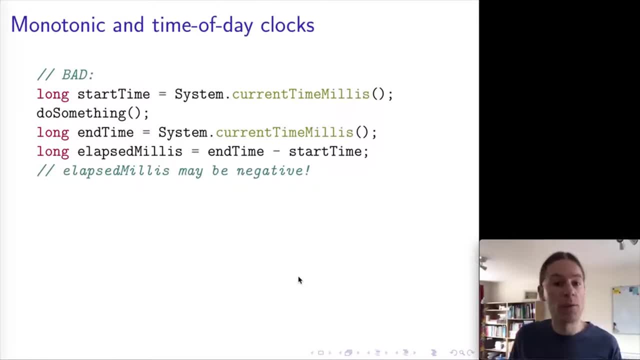 certain pieces of code. So this is a piece of code that is very likely going to occur in all sorts of different software, where you have some function that does something, do something here, and you want to measure how long that function takes to run. And so, in order to measure that, time. you simply take a timestamp from the clock before you start the function and you take another timestamp after you finish the function, and then you calculate the difference between the two. This is an example here in Java, but this could just as well be in any other programming language. 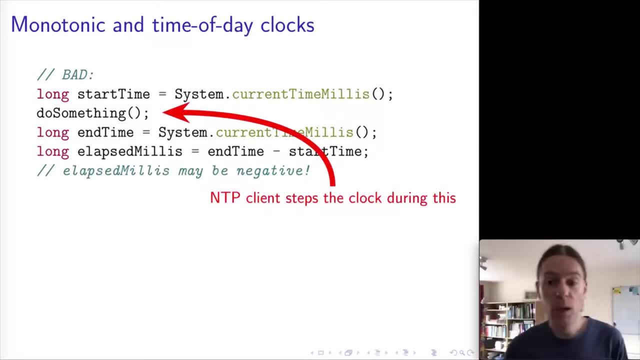 it's not specific to Java. Now what could happen is that NTP decides to step the clock right while you're in the middle of executing this do something function, And this stepping the clock means that now the timestamp returned by current time, millis after the do something, is going to be somehow wildly different from what it was before. So it could be that the clock was moved backwards, in which case this difference in timestamps could end up being negative. and who knows what your software is going to do if it measures a negative amount of time elapses. Things could crash or things could go badly wrong in all sorts of interesting ways. 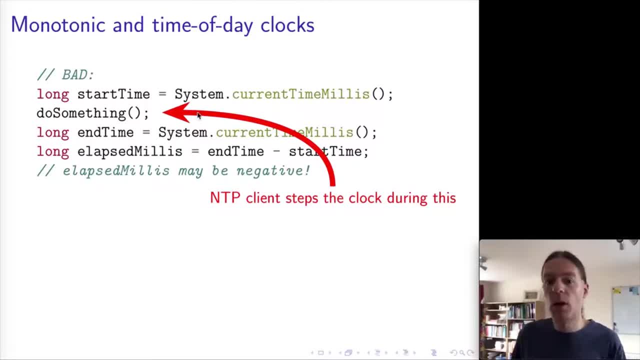 Also, it could be that the clock is moving backwards and the timestamp is moving backwards. Also, it could be that the clock is moving backwards and the timestamp is moving backwards, that this number ends up being far too large, because if the NTP client steps the clock, 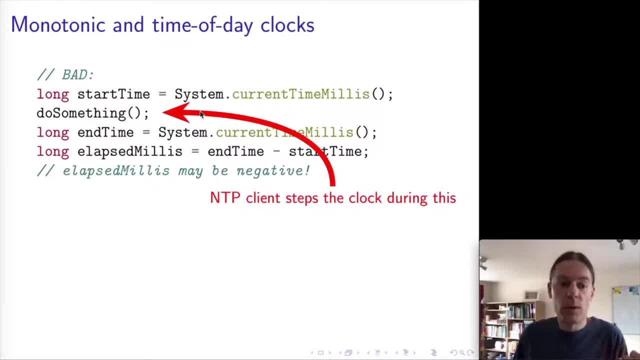 forwards. in that case, now it's going to have end time being much bigger than it, a much greater timestamp than it ought to be, and so the difference will be greater than it ought to be. So if you want to do this kind of time measurement, it is not good to rely on a clock. 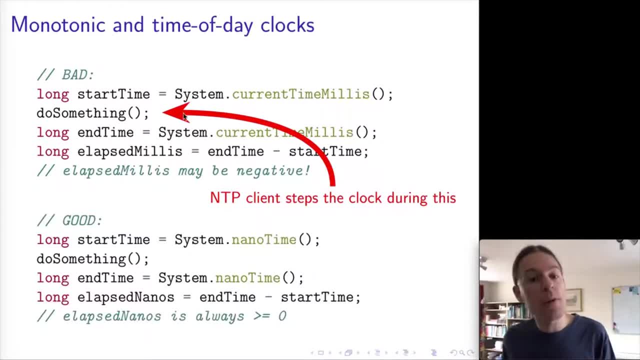 like CurrentTimeMillis. Instead, what you should do is use a different API. So Java provides this other function here called systemnanotime, and nanotime is designed for this kind of thing. So there's the superficial difference. CurrentTimeMillis uses milliseconds. 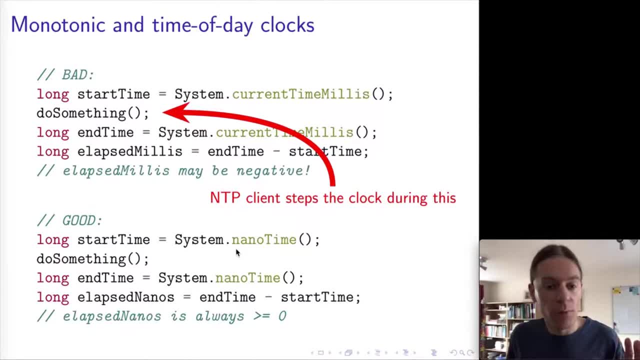 nanotime uses nanoseconds. That's just the superficial difference. The real difference is that nanotime is what's called a monotonic clock, and monotonic clock is one in which NTP stepping will not affect it, So this clock is not going to suddenly jump forwards or backwards. 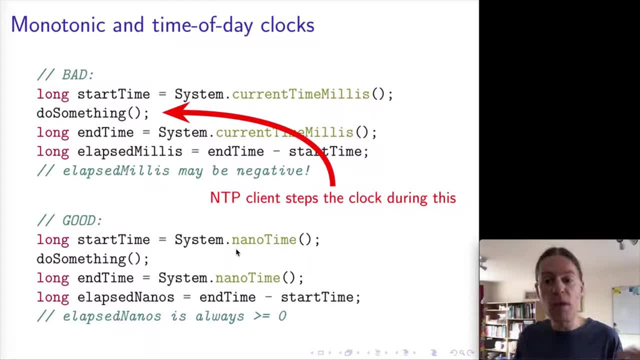 as the name says, Monotonic clock means that it moves forward at a more or less constant rate. Slewing will still affect it, because that improves the accuracy of the clock, but it's not going to suddenly jump with a discontinuity, And so using nanotime here to measure the time elapsed is the correct way of doing this. 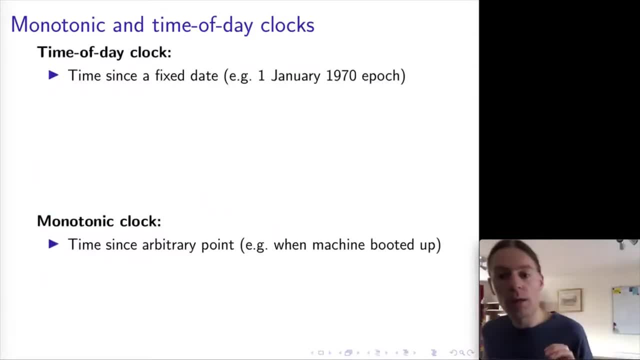 So this difference between monotonic and time of day clocks is very important. So a time of day clock is, for example, the Java's CurrentTimeMillis, which gives you the time elapsed since a fixed reference point. So the time of day clock is, for example, the Java's CurrentTimeMillis, which gives you the time elapsed since a fixed reference point in the clock. 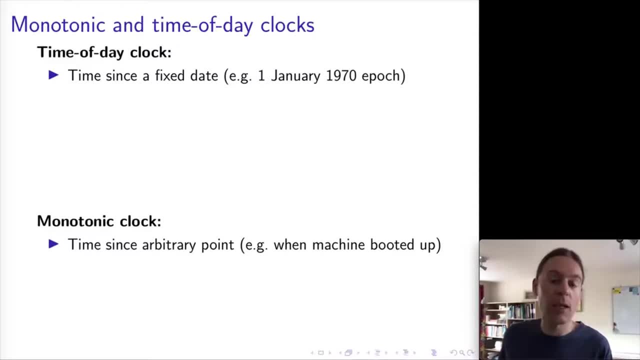 In the case of Unix timestamps, it's this 1st of January 1970, epoch date, Whereas a monotonic clock, the value you get back from it, is some arbitrary time since, for example, this particular computer booted up. So this means that the timestamp by itself doesn't 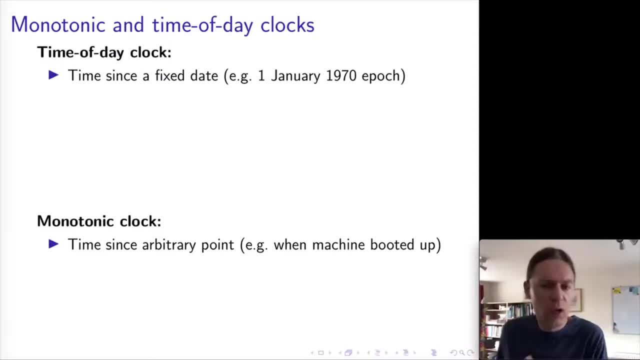 really mean anything. You can't send the timestamp over a network to another computer and compare those, because two different computers will have booted up at different times and so their monotonic timestamps are simply not comparable. But you can use the monotonic clock for time measurements, because if you calculate the difference between two 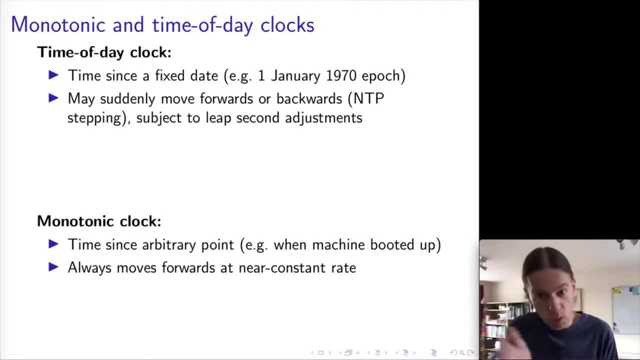 timestamps from a monotonic clock, then the time will have moved forward at a near constant rate between those two timestamps, and so that's a meaningful measure of time elapsed, Whereas if you do that sort of difference with time of day clocks, then you are affected by jumping due to 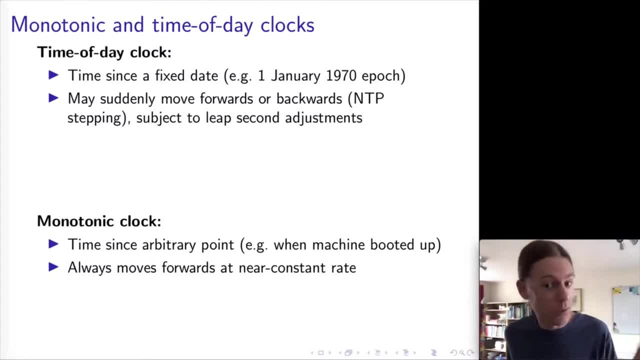 NTP, You're also affected by leap seconds potentially, which we talked about earlier. So these are very bad for measuring elapsed time But on the other hand, time of day timestamps you can compare across different computers, If you remember earlier the example I had of the TLS certificate. 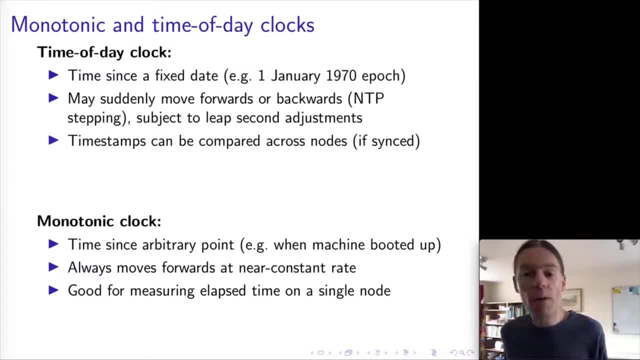 which was valid until a certain date. if my computer wants to check whether that certificate is still valid, well, it has to have the accurate current date. Otherwise it's not going to be able to compare the timestamp in the certificate with the current timestamp on that computer. 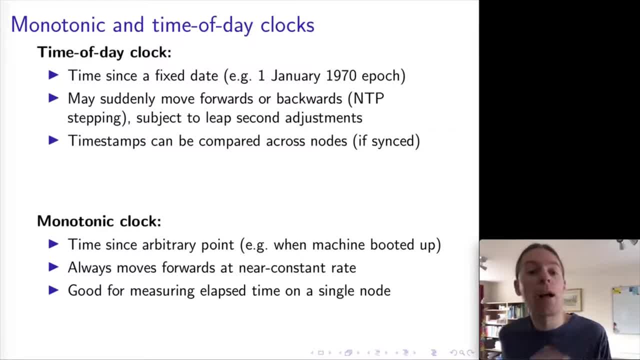 So in this case we do have to use a time of day clock and do we do have to synchronize those clocks across multiple machines, because otherwise we won't have accurate timestamps. So, as I said, many programming languages and operating systems provide APIs for. 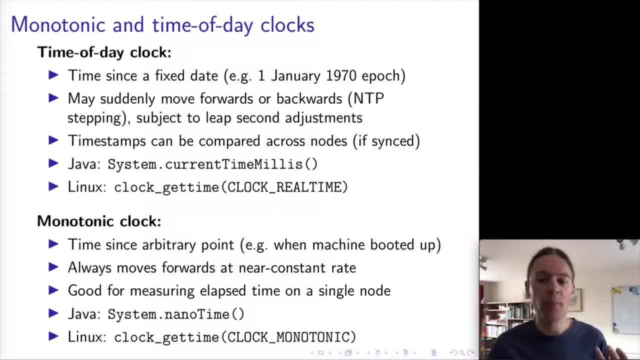 this. In Linux, for example, there's the clock get time call and you can pass an argument to it which tells it whether you want the real time clock, which is the time of day clock, or you want the monotonic clock. But in other languages there will be similar APIs for this. 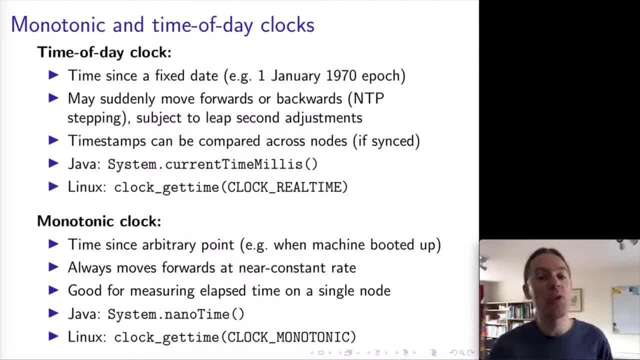 You will have to check the API documentation, But it is important to keep in mind the distinction if you do need to measure times. It's not just about the resolution of the clocks, but the distinction between a monotonic and a non-monotonic clock is very important. 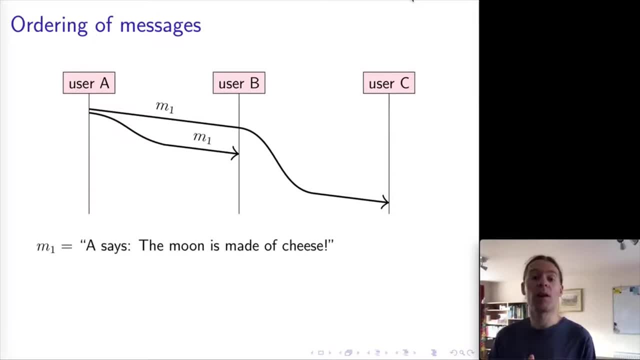 In the last part of this lecture we are going to look at the relative ordering of different messages and different events that can happen in a distributed system and how we might use time in this context. So let's start with an example. again. Let's start with an example of a discussion. 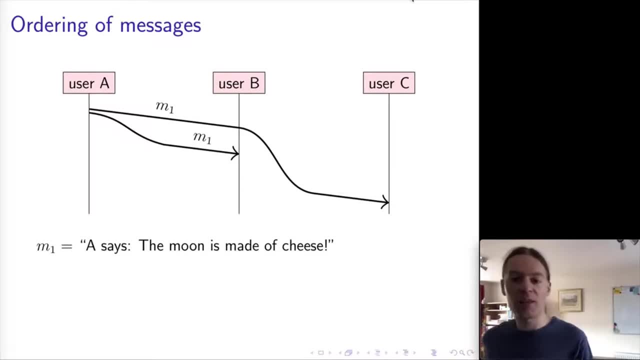 thread on the internet And you know one of those typical highbrow discussions where one user says the moon is made of cheese and another user responds to them saying no, you were wrong. So we are going to model this kind of discussion thread here. Let's say we have user A here who 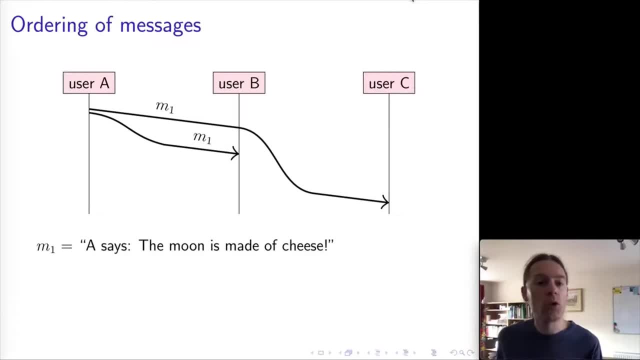 says the moon is made of cheese, sends that message M1 to users B and C And we're going to just assume our usual system model of, let's say, reliable network links. but messages might be delayed or might be reordered as usual. 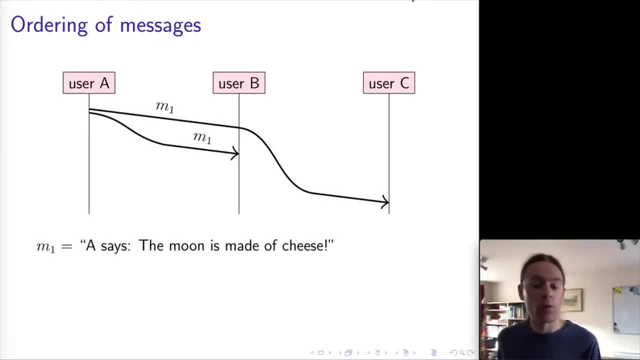 And so it can happen that user B receives message M1 fairly quickly and user C receives that message a little bit later, just because it's been delayed a bit in the network. That's fine. Now then user B responds to message 1.. User B receives M1 and says no, the moon is not made of cheese, and sends that. 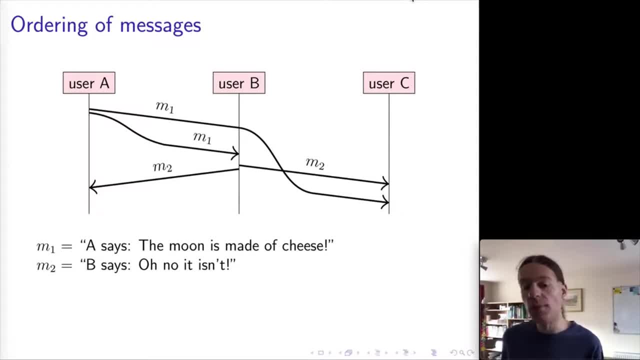 message M2 back to user A and also to user C. Now what can happen is what you see in this diagram here is that user C actually receives M2 before receiving M1.. And this is kind of confusing because if you imagine user C is looking at this thread, user C first sees, oh no, it isn't. and then 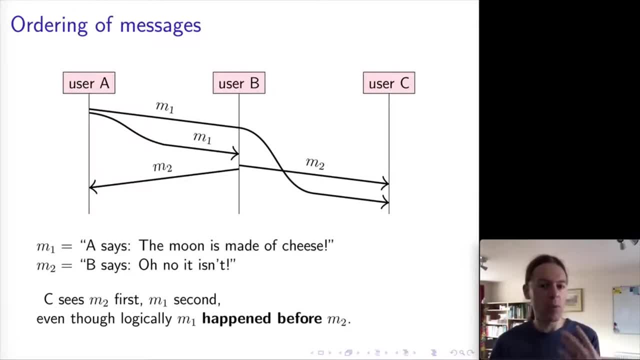 the moon is made of cheese. So even though- oh no, it isn't really should be a reply to the moon is made of cheese. user C has ended up reordering those and we've got the reply before the thing that it's replying to. 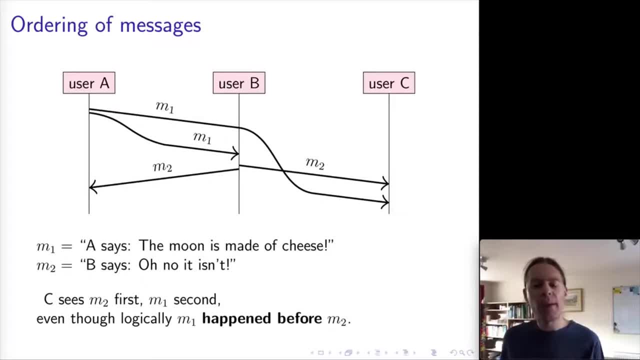 This is pretty confusing. So let's think about how we might be able to formalize this problem and how we can create algorithms that solve this problem. So this is based on this idea that one thing happened before another. I think we can agree that M1 happened before M2, because 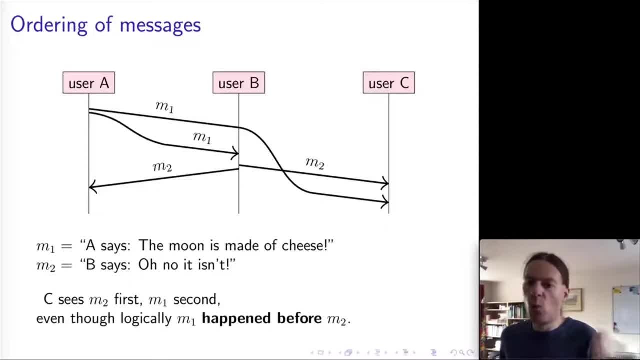 if M2 is a response to M1, then M1 must be a response to M2.. And if M1 is a response to M1, then M1 must have happened first. There's some kind of logical time in the system here. 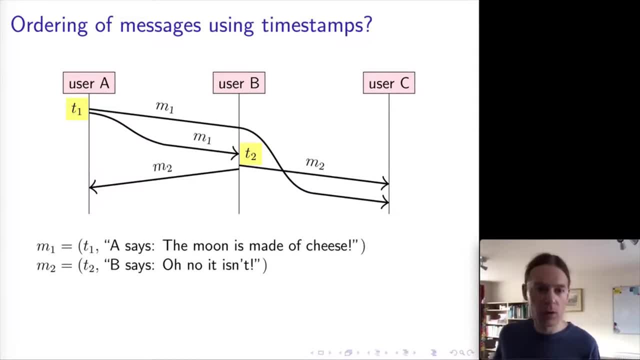 But let's see what happens if we attach timestamps to each message. So let's say that when user A sends message M1, user A also uses A's local clock to generate a timestamp T1 and attaches that timestamp T1 to the message M1.. And then also, when user B receives M1 and sends M2, user B gets a timestamp T2,. 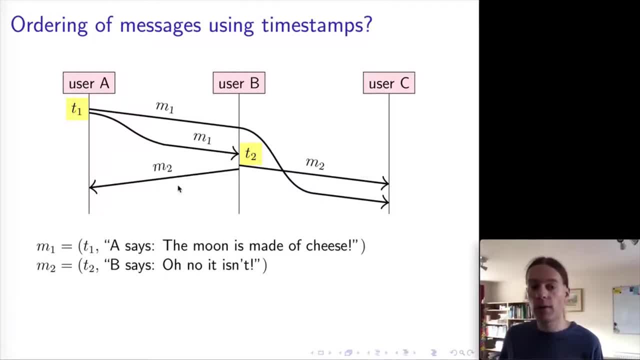 from B's local clock and attaches that timestamp to the M2 message that is sent to the other two nodes. And now we're going to assume that these are, of course, physical time of day clocks. We're going to assume that the clocks are synchronized using something like MTP, But it could still. happen even if synchronized. if clocks are synchronized, it could happen that the timestamp T2 is actually less than the timestamp T1. This could happen because the clock skew between two nodes in a system might be greater than the one-way network delay between those two nodes. And even with NTP synchronization we cannot rule out the possibility. 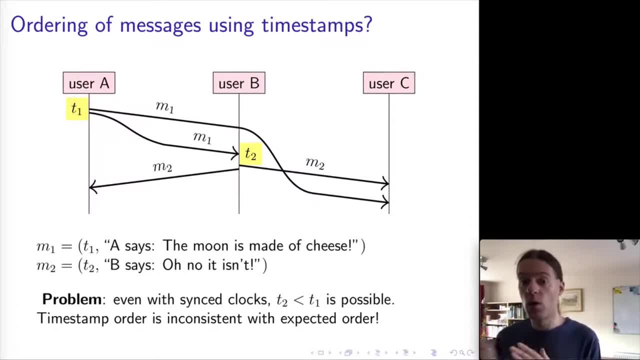 that the clock skew is greater than the one-way network delay, the one-way network latency, And so in this case here M1 is experiencing some kind of latency, but that latency is smaller than the clock skew between users A and B, And in that case, if users B's clock is running slightly behind and users A's clock is running, 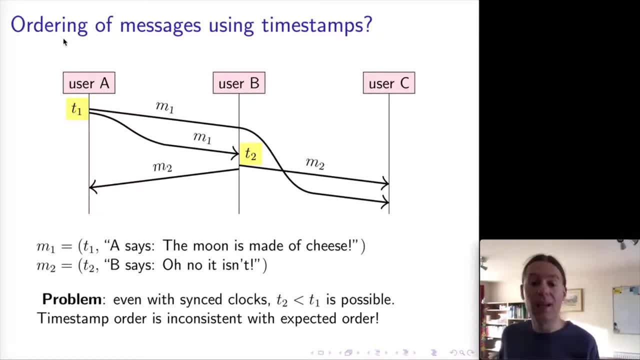 slightly fast, then you could end up with T2 being less than T1. And so our whole aim of this exercise was to ensure that messages get put in the right order according to time. But even using time here, we have not actually been able to put the messages in the right order. 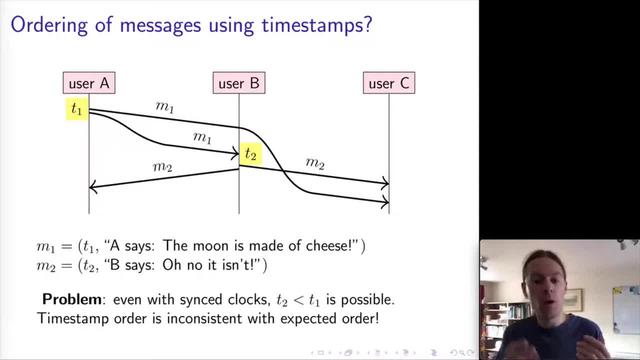 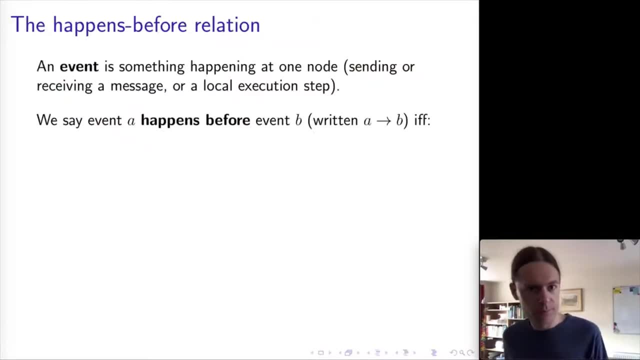 because the timestamp order is inconsistent with our understanding of which messages are replied to which other message. So how do we solve this problem? What we do in distributed systems is we use something called the happens-before relation, And so this is a mathematical model of activity. 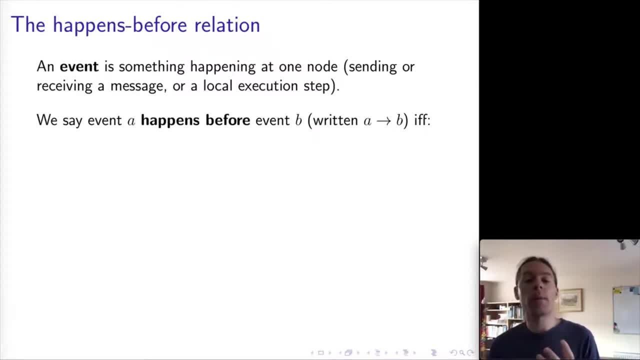 that has happened in a distributed system. And so when we're talking about activity in a distributed system, first of all we need to define what are the things that happen. So we'll say the things that happen are events. An event can be just one process, sorry, one node in the 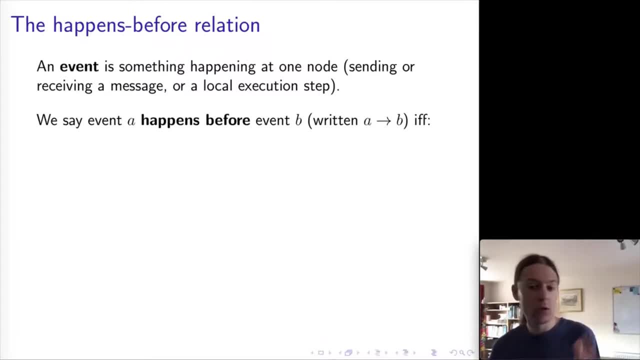 system making a local execution step, one node doing something That can be an event, Or an event could be a message that one node sends to another. So the sending of the message is one event And then the receiving of the message is another event, If the message arrives. 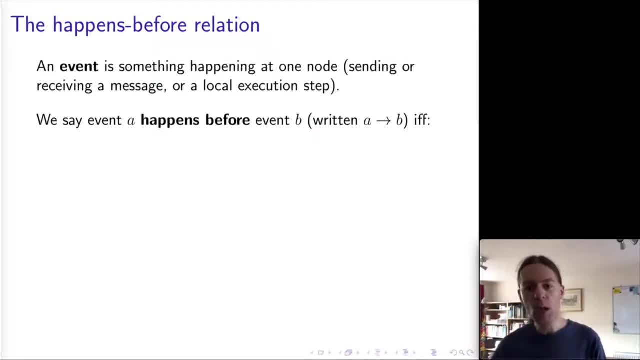 then the receiving would be another event, And so now we can define a relation, which is a set of pairs of events that describes how those events relate to each other, And this happens-before relation is written as A arrow: B if A happened before B. 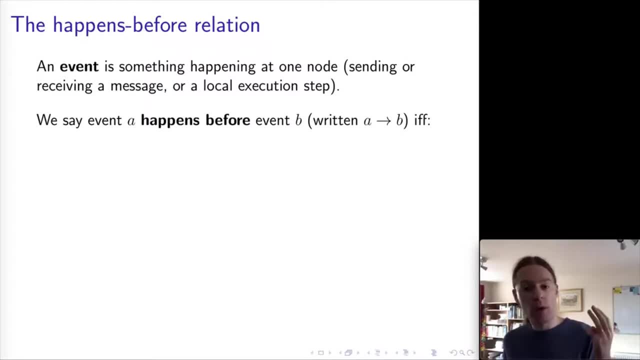 And we say that A happened before B if at least one of three things is true. So the first thing is that the two events, A and B, happened in the same node, and A occurred before B in that node's local execution order. So that means we are here assuming that each node is a single-threaded. 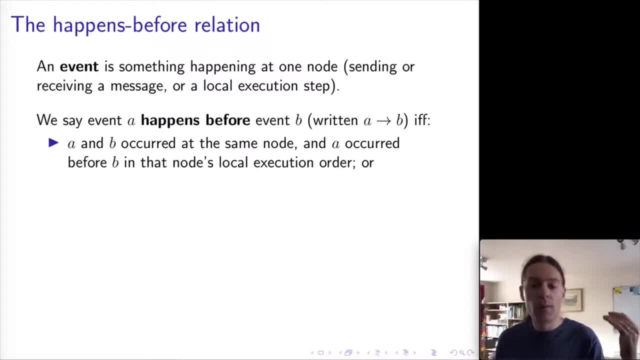 process that is just doing one thing after another. So there's no ambiguity about the order in which things happened on a single node. If there's a single thread, then things only happen one after another and we can define exactly which thing happened first and which happened second. So we're going to assume that for each node there's a strict 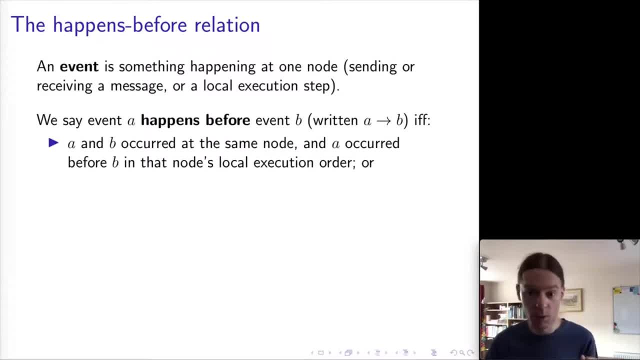 total order of all of the events that happened on that particular node. If we did want to support multi-threaded processes, then we could have each thread being a separate node for the purposes of this model here, So we can just assume single-threaded. 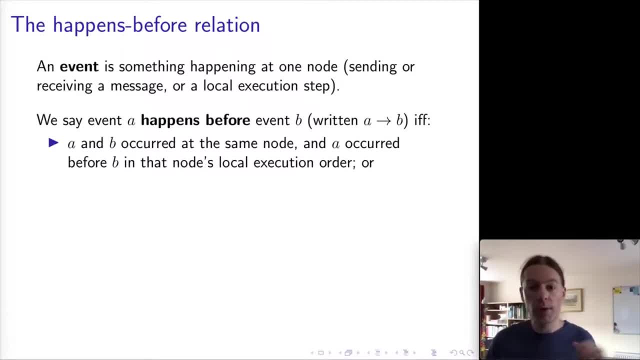 And so we're going to say that A happened before B. if they happened on the same node and they were executed, A was executed before B. That makes sense. Secondly, we're going to say that A happened before B if A is the event that a certain 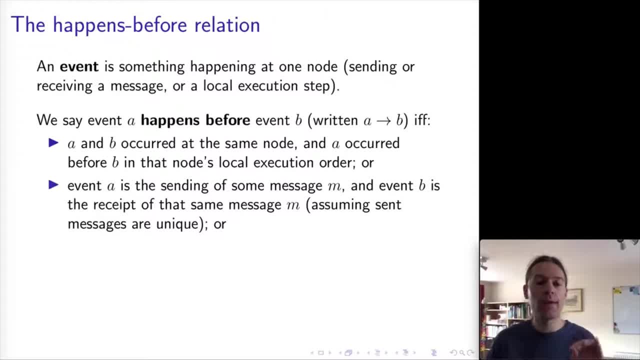 message M was sent and B is the event that this same message was received. So, for the purpose of making this unambiguous, we have to assume that messages are unique, Because otherwise you could have two different events for the sending of the same message. 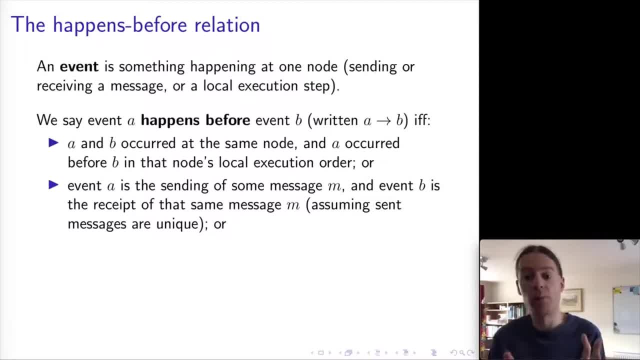 which of course could happen in a real system, but it makes the thing difficult to model mathematically. So for simplicity's sake here we just assume that every message that is sent is unique. And if we wanted to actually make messages unique in practice, we could attach: 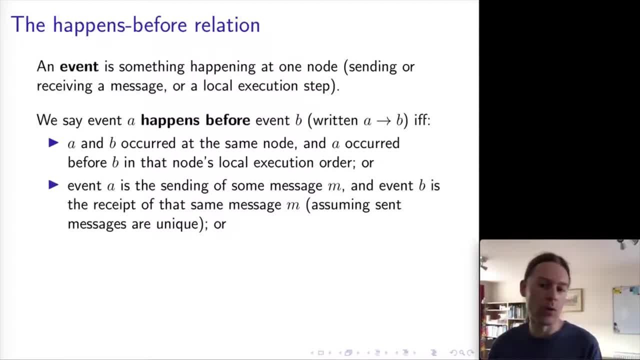 some kind of sequence number and the identifier of the node that sent the message. For example, we could attach that to every message, or we could pick a long random number for every message and that would be sufficient to make every message unique. So we could attach that to every message, or we could pick a long random number for every message and that would be sufficient to make every message unique. 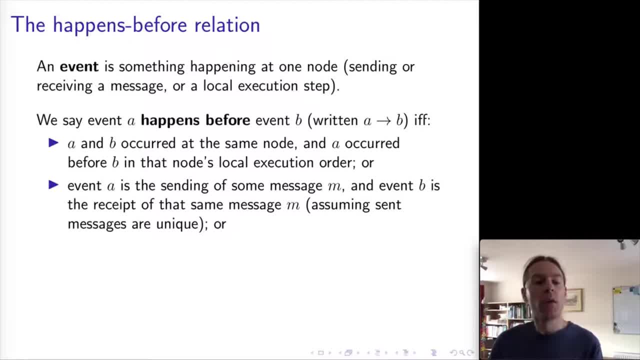 So we could attach that to every message, or we could pick a long random number for every message, and that would be sufficient to make every message unique. And so this again, this happens before relationship- makes sense because a message can only be received after it has been sent, and so it makes sense for the 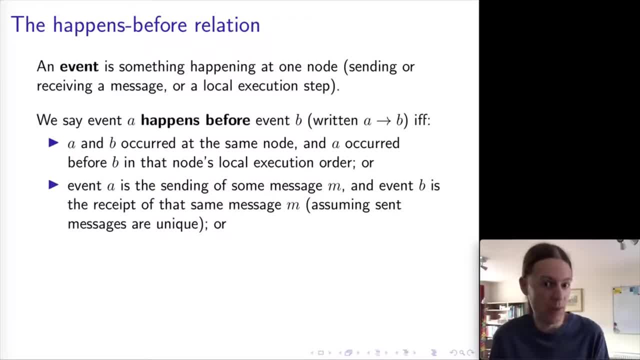 sending of that particular message to happen before the receipt of that message. So those are the first two clauses of happens before. The third is simply, if we can find some event C such that A happened before C and C happened before B B, then it must also be the case that A happened before B. So this is simply taking the transitive. 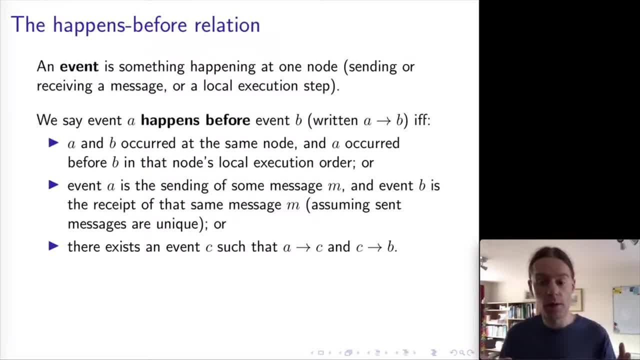 closure of the first two points and extending the whole thing into what is called a partial order. So a partial order is? it behaves a bit like a less-than relationship between two things. so it allows you to compare two things and say which one happened first. but 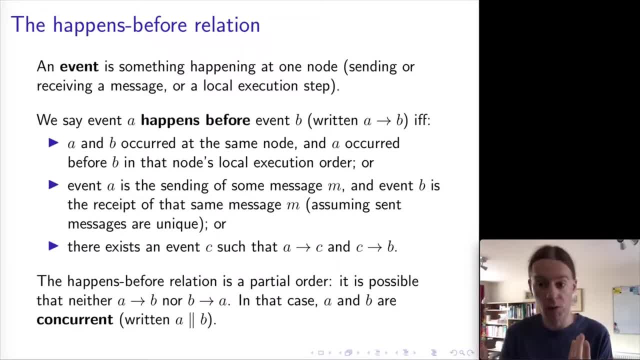 there might be some things that are incomparable according to this order, where we simply it is not the case that A happened before B or B happened before A. the two are simply unrelated. It is not the case that either one happened before the other, and in that, 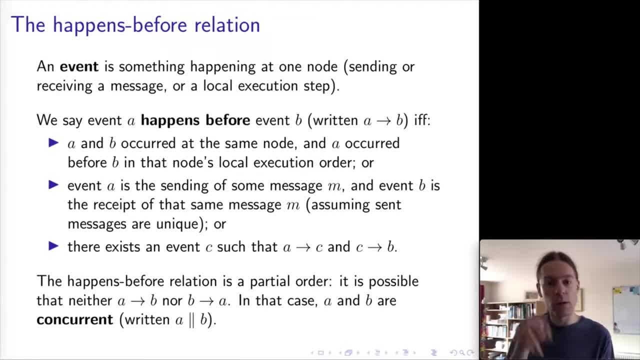 case we say that A and B are concurrent and we write it with this little double bar, this parallel sign here. So this is interesting here. now, For any two events, A and B, it turns out that there are only three possibilities: Either A happened before B or B happened before A, or the two are concurrent And one 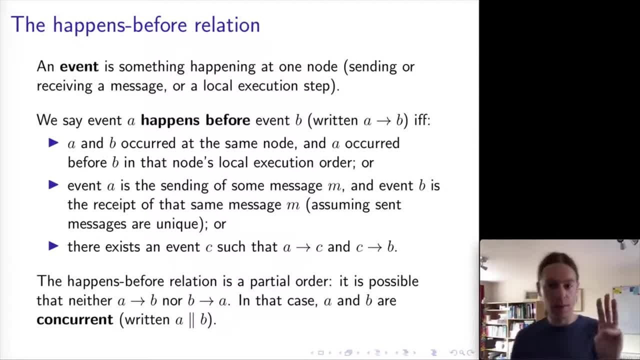 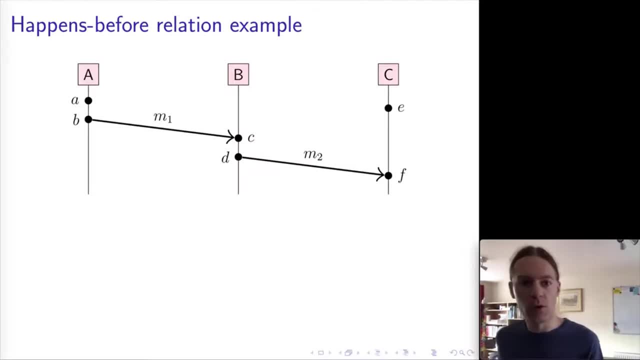 of the exercises in the notes asks you to actually prove the fact that these are exactly the three possibilities that can happen. So let's look at an example of the happened before relationship. So here we've got. events are represented as these little black blobs, and messages are sent over the network with 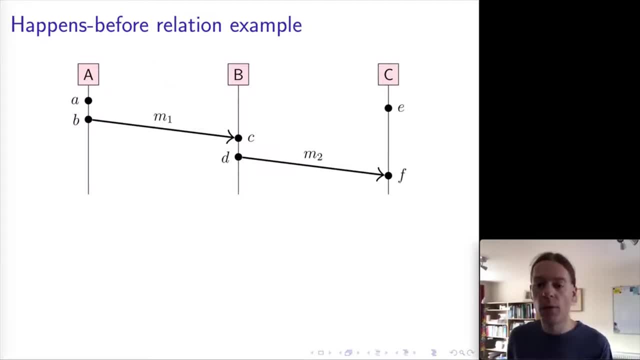 these arrows, as usual, And we've got three nodes here, And so we're going to build a relationship, We're going to build up the happens before relationship from the individual clauses And so, firstly, due to the order of events happening in a particular node, 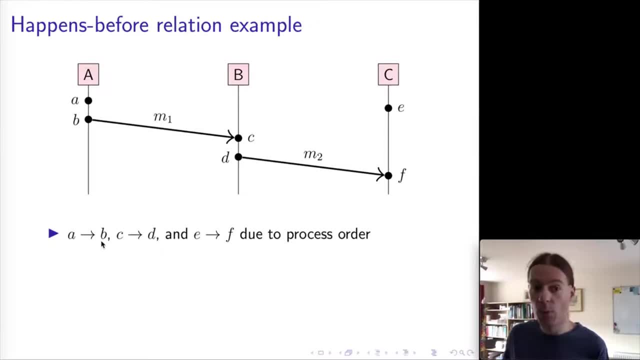 well, here, node A executed A before B, therefore A happened before B. Node B executed C before D, so therefore C happened before D And node C executed E before F, so therefore E happened before F. So far, so clear. Secondly, now, due to messages sent and received, the sent and 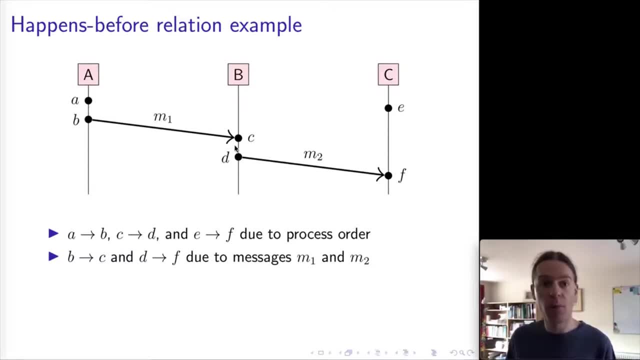 received and received events are now represented. And there's one last example where one of these events has gone past the other, And this means that A happened before B because D happened before F, and it's a positive thing if a message happens before the receipt of. 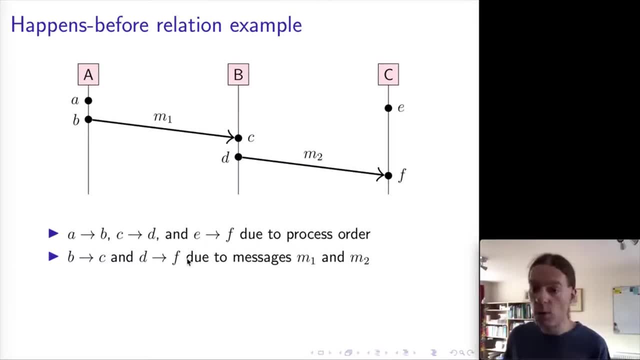 that message. So therefore B happens before C because that is message M1 traveling over the network, and also D happens before F because that is message two traveling over the network. So now we've got all of these relationships between. we can take a path through this graph. You can imagine any path that moves forward in time on. 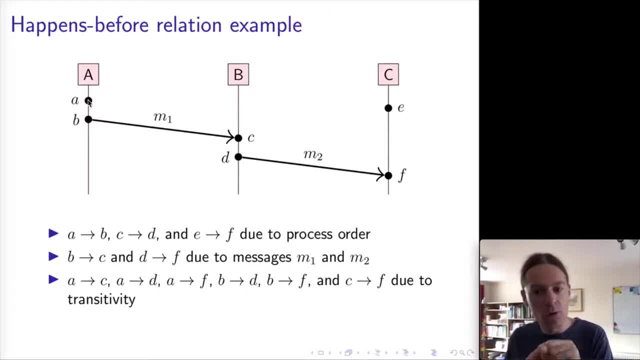 a node or that moves from the sending of a message to the receipt of that message and then move through other nodes, And you can take any path through this graph. as long as you're always moving forward in time, then you will get from any A that happened before any other event. 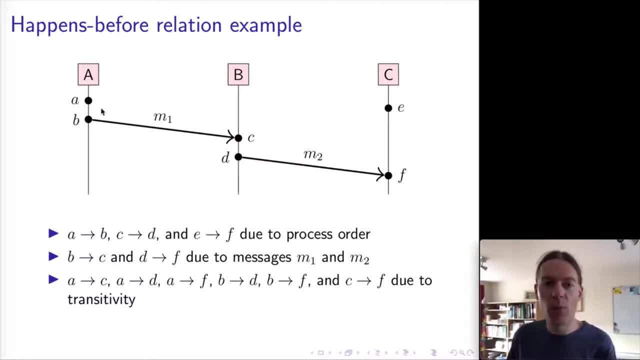 And so here, for example, you can get from A all the way to F. A happened before F, because you can go from A to F by traversing these two message sends. But, for example, you cannot get from A to E, because going from A to E would 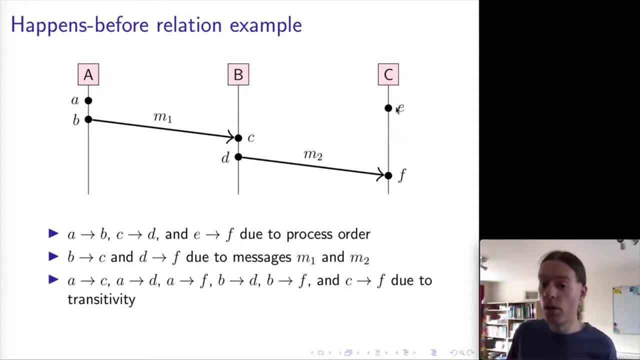 require going backwards in the node order of C, and that would not be allowed. And so that means that, for example, A and E are concurrent. so A did not happen before E, E did not happen before A. the two are simply concurrent, which means they are independent. 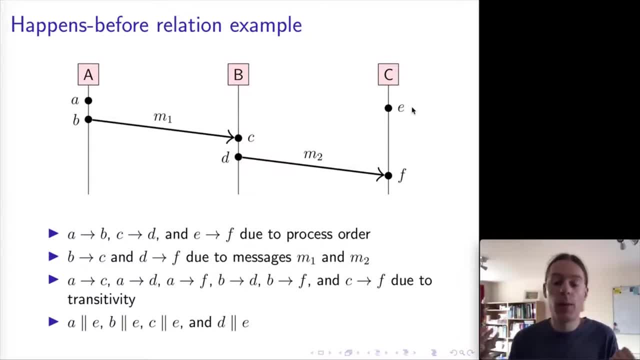 One event did not occur and no event achieved, One event did not occur and no event directed against one event. And so what happens then? not know about the other when it happened. Concurrent does not literally mean simultaneous, it doesn't mean happened literally at the same instant in time, it just means the two. 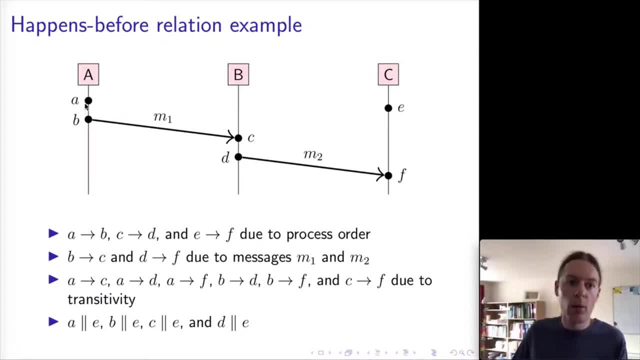 events did not know about each other when they occurred, And so therefore A is concurrent with E, B is concurrent with all- A, B, C and D, they're all concurrent to E, But E and F are not concurrent, of course, because of the order on C, on user C. 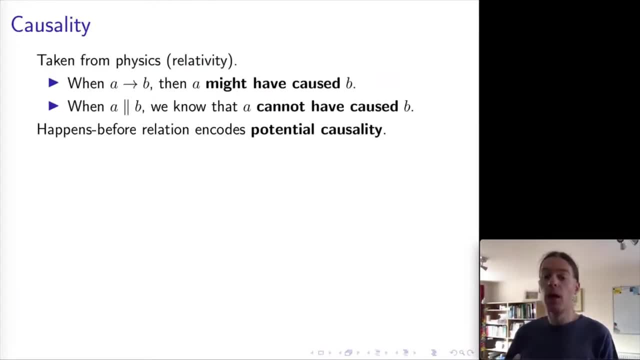 So that's the happens-before relation, And the happens-before relation is very closely connected to the concept of causality. in distributed systems In particular, if A happened before B, then it might be the case that A caused B or A influenced B in some way. So there's 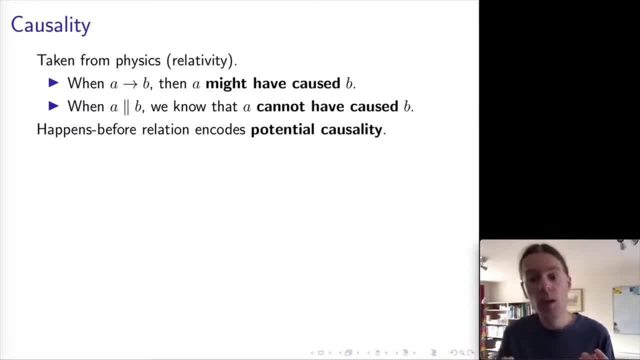 some information flow that has happened from A to B, Whereas if the events A and B are concurrent, we know that A cannot have caused B and B cannot have caused A. There's no causal relationship between the two. So this concept of causality is actually taken from physics, where typically people reason. 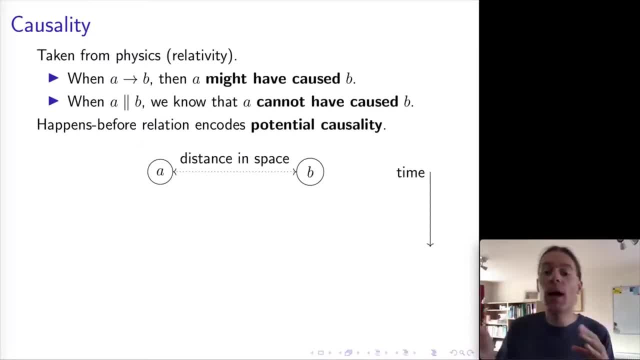 about events that happen far apart in space and the distance and the time that it takes the speed of light to travel between those things. So if you have two events happening on different planets, say, or even in different galaxies, and so they are very far apart in space, but you could have those events happening around about 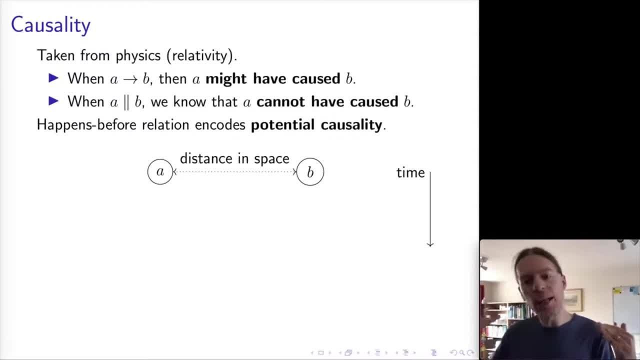 the same time. They don't have to be exactly at the same time, but they're happening fairly close together in time but fairly far apart in space. Then we can draw this space-time diagram here. So we can draw this diagram where, imagine: 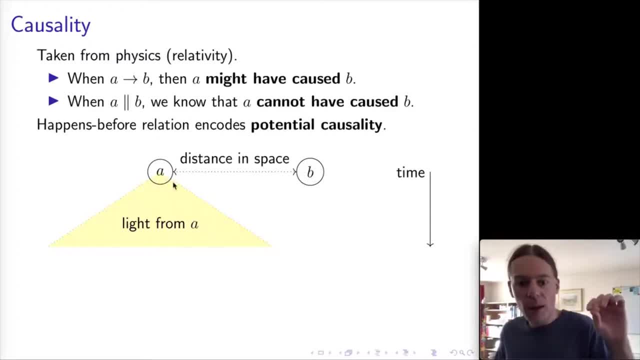 that you send out a beam of light from event A at the time when event A occurs, and you send it out in all directions, And so then, as time goes here downwards, and space is from left to right- Sorry, this light just spreads through space. 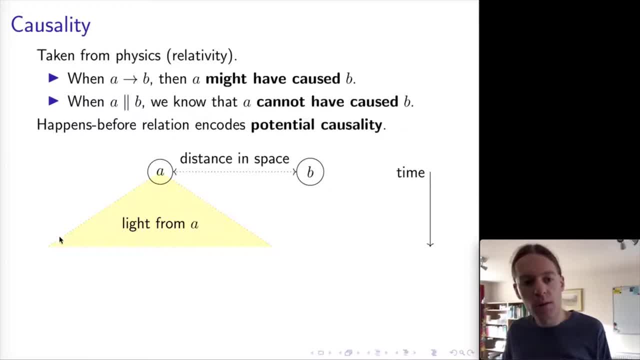 at the speed of light and any event that happens within this cone- here this is called a light cone. That event might somehow be dependent on A, but you can see B here is way outside of the light cone of A And also A is outside of the light cone of. 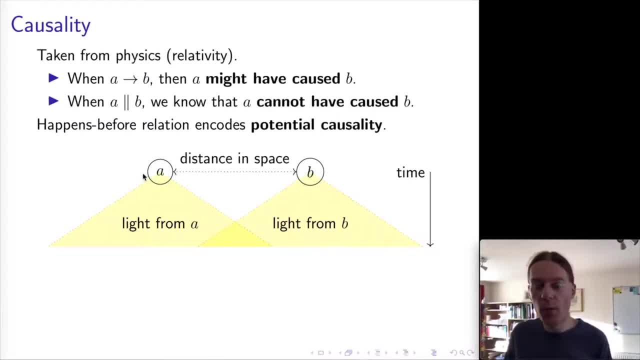 B. information from B at the time when B occurred could not possibly have got to A by the time A happened, And likewise the information when A happened could not possibly have got to B by the time B happened, simply because that would have required information to travel faster than the. 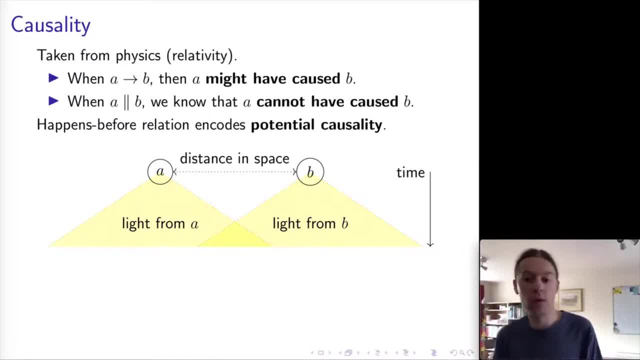 speed of light, And as far as we know, in our universe it is not possible for information to travel faster than the speed of light. So this event C here, for example, that could be influenced by A or B, but B and A cannot influence each other, And so this concept. 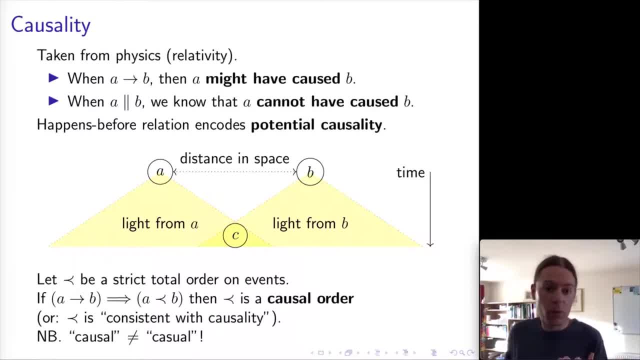 from physics is very closely related to what we have in distributed systems. In distributed systems, we typically talk about messages flowing over a network rather than light traveling through the universe, But essentially it's the same idea. It's reasoning about which events could. 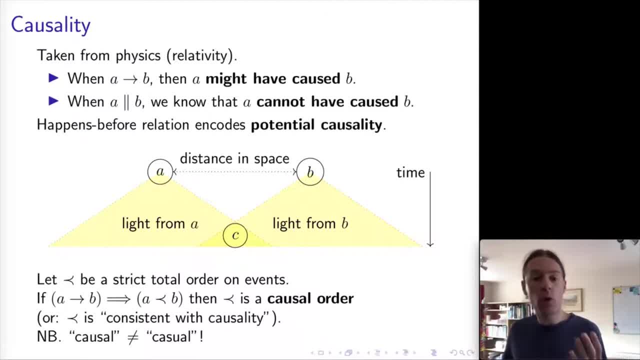 possibly have affected each other. And once we have got this potential causality- and this happens before relationship- we can now order events. And so remember, in our case of first, the moon is made of cheese, and then the reply to it: oh no, it's not. What we want is. 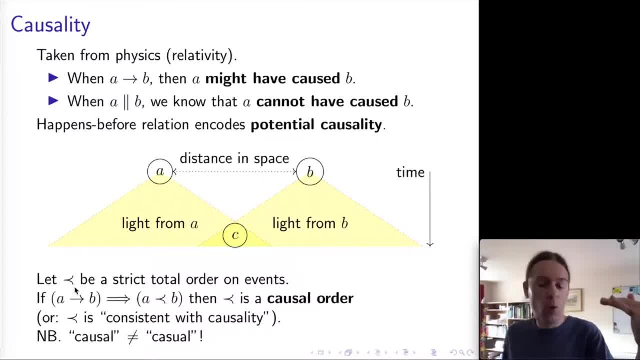 for the moon is made of cheese to come first in this order of the conversation thread and then the reply to come second in that order. And here because we have a causal relationship between M1, which is the moon is made of cheese, and M2, which is 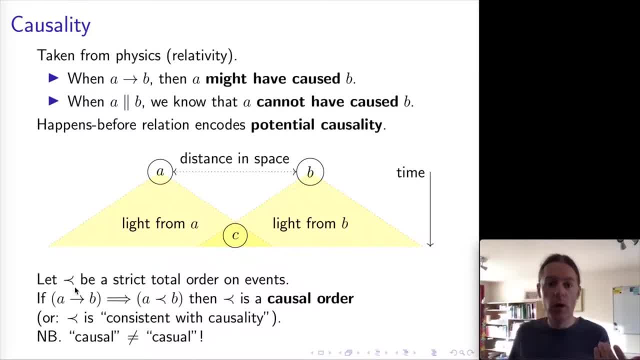 the reply to M1, so there's a causal relationship between the two, And so therefore, A happened before B, the message one happened before message two. What we want is that any order that we put the messages into should be consistent with that. So whenever A happened before B, then A occurs. 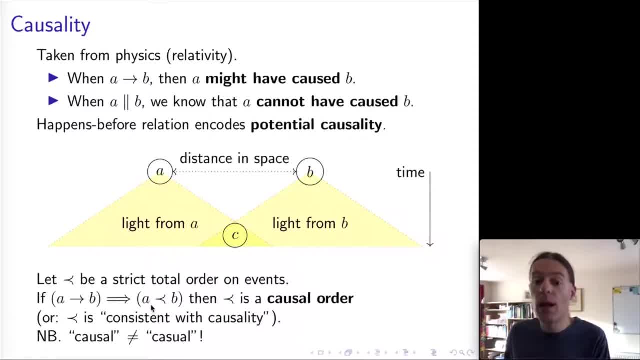 before B in that causal order. This is called a causal order, That is, it's a way of putting the events in the system into an order in such a way that they are consistent- consistent with causality, That is, if one thing happened before another thing, then they appear in. 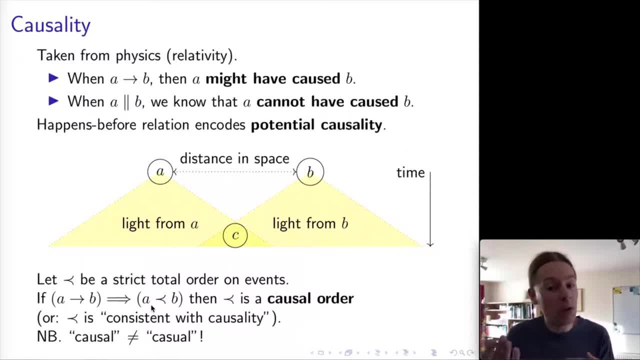 the correct order. But if two things are concurrent, then they could appear in either order because you know one could have happened before the other. There's no real way of saying which one happened first, So in that case they could be ordered arbitrarily. So this is a very useful 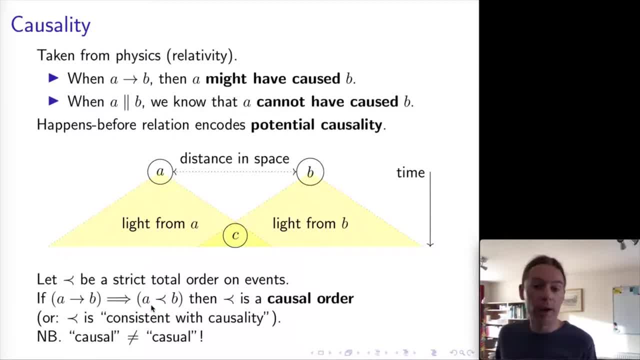 concept and we're going to use this in the next lecture when it comes to building upon this idea of the happens before relationship and making some actual distributed systems that implement this. The last thing I will just point out is it's very easy to confuse the 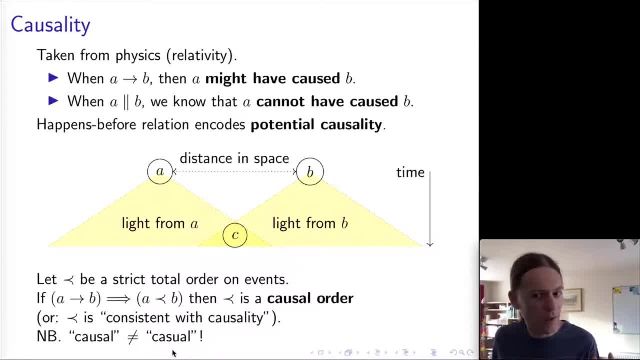 word causal with the word casual, because just two letters are swapped around. I keep having to double check it myself as well. So just that as a little detail to watch out, for if you're writing about distributed systems, you probably mean causal, not casual. So see you next time. 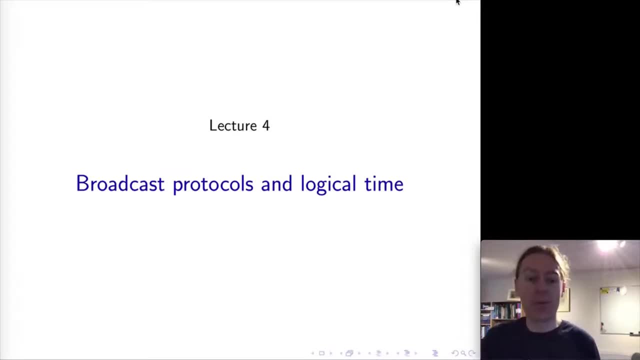 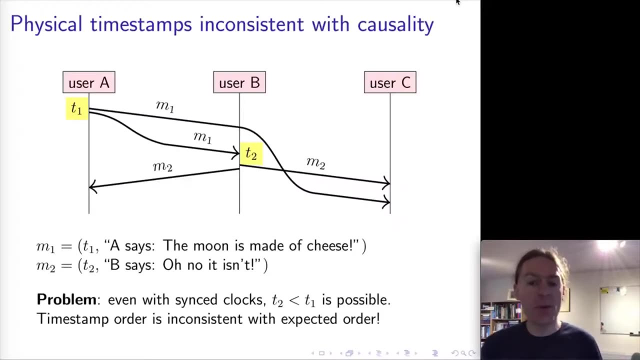 Hello everyone, Welcome to lecture four of distributed systems. Today we will be talking about broadcasting. We will be talking about broadcast protocols and logical time As background. remember this slide here from the last lecture where we had the case of two messages. First message one is: user A says: 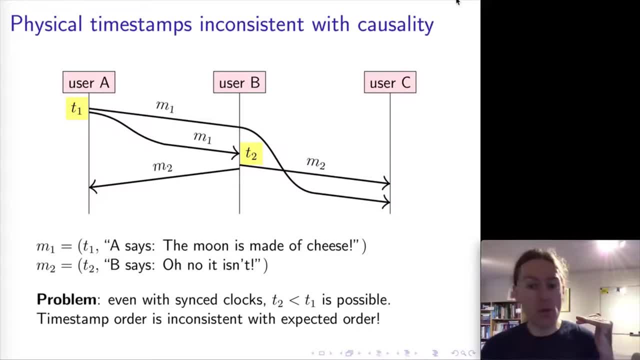 the moon is made of cheese. Message two is user B replies to this. replies to M1 saying: oh no, it isn't. And what could happen with physical clocks is that the timestamp of message one ends up being greater than the timestamp of message two. 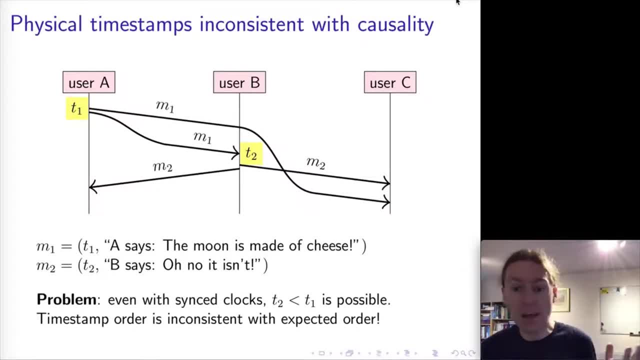 So it could be the case that those timestamps are inconsistent with the order that we intuitively expect of those two messages, that those messages are inconsistent with causality. Now, this is a problem with physical clocks, Even after we've gone through all of this effort to synchronize. 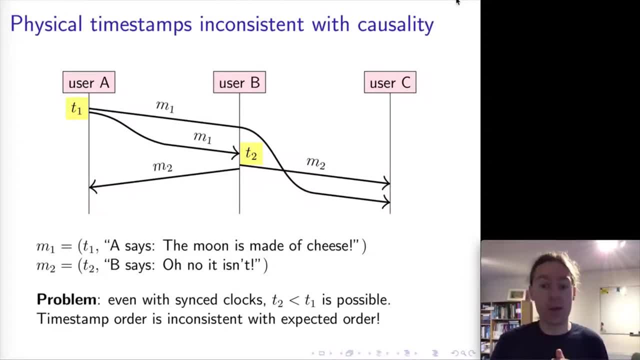 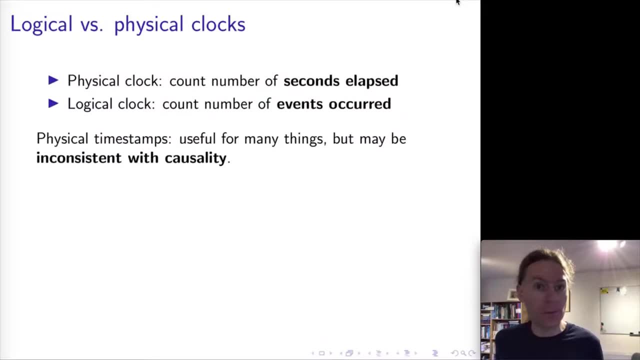 them using using NTP. even then, it could happen that you get these inconsistencies with causality. So this is where logical clocks come in. Logical clocks- these are alternative definitions of clocks that are used in distributed systems, which are specifically designed to capture the causal relationships between the events that happen. 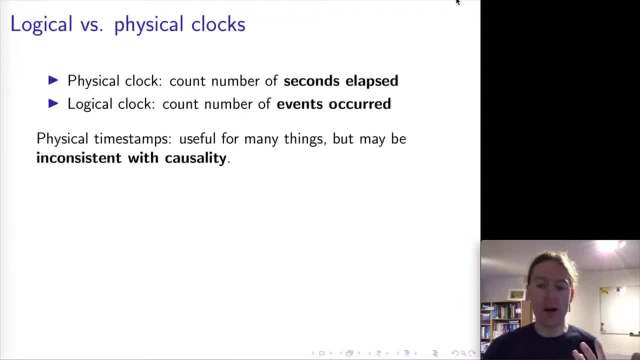 in a system, And so logical clocks are. they are sort of clocks. they're not clocks in the sense of measuring how long it's been, measuring how far the sun has the earth has turned around the sun, measuring how far the earth has rotated around its own axis. those 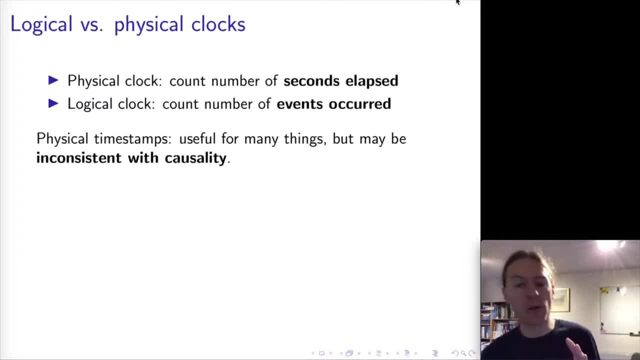 kind of things: physical time In logical time. we're not actually interested in how many seconds have elapsed. Instead, what we're interested in is how many events have occurred, And so logical timestamps are essentially just counters that we increment every time when something happens. 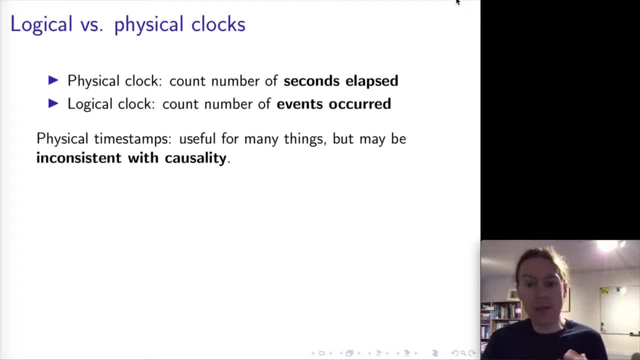 And so this means they do move forwards in time, they get greater as stuff happens, but they don't have a direct relationship to physical time. So the key thing that we want of a logical clock is that it captures causality. It captures the happens-before relationship. In particular, if event 1 happened before event 2, then we 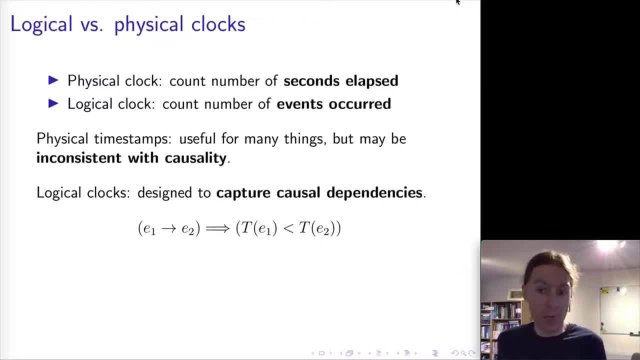 want the timestamp of event 1 to be less than the timestamp of event 2.. This is like a minimum basic thing that we expect of our logical clocks, And we're going to look at two different constructions of logical clocks: Lamport clocks and vector clocks. 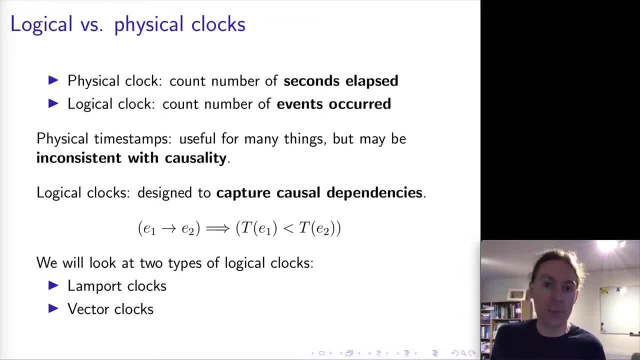 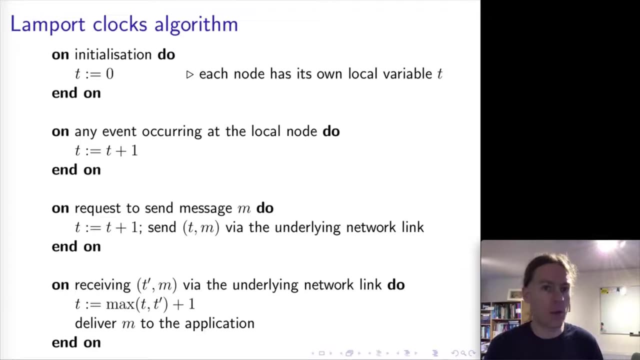 Both of these satisfy this need to capture causality, but they have slightly different properties in other areas, as we shall see. So let's start with Lamport clocks. These are named after Leslie Lamport, who published this algorithm in about 1978 or so, And this has really been a classic of distributed systems. 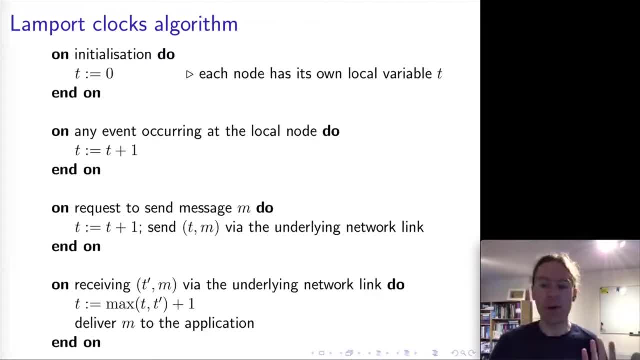 And the algorithm is fairly simple. So the algorithm starts at every node. we have a variable that we call t, And this variable is initialized to 0 when we start up the system And each node has its own copy of this variable. Each node has its own t And every time when some event 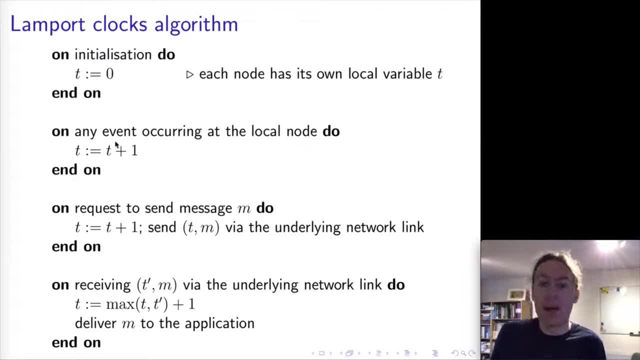 occurs at a node, we just increment t. So an event could be some local execution step taking place, or it could be sending a message or receiving a message. In all of these cases, we just increment t. Now, every time we want to send a message over the network, we increment t as usual. as for 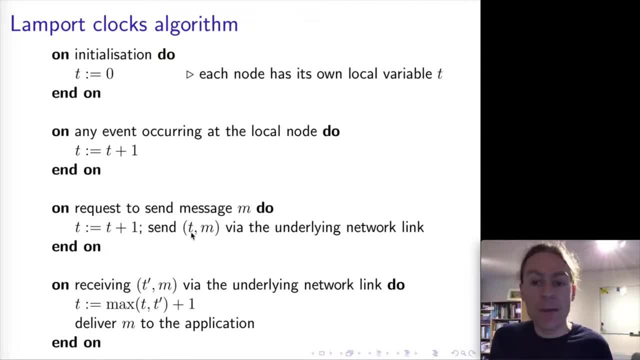 any local event. So we take the value of t after incrementing it, and we attach that to the message. So the message we send is actually this pair over timestamp and the actual message, And that is what gets sent over the network. Now, when one of these pairs is received at the 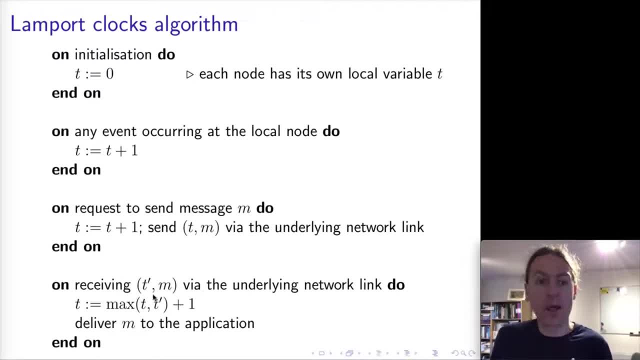 other end the node that is receiving the timestamp. Sorry, the node is receiving the message. takes the timestamp out of the message. t prime is the timestamp in the message And it looks at its own local variable, t, And it then takes a number from the response. which we'll solve between these two. So the first is a В and the second is is equals time and so on to one of them and Dee isключing each of these values and interlying them together. foraka nos always run Z and önc where her Q variables appear as Pig, right in that fret edge of the. 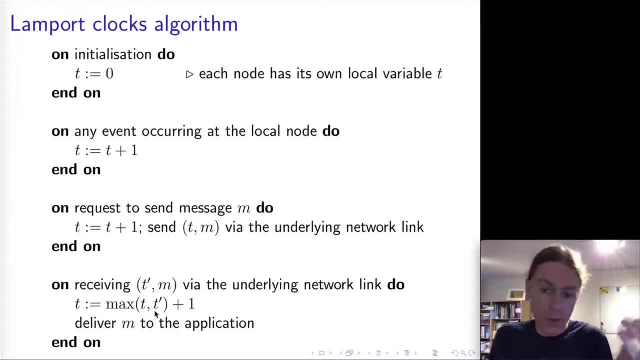 And it updates t to be the maximum of either its own local existing timestamp or the timestamp in the message, plus one incrementing it again, like for every local event. And so, after this has been done, we've got an updated value t and we deliver the message to the application. 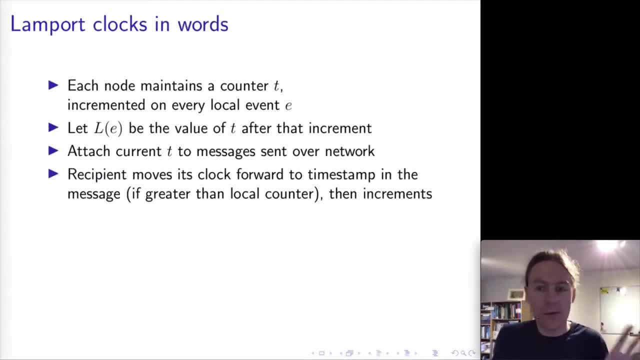 So let's look at a bit of around Lamport clocks. So we have this counter t here on each node and we can associate a particular value of t with every event. So let's say that some local event occurred and call that event e. 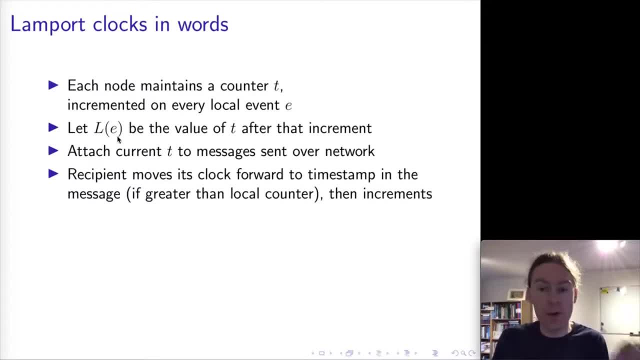 For every local event we increment the counter. So after that increment we take the value of that counter and associate that with that event, e, and call that L of e for Lamport clock. As I said, we attach those values Over on the messages that we send over the network as well. 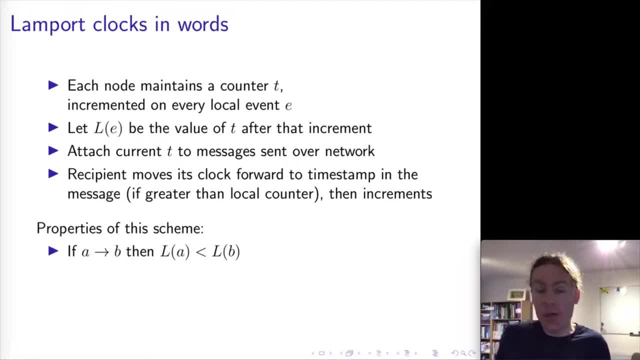 And so these Lamport clocks have some very nice properties. First of all, if event a happened before event b, then the scheme guarantees that the Lamport timestamp of event a is less strictly less than the Lamport timestamp of event b. 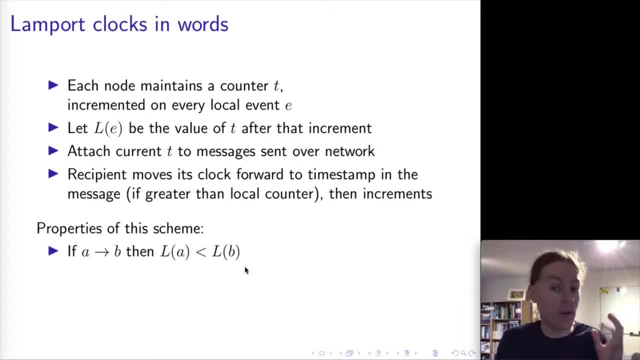 And there's actually an exercise in the lecture notes that asks you to prove that this is indeed the case. However, we The converse is not true. So if we have two Lamport timestamps and we compare them and we find that L of a is less than L of b, that does not imply that a happened before b. 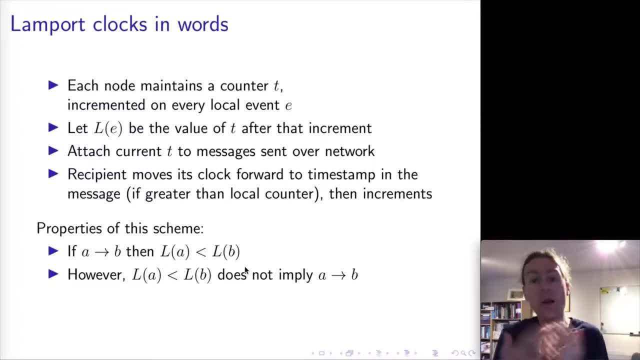 It could also be the case that a and b were concurrent. So the Lamport timestamps don't allow us to tell whether a or b were concurrent or if a happened before b. The only thing we can do is we can rule out that b happened before a, because if b happened before a then timestamps would have to be the other way around. 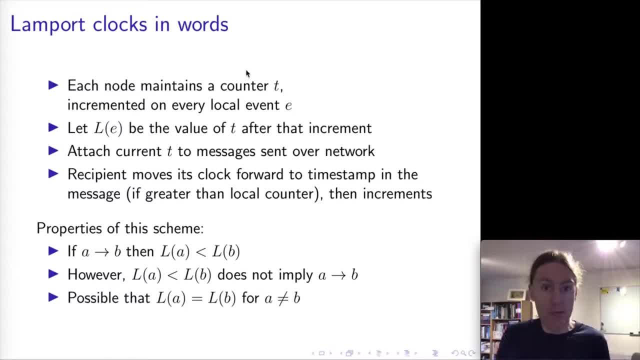 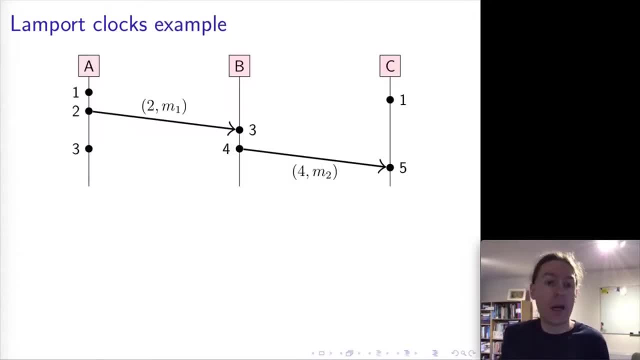 Another thing that can happen with these Lamport timestamps: it's possible that we have two different events with the same timestamp. There's nothing preventing this, So let's have a look at a concrete example here. So here we've got an execution with some events. 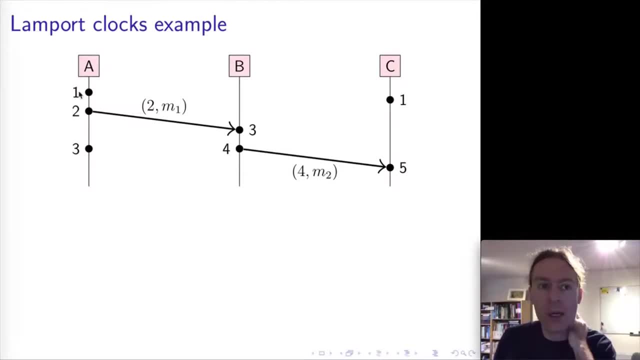 The events are again little black blobs and we have messages sent over the network. So here for the first event by node a, we just increment the counter for that local event. The second event by node a is that we send the message m1 over the network. So here for the first event by node a, we just increment the counter for that local event. The second event by node a is that we send the message m1 over the network. The second event by node a is that we send the message m1 over the network. 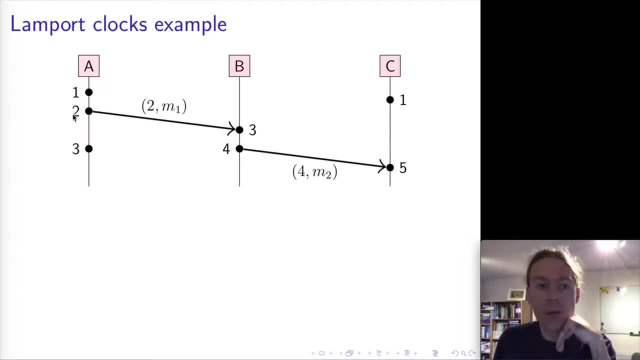 The second event by node a is that we send the message m1 over the network, over the network, and so here we have the, the timestamp 2 associated with that event, and we also copied that timestamp into the message that we send and attach it to the message. 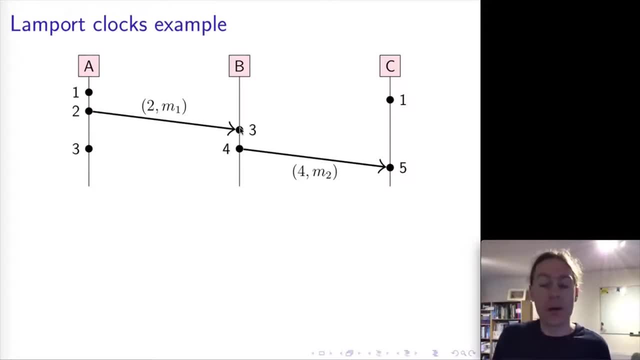 Now here, when b receives m1, the before that the local timestamp or at b will just be zero, because no events have happened so far at b. But when the time when the message with timestamp 2 arrives at b, we move the local timestamp forward to b and increment it by one again. so we end up with three. 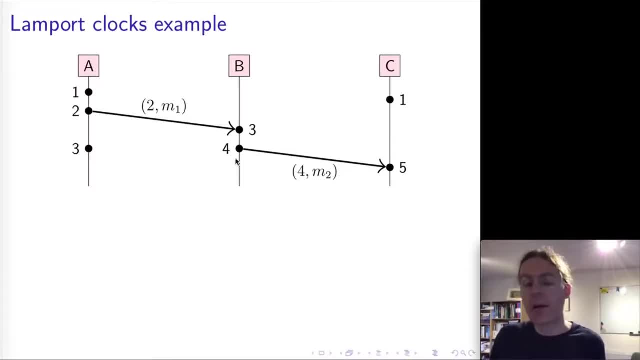 as this timestamp of the receive event. Then next local event happens at b and that gets the timestamp of four. that timestamp before gets attached to the message m2 that's sent over the network, and so here, likewise, at node c, again the local timestamp at c gets moved forward to. 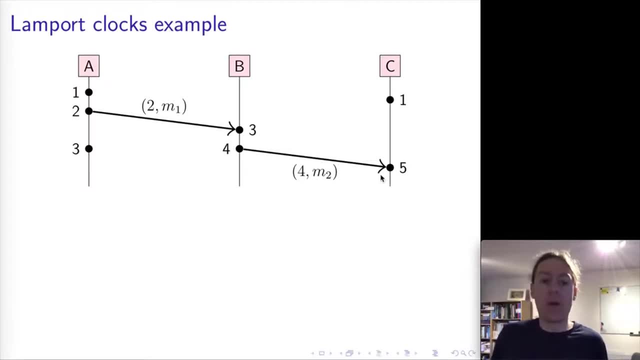 four plus one, which is five. Now, a few things to notice here. one is, for example, that there are two different events with the same timestamp three, and they're also two different events with the timestamp one, and so one thing we might want to do is to have timestamps that. 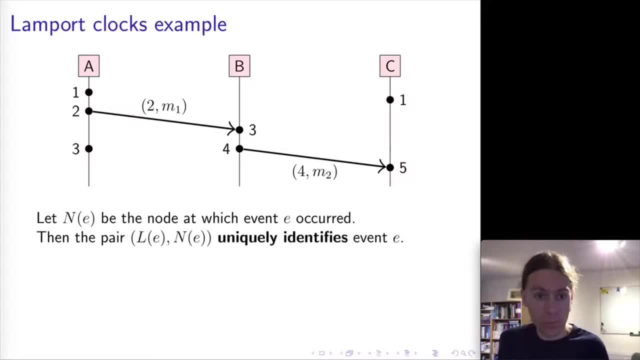 uniquely identify events in the entire system, and we can do this by combining the Lamport timestamp with the name of the node at which that particular event occurred. So if we say here, for example, if you look at the events that happened at a within the scope of a, each of the events has a unique timestamp. 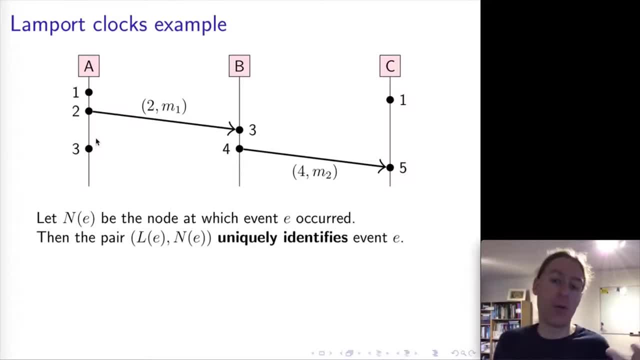 because we always increment, we never generate two events at the same node with the same timestamp, and so therefore, within one particular node each event timestamp is unique. so if we combine, if we assume that each node has a unique name here, like a, b and c, and we combine the Lamport, 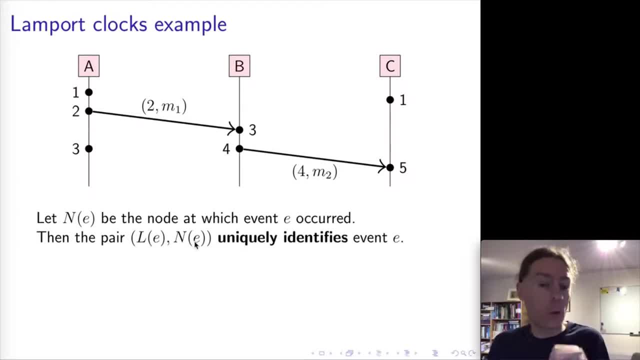 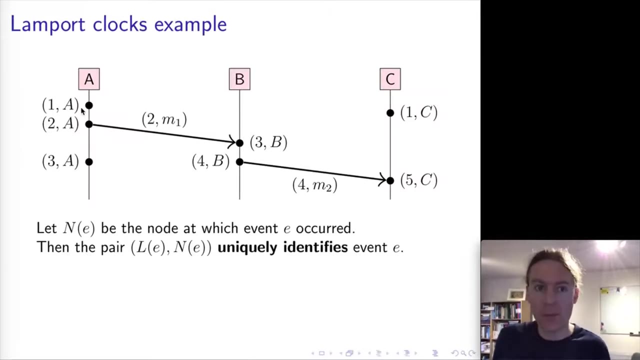 timestamp of an event with the name of the node at which that event occurred. those two taken together will uniquely identify a particular event. that combination is a unique identifier. so we could actually update this diagram here and instead of just having the timestamp at each, we have the pair of the timestamp and the node, and now we can see here: this event here has an identifier. 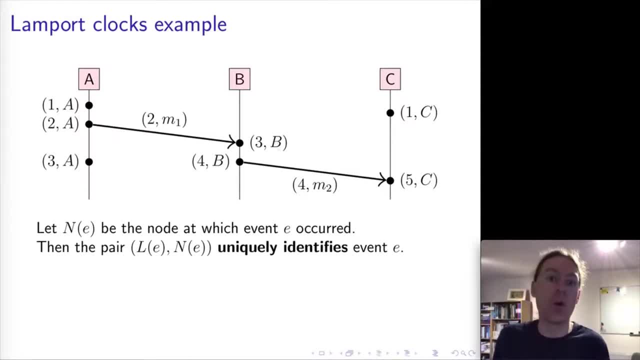 of three comma a, whereas this one here is three comma b. so they no longer have. they're no longer the same. Now there's one more thing that we can do with Lamport timestamps- and this is extremely useful, and that is, we can define a total order using those. so let's say we have two events, a and b. 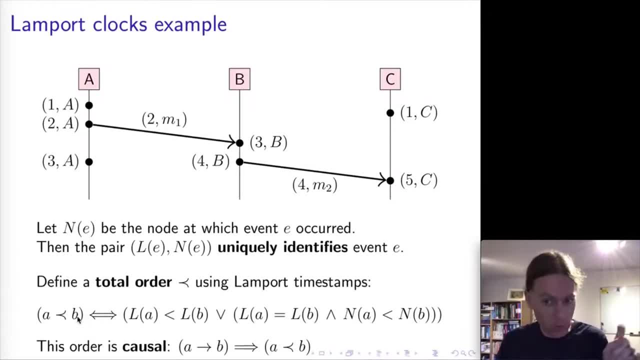 and we can define that a is less than b according to this little curly, less than symbol. here: a is less than b if, and only if, the Lamport timestamp of a is less than the timestamp of Lamport timestamp of b, or if a and b have the same Lamport timestamp but the name of a of the event, a. 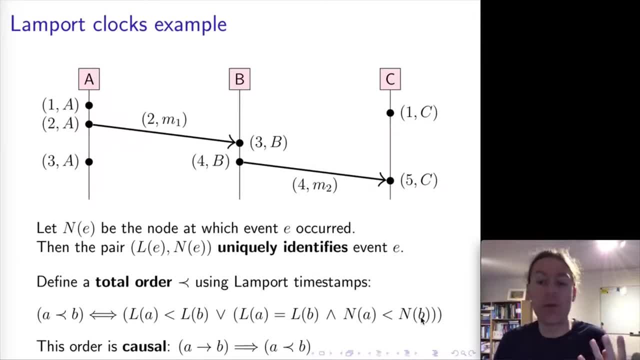 is less than the node name of event b. so this is assuming we have some way of comparing node names like a, b and c. we could just have like a lexicographic comparison of those, so that a comes before b and b comes before c, for example, and so this now means we can define an ordering. 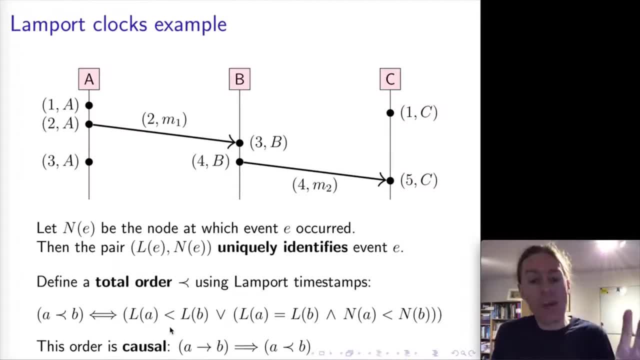 on these events by first of all looking at their Lamport timestamps and if the timestamps are the same, we break ties using the using the name of the nodes and this ordering. here it's a total order. that means for any two events. if they're distinct events, it is always. 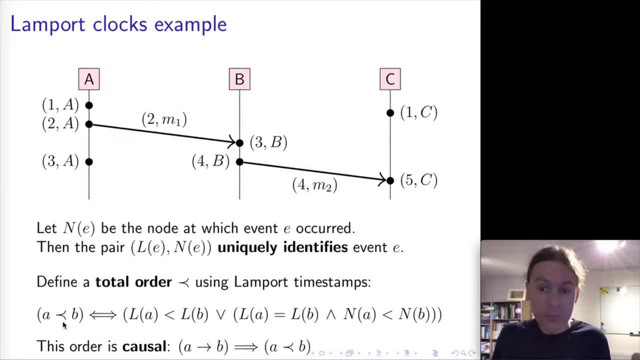 the case that either a is less than b or b is less than a. that's not a partial order that happens. before. relationship was a partial order, in which some events are incomparable if they are concurrent, but here this is a total order, which means any event that happened anywhere in the system. 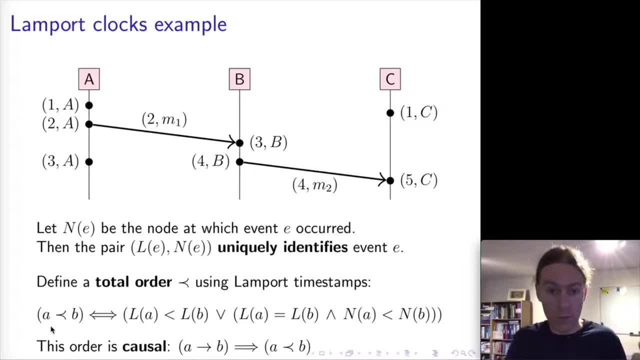 we can always put them one after the other according to this order, and this order is consistent with causality, which means that if event A happened before event B, then it is always the case that A is less than B according to this total order, And that follows directly from the fact that the Lamport timestamps 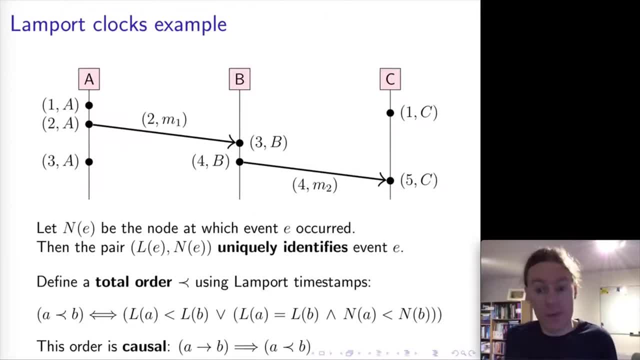 are consistent with causality. So that's what Lamport timestamps are. They essentially give us a way of attaching timestamps to all of the events in a system, in a way that captures the happens-before relationships. So we can now define this order, this total order over. 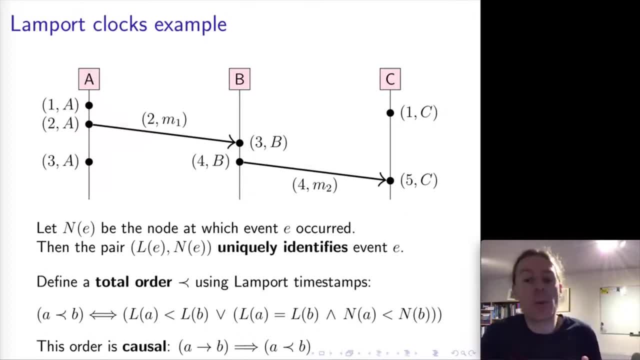 the events using their timestamps. So we can use the timestamps as a way of detecting the order of the events that happen in the system. And in our example of the moon being made of cheese, it would certainly be the case that the first message would have a lower. 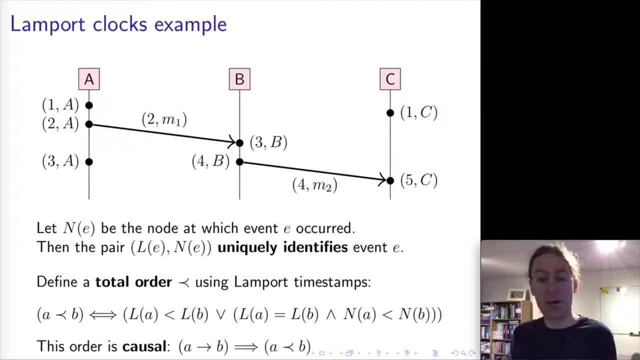 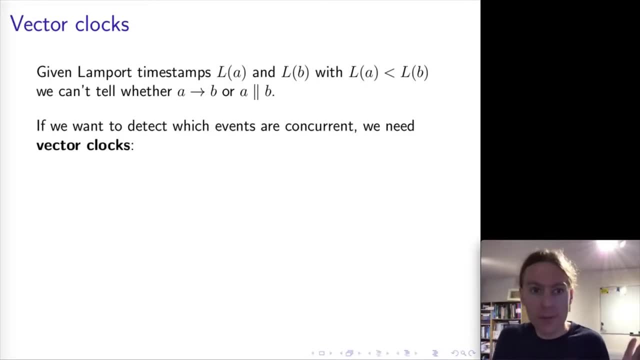 timestamp than the reply to that message. This is what Lamport timestamps, Lamport clocks guarantee, But there are still limitations, So Lamport clocks are not perfect. One limitation is that if you're given the two Lamport timestamps, L of A and L of B, and let's say L of A is less than L of B, you can't actually tell. 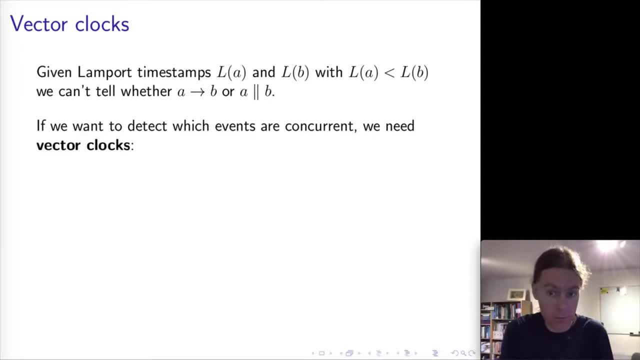 whether A happened before B or if A and B are concurrent. We can tell that B did not happen before A, because if that were the case, the Lamport timestamps would have to be the other way around. So we can tell something, but we can't actually tell the difference. 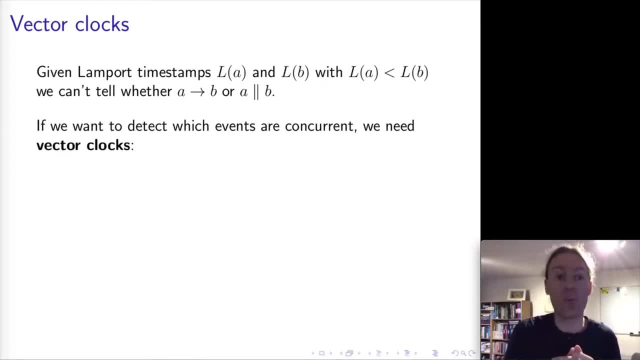 between two events that are concurrent and two events where one happened before the other. So it might also be useful to have a scheme of logical clocks in which it is It is possible to tell the difference between two events that are concurrent and two events where one happened before the other. And this is where vector clocks come in. So vector 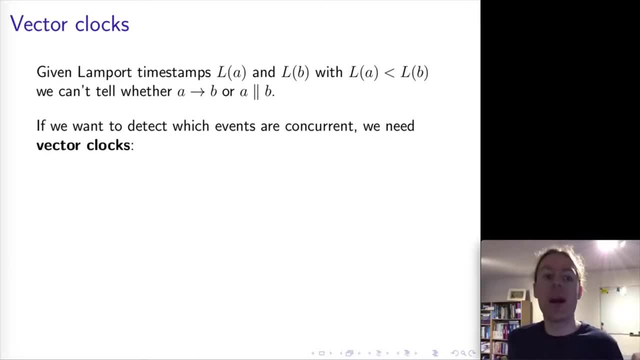 clocks are a different scheme. for logical time that allows us to tell this difference. So vector clocks work as follows. First of all we're going to assume we know the names of all of the nodes in the system. Let's say we have lowercase n nodes in the system and 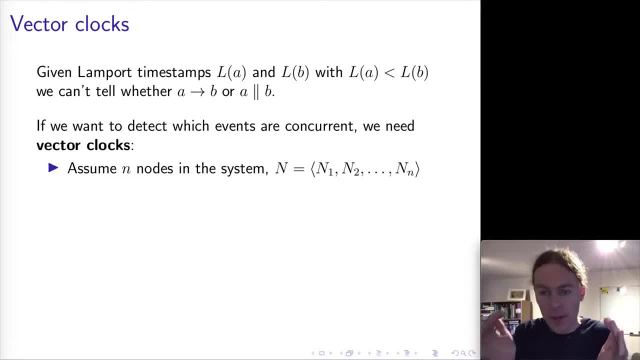 we're just going to put them in a vector. So this is an n-dimensional vector where each of the elements in the system are a vector, And we're going to put them in a vector. We can define timestamps to know which time stamps which are also vectors. 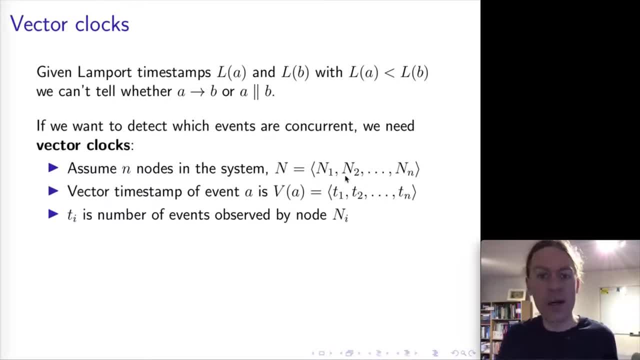 So in this case we have a timestamp here. This time stamp here consists of a sequence of integers, and we have one integer for every node in the system. Now this is written here using these angle brackets as vector notation. You could equally well think of this as a list or an array of integers. 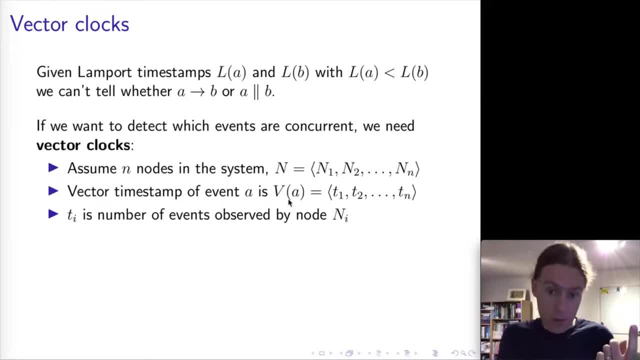 And so, In a better sense Now, for every event, rather than associating a single number with it, we associate this vector of numbers with each event, And the meaning of these numbers is that, for the ith entry in this vector here, ti, that is the number of events that we have observed happening on node i. 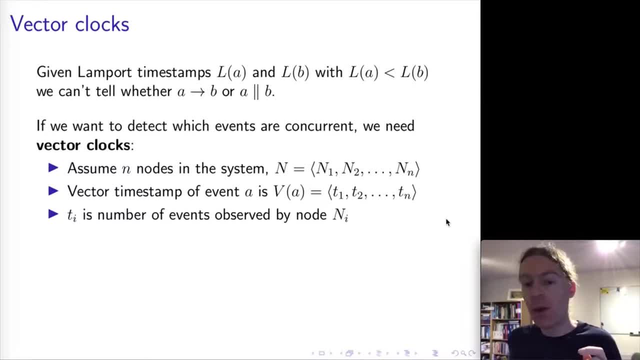 So we're counting events like we did in the Lamport timestamps, but now, rather than mixing all of the nodes together into a single counter, we actually have a separate counter for every node for the number of events that have occurred on that particular node. 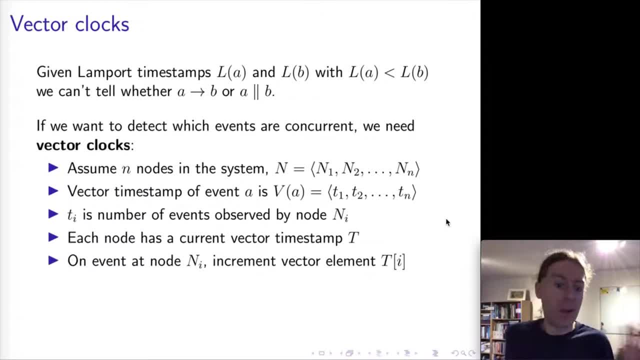 Now, like with the Lamport timestamps, we can attach a vector timestamp to every event and there are certain rules for updating these timestamps. So if we want to compute the timestamp for a particular event, the first thing we do is every time that an event occurs. 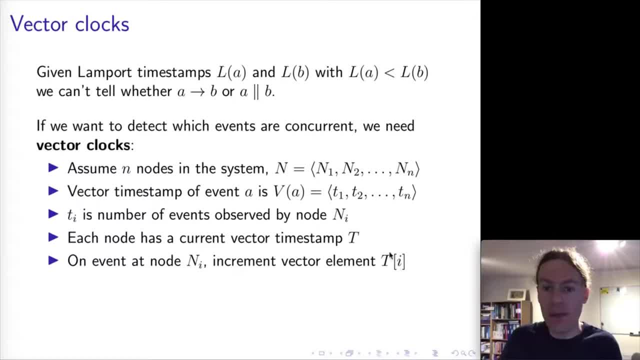 we increment the particular entry, the particular element of that vector corresponding to that particular node. So I'm going to just use these square brackets here, this notation, just like the array subscript in many programming languages. It's just a way of referring to the 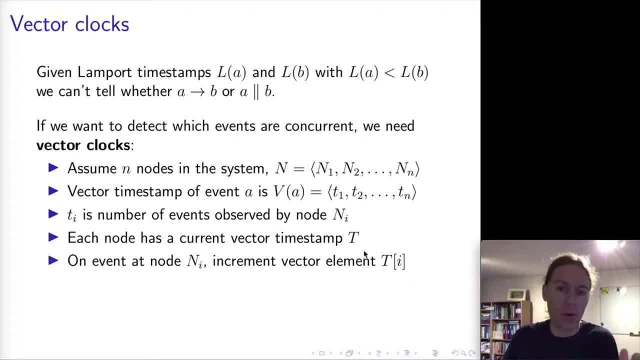 the ith element of this vector or this array ti. here, Like with the Lamport timestamps, we're going to attach vector clocks to messages that get sent over the network, and there's an algorithm to do that, So let's do that. 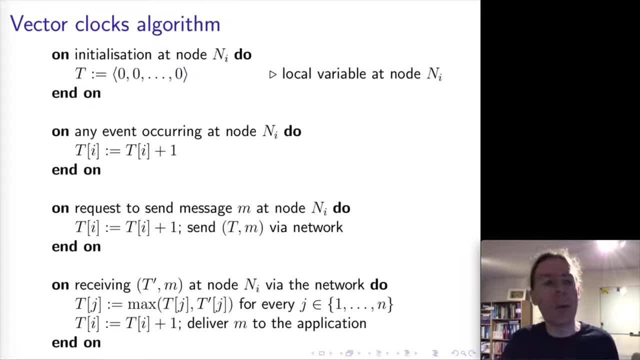 So let's look at this algorithm for merging those, and we're going to look at this algorithm now. So here we start in a way that is somewhat similar to the Lamport clocks and that is, every node locally has a timestamp. In this case, the timestamp is not just an integer, but it's a 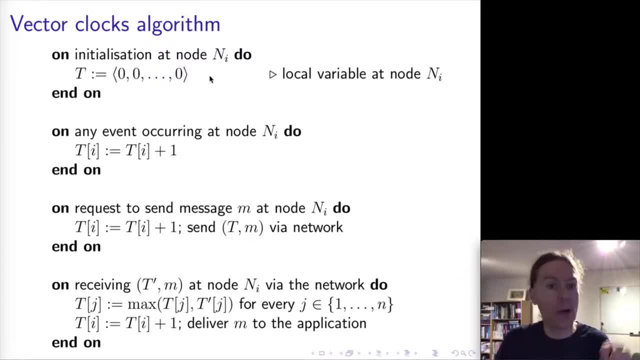 vector of integers which starts off as being all zeros. So we have one entry in this vector for each node in the system. So this is a vector that is n elements long here And we're going to increment the vector element corresponding to the node at which that event. 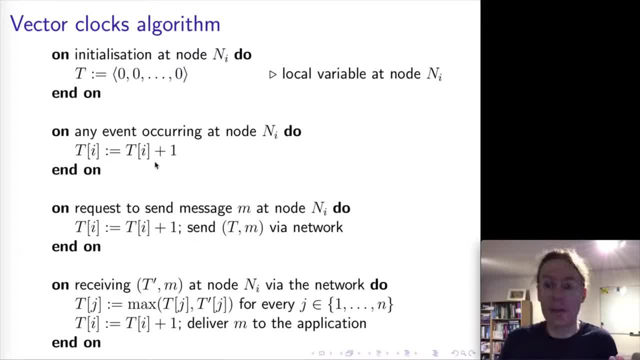 occurs. So an i processes some event, it increments its own entry in the vector. When we want to send a message over the network, again we increment our own entry in the vector, like for every local event, And then we attach the vector t to the message that gets sent over. 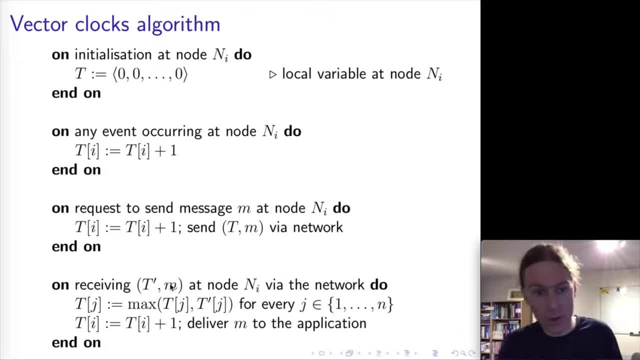 the network. Now, when we receive one of these messages over the network, say t prime is the timestamp in the message. Now we are going to merge the recipient nodes current local time t with the timestamp in the message: t prime. 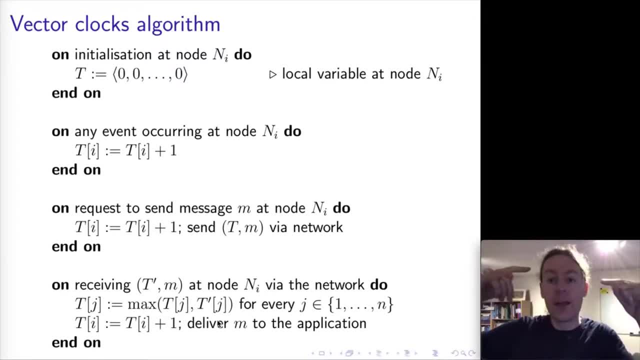 And the way we're going to merge those is we're going to go through the two vectors element wise, And so we're going to take the first element of t and the first element of t prime. we're going to take the maximum of those two and that becomes the first element of t. 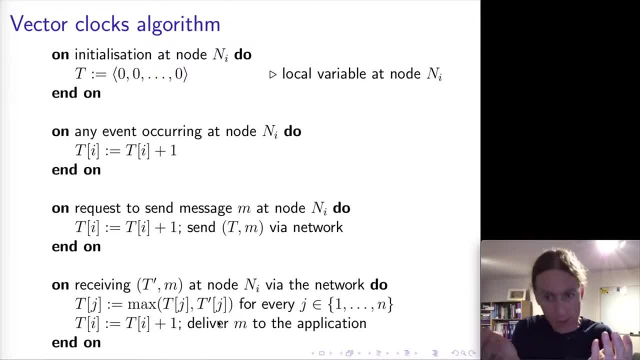 We're going to take the second element of t, the second element of t, prime, take the maximum, and so on. So, element wise, we take the maximum and the result is this: updated variable t here, Then again, we increment the local entry in t and we deliver the application. So let's look at: 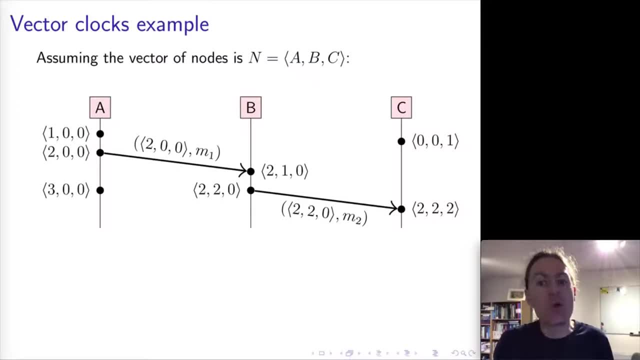 an example of what this actually looks like here. So I'm going to write my vectors as being: a is the first entry in the vector, b is the second entry in the vector and c is the third entry. And so when the first local event happens at a, that means a increments its own entry in the vector. 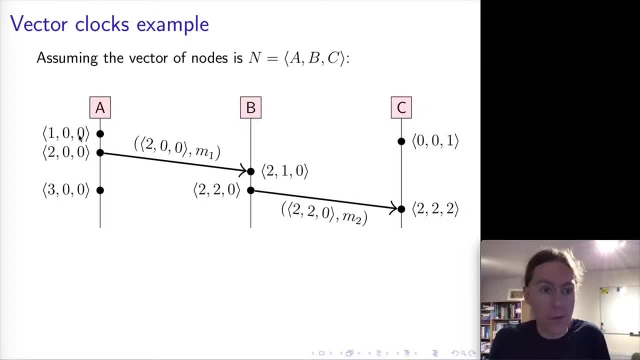 so that means the first entry becomes one and the remaining entries in the vector remain unchanged. On the second event, here again we increment its own, a increments its own entry. so this becomes two zero zero, and two zero zero is the vector that is attached to message m1 as it's sent over. 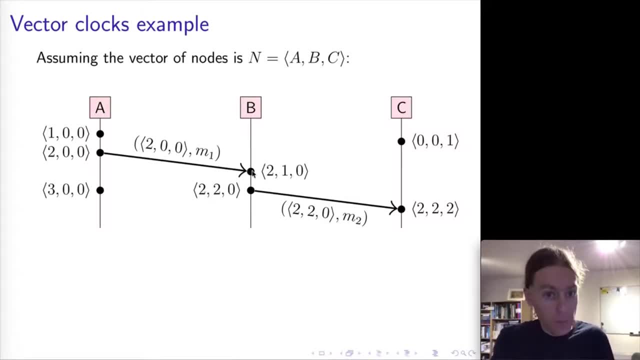 the network. Now, when two zero zero is received by b, it does the element wise maximum. so that means that it increments its own entry as well. So a time stamp gets sent over the network so it ends up with two zero zero and then it increments its own entry because this is b executing now. 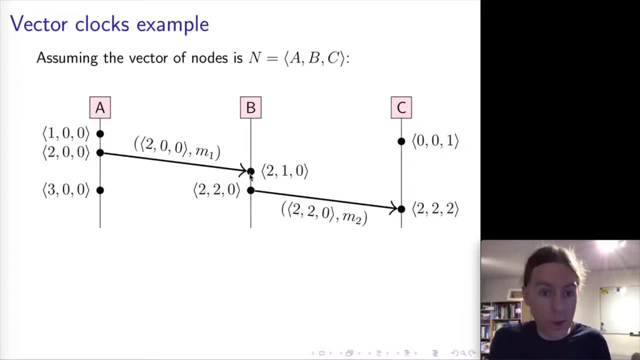 it increments the second entry of the vector clock, And so we end up with two one zero as the time stamp of this particular event. On the next event, by b, we have two two zero because again it's a local increment. Two two zero is the message, is the timestamp that gets attached to message m2,. 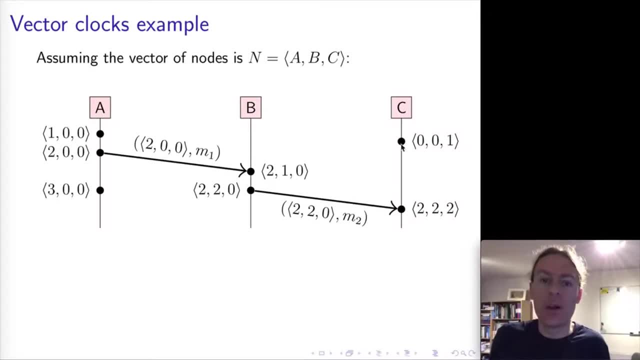 as it gets sent over the network, And again we have the element wise maximum here. when it gets sent over the network, we have the element wise maximum get received. So here, even though there was a previous event on C, that previous event will. 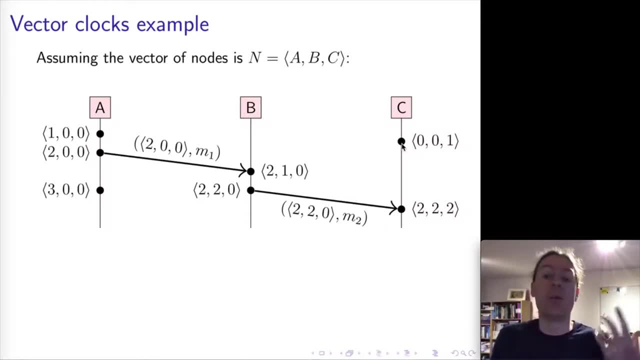 have had 0,, 0,, 1, because it's executed on node C, which is incrementing the third entry of the vector. But then here we do the element-wise maximum and the increment of C's entry, so we get: 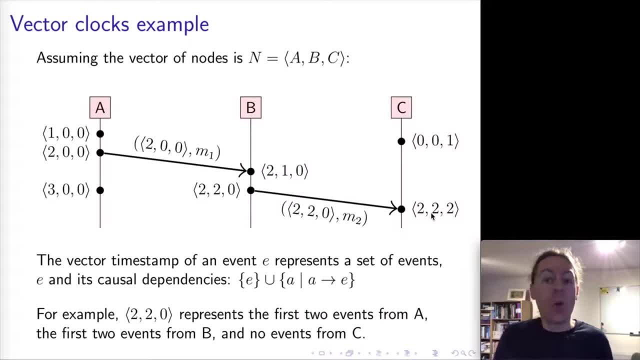 2, 2, 2.. So one way of thinking about these vectors here is that a vector represents a set of events, And so let's take, for example, this: 2, 2, 2, sorry, 2, 2, 0. here, the second event on B. 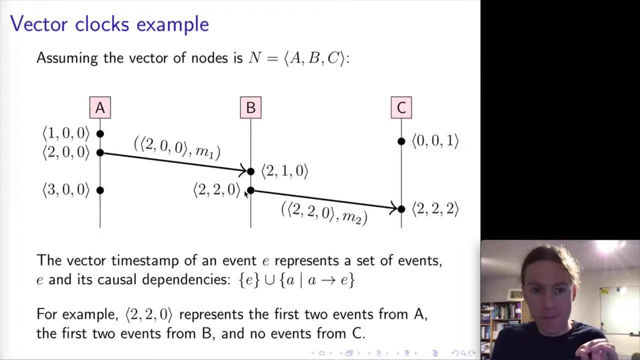 This represents the set of events, which is this event itself plus all of the events that happened before it. So if that's this event E, that's the set of E union, all of the events that happened before E, And so visually we can think of this in the diagram by traveling. 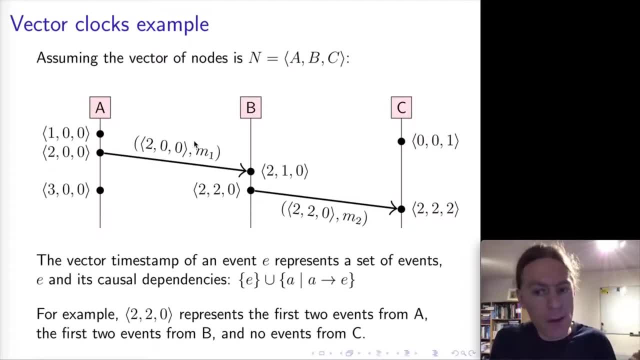 back and forth between the events that happened before E and the events that happened before E. So we can think of this in the diagram by traveling back and forth between the events that happened backwards in time and finding all of the elements, all of the events that we can reach. 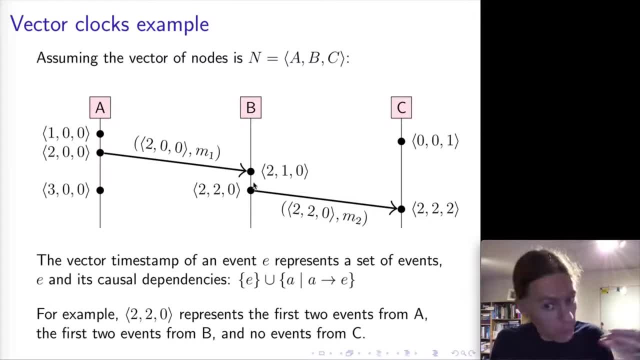 through tabling backwards, either on each node's individual execution order or by going backwards from the receipt to the sending of each sending of messages. And so here that means: from two to zero we can get back to two, one zero. we can get back to two zero zero and one zero zero. 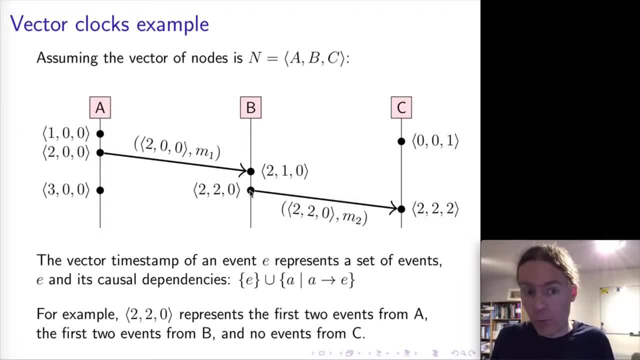 So we can reach these four events here by going backwards from two to zero. We can reach the first two events on A and we can reach the first two events on B, but none of the events on C, by going backwards from this event. 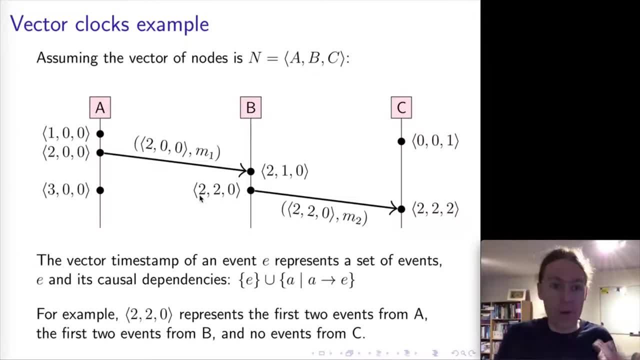 And that's why it has two to zero. It means the first two events on A, the first two events on B and no events from C. So here you can see this correspondence. There's a direct correspondence between these vectors and the set of events in the system. 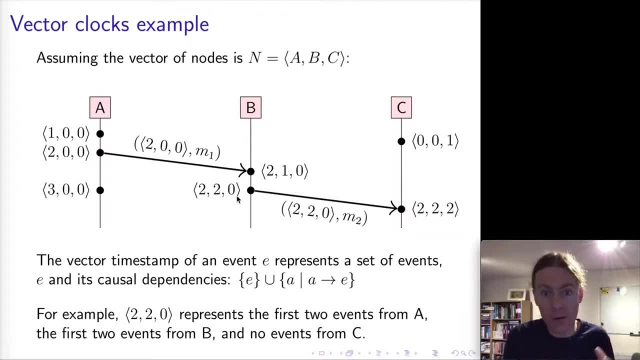 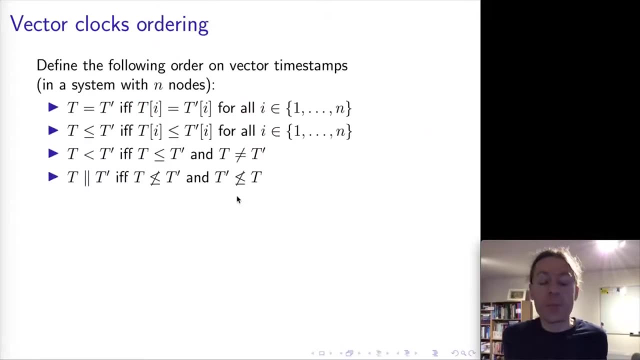 The vector is essentially a way of summarizing a set of events that occurred in the system simply by counting for each node from the start of that nodes execution. of how many events down do we go in? that nodes history. So now that we've defined these vectors, 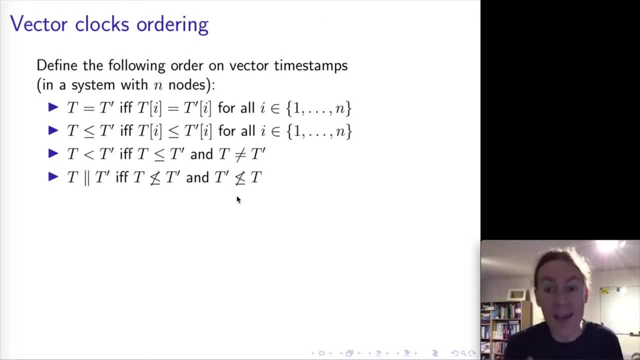 and the algorithm for computing the vectors. we can now compare them, And so, first of all, we're going to say that two vector timestamps are equal if each of the elements are equal. So T equals T prime. if, for each of the elements, T, subscript I equals T prime. 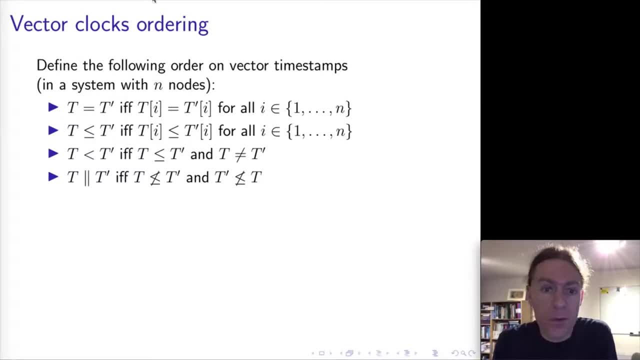 So this is just a straightforward equality. Also, similarly, we define the less than or equals operator, So T less than or equals T prime. if, element wise for each we compare the two vectors, look at the first element of T and the first element of T prime. 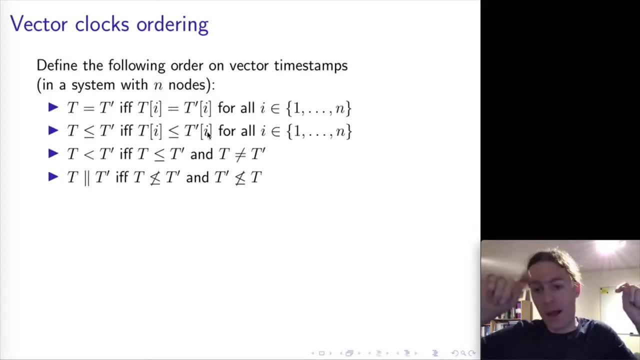 And if that's less than or equal and the second one is less than or equal and the third one is less than equal, If all of them are less than or equal, I can say that T the second one is equal, And so each of them is less than or equal. 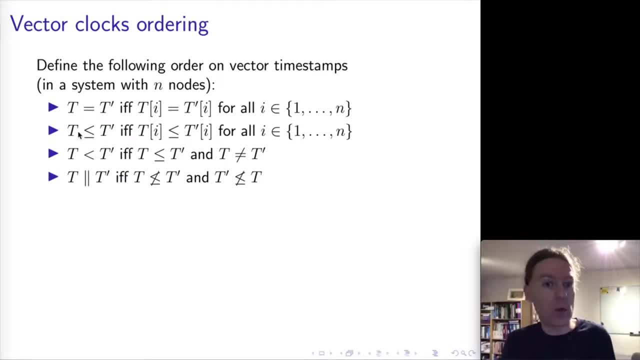 then we say that t as a whole is less than or equal to t' We can define strict inequality, strictly less than, simply as being t less than or equal to t' and then not being equal, which means that there must be at least one element in which they differ. 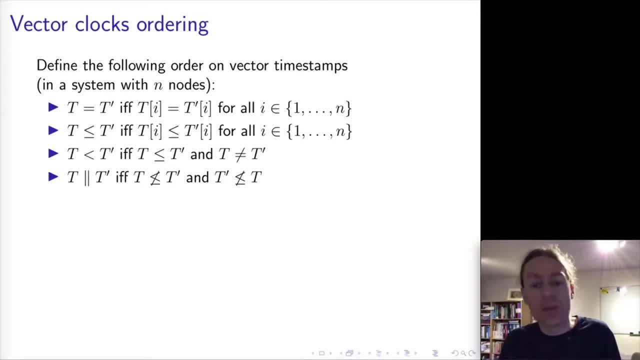 but they might be the same in all of the other elements. And finally, it is possible that for two vector timestamps, t and t', neither is t less than or equal to t', nor is t' less than or equal to t, And in that case we say that t and t' are incomparable. 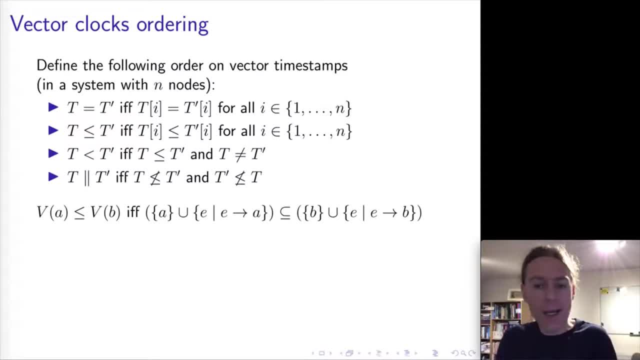 And now this: here you can relate back to what I just said about sets of events. So remember we said that here. this vector clock of a here corresponds to the set of events of a plus all of the events that happened before a. 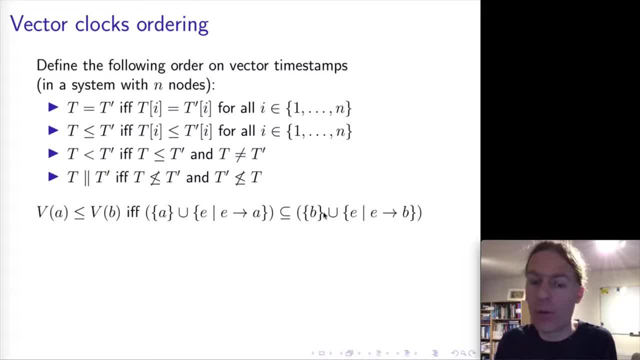 And the vector timestamp. The vector timestamp of b corresponds to the set of events b plus all of the events that happened before b And now. this less than or equal relationship on the vectors corresponds exactly to a subset relationship on those two sets of events. 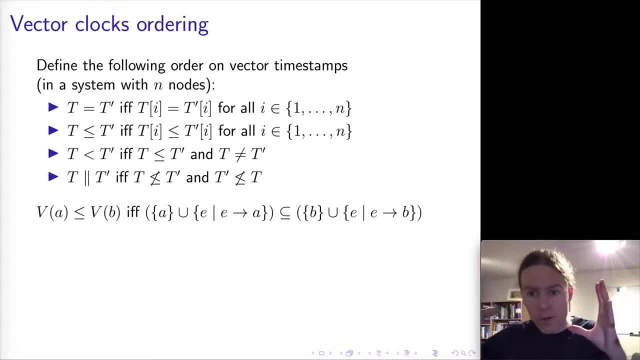 This is quite interesting. Now, this gives you a nice way of reasoning about what these vectors actually mean, because, since they correspond to sets of events, there's a subset relationship between the two, And it might Be the case that one is a subset of the other, or it might be the case that neither is a subset of the other. 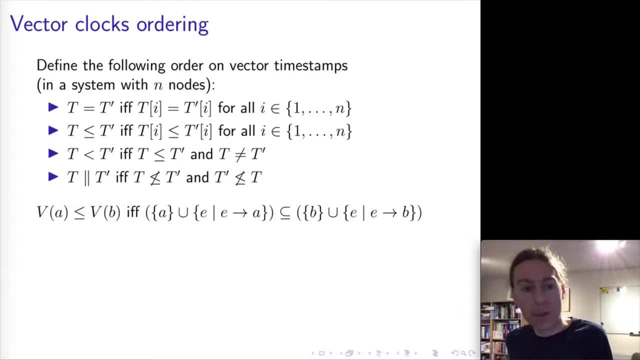 because there are some elements that they don't have in common. And so now this order that we have defined on these vector timestamps is very useful because it corresponds exactly to the happens before relationship. So it gives us a partial order, And this partial order is consistent with causality. 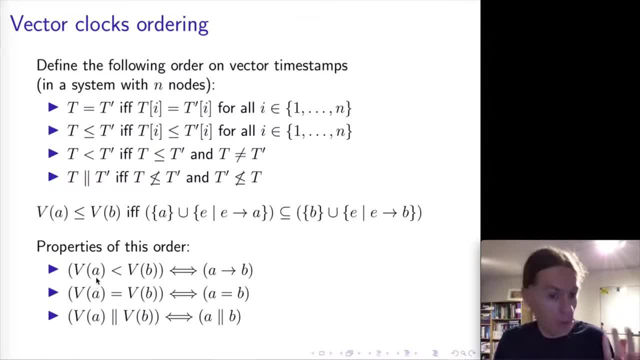 So first of all, we have the fact that, given two events, a and b, the vector clock, The vector timestamp of a is strictly less than the vector timestamp of b, according to this order above here, if, and only if, a happened before b. 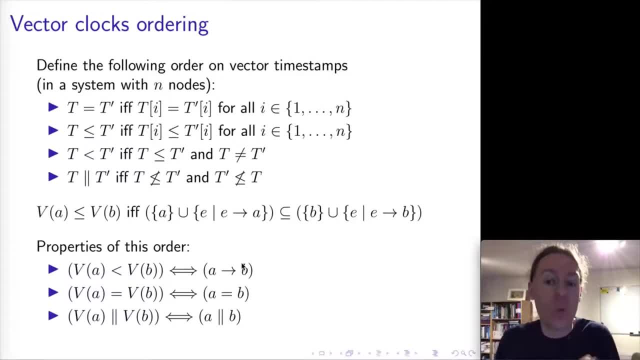 So this is now for the Lempel timestamps. We only had a one way implication. We had that if a happened before b, then the timestamps are less than one, less than the other. But with vector clocks we have an if and only if relationship. 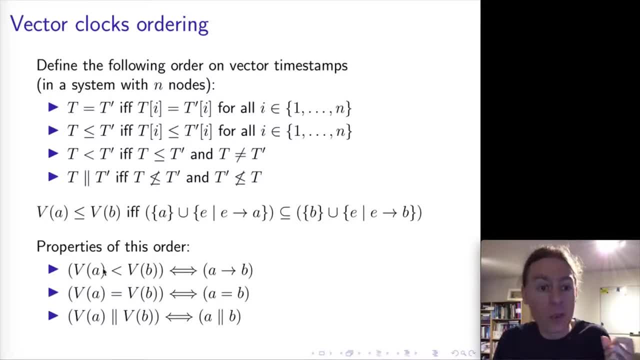 It's a bidirectional implication. So we can also conclude that, Looking at two timestamps, if one is less than the other, then we know that a must have happened before b. It's also the case that the timestamps uniquely identify events. So if two events have the same vector timestamps, that means that those events are the same. 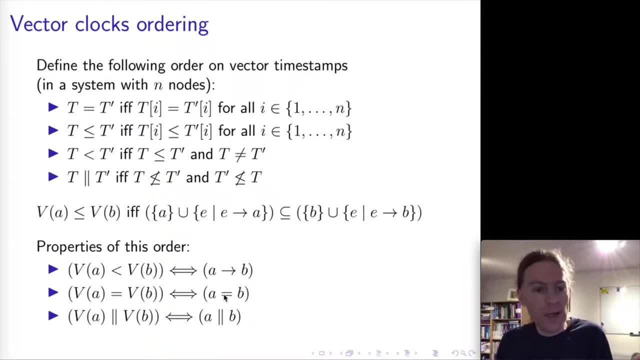 And so this is again a bidirectional implication. It's an only if and only if. And finally, if the two timestamps are incomparable, according to the definition up here, that means that The two events are concurrent. and if the two events are concurrent, then their timestamps will be incomparable. 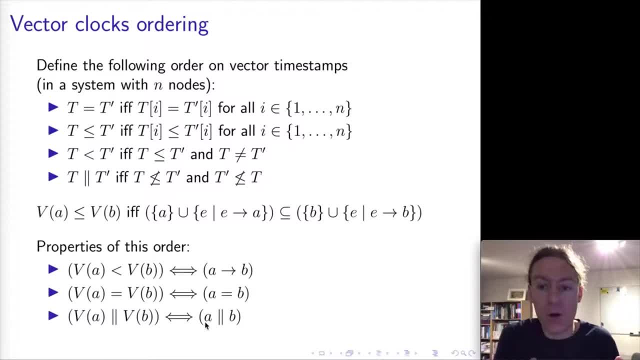 So what we now have here, using vector clocks, is a way of computing the happens before relationship. So far, the happens before relation has been essentially this abstract definition. We can, by looking at a diagram of the events on paper, we can work out what thing happened before which other thing, but that's not an algorithm for computing it. 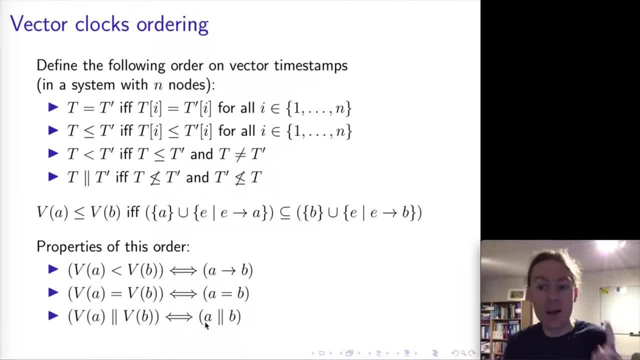 Whereas here with vector clocks, we actually have an algorithm for computing exactly Which event happened before which other event, and we have a way of telling whether two events are concurrent or not. So this is the really interesting thing about vector clocks that lamport clocks do not have. 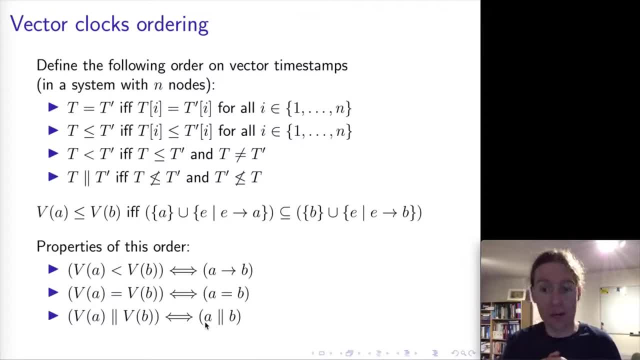 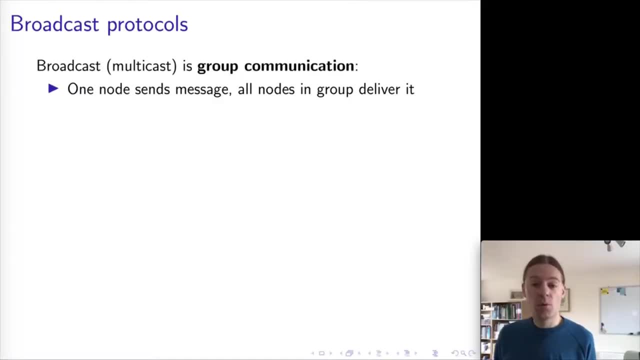 So these have been the two types of logical time that we're going to look at in this, in this section. Next, we are going to look at broadcast protocols. This might seem like a bit of a sudden jump from logical time, But actually, as we 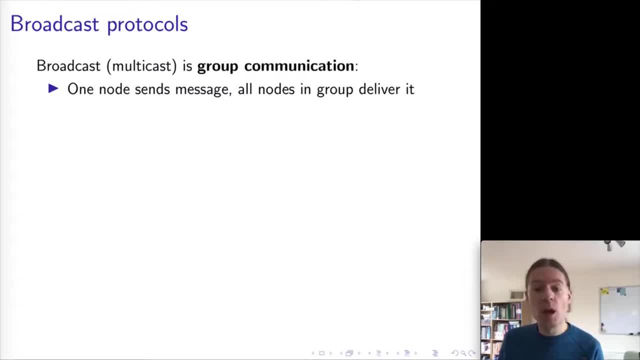 Will see in a moment. there's a strong connection between the two. So broadcast protocols generalize the type of network communication that we can do in a distributed system. So so far we've been considering point to point communication, where one sender sends a message to one recipient over the network. 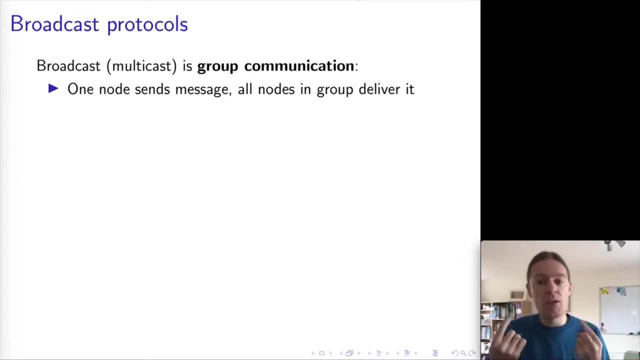 The message may or may not arrive, but it's still one to one communication between two nodes in broadcast or multicast communication. We generalize this to a group of Nodes so that one node may send a message to all of the nodes in the group at the same time. 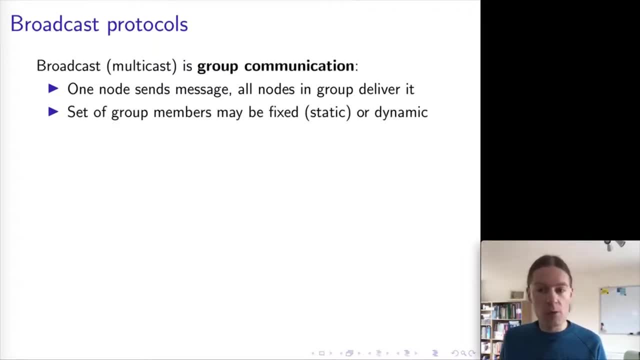 Now for this. for the purpose of this course, we're mostly going to assume that the set of nodes in the group is fixed and known in advance. But in general you may well, of course, have a system in which nodes can join and leave, or be added or removed by an administrator. 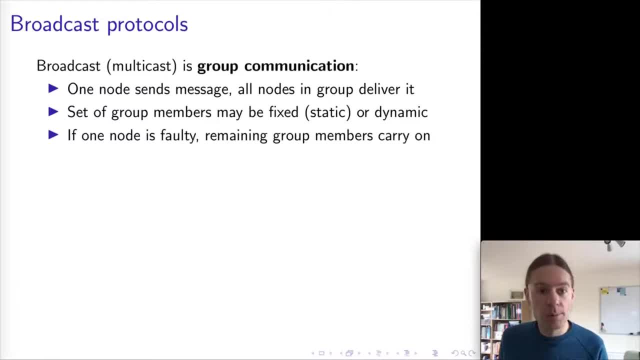 And that is certainly something that real protocols need to deal with. So one particular thing that we want of a broadcast protocol Is fault tolerance, and this means that, say, one of the nodes in the group is faulty, all of the remaining nodes should still be able to continue broadcasting and delivering messages as before. 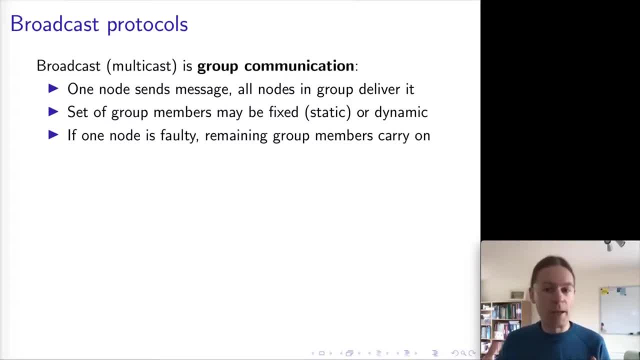 So we don't want a single faulty node to make the entire system grind to a halt. There are a couple of different implementations of broadcast or multicast. one that you might have come across in the context of computer networking is that some local area Network. 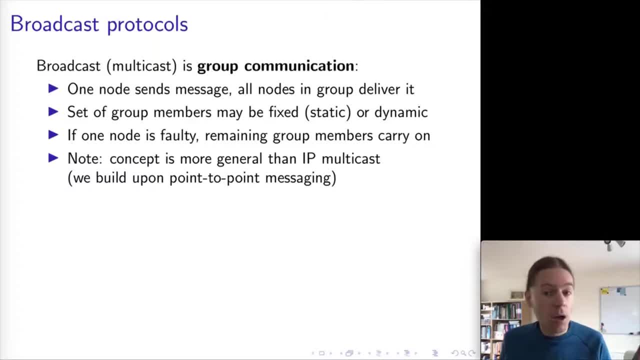 Networks support broadcast or multicast at the hardware level actually, and this is quite useful on local area networks. Generally, that kind of multicast does not work over the public Internet, And so what we will consider in this course is more general form of multicast or broadcast, where we assume that the underlying network only provides point to point messaging, as in unicast. 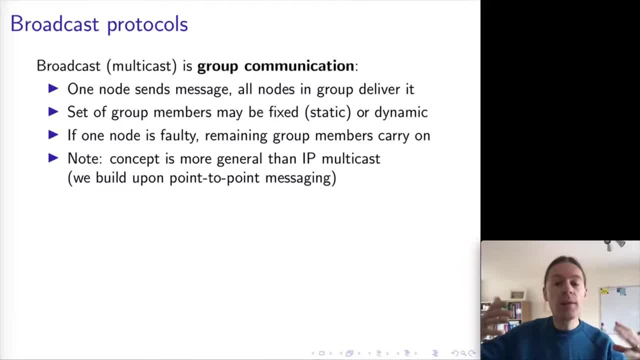 And we are going to build broadcast protocols on top of that. So the underlying network just allows us to send a message from one node to one other node, but on top of that we can build broadcast as an abstraction that we can then use for higher level protocols. 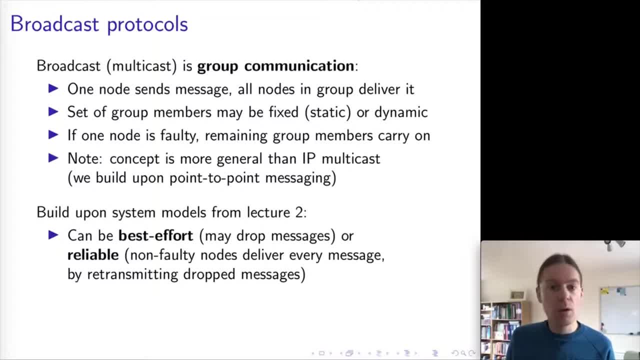 So if you think back to the discussion of system models in lecture two, we have the distinction between fair loss links and reliable links, And of course most network links are fair loss but you can make them reliable by retransmitting messages. 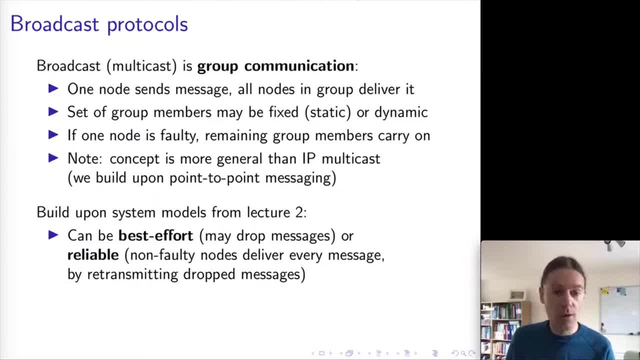 Exactly The same distinction happens in broadcast protocols, except here that a network that might lose message we call best effort broadcast. typically Best effort broadcast just means one node tries to send message to all the other nodes, but it may or may not arrive, especially if the sender crashes. 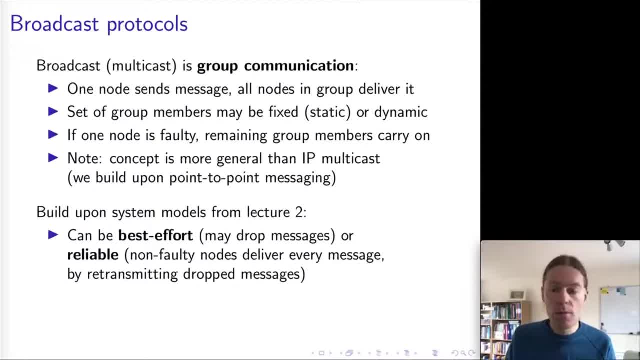 For example, the message might not reach all of the other nodes, Or we can make it reliable, which again relies on retransmitting lost messages. Like in the context of system models, we are going to assume not a synchronous system, not a synchronous system model, but an asynchronous or partially synchronous system model, which means that we're not going to assume any upper bound on message latency. 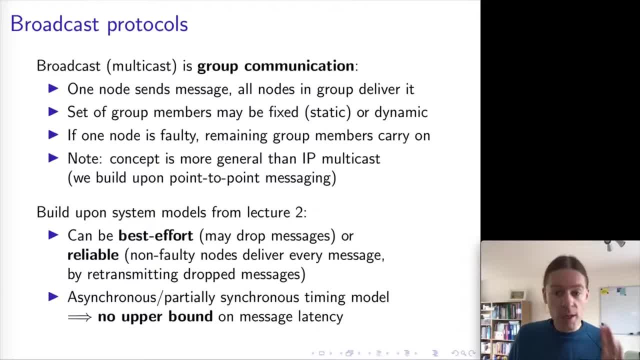 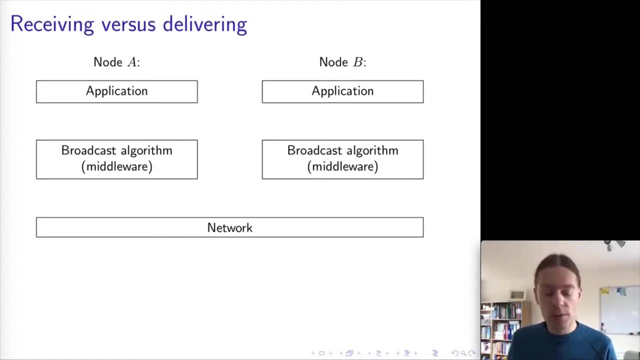 So in a reliable broadcast protocol we can say that the message will eventually get through, but we're not making any promises about how long it might take until the message might get through. Okay, So That's the background on broadcast. I should introduce a little bit of terminology before I get into the details. 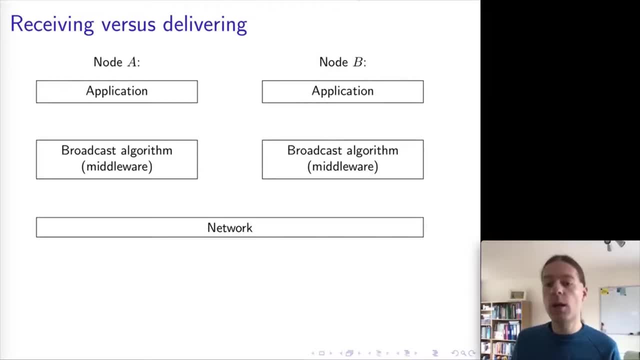 And that is in the context of point-to-point network links. we have talked about sending and receiving messages over the network, Whereas in the context of broadcast protocols we talk about broadcasting a message and then delivering it as the counterpart. So what happens is the application on one node wants to broadcast a message to the entire group. 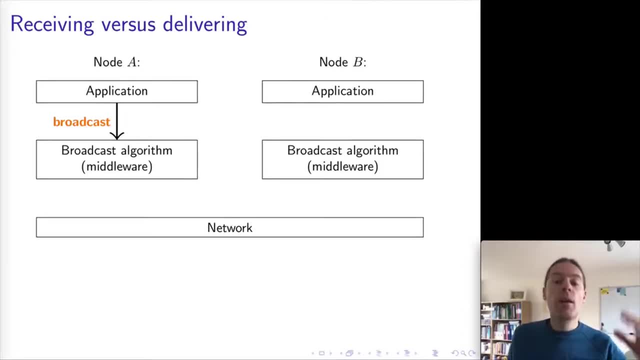 We call this action to broadcast, And then the underlying broadcast algorithm may send or receive multiple messages over the network And these are then point-to-point messages that are sent or received And on some other node those messages might be received. They get again picked up by the broadcast algorithm and the broadcast algorithm at that point then, at some point then delivers the message to the application. 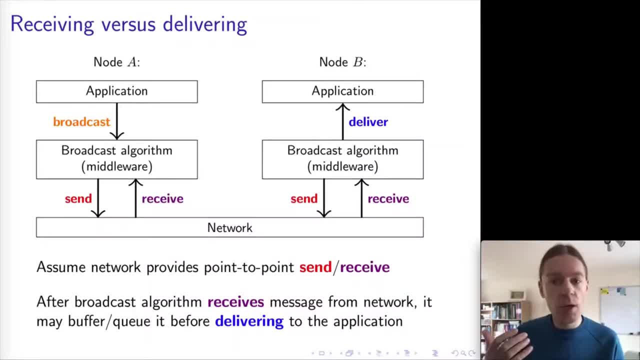 So here the delivery is the counterpart to the broadcast. Okay, And one detail that happens here is that when the broadcast algorithm receives a message, it might not immediately deliver that to the application. It may actually have to wait for a little bit before that message is ready to be delivered, because we want to ensure that the messages are delivered in a certain order. 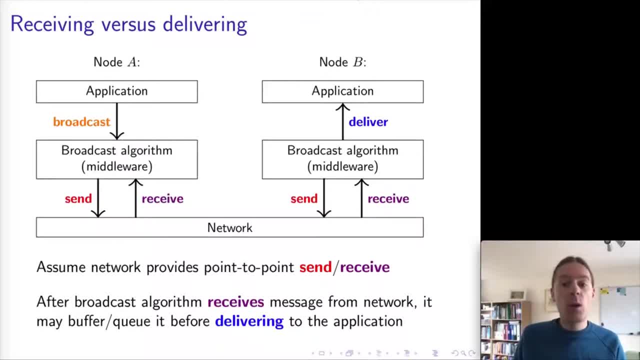 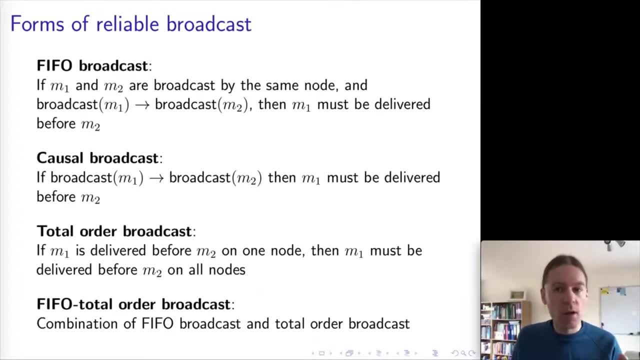 So this is just the terminology. We are now going to look at a couple of different broadcast abstractions And I'm going to talk about each of them, And I'm going to talk about each of them. I'm going to talk about each of these individually, so I won't go into too much detail right now. 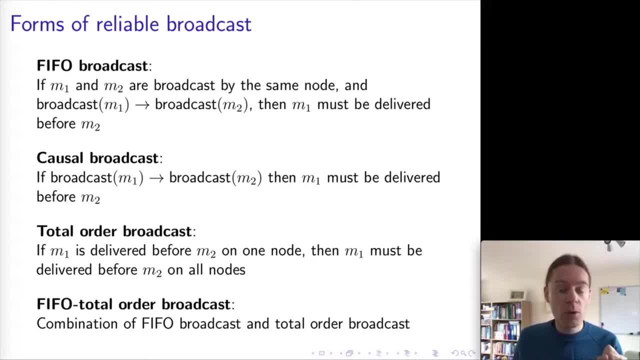 The point here is that these are all forms of reliable broadcasts, So we're assuming we have a mechanism for retransmission which ensures that all of the messages eventually get through. Now we want to distinguish different types of broadcasts based on the order in which messages get delivered. 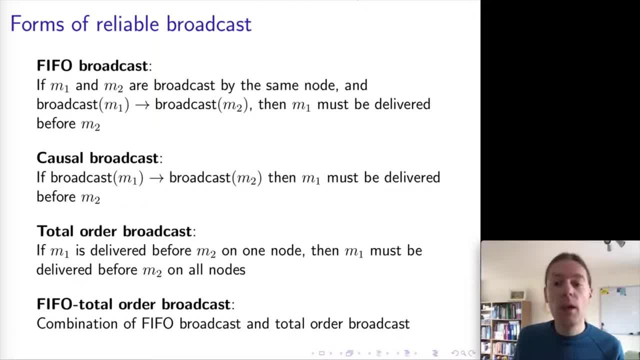 And so the first one that we're going to look at is FIFO broadcasts, And in FIFO broadcasts, the ordering property is that If two messages are broadcast by the same node, then all nodes will deliver those messages in the same order as they were broadcast. 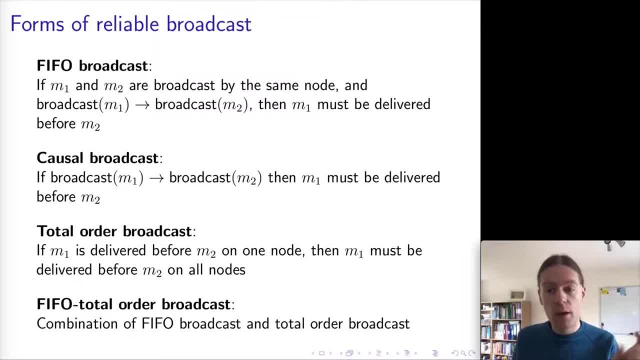 So for any messages broadcast from one particular node, they remain in order, But for any messages broadcast by two different nodes, there's no guarantee about the order in which they might arrive. So let's look at an example of what this actually looks like. 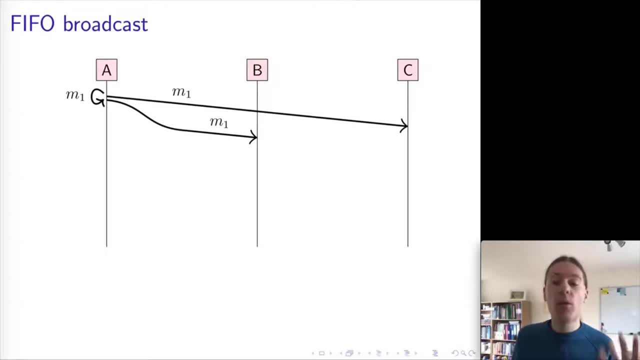 So here we have again three nodes: A, B and C. A wants to broadcast message M1 to the group, And so It sends that message over the network to C and to B, And notice also that A sends the message to itself, which is here denoted by this little loopback arrow. 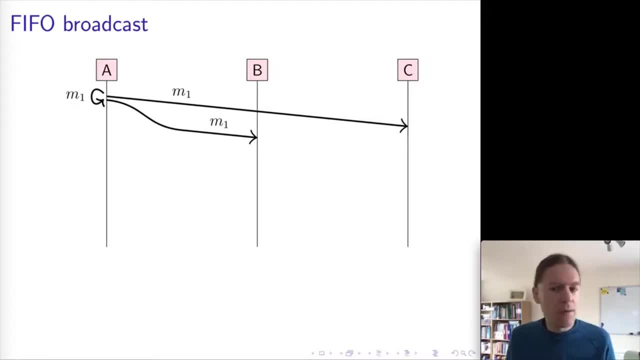 Now this might seem unnecessary, because why do you need to deliver a message back to yourself? Because the sender of the message already knows what message it has sent. It doesn't need to receive it again. The reason why a node delivers a message to itself will become apparent. 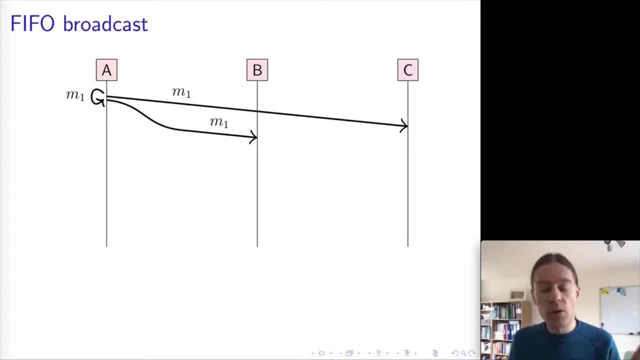 When we talk about total order broadcast shortly. So for now just assume this as a little quirk- that the guarantee of the broadcast protocol is also always that it delivers a message to itself. Then, after M1 has been delivered, node B decides that it wants to broadcast message M2 to the group. 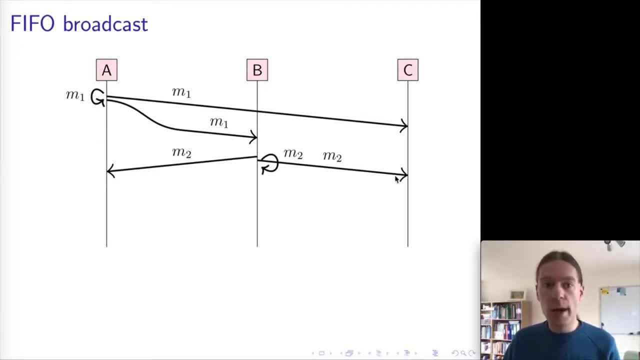 And so it sends M2 of the network to A and C and it also delivers M2 to itself. And then, finally, node A wants to broadcast message M3. So again, it sends that message over the network to B and C and it delivers M3 to itself. 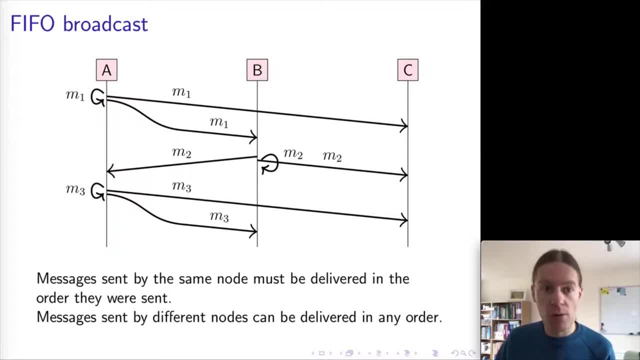 Okay, so this is FIFO broadcast. So what we require- FIFO broadcast, as I said just now- is that, because M1 and M3 are both broadcast by the same node A, we require that all nodes deliver M1 before they deliver M3.. 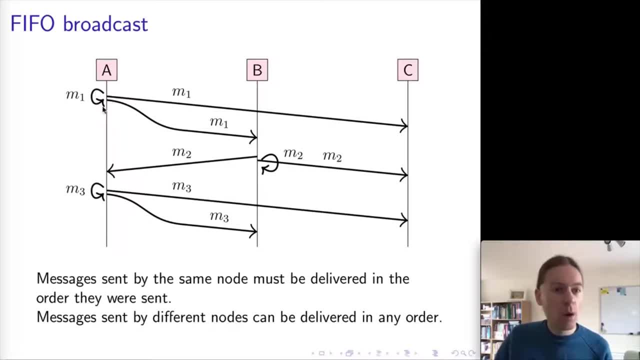 And we can check that this is the case here. A delivers M1 here and then delivers M3. Okay, B delivers M1, then delivers M3, and C also delivers M1 and then delivers M3.. Okay, all fine. 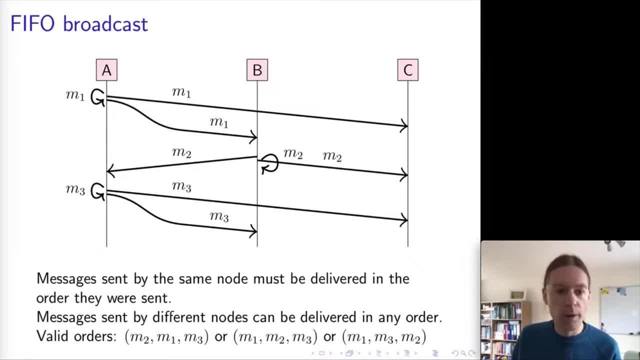 All of the nodes deliver these messages in the right order. Now there are actually several possible orders that would be valid here under FIFO broadcast, In particular the message M2 that is sent by B. that can be ordered arbitrarily with respect to A's messages. 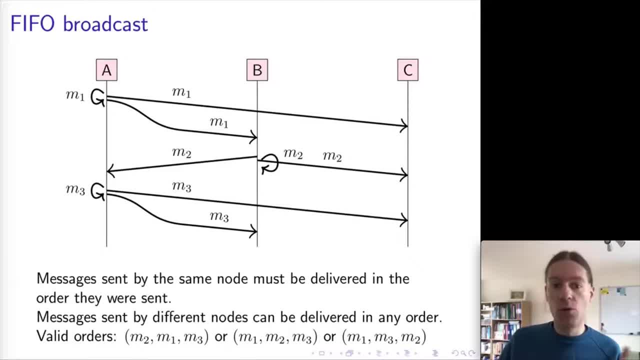 Because we are not making any guarantees about ordering across different nodes and M2 was sent by B, So this means that it's okay for M2 to be delivered before M1 and M3, or in between the two or after the two, and all of those are fine. 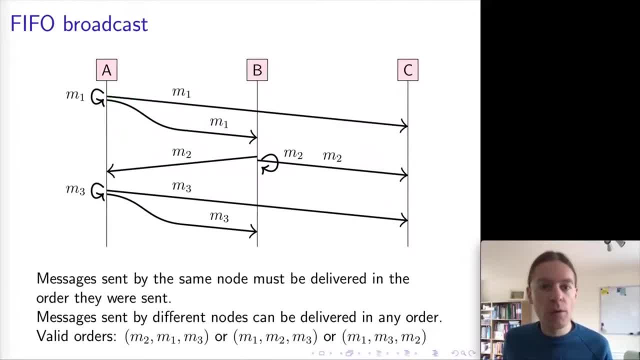 And so here, for example, we can consider these two different executions, in which the messages are delivered by C in a different order. So in this case here M1 is delivered first, then M2, then M3.. In this case M2 is delivered first, then M1, then M3. 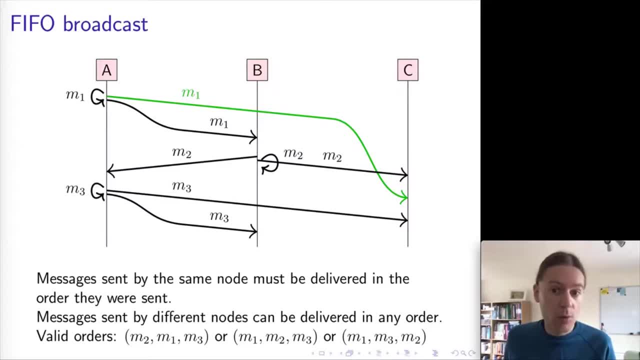 And both of these orders are valid under FIFO broadcast, Even though in this case, here, for example, the message M2, you would say that happened after M1 in a causal sense. But still, FIFO broadcast makes no guarantees about delivering M2 after M1. 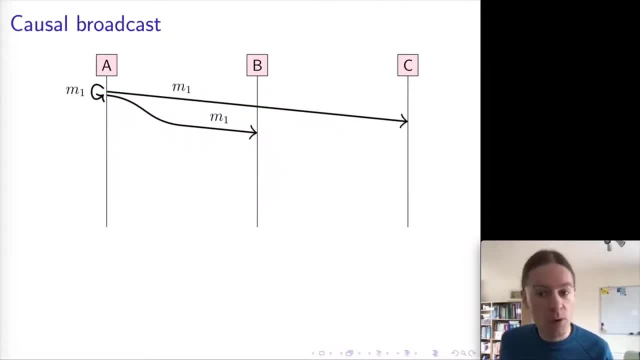 If you do want that kind of ordering property, you need causal broadcast. So causal broadcast It ensures that messages are delivered in causal order and that means that if the broadcasting of one message happened before the broadcasting of another, in the sense of the happens before- 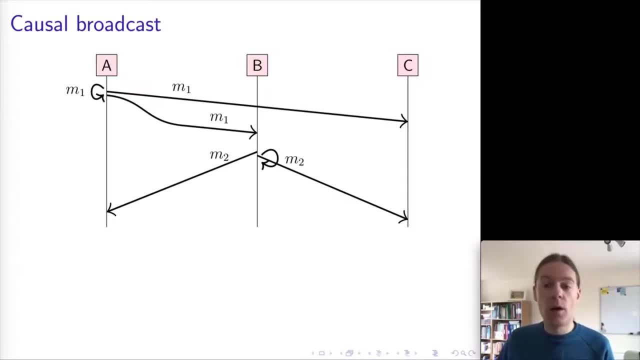 relation, then those messages must be delivered in that order that matches the happens before relation And that's what we have here. So, first of all, M1 is broadcast by A and it's received by B and C and it's delivered. 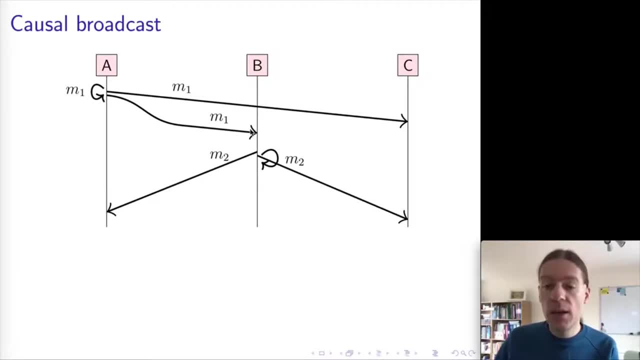 by B here, And then, after B has delivered M1, M2 is delivered by A, And then, after B has delivered M1, M3 is delivered by A, And then, after B has delivered M1, M3 is delivered by A, Then, after B has delivered M121, they are the same two messages that. 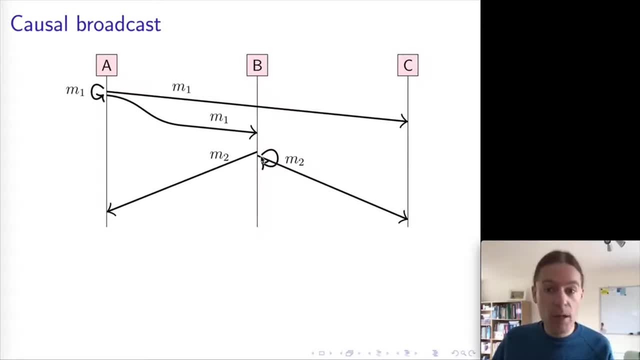 they are sent by M1.. B wants to broadcast M2. And so here M2 may have a causal dependency on M1. And therefore we require that all of the nodes must deliver M1 first and M2 second. Next, the node A might broadcast a message M3. 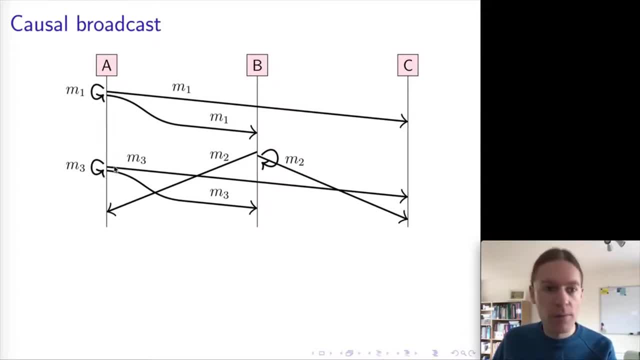 Again, it sends that over the network to the other two nodes and it delivers the message to itself. And in this case, notice that the broadcast of M2 is concurrent with the broadcast of M3.. on A, M2 is delivered after M3 is broadcast and on B, M3 is delivered after M2 is broadcast. 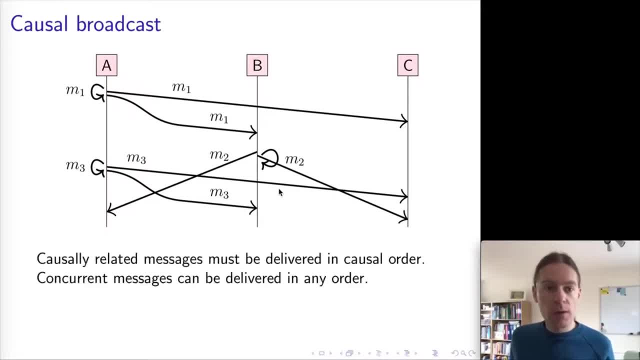 So these two messages do not depend on each other. So in this case here what we require is that any messages that have a causal dependency are delivered in causal order, And so in this case here we have a causal dependency between M1 and M2, and we have a causal dependency between M1. 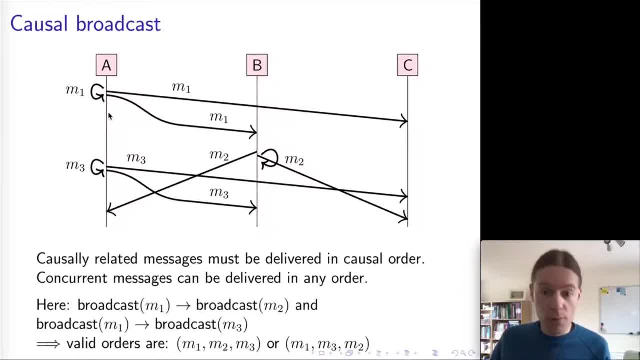 and M3, because M1 and M3 were broadcast by the same node A, But there's no causal dependency between M2 and M3. And so this means M2 and M3 can be delivered in either order, which means that here again we have two different orders of delivery for C, and both of these are okay under. 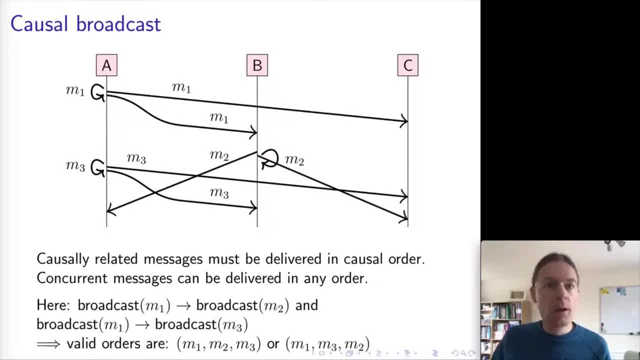 causal broadcast. So here, in this case we have C first delivering M1,, then M3,, then M2.. In this case, here we have C first delivering M1,, then M2,, then M3, and these are both valid orders. We can swap around. 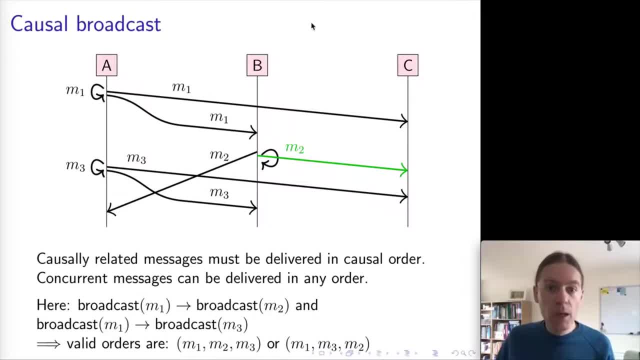 the delivery order of M2 and M3.. Now notice here, for example, that A delivers first M3, then- Sorry, first delivers M1, then M3, then M2, whereas B delivers first M1, then M2, then M3. 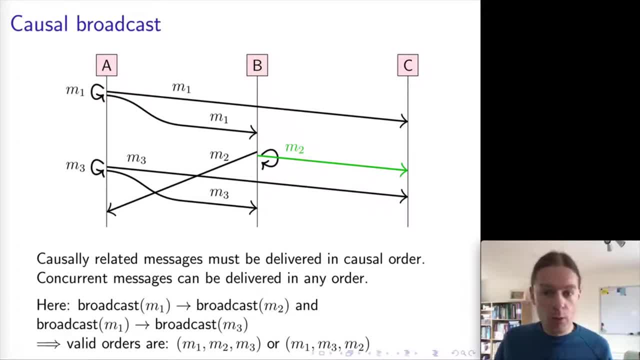 So both of these orders are valid causal orders, but they are not the same, And in some cases they are not the same. So in this case here we have C first delivering M1, then M2,, then M3.. In some cases we actually want to require that all of the nodes deliver messages in. 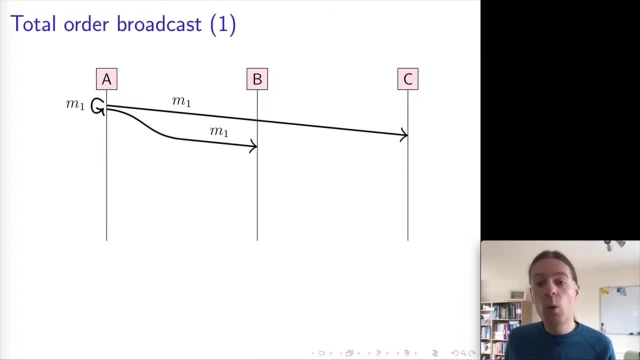 the same order, And if that is what we want, we need to move to what is called total order broadcast. So total order broadcast puts all of the messages that are broadcast in the system into a total order. That means it's always clear which one came first and it. 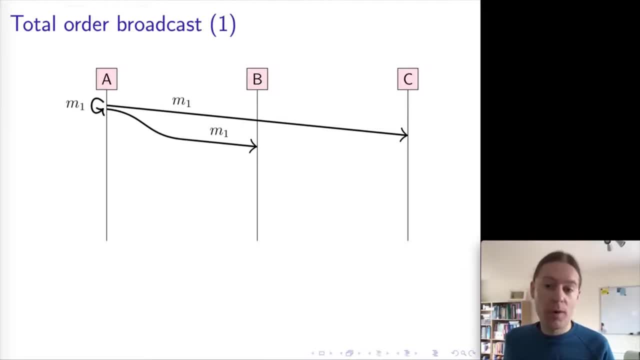 ensures that all of the nodes deliver messages in that same order. So there's agreement between all of the nodes on the order in which the messages should be delivered. So in this example again, we start with M1, broadcast by A, then we have M2 broadcast by B. 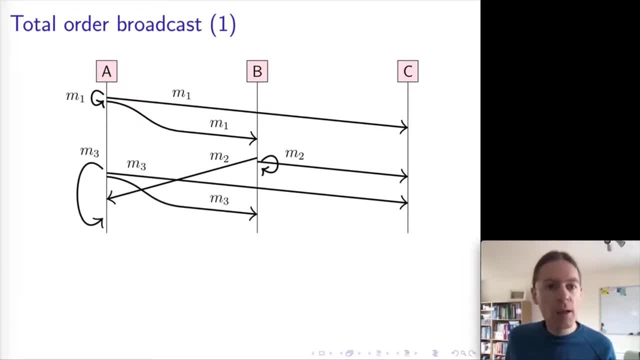 which happens after M1.. And finally, we have a message M3 that is broadcast by A again. Now, in this case, something somewhere has to decide on the order in which these will be delivered. Let's say that the order that was decided is to deliver first M1, then M2, then M3. 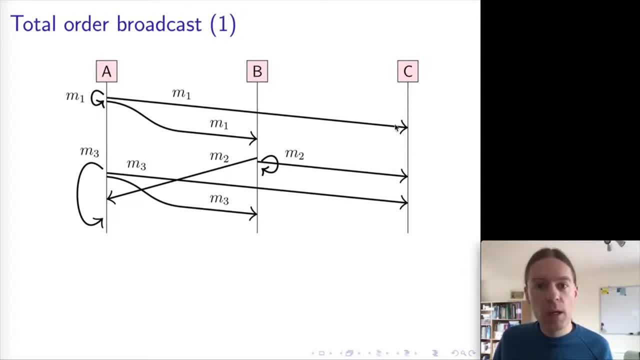 Okay, And so we can see. on C, for example, that's what happened. C first delivers M1, then it delivers M2, then it delivers M3.. So C is delivering them in the correct order. Let's look at B here. B first delivers M1, then it delivers M2 to. 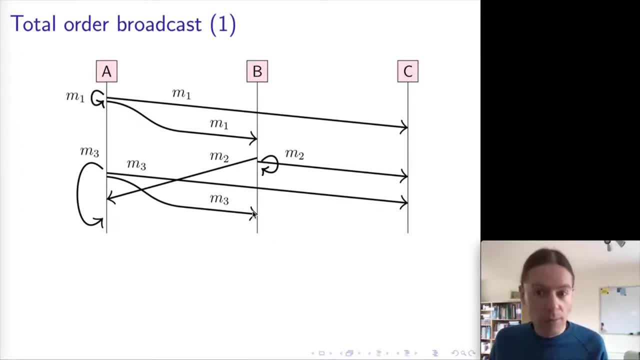 itself, then it delivers M3.. Okay, So B also delivers the messages in the correct order. Let's look at node A here. Node A first delivers M1 to itself, then it broadcasts M3. But wait, it's not allowed to deliver M3 to itself yet, because the order that was decided. 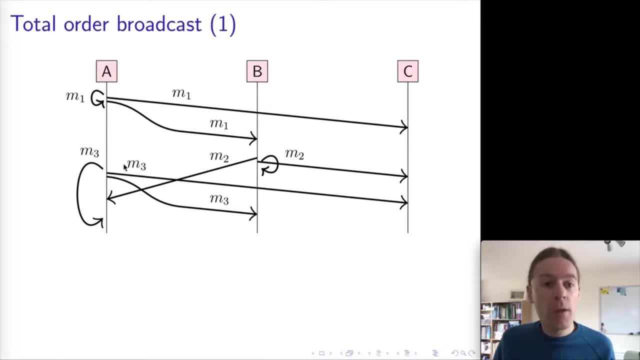 is that M2 must be delivered before M3. So therefore, node A cannot immediately deliver M3 to itself. Instead, it has to wait for first for M2 to arrive and M2 to be delivered by A, and only then is A allowed to deliver M3 to itself. So this is now where this delivery to 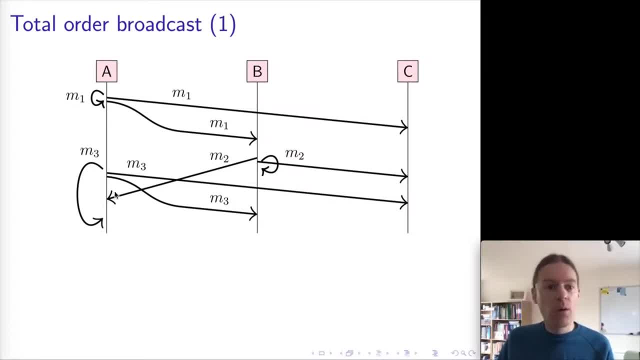 itself becomes very interesting and crucial, because you can see that sometimes there has to be a delay. if a node wants to deliver a message to itself, Now, here, M1, M2, then M3 is one possible order of delivering these messages. It could also be that we decide on a different order. 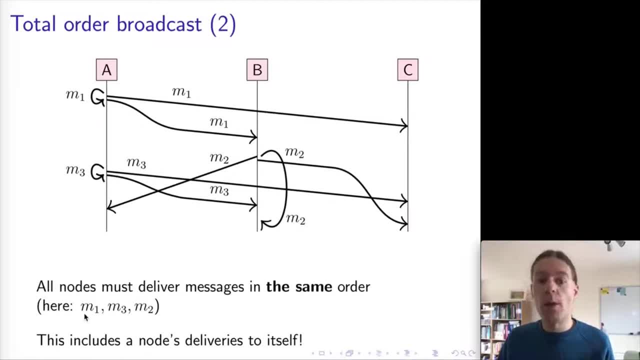 So a different valid order might be for the delivery order to be M1, M3, M2. And that is also fine as long as all of the nodes deliver the messages in that same order. And so here again we have start with C, so C first delivers M1, then M3, then M2.. Notice here that it's possible. 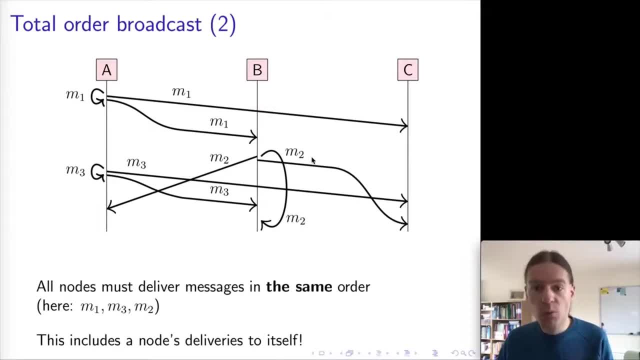 that C receives M2 over the network before it receives M3, in which case C will have to delay the delivery of M2 until after M3 has arrived. So here this is called a holdback. In the broadcast algorithm, it's often necessary for a message to be held back if it's not yet ready to be delivered. 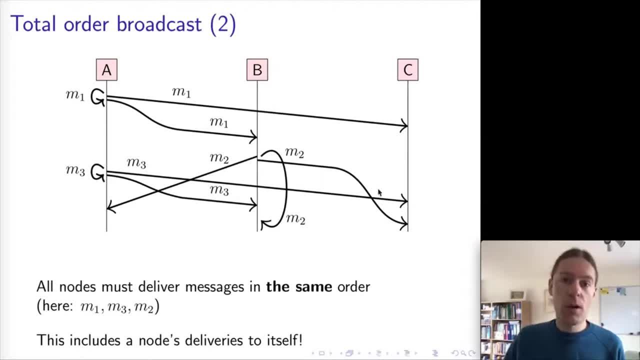 because if we're waiting for some other message to arrive first- and that has happened here in the case of C In the node B- for the delivery order to be 1,, 3, 2,, well, first we deliver 1, then M3, but we can't sorry, then we broadcast. 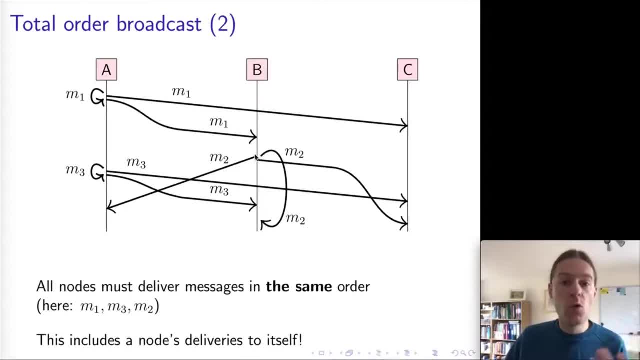 M2, but we can't immediately deliver M2 to ourselves. We have to first wait for M3 to be delivered and then we're allowed to deliver M2 to ourselves at B And on node A things are simpler now. So first we deliver M3 to ourselves and then we're allowed to deliver M2 to ourselves at B. 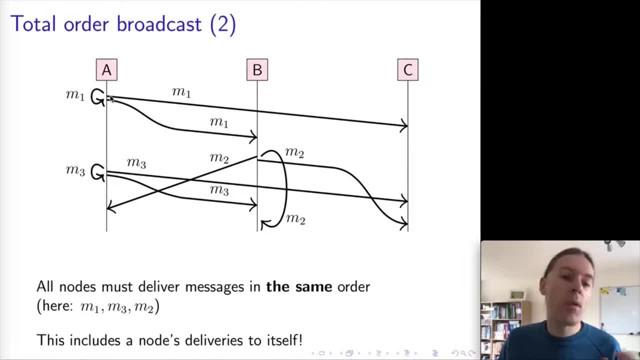 First we deliver M1 to ourselves, then we deliver M3 to ourselves and finally M2 arrives over the network and we deliver M2 to ourselves. So both of these here are valid executions of total order broadcasts. The crucial thing is just that, whatever order the messages get delivered in, 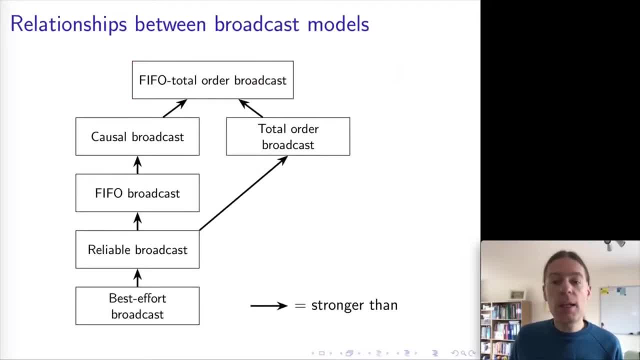 that order has to be the same for all of the nodes. Finally, there's something called FIFO- total order broadcasts, which just combines total order broadcast with FIFO ordering. So that means all the nodes have to deliver messages in the same order and also messages sent by the. 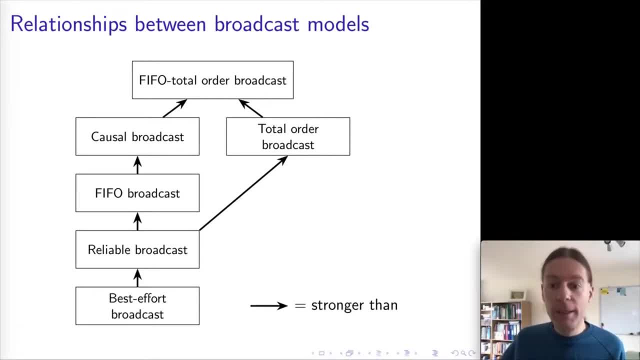 same node have to be delivered in the order they were sent. And it turns out that FIFO total order broadcast is strictly stronger than causal broadcast. so every execution of FIFO total order broadcast also meets the requirement of causal broadcast, and every execution of causal broadcast also meets the requirements of FIFO broadcast. 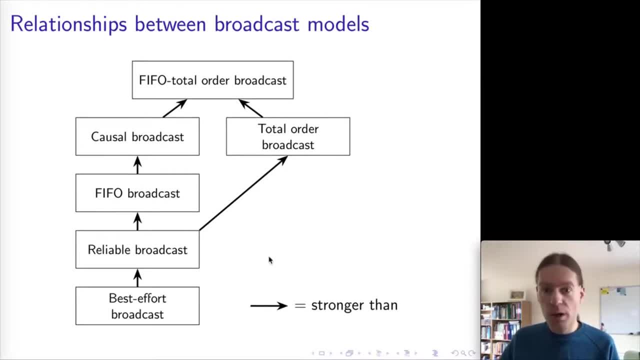 Thank you. Every FIFO broadcast meets the requirement of reliable broadcast and so on. So there's actually an exercise in the lecture notes for this lecture that asks you to prove some of these relationships between the broadcast models. In the next section we will then look at how to actually implement some of these broadcast algorithms. 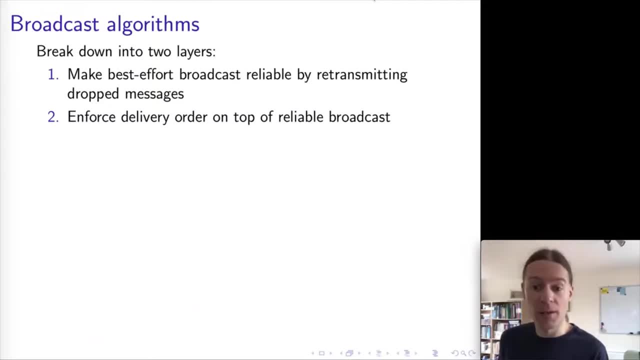 Next let's have a look at algorithms for actually implementing these different models of broadcast. So we're going to do that in two separate stages. First of all, we'll show how to take best effort broadcast and make it reliable, And then, once we've got reliable broadcast, we can layer on top of that modules for doing the delivery order. 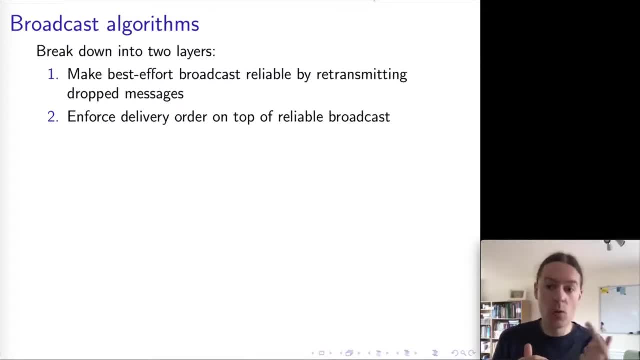 which allows us then to do either FIFO or causal or total order broadcast. So let's start with the reliability layer here. The most obvious thing you might think about like as a broadcast algorithm is: you have the node that wants to broadcast a message. 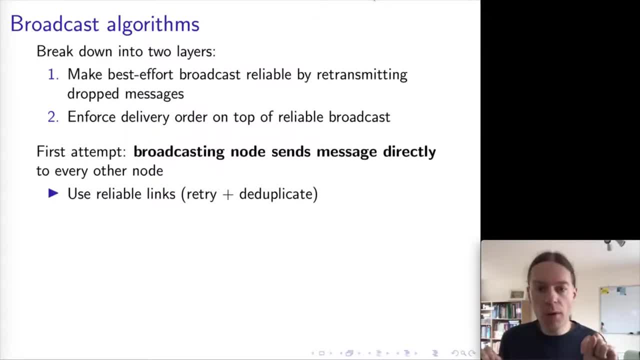 Just sends that message individually to every other node via point-to-point links, and make those point-to-point links reliable so that if the message gets dropped along the way then the sender will resend it. And so because then, through retransmission, the message will eventually get through to every other node. 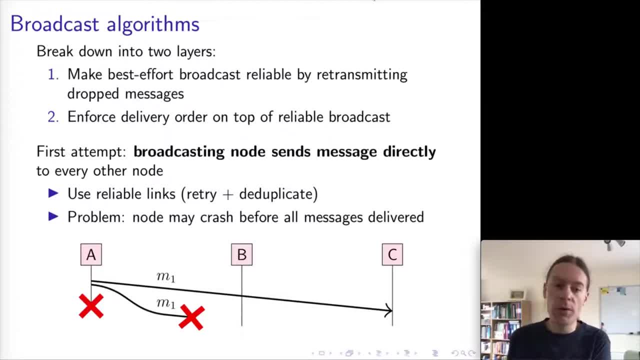 This unfortunately does not quite work, because what could happen is this here: A could try to broadcast message M1 to B and C. The message gets through to C, But the message gets dropped on its way to B, So A has to retransmit the message to B. 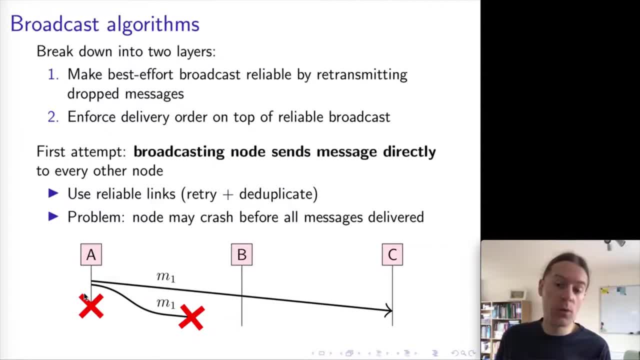 But then A crashes before A is able to complete this retransmission, And in this case, nobody is ever going to retry the sending of message M1 to B, And so therefore, C will have delivered a message that B did not deliver. 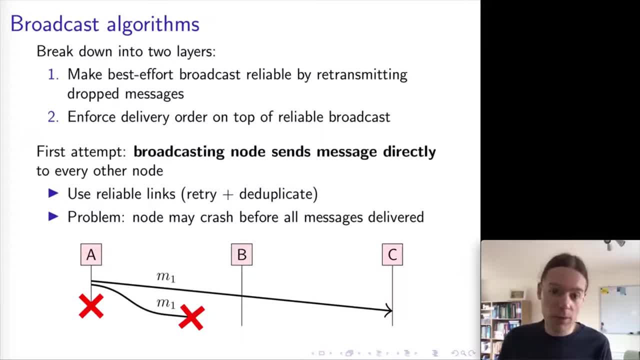 B is never going to deliver this message And therefore we have an inconsistency. So we have to now design an algorithm which is robust, so that, even if the sender of a message crashes, all of the remaining nodes will still agree on which message was actually delivered. 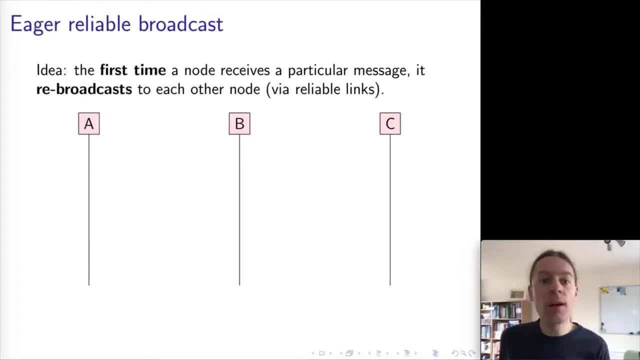 And so one technique we can use is called eager, reliable broadcast, And that relies on essentially just everybody sending messages everywhere. So, first of all, A wants to broadcast M1 to B and C. When B first receives M1, it rebroadcasts the same message again via point-to-point links. 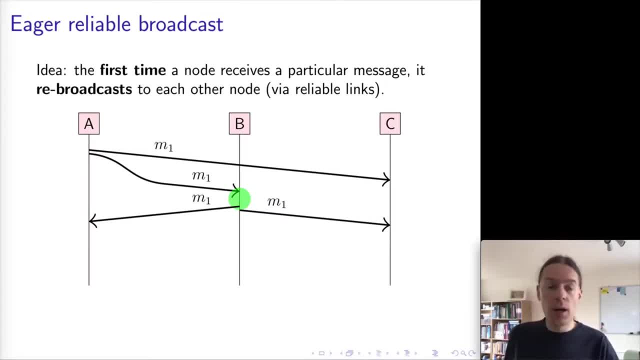 To every other node, And so this way then, even if A crashed, B will have further disseminated the message, And when C first receives the message, C will also rebroadcast the message to everyone else, And so this algorithm actually does ensure reliability. 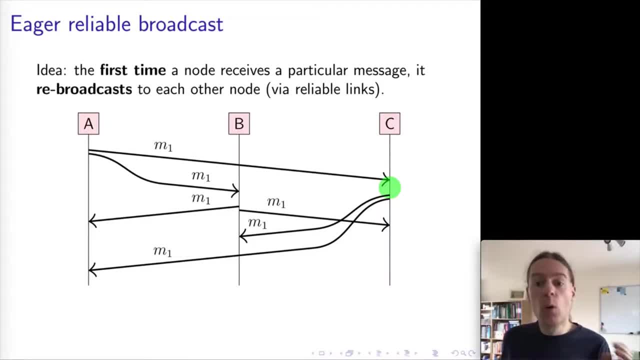 It ensures that, even if nodes crash, all of the non-crashed nodes receive the message. However, it is quite expensive, because every node that receives a message will again send that message to N-1 other nodes, And so in total we're going to end up with 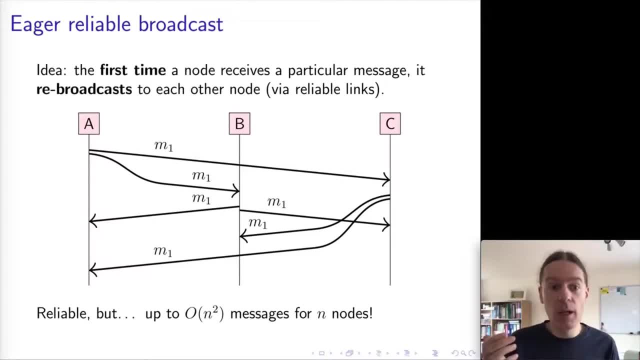 on the order of N squared messages being sent for every single message that a node wants to broadcast. So we get reliability, but at the cost of fairly high network bandwidth. Now, lots of different algorithms have been designed to optimize this, And one particular interesting group of algorithms 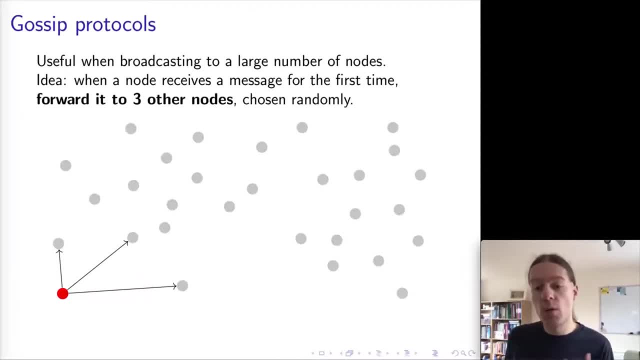 are called gossip protocols. So they are modeled in the way how gossip might spread through a network of people, where one person hears gossip from somebody and they then tell a few other people about this gossip, And so eventually this information spreads through a group, through a population of people. 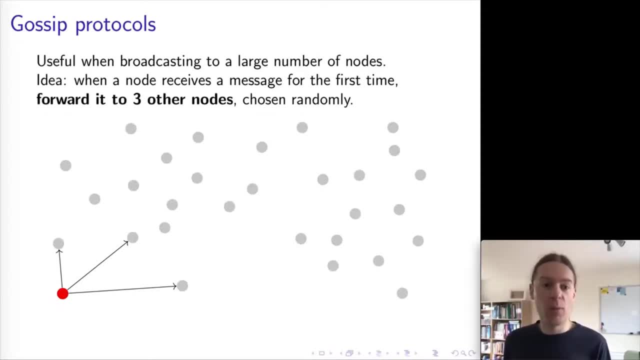 They're sometimes also called epidemic protocols, because they're somewhat similar to the way that an infectious disease might spread through a population, And so in this example here, each little blob is a node in the system, And I've just taken as the parameter for this algorithm. 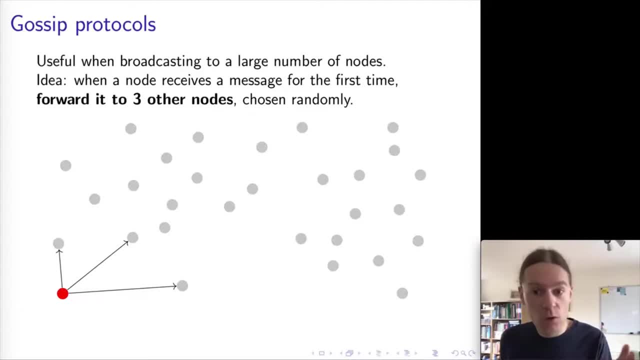 that each node sends on the message to three other nodes And those three other nodes are picked at random. And so here the red node is sending the message to three other nodes, And then these three other nodes each receive the message and they each rebroadcast the message. 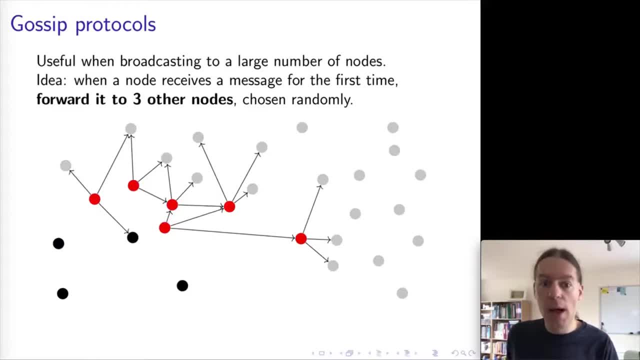 to three other randomly selected nodes And those recipients of those broadcasts. they again broadcast them further to others And you see that sometimes messages go to a node that has already received the message previously. Sometimes messages even go back to a node that had the message sometime in the past. 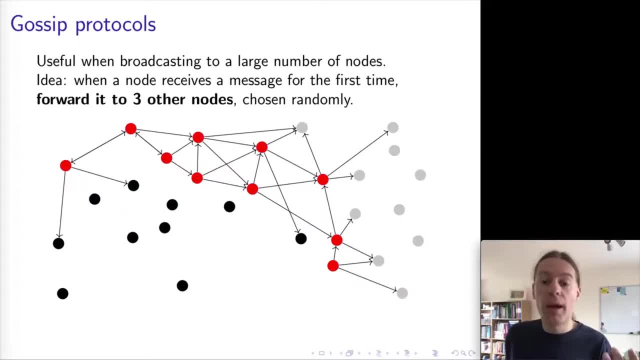 But eventually, over several rounds of this protocol, with very high probability we reach a stage in which the message has received all of the nodes, and now all of the nodes are black. Let me just go through that animation again, Because it's so beautiful. 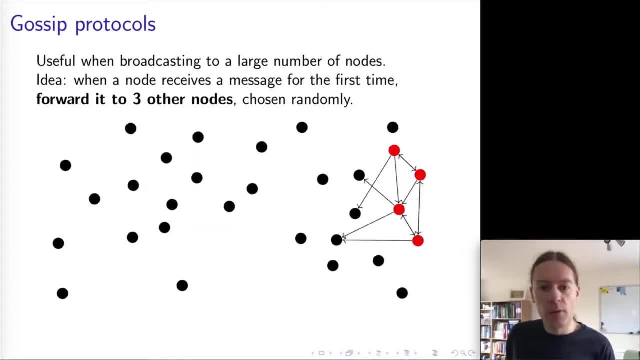 So we have the message spreading here And so in this case, all 30 nodes in this example have received the message after about six rounds of communication. So there are lots of details that you can tune about gossip protocols, about how exactly they decide when to send messages. 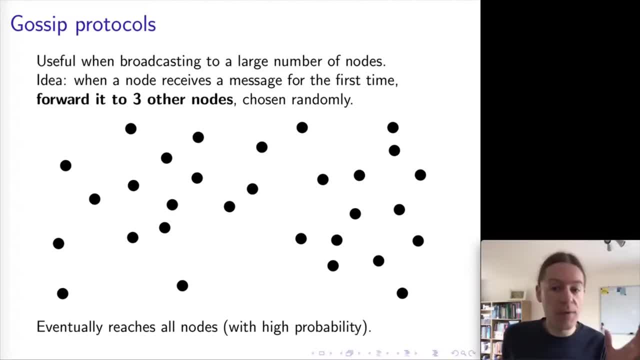 and when to stop sending messages and so on, But the basic principle is this: They are a way of achieving reliable broadcasts. They are quite robust so that even if some of the nodes crash or some of the messages get lost in the network, 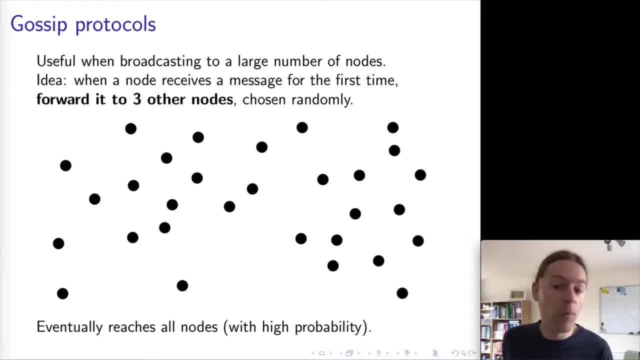 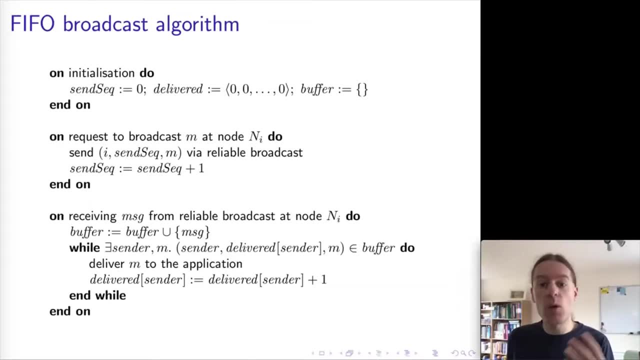 we still have very high probability that all of the messages get through to all of the nodes. Okay, so that gives us the reliability. Now, next, let's look at the ordering. So if we want to achieve FIFO broadcasts, for example, that means we have to ensure 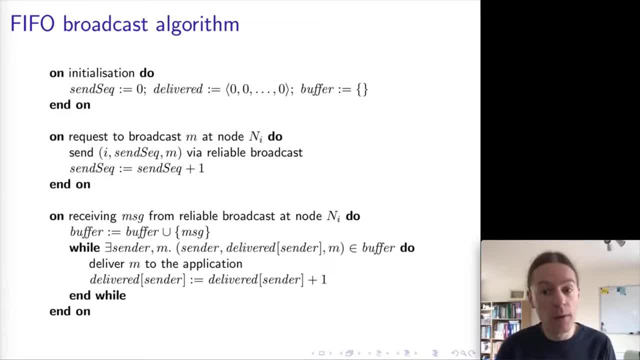 that all of the messages by the same sender are delivered in the right order. This is an algorithm of how we might achieve this, So each node here maintains three variables. Sender sequence number is just an integer that gets incremented for every node, for every message broadcast by this particular node. 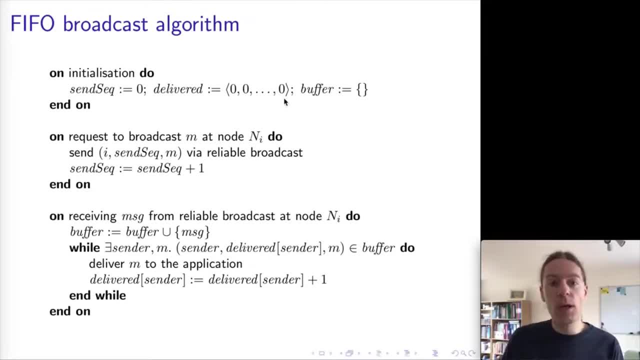 Delivered is a vector of integers indicating how many messages from each particular sender we have delivered, And buffer is a holdback queue of messages, so that if a message is not yet ready to be delivered, we put it in the buffer and then pick it out of the buffer sometime later. 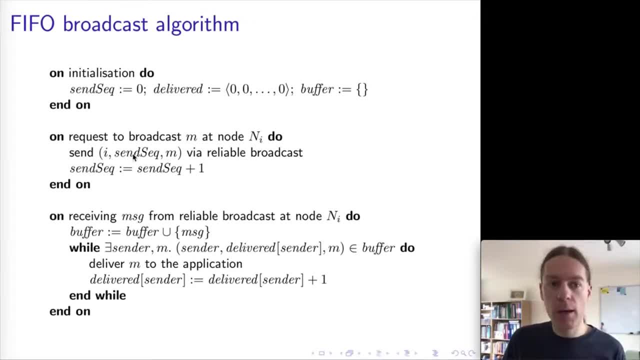 So if we want to broadcast a message, we attach the node number of the sender, i, and we attach the sequence number of the sender to the message and this triple gets disseminated to all of the nodes via reliable broadcast and then we increment the sequence number. 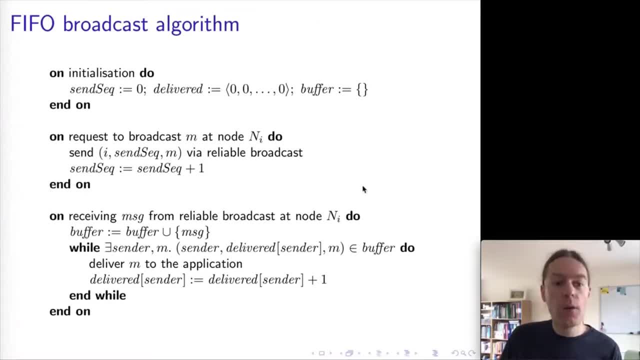 for next time we want to broadcast. Also, when we receive a message via reliable broadcast at node ni, we first of all add the message to the buffer and then we look at the buffer trying to find any messages that are ready to be delivered. 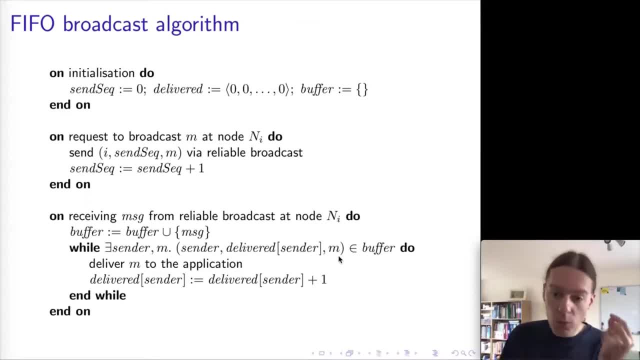 And here ready to be delivered, means that for any given sender we have a message in the buffer where the sequence number is the next integer that we are expecting, in the sequence of sequence number, from that particular sender. And so if we have a message matching that, 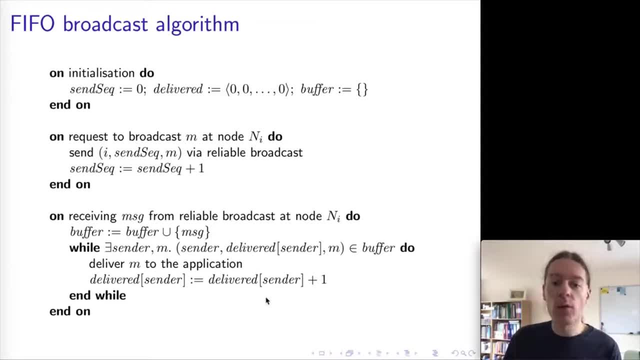 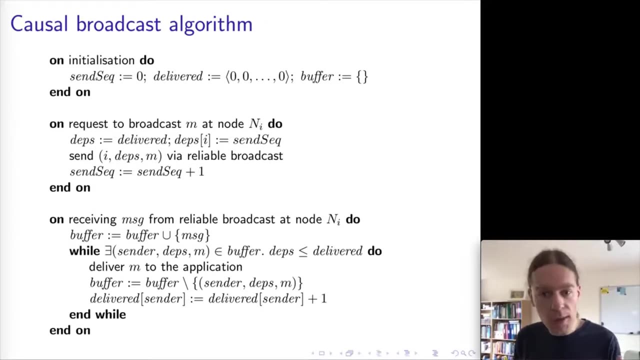 then we take that message delivered to the application and we increment our local vector of the number of messages we have delivered from a particular sender. And so this is it. This achieves FIFO broadcast. Next, let's have a look at causal broadcast, The algorithm, the structure of the algorithm. 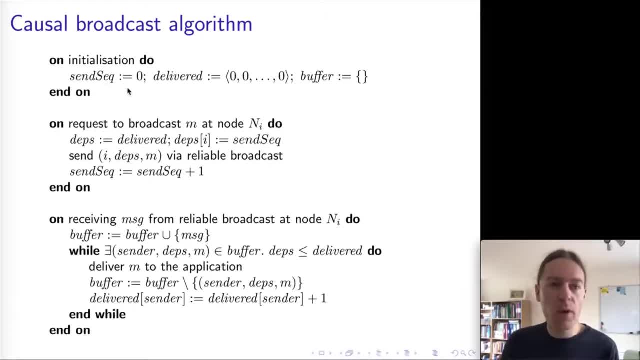 is very similar. We start with the same three variables. So again, we have a sender sequence number, we have a vector counting the number of delivered messages and we have the holdback buffer When we want to broadcast a message at ni. 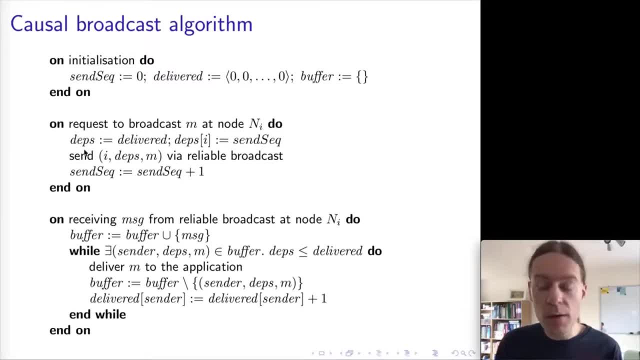 first of all, we create this new variable dependencies So that captures the causal dependencies of this message. So it's a way of determining which messages happened before this particular message, And those will have to be then all of the messages that have to be delivered. 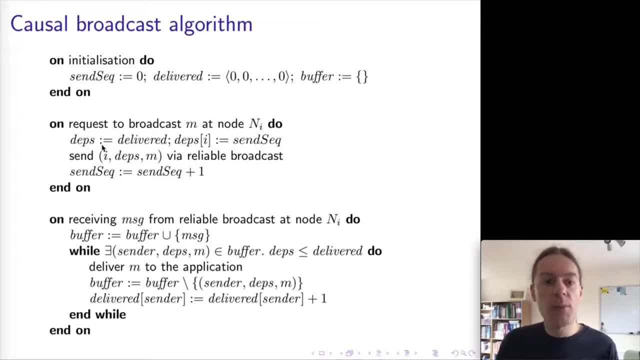 before this message being broadcast. So we take dependencies to be a copy of our delivered vector And we update the sending the broadcasting nodes own entry to be equal to the sequence number And then we send the message via reliable broadcast. again, This time we don't attach the sequence number. 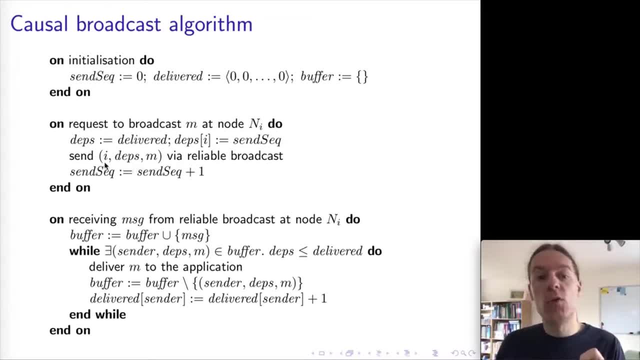 but we attach this dependencies vector in addition to i, which is the index of the node, And then we increment the sender sequence number as before. So this time we've got messages that have a vector attached to them rather than a single integer When one of these messages gets. 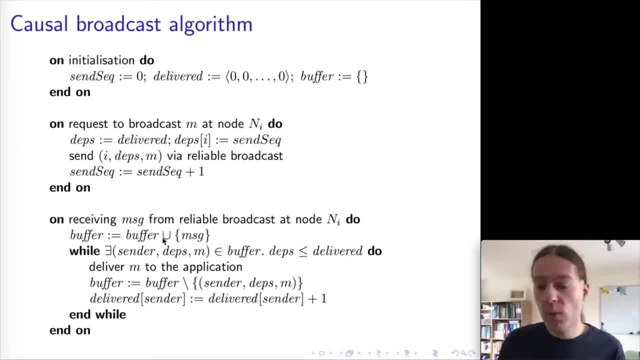 delivered at a node. we first of all put the message in the buffer, as usual, and now we search for any messages that are ready to be delivered, And these are any messages whose causal dependencies have been satisfied, So any messages that were broadcast before the current message. 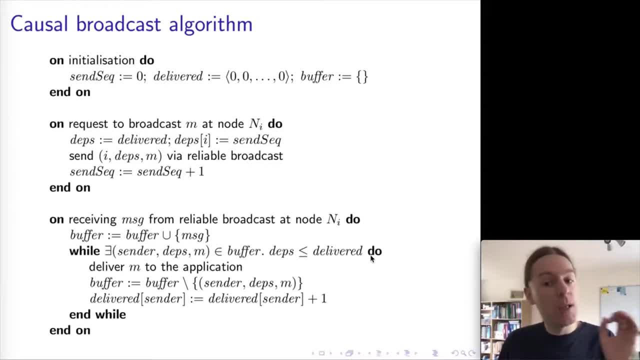 they have already been broadcast by. they have already been delivered by the local node. If those have been delivered, then this message is ready to be delivered because its causal dependencies have already been delivered. So here we search for any sender, dependencies and message in the buffer, such that 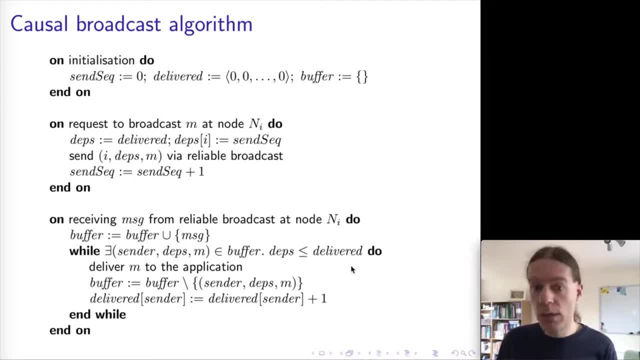 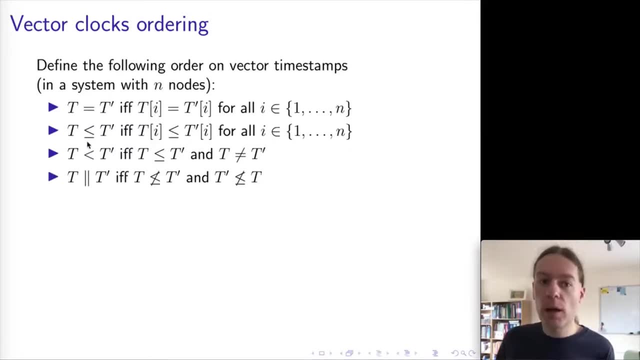 the dependencies vector is less than or equal to the delivered vector, And this less than or equal operator is exactly the less than or equal operator that we defined on vector clocks a little while back. So, even though this algorithm is not exactly the same as the vector clocks algorithm, 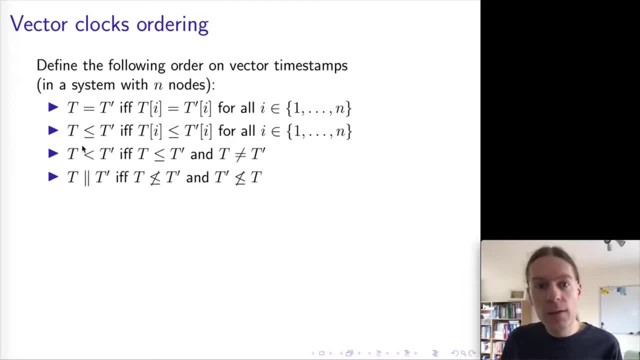 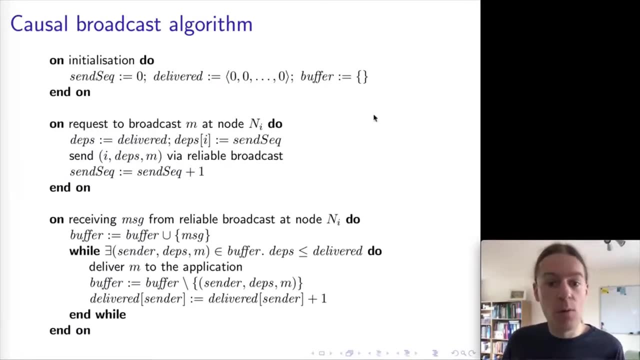 it's similar in the way that it does use these vectors of numbers and it uses this less than or equal comparison as a part of its algorithm For causal broadcast. if we have a message that satisfies the dependencies, we deliver it. we remove the message from the buffer. 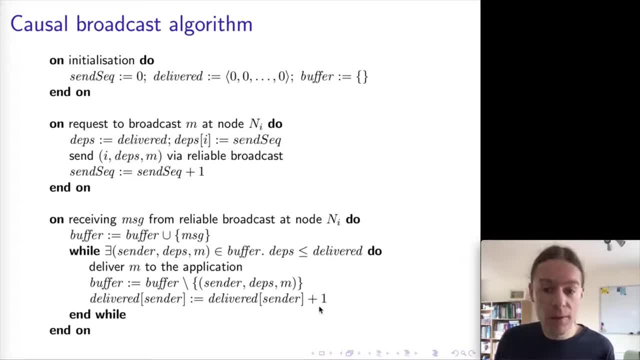 and we increment the number of messages we have delivered from that particular sender, And this ensures causal broadcast. You might have to think about the algorithm for a little bit to convince yourself that it really is correct, but I think it is correct, So that is causal broadcast. 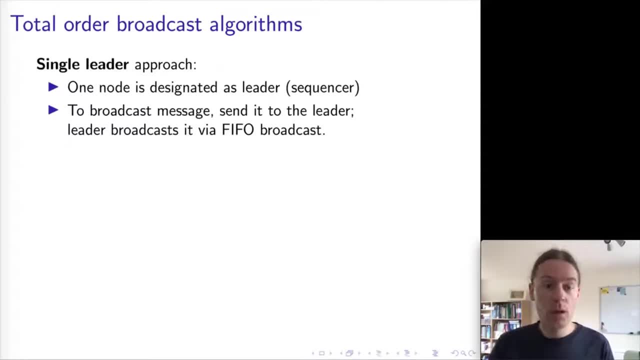 Finally, total order broadcast. So total order broadcast is a bit harder Because, remember, we have to somehow agree on what this total order is of messages, in which order the messages are going to get delivered. Let's say one simple way of doing this. We're going to pick one. 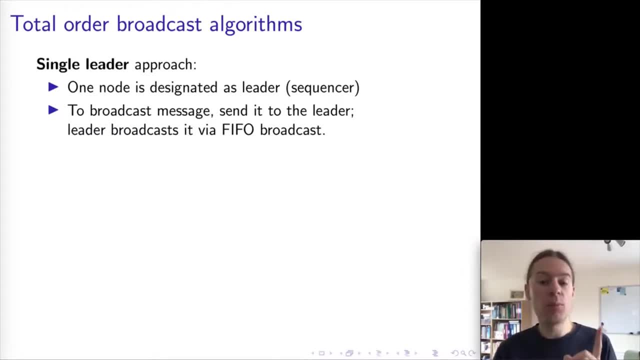 of the nodes as the leader, And this leader is going to be in charge of determining the order in which the messages get delivered. That's why it's also sometimes known as a sequencer, because it sequences the messages, And if one node wants to broadcast a message, 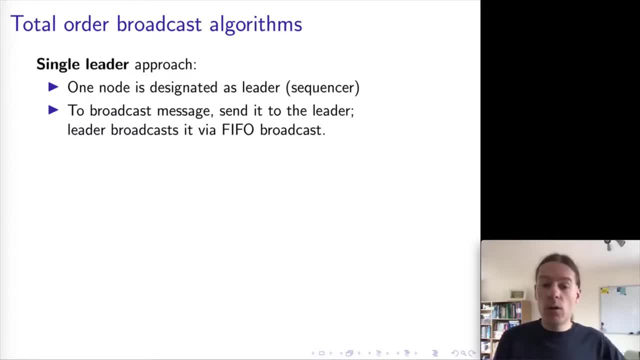 it doesn't directly broadcast it to the other nodes. Instead, the node sends it to the leader via a FIFO link probably, And the leader then broadcasts it via FIFO broadcast to the entire group. And so because all of the messages are going, 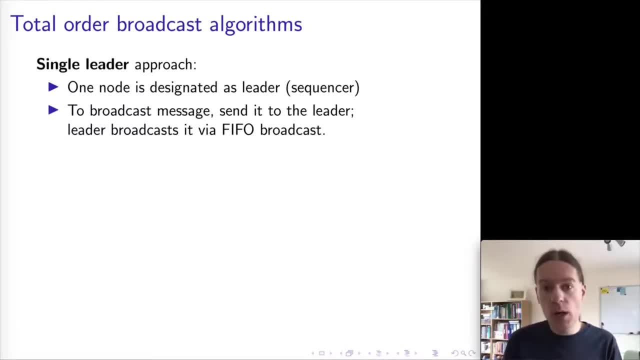 through the leader. simply, the order in which the leader broadcasts the messages then is the order in which all of the other nodes will deliver the messages, since we're talking about FIFO broadcast here And this works quite nicely. It just has the problem that if our leader 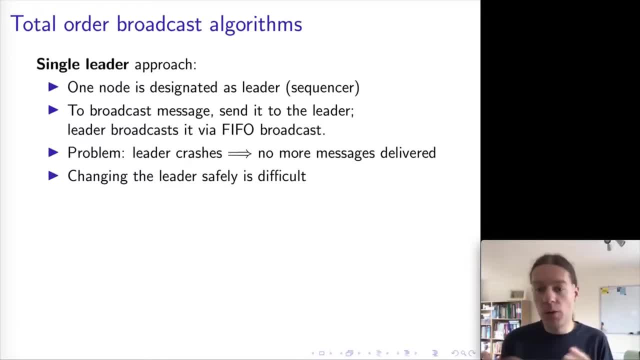 crashes, then no more messages can get delivered because we're requiring all of our messages to go through the leader. So really we would need some kind of way of changing the leader from one node to another in case the leader crashes. but this is quite difficult. 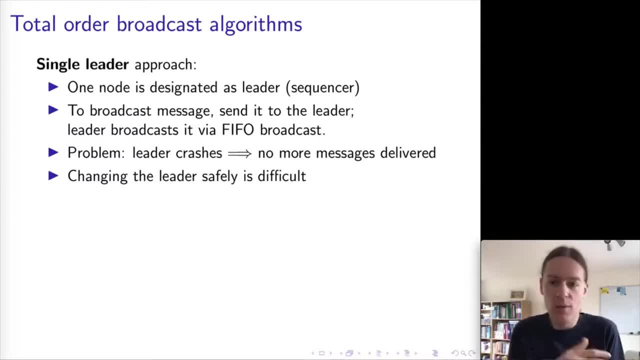 to do safely, because you know what, If you end up with two different leaders, then your guarantee of total order is gone. So we will see ways of actually doing this kind of leader change safely in a later lecture when we come to talk about consensus. 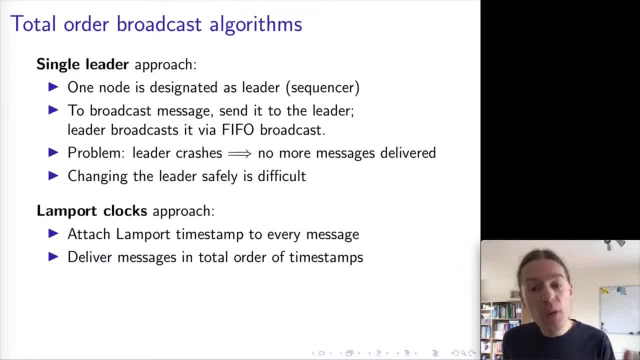 But for now I'm just going to leave this as an open problem. There's another way you could achieve total order broadcast which does not rely on a leader. Instead, you could rely on Lamport clocks. So remember, Lamport timestamps have an associated 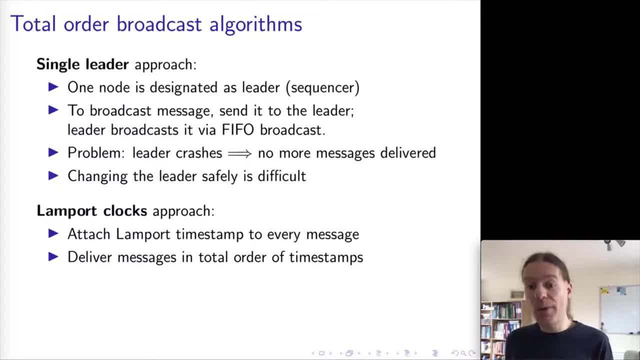 total order and we can use that total order as the order in which we are going to deliver the messages. So we attach a Lamport timestamp to every message. we create those Lamport timestamps in the usual way, like we have discussed, and then 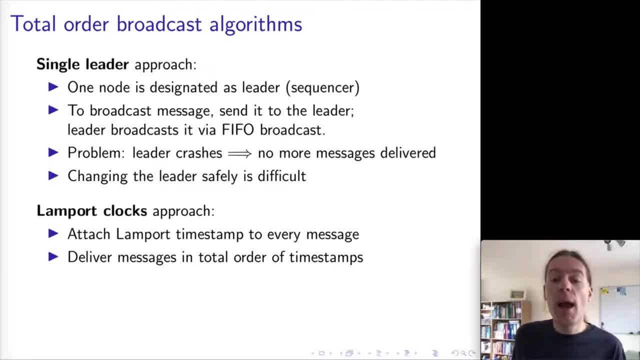 broadcast those messages via some kind of reliable broadcast. and then each node needs to ensure that it delivers messages in increasing order of their Lamport timestamps. And this works, but it does rely on one particular piece of knowledge which is a node needs to be sure, at the time when a node 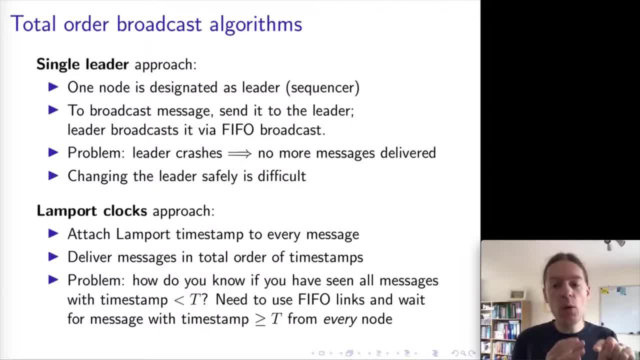 delivers a message, it needs to be sure that there will be no future messages with a Lamport timestamp less than this message that it's about to deliver, Because if it did deliver the message now and then later a message with a lower timestamp arrives, then it would have delivered them in the wrong order. 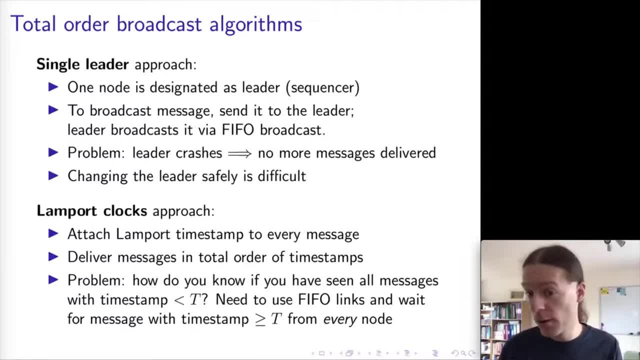 because it has to deliver them in the messages in strictly ascending order of Lamport timestamp. So therefore we need some way of knowing that there will not be any future messages with a timestamp less than some particular threshold. And it is possible to know that because if we use FIFO, 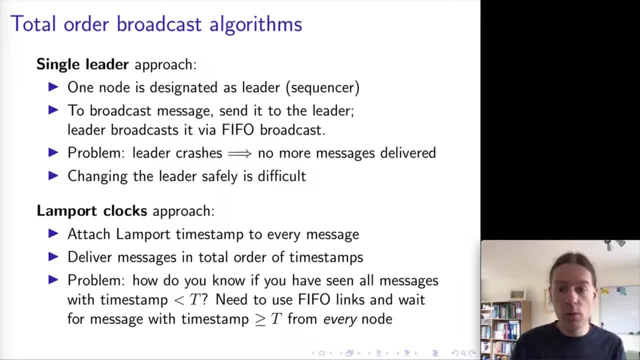 links between the nodes, then actually we know that each node will send messages in increasing order of Lamport timestamp and we receive those messages in increasing order. So therefore, if we've heard from every other node, then we know that the minimum timestamp that 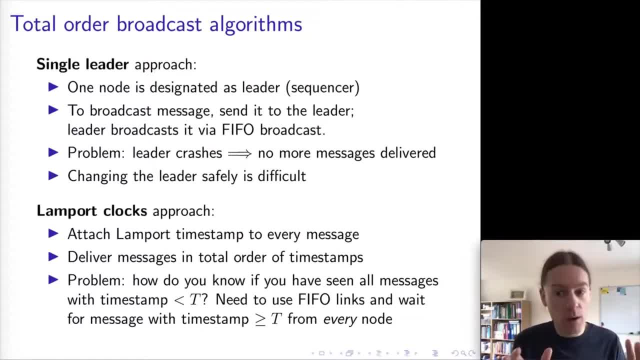 we've seen across any of the other nodes is going to be the minimum we're ever going to see, So there will never be any later timestamps than this one, And so, based on that, it is now possible to again create total-order broadcast Again. 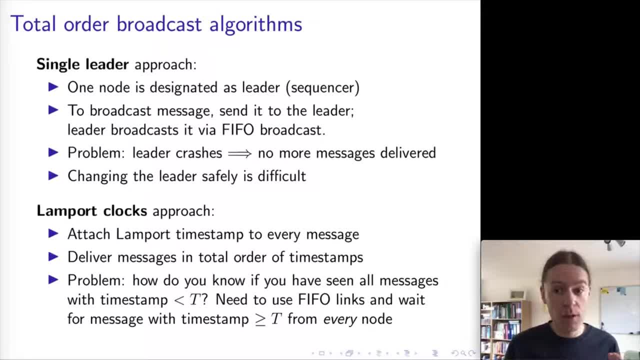 unfortunately, this approach is not fault tolerant, because in this case, if just one of the nodes crashes, it will not be sending any more messages, so the Lamport timestamps won't be moving forward anymore and so no messages get delivered anymore. So these two algorithms- 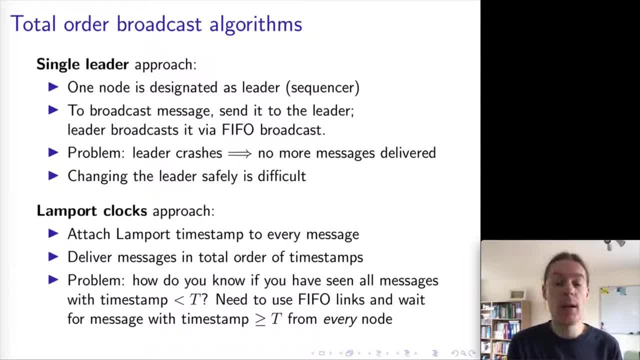 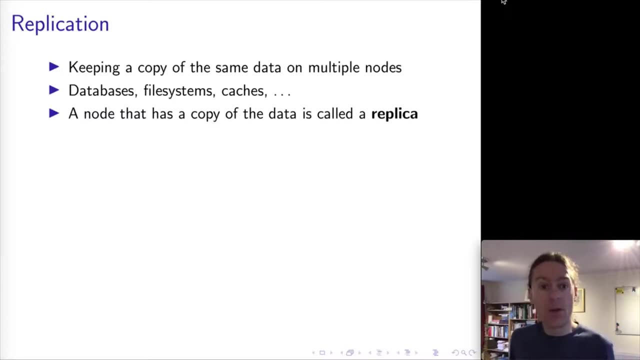 do work, but neither of them is fault tolerant, and later, in a later lecture, we will see ways of achieving total-order broadcast in a way that is fault tolerant. Welcome to Distributed Systems, Lecture 5.. Today we will be talking about replication, So replication. 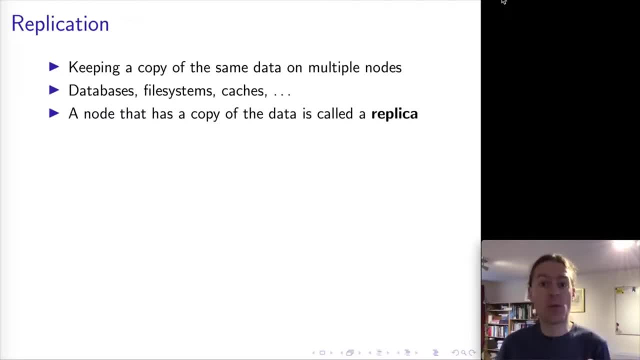 simply means having a copy of the same data on multiple nodes in a distributed system. Replication is very widely used, so, for example, many distributed databases use replication as part of their normal setup. Many distributed file systems allow you to have a copy of some files on multiple. 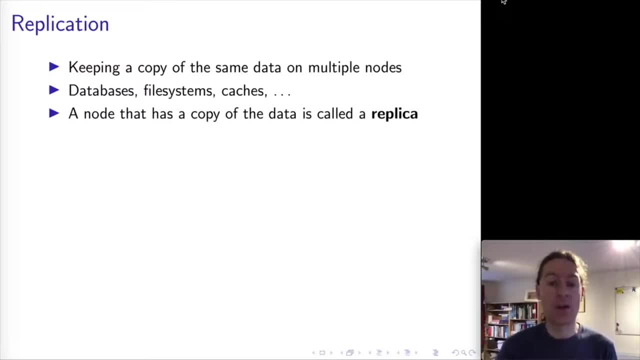 different nodes, Many caching systems that are essentially forms of replication, And we're going to be talking about algorithms that fit for all of those types of systems. Now, in a distributed system, any node that has got a copy of the data is called a replica. 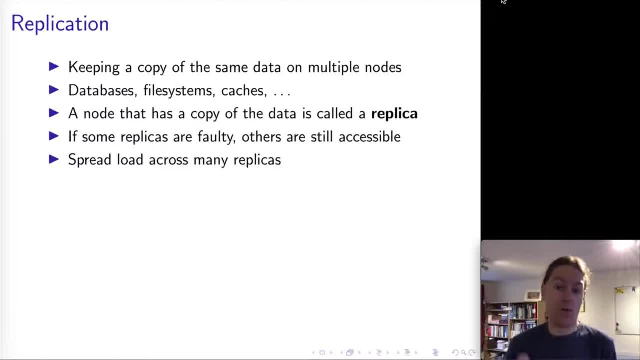 And there are several reasons why you might want replication in a system, The most important one of which is that if some of the replicas are inaccessible for some reason, you've still got the other ones and the other copies of the data you can still use to serve. 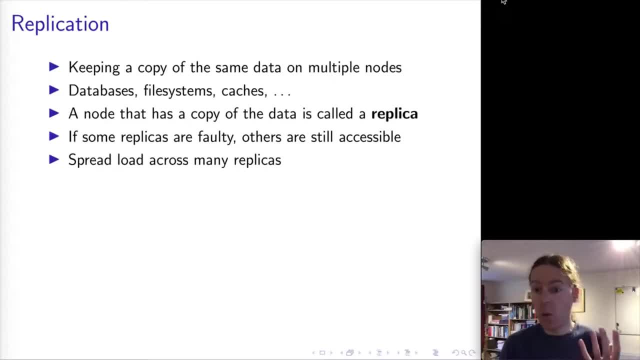 user requests. So there are quite a few different reasons why a replica might be inaccessible from time to time. There might be a software problem causing it to crash. there might be a hardware problem causing it to just stop working. there might be a network problem, which means 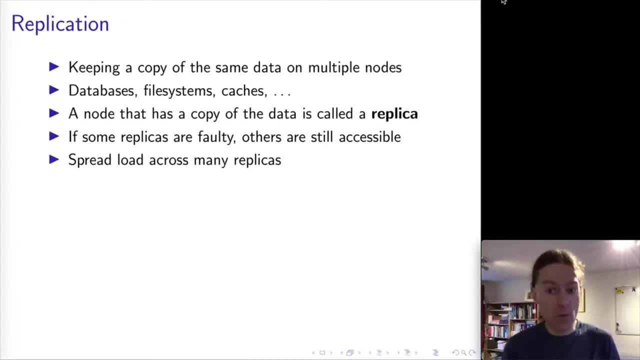 you might have a network partition so you might be able to communicate with some of the replicas, but not with others, especially if the replicas are distributed across different locations. You might be able to talk to your local replica, but not a replica that is somewhere. 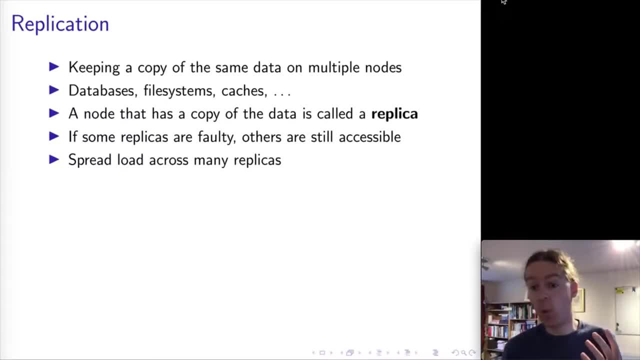 remotely. And another reason why you might want replication is you might deliberately make nodes inaccessible from time to time, For example, you might choose to reboot a node in order to install software updates, and while that computer is rebooting, it can't be. 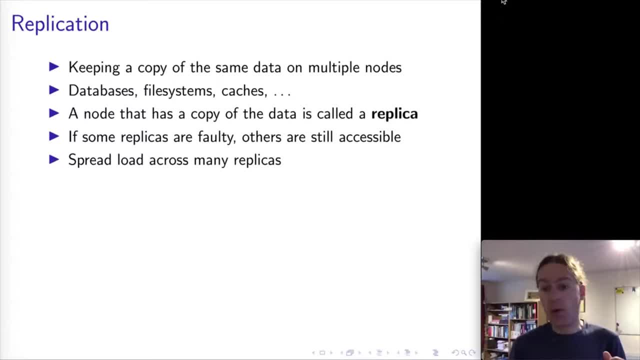 processing any user requests or any messages, and so during that time that node is unavailable. and really what we want is that a service as a whole- of a database, for example- it continues working even if some of the nodes are unavailable and replication is one. 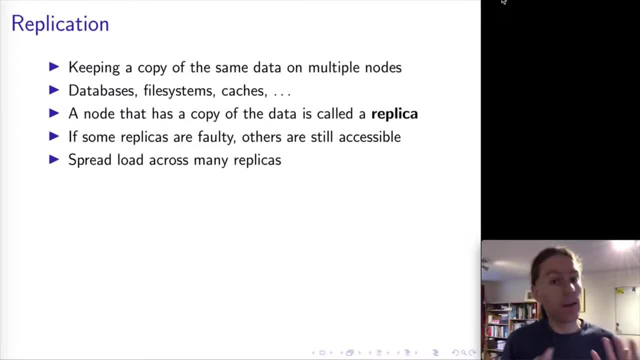 of the mechanisms we have which allows us to provide that sort of fault tolerance, which is very useful, especially if you need to do maintenance of a system, because it means you can reboot one node at a time, as long as you're not turning them all off at the same time. 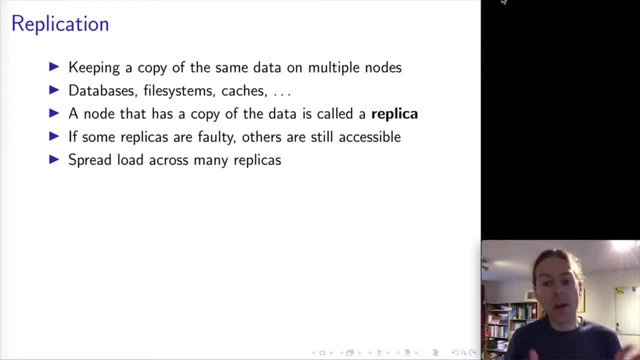 as long as you just reboot one at a time, then the remaining nodes at any one time can continue processing requests. Another reason why you might want replication is if there's very heavy load. for example, lots and lots of different users around the world all want the same. 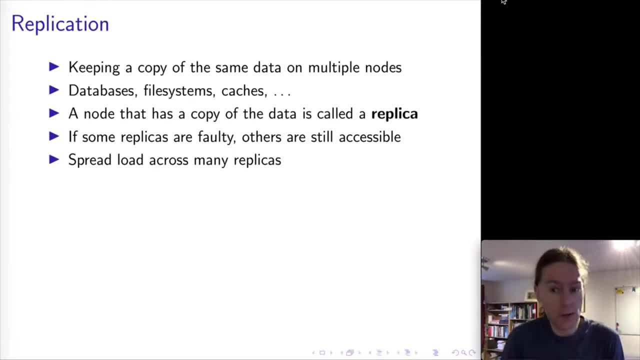 piece of data, then that might be too much for a single node to handle, and in which case, having copies of that data on multiple nodes simply lets you handle more requests from more users, which is important in internet scale systems. Now replication is really easy. 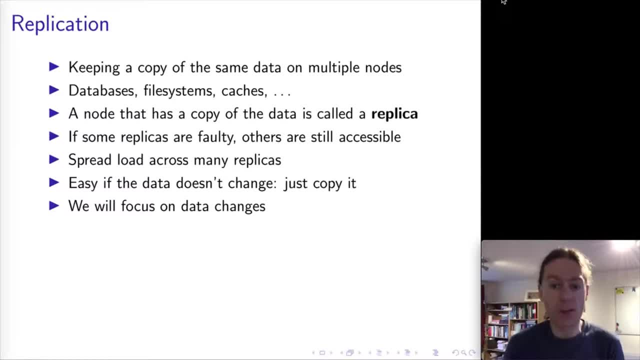 if the data that you're copying doesn't change. This is kind of obvious. If you've got some data that is static, you can just make a copy of it, a one-time copy across all of your nodes, and job's done. So what we're all. 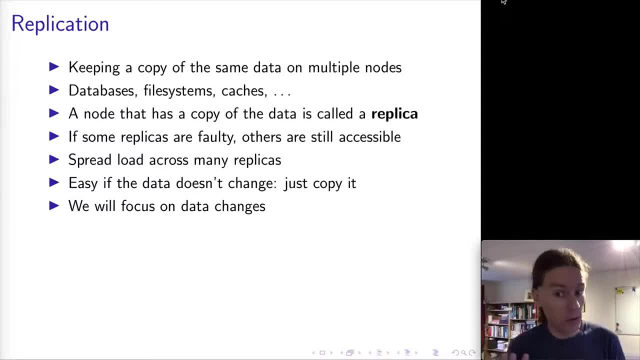 going to be focusing on in this lecture is data that changes, because that's the bit that is hard. Data changes are the bit that is hard and that requires the most care. Now, one form of replication that you might have come across in the context of operating systems: 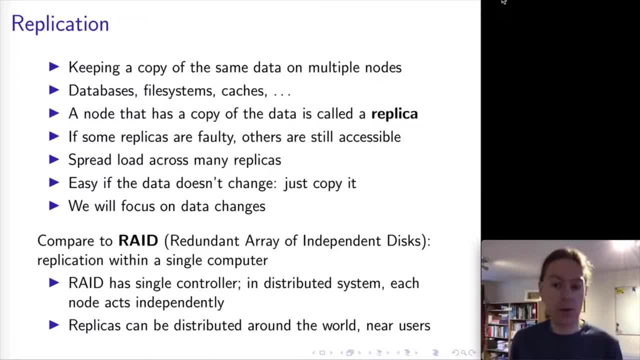 is called RAID, And so this is: if you have multiple hard disks attached to the same computer, you can use RAID to redundantly store data on more than one hard disk. So, for example, in the case of RAID 1, you actually have 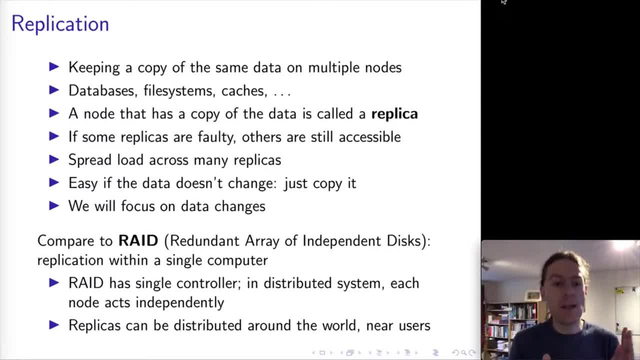 two separate disks that are basically mirrors of each other. So any file that is written to one disk is also written to the other disk, which means that if one of the disks experiences a hardware failure, you've still got the data on the other disk. 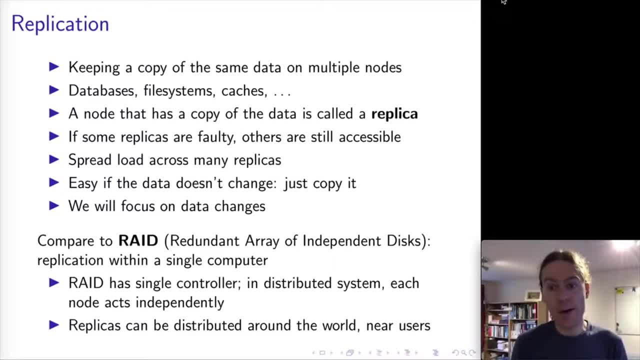 Extremely useful if you don't like losing data. Now, the replication that we talk about in distributed systems is somewhat similar to that, except the techniques that are used for RAID don't immediately apply in a distributed system, because RAID is designed for a single computer. there's 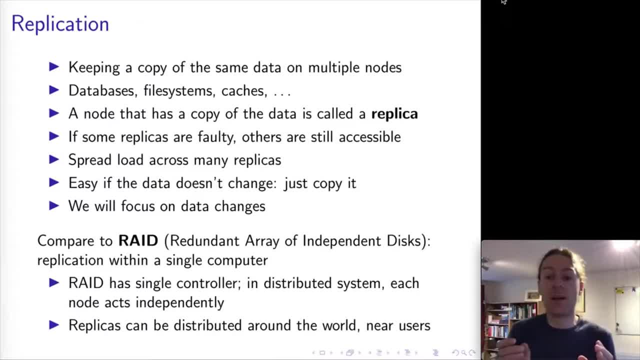 a single controller that manages all of the data In a distributed system. as you've seen in the previous lectures, we've got each node acting independently. we've got the unreliable network in between the two nodes. the nodes might be distributed around the world so they might be not located in the 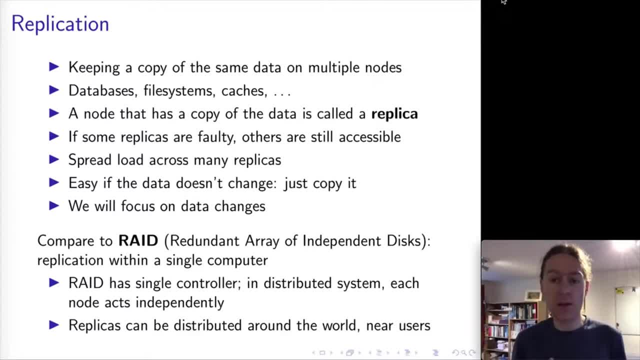 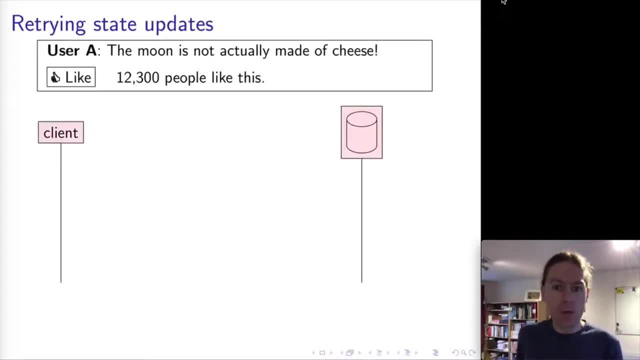 same location, but they might be on different continents, communicating over the internet, and so we have to deal with all of the challenges that this sort of distributed setup brings. So let's look at one example, just to get us started, of cases where 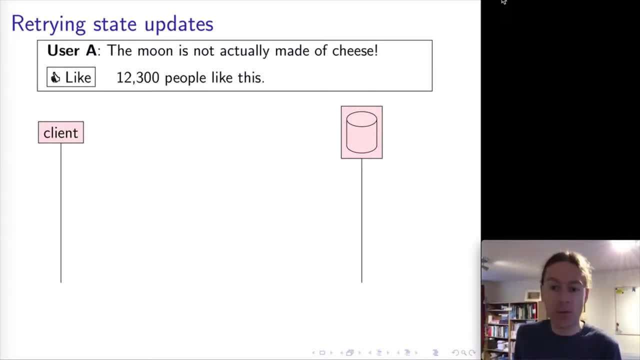 we've got a database that is storing some state and that state changes. So here we have an example of a social network and some user posts an update saying the moon is not actually made of cheese, and you want to press the like button on that. 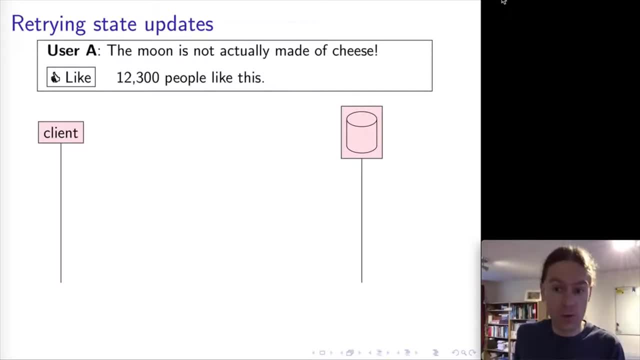 Okay, so the fact that you have pressed that like button needs to be stored somewhere, and also the fact of how many people have clicked that like button needs to be stored somewhere, and that somewhere is typically a database that is running somewhere on the servers of. 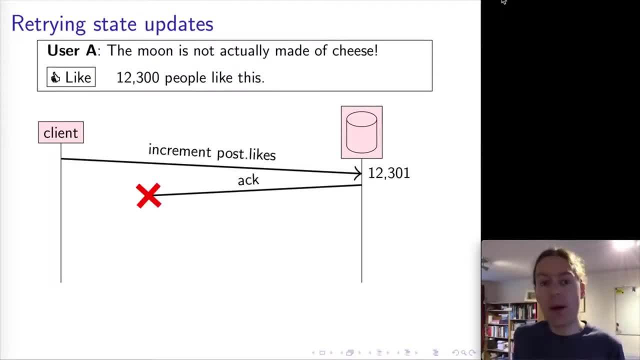 the social media provider, And what could happen now is: I'm just going to consider the count of likes for now. So the client, just as you press the like button, the client needs to tell this counter that is stored somewhere that, oh, you need to increment the. 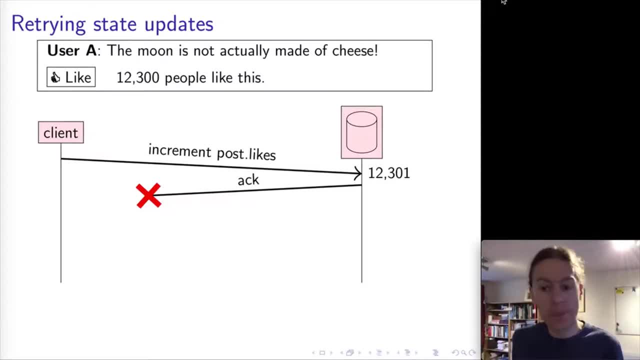 counter, because one more person has liked this particular update now. But networks being what they are, of course it could happen that either the request or the response is lost in the network, And so let's consider, in this example, that the request got through. 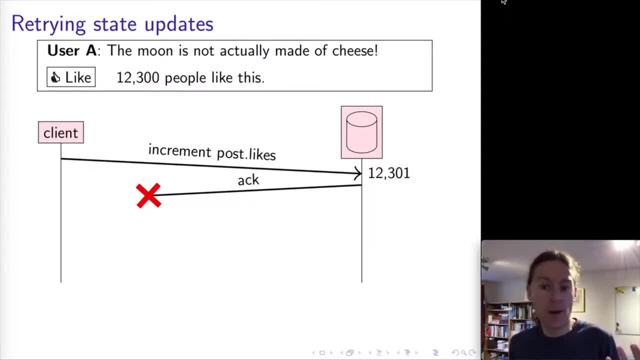 but the acknowledgement back to the client that, okay, I incremented the counter, The acknowledgement got lost in the network And so the client says: well, it seems like the request didn't get through. Let's try it again. Let's send. 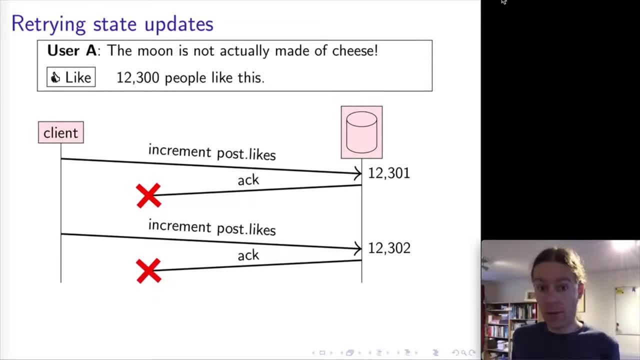 the request to increment again. The server receives that request again, and so it ends up incrementing this counter twice, And so we go from 12,300 to 12,302, even though you actually only pressed that button once. Now this might seem like a. 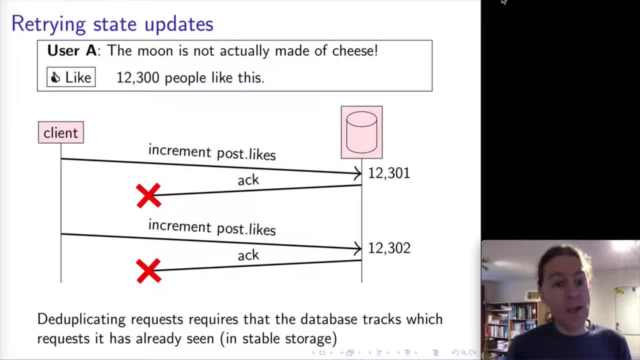 bit of a hypothetical example, but it really does occur. Now, the first thing we can do to try and prevent this kind of thing is to do deduplication, and we've seen that in the context of the broadcast protocols, for example. 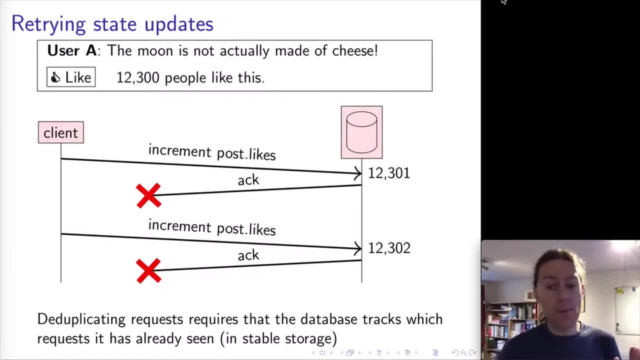 However, with databases, with a database generally, we want to support a crash recovery type system model. That means you know if a node crashes, it doesn't stay offline forever, It will come back, which means that any data that needs to be not 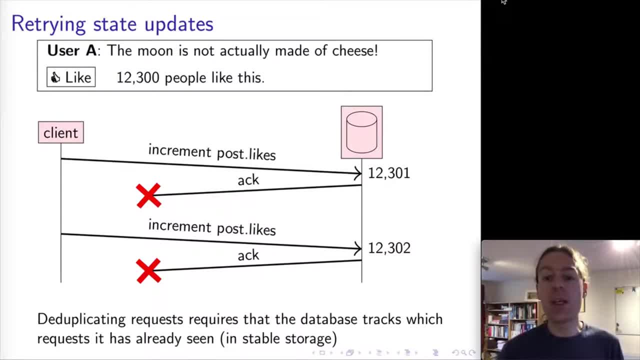 lost in the process of that crash and restart needs to be stored on disk in stable storage in some durable form, And if you want to deduplicate requests to a database in a way that will work even across crashes and restarts, that means that all of the requests 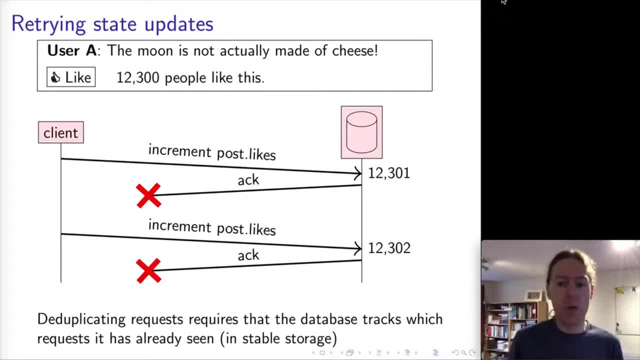 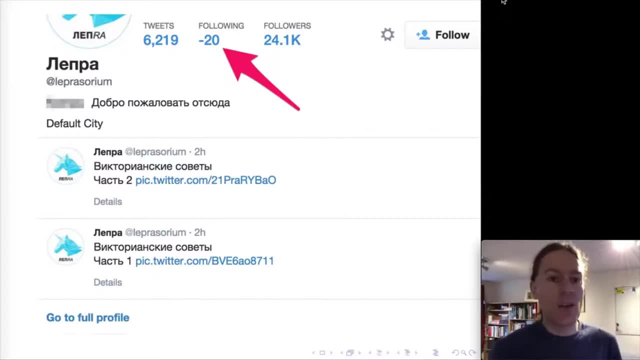 actually need to be stored in the database as well. That can end up being quite a lot of data. Now, you might think that this sort of thing is just a hypothetical problem, but it really does occur. This is an example. this is a screenshot. 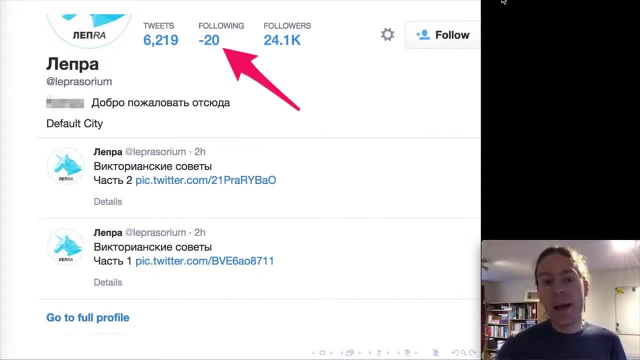 a genuine screenshot that I made of Twitter a few years ago and it shows a user account who is following minus 20 people. So this should be impossible, because, of course, you can only follow a positive number of people in real life. 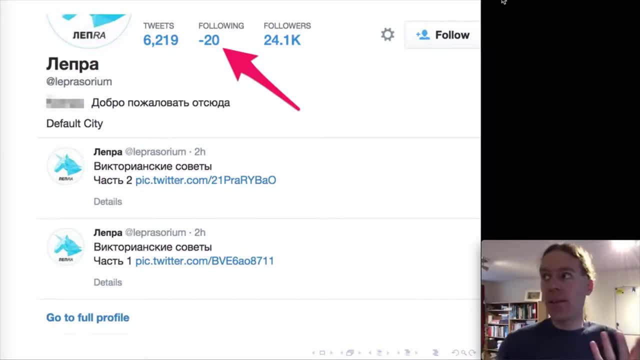 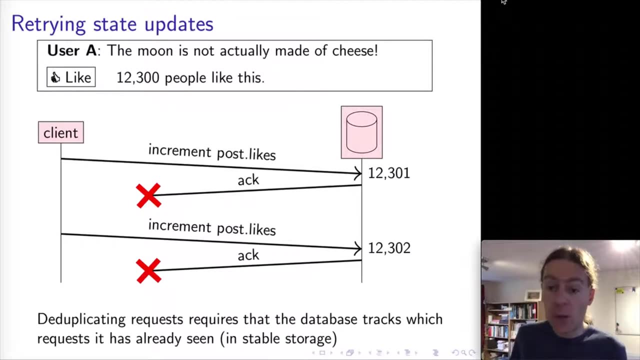 There are no negative users, and so I don't know exactly what happened in this scenario here, but I suspect that something happened was very similar to this example, So probably the user was following some number of people. then they unfollowed those people. 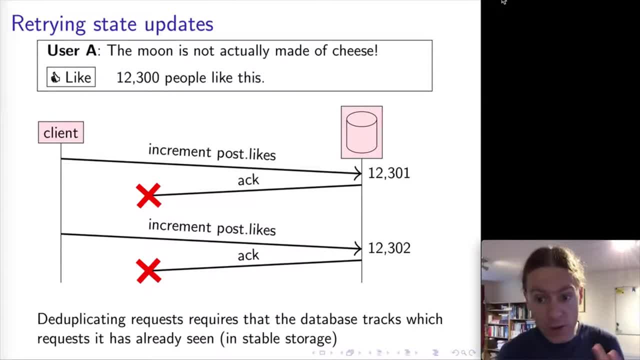 in the process of unfollowing those people, some counter of how many people this person is following had to get decremented and so there was some network failure somewhere and so that decrementing of the unfollow counter- sorry, the decrementing of that follow count got. 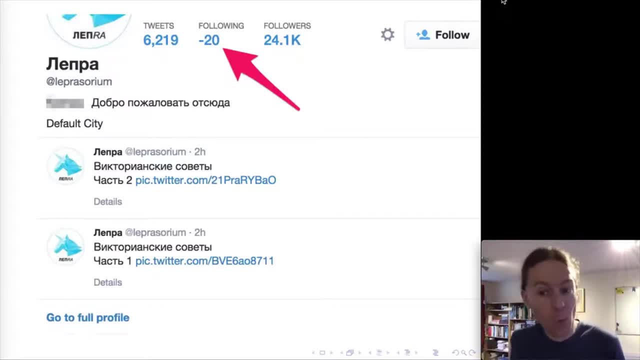 repeated, and so we end up decrementing more than there were actually followers, and so that's why we end up with a negative counter here. So, okay, I think Twitter has probably fixed that bug in the meantime, but let's look at how we would deal. 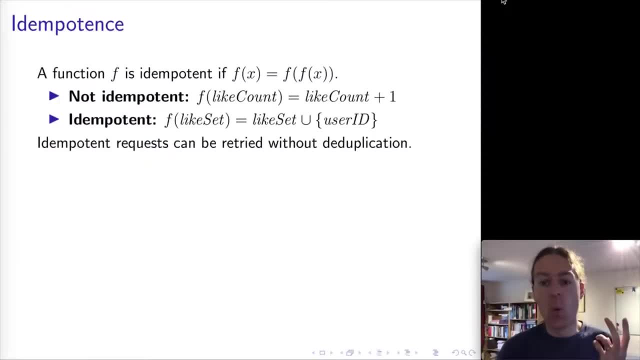 with this kind of problem in our systems, and one tool that is very useful in the context of these kinds of retries is to make the operation idempotent. So idempotence is a concept from maths, which just means that if you apply a function once, 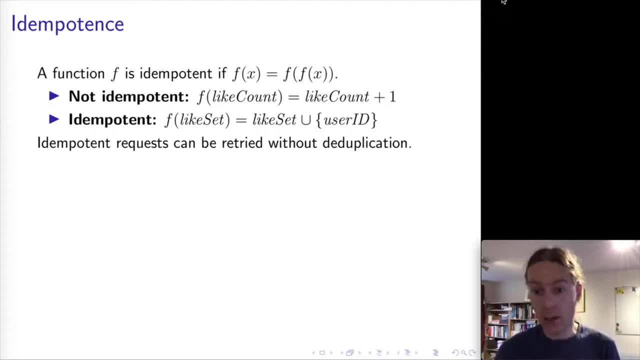 to some argument, it has the same effect as applying it twice, or applying it three times, or applying it any number of times, and so an example of a function that is not idempotent is to increment a counter, like we have just seen, because if you increment, 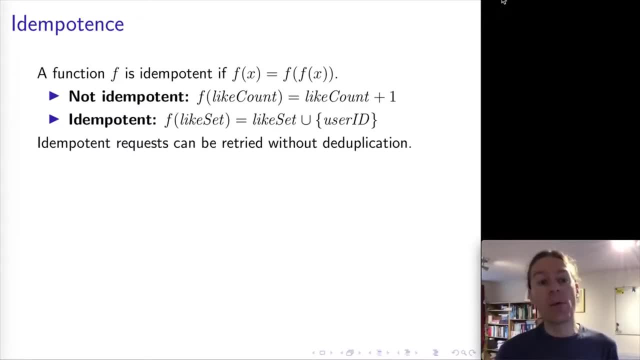 a counter once, that's not the same as incrementing it twice. However, adding an element to a set is idempotent, because if you add an element to a set and then add the same element to the set again because the set doesn't count, how? 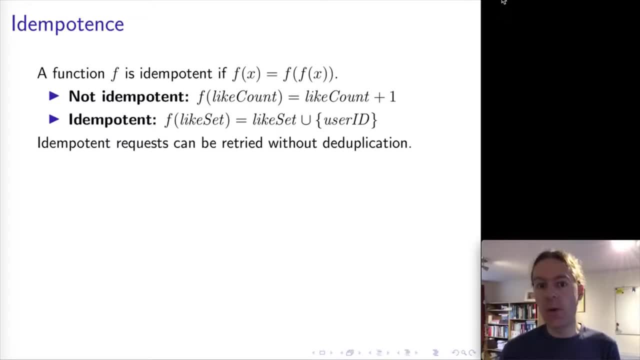 many times an element is there. it's either there or not there, and so therefore, doing the set union operator, that is idempotent, And so this means now, if we represent these likes or the user follows in the case of Twitter, as a. 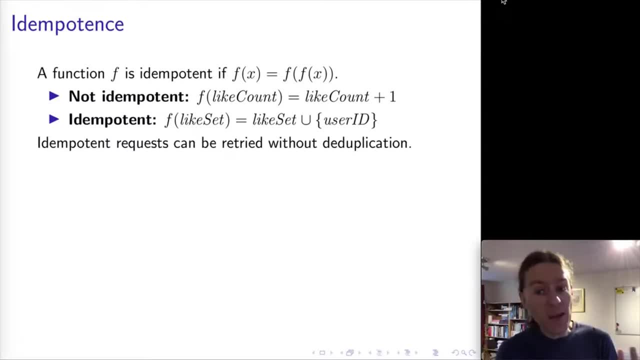 set rather than as a counter. then we can safely retry, because even if the request gets lost or so we can just send that request to add an element to a set, we can do that again, and applying it twice does no harm, because 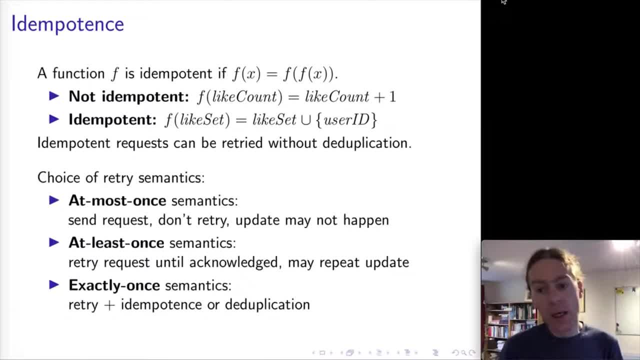 it just does the same as applying it once, Which leads to a choice of different semantics that you get in these types of distributed systems. They're just terms that you might see, and so I wanted to mention them briefly, which are at most once, at least once, and 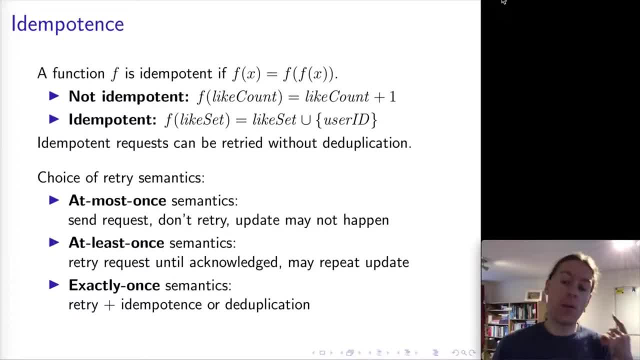 exactly once. So at most once just means you send a request over the network once. it may or may not get there, but you're not going to retry So it might arrive. it might not arrive, but you're not going to try and make this reliable in any way. 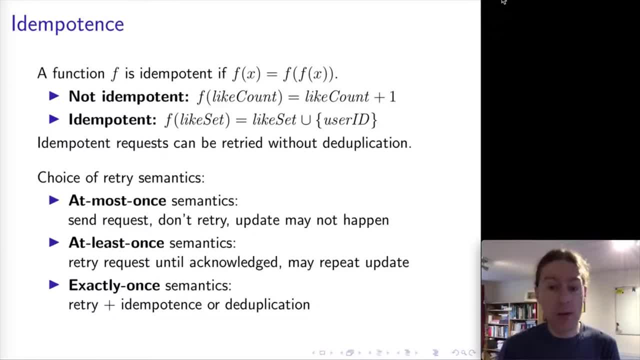 At least once means you're going to retry until you get an acknowledgement, which means the request may arrive multiple times. but really what we typically want is exactly once, which means the operation takes effect exactly once. So the effect is as if the operation 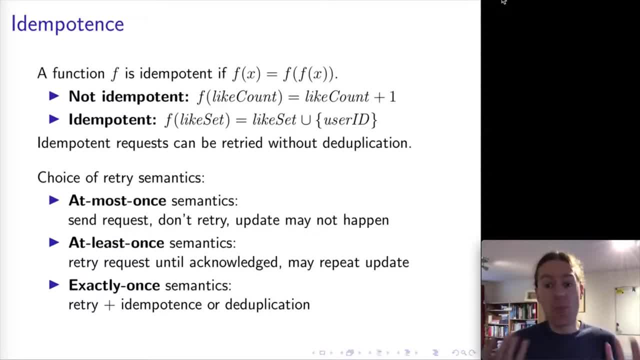 were received exactly one time, even though in practice, due to retries and due to message loss, it may actually be some different number of times. And so if we retry and also have an operation that is idempotent, then we can achieve exactly one semantics, So that 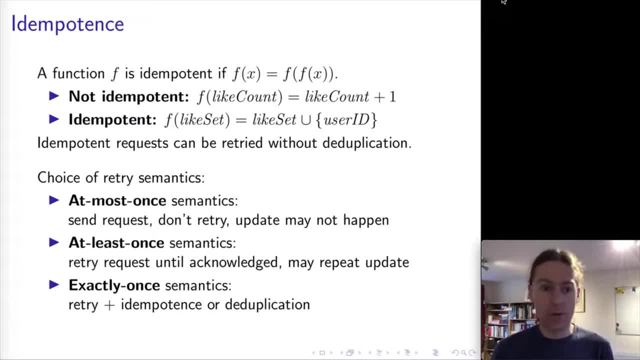 means even if the operation is applied multiple times, the effect is as if it had been applied exactly once. Or, of course, we can achieve exactly once through deduplication as well, as long as we're willing to store the requests that have already happened. 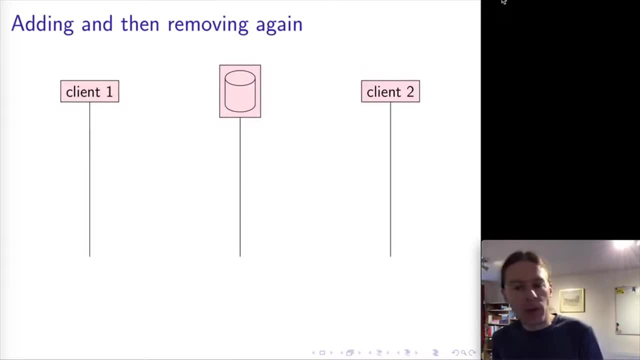 in some form. So let's have another problem. look at another problem which highlights the limitations of idempotence, And that is we've got two different clients this time, and client one wants to add a like or add your user ID to the set of. 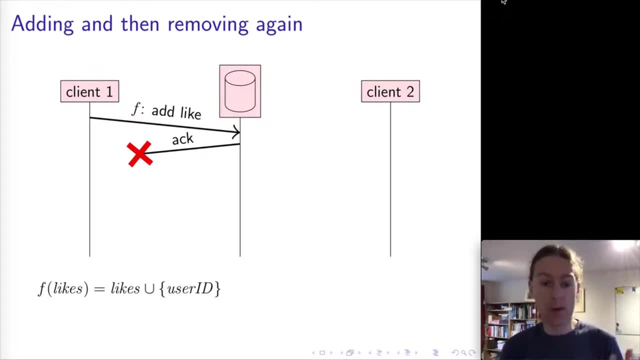 users who have liked a particular update And, as we've seen, this is an idempotent operation. this function f is idempotent. Now client two reads from the database. it reads the current set of users who have liked it and decides to unlike this. 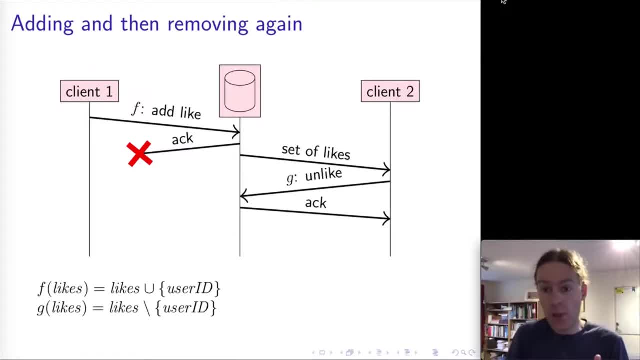 And so what this means is to remove a particular user ID from the set of users who have liked a particular update, And client two makes this request g and sends it to the server, and the server acknowledges it. Now, the first request that client one made. 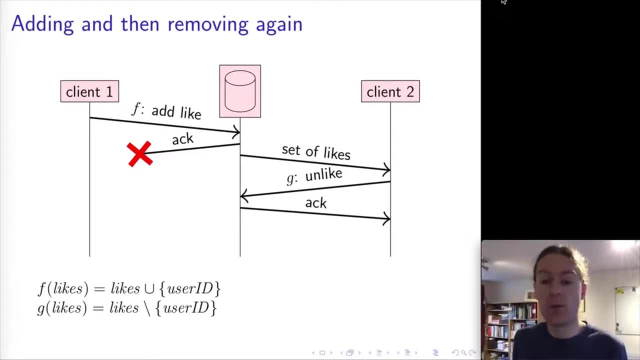 the acknowledgement got lost in the network, and so client one is going to retry this request, And so what the effect is now is that client one sends this request to add the like back to the server again, and the server, though, has actually just removed the like. 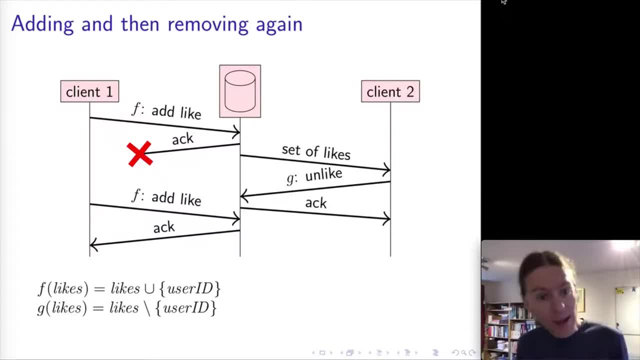 from the set of user IDs, and so it's going to add it back in again. And so here, even though the function f is idempotent. so applying the like twice has the same effect as applying it once, in the context of also having. 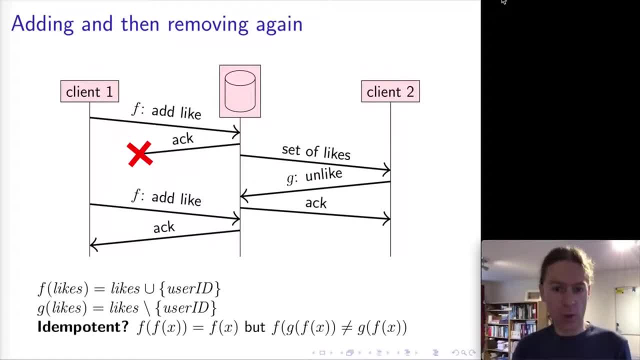 this unlike operation. actually the idempotence doesn't quite work anymore, because if we apply first f, then g, then f, then this is not the same as just applying first f then g, because the second application of f is going to add the element back into. 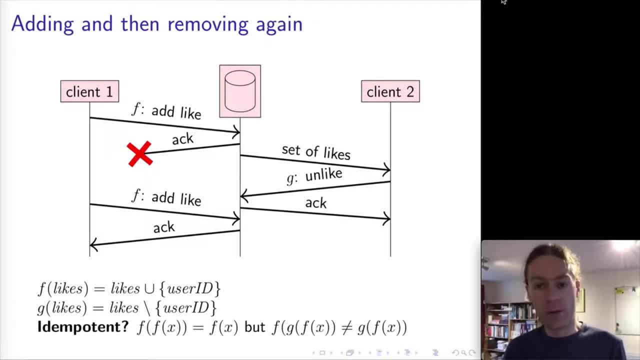 the set again, And so here the user intention was that this item should not be liked, because the user first liked it and then unliked it, and this retry of adding the like still causally belongs to this first request here. So it's not. 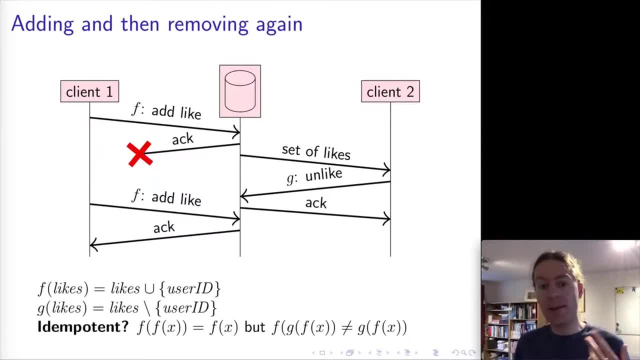 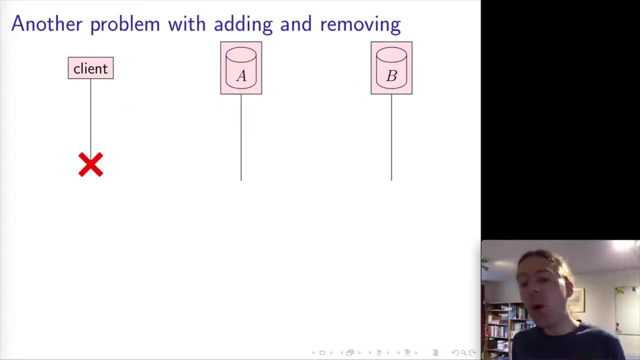 a separate request to add it back in again, but the actual intention is that the end result is: this update is not liked. So let's have a look at an approach that we can use to solve this problem, And I will illustrate this with another. 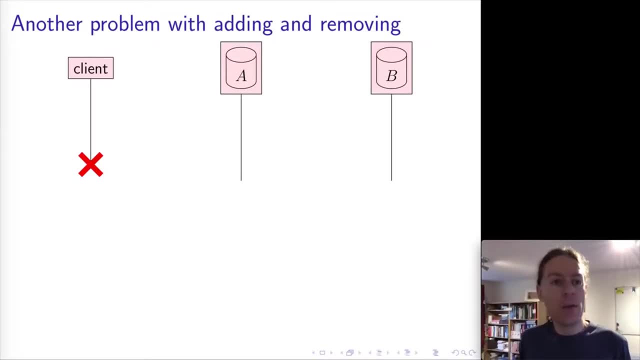 problem that can happen with replication, And so in this case, here, what we have is a client that wants to add an element x to a set, And so I'm just going to treat it more abstractly. let's forget about status updates and likes for now. 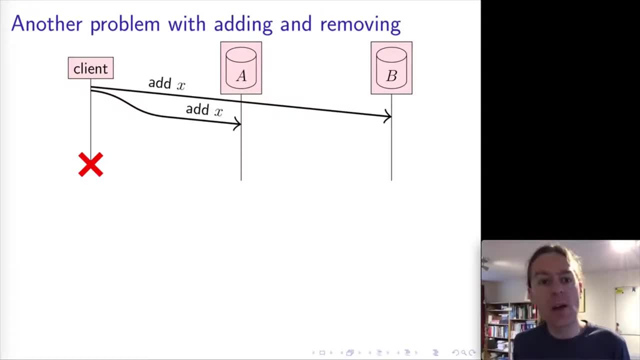 Just more abstractly, we have some element x that needs to be added to a set on both replica A and replica B, And first the user adds it and then the user wants to remove it again, Because people can change their minds. okay, fine. 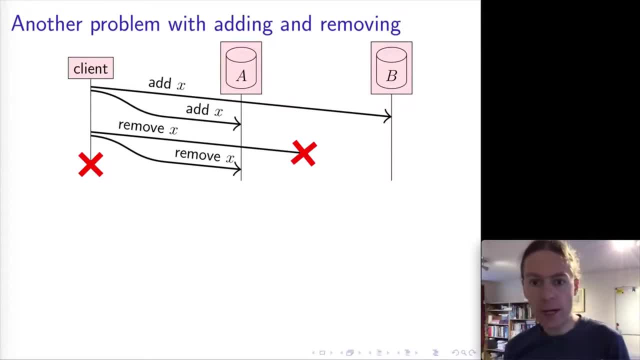 And so first we have an add request that goes to both replicas, then we have a remove request. Now, unfortunately, the remove request is lost in the network on its way from the client to replica B, So replica A receives both the add and the remove. 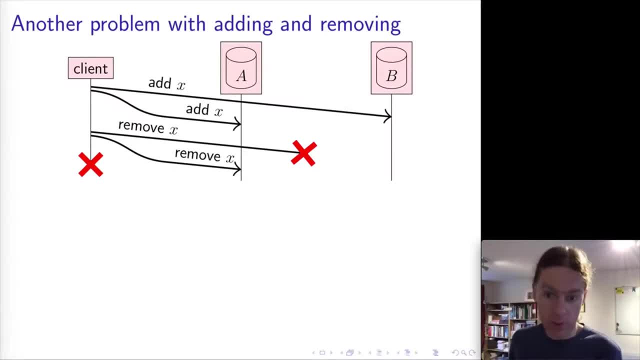 but replica B only receives the add and it doesn't receive the remove. So the end result now is that the element x is in the set on replica B, because it hasn't been removed, but x is not in the set on replica A because there it has been removed. 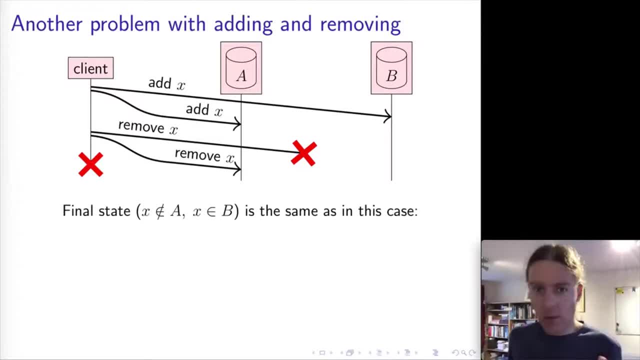 Now, if you think about this, the state of the two replicas in this example here is exactly the same as in this example. So in the second example the client wants to add x to the set. The addition goes through and reaches replica B, but the addition 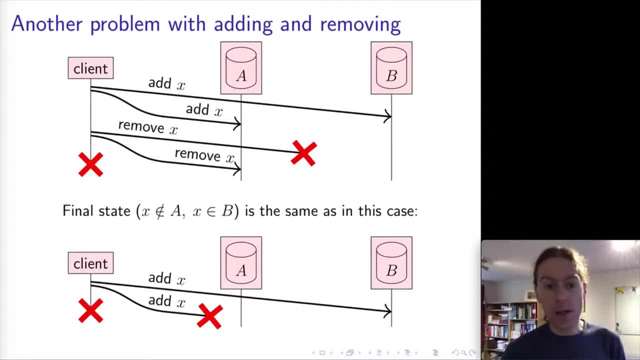 is lost on its way to replica A. So again we have the same state, that x is present on B but absent on A, And these two so that the final state of the two replicas is the same in these two examples. But actually we don't want it to be the same because 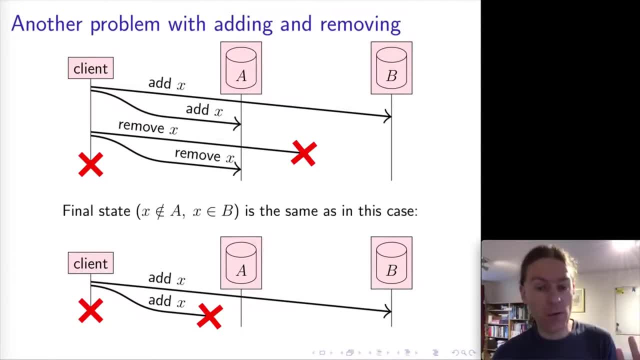 the user intention was different In the case of the first scenario. here the user first added, then removed. So the user intention was that the final state should be that x is not in the set, Whereas in the second scenario the user only added. 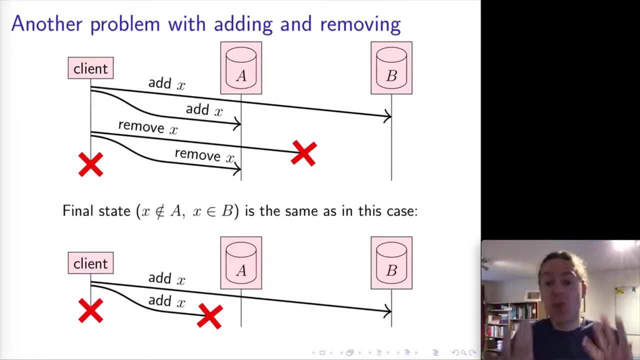 the user didn't remove anything. so the user intention is that x is present in the set. So the user intention is actually different in these two. but from the point of view of the replicas these two outcomes look the same, And so we have to. 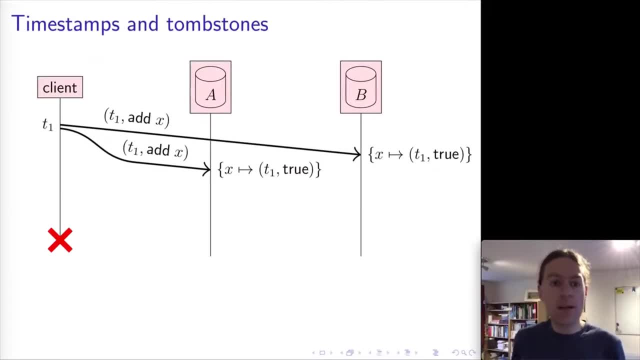 distinguish these two outcomes, And the way we can do that is by adding timestamps to things. So we're going to reuse what we've learned before about logical timestamps And we're just going to have the client generate a logical timestamp when it makes the 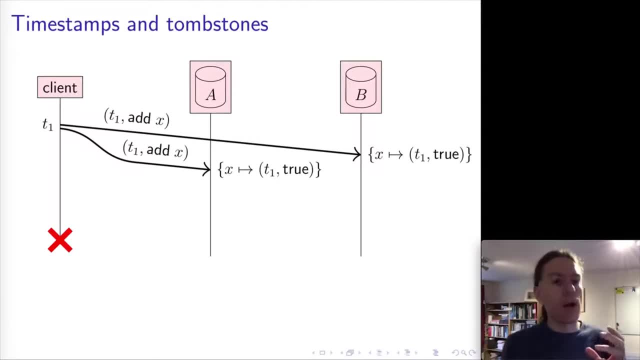 request to the two replicas. And so the client generates this timestamp t1 and it attaches t1 to the add request that is sent to both A and B, And now A and B both store this timestamp t1.. And I'm also going to associate: 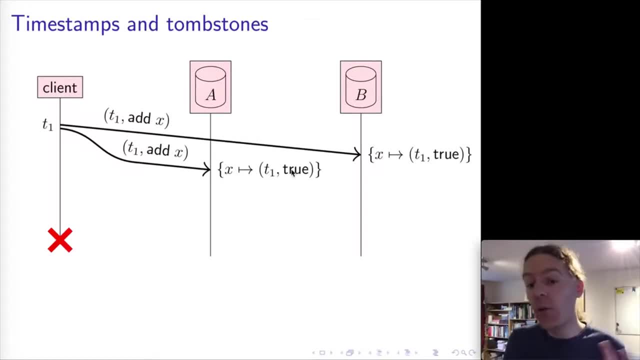 here x with a value true, And true here just means that x is present in the set, And we will see in a moment why we need this. because what happens next is now that the client makes a remove request And because this is a new request, it makes a 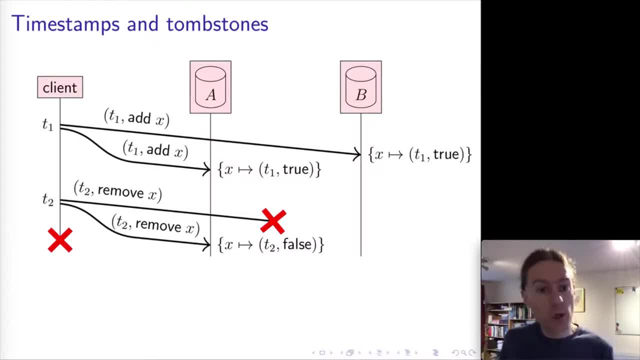 new logical timestamp, t2, attaches t2 to the request. The request is sent to both A and B Now because this is a logical timestamp and the remove happened after the add. this means that t1 will be less than t2, t2 will be greater than t1.. 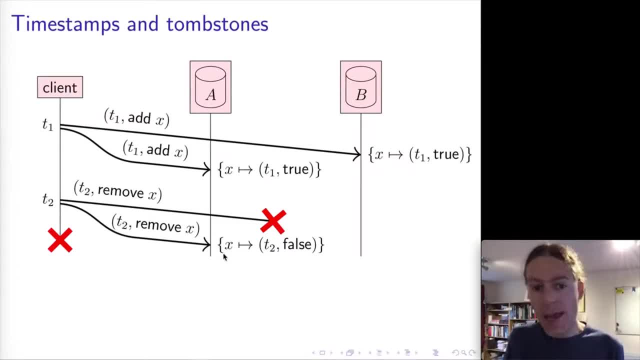 And so here we have replica: A receives the request to remove it, remove x. And so, instead of actually removing x from the database, A leaves x in the database and says, actually we're just going to attach this value false here to x, And false means: 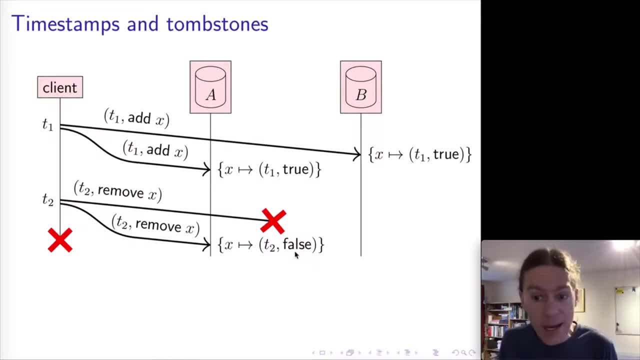 treat the value x or treat the element x as if it were not present in the set, Because the user asked that we remove it. but we're not actually going to remove it because otherwise we wouldn't know whether the user added or removed it. So 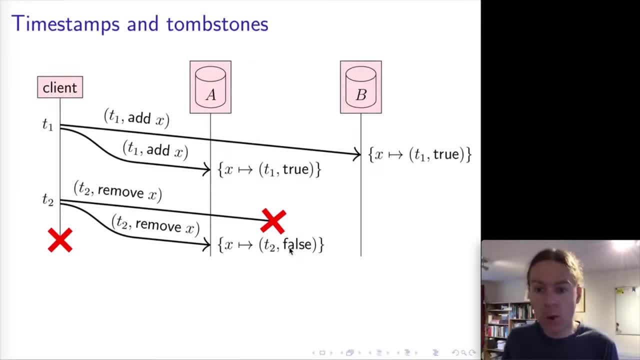 we're going to leave this marker in the database marked as false, saying x is not actually in the set and the deletion happened with a timestamp of t2.. So here now we can distinguish. on B we have that x is present because it has a value of 2 with a. 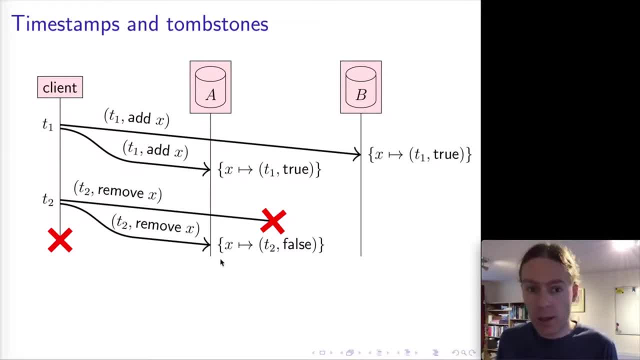 timestamp of t1.. On replica A, x is absent because it has a value of false and a timestamp of t2.. So this construction, where we don't actually delete something but just mark something as deleted, is called a tombstone, and this appears in various different distributed. 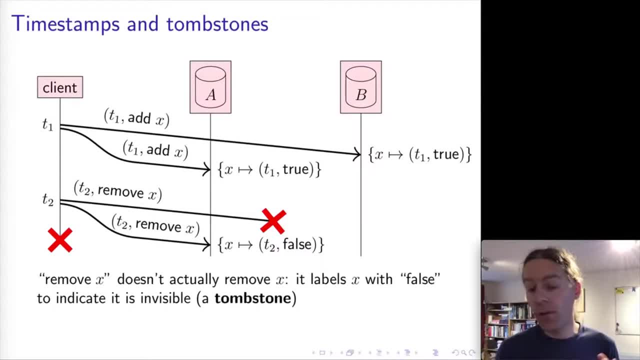 algorithms when we have to deal with deletion. So tombstone just means something was supposed to be deleted, but for internal reasons we have to actually keep it, and maybe tombstones can get garbage collected at some later point in time. that's a separate question, but 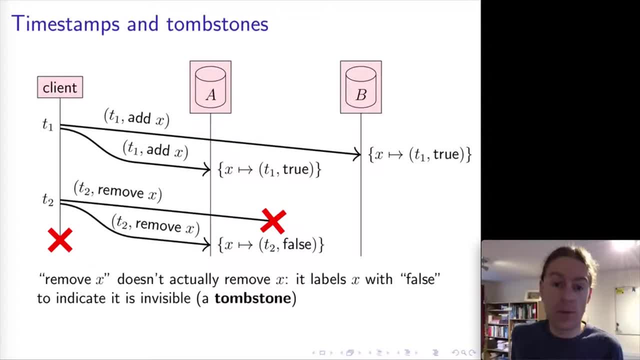 for now we just need to keep remembering this item, even though it has been deleted, And of course, we attach this logical timestamp. so every time some object in the database is written, we attach the timestamp of the last operation that wrote it, and this allows us to tell which values are. 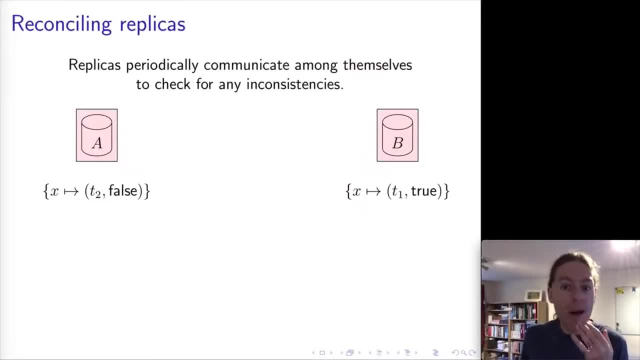 newer and which are older. So this means now that, after this has happened, A and B are no longer in the same state, because A received the request to delete x with a timestamp of t2, whereas B did not receive that request because it got lost in the network and so, according. 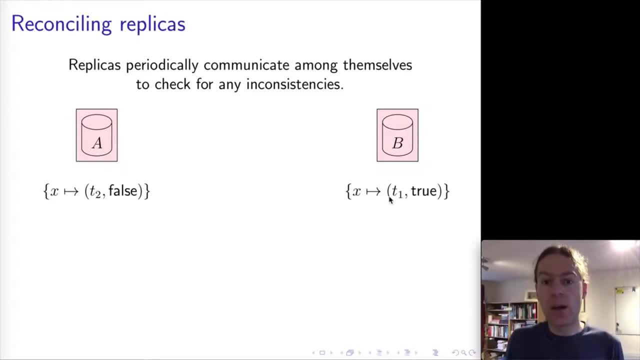 to B x is still present in the set and it has a last modification timestamp of t1.. And now the two replicas can run a protocol in which they compare what they have, they compare their data, and this protocol is called an anti-entropy protocol because 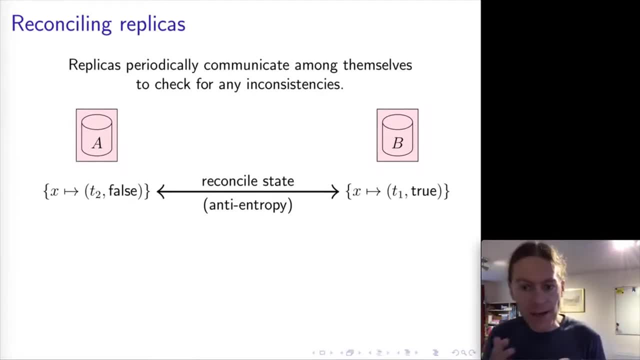 I guess it's sort of it's supposed to clear the entropy in the confusion and the uncertainty in the system and bring all of the replicas back into the same state, And so as A and B reconcile their state and perform this anti-entropy protocol, they will compare their timestamps. 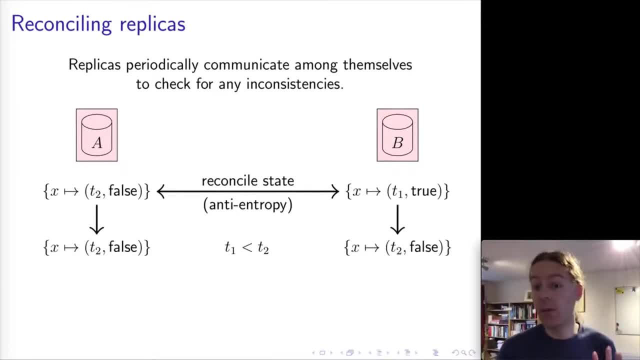 and since we have these logical timestamps attached to every data item, they can realize that t1 is less than t2. so, therefore, this value that B has must be older, the value that A has must be newer, and so therefore, the object the record on B is going to get. 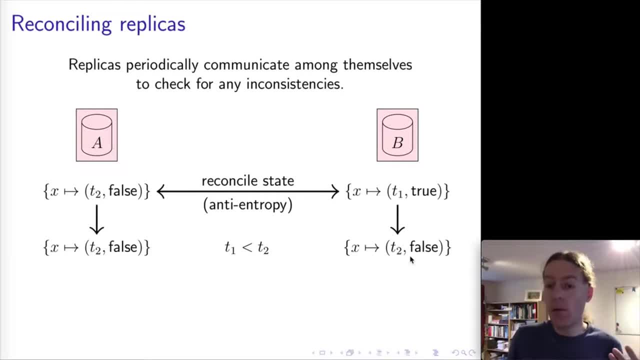 replaced with the one from A. So the one from A is the more recent one, so that gets propagated to B, And so here the timestamps have helped us because they tell us about the recency and the relative ordering of these updates. so timestamps have been very useful. 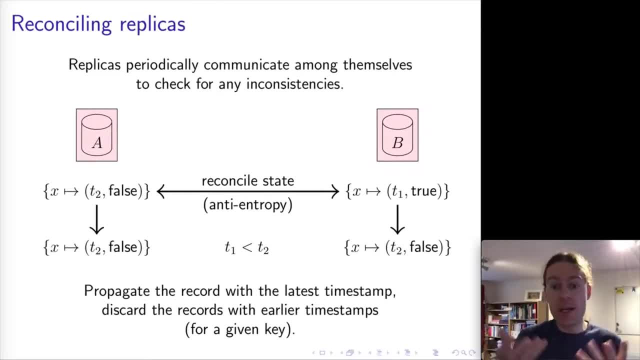 And so typically we will probably have one timestamp for every given key or every object in the database, because that's the granularity at which we're going to do that reconciliation. Now, what kind of logical timestamps do we use here? So in our last lecture we saw the 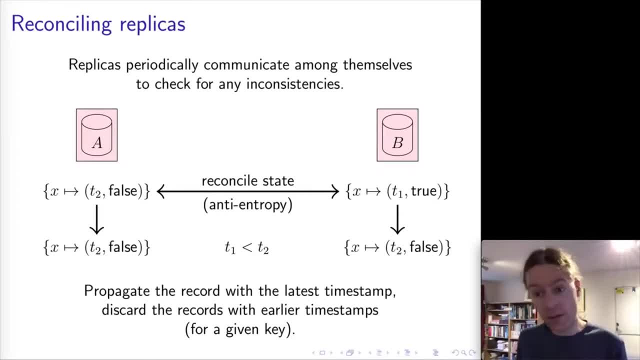 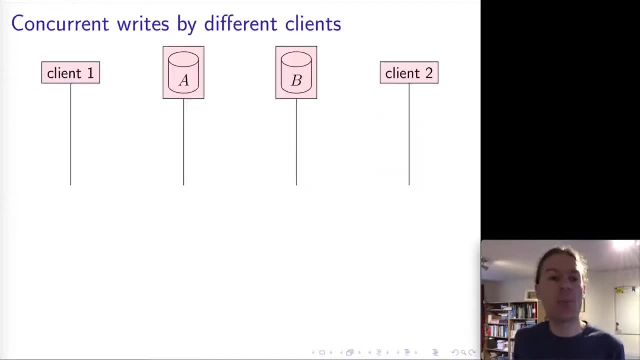 distinction between Lamport clocks and vector clocks and in fact we can use both in databases and we get slightly different behavior. so it really depends what behavior we want, And this becomes apparent if we consider two clients that are making writes to this replicated database concurrently. 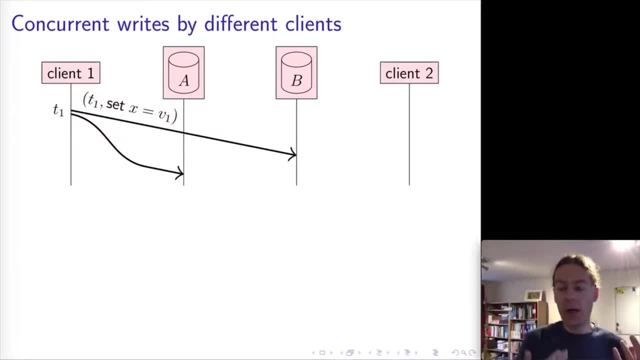 So here on client 1, client 1 wants to update the value that is associated with some key x. So x is the key, v1 is the value that client 1 wants to attach to x, and this operation is going to have a logical timestamp of 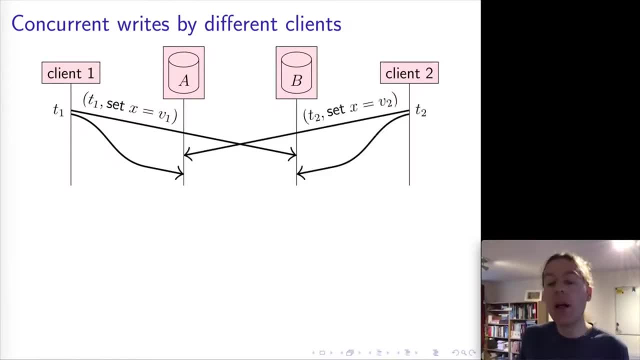 t1.. Concurrently, while this is happening, client 2 also wants to set the value of x. It wants to set it to a different value, v2.. So client 1 also generates a logical timestamp. t2 sends an operation of the. 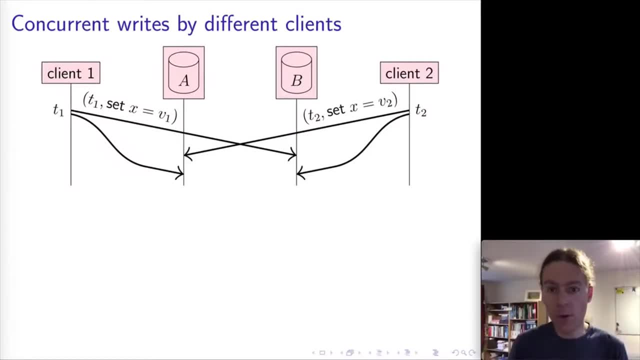 network. attached t2 to this operation. The operation is: I want to set the key x to the value v2.. Now notice that replica a first receives the request from client 2, second receives the request from client 1,, whereas replica b receives them in the. 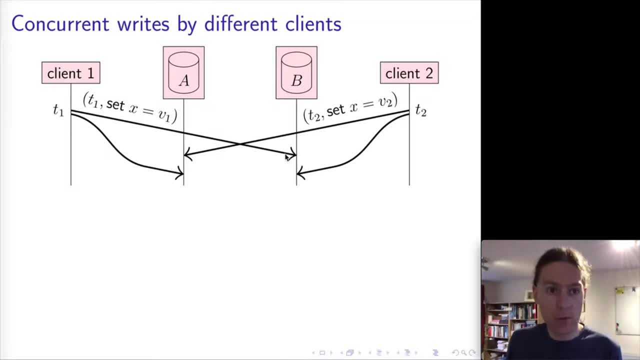 opposite order. Replica b first receives the request from client 1, then the request from client 2.. So this means the replicas can't just use the order in which they see the requests in order to determine whether v1 or v2 is the final value. 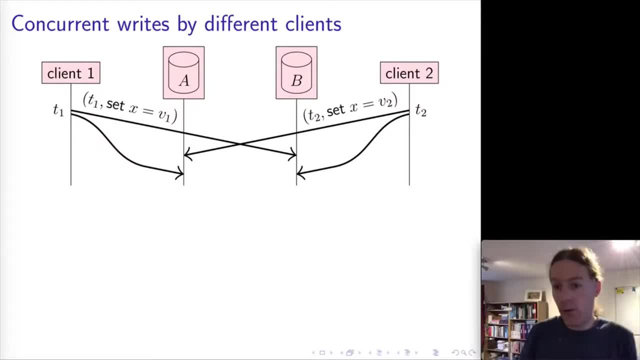 for x, because if they did just use the order in which the requests arrive, then they would end up in different states. They would end up inconsistent at the end, And so what we want in a replicated system is that all of the replicas end up being in the same state. otherwise, 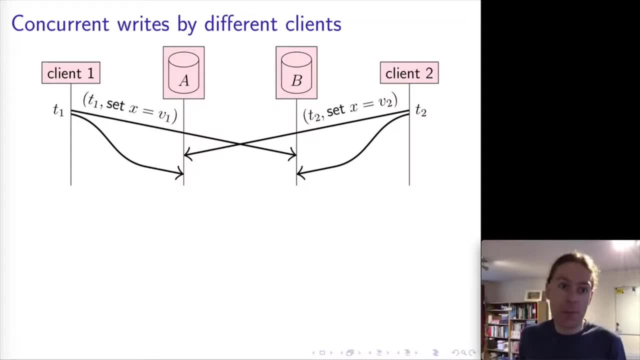 it's not replication, And that's why we need to use the timestamps here, because the timestamps provide a relative ordering of these two operations. Now, one option is that we use Lamport clocks, and if you remember, what we have with Lamport clocks is they give us a total. 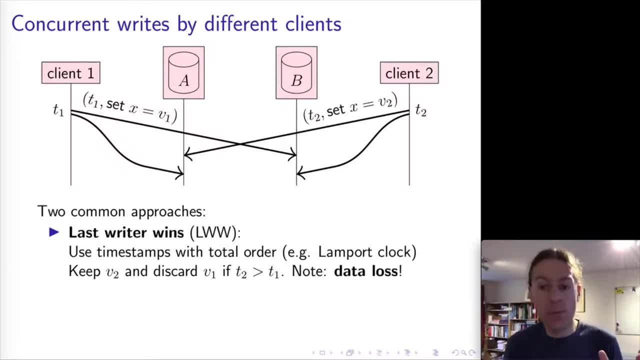 ordering. So total ordering means that for any two timestamps that exist in the system, we can always compare them, and it will always be the case that one is less than the other, And so in this case, for example, we can say that t1 is less than. 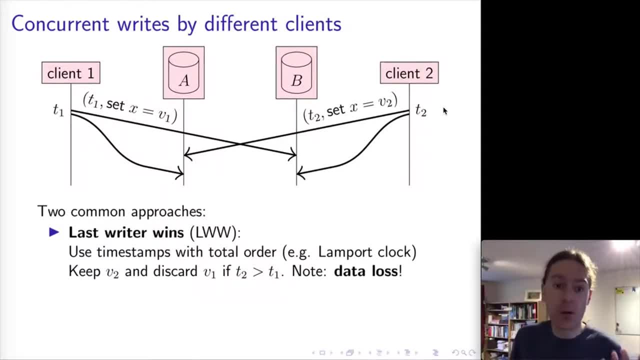 t2,, but it might just as well be the other way around, because in this case the two operations are concurrent, and so the ordering that the Lamport timestamps provide us is arbitrary, essentially, And so what we can do here, for example, is that 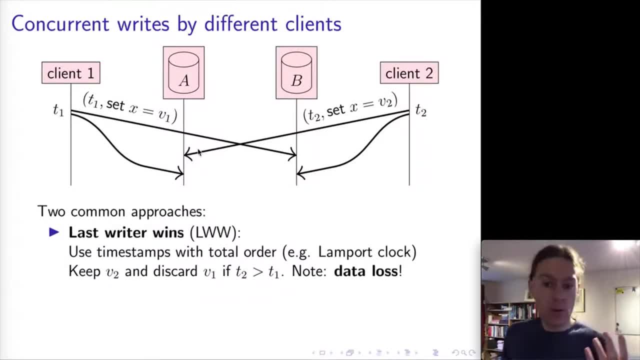 we compare t1 and t2, and we just keep the value with the higher timestamp, And this will work, because then, as the value gets overwritten, we know that the overwrite happens after a previous operation and therefore it will always have a greater timestamp. So 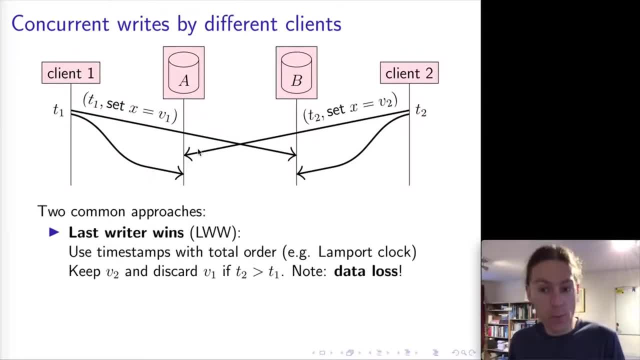 therefore, overwriting a smaller timestamp with a greater timestamp is a fine thing. you can do that, And this behaviour is called LastWriterWins, because we assume that the last one, the last writer, is the one with the highest timestamp, and so the highest timestamp wins. 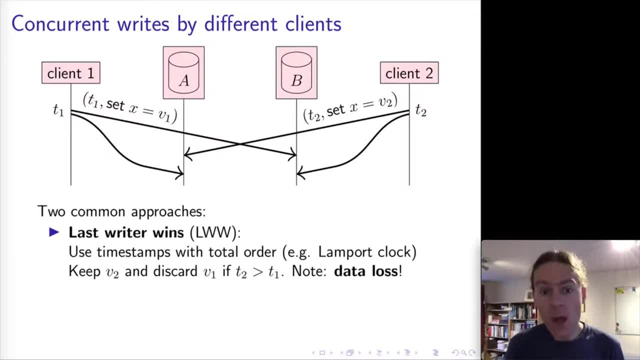 if there are several concurrent updates with different timestamps. Note, however, that this means that if, say, t2 is greater than t1, this means we keep v2, which was written by client 2, and we simply discard v1.. So 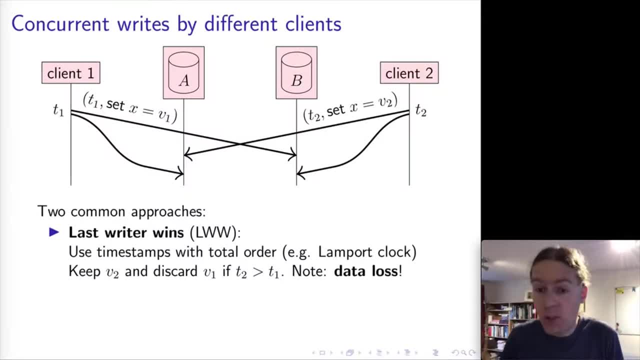 value v1 is simply gone, So we're not even storing that value anywhere. it simply gets overwritten and forgotten, And this might be okay depending on the application. There might be applications in which, actually, if there are two concurrent writes, it's fine to just keep one and 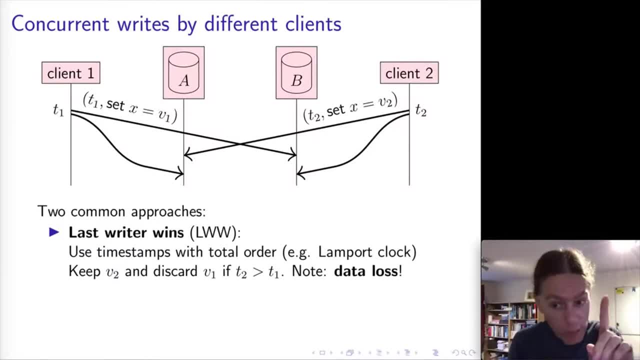 throw away the others. If there are five concurrent writes, we're going to keep one and throw away four of them. But there might also be scenarios in which, actually, if there are several concurrent writes, we want to keep all of them and we want. 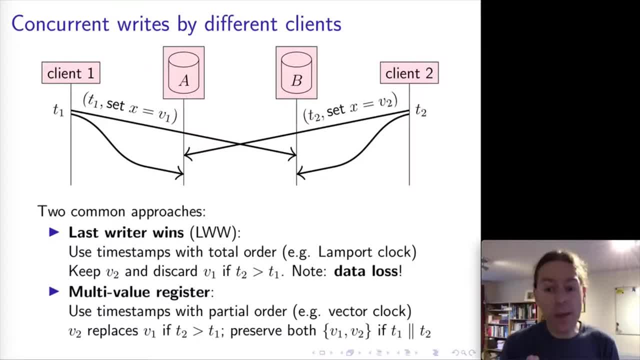 to explicitly resolve this situation And if we want that well, we use a vector clock instead of a Lamport clock. If we use a vector clock, then if we generate two different timestamps- t1 and t2, and these two operations are concurrent. 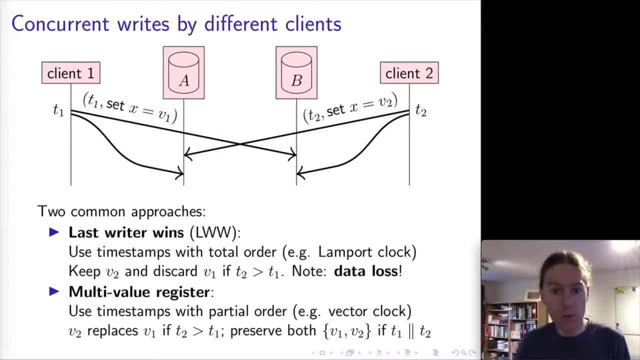 then the vector clocks will also be incomparable. We will end up with t1 and t2 being incomparable, and this allows us to detect the fact that these two operations are concurrent. And so in this case now, we will only overwrite one value with another value if 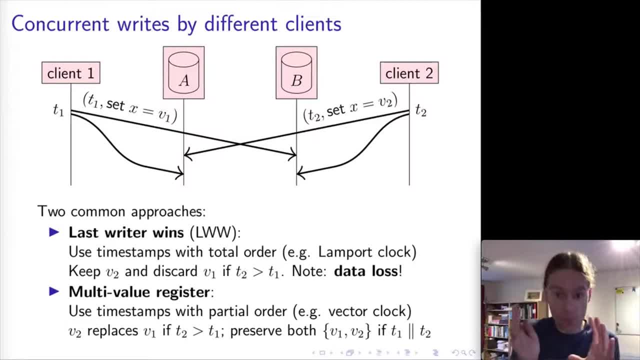 their vector timestamps are the later ones strictly greater than the earlier one under the strictly greater than relation that we've defined previously. But if we have two concurrent updates, then we will keep both of them, And so in this case, now there's not. 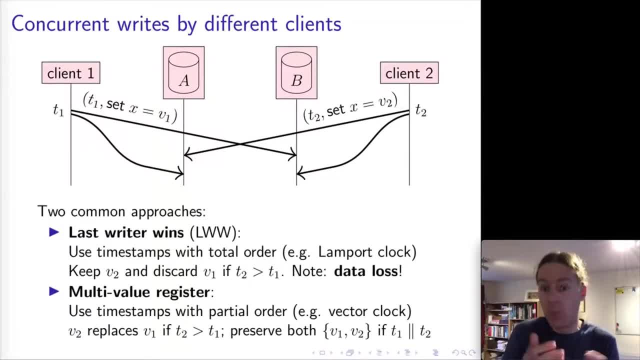 a single value attached to the key x, but there could be multiple values, in this case v1 and v2.. And so in this case we can give those two values back to the application and the application can then resolve this. This is called a conflict. 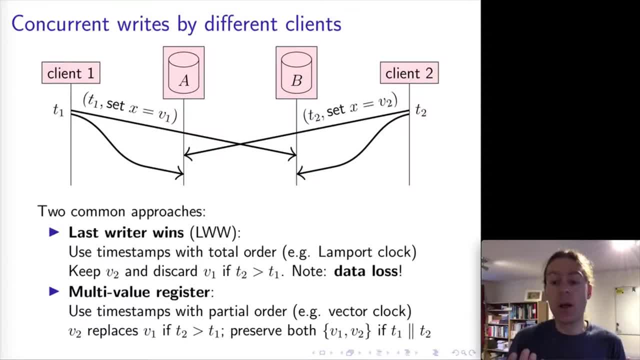 and the application can have explicit logic for conflict resolution, so that if these two updates happen concurrently and we have two different values written by different clients, then we can avoid throwing away data. We can combine the information from these two values that were written concurrently. 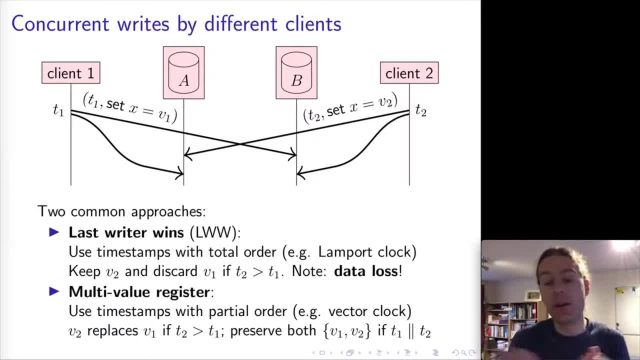 into a single value, write it back to the database again, and that ensures then everyone is happy and no data was lost. So we have this choice here, using either the totally ordered Lamport timestamps or the partially ordered vector timestamps, depending on which kind of behavior we actually want. 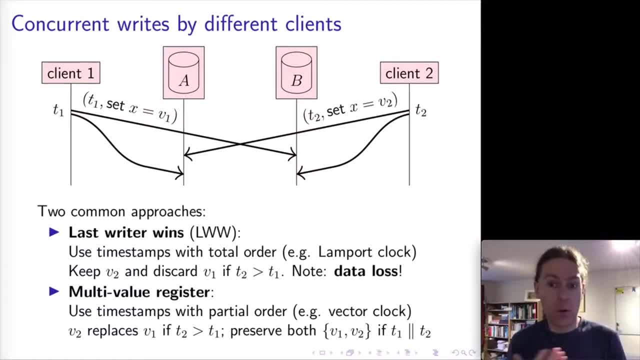 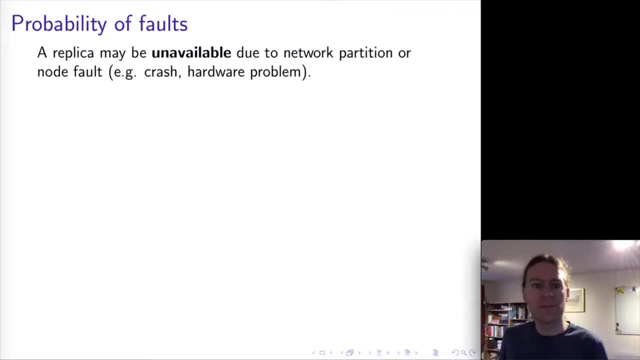 Different database systems actually make different choices with regard to what sort of timestamps they want to use, because for different applications, different methods are appropriate. So far that, and next we will look at fault tolerance in replication. The reason we want replication is typically to make systems. 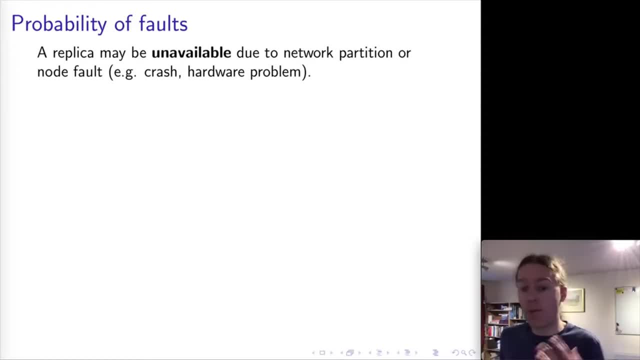 more reliable. So a node might be unavailable for all sorts of reasons: It might crash, it might have a hardware problem, it might be just rebooting due to routine maintenance. Let's assume just there's some probability p that a node is unavailable. 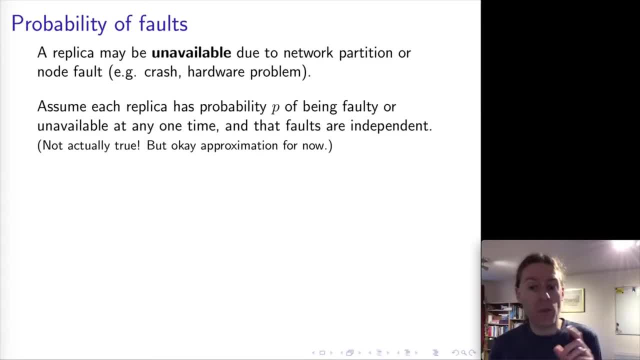 at any given time. Let's also assume that whether one node is unavailable is independent from whether another node is unavailable, So we're going to assume that faults are not correlated. This is not actually true. There have been studies that have shown that actually. 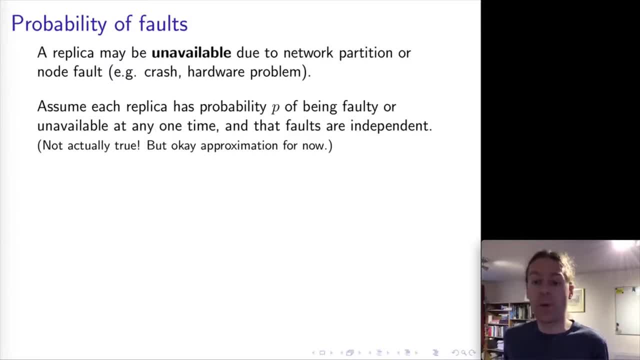 faults do tend to be correlated in practice, but just for the purposes of some rough estimation, it's okay for now to assume that they are actually independent. So now, if p is the probability of 1, any one node being faulty, that means the probability of all. 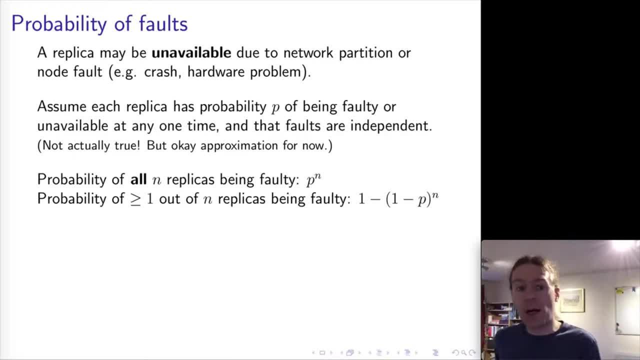 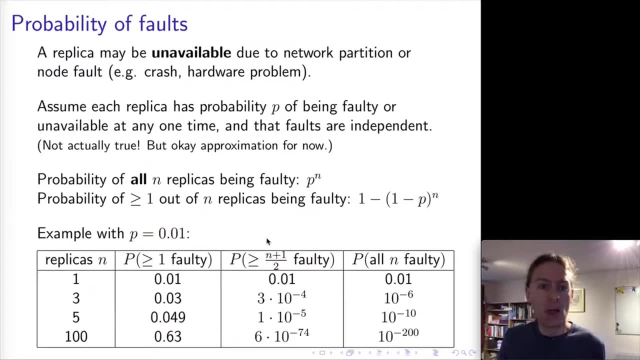 n replicas being faulty is p to the n and we can work out what is the probability of one or more being faulty and we can make a little table. And what this table shows here is, if you look at the column, for at least one. 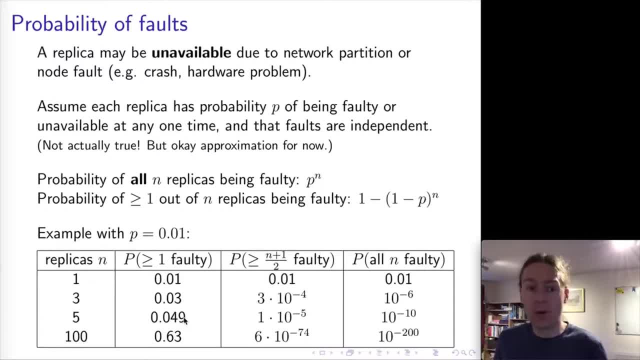 node being faulty. as you increase the number of replicas, it becomes almost certain that at least one of them is faulty at any given time. So, in that sense, as you add replicas, the system becomes less reliable because given any one has a chance of failing, as you have loads of replicas. 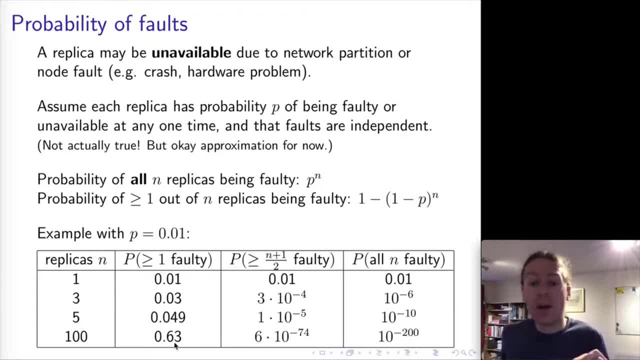 there will always be one that is failed at any moment. However, if we take the probability of all of them being faulty, this probability decreases exponentially as you increase the number of replicas. And even if you consider not the probability of all of them failing, but just the probability of half, 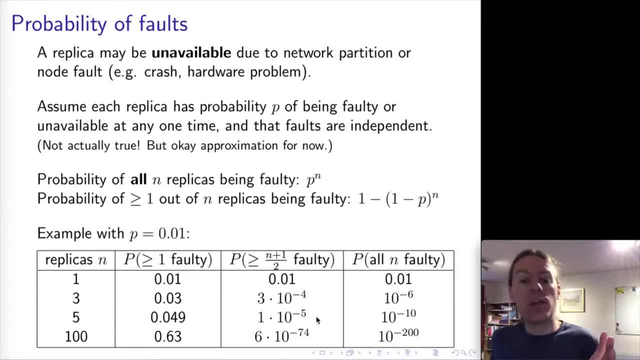 of the nodes, half of the replicas failing. this probability also decreases exponentially with the number of replicas. So this is why we can achieve fault tolerance, because as long as it's okay if some of the nodes are unavailable, some of the replicas are unavailable. 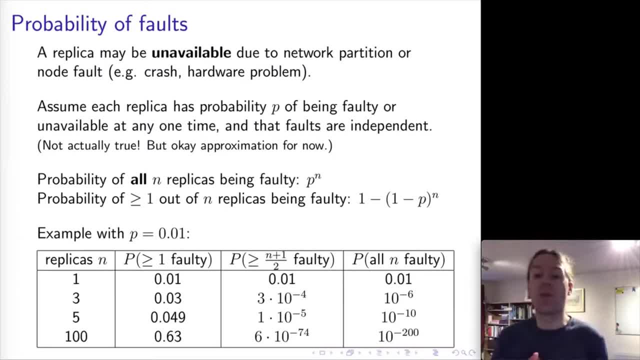 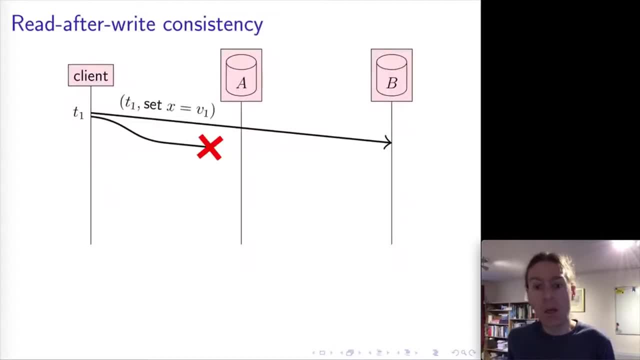 we just have to make sure that, given at least most of the replicas are available, then the system continues working and then we can actually achieve very high reliability. So let's look at one particular property that we might want in a fault tolerant replicated system, And that is called read-after-write. 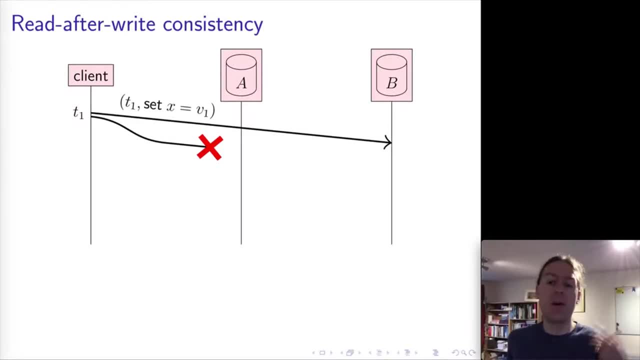 consistency. So what happens here is that a client first writes some data and then it reads the same data back again, and you would naturally expect that client to just see the data that it has just written. So here the client wants to set the key x to the. 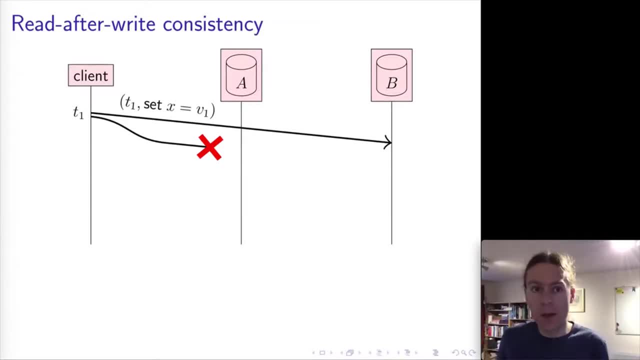 value v1 and we attach a timestamp of t1 to that operation. It sends that update to both replicas of the database a and b. The replica b receives that update and processes it, whereas replica a is unavailable, and so the update is not processed by a. 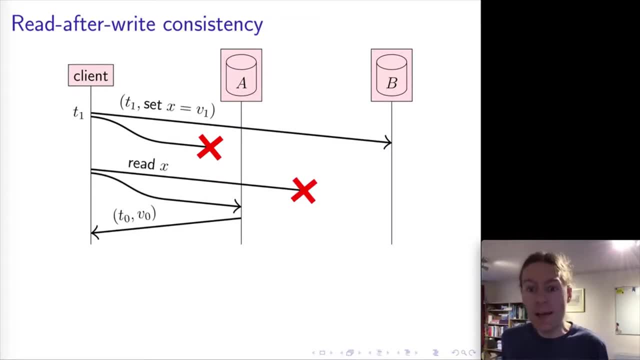 Then subsequently the client goes and wants to read x again, but for some reason now the things have flipped around and now a is available but b is not available, And so now the response that the client gets back from a does not reflect that value. v1. that has been written. 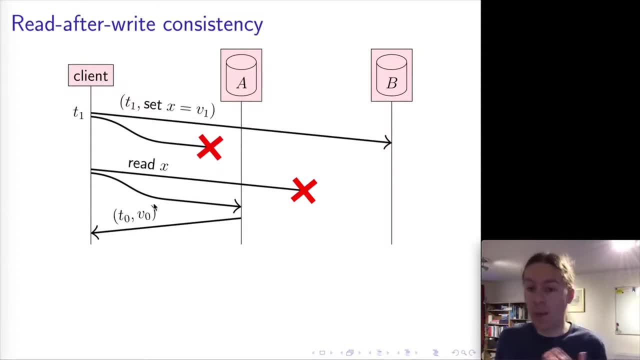 So the response is going to be some earlier value v0 that the replicas had before this scenario here started. So in this case we have violated read-after-write consistency, which is kind of unfortunate because it's very confusing if you write some data and then the data disappears and then 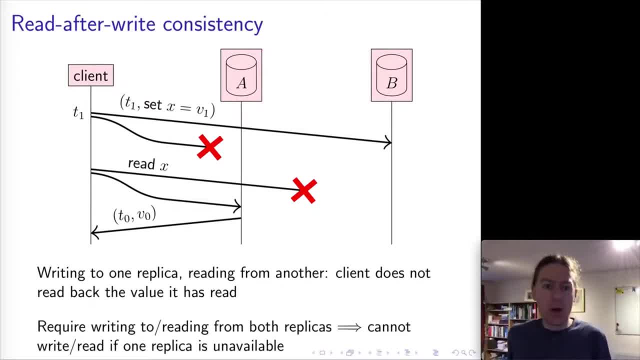 sometime later, the data reappears again. Now what we could do here in this case is that the read and the write have to go to both replicas, and so that way we would ensure that we don't get this crossover problem where only one of the replicas 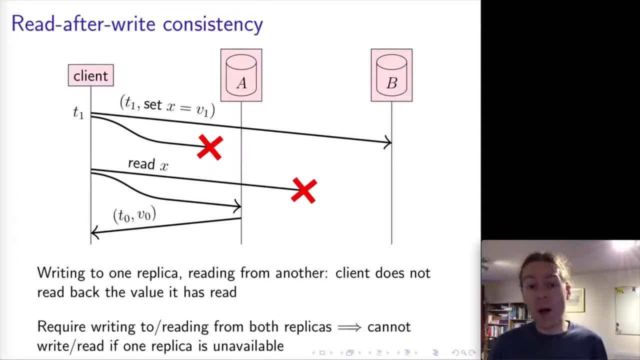 has seen the update and we read from the other one. But now if we require a read or write to go to both replicas, then the system is not fault tolerant, because if just one of the two replicas becomes unavailable, then we can't process reads or writes anymore. 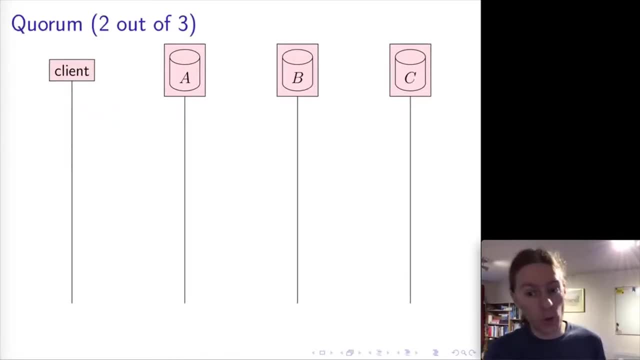 So we can solve this problem using something called a quorum, And what we do here is here I've got an example quorum of two out of three, And so when we want to make a write, the client sends its request to. 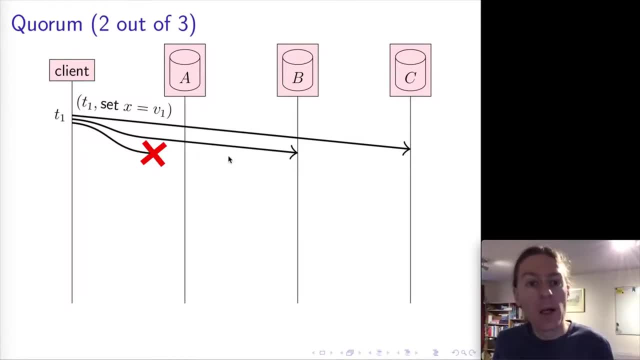 all three replicas. We're going to assume here there are three replicas and for some reason the request reaches two out of three of these two replicas. So the request reaches B and C but not A, And then B and C are going to respond to the client saying: 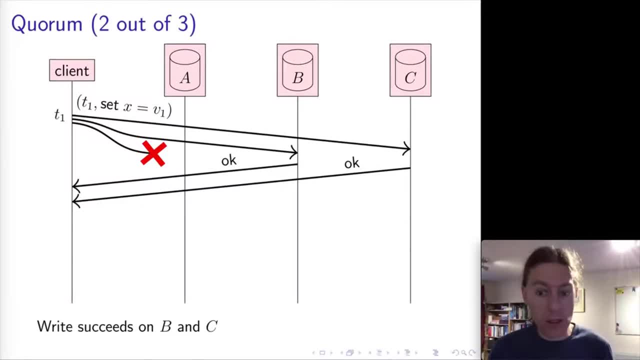 OK, yes, I got your request to update this particular key x, and once the client has collected two positive responses, then it's happy. So the fact that the response didn't, the request didn't get through to A, is OK, So maybe A is unavailable. 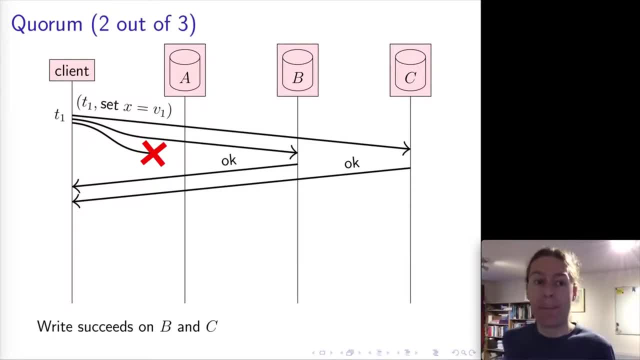 as long as B and C still respond, that's still fine. Now, second, the client goes to read, and it sends its read again to all three replicas. As before, only two of them get it, And so in this case, for some reason, the read to C doesn't go. 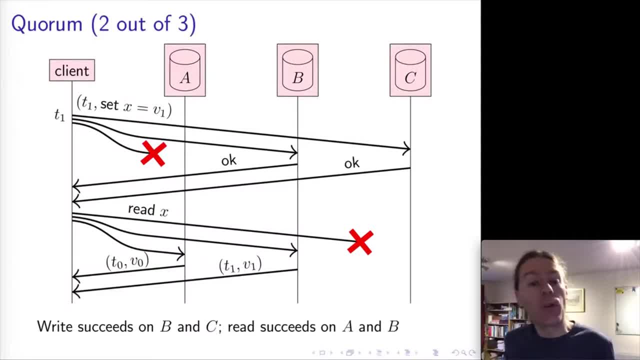 through, but the reads to A and B do go through, And so in this case now the client will receive responses from A and B. It will get the correct response that it was expecting from B, because B has seen the write. It will get an outdated response. 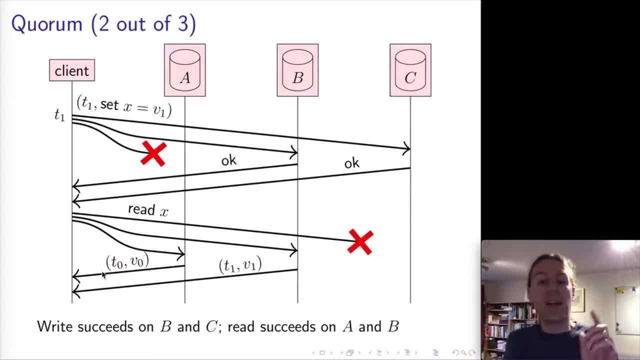 from A, because A didn't get the write, But at least one of the responses that the client got back has the updated value, And so now the client can use the timestamps T0 and T1 to figure out which is the more recent update, and this now allows. 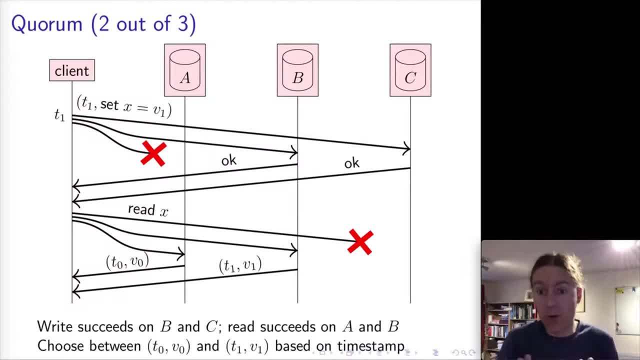 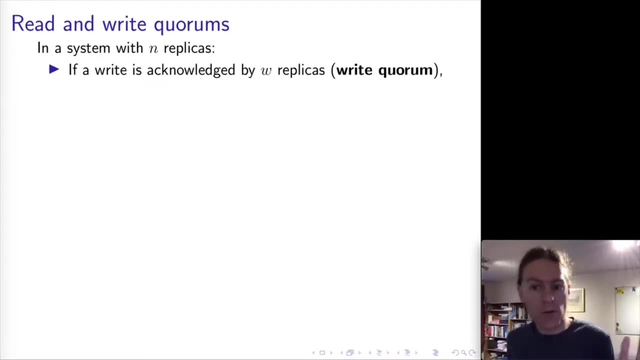 the client to know what the correct response should be: that it returns to the application and the application is happy because it has read after write consistency. So what do we have to do exactly to achieve this? We use quorums and whenever you want to make a write to some number, 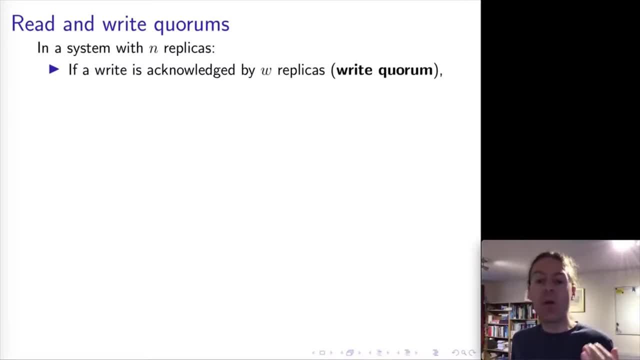 of replicas. the write will be considered successful as long as it has been acknowledged by at least W replicas. So this is our write quorum And then when you read, if you get a response back from at least R replicas. So now we have W and R as our two parameters. 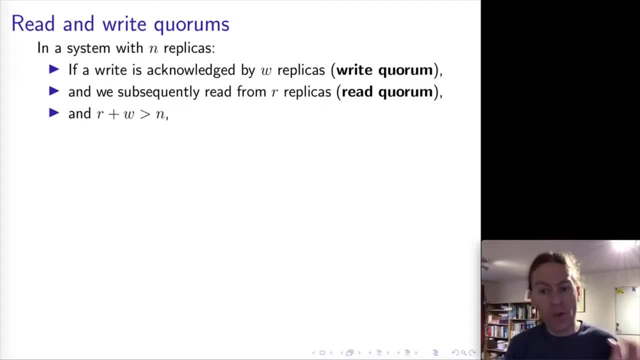 of this algorithm and we require that the sum of W and R is strictly greater than the number of replicas in the system. So in our example here W was 2, R was 2 and N was 3.. So 2 plus 2 is greater than 3.. 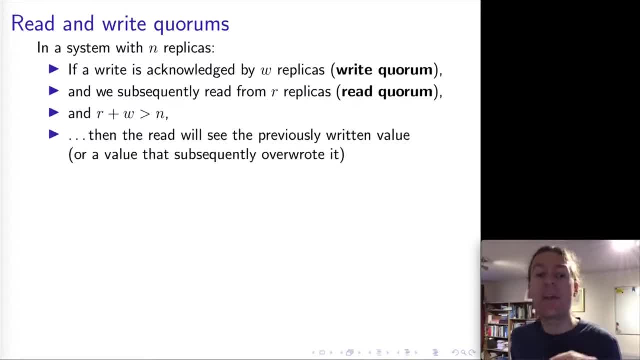 And so in this case we can guarantee that the read will see the previously written value- or maybe it was concurrently overwritten by another client, but it will see an up to date value, whereas if we have, if this R plus W is less than or equal to N, it could happen. 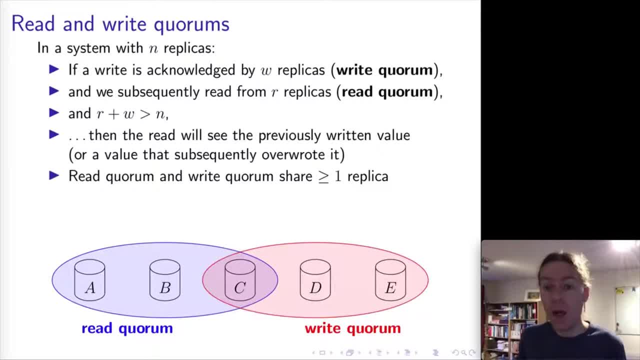 that we don't get the value back that we were expecting. So the idea here is that the write goes to some subset of nodes, the read goes to some subset of nodes, and we want those two subsets to overlap And we can guarantee that they will. 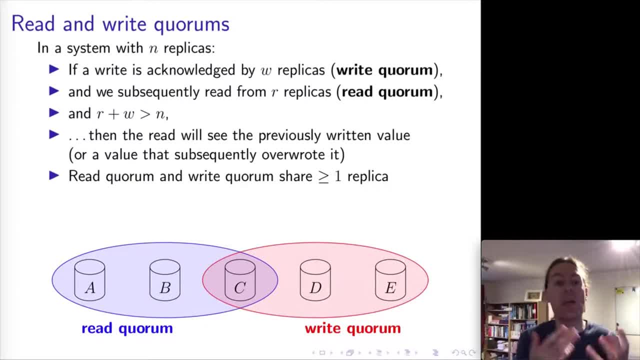 overlap in at least one replica. if we have this R plus W greater than N, this quorum condition. Another way of putting this is that we have these two subsets, and subsets of nodes have to have a non-empty intersection. So, for example, if we have 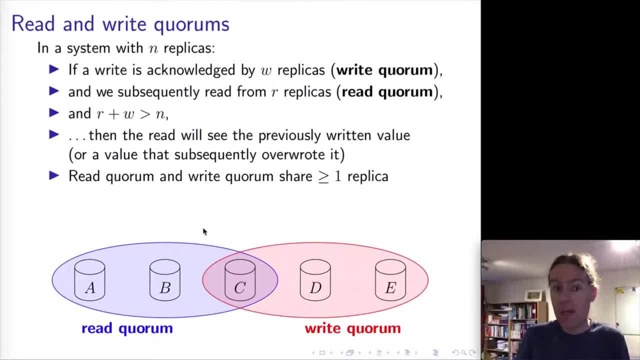 5 nodes, we could require a write quorum of 3 and a read quorum of 3 that would satisfy this condition, and in this case those two subsets of nodes are always guaranteed to have at least one element in common, so they will have a 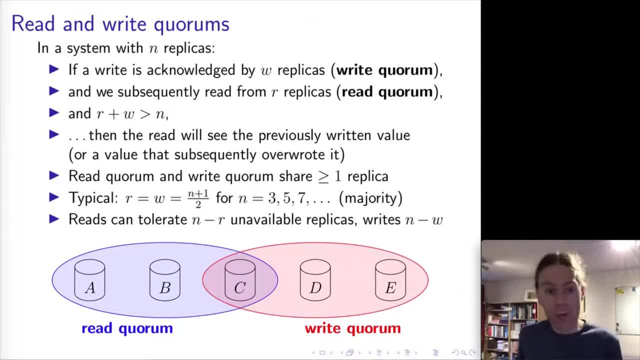 non-empty intersection. One common way of constructing these quorums is what are called majority quorums, where we say that we are going to assume that we have an odd number of nodes and as long as the read quorum and write quorum are strictly. 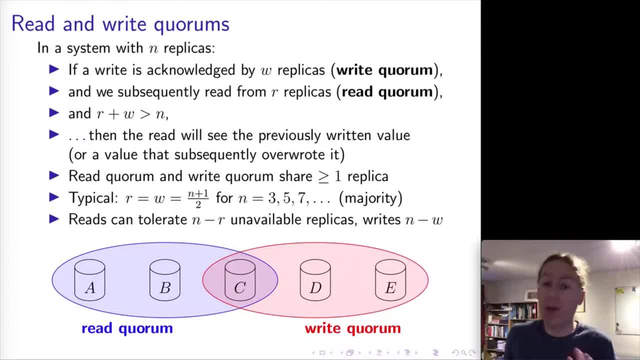 more than half of the number of nodes, then it's fine. So that means we require 2 out of 3, we require 3 out of 5, 4 out of 7 and so on, And this means now that in a 2 out of 3, 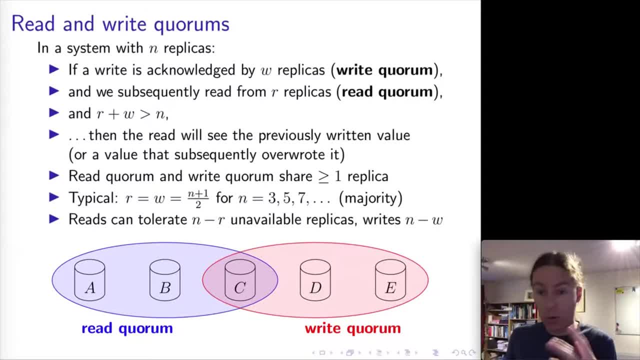 case, we can tolerate one node being unavailable as long as the other two respond. In a 3 out of 5 case, we can tolerate 2 replicas being unavailable as long as the three remaining ones respond, And so on. So this is all. the quorums are bad. 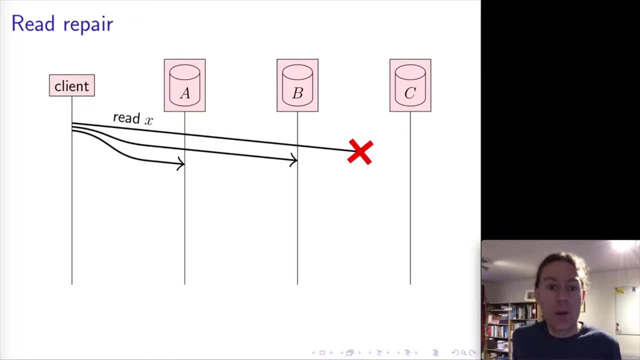 really, Now that we've done these- quorum reads and writes- one thing that we can do is for the client can help get those different replicas back in sync with each other again. So in this case here, the client received an outdated value from A and it received 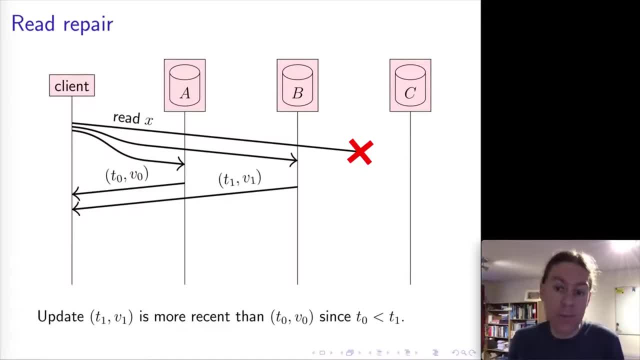 the up-to-date value from B and it didn't receive anything at all from C, And so the client already knows now that A and B and C are inconsistent with each other, And so the client can help clean this situation up by actually sending the update back to A and C. 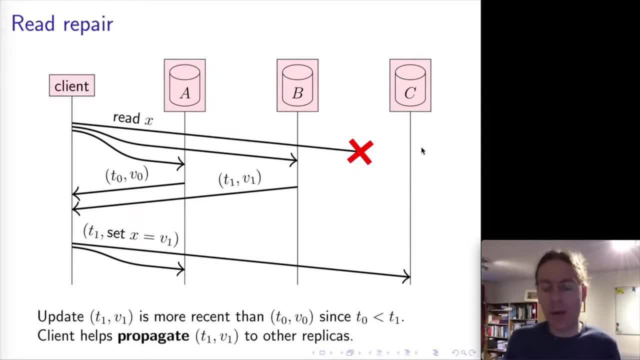 So C might not need it, because it might be that C actually has the up-to-date value. but it just didn't respond. But there's no harm in sending it again, And certainly we want to send the update to A so that now A and B both have the updated. 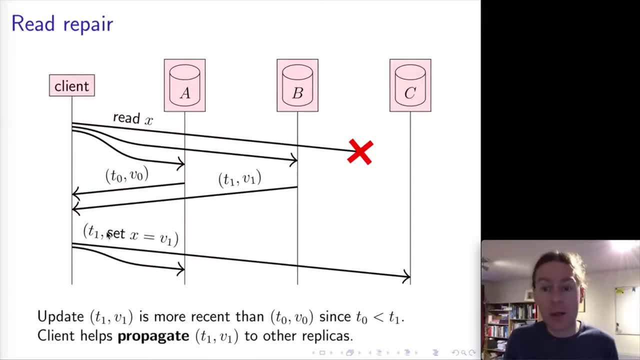 value B1.. So notice that we use the original timestamp here, because this is effectively just a retry. This is not a new set operation and therefore it's correct to use the right timestamp, And the client can thus help propagate the values between the replicas. 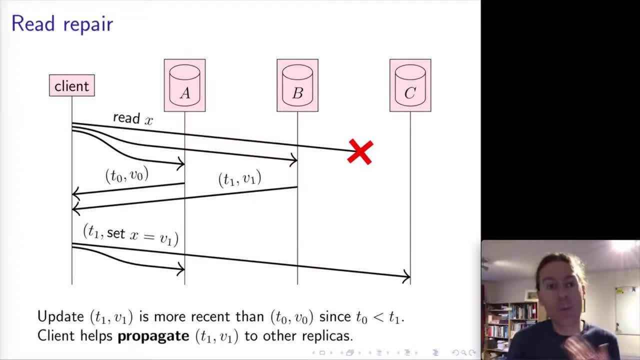 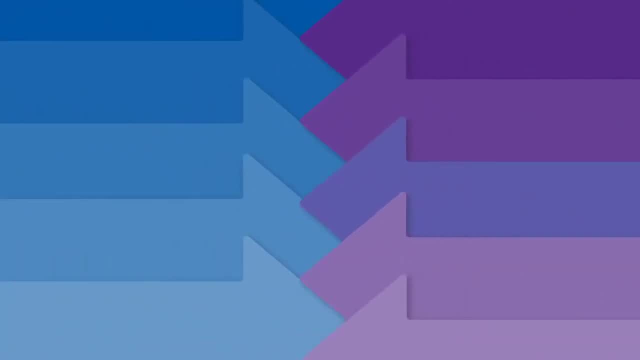 So we have the anti-entropy that we discussed earlier as one mechanism for the replicas to get back in sync, And this process- here, read-repair- is another way that helps the replicas get back in sync with each other. Hello and welcome to lecture. 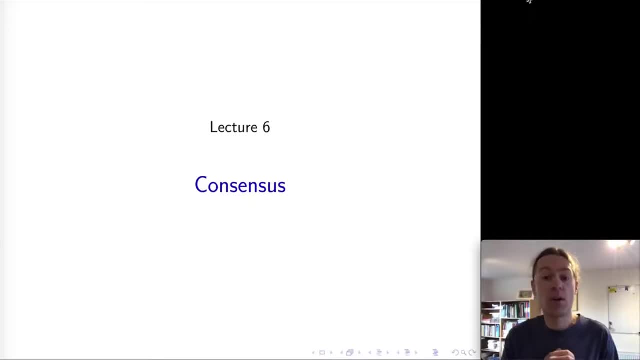 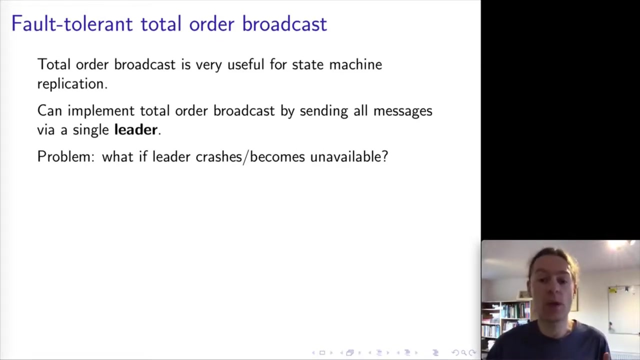 six on distributed systems. Today we will look at consensus, which is one of the most tricky but also one of the most important problems in distributed systems, And the context of this is last lecture. we talked about state machine replication, which is a great way. 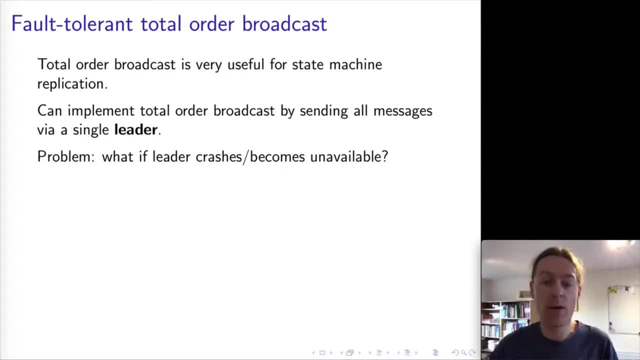 of replicating some data from one node to another, from one replica to another, And in order to do state machine replication, we need to ensure that all of the replicas see the same updates in the same order, which we can do with total order broadcast. This 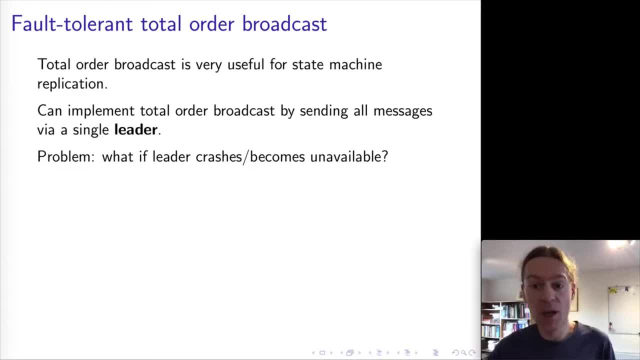 now raises the question of how do we implement total order broadcast. We saw one way of doing this is to send all of the messages via a particular dedicated node that we call the leader, And this node is going to order all of the messages and make sure. 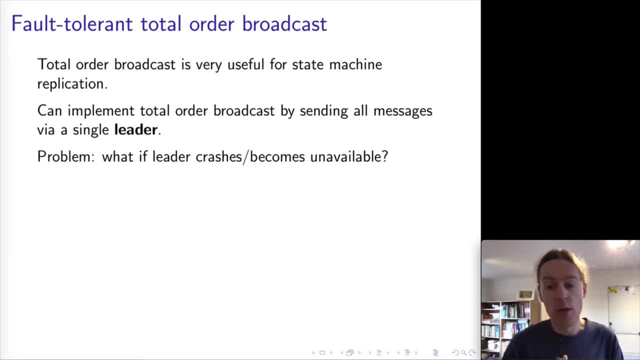 that they get delivered in the same order on all of the nodes. Unfortunately, if that leader crashes or it becomes unavailable due to a network problem, or it has a hardware failure or whatever anything goes wrong, then this approach to total order broadcast stops working. 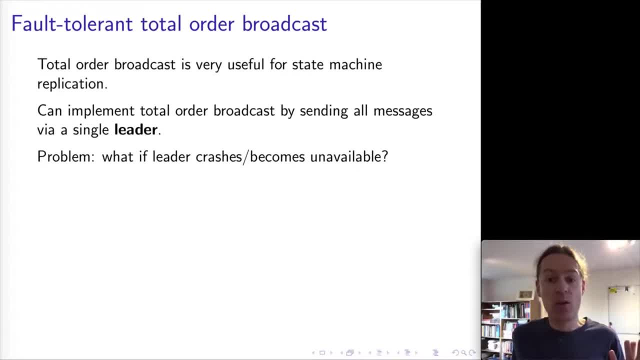 Now the question is now really: how can we deal with the problem of a leader becoming unavailable? One option is to manually switch over to a new leader, and this process is called failover. So manually means there's a human operator who gets notified. 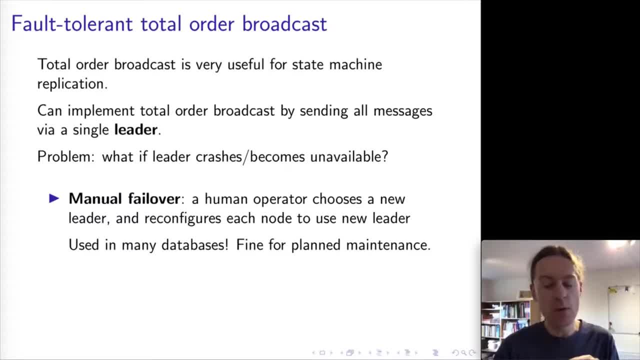 if the leader fails and this human is then going to choose a new node as the new leader and it's going to reconfigure the system. so change all of the followers to accepting this new node as their new leader, telling this new node that it now has to be the leader. 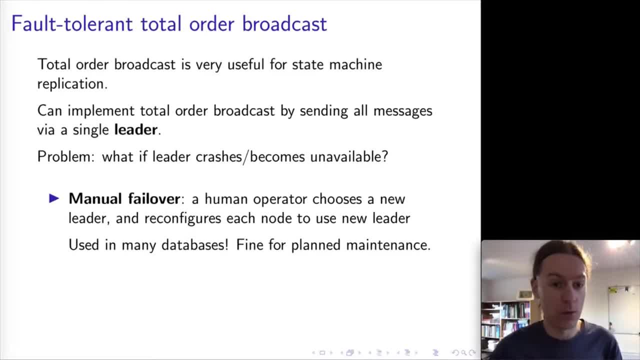 and act in this capacity to implement total order broadcast. And this works fine if you know in advance if the leader is going to go down, which could happen, for example, if the leader is going down due to planned maintenance. So if you know in advance. 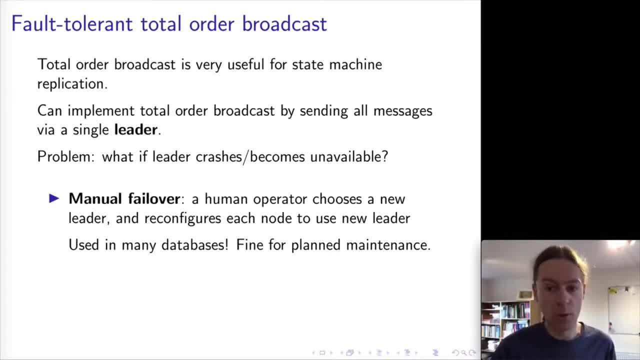 that you want to reboot the leader tonight in order to install some software updates, then you just move the leader role to a different node before you install the software updates and then you can take it down in peace and quiet and no problems at all, Unfortunately, 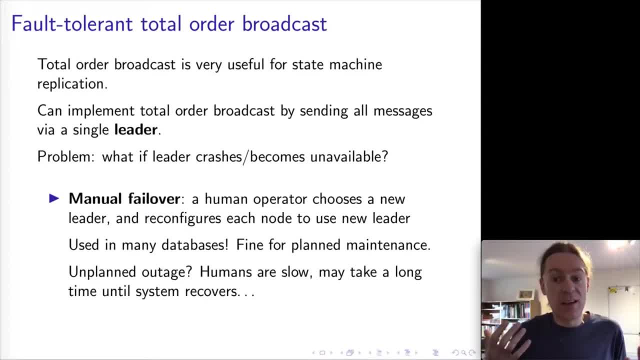 this doesn't really help you in the case where the leader crashes unexpectedly or if the leader suddenly develops a hardware fault and suddenly just stops working- And you know computers do that sometimes. They do sometimes just stop working. In that case it'll probably stop working. 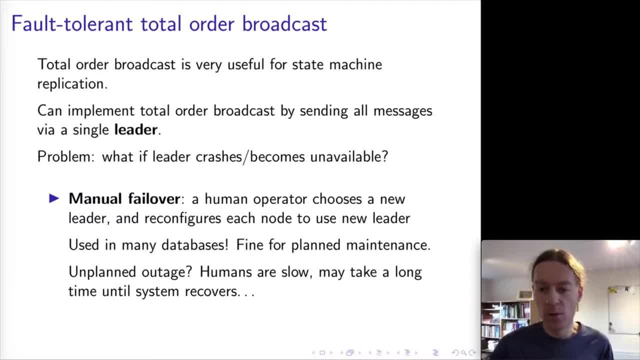 at the most inconvenient time, so like 3 in the morning, and so somebody then has to get phoned and they have to get out of bed and log into their computer and reconfigure the system to use a new leader, and so on. 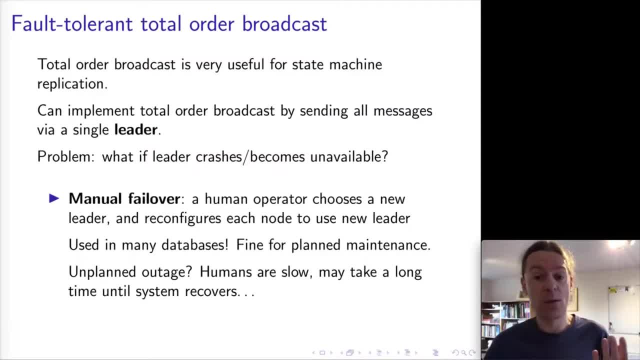 And so this is possible, and some database systems do implement replication in this way. but it does beg the question: can we somehow do this leader transition automatically, so that we don't have to wake people up at 3 o'clock in the morning? 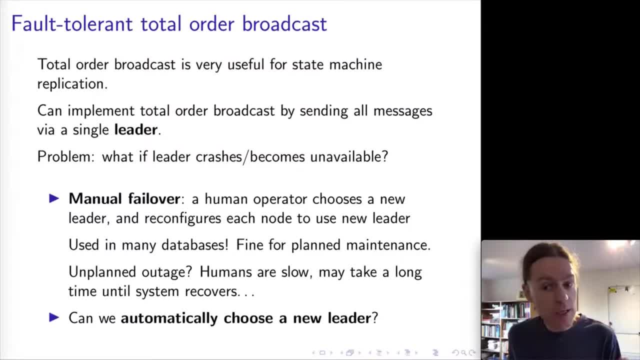 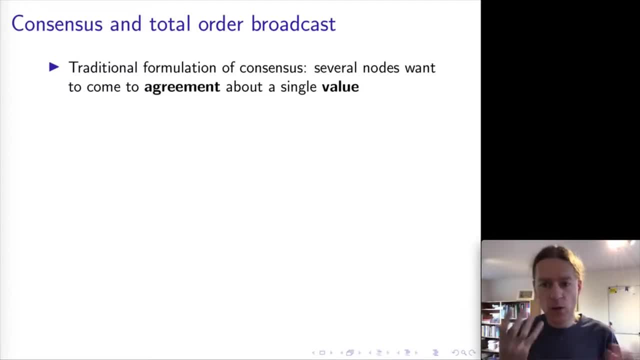 And this transition to a new leader is exactly what consensus algorithms are all about. So consensus and total order broadcast are two different problems, but they're actually quite closely related, as I'll explain now. So the traditional way in which consensus is formulated in distributed systems: 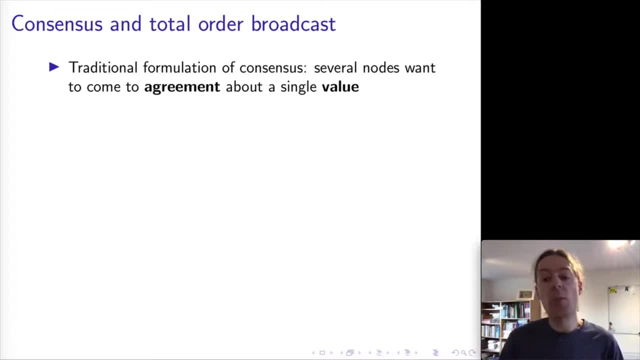 is that you've got multiple nodes. each node may propose a value and you want all of the nodes to decide on the same value. So think of it as like several friends deciding where to go for lunch today and like they propose different restaurants. 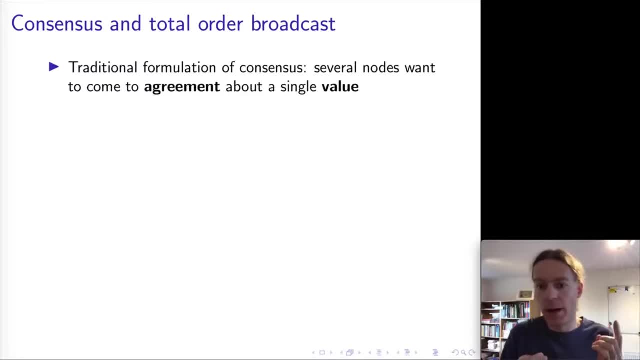 or shops to go to, and then, by some kind of process, one of those proposals is going to get picked, and then everybody is going to go to the same shop or restaurant for lunch. And so this is the consensus problem. we want the nodes to agree on. 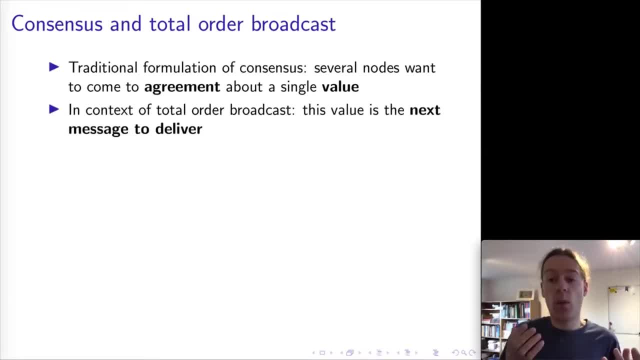 one of the values that was proposed. Now you can think of this as being equivalent to total order broadcast, because in total order broadcast, what happens is we want all of the nodes to deliver the same messages in the same order, and so this agreement. 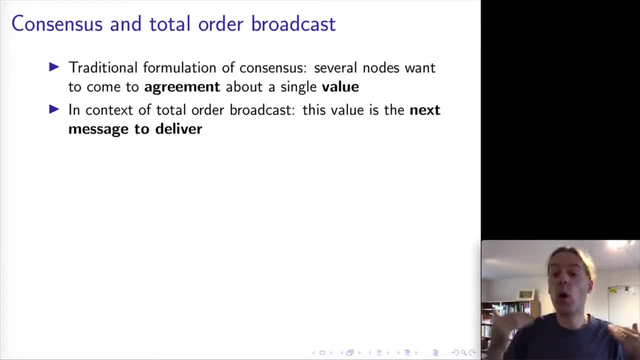 that the nodes need to come to is the agreement on what is the next message to deliver in this total order, And so you can keep doing consensus once for each message that needs to be delivered, and the consensus will guarantee that all of the nodes will make the 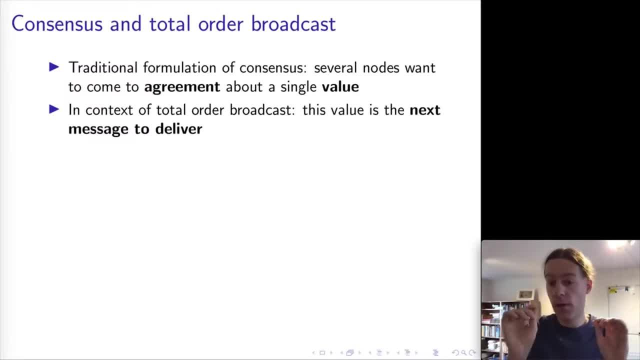 same decision. and so at some point a node decides that on a certain value, which means in total order, broadcast terms, it delivers that message, and consensus guarantees that once a value has been decided, it's not going to change its mind about it. and so 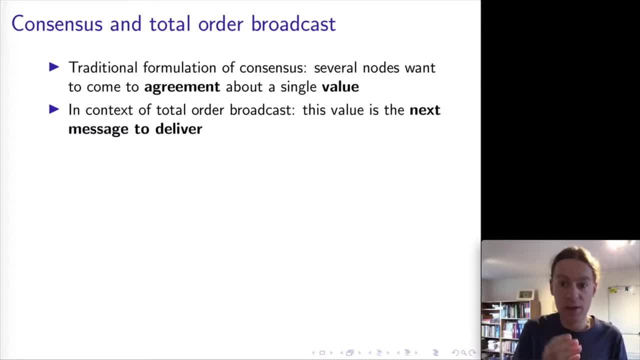 for total order broadcast. this means now, once a message has been delivered, it has been delivered at a certain point in this total order, And so, for this reason, the consensus problem and total order broadcast are actually formally equivalent to each other, which means that if you have 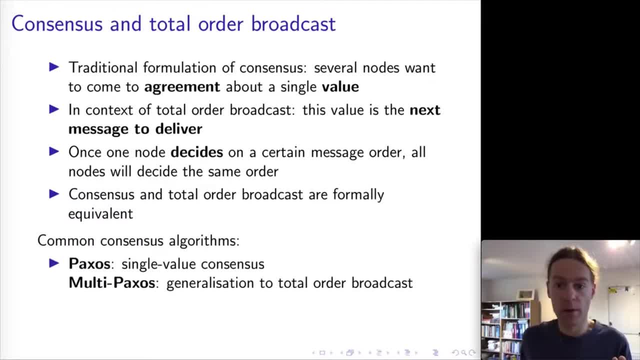 an algorithm for one, then you can convert it into an algorithm for the other, and vice versa. Now the classic consensus algorithm is called Paxos, and what Paxos does actually is only a consensus on a single value, but there's an extension to Paxos. 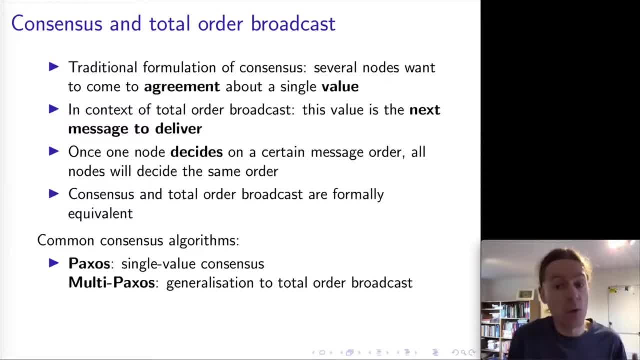 called Multipaxos, which actually provides total order broadcast. so that provides agreement on a sequence of values, ie a sequence of messages to be delivered. and there are a whole bunch of other consensus algorithms, including Raft, uStamp, for application. 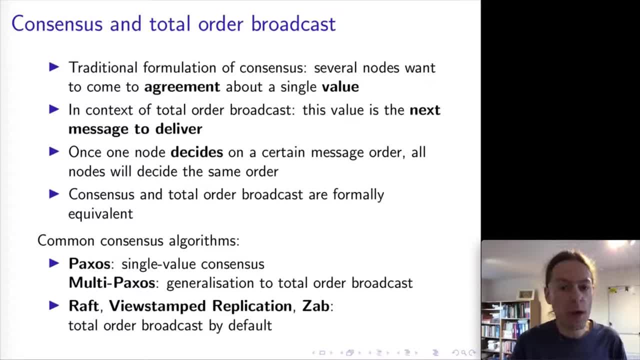 and ZooKeeper's ZooKeeper Atomic Broadcast, ZAB, and they are actually designed to provide total order broadcast right out of the box. So in this lecture we're going to look at Raft in a more detailed way, because that is perhaps the 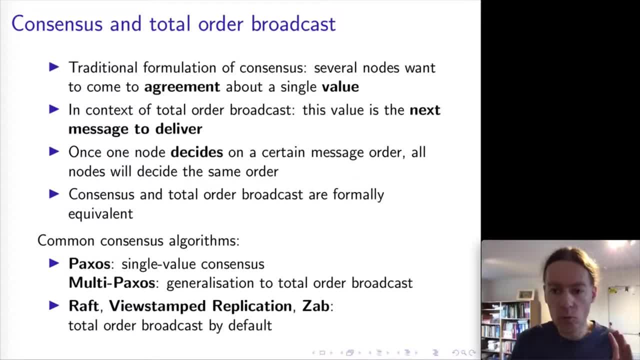 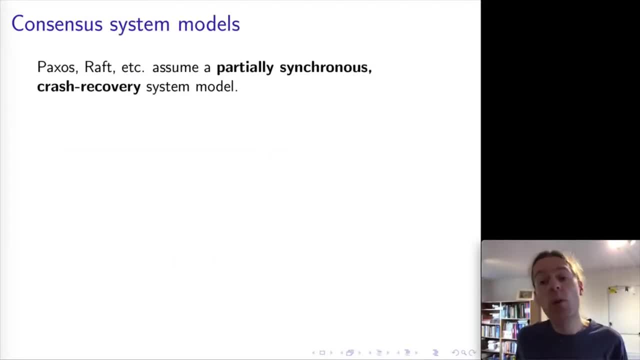 easiest to understand, although all of these algorithms are rather complicated and rather subtle. Now remember from lecture 2 we talked about different system models and this becomes very important now when we are talking about consensus. So remember that when we were talking about node behavior, for example, 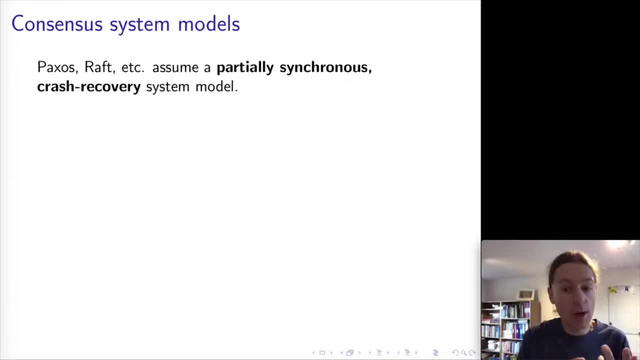 we could choose between. do we want crash stop or crash recovery, or Byzantine in which nodes can behave arbitrarily, maliciously in terms of network? do we want to assume fair loss, for example, and in terms of synchrony timing? 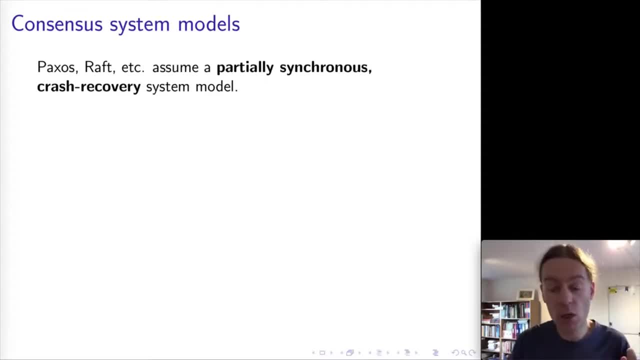 are we going to assume an asynchronous system or a partially synchronous system or a synchronous system? And what Paxos and Raft and all these popular consensus algorithms do, is they choose a partially synchronous crash recovery system model. And you might wonder why particularly these choices? 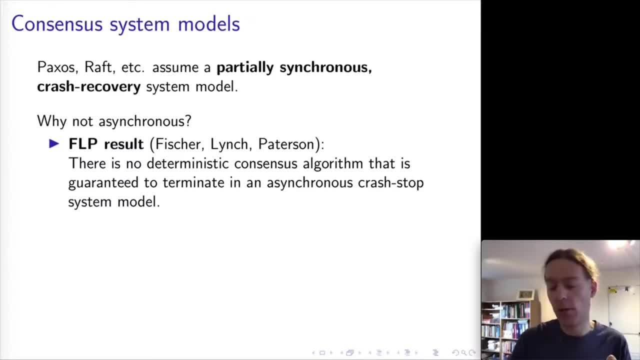 So, in particular, the question of synchrony is an important one, because we have said that a fully synchronous model is unrealistic, because in real systems you do get network delays and you do get various delays that happen at various points, and so we can't rely on any upper bound. 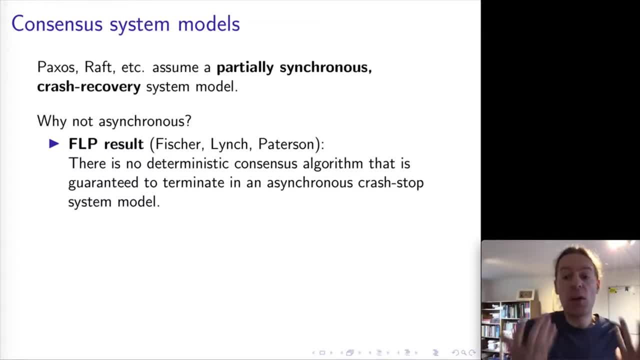 of message latency when sending over the network. So the best we can hope for really is partially synchronous, where most of the time the network is well behaved, but occasionally it has periods where messages are delayed for a long time or nodes pause their execution for a long time Now. 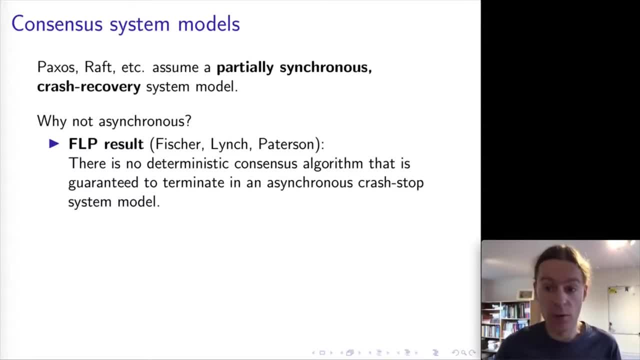 ideally we would want consensus to even work in an asynchronous system where we make no timing assumptions at all, But it turns out that this is actually impossible. So there is an impossibility proof, which is called the FLP result, which proves that it is not possible. 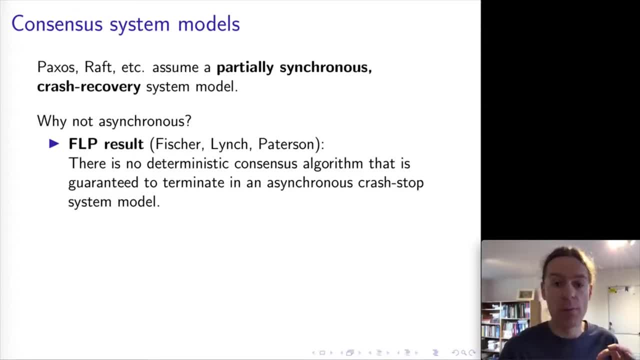 to implement a consensus algorithm in an asynchronous system in such a way that this algorithm will always terminate. So if you have an asynchronous system and even if you only allow crash stop failures, so even not any of the more complex failures, then there will always be some executions. 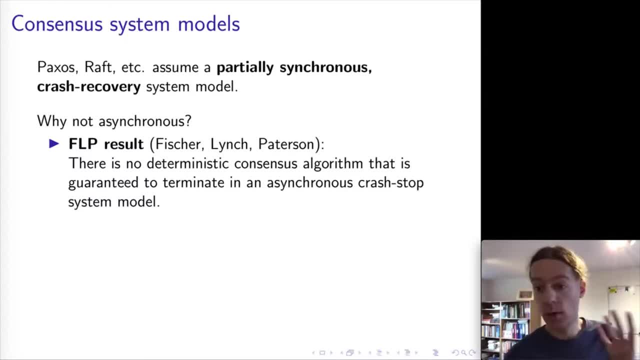 of the consensus algorithm, in which the algorithm doesn't terminate. And so if you want termination, that is, if you want the algorithm to make progress and eventually decide on something, or for total order broadcast to eventually deliver a message, then we have to make these timing assumptions. 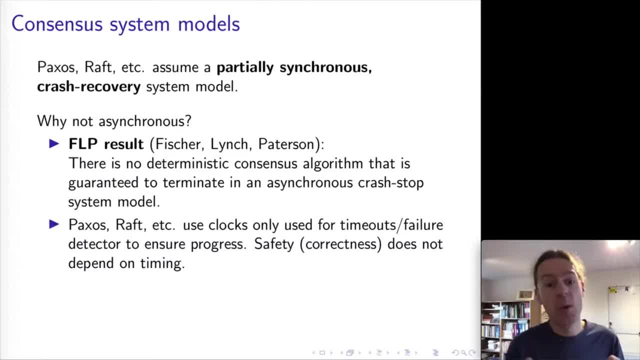 So we have to assume at least partial synchrony, which means, in effect, that we use clocks for timeouts, or in other words, we have a timeout based failure detector which we use in order to figure out if the leader has failed or not. Now, importantly, the correctness of the algorithm. 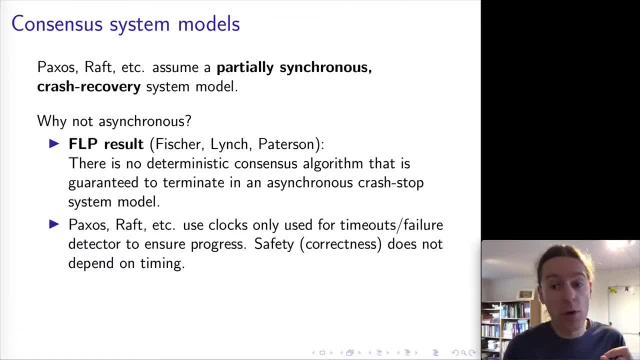 doesn't really depend on the timing at all. So even if the timing in the system goes really bizarre, consensus algorithm will still guarantee that the same sequence of messages is delivered in the same order. The only thing that timing affects is when that delivery happens, And so if 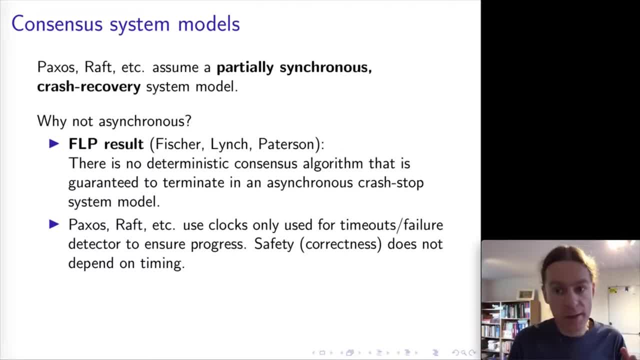 you have a system in which there are lots of weird delays happening, then it could be that the timing that the delivery of the messages is delayed for some amount of time until the system sorts itself out. So the timing does affect the liveness of the system here. 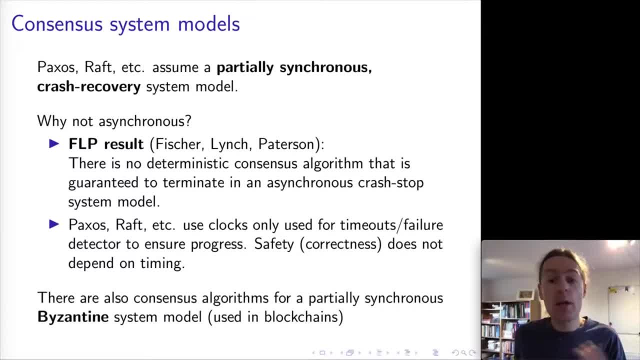 but not the safety. Now it is also possible to weaken the assumption about the crash recovery system model, And so it is actually possible to go all the way down to a Byzantine system model, where we assume that some of the nodes may behave maliciously And it is possible to do consensus. 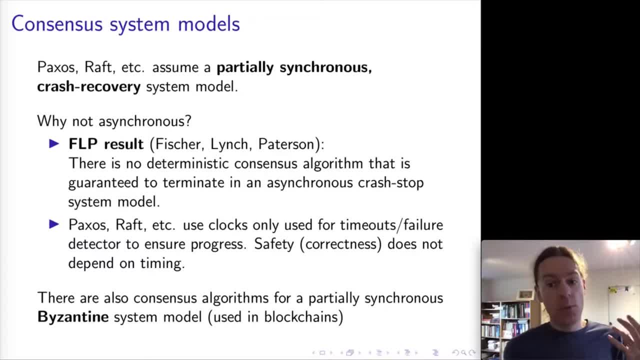 in that kind of system And these types of Byzantine fault tolerance consensus algorithms are used in the context of some cryptocurrencies and blockchains and that sort of area. However, these Byzantine fault tolerance algorithms are rather more complex than the crash recovery algorithms and 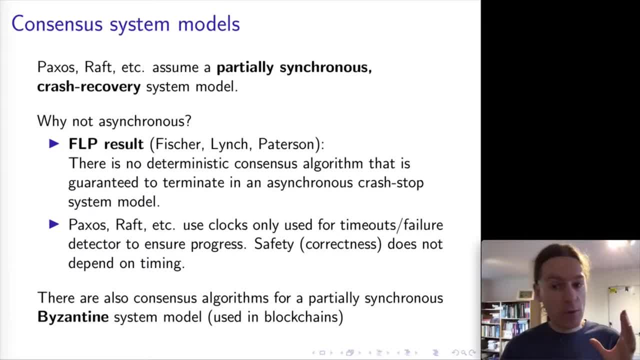 they are also a lot less efficient, And so, for the purpose of this course, we are just going to concentrate on Raft, which is a non-Byzantine algorithm, So it just assumes a crash recovery model, and we will leave the Byzantine algorithms out of scope. 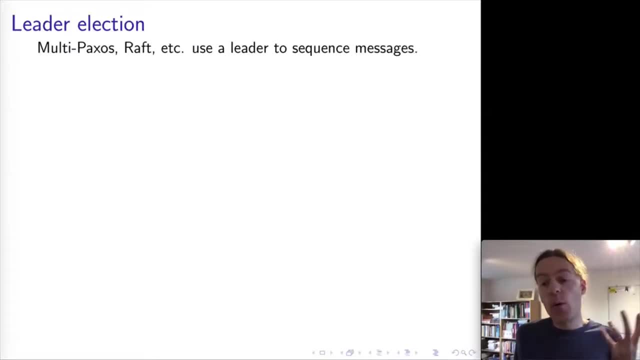 for now. So, as we said, the key thing that we need of consensus is to elect a leader and then, once we have got a leader, that leader can decide on the order in which the messages should be delivered, And all of the consensus algorithms I just mentioned do actually. 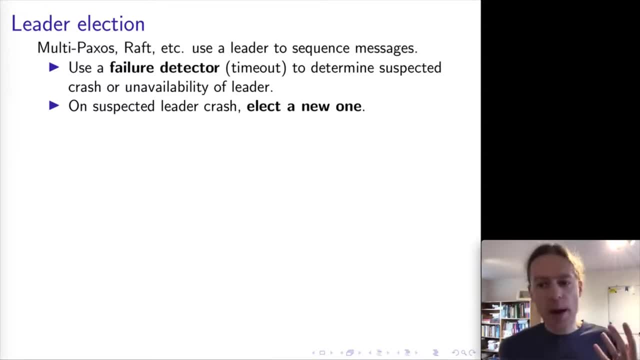 use a leader in order to sequence the messages, The details of how exactly they use the leader and how they elect a leader. they differ from algorithm to algorithm, so I will be focusing on what Rafts does in particular, And so what we have is we use a timeout. 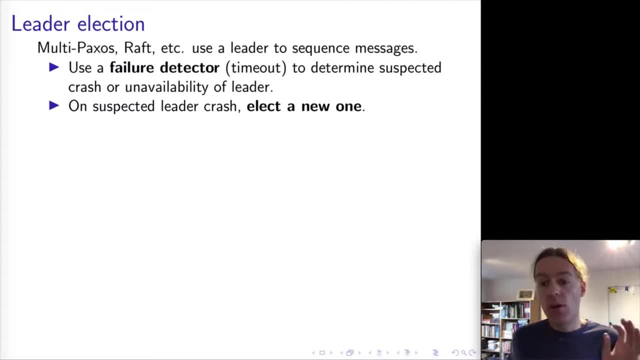 we use local clocks in order to suspect whether a leader has failed or not. So, if you remember, the failure detectors that we can have in a partially synchronous system are not always accurate, So it could be that we think that a leader has crashed when in fact the leader is working just fine. 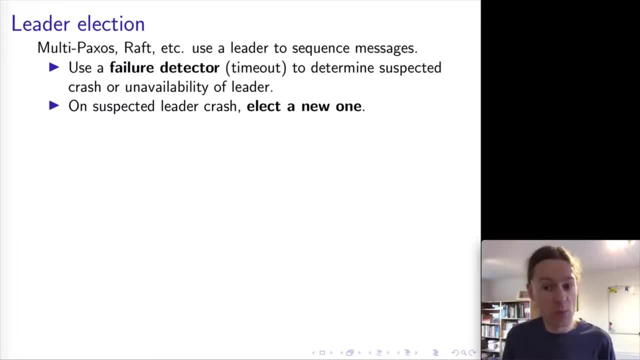 but there is just a network problem which is stopping us from communicating with the leader. So that's why I say we can only have a suspected leader crash. We can never be actually certain, if the timeout happened, that it was in fact a leader failure. 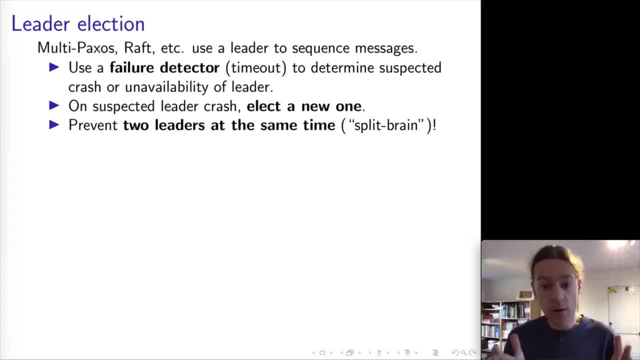 And what we want is that the consensus algorithm should prevent having two leaders at the same time, Because if we have two leaders, they might make contradictory decisions and then all of our algorithm's guarantees are off. And this situation where you have two different leaders- they both believe that they are the leader. 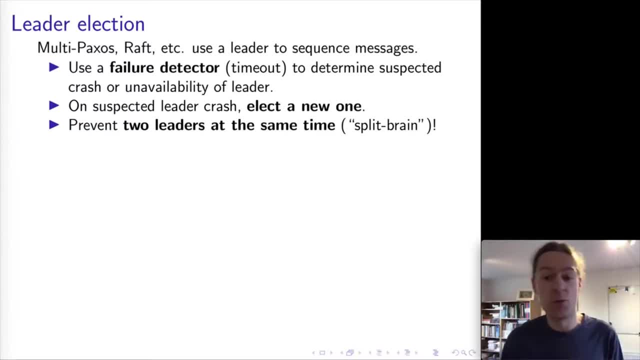 this is called split brain, and if this happens in a distributed system, it's usually really bad news, Because it's probably going to mean that some data is going to get corrupted or you're going to lose some data, And so we want to avoid split brain and the consensus. 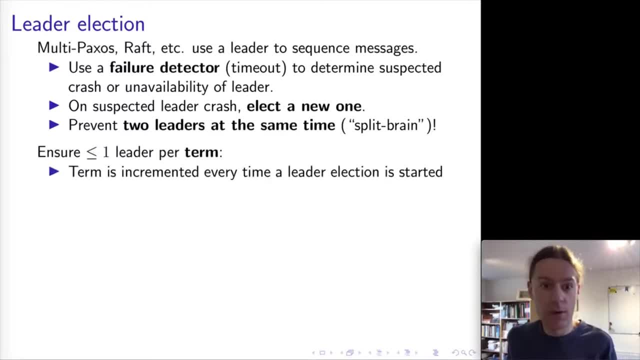 algorithm has to be designed in a very careful way so that it doesn't suffer from split brain, And the way this works in Raft is that we have a concept of a term. So a term is just an integer variable and every time that there's a leader election, that leader election. 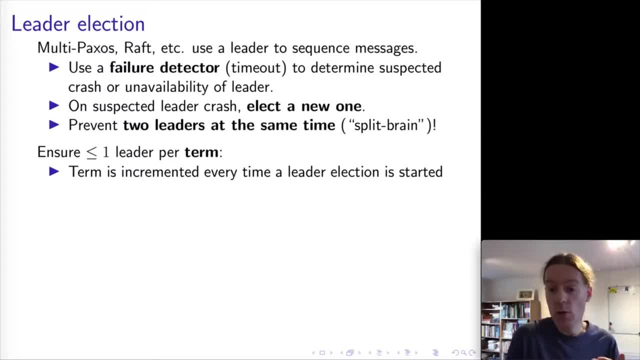 takes place in a certain term. So every time we start a new leader election we just increment the term, And the guarantee that the leader election provides in Raft is that there will be at most one leader elected in a given term. It could be that a leader election fails. 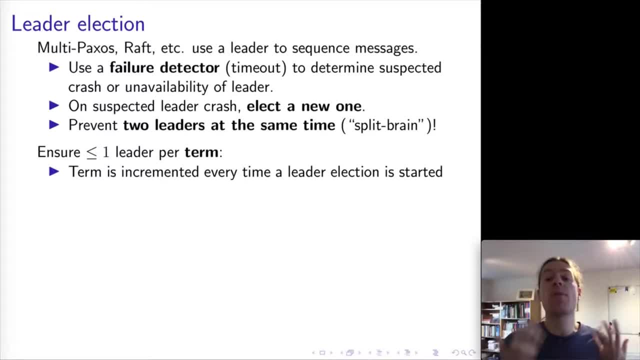 and that no leader is elected in a term, but there will never be more than one leader in a given term, And the way this is ensured in Raft is that we have a rule that in each term, a node is only allowed to vote once. 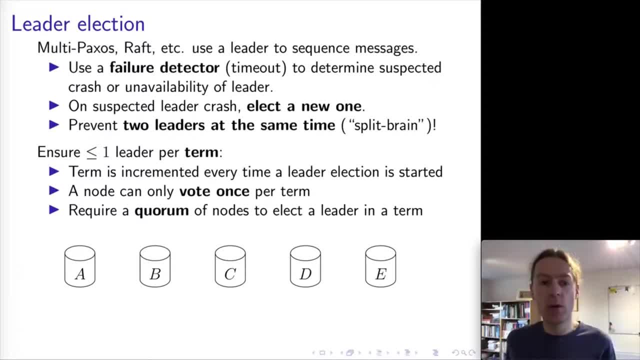 So, just like in a parliamentary election, you're only allowed to cast one vote. very similar here. Say, if we have five, a system of five nodes, and say three out of the five elect a new leader. A, B, C have voted in favor of the new. 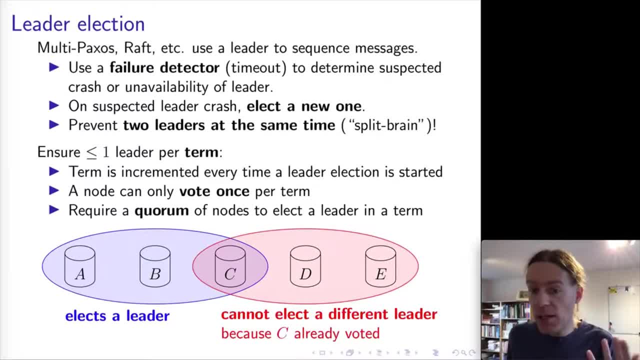 leader Now. later, if C, D and E try to elect a different leader in the same term, they will not be able to because C knows that C has already voted once in this particular term And therefore it will not vote again for a different candidate in the. 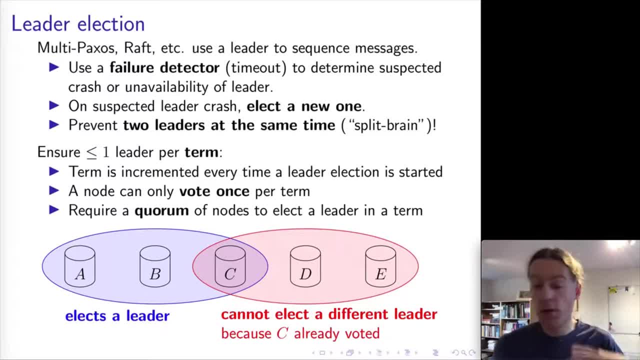 same term In a new term, new start, new leader, election. so in that case, every node can vote again, And so what we typically require in a consensus algorithm is that every time we want to elect a leader, we need a quorum. 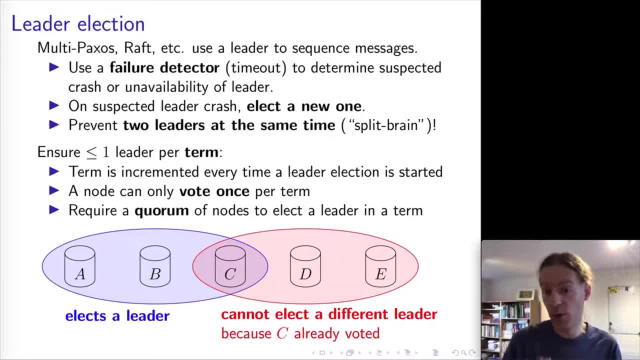 of nodes to vote in favor of that leader in that particular term. And so in this case here, if we have three, if we have five nodes, for example, then we could have a majority quorum of three out of five. So any three out of five nodes are able to elect a new. 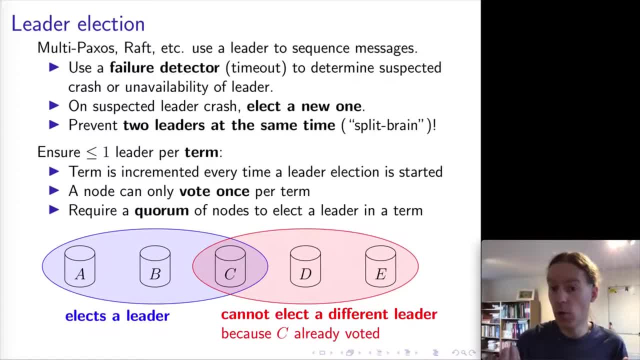 leader, which means that the system can tolerate two nodes being unavailable and the remaining three nodes out of five can still make progress and still elect a new leader if necessary. So this is what gives us the full tolerance, And so this approach here of allowing a vote only once. 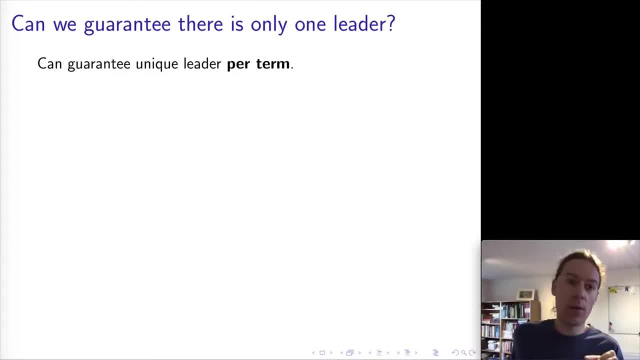 per term ensures that within a given term, there is a unique leader. However, this does not actually guarantee that we will not have multiple leaders, Because what could happen is that there are different nodes that are leaders in different terms and they just don't realize it. So 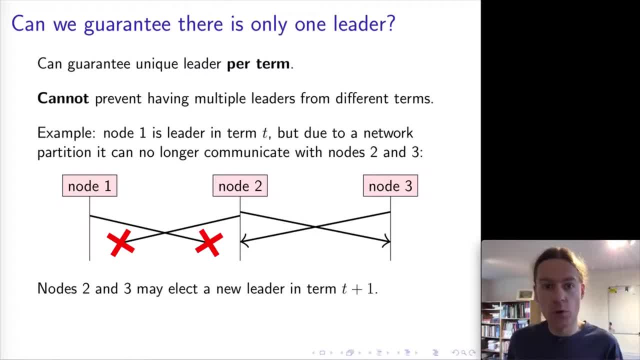 imagine this scenario here: We've got three nodes- one, two and three- and say that node one was elected to be the leader in term T, But then a network problem happens and node one is no longer able to communicate with nodes two and three. Node one is still. 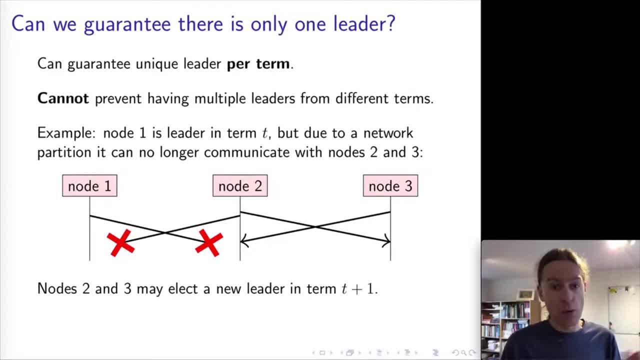 alive. Node one is still a leader, But now node two and three don't hear anything from their leader anymore, And so at some point node two and three are going to say, well, probably our leader is dead, So we're going to elect. 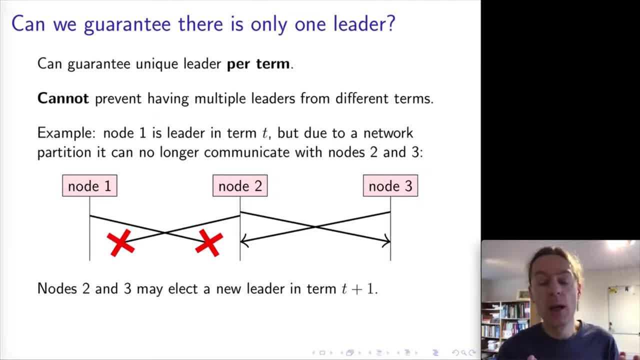 a new leader in a new term, So call it term T plus one. Node two and three are going to elect a new leader among themselves. Maybe node two is going to be the new leader, for example. And now the system has actually got two leaders. It's got node one. 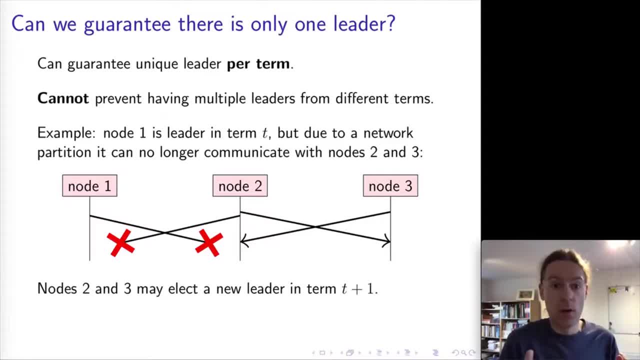 which is the leader in term T, and node two, which is the leader in term T, plus one, And this looks like split brain, doesn't it? So we've got two leaders. This is bad. We want to not be in the situation, But unfortunately because 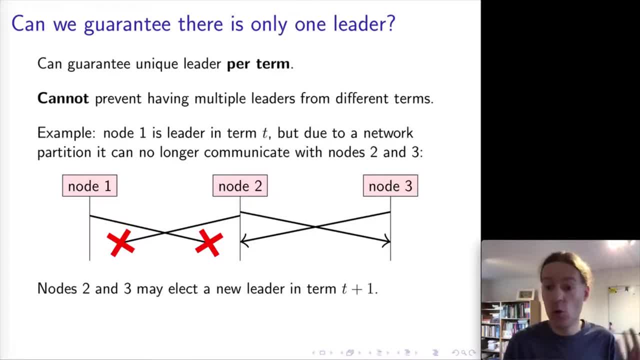 the network is interrupted, there is no way for node one to know that it is no longer the leader that has been superseded, because the communication simply isn't getting through, And so, therefore, we need to actually deal with this possibility that there are different leaders existing in the 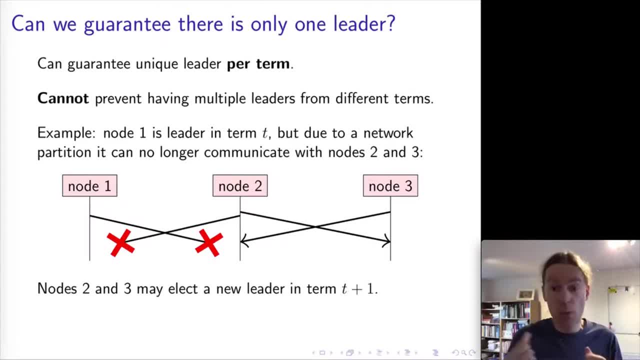 system at the same time, in different terms, and those leaders may, for a little while, make contradictory decisions, and we have to nevertheless ensure that we have total order broadcasts, that we don't violate our properties, even though we might have multiple leaders And the way that 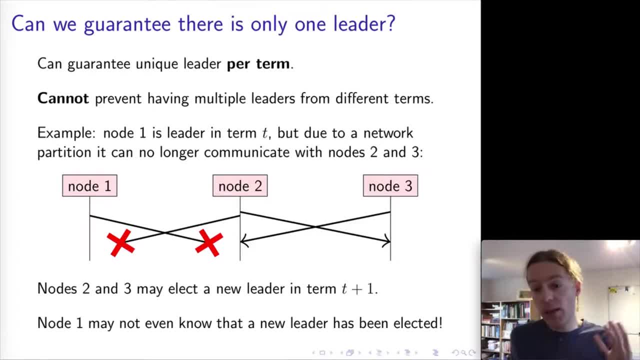 consensus algorithms do this is that if a leader wants to decide to deliver a certain message, for example, the leader cannot actually make that decision by itself, but the leader has to again go and ask a quorum of nodes if they are okay to deliver a certain message. 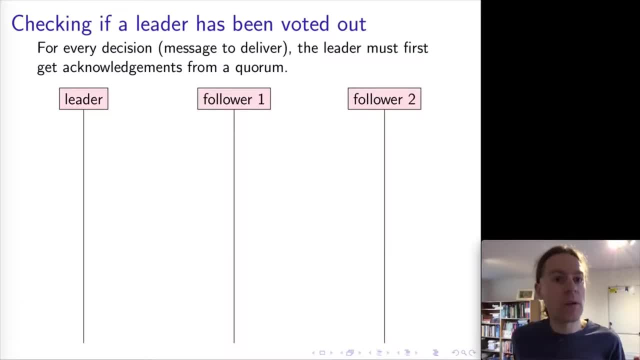 And so what the communication flow looks like is something like this: now, Say: we have leader on the left and two followers, and so, first of all, the leader needs to, the node on the left needs to be elected, the leader, and so it's going to contact the other. say: 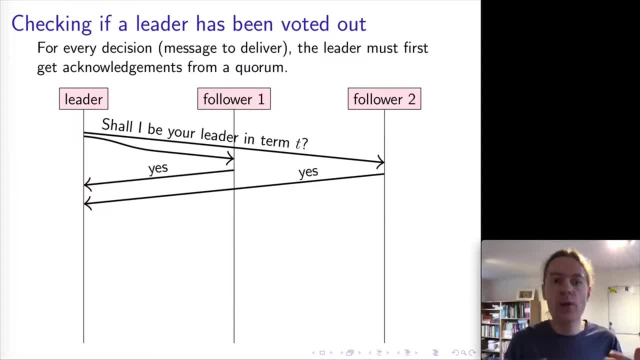 are you okay for me to be your new leader? and then the others respond: okay, Now it's got a quorum of votes in favor of being a leader. so now the node on the left is the leader. after one round of election, Now the leader wants to deliver. 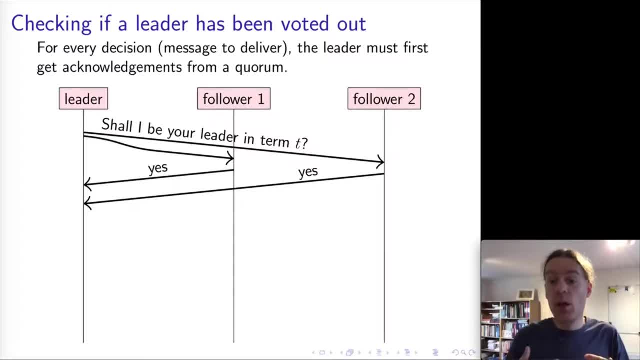 a message. but, as I said, the leader cannot just make that decision by itself to simply deliver a message, but instead the leader has to go to the followers again and say: are you okay to deliver message m in term t as the next message and only if a quorum of followers again. 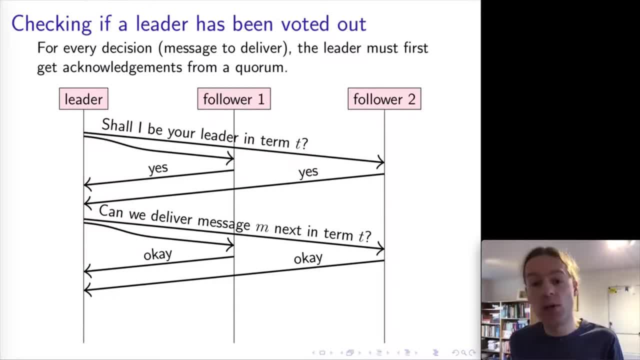 respond here and say: okay, yes, we're okay with this message m in term t and the followers will only respond positively if they haven't heard of any other leader in term t plus one. So now, if the leader again gets this quorum of positive responses now 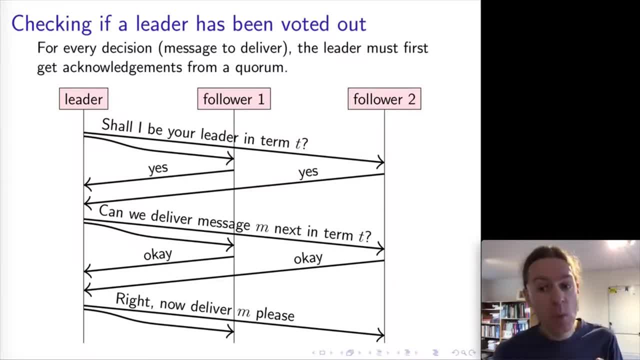 the leader can safely make the decision to deliver m and it can tell the other nodes that, okay, m is now the next message to be delivered in our total order broadcast. So this is the principle: that we have effectively two phases of voting. First of all, 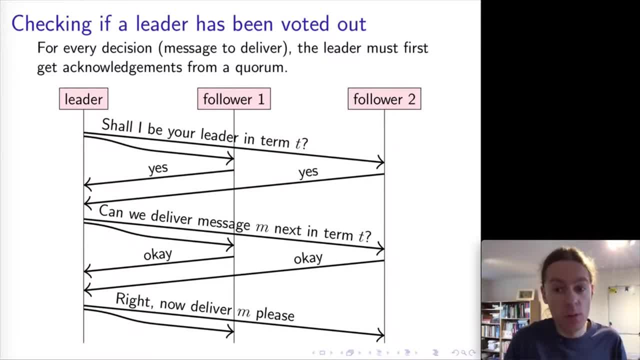 a node needs to get elected leader by a quorum of nodes, and then a second round happens in which the leader checks if it's okay to decide on a certain message. next, and this is actually the underlying principle of all of the consensus algorithms that we've seen, 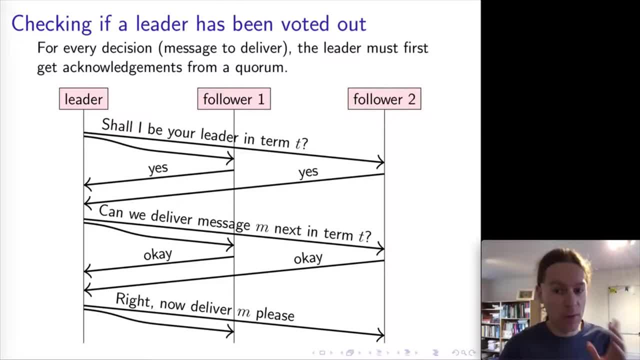 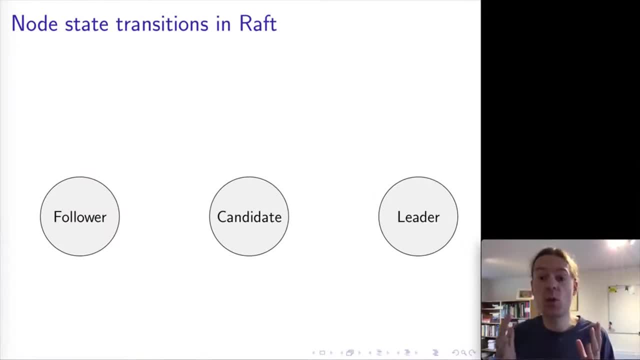 and in the next section we will look in detail at how Raft implements this particular system. Now, in this section, I'm going to walk you through the entire Raft algorithm. Just to warn you, this is a rather complex and subtle algorithm. it's by far the most complex algorithm. 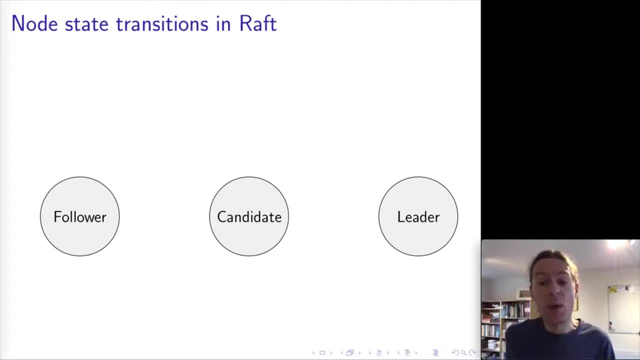 that we're going to look at in this course, and I'm not expecting you to memorize every single line of it- it's far too much for that- but I would like you to understand the principles of how it works, because, although it's subtle, it's very instructive as a way of 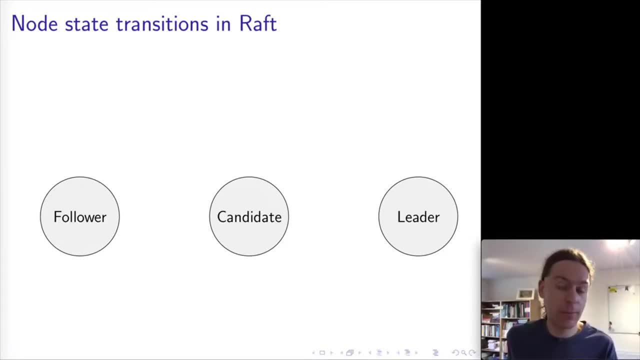 how to think exactly about behavior in a distributed system. So the foundational part of Raft is a kind of state machine where a node can either be a leader or a candidate or a follower, and so I'm going to first explain this state machine before we go into the code. 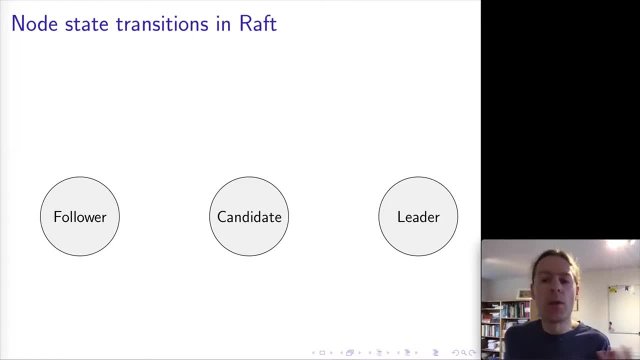 because this is useful just to keep in mind for what is actually happening, and then we'll go into the details. So initially, when a node starts up, it is in the follower state, and so this could be either when it starts up for the first time, or if a node crashes and restarts. 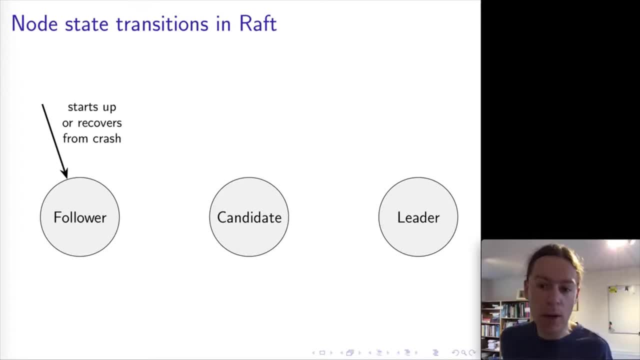 after it recovers, it also goes into the follower state, no matter what state it was in before. Now, eventually, the system needs to have a leader, and so, in order for a node to become a leader, it has to first become a candidate, and a node becomes. 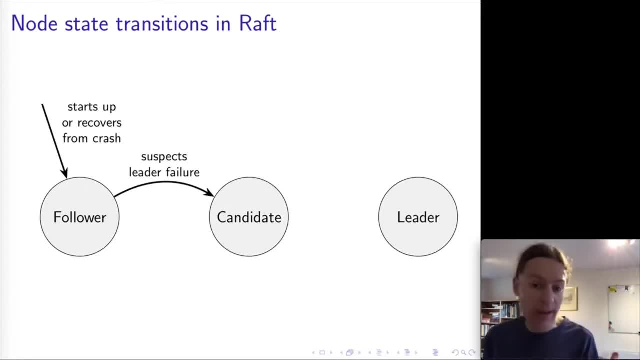 a candidate if its failure detector tells it that there is a suspected leader failure. so, essentially, if it hasn't heard from the leader for some period of time, there's a timeout at which point one of the followers will say: okay, I just assume the leader is dead. I'm going to become the candidate now. 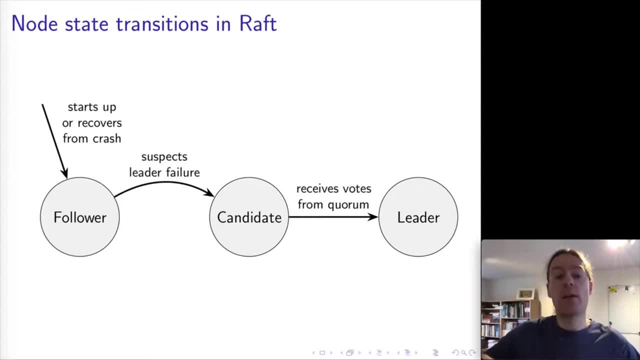 and so then, when the node becomes a candidate, it asks for votes from the other nodes, and if it successfully obtains a quorum of votes from other nodes, then this candidate can become a leader. however, it could also happen that, while this leader election is happening, the follower hears about some. 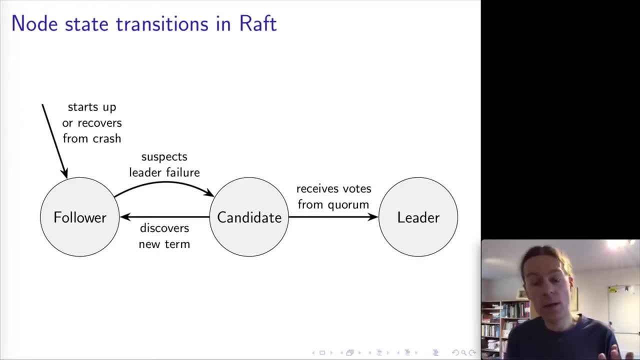 other candidate with a higher term number. and if it does discover one of these nodes, a different node with a higher term, then the candidate will just step back immediately and say: okay, fine, I'm going to leave the higher term to somebody else and become a follower again. 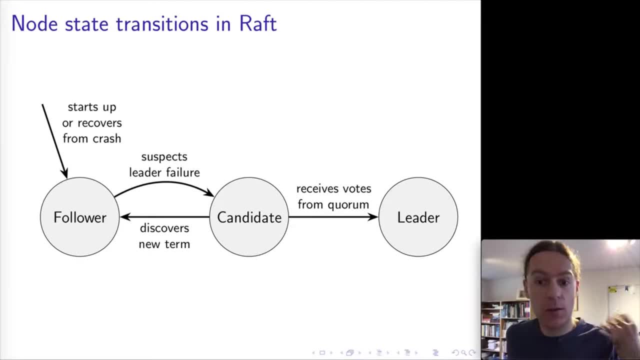 but what could also happen is that the candidate starts an election and it doesn't receive enough votes within some period of time, but it doesn't discover any new term either, in which case, eventually, the election will time out and it will restart a new election with the same node being the candidate. restart a new election with a higher term number and hopefully the next time around then it will be able to get votes from a quorum of nodes. so now, once a node is leader, it remains leader for potentially a very long time, until either that node crashes or gets. 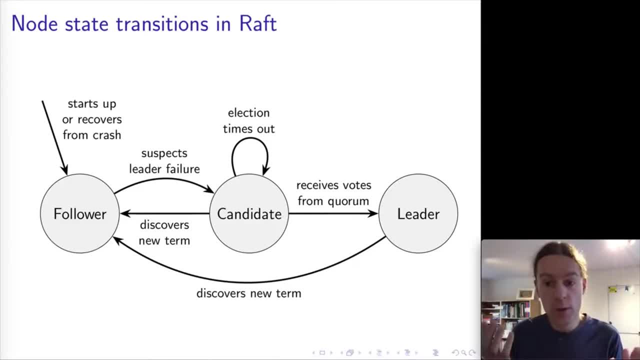 shut down for whatever reason, or if the node discovers a new term. so if the node has been happily leader-ing but then some other nodes on the side have decided that the leader is dead. they've run an election. they've elected a new leader with a higher 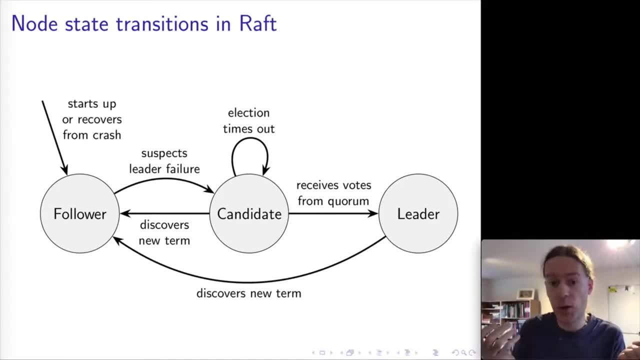 term and then eventually the old leader finds out about this higher term. at the point where it finds out about the higher term, then immediately the leader just steps down to be follower. so we have a very peaceful transition of power in Raft, in the Raft algorithm. 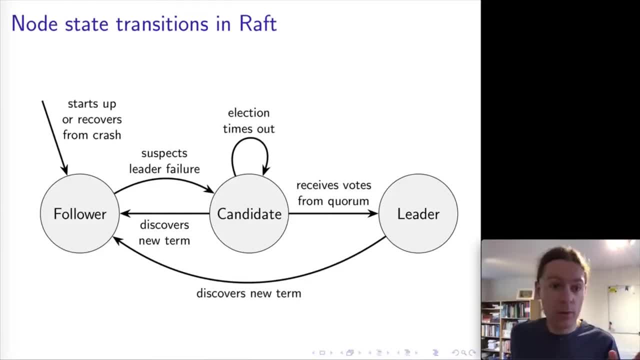 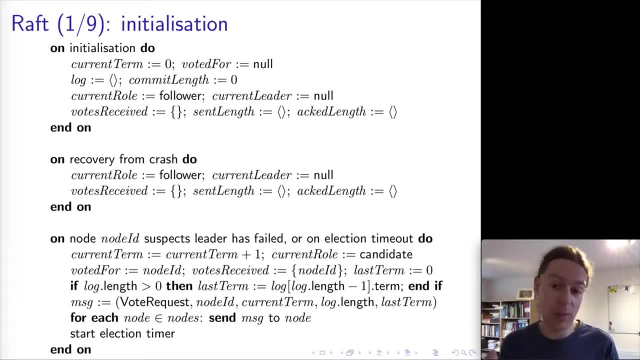 so that's the entire state machine for the follower, candidate and leader states. let's start digging into the code. so the code is spread over nine slides because there's rather a lot of it. but don't worry, I'm going to walk you through step by step and hopefully it will make sense. 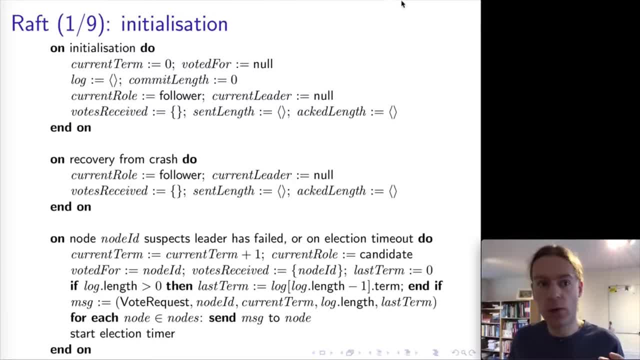 so first of all we have the initialization block, and so here we set the initial values for a whole bunch of variables. I'm not going to explain those variables now. I will explain them as we actually start using them in the course of the algorithm. the important: 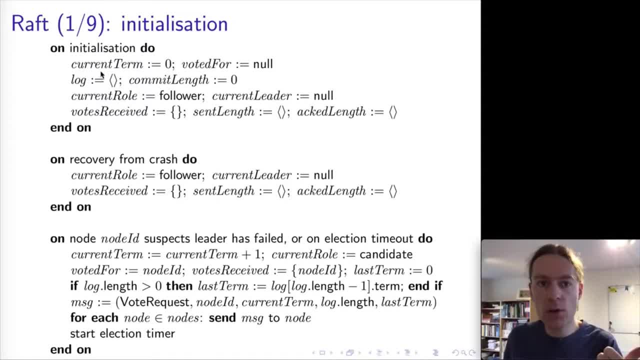 thing is just that the first four variables here, that is current term, voted for log and commit length. the first four variables have to be stored in stable storage, so they have to be on disk and whenever a node updates one of these variables, it has to write that update. 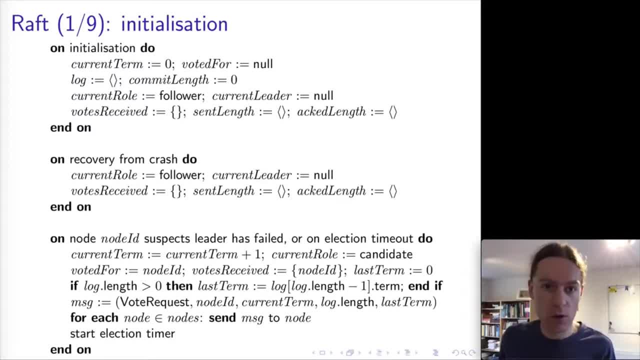 to disk before it does anything else, before replying to any messages or so. this is important for the crash recovery purposes of the algorithm. on the other hand, the later variables here, so the ones that are not the first four, they can be just in RAM, they can be in. 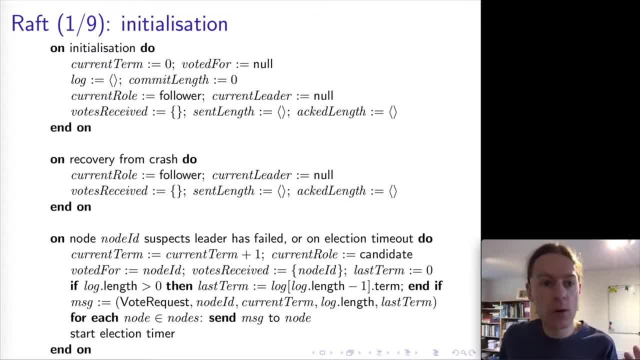 volatile memory and so their contents will be lost if a node crashes. and then, indeed, if a node crashes, then we have this block here which resets them to their initial state. so you can see, for example, that after a crash and we recover, we go back into the follower state. 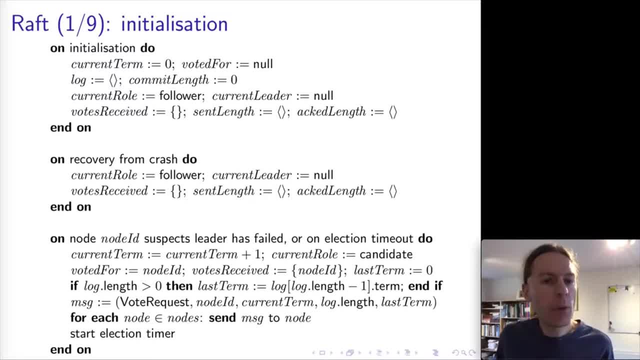 and so on. now, the most interesting of these variables is probably the log, and so actually first the current term. so the current term, as I said earlier, is just an integer which gets incremented every time a lead election happens. voted for is to ensure that a vote only votes once. 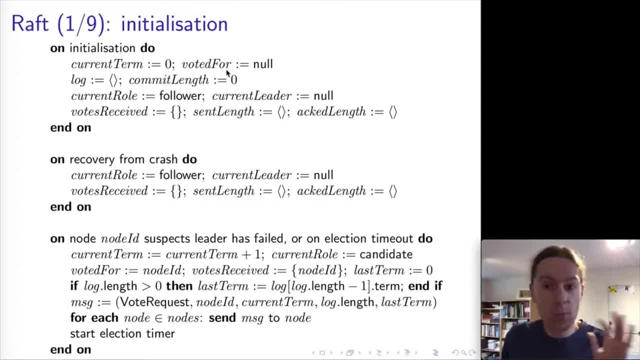 per term, so to ensure that within a particular term a node can only vote once. then the log is what is interesting. so the log is an array, it's a sequence of values, of sequence of entries. every entry in the log consists of two things. it consists of a: 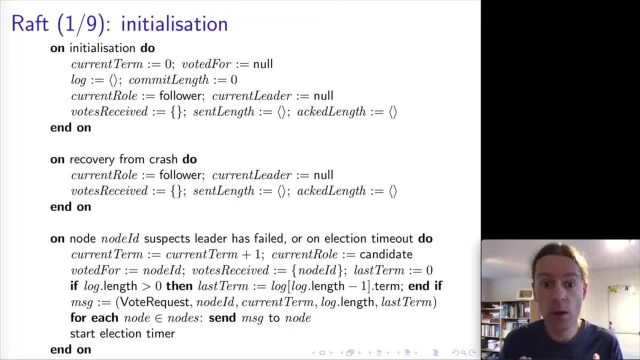 message that we want to deliver by a total order broadcast. so that's our value that we are deciding on. and the entry also contains the term which was the term of the leader at the time that we broadcast this particular message. so those are the two pieces of information that 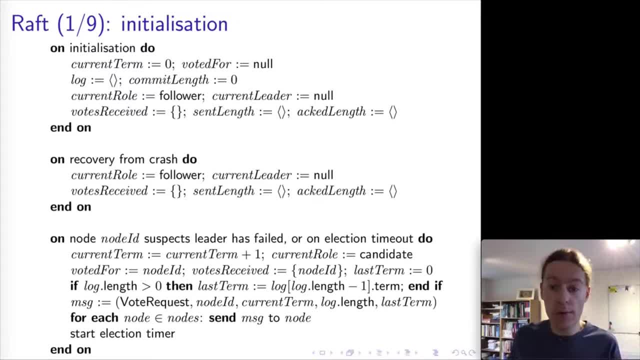 we have for each entry in the log, and so the log is now just going to be. think of it as an array that starts with log and it has a certain length, and the order of entries in this array is going to be the order in which messages. 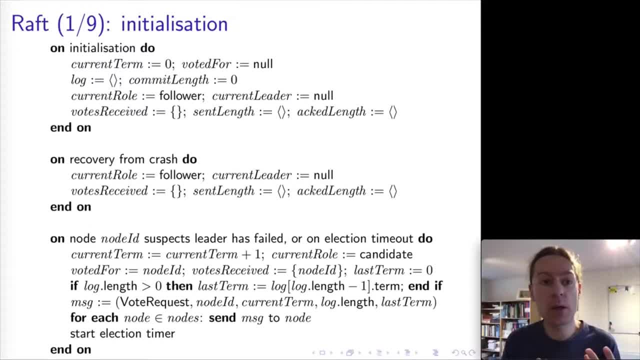 get delivered by total order broadcast. so what we want to ensure is that all nodes have a copy of the same log. now, there can always be a little bit of uncertainty around the last few, the most recent few log entries, and so what we have is this concept of a commit. 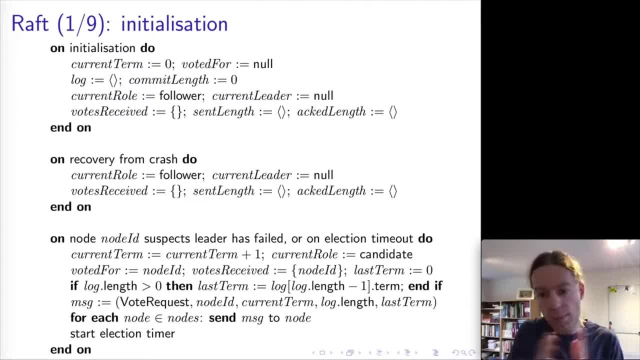 and so a certain prefix of the log. so the log from the start up to a certain point will be committed and that means once that section of the log has been committed, those entries in the log are not going to change anymore. so after a log entry has been committed, we know. 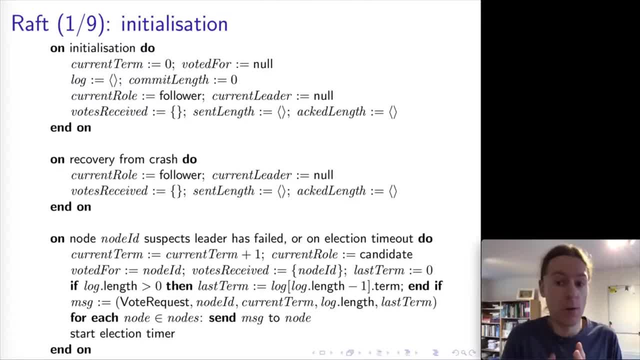 that everything up to that point is safe to be delivered via total order broadcast. but any entries in the log after the commit point, they are still a bit uncertain and so we can't deliver those quite yet. okay, so that's the principle of the log and the commit length tells us. 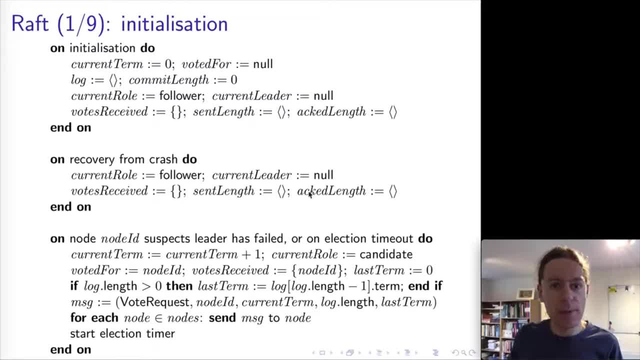 how far we have committed along this log. but we'll get to the commit length later, so let's start with the first leader election. so if a node with id nodeid suspects that the leader has failed, or if that node was previously a candidate and it started, 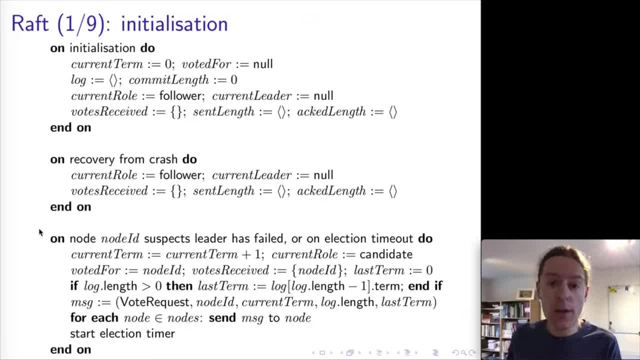 an election, but it didn't get enough votes within the election timeout, then the node executes this vote here. so, first of all, the node increments its current term. as I said, the node transitions into the candidate state and the node votes for itself. you know, like in any good election, of course everybody votes. 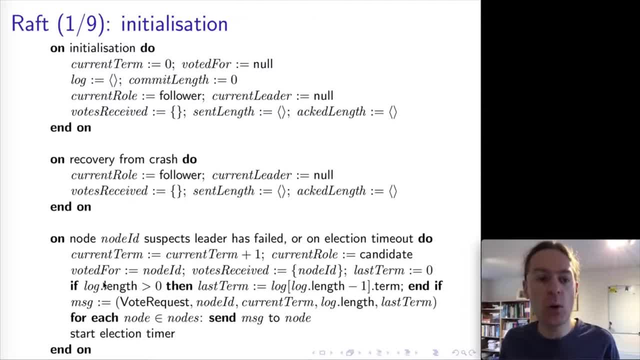 for themselves. so here the node is going to set its own voted for variable to itself and for the set of votes that it's received, it's immediately going to put itself into that set. it's going to set last term here, initially zero, but if our log is non-empty, then this: 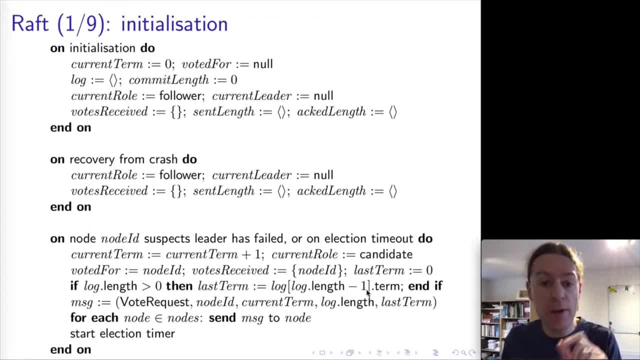 last term variable will be the term of the last entry in the log. so the log here is zero based index. so log dot length minus one is the index of the last element in the log, just like with an array in most programming languages, and the dot term property. that's: 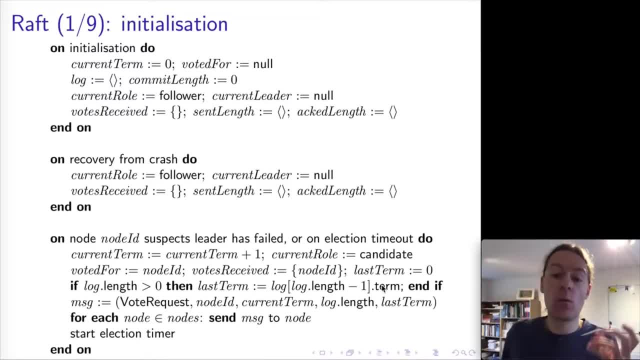 the term in which that last log entry was added to the log, and so this variable here, last term, and all of the other things get packed into a message and that message is sent to all of the other node, and so this message is called a vote request message. so 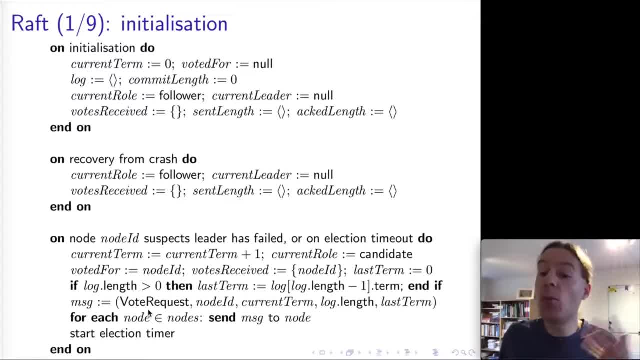 this is the leader asking the other nodes to please vote for it. sorry, this is the candidate- the candidate asking whether the other nodes will vote for it to become the new leader and so included in this vote. request message is the id of the candidate, which is node id. it's the current. 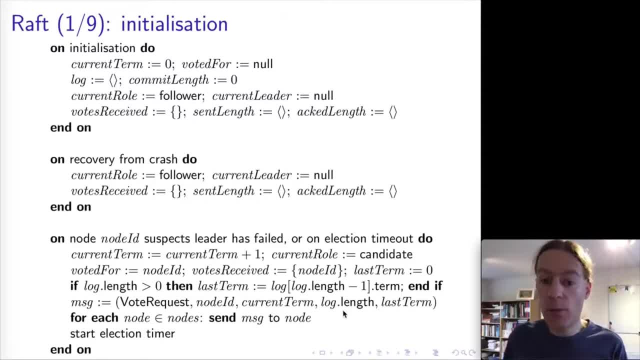 term of the candidate, which we just incremented, the length of the log to the candidate has and the term of the last entry in the log, and so this will get sent to all of the other nodes and then the candidate starts a timer, which is just so that. 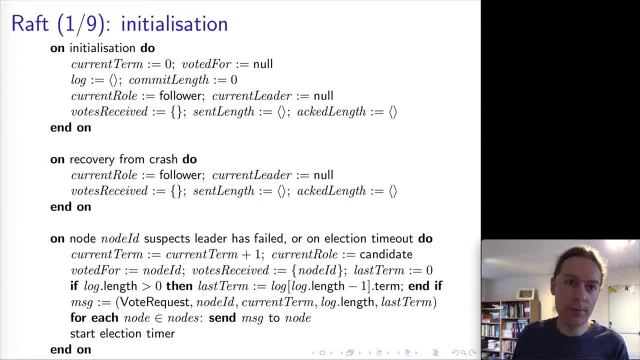 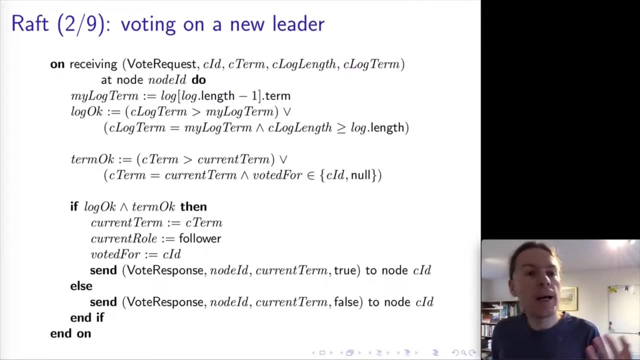 eventually, if it doesn't receive enough votes, then it can restart the election. okay, so that's starting the election. here at the top is a little diagram of what the log looks like. so we've got. each log entry has a message and a term property. um, so next is what happens. 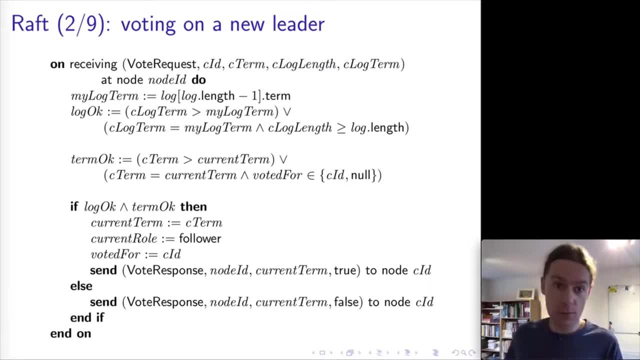 to a node that receives one of these vote requests messages. okay, so we're now on some different node. it receives a vote request with a certain candidate id, candidate term, candidate log length and candidate log term, the term of the last log entry and node id is now the recipient. 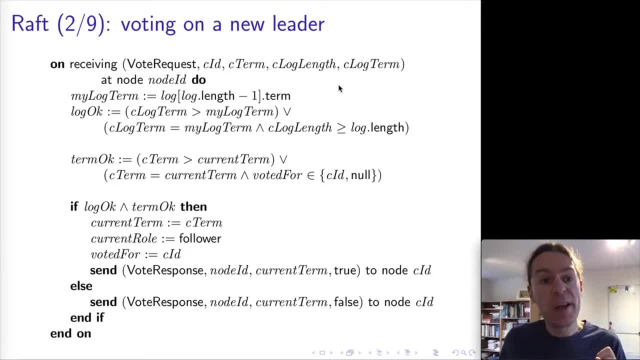 of this message. so now, first of all, the recipient is going to check if its local log is consistent with what the candidate says, and so what we're going to look at is the recipient of this message is going to look at its own log and look at the last entry in that. 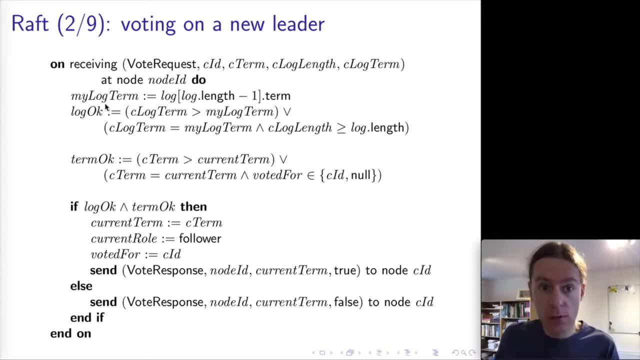 log and look at the term of the last entry. that's going to be my log term now. if the candidate has a last log entry with a higher term than our own term, then the log is okay. alternatively, if the candidate has the same term on the last log entry. 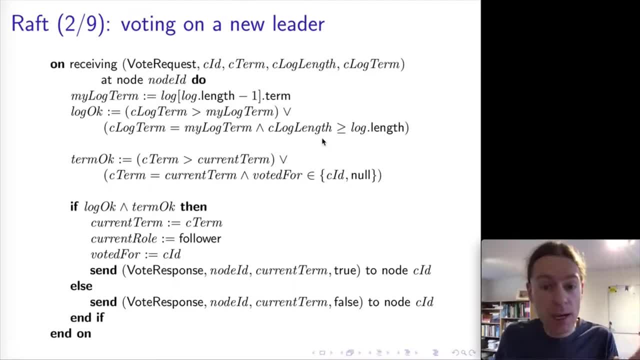 but the candidate's log length. the length of the candidate's log is at least as long as our own log, then the log is also okay. however, if the candidate has a shorter log, for example, or the candidate's log term is lower, in that case we will not accept. 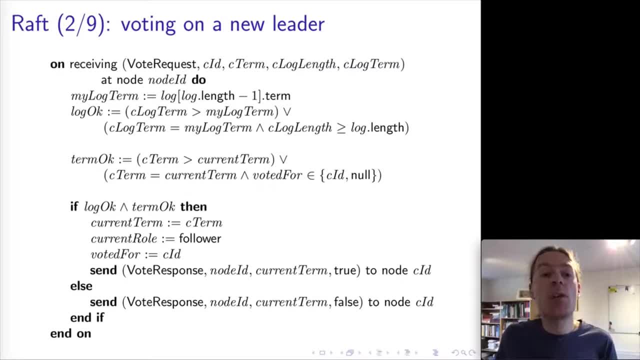 that log, and so the purpose of this is to ensure that the candidate has an up to date log, because we don't want to vote for a candidate that has a really outdated log, because that might cause us to violate the property of our algorithm that once a message has been committed. 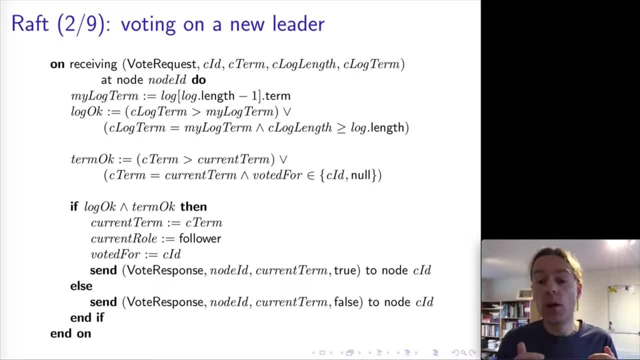 it is not going to change anymore. so, in order to make sure that committed messages don't change, we have to ensure that we vote only for candidates whose log is sufficiently up to date, and this is the check of whether the log is up to date, the other thing we have. 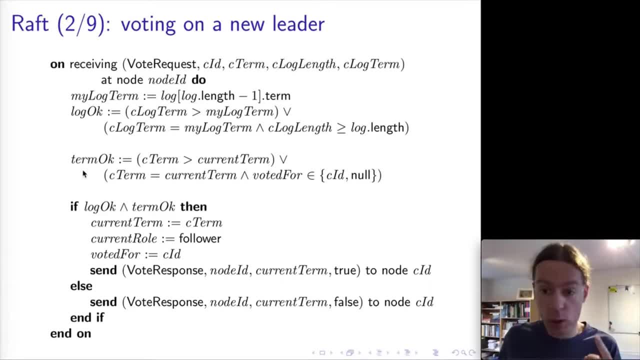 to ensure is to make sure that we don't vote for more than one candidate in a given term, and this is what this condition here does. so if the candidate's term is greater than our own term, then it's fine, or if the candidate's term is equal to our own term. 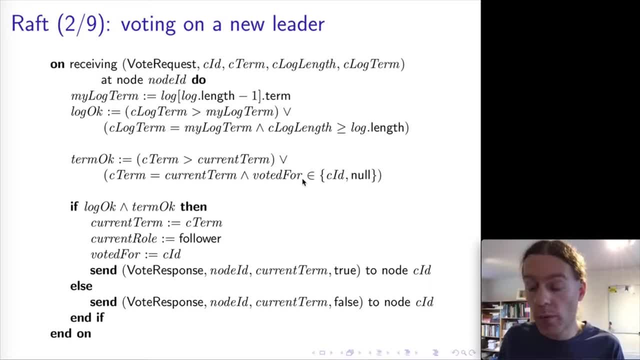 but the value of the voted for variable is either the candidate that we are being asked to vote for or we have not voted previously in the current term, which is indicated by the value null. so in this case the term is also okay. but if the candidate's term is lower than, 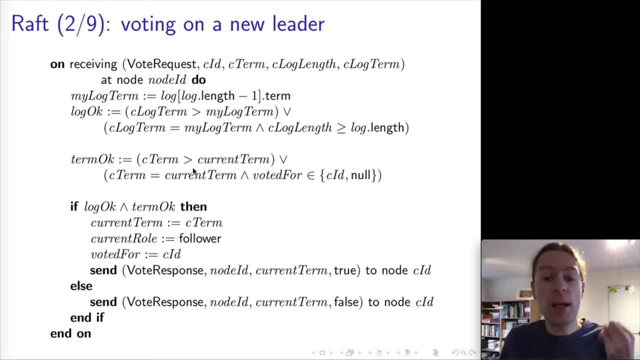 the current term. it's definitely not okay. so we've checked. if the log is okay, if the candidate log is okay and the candidate term is okay, if both of those are okay, then we are going to vote in favor of the candidate and the way we're going to do. 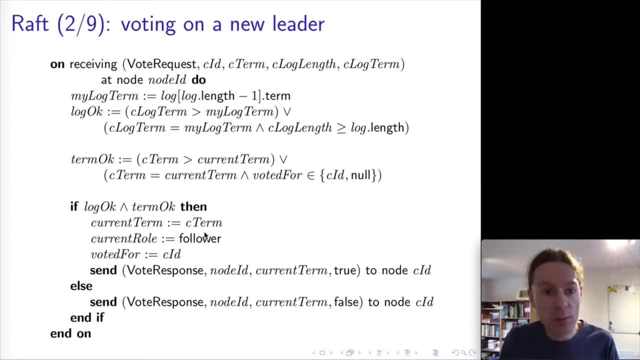 that is, first of all. we're going to update our current term to be the term of the candidate. we're going to update our own role to be a follower. we're going to say that we voted for the candidate and we're going to send a vote response message back. 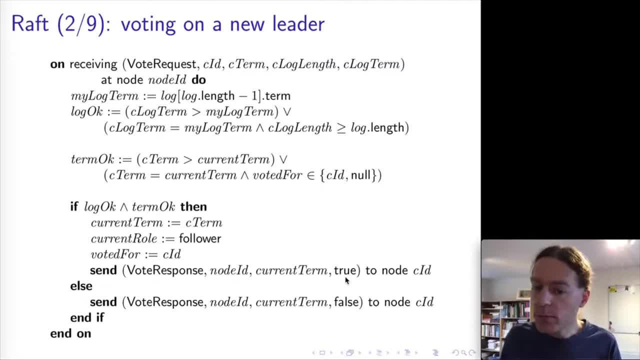 to the candidate, with this last field being true. so this last true means yes, we are voting in favor of you as candidate and we include the node that is voting, and we include the current term in this message as well, so that the recipient knows which term we're talking about. 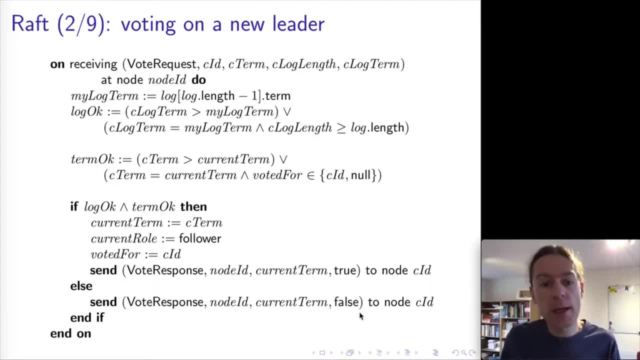 however, if the log is not okay or if the term is not okay, then we send a vote response message with a value of false, and this false here just means that we are not voting in favor of this particular candidate. okay, so now we're back on the candidate. 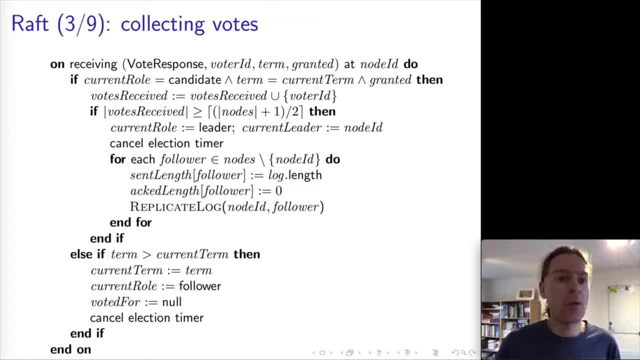 side and on the candidate side. we need to look at handling those vote responses. so first of all we're going to look at the term in in this message, in the vote response message. so we get a vote response message containing a certain term. so if that term is greater, 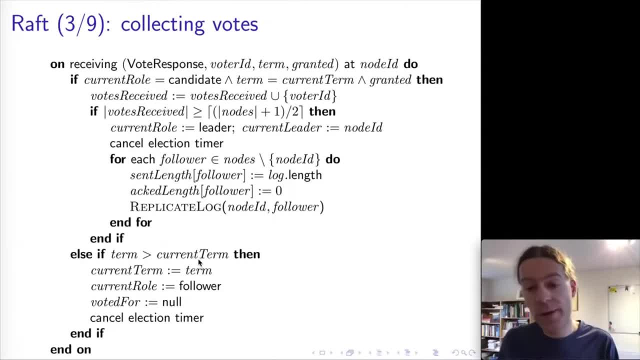 than the candidate's term. then remember the state transition diagram earlier. this means that we're going to transition back to follower state and we're just going to let the other candidate do its election. so in this case here we update our current term to be the higher term, we transition to follower. 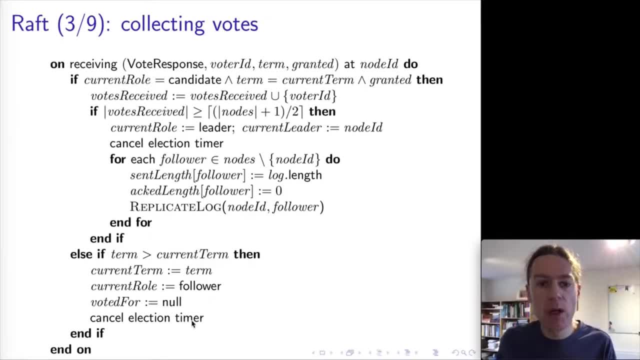 state, we forget what we voted for in the previous term and we cancel our own election. if this term is less than our current term, we just ignore the message. but if the term is equal to the current term and if we are in the candidate state and if the 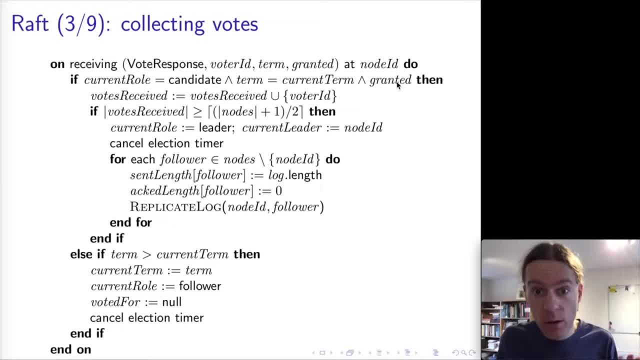 if the voter voted in favor of us, so this granted field here. if that is set to true, if all of those are the case, then we have a successful vote in this particular election, and so what we're going to do is we have this set here of votes that we've 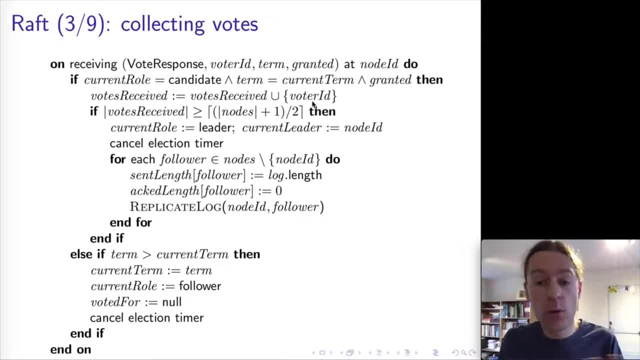 received and we're going to add the ID of the voter who's voted in favor of us to that set. note that this is an idempotent operation, so if that vote got duplicated for some reason, we're not going to count the same voter twice, so we're only going to count. 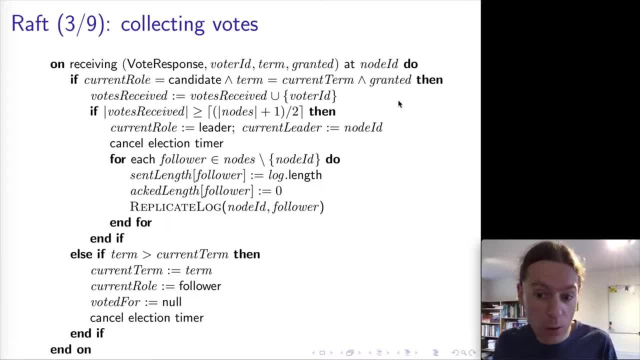 the unique nodes that have voted in favor of a certain candidate. we're not going to count how many times they voted if it's more than one. so now we have this set of votes and if this is a quorum, then we can transition to leader state. so 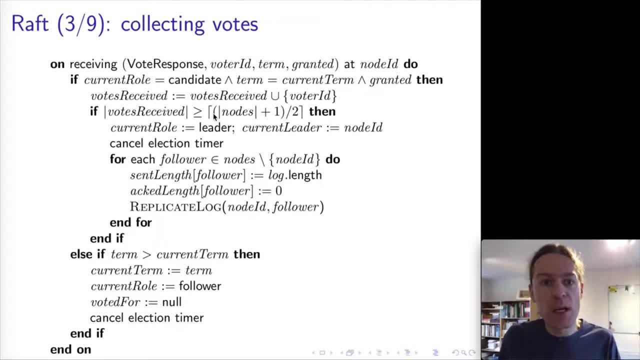 we define here a quorum to be a majority quorum, which means we take the number of nodes that we have in the system, add one, divide by two, round up, that gives us the minimum number of votes that we need in order to have a quorum. so, in order to 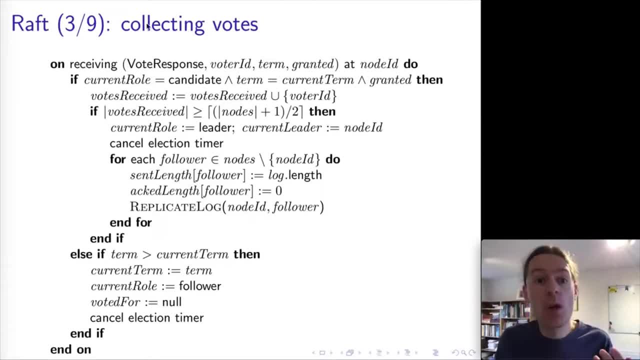 for this vote, this leader election, to be successful. so if we have that number of votes, then we can transition into leader state. we can say that the current leader is ourselves. we can cancel the election because we're done, now we've got sufficient votes and now we're. 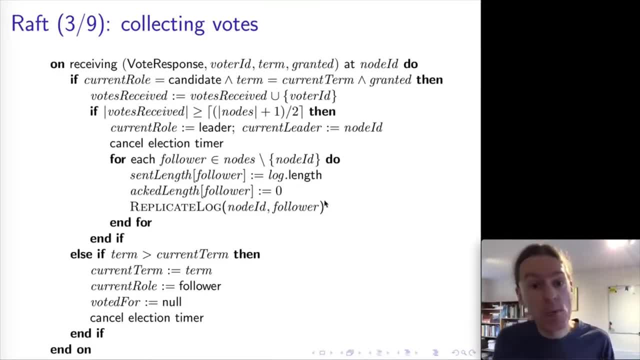 going to initialize some state that is needed for the leader. so what the leader needs to do is it needs to set these variables here- sent length and act length- and these map a node id to an integer, and so the initial value for these maps here is going to be that for each follower. 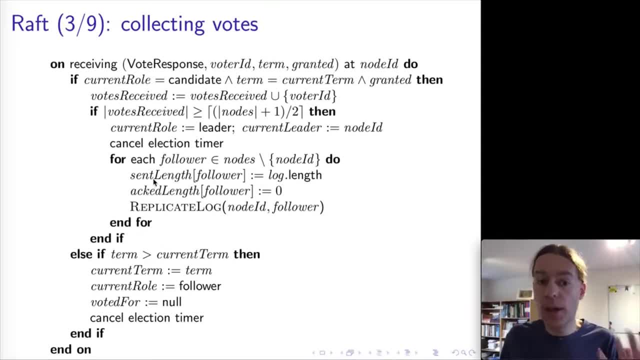 in the system. we set the initial value for that in the set length object. we set the current value to be the current length of the log and we set the act length to be zero. so the meaning of these two things is sent length is the length of the log. 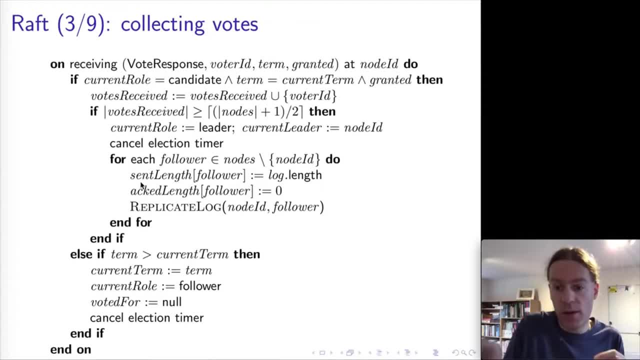 since the beginning of the log that we think we have sent to this particular follower and act length is the length of the log, counted from the beginning of the log of entries that have been acknowledged by the follower as having been received, and so the distinction between these two will become. 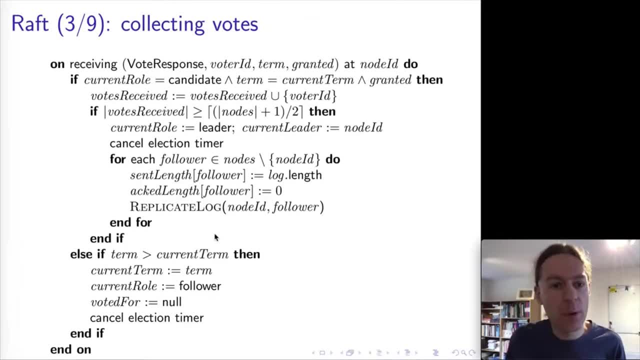 important later. for now, just take them as some variables here. and finally, we call this replicate log function here, which is discussed on a later slide, and the purpose of this replicate log function right now is just to send an initial message to all of the followers saying: hey, i'm. 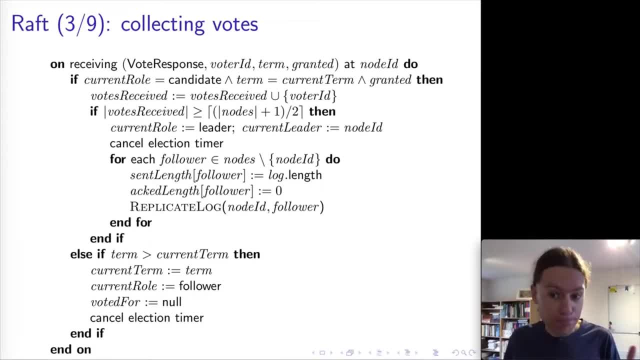 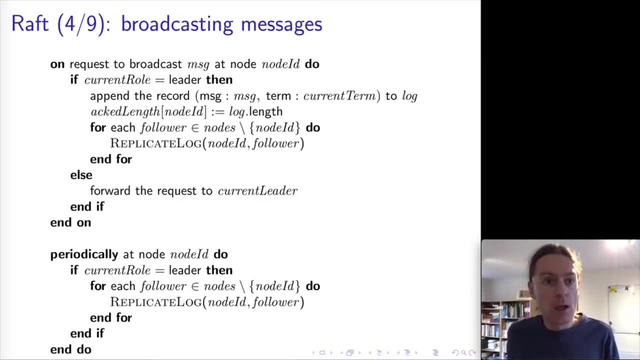 your new leader. please accept me as your leader. okay, so this is what the what the node does on transitioning to leader. now we also need to look at now what happens if a node wants to broadcast a message via total order broadcast. so that's, after all, what we're here for. but 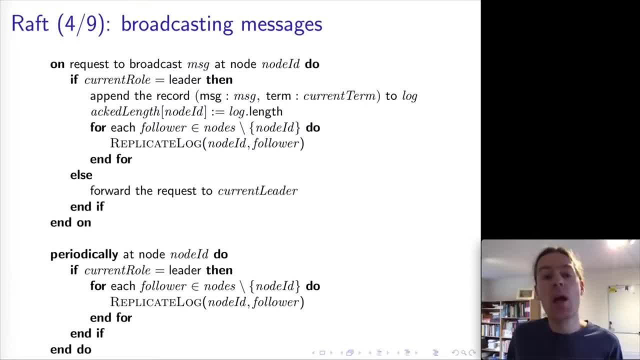 the whole purpose of this exercise is to implement total order broadcast, and this is what this first block here does. so if we want to broadcast the message msg here at some node, well, first of all it depends if this node is actually the leader or not. so if it's not the leader, then 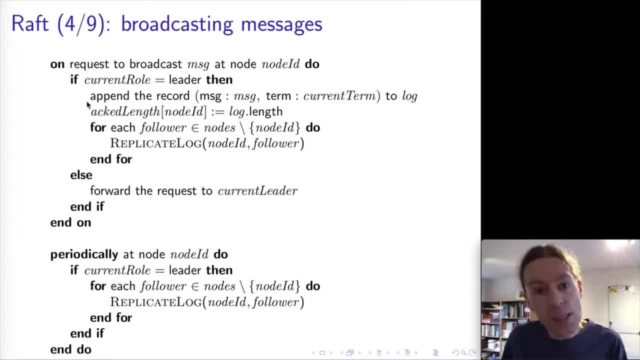 we just forward the request to the current leader. what the leader does if it wants to broadcast a message is well, first of all, it appends an entry to its log. so the entry, as i said earlier, consists of the message that we want to deliver and the current term of the leader at 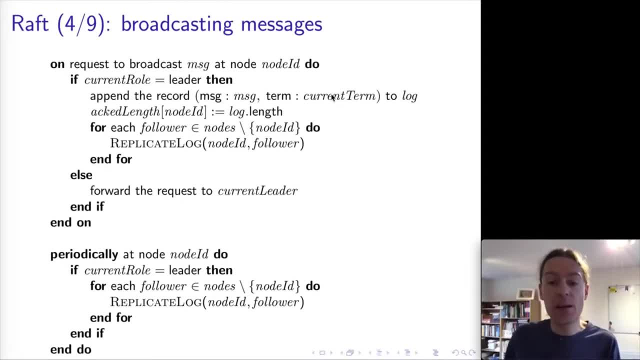 the time when this message is broadcast. so simply appending the message to the log is essentially the act of broadcasting that message. now we need to tell all of the followers about this message that we've added to the log, and so, first of all, we're going to update this. 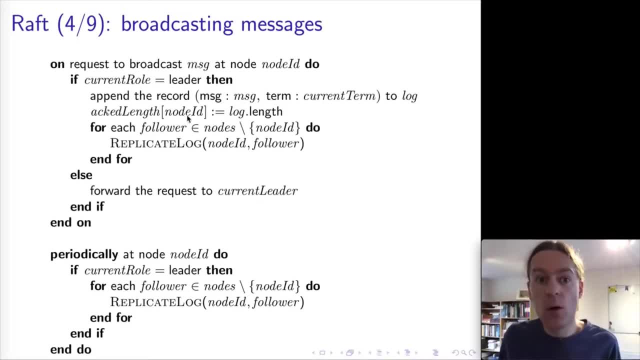 act length variable here, which is just to say that node id is just the leader itself, so the leader itself acknowledges that it has received this log. this is just something in order to make the quorums work later and then for each of the followers, which is just each node except to the leader. 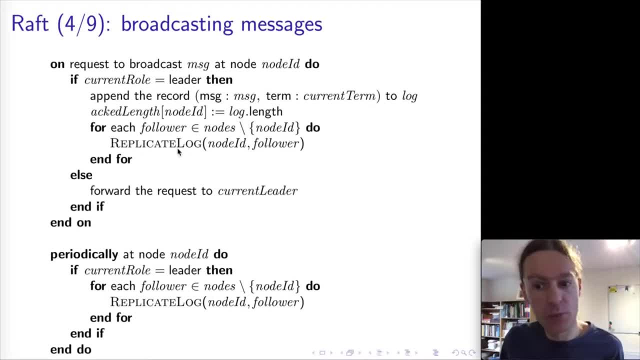 itself. we again call this replicate log function, which i will come to on the next slide. so the replicate log function then does the actual work of taking the new entry in the log and distributing it to all of the followers. so in addition to this, we also call this: 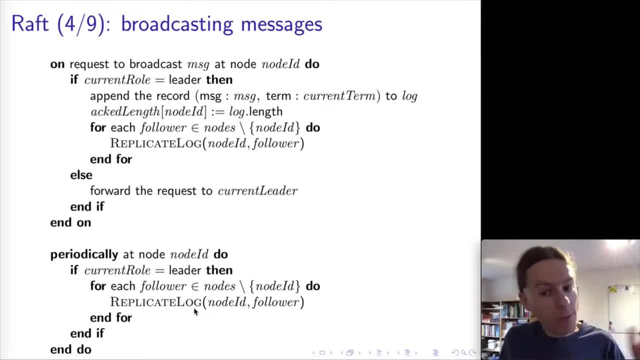 replicate log function periodically. so we can just have a background timer on the leader, and as long as this node is the leader, it's just going to periodically call this replicate log function once for each follower, and the reason for this is several fold. so, first of all, 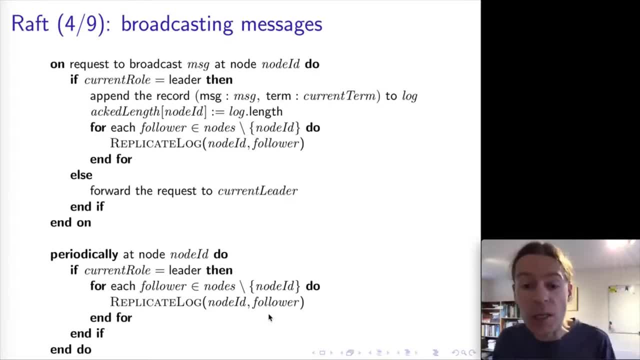 it's going to do this as a kind of heartbeat, so as a way of letting the followers know that the leader is still alive, because every time you call this replicate log function, as you see, it's going to send a message to that follower and the follower can just sit there and 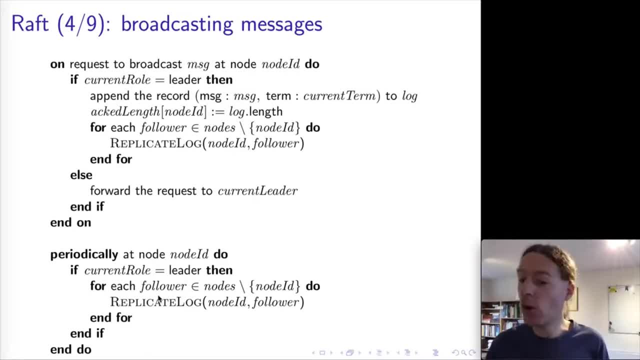 see like: oh, am i getting messages? as long as it's getting regular messages from the leader, then everything is fine. it doesn't need to start any new election. another purpose of sending this calling this replicate log function periodically is that some messages might be lost in the network and we 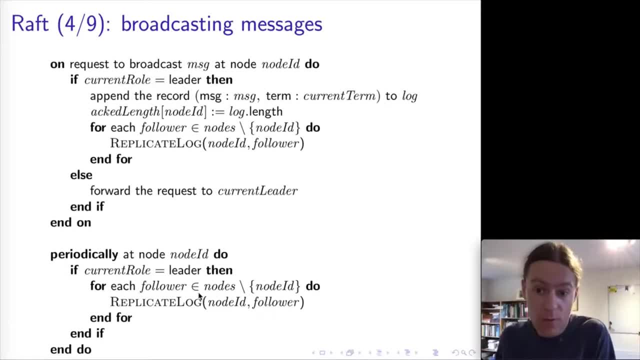 still want every log entry to end up on every follower, and so therefore, calling this periodically will also retransmit any lost messages, if necessary. okay, so finally, the the reason for calling replicate log repeatedly is also for the commit purposes, but we'll come to the committing of log entries later. 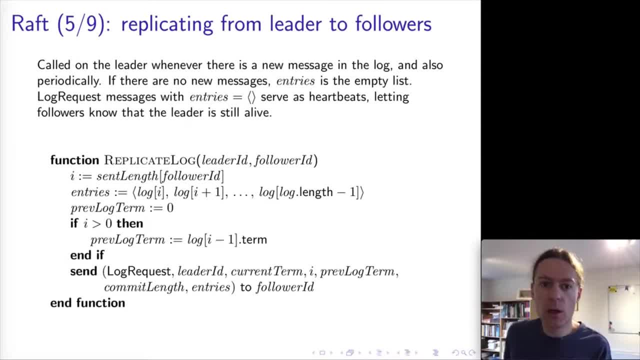 so let's have a look at this replicate log function here. so this has two arguments, the id of the leader and the follower, and what we want to do is we want to send to the follower any log entries that the follower doesn't already have, and so, remember, we have this variable. 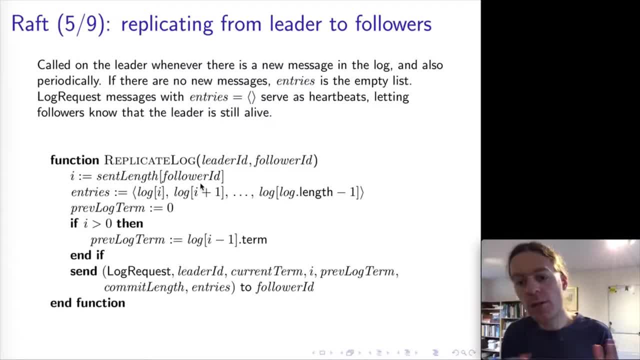 here the sent length, which, for each follower, tells us the number of log entries, counted from the beginning of the log that we think we have already sent to that particular follower. and so i'm just going to call that i, and now i'm going to take a suffix of the 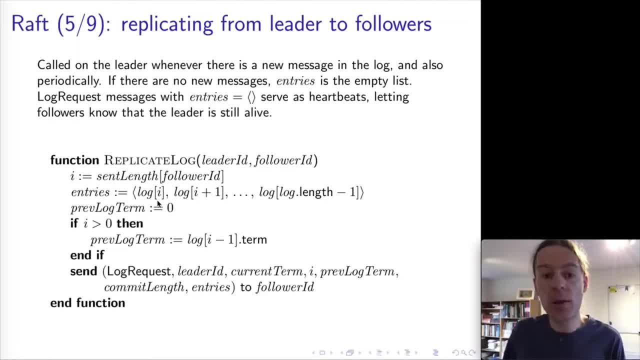 log. so i'm going to start at index i in the log and take all of the log entries from i onwards up until the end of the log. so log dot length minus one is just the last entry in the log and so this might be empty. so if 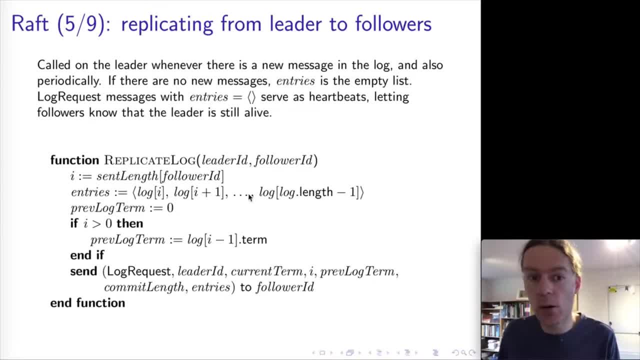 the send length for the follower id is actually equal to the log length, in which case? in that case, then, entries will just be an empty array, but it could be one log entry, it could be more than one entry log entry as well. so these are the log entries that we're. 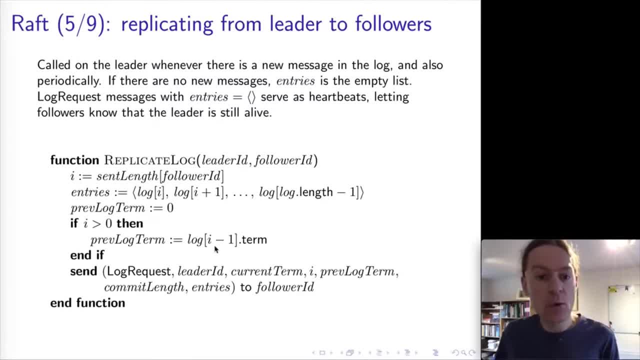 going to send to the follower. the other thing we need to do is now look at the last log entry just before this suffix that we're sending to the follower. so that's the i minus one entry, and we're going to get its term and we're going to need that later to do. 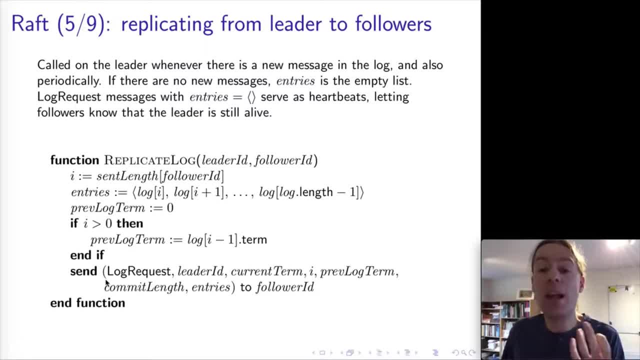 a consistency check on the logs. so now we're going to send a log request message to the follower, and this message is going to contain a whole bunch of things, so it's going to contain the this entries. so the new entries, log entries that we want to send. 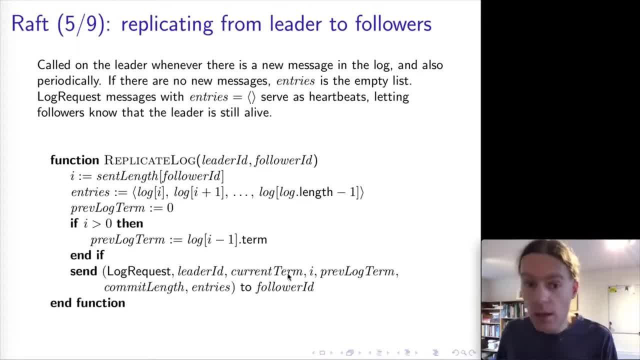 to the follower. it's going to contain the id of the leader. it's going to contain the leader's current term. it's going to contain i, which, if you remember here, is the, the length prefix that we think we have sent the this follower previously. we've got 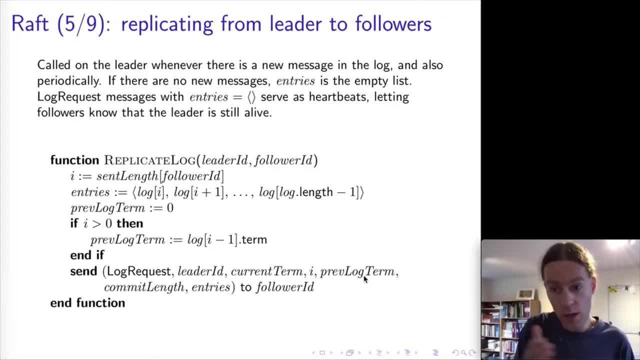 the log term of the last, the last log entry in this prefix and finally, the value of the commit length variable, which will become useful later when we are dealing with commits of log entries. so all of that gets packaged into a message and that gets sent to the follower now. 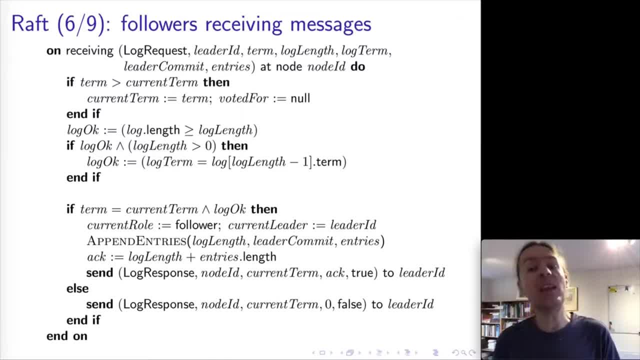 we are on the follower and we're going to look at what happens when we receive one of those log request messages. so it has exactly those fields that we just talked about. the follower node is now going to be node id and, as usual, the first thing we're going 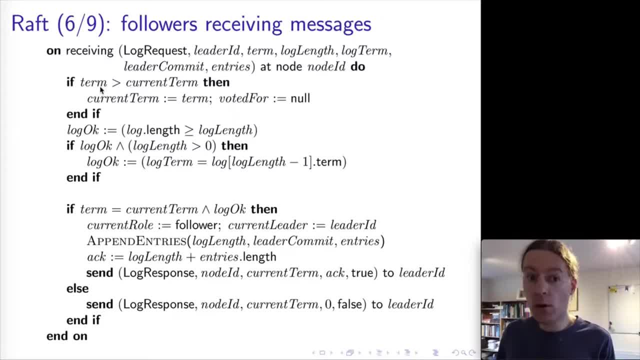 to do is check the term. so if the term of the log request is greater than the current term of the follower, then we're going to update our current term. so we're always going to move to newer terms and if we move to a new term, we're going. 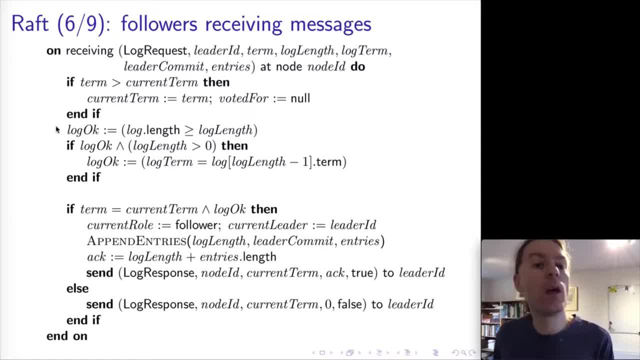 to forget about who we voted for in the previous term. and then we need to check the consistency of the log, so the follower may or may not accept these log entries from the leader, depending on what the state of the follower's own log is, because it could be that, for example, 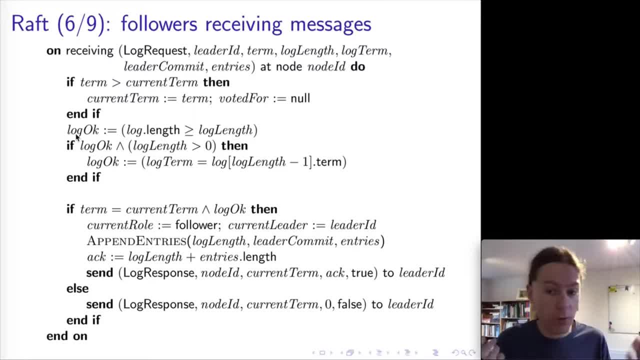 the follower missed a whole bunch of messages because it was offline for a while, and so it might have a gap in the log. so it could be that the follower is not a member of the leader and so it could be that the the leader has some some log. but 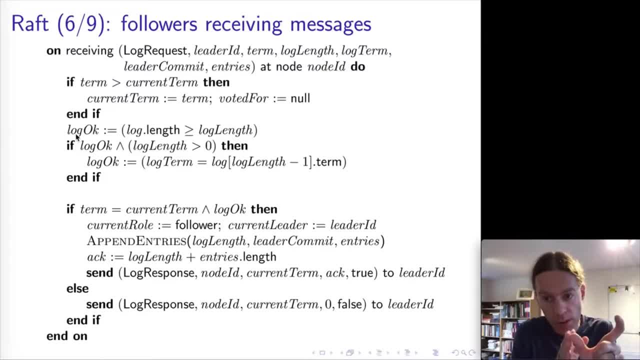 there's a gap between the end of the prefix that the leader had earlier and the message that the leader is trying to send to the follower, and so we have to detect if that kind of gap has occurred. so first of all, remember this log length here, which is one of the fields in the 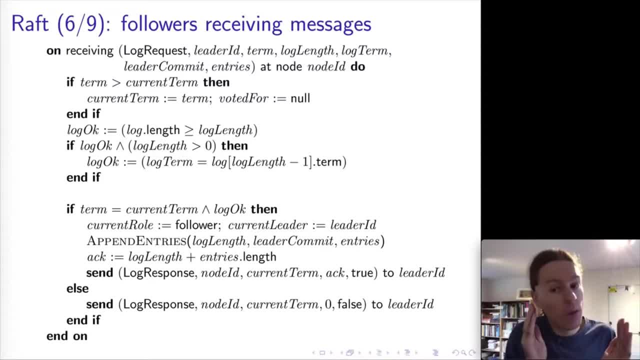 message. this log length is the length of the suffix that we're not sending to the leader, that after which we've sent the suffix, which is the entries. so we've got the whole log. it consists of a prefix that we're not sending and then the last few entries, which is a 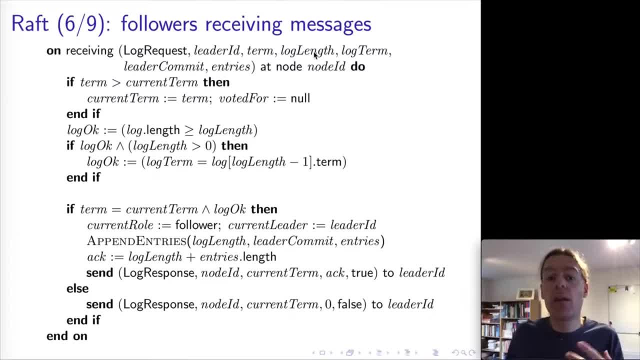 suffix which we are sending. this log length is the length of the prefix that we're not sending, and so first of all, we need to check that the follower's own log is at least as long as this prefix, because if the follower's own log is shorter, that means we have a gap in the 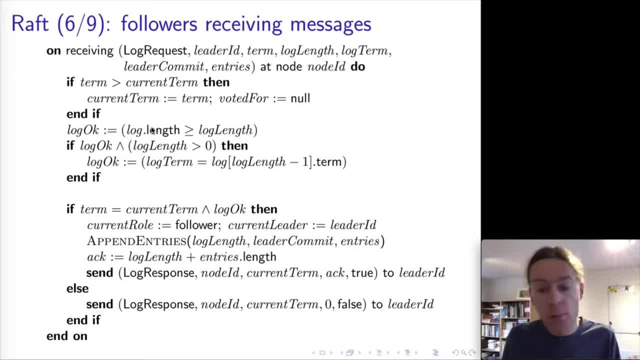 log. so we definitely can't accept the entries because we're missing some, some entries. so we have to ask for those missing entries first. um, but if our follower log is long enough, then we also have to check the terms, and so, in particular, we we require that if we look at the followers log. 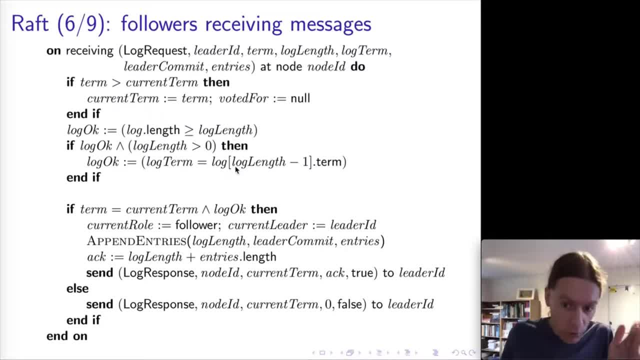 and we look at the last entry that just precedes the new set of entries that we've been sent by the leader. we look at the term of that entry and we compare it to the equivalent term of the message that we received from the leader. what we want is for those to be the same. 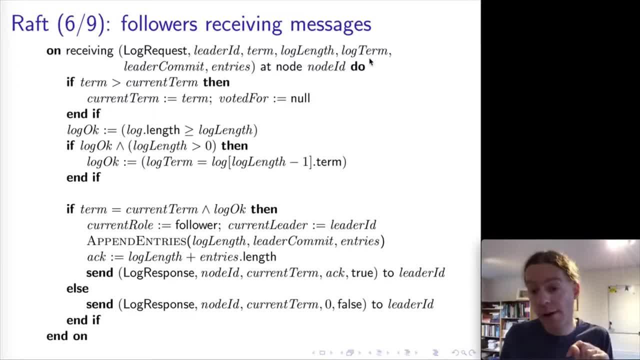 term, because if it's the same term, then ralph guarantees that this is actually the same log entry and also that all of the log entries before that point are the same. so this is a very nice property to have. if these terms are the same, we can. 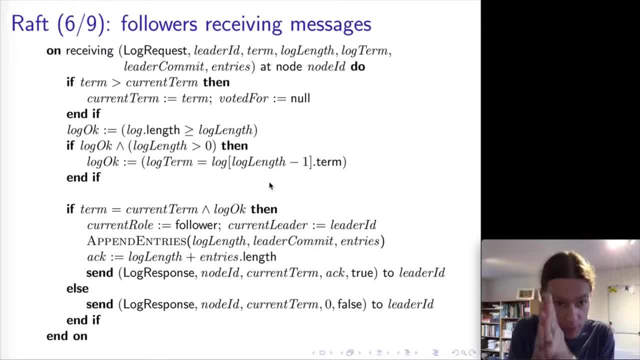 guarantee, actually, that the logs are consistent up to this point log length here. and so if this is the case, then the log is okay. but if the log is not okay, then we're going to send a message back to the leader saying: hey, you need to give me some earlier log. 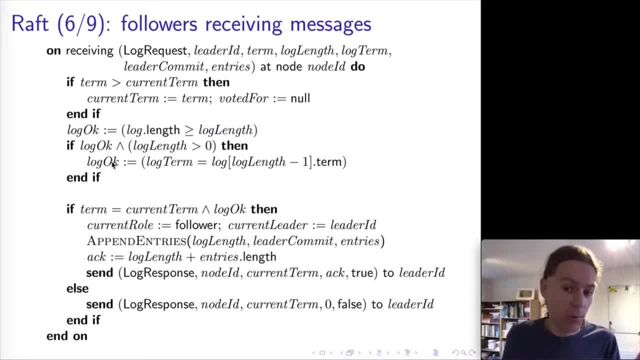 entries because we've got a gap or we've got an inconsistency in the logs. so now, if the followers term equals the leader's term and if the log is okay according to this rule here, then well, we will stay in the follower role. we will accept the 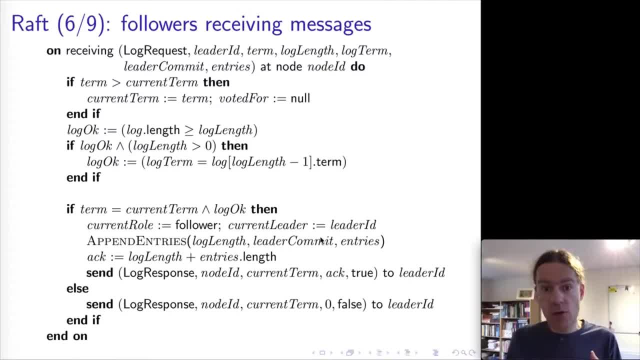 the leader, who is just sending us entries as our leader, and we're going to leader And we will call this append entries function here in order to take the entries that we've been just sent by the leader and to add them to the followers log. 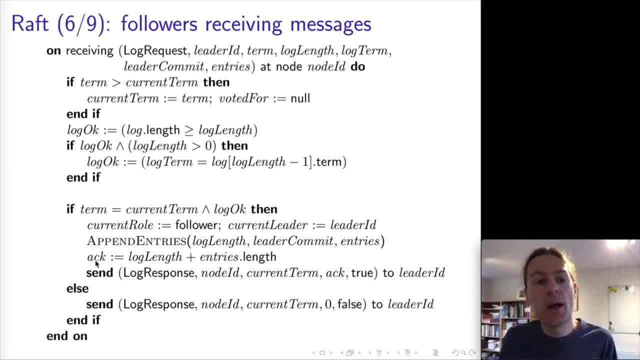 So I'll come to that append entries in a moment. Then we need to acknowledge back to the leader that we have received these log entries. So we're going to compute the length of the log, So all of the prefix plus the length of the entries, the suffix that we've been sent. 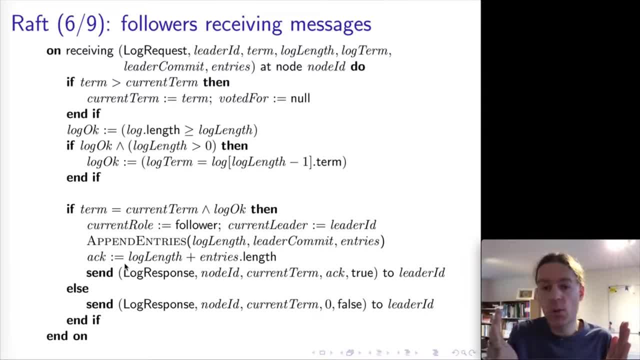 that's the whole length that we are now acknowledging. So we're acknowledging we've received the entire log up to a certain length and that's this variable acc here, And then we're going to send back this message, a log response message, back to the leader And 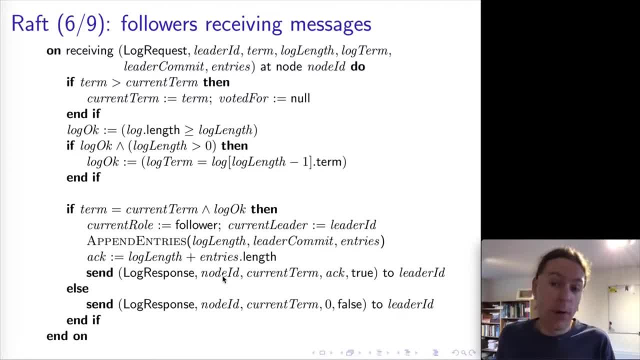 log response is going to contain the ID of the follower that is responding, the current term in which this is happening, the acknowledgement, which is the length of how long of the log we are acknowledging, And true means that it's all okay. We are acknowledging that this log is. 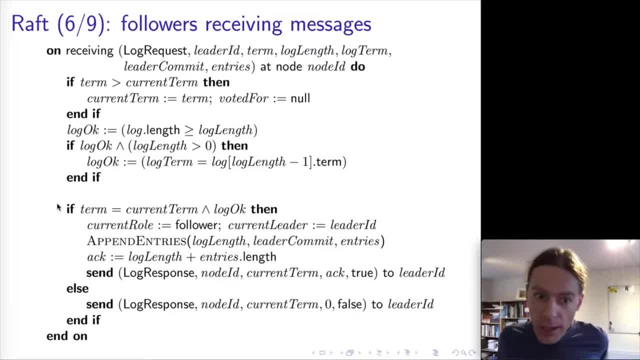 fine. On the other hand, if the log was not okay or if the term was a mismatch, then we're going to send back a log response message in which this last field is false. We're going to send that back to the leader, And so that way, the leader is going to know that oh, we've got a problem. 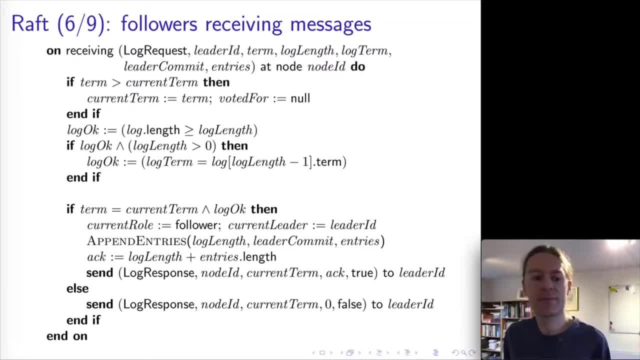 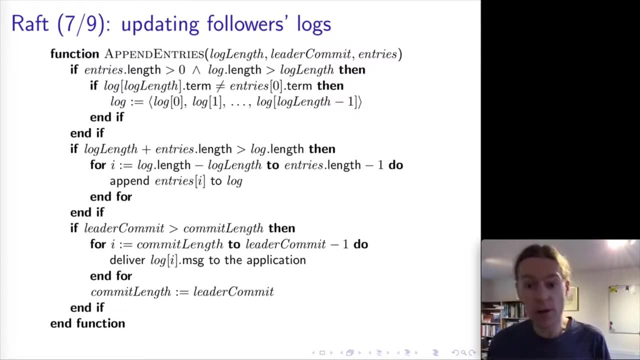 with the log here. So that is the whole logic for the follower receiving the log request from the leader, except for the append entries function. So I will go to that function next. So the purpose of this function is to update the followers log from the entries that is received. 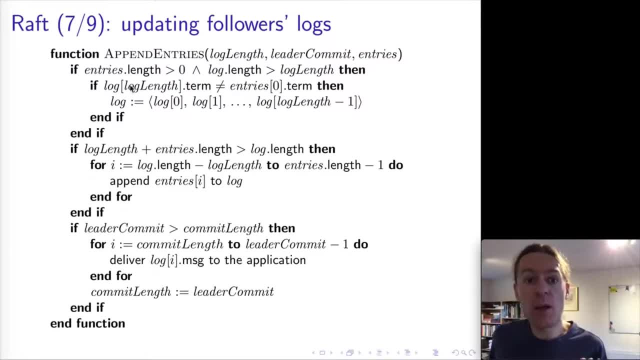 from the leader, And the first thing we have to do is to check whether those two logs are consistent with each other. So here, first of all, in the case where we've received at least one entry from the leader and where the followers log is long enough that it overlaps with those, 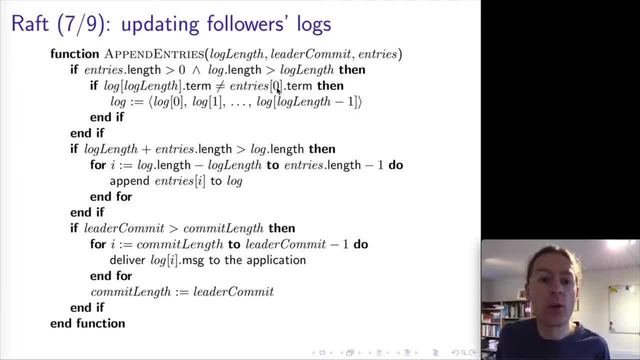 entries received from the leader. we're going to actually compare the term of the first log entry that we've got from the leader And we're going to compare that to the corresponding log entry on the follower. So this should be the same term if the logs are consistent with each other. 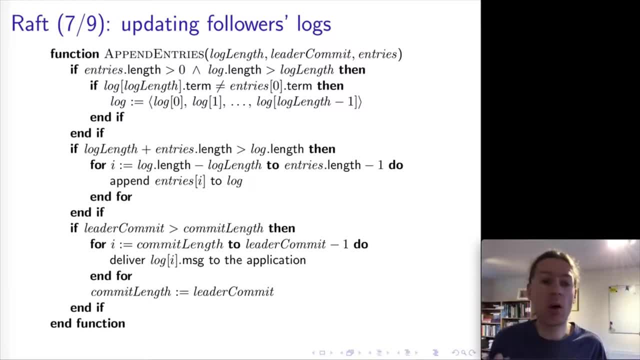 But it could be that the terms are different because, for example, maybe the follower saw some updates from a different leader that then crashed and then was superseded by a new leader, And so for that reason it could be that the two nodes have some log entries that are not the same. 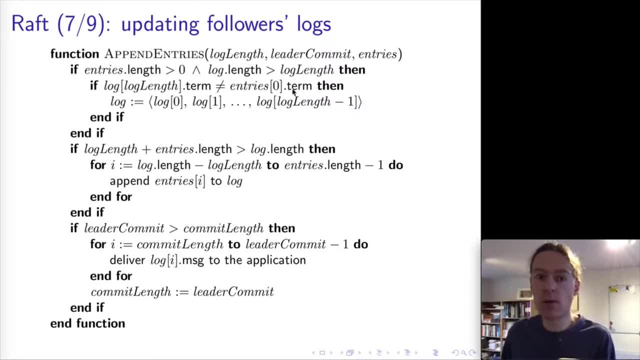 that have different, And so that's why we're going to compare these terms, And if it turns out that these terms for the same log entry are different, then we're going to truncate the log. So truncating the log means we're going to cut off all of the log entries on the follower that are after the length. 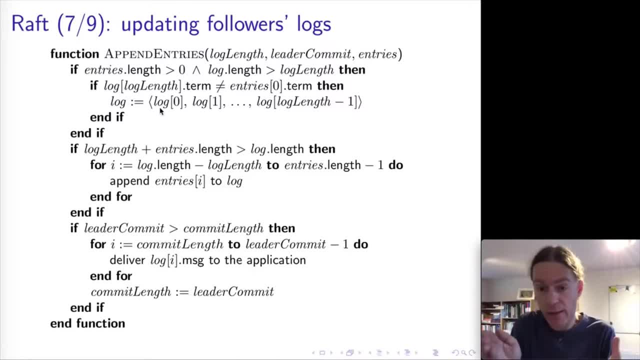 log length. So we're going to take the first log length entries from 0 up to log length minus 1, and those log entries are staying unchanged, But everything after that point we're cutting off and we're going to truncate the log. So that's why we're going to cut off all of the log entries on the follower. 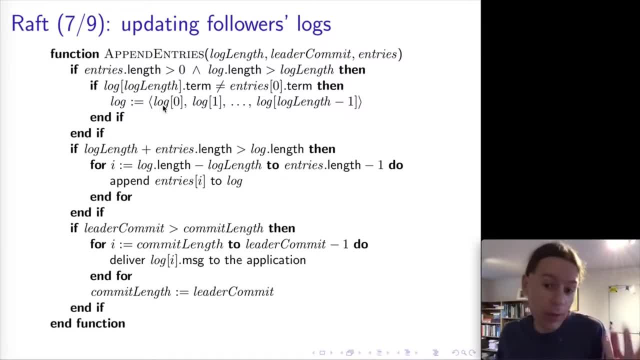 But everything after that point. we're going to truncate the log. So truncating the log means we're going to just forgetting about it, And Raft guarantees that any log entries that are discarded here will not yet be committed, And so therefore it's fine for us to discard those and replace them with new log. 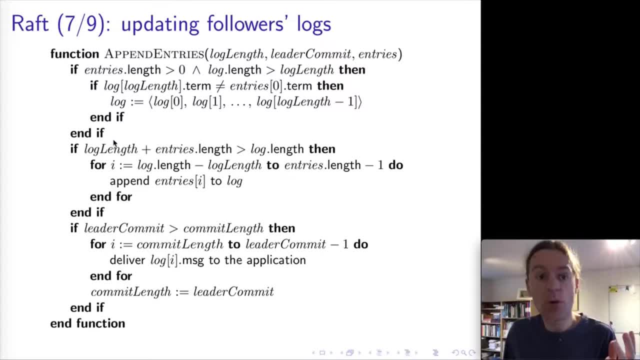 entries. So here we have truncated the log. Next, we want to append any new entries to the log, But it might be that there are duplicates here, So there might be that our log already contains some of the entries that the leader has sent us because of a message. 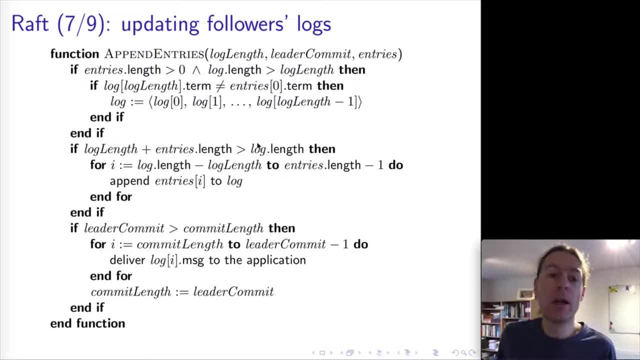 So we have to make this idempotent, And the way we do that is we look. well, if the log length plus the new entries of the length indicates that there are some log records that we don't yet have in our own log, then we're going to go through those additional log entries that are 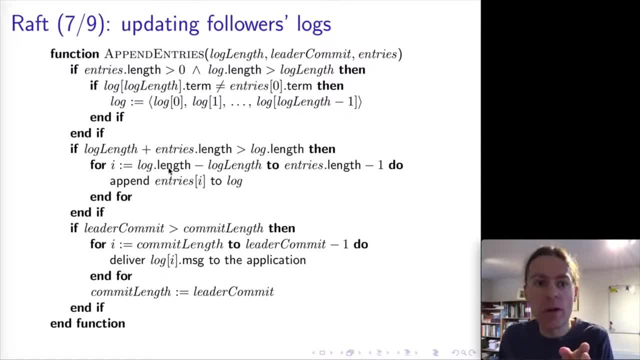 beyond our existing log length and up to the end of the log entries And each of those we're just going to append to the followers log. Now, after we've done that, there comes the commit. So here the leader commit. here is an integer variable that we were sent by the leader. 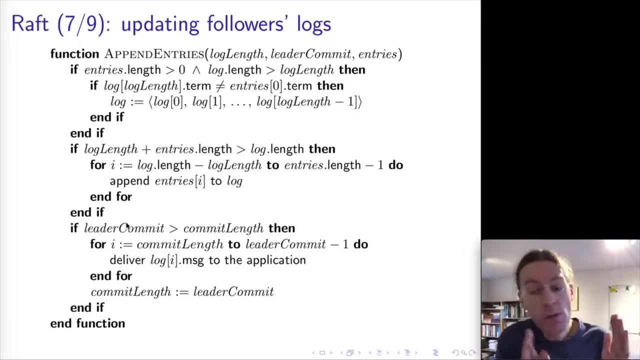 telling us how many log entries, counted from the start of the log, are ready to be committed. And this starts off as zero, because no log entries are committed initially, And then some log entries are added And then sometime later the commit length moves forward. 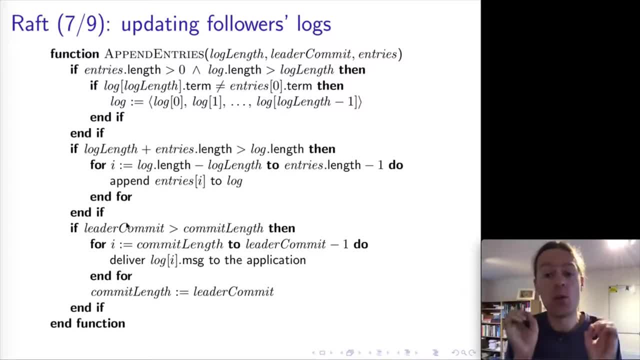 When those log entries are ready to be committed. And to be committed here means we can actually deliver them to the application via total order broadcast. So at this point these log entries are final and they're not going to change anymore, So they're safe to be delivered. 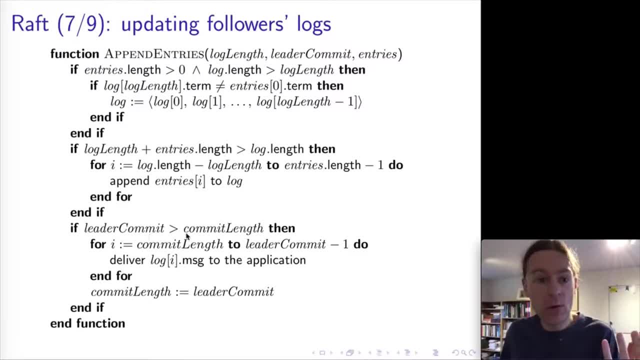 And so here we look at this leader commit value that we've been sent by the leader and we compare it to the followers local commit length value And if the leader commit is greater, that means we have new records that are ready to be committed, And to commit them here just means we're going to 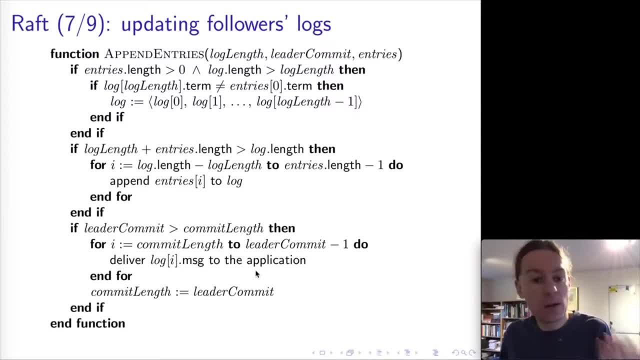 deliver each of those log entries the message. we're going to deliver that to the application And then we're going to move the followers commit length forward to match with the leader's commit length. Okay, so that's actually everything from the followers point of view. Now we just need to. 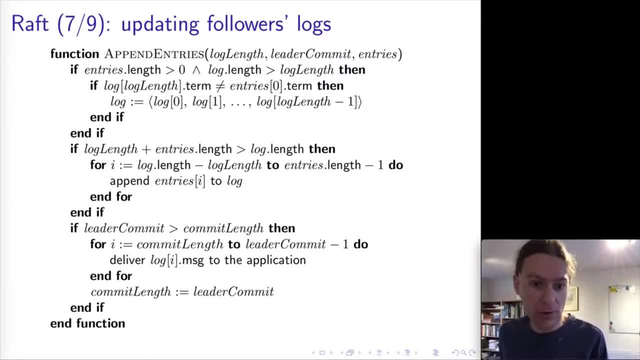 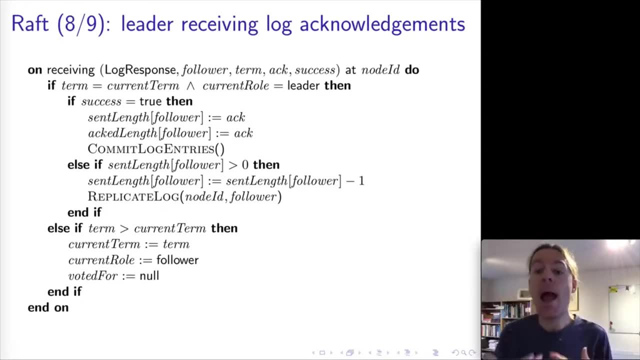 go back to the leader and actually deal with this committing business. So remember the followers send log response messages back to the leader And then we're going to move. the followers commit length forward to match with the leader And now the leader has to receive those log response messages. 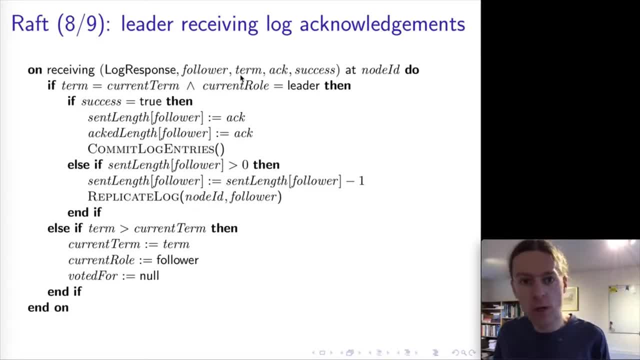 And so it's going to receive a log response from a certain follower in a certain term, acknowledging the receipt of a certain length of the log, And the success field will be either true or false, depending on whether the logs were consistent or not. And so this is the leader. 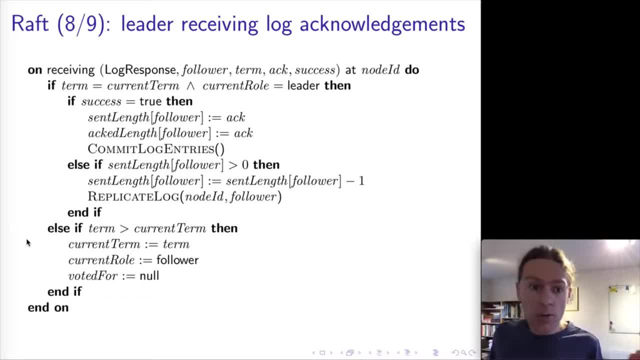 receiving this message. As usual, we first check the term first. So if the term in the message is lower than our current term, we just ignore the message. If the term is greater than our current term, that means, oh, there's a new leader in the system, So we're going to step. 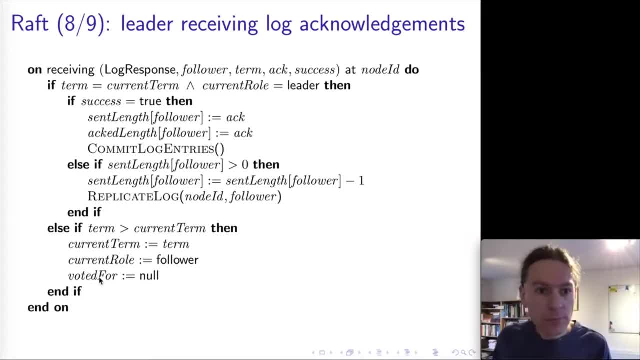 down to follower and we're going to update our current term. And here the interesting case is where the term equals our current term, the term in the message equals our current term and we are in the leader role. And in that case we're going to look at the success field and either see, is it? 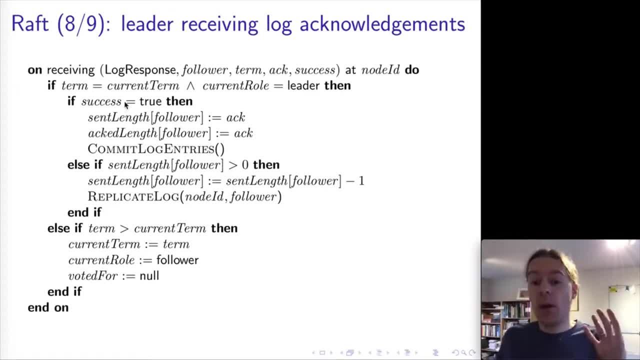 false or true. So if it's true, that means the follower has accepted these log entries. It's acknowledging receipt of those. And remember this ACK field. here is now an integer that tells us the number of log entries from the beginning of the log that have been received by the follower. 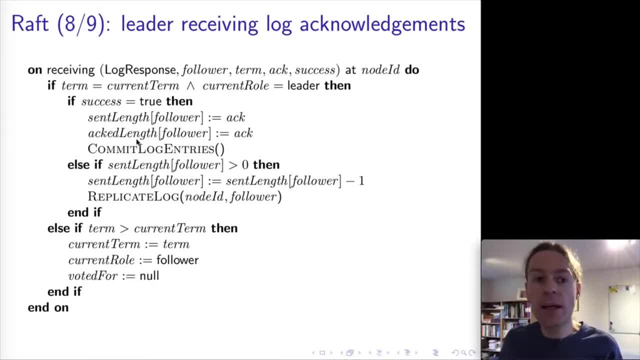 And now this variable sentLength and actLength. they're both going to be updated to this value ACK And we will see in a minute how these values are used when we look at the commitLogEntries function. So that's what we're going to look at in a minute And we're going to look at the 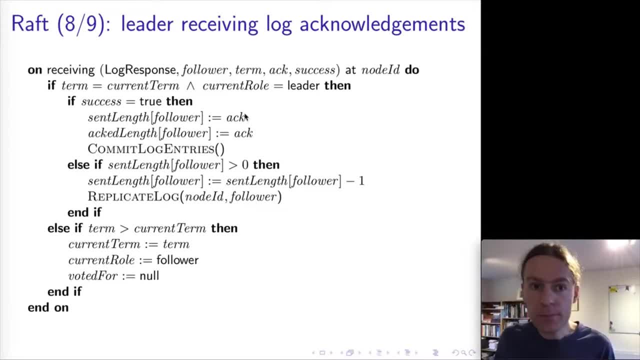 commitLogEntries will be on the next slide. So that is the case when this is a successful response from the follower. If it's not a successful response from the follower, well, that means in this case that the logs were inconsistent with each other or there was a gap. 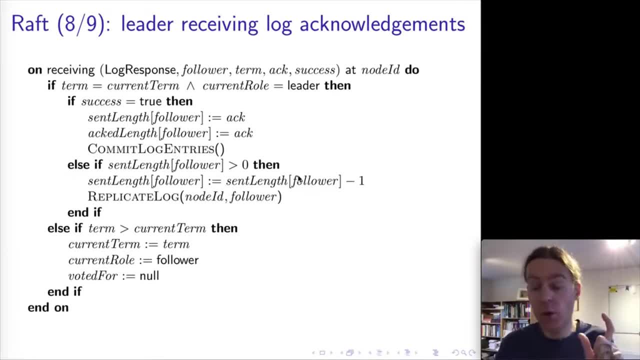 in the follower's log. So what the follower now is saying is: please give me some of the earlier bits of the log so that I can fill in my gap and fix my inconsistency in the log. So for that reason, here we're just going to decrement the sentLength variable for this. 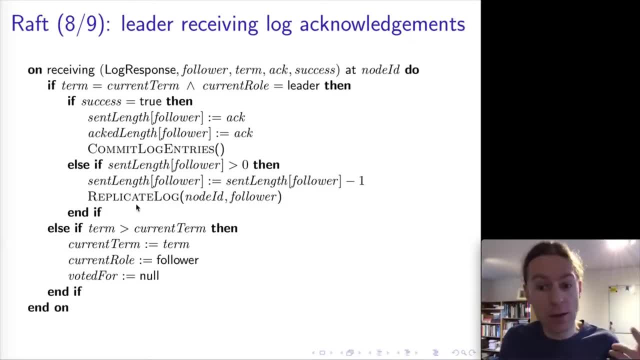 particular follower. We're just going to reduce it by one and we're going to replicate the log again. So we're going to retry And what this is just going to do is, earlier, we have this suffix of the log that we sent as the list of entries to the follower, And we're going to make this. 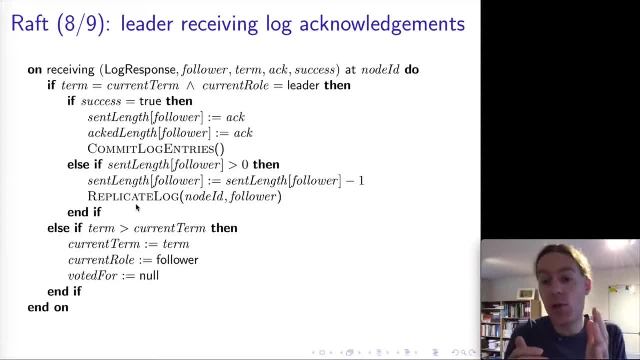 suffix bigger by one now. So we're just going to start one entry earlier in the log and send that entry to the follower, And if that doesn't work we might have to go around this loop a couple of times until we've filled in the whole gap between the follower's log and the leader's log. But 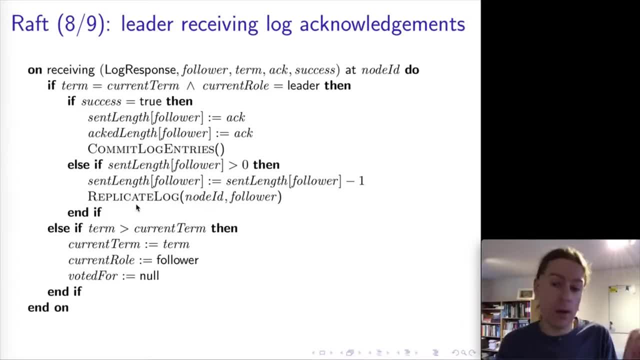 eventually, as you go back one by one, you will reach the point where the follower and the leader are consistent, which may be right at the beginning of the log, And so this here is handling the case where the follower is saying: we have a problem with the log. So here the leader is now. 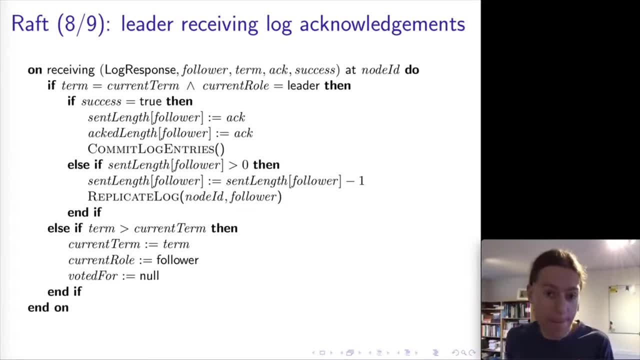 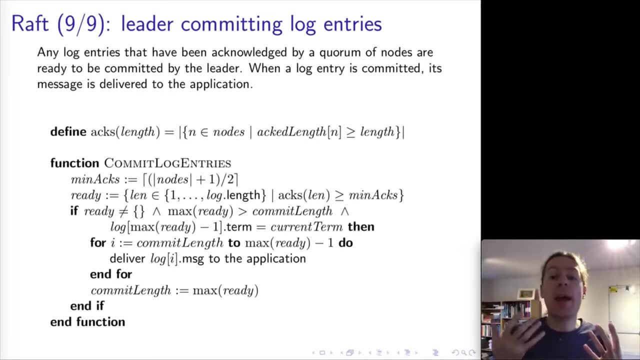 simply filling in this gap in the follower's log. So the last thing we need to look at now is this commit log entries function, And remember what I said earlier was that a leader can commit a log entry once it has been acknowledged by a quorum of nodes. So again for this delivery of a of a 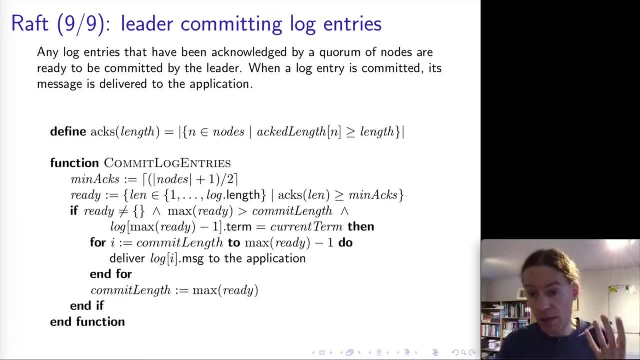 message in Total Order Broadcast: to be safe, we require it to have been acknowledged by a quorum first before we can deliver it. And this logic is done, is implemented by this function here. So first of all we have this little helper, function x, which, given a set of nodes, 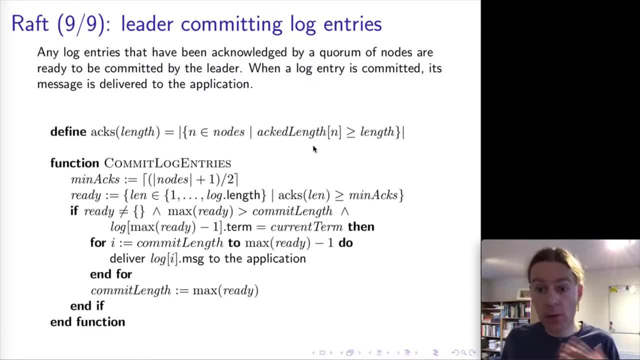 it looks at the act length variable of the current node And it tells us how many nodes have an act length that is greater than or equal to some integer length. So this is saying, given some length prefix of the log, how many of the nodes have acknowledged the log up to that point or later? 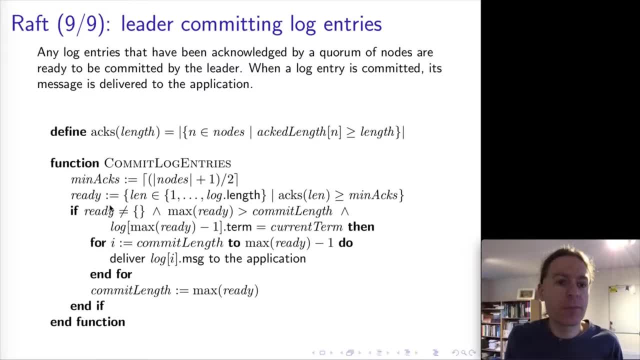 Okay, so this gives us back a number, a number of nodes, And what we're now going to do here, when we want to commit the log entries, is we're going to look at all the possible lengths of the log, So from one up to the whole length of the log, And for each of those lengths, 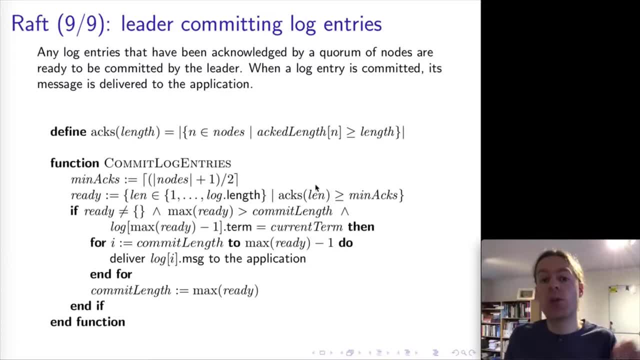 we're going to find the length for which the number of acknowledgements is greater than or equal to the minimum number of acknowledgements that we need. So the minimum number of acknowledgements is again a majority quorum, like before, more than half of the nodes. And so here this now gives us. 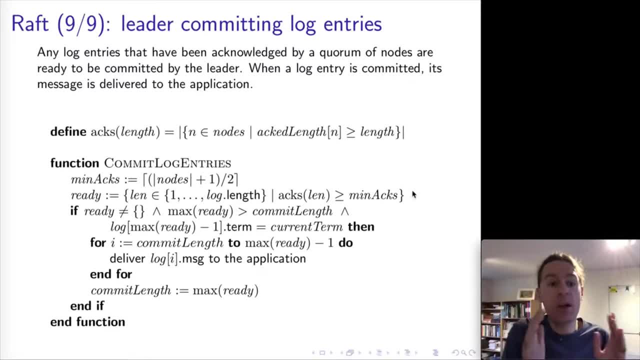 the set of all prefix lengths that are safe to be committed because they have been acknowledged, but by at least a quorum, And if this is a non empty set, that means that there's at least one log entry that is ready to be committed. 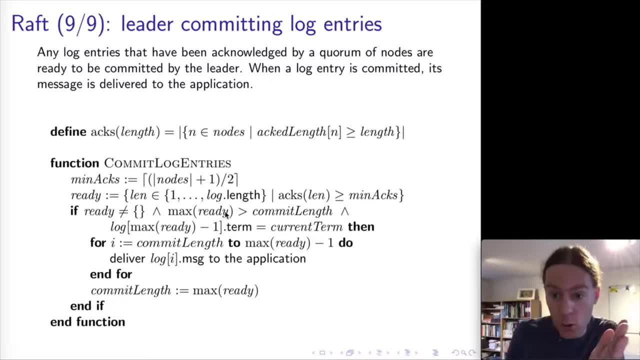 Then this set has a maximum and that is the latest log entry that is ready to be committed. So if this latest log entry that's ready to be committed is greater than the current value of our commit length variable, that means there are now new log records that are ready to be committed. 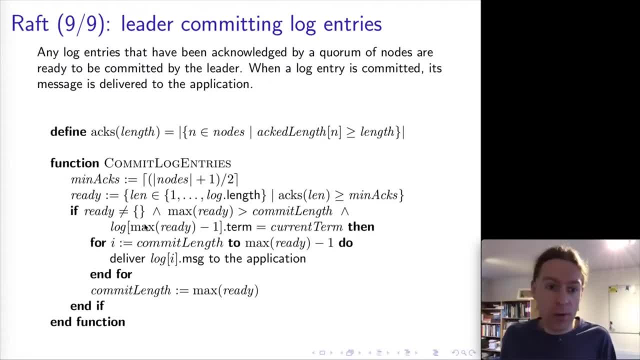 And if this is the case, and we need one extra consistency check, which is, if we look at the index of the last, the last log record, the last log entry to be committed, its term must match the current term. So this means we can't just commit a previous leader's log entries. we have to add at least: 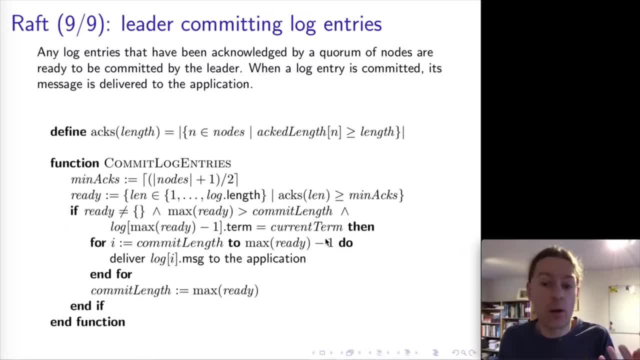 one log entry of our own. The leader has to add at least one log entry of its own to the log before it can actually commit anything. So if all of those things are satisfied, now we can commit the log entries, And so we're going to just loop over those log entries and we're going to deliver. 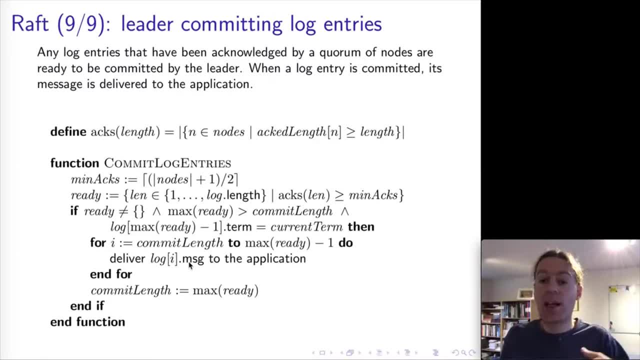 each of them to the application. So this is delivering it to the application on the leader node. And then we're going to update the commit length variable to be this, the maximum length up to which it's safe to commit. And this has no effect immediately, but the next time we send. 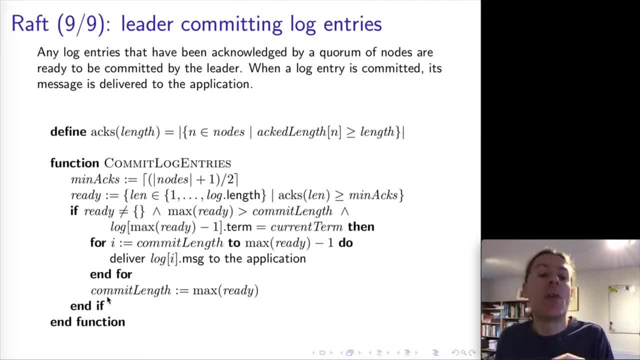 a log request message from the leader to the followers. the value of this commit length variable will be included in that message and that will then tell the followers up to which point they can commit and they can deliver messages to the application And that gives us total-order broadcast. It gives us total-order broadcast in a way that 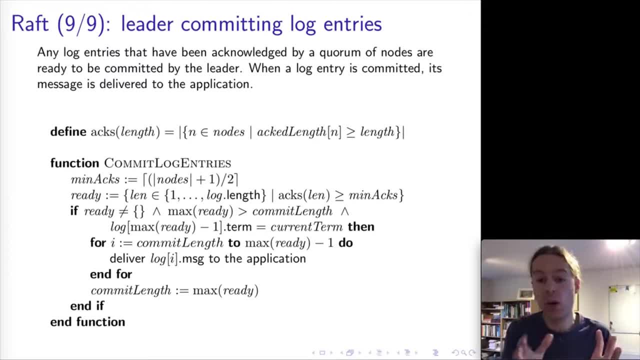 is fault tolerant, so it still works as long as a quorum of nodes is alive and able to respond to requests And it is safe. so even if weird timing behavior happens, you know you might get a couple of leader elections. it might take a while but the algorithm always guarantees that. 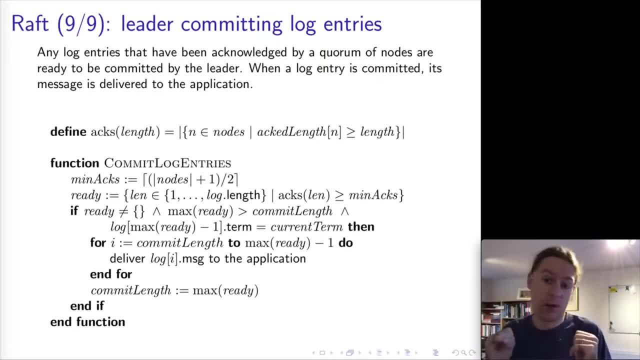 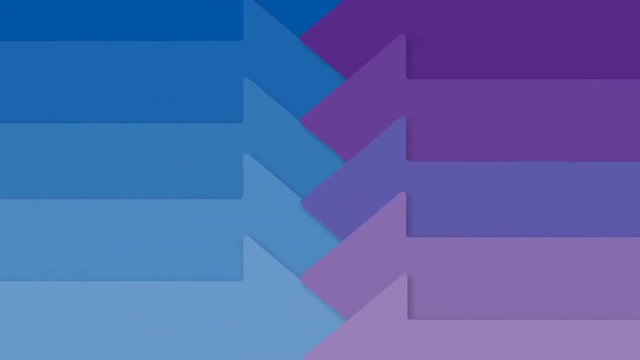 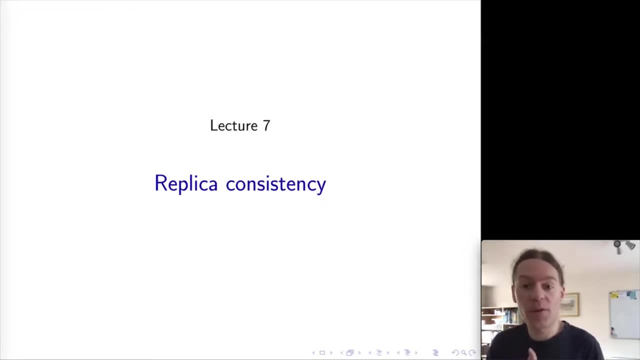 all of the nodes will deliver the same sequence of messages in the same order, And that's amazing. So I hope you were able to follow that. even though it's a rather complex algorithm, it is also a very interesting one. Hello everyone, and welcome to lecture seven of distributed systems. 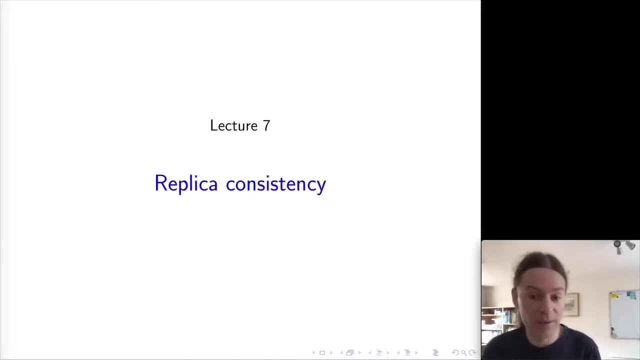 Today we will be talking about consistency of replicas. Now, consistency is a bit of a terrible word, unfortunately, because it means so many different things, depending on who you're asking and which context you're talking about. So just some of the things that you might have seen. consistency is in the context of transactions, So an ACID. 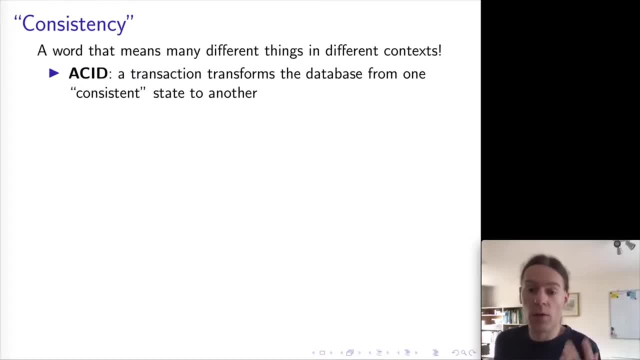 transaction. the C stands for consistency And in this context the meaning of consistency is a property of a database state. So we're saying the database is in a consistent state and if you apply a good transaction to it then it moves the database from one consistent state into another. 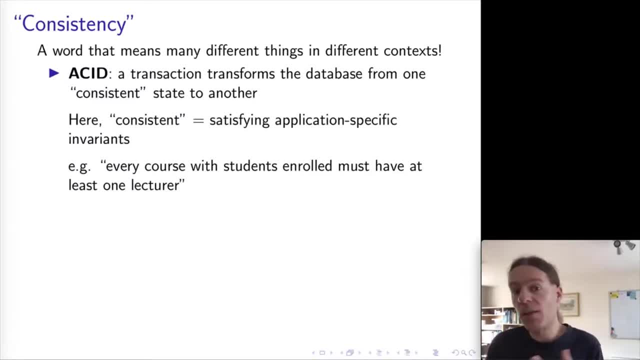 So here, consistent really means that the state of the database satisfies certain invariants or a certain consistency that the application has set. As one example, if you have a university database, you might have a consistency requirement that whenever a course has at least one student enrolled, 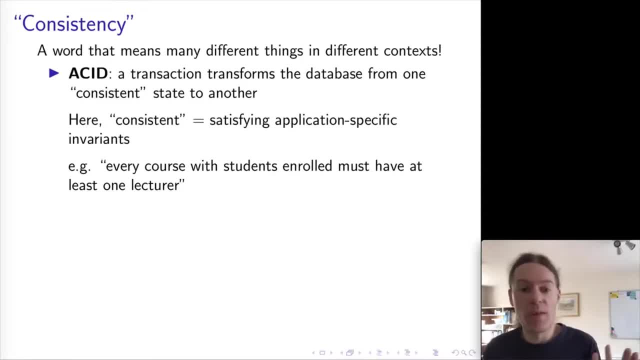 in it, then it must also have a lecturer, so it must not be without lecturer. For example, you could have those kinds of consistency properties, But this ACID consistency is not actually what we're usually talking about in distributed systems. We saw a different model of consistency a few lectures ago. 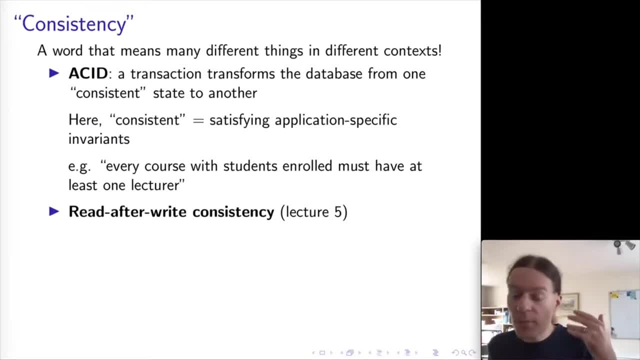 read after write consistency, which was that if a client makes a write and then reads back what it has just written, it should be able to see what it has just written. That has got nothing to do with the consistency in the sense of ACID. 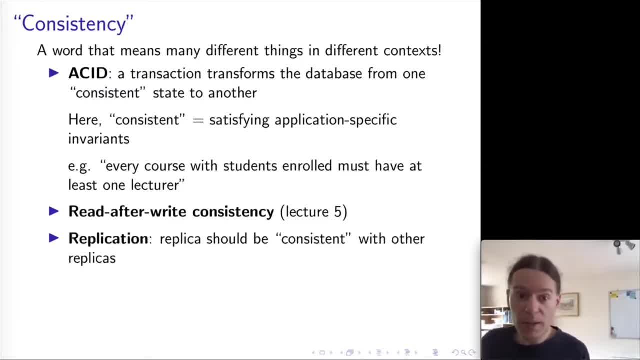 It's a very different meaning of the word. So, in the context of replication, what we often say is we want one replica to be consistent with another replica, which again raises the question of what exactly we mean. So does that mean the replicas are in the same state? 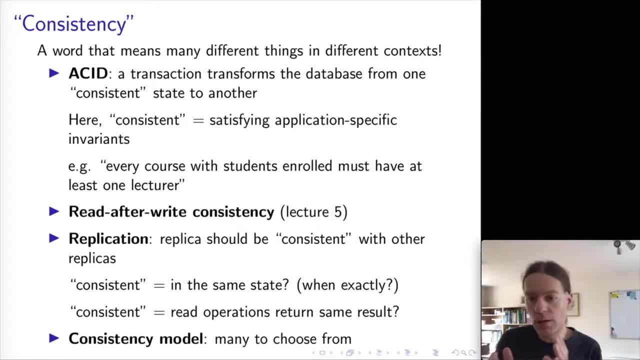 but when exactly do they have to be in the same states? They could be in the same state at different points in time, for example, or in different states at the same time. We could express consistency in terms of what the results of read operations should be, what we expect. 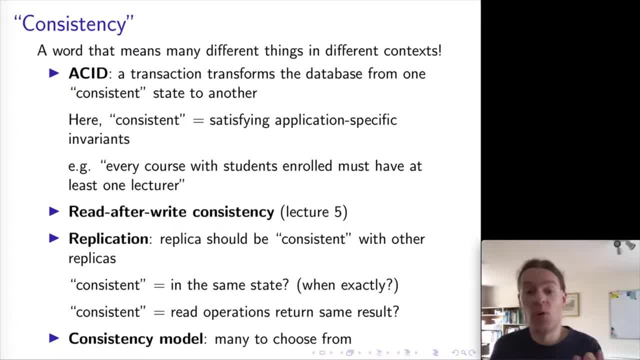 So I'm just saying here there are lots of different forms of consistency and no one true definition of consistency. There are, in fact, a whole bunch of different consistency models And in this lecture we're going to look at some of those consistency models and see the contexts. 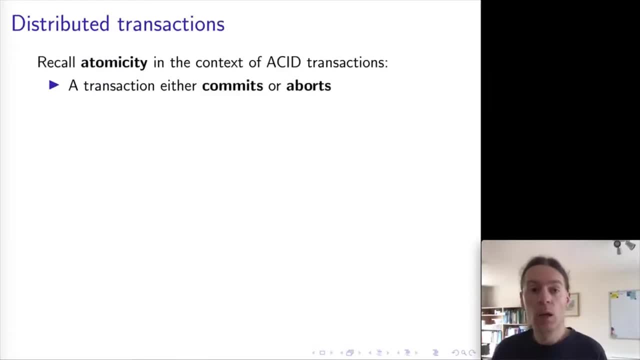 in which they are useful and how they are defined. So what I want to start with is distributed transactions. So you've covered transactions in the first half of this course on concurrent systems And if you recall the ACID properties- the A stands for atomicity. 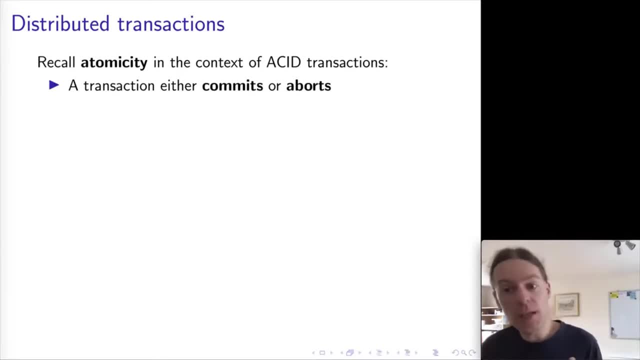 which means that if a transaction makes a bunch of updates to the database, then even if the database crashes or something goes wrong either, all of those updates are applied to the database and they are made durable, in which case the transaction is set to commit. 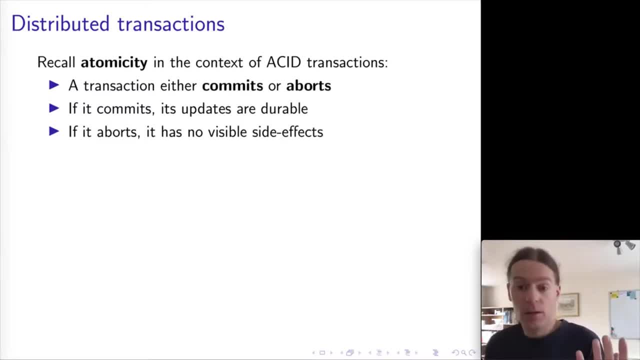 or all of the updates. none of the updates take effect, in which case the transaction is set to be aborted. So we have this kind of binary choice of a transaction: either it commits or it aborts. but we don't end up with this kind of half state. 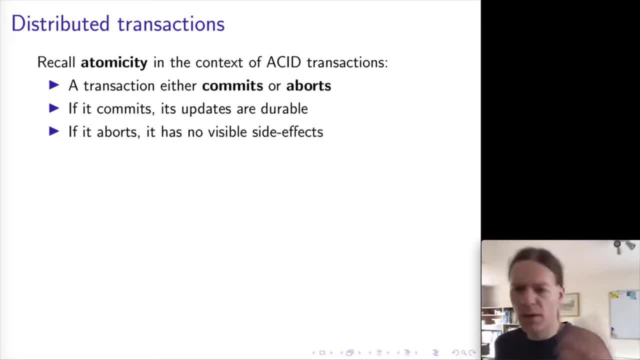 where some of the transactions updates have happened and others have not have happened. And this is very important, because if you want to ensure something like consistency in the sense of ACID, you do have to have atomicity as the foundation of that, because otherwise you could end up with two changes. 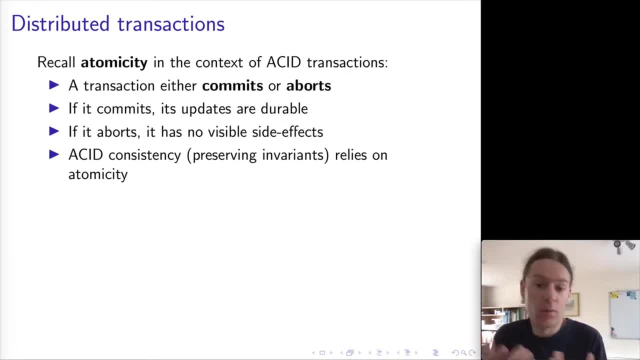 that need to be coordinated in some way, And if only one of the two happens, then you'll end up in an inconsistent state. So that's why we need atomicity Now. in a distributed system, we might have a transaction that involves more than one node. 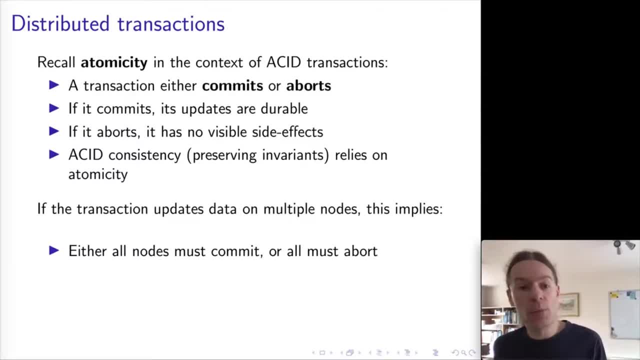 in a distributed database, for example, And in this type of system we have to ensure atomicity across all of the nodes that are participating in the transaction, So all of the nodes on which data is being read or written in the course of a transaction. 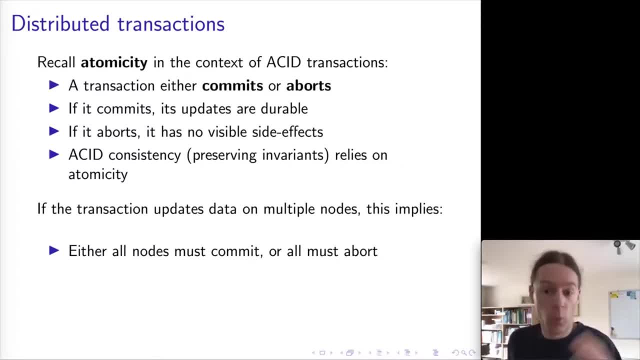 And so we must ensure that the transaction either commits on all of the nodes or it aborts on all of the nodes, So that would then give us atomicity for the transaction as a whole across all of the nodes. Moreover, if one of the nodes involved, 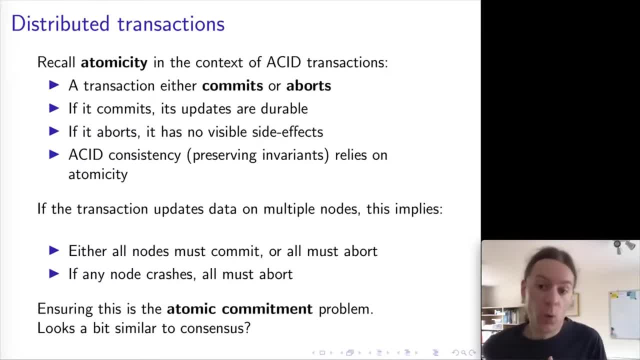 in the transaction crashes, then we also have to make sure that we abort the transaction on all other nodes, because the crash node cannot complete the transaction, It cannot commit the transaction, And this is known as the atomic commitment problem in distributed systems. So you might think 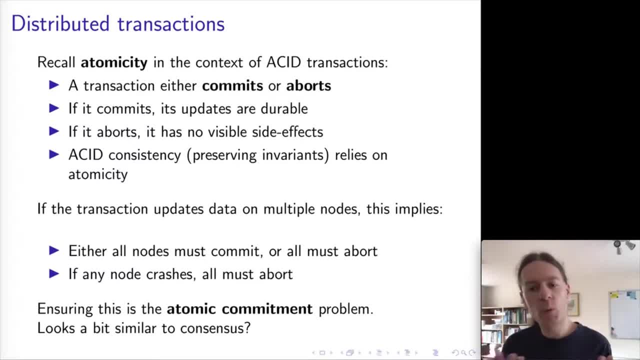 this looks kind of a bit similar to consensus, because what we want here is all of the nodes to agree on- whether to commit or abort the transaction, which kind of smells like consensus Now. yes, superficially, but if we look at it in more detail, 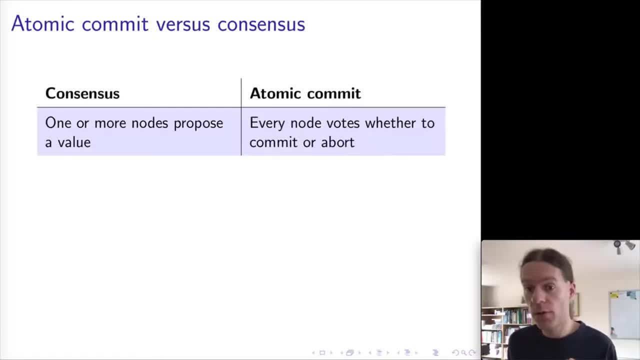 actually atomic commitment is quite different from consensus, And so let me just explain why. With consensus, the way I explained it previously was that you have multiple nodes, or one or more node may propose some value, And one of those values gets decided by the consensus algorithm. 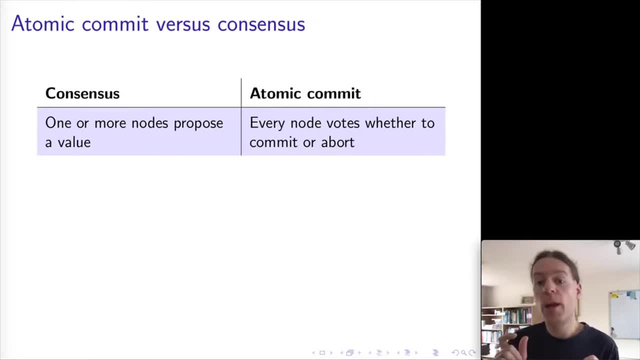 Whereas in atomic commit we're a bit more constrained. We have to have all of the nodes voting on whether they are able to commit a transaction or not, And we have to take all of those votes into account. So while in consensus it's okay to simply pick any one of the values. 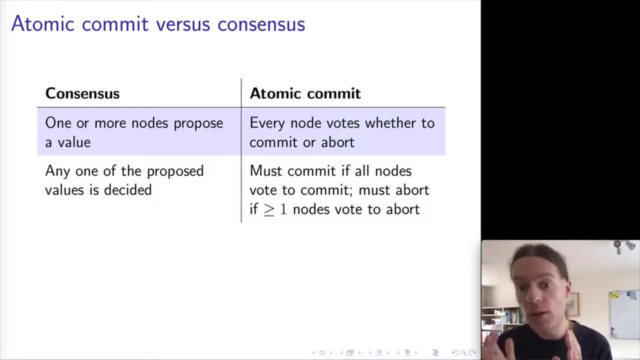 that has been proposed. In atomic commit it's very clearly defined what must happen. If all of the nodes vote to commit, then the transaction must commit. If any one of the nodes votes to abort, then all of them must abort. So atomic commit is much more constrained. 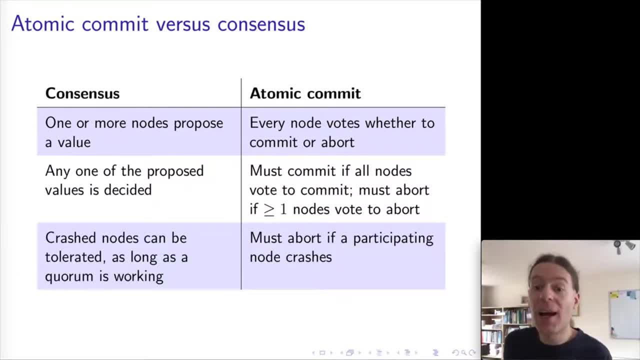 in the decision that the algorithm has to make And finally, with consensus, we've seen that we can have algorithms like Raft, which can continue working as long as a quorum of nodes is reachable and responding to requests, Whereas with Atomic Commit, 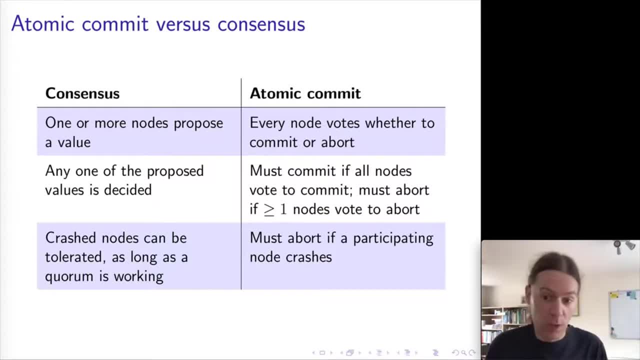 because we have this requirement that all of the nodes must vote and we must get consensus across all of them. this means now that even just one single node crash will cause the entire transaction to abort. So Atomic Commit is not able to tolerate any faulty nodes. 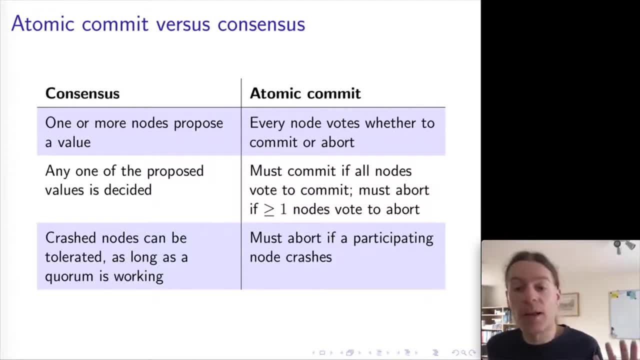 whereas a consensus algorithm, a fault-tolerant consensus algorithm like Raft is able to tolerate a minority of faulty nodes in the system. So this is Atomic Commitment, and the way we typically implement Atomic Commit is using an algorithm called Two-Phase Commit. 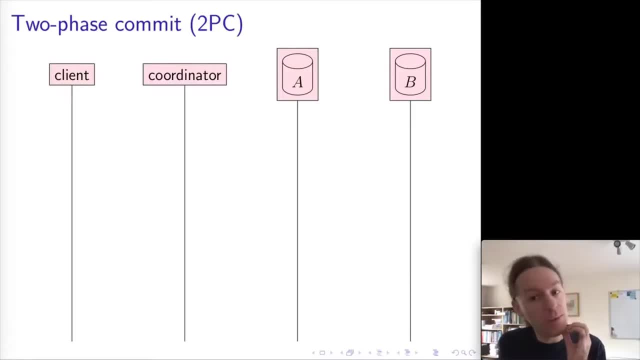 Now Two-Phase Commit sounds a bit like Two-Phase Locking which you've seen previously. Don't confuse the two. they sound very similar but they're very different things. So Two-Phase Locking is around serializable isolation. 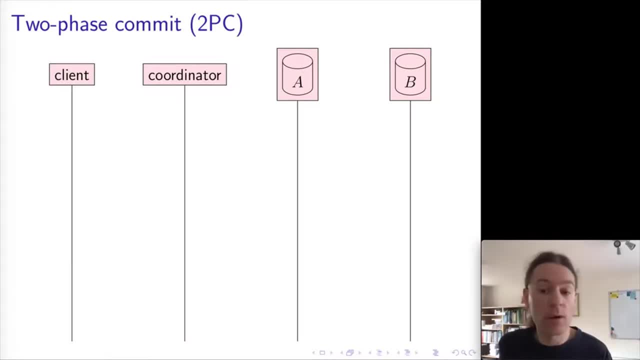 whereas Two-Phase Commit is around getting atomicity very different area. So the way we start Two-Phase Commit is that the client wants to open a transaction, begin a transaction on multiple database nodes and it just starts a transaction as usual. 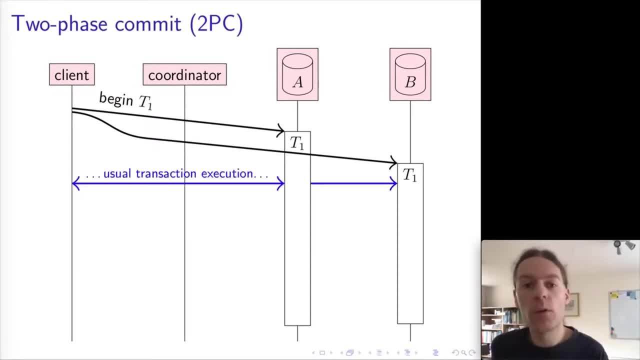 sends some transaction identifier T1 to those nodes and then does its usual thing. So the transaction may read and write arbitrary objects in the database and do whatever it needs. to do any kind of logic Two-Phase Commit only starts when we're ready to commit the transaction. 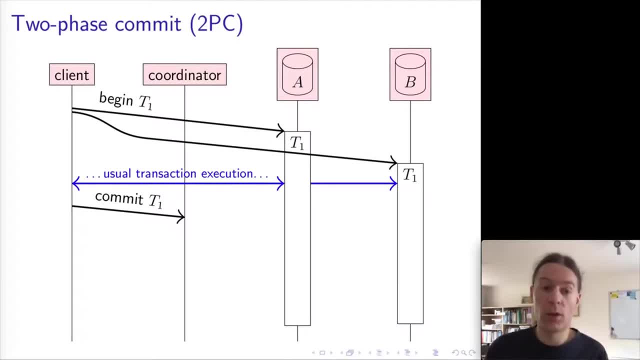 So, rather than the usual form of transaction commits where the client just sends directly to the database, hey, commit now please, With Two-Phase Commit instead, the request to commit goes to a new node in the system called the Transaction Coordinator. 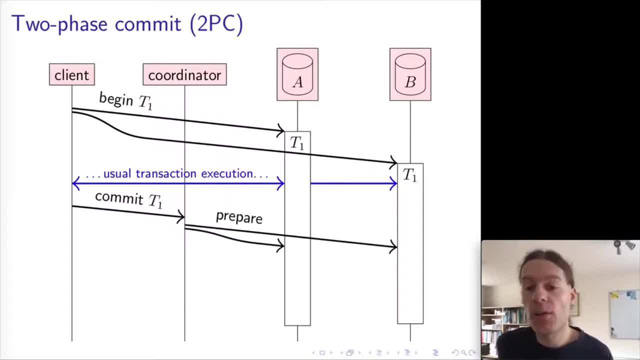 So this commit request goes to the coordinator and the coordinator then sends a prepare message to all of the database nodes that are participating in the transaction. And the purpose of the prepare message is it's kind of like commit, except it doesn't actually finish the transaction yet. 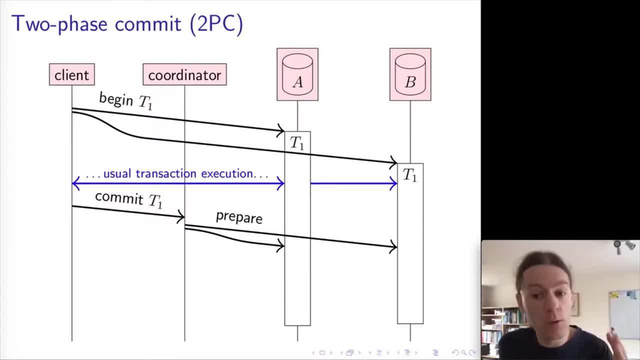 So what prepare does is when a database node receives the prepare message, the database node has to write all of the changes, all of the updates from that transaction to disk and it has to check any constraints to make sure that we have consistency of the database. 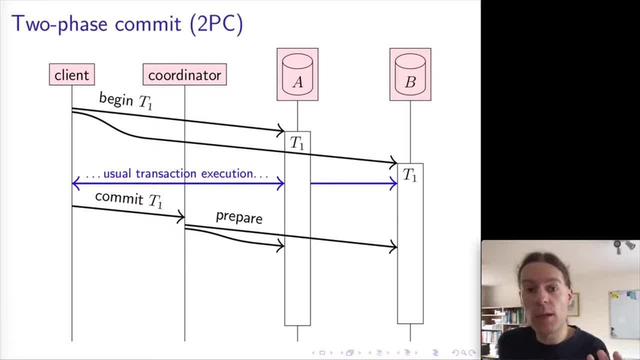 Because, in response to that prepare message, the database node now has to reply with either yes or no, whether it's willing to commit that transaction or not, And so, as we said, any one node response to this will cause the transaction to abort. 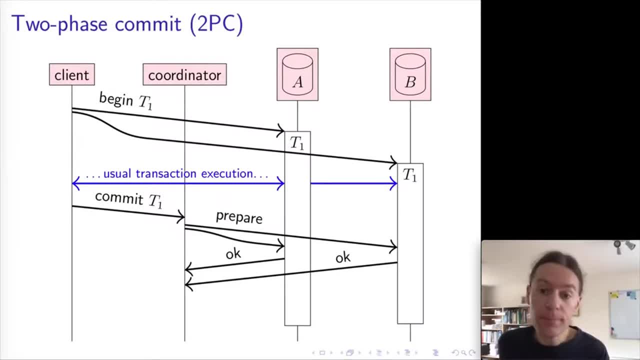 but if all of them vote yes, then the transaction will commit. So this means that once the database node replies saying okay, I'm happy to commit this transaction, it is promising that it will definitely be able to commit that transaction in the future. 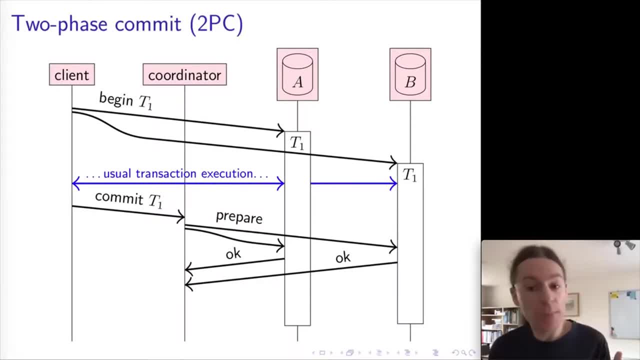 Because there's at this point the database node has abdicated its responsibility. Now it's up to the transaction coordinator to make the decision whether or not to commit the transaction. So the database node just has to promise that if it is asked later by the coordinator. 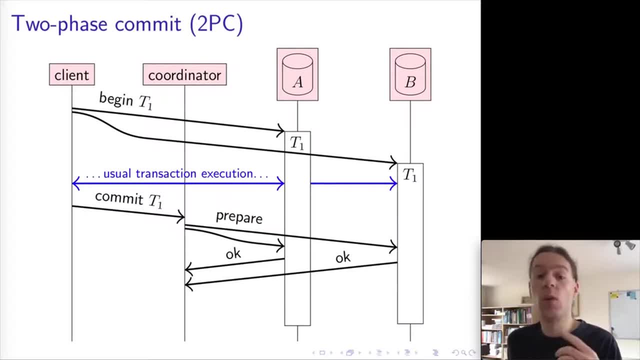 to commit the transaction. it will definitely be able to commit it. So it's not allowed to back out and flake out afterwards and say, oh sorry, I didn't want to commit this after all, because by that point it's too late. 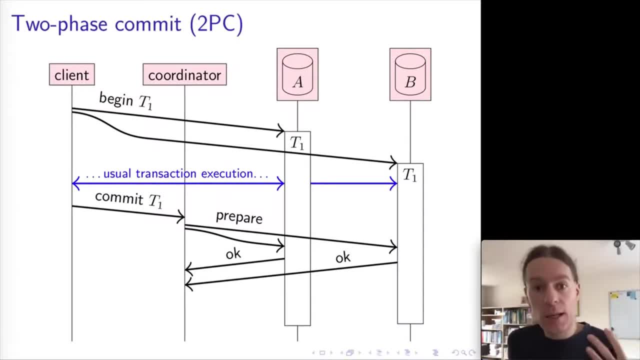 So by the time that the prepare message is telling the database nodes that it must get everything ready to be able to commit, but without actually ending the transaction yet. And then if the coordinator says in phase two of two-phase commit, if the coordinator says, okay, now we're going to commit, 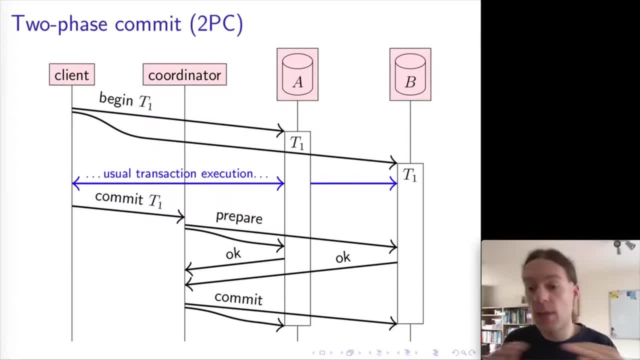 then the individual database nodes go, they do the actual commit, they end the transaction, they release all of the locks and everything is done. So this is the the model of two-phase commit, And the key moment in this protocol is here. 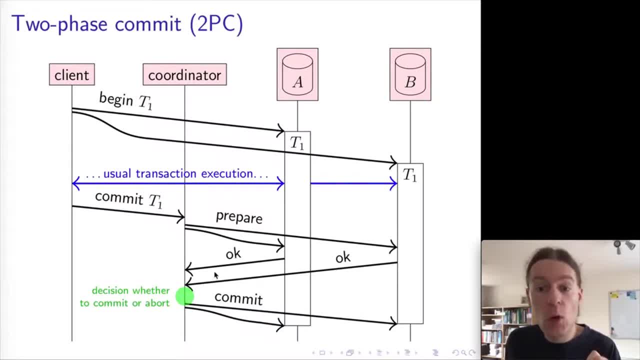 So, after the database nodes, the participating nodes have replied to the coordinator saying whether or not they're willing to commit this transaction. At this point the coordinator makes the decision whether to commit or abort, And this is really a key moment in the protocol. 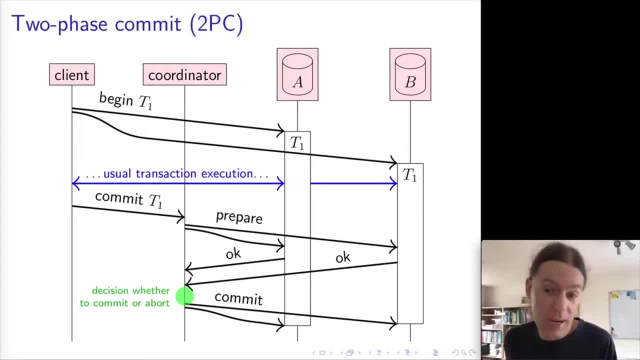 Now we can think about what happens if some of these nodes crash. So if the database node crashes, then we've discussed that- that means the transaction coordinator will timeout and it will say: okay, we're going to abort the transaction for everyone. 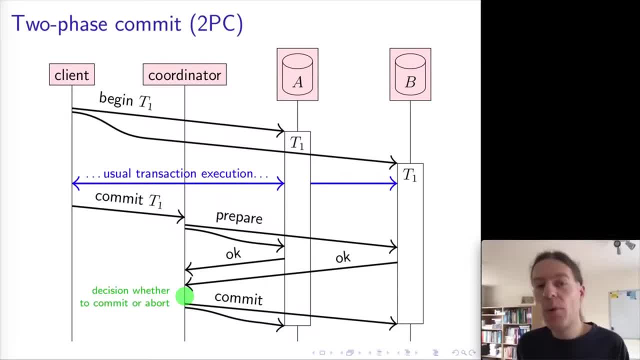 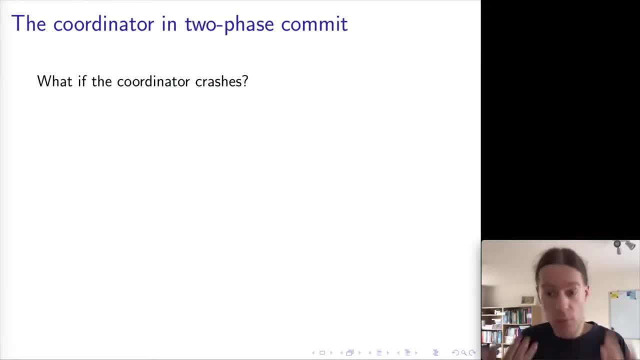 So that's fine. The question is: what happens if the coordinator crashes? So if the coordinator crashes, well, first of all it has to make this decision on whether to abort or commit the transaction. So it can write that decision to disk. 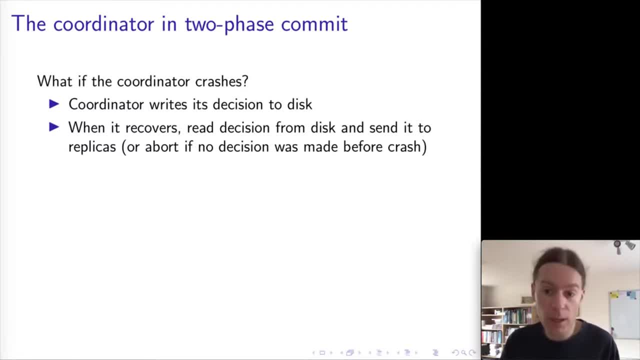 And so then, when the coordinator recovers from its crash and starts back up again, it can read this decision from disk and send the decision that it made to the replicas that were participating in the transaction, Or, if there was no decision record on disk. 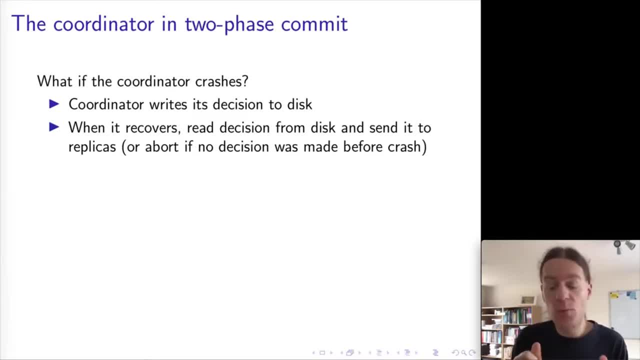 then the coordinator can just abort. But it has to be even if the coordinator crashes. if it made the decision before the crash to commit, then it must honor that decision after it restarts, because it might have already sent the commit message to some of the nodes but not all of them. 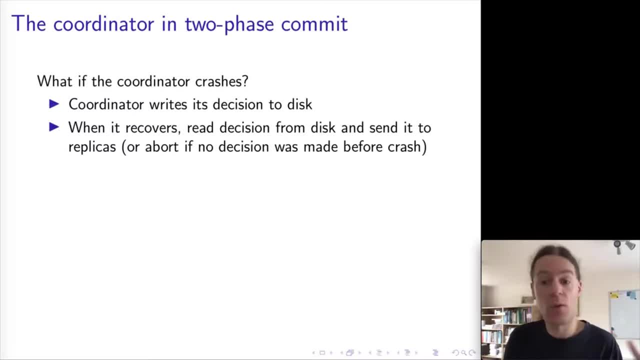 And so some of the nodes may have already committed and released all of their locks. So now we have to ensure that everybody else commits as well, And likewise, if one aborts, then all of the others have to abort as well. But this leaves us in a problem. 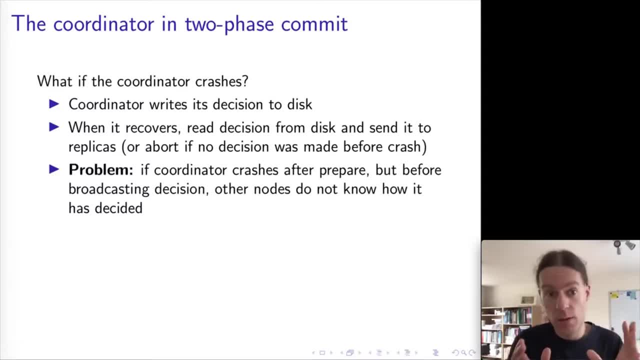 because the coordinator is now this linchpin in this protocol. because if the coordinator crashes just at the moment after the prepare requests have been sent out, but before the coordinator has sent out its decision on whether to commit or abort the transaction, then all of the other nodes don't know what the coordinator is doing. 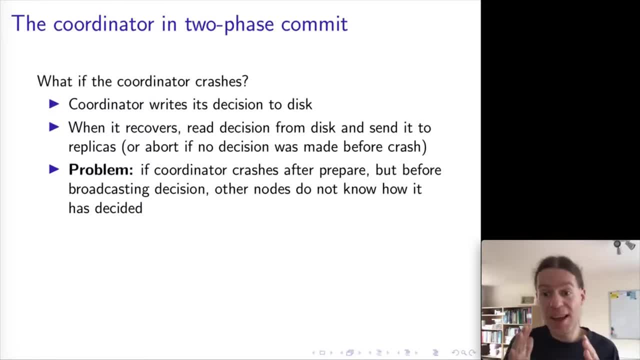 And so the coordinator has decided they are simply stuck. They cannot end their transaction. yet They can't abort their transaction because, as I said earlier, they have promised that they will be able to commit it. So if they abort it, then they wouldn't be able to commit it anymore. 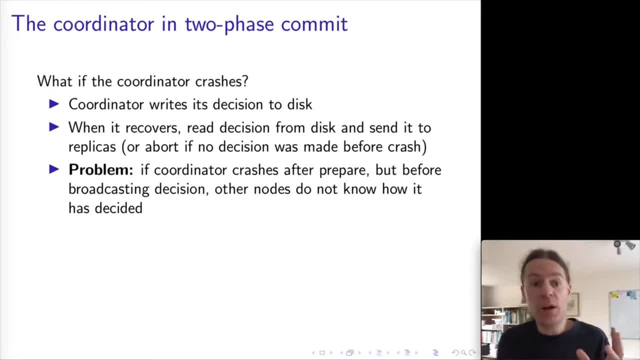 So they can't commit or abort their transaction. They're all stuck in this state of being uncertain of what the state of the transaction is, And so the individual nodes can't just decide for themselves to abort or commit, because that would risk violating atomicity. 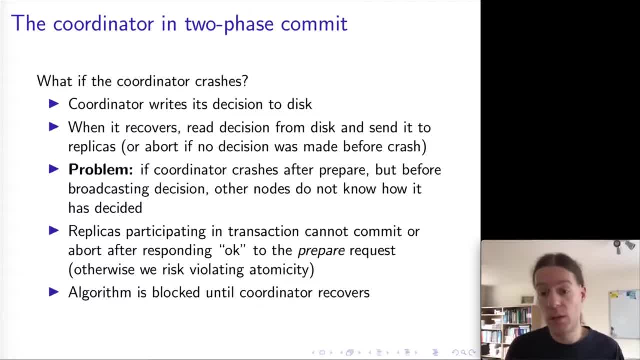 So the entire algorithm is blocked until the coordinator restarts and recovers its state from disk. So this is not great, because if a coordinator crashes it might take a while to come back up again If the machine where the coordinator was running on experienced a hardware failure. 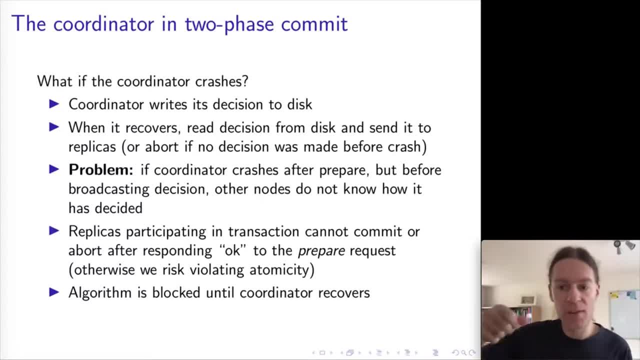 it's even worse because somebody has to go and take the hard disk out of that machine and put it into a new machine and so on. So the whole system could be down and locked up for quite a significant amount of time. Fortunately, there is a way around this. 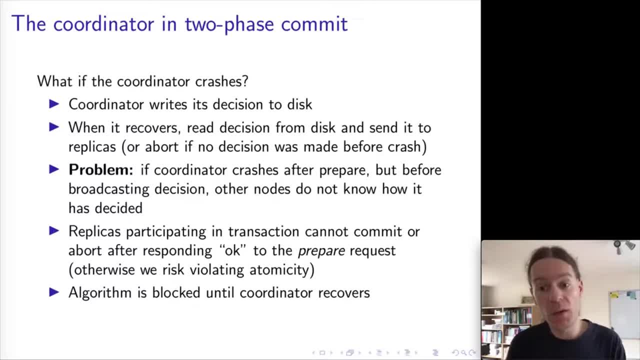 And there is an algorithm, a variant of two-phase commit that is fault tolerant And it relies on what we talked about in the last lecture on total order broadcast, ie a consensus algorithm, And it works like this. This algorithm is just two slides long. 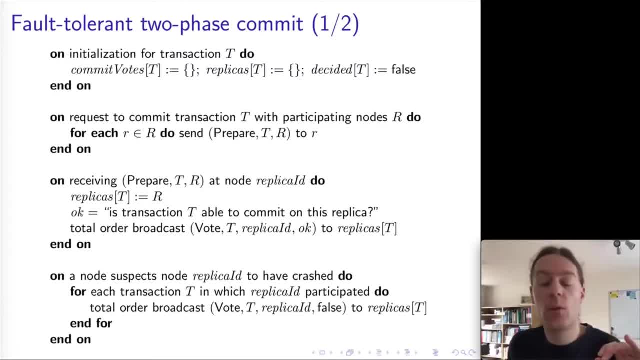 And the idea here is that we use a total order broadcast algorithm to disseminate each node's vote on whether to abort or to commit, And so for each node we're going to have some state here. So for each transaction we're going to have a set. 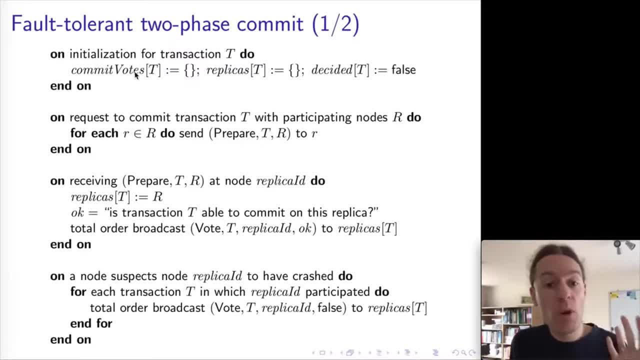 containing the replica IDs that have voted in favor of committing a certain transaction. We have the set of all of the replicas that are participating in a certain transaction And for each transaction, we have a flag telling us whether we have decided yet or not. 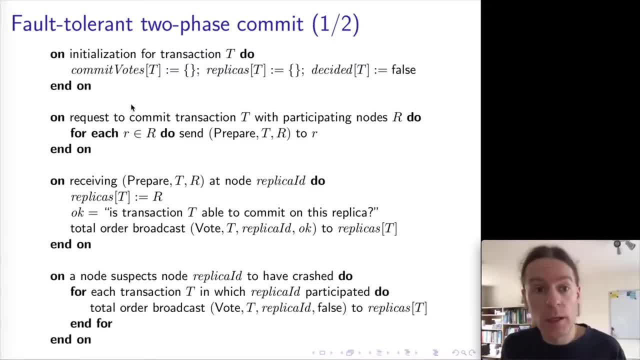 And so now, when we want to commit a transaction, we do the same as we do usually the coordinator, what the coordinator would usually do, which is it just sends a prepare message to all of the nodes participating in the transaction. okay, That's just the regular prepare message, as before. 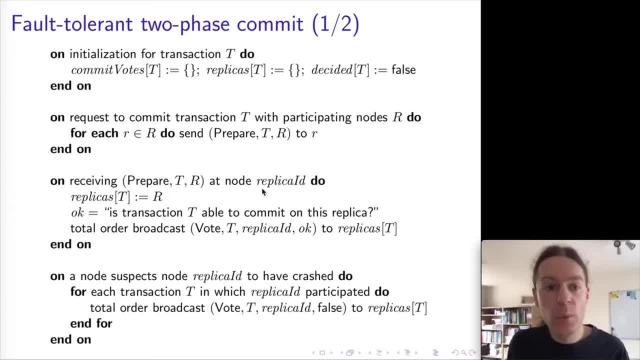 When a node or a replica receives this prepare message, it's now okay. it now knows the set of replicas that are participating in this transaction called R, So it remembers that This is the set of replicas participating in transaction T. And now okay. 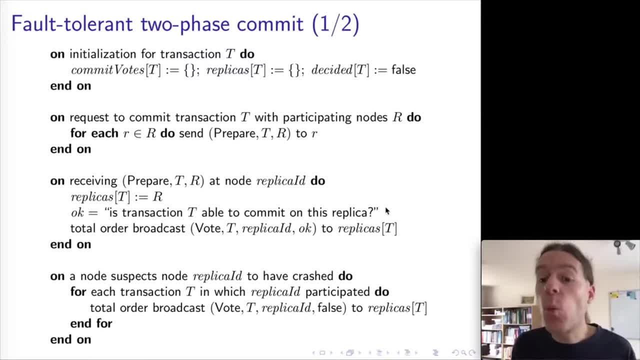 now as before, the replica needs to check whether it is able to commit the transaction and it will reply to the prepare request saying either yes or no. and if it says yes, it promises that we'll definitely be able to commit this transaction in the future. so this okay, will simply be a. 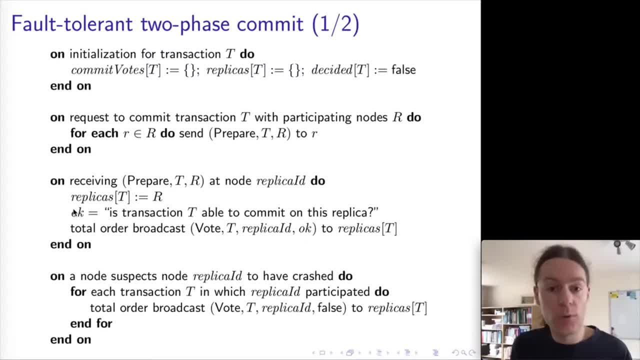 boolean here, saying true or false, whether it is able to commit the transaction or not. and now, rather than sending this vote back to the coordinator, we use total order broadcast to send this vote to all of the replicas that are participating in this transaction. so now all of the replicas find out about each other, of who is able to commit what. 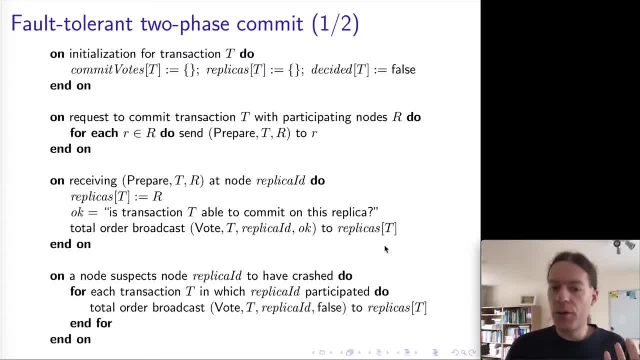 and this gets us most of the way there. the question is just what if one of these replicas has crashed? and so if that replica has crashed, then it is not able to broadcast its vote, so all of the others would be stuck waiting forever until this vote never turns up. so what we have in 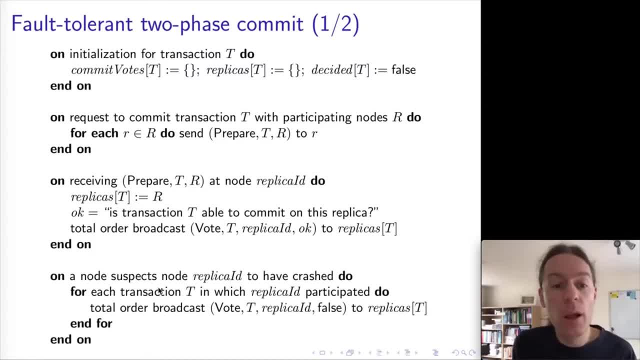 addition is a failure detector and this failure detector, this, this can be running on any node, for example on some of the other database replicas or even on the client, and it just checks whether it suspects any of the replicas to have failed. so if it has sent the prepare request to some replica and the 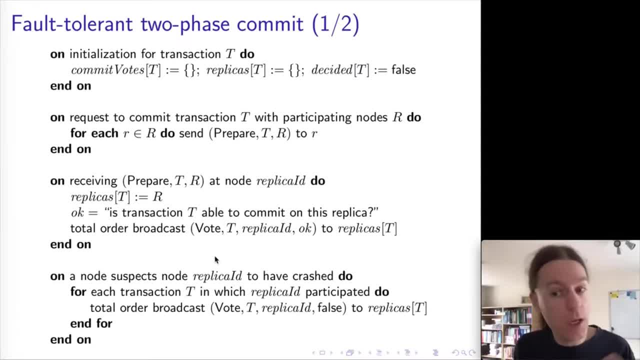 replica has not broadcast its vote yet. after some amount of time, some time out, then this other node is just going to broadcast a vote on behalf of the replica that it has suspected to have failed, and it just votes false. so it votes to abort on behalf of this replica. now what could happen? 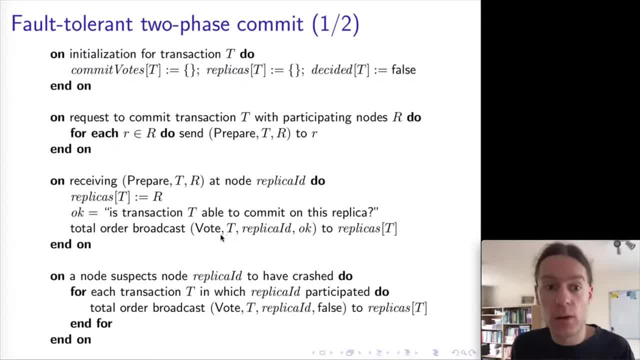 as you can see here, is that actually? it could be that the replica here that is suspected to have crashed hasn't actually crashed. it might be fine, it might just be a bit slow, and so it could be that just around about the same time, we get two conflicting votes for the same replica. that is one. 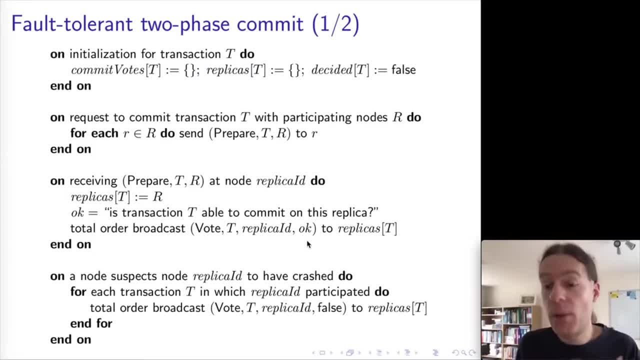 genuine vote from the replica that the replica itself is sending and one vote, or maybe even several votes, from other replicas who think this particular node has failed. and so now we are relying on the property of total order broadcast, which is all of the participants, all of the nodes in the system will deliver the same messages in the same order. 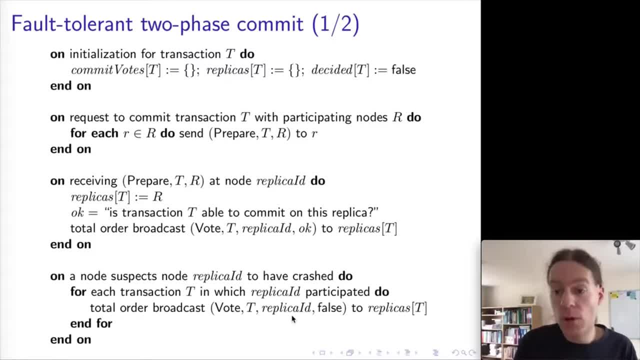 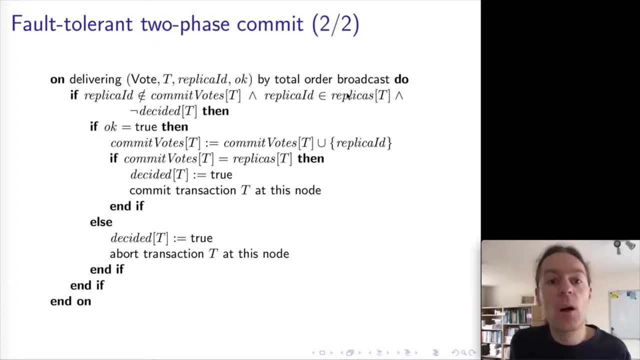 and because of that, this race between the different votes for the same replica is no longer a problem, because we can ensure that the first vote that we see from a given replica will be the same for all of the nodes, and so this means here whenever we deliver one. 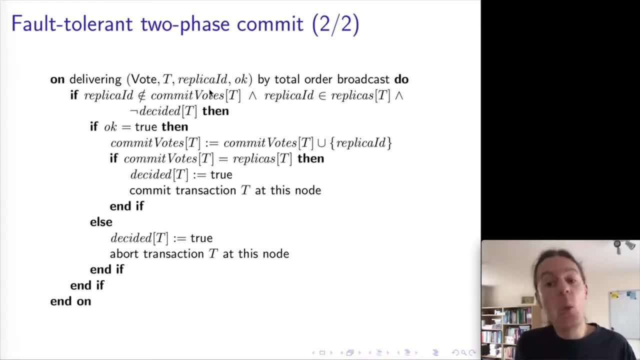 of these votes here by total order broadcast, we can just consider the first vote from any given replica and ignore any future votes, and this will ensure that all of the nodes then come to the same decision as to whether to abort or commit the transaction. so first of all here: 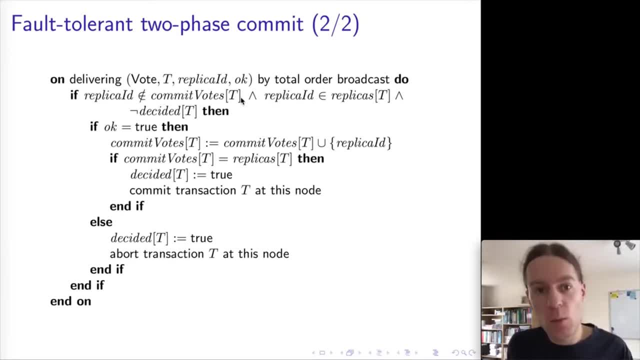 if the replica that is voting is not already one of the the votes that has committed, and if the replica is one of the replicas in the transaction T and we have not already made a decision for transaction T, then well, okay, it depends. 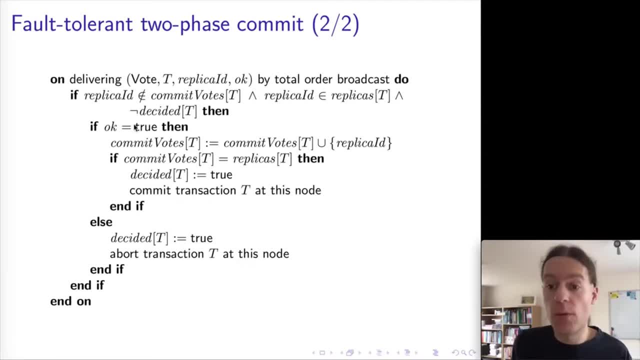 whether we voted in favor or not. So if we voted true, which means vote in favor of committing, then we add the replica ID to the set of replicas that have voted in favor of committing this particular transaction, And if the set of replicas that have voted in favor 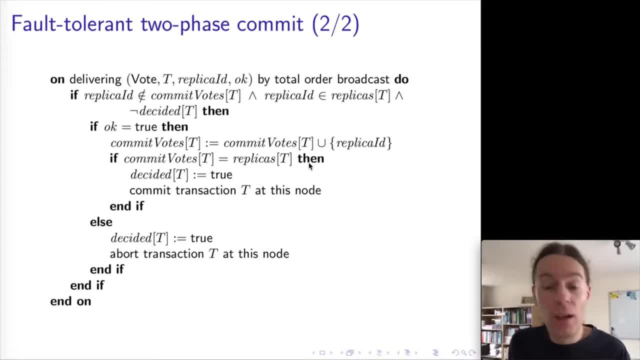 equals the sets of all replicas participating in the transaction. that means now we have the unanimity that we require, we can decide to commit the transaction and do the actual commit at this node. On the other hand, if the vote was false, it was in against committing. 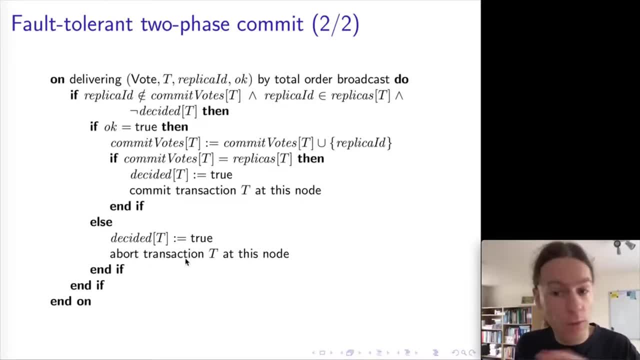 that means we can immediately abort, because one single vote against is already enough to scupper the whole transaction. We can set our flag to be decided to be true and then we're going to abort the transaction at this node. And if you think about this, 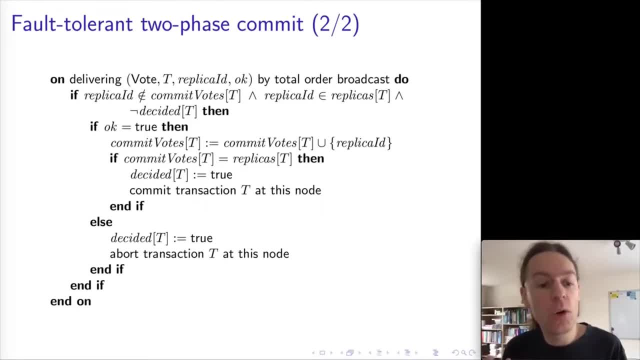 the logic that we have here ensures that we only count the first vote from any given replica And, because all of the nodes will agree when they're delivering these votes, they will agree on which the first vote was from a given replica. this will ensure that all of the participants see the same. 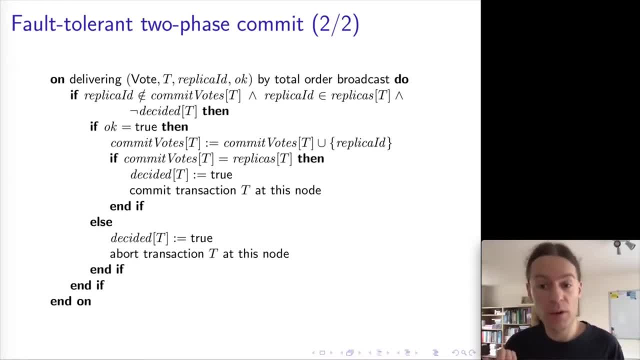 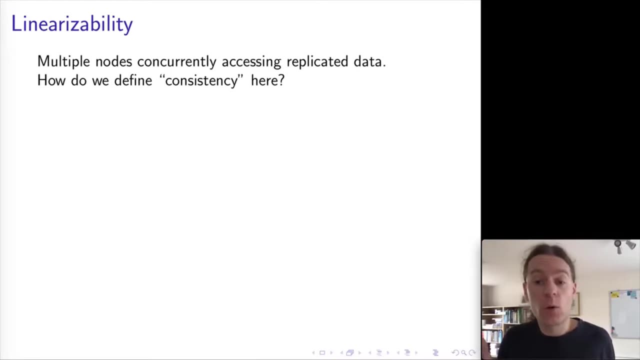 and come to the same decision as to whether to commit or abort this transaction. Isn't that nice. We have this total order broadcast algorithm and we can use it to solve this quite different problem in a reasonably simple way. I would now like to talk about a consistency model. 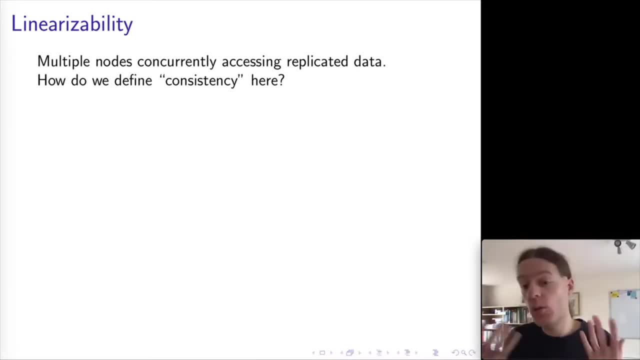 called linearizability. So what we've seen so far with two-phase commit and atomic commitment is ensuring consistency in the face of crashes, So ensuring that even if nodes crash, all of the nodes will either commit or abort a transaction. But we also have to worry about consistency. 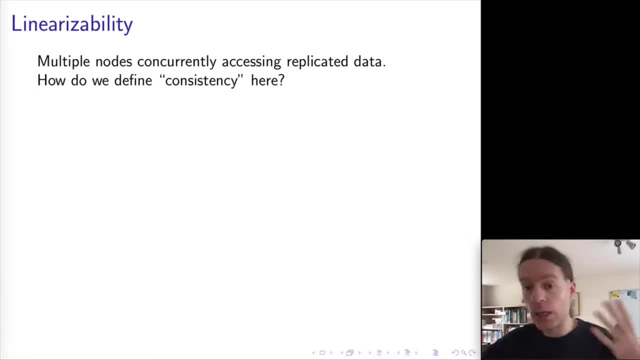 in the face of concurrency. So what if multiple nodes are concurrently reading and writing some data? how do we ensure those operations are consistent with each other? for some definition of consistency- And this is what linearizability is about- So it's one particular definition of consistency. 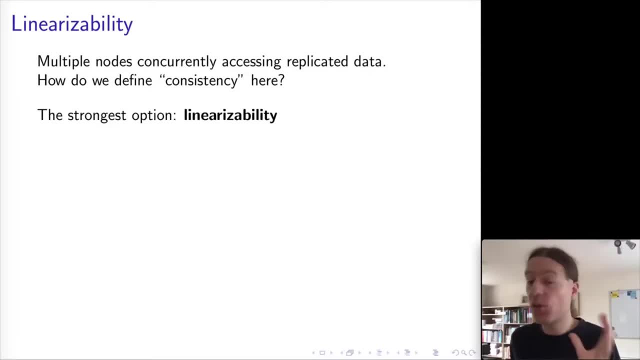 for concurrent systems, And it is the strongest such model that is in widespread use. And the idea behind linearizability is that the system as a whole behaves as if it was not replicated or distributed at all, So it behaves as if there was actually. 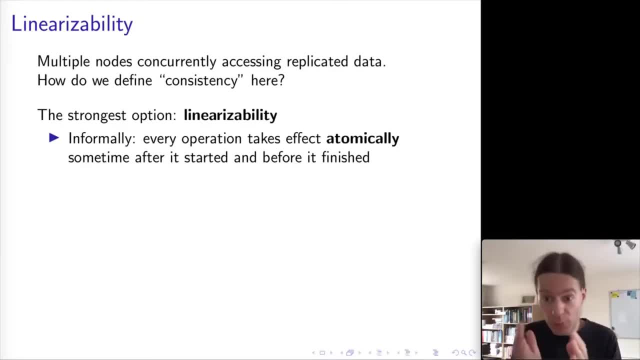 only a single copy of the data and all of the operations happen atomically on that single copy of the data. So when you issue a read or write operation, that operation will take effect atomically at some point in time And even though there might be multiple replicas. 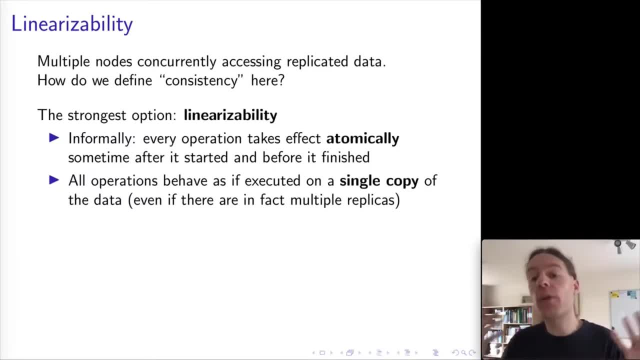 in the system. from the point of view of the client, it looks as though there was only a single copy of the data. And so this is very nice because it's easy to program against. And so this is very nice because it's easy to program against. 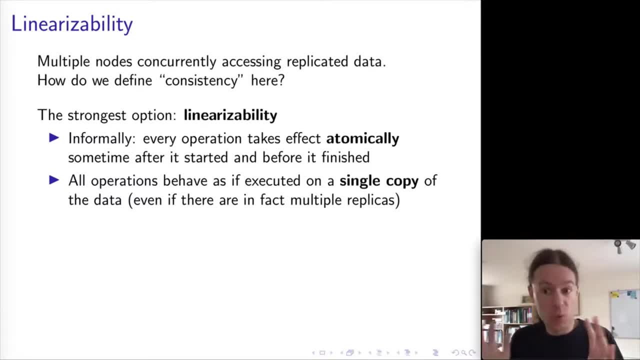 And so this is very nice because it's easy to program against, And so this is very nice because it kind of reduces all of the distributed system's complexity down to something which is very nice and manageable and small, like a single copy of the data. 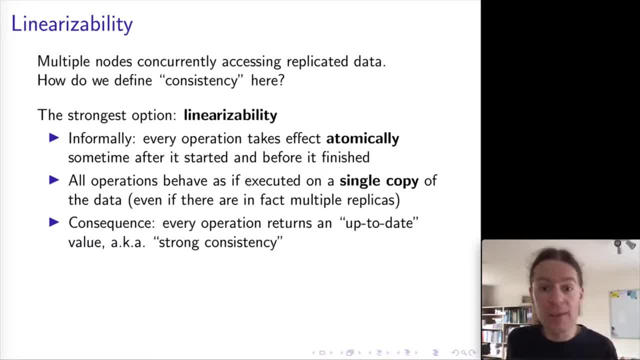 A consequence of this definition of linearizability is that whenever you read some data, you're guaranteed to get an up-to-date value for some definition of up-to-date that we will see in a moment, And this is sometimes also called strong consistency. 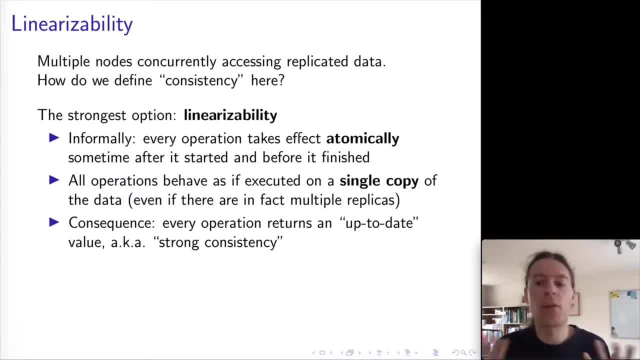 But the term strong consistency is a bit poorly defined. But the term strong consistency is a bit poorly defined. It's a bit vague and hand-wavy. So we're going to stick with linearizability, which is formally defined. We will not go into the exact formal definition in this course. 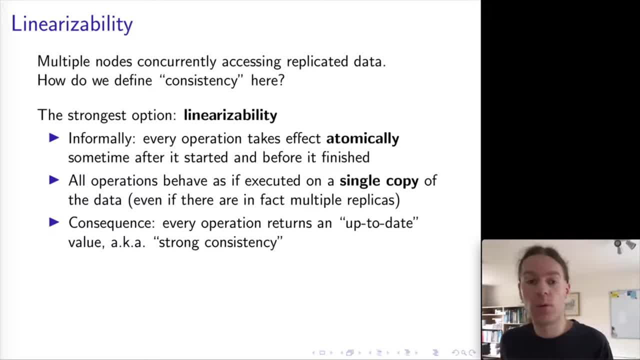 I'm just going to give you the intuition behind linearizability through some examples. Interestingly, linearizability is not only important in distributed systems, but it actually is used also in the context of shared memory concurrency on a single computer, And the reason there is that if you have multiple CPU cores, 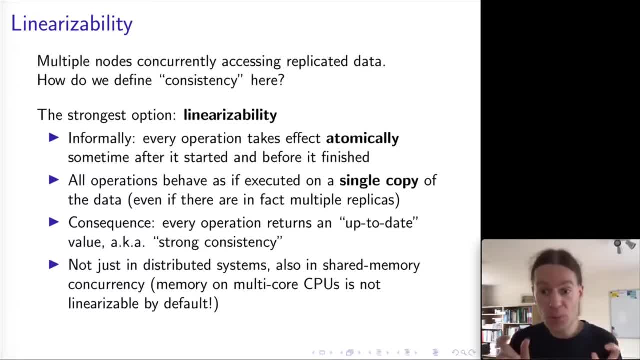 then actually each CPU core has its own memory caches And if you have threads running on two different CPU cores, you might have one thread writing a value to memory which actually goes to its cache, and then a different thread reading that same location. 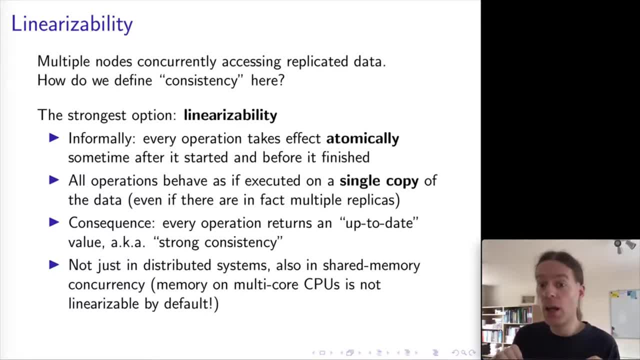 in memory and it might not see the value that was written by the first thread because its cache hasn't yet been updated with that value, And so you get actually within the scope of a single computer. you get this similar kind of behavior. 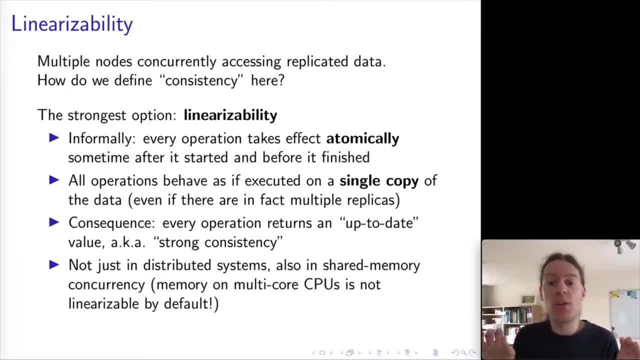 as in a replicated system, because these different, different levels of caches gives you, give you something quite like a replication. I think this is interesting because you know we are taking now the, this idea from distributed systems and a single computer starts actually behaving. 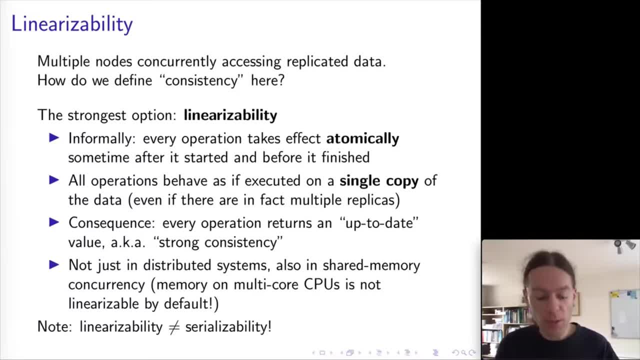 a little bit like a distributed system too. Another piece of terminology just to be careful of is linearizability and serializability are not the same thing, even though the words look kind of similar but they mean totally different things. So serializability. 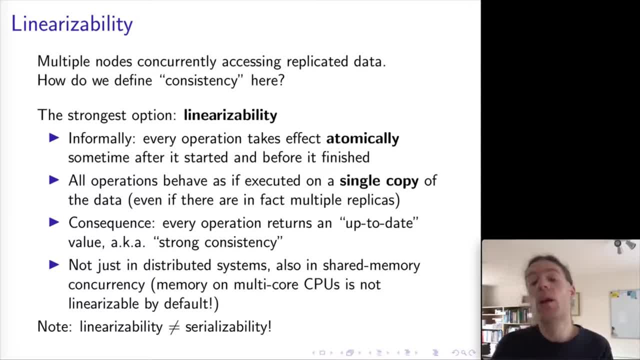 is a form of isolation between transactions. It's about transactions having the same effect as if they were executed in some serial order. Linearizability is around multiple replicas behaving as if there was a single replica. So they're very different things, Okay. so in order to give you a sense, 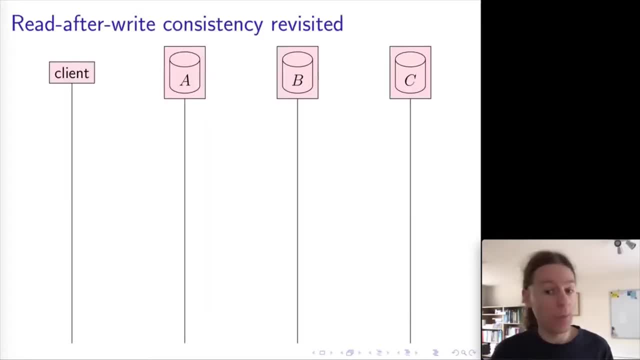 of what linearizability means. I'm going to go back to something we saw in a previous lecture, which is read after write consistency. So if you remember what we discussed back then, this was in the context of read and write quorums. 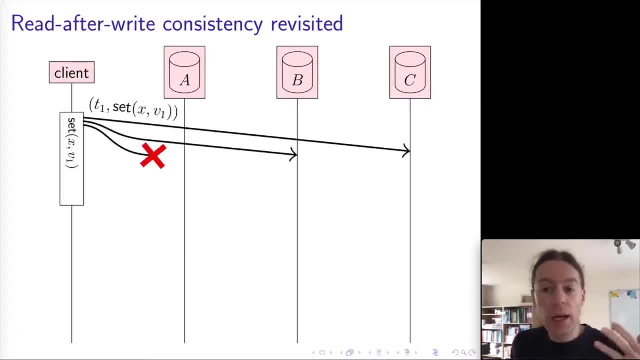 So if you have a client that wants to write some value V1 to some object X, it can make this write request to a quorum of replicas. If a quorum responds okay, then this set request is successful And then subsequently that same client. 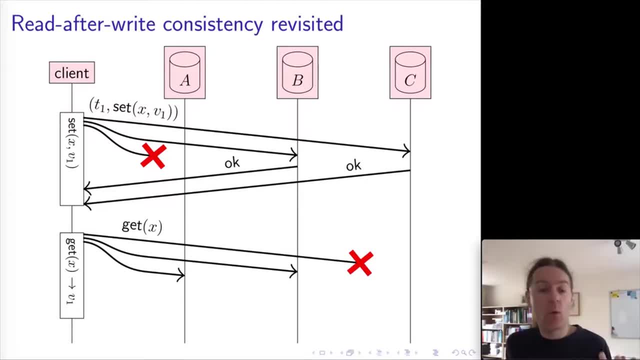 might make a get request and send that get request. get request to a quorum of replicas. get some responses back. use the timestamps to figure out which is the more recent value in the responses and return that value from the get request. So what is new here in this notation is now: 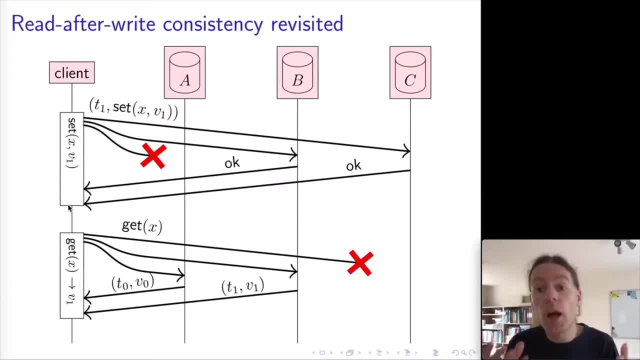 I've got these boxes which indicate the execution time of this particular operation. So when the operation begins we start by sending out these requests And then, after a quorum of responses have been received, we declare the operation to be finished. So the box here, this rectangle, shows the duration. 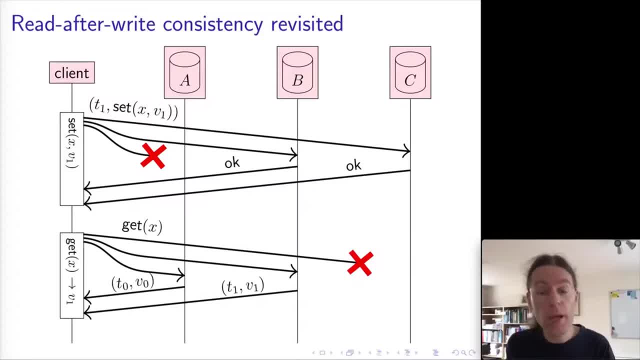 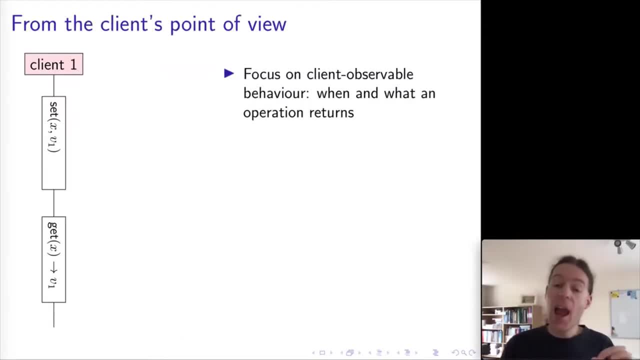 of the operation And then we can define the consistency model purely from the client's point of view. Now we can actually abstract away all of the internals and this message, communication on all of the replicas, And we can define a consistency model purely in terms. 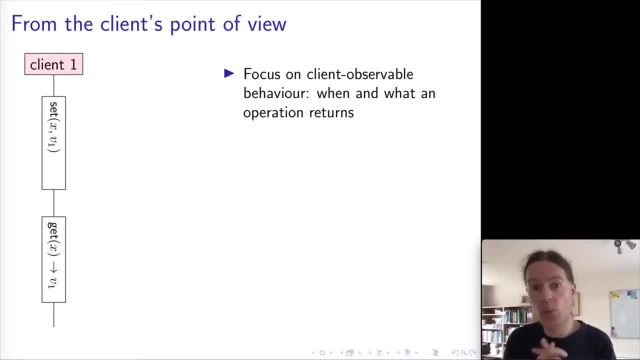 of what the client sees. So, looking at things only from the client's point of view, And this is useful because it means we, our consistency model, is now not tied to one particular implementation of a system or one particular distributed algorithm. We can define the behavior only from the client's point of view. 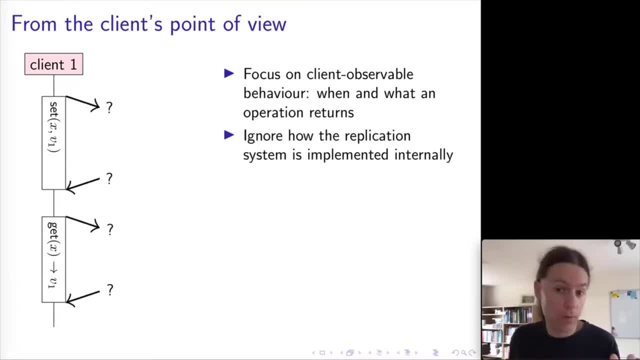 regardless of how the internals of this system are implemented, And so within the execution of each operation, there might be multiple messages sent and received, and we don't care particularly what those messages are. exactly What we do care about here is that this get operation here. 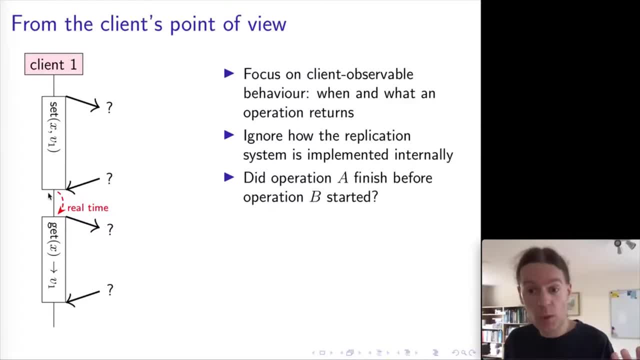 started after the set operation finished. So there's this time dependence here that the get operation happened later in time than the set operation, And therefore we would expect the get operation to see a value of X that is at least as recent as the value that was written by the previous set operation. 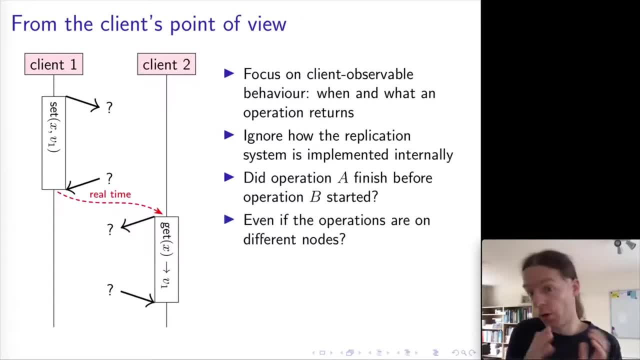 And we can generalize this timing dependency to be not just on a single node but actually across multiple nodes, So we could have the client, client two here, which starts a get operation sometime later in time, after the set operation by a different client has completed. 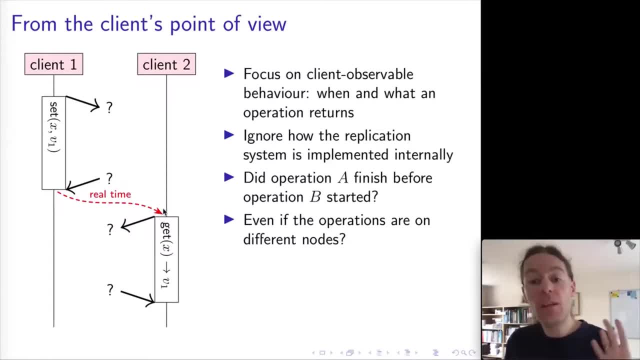 And again we have this real-time dependency here. So linear under linearizability, we expect that this client two will also see the up-to-date value V1, because that's the behavior we would get if we have a single copy of the data. 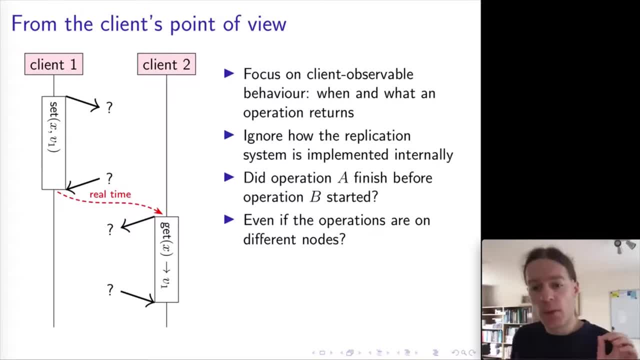 on which all of the operations are atomic. Now this timing dependency: here it looks like the happens before relationship, but it is not the same as happens before, as we discussed in previous lectures. So, if you remember, the way happens before is defined. 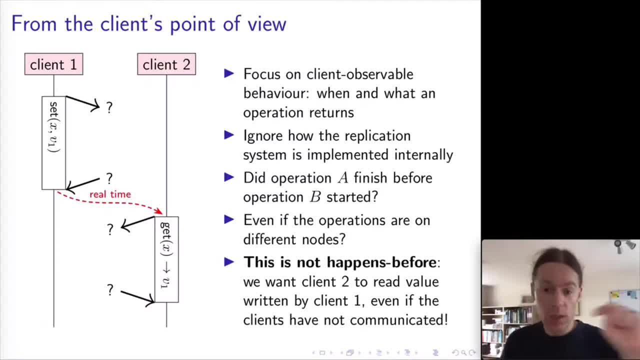 is. it's defined in terms of sending and receiving messages. So it's: if there is some path through our message send and receive graph so that you can get from one event to the other event, then we have that one event happens before the other event. 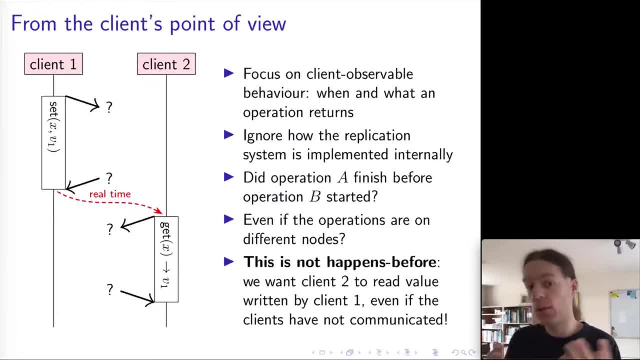 So happens before, is not defined in terms of real-time. it's defined in terms of message sending and receiving, Whereas linearizability is defined in terms of real-time. So we are assuming if there's some hypothetical observer who can see exactly when which operation finished. 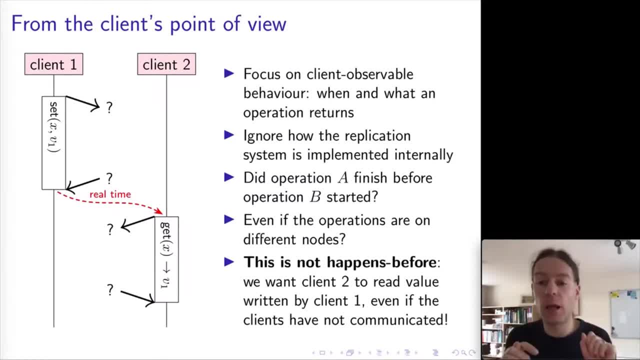 and when which operation started. this observer can tell us whether a certain operation started after another operation finished and therefore it should be able to observe its operations, its up-to-date state, And we have that dependency even if those nodes did not communicate. 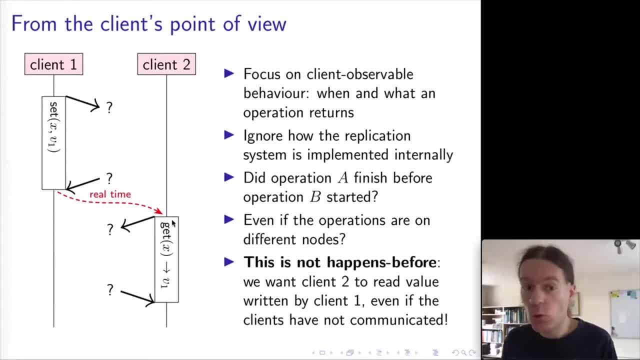 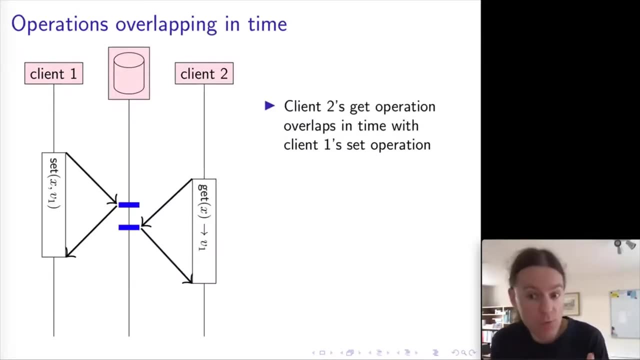 So even here client one might not send a message to client two at all, but nevertheless we have this real-time timing dependency between the two operations, because this operation by client two definitely happened later in time than client one's operation, And if the two operations overlap in real-time, 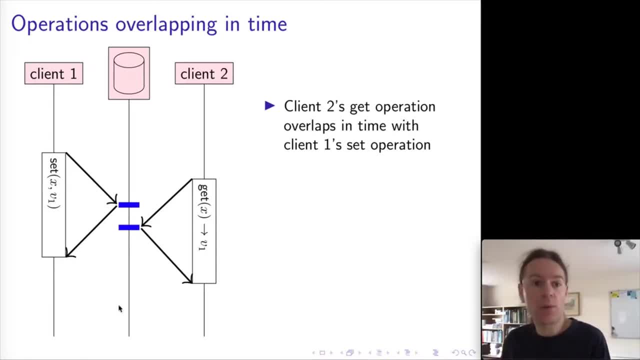 then they can take effect in either order. So in this case here, for example, we might have the set operation taking effect first and then the get operation taking effect second, in which case the get operation will return the value v1,. but it could just as well be the other way around. 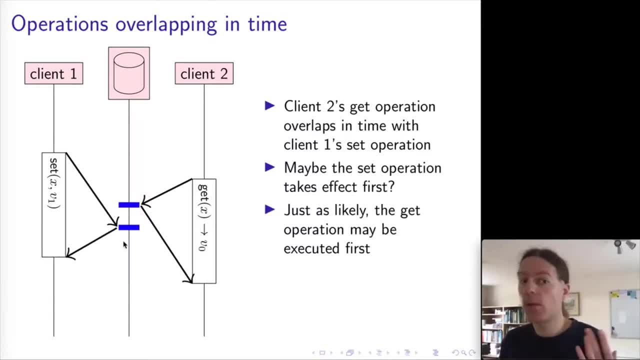 So it could be that the get operation takes effect first, the set operation second, and both of these two behaviors are absolutely fine under linearizability. So because linearizability just says that the time when an operation takes effect must be sometime after it started, 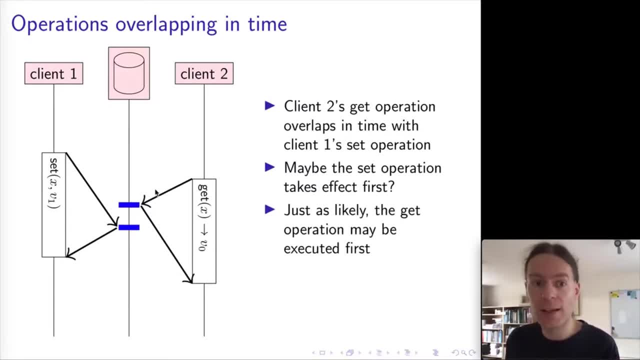 and before the operation finished. So sometime somewhere within this rectangle has to be the moment in time when the operation takes effect atomically, but we don't know where exactly within this rectangle, because we don't know what the exact network latency is going to be. 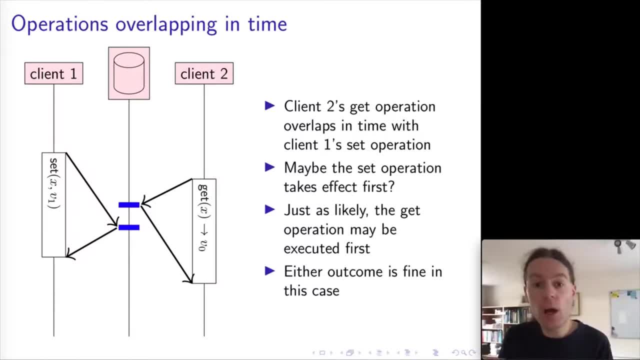 And so in this particular case, where two operations overlap in time, they can be ordered either way. but if they do not overlap in time, so one operation finished before the other one started, then we have this timing dependency under linearizability that tells us what value we must read. 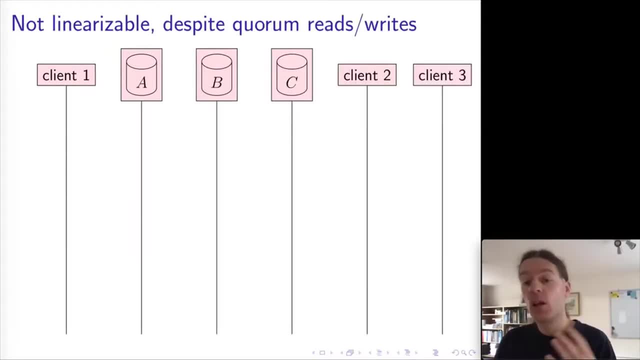 So we talked about read after write consistency, and that is ensured using quorum writes and quorum reads, And you might wonder if those quorum reads and writes are sufficient in order to ensure linearizability, And the answer is no, interestingly. 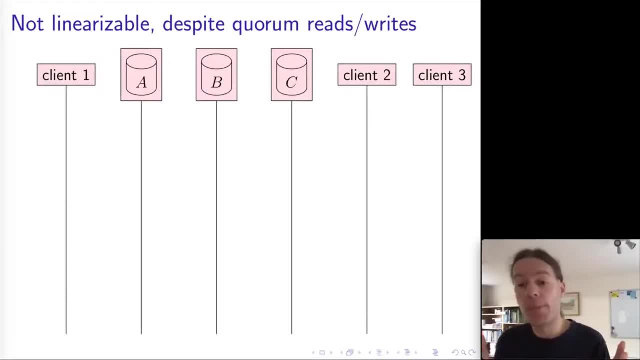 it is not sufficient to ensure linearizability just to have these quorum reads and writes, And I'm going to show you with an example why that is the case. So in this example here we have first of all a set operation by client one. 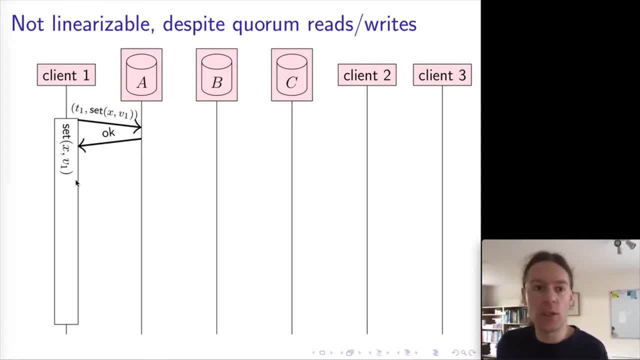 So, as before, client one wants to set the value of X to be V1. And so it sends this set request to all three of the replicas. And let's just assume for now that for some reason the request to replica A goes through very quickly. 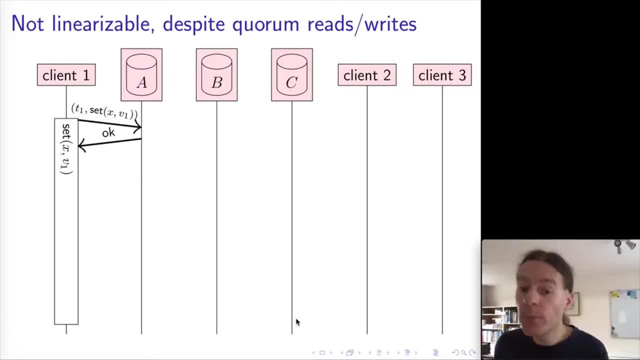 but there's a network delay in communicating that request to B and C. So eventually B and C will get updated with the value V1, but right now only replica A can see the value V1, just because of the way the network happened to time things. 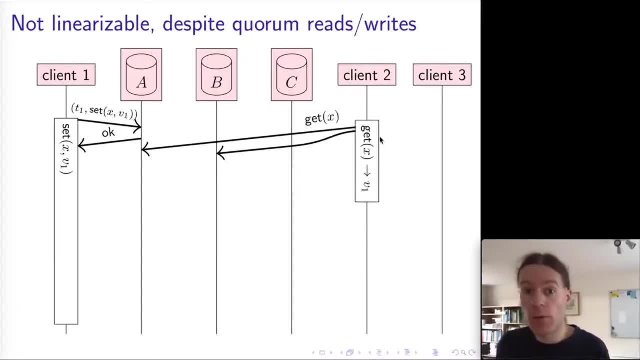 Now client two starts and makes a get request and it requests the value of X from a quorum. It gets a response from a quorum consisting of replicas A and B and it's going to compare the timestamps as usual and it's going to see that V1 is the more up-to-date. 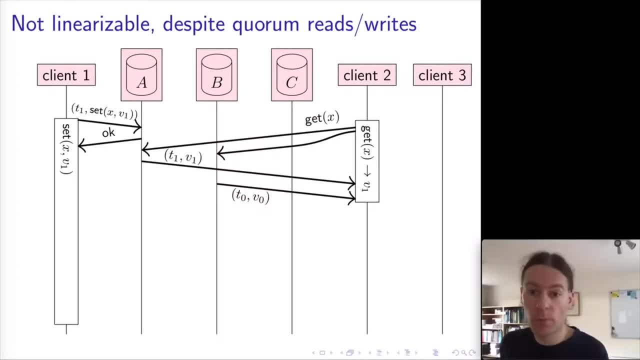 value and so it's going to return value V1 from this get request. Next, client three comes along and client three also wants to read the value of X. It sends a get request to the nodes. it receives a quorum of responses. 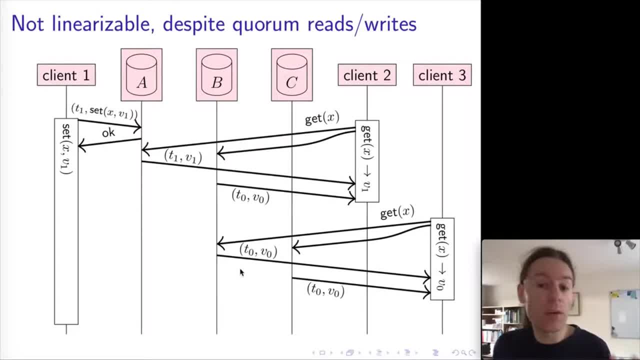 In this case it happens to get responses from nodes B and C. Now, this is also a valid quorum, so this is fine. but it happens that B and C- neither of them- has seen that up-to-date value V1 yet, because so far 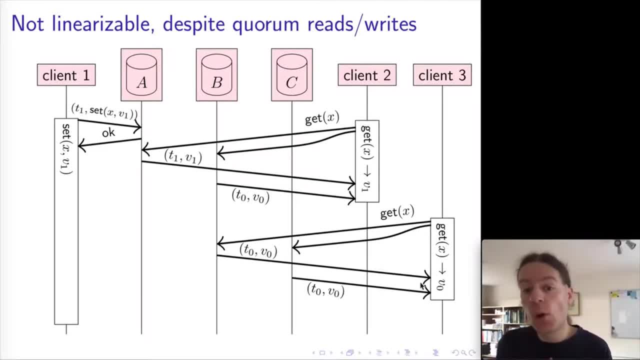 the value V1 is only on replica A but not on B and C. So client three is going to only see the value V0. It is not aware of V1.. Now, after this has happened, now client one's set operation reaches replicas B and C. 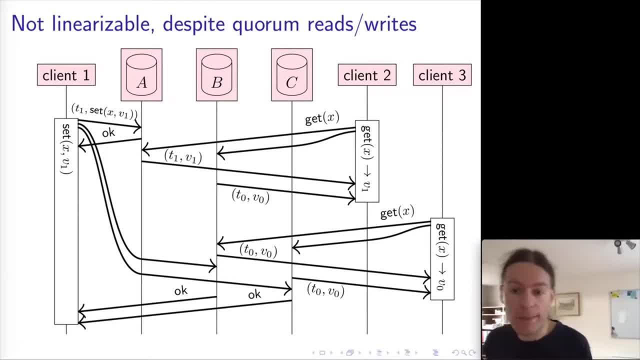 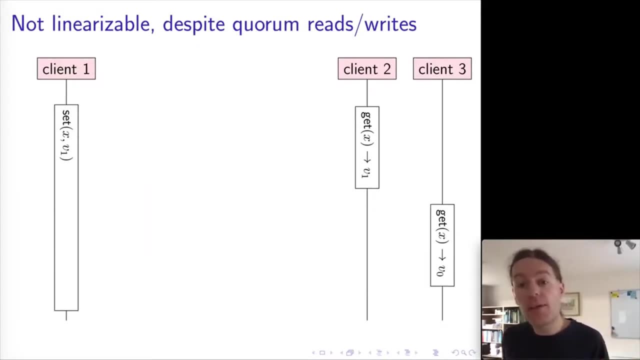 so now replicas B and C get updated and they respond: okay. So all of these requests here satisfy the quorum condition, So all of them have acknowledgement from a quorum of nodes and there are no errors happening here. But nevertheless, you can see that we have these two get. 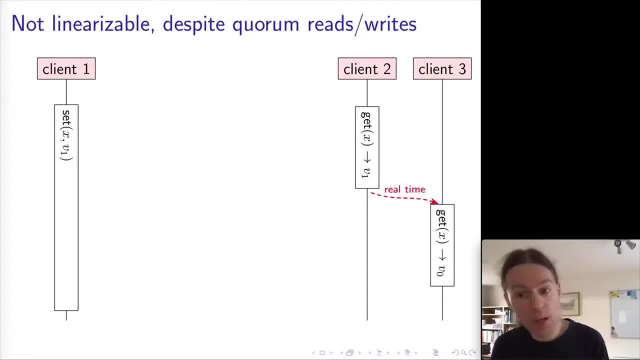 requests from client two and client three, and we have a real-time dependency between these two requests because client three's requests started later than client two's requests finished. So, as before, we have this real-time dependency between these two operations, and linearizability is not only. 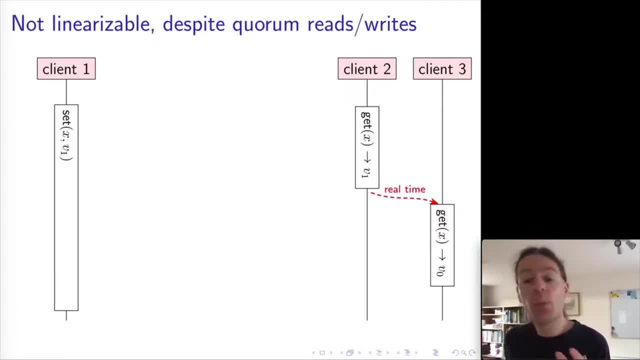 about this dependency between set and get operations, but also from one get operation to another get operation. And so, as before, we would expect here, under linearizability, we would expect client three to read a value that is no older than the value read by client two. 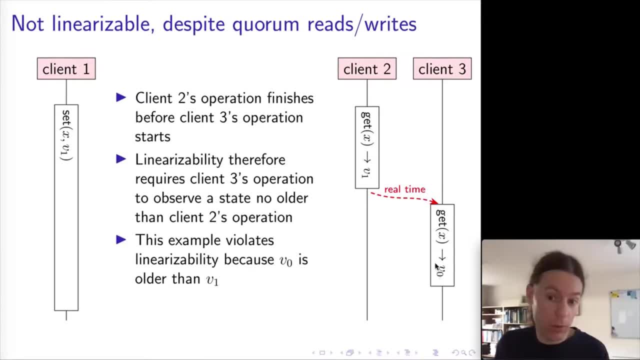 So we expect this to return V1, when in fact it returned V0. And so this is a violation of linearizability. Now you might be wondering: can we fix this? Can we fix this quorum read and write algorithm? 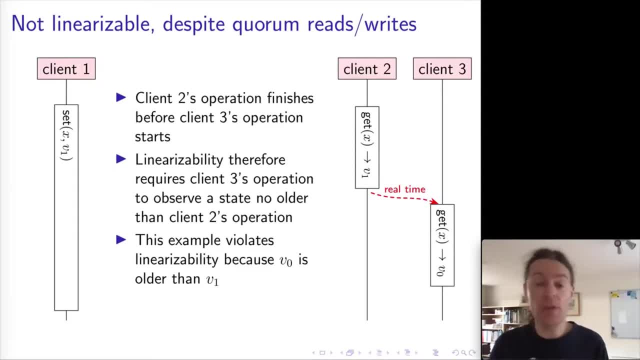 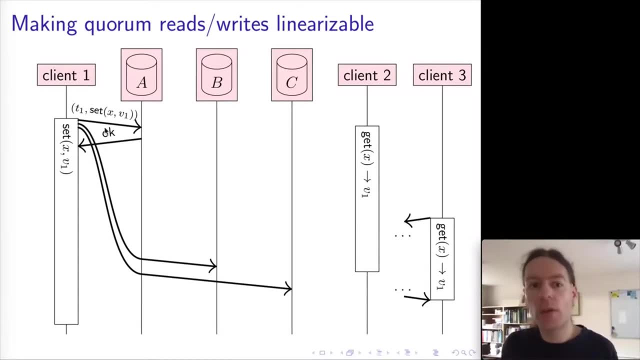 in order to make it linearizable under all circumstances. And the answer is yes, we can do that and it works like this. So, first of all, the set operation from client, one that's exactly the same as it was before. 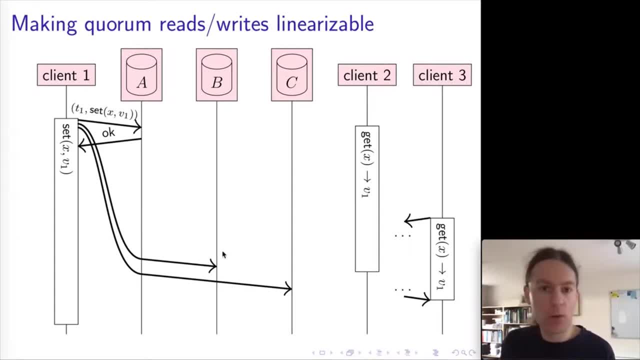 So it gets sent immediately to A and it's delayed on its way to B and C. That's fine. And next client two. So client two, as before, sends a, get request, gets back responses from a quorum consisting of A and B. 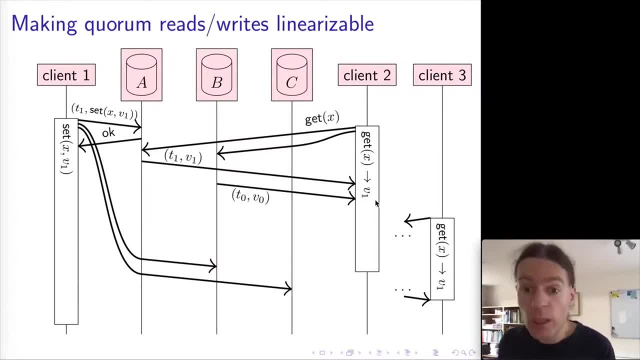 It decides that V1 is the new value based on the timestamp. But now we don't just return V1 immediately, But client two now knows that you know: V0,, V0,, V0,, V0,, V0, V0. 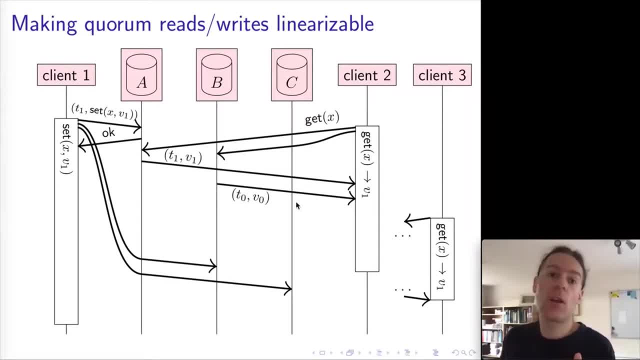 Replica B has an outdated value, And client two doesn't know what the value on replica C is, but it might be outdated as well, And so what client two is going to do is now it's going to resend the set request to any replicas that did not have the latest value. 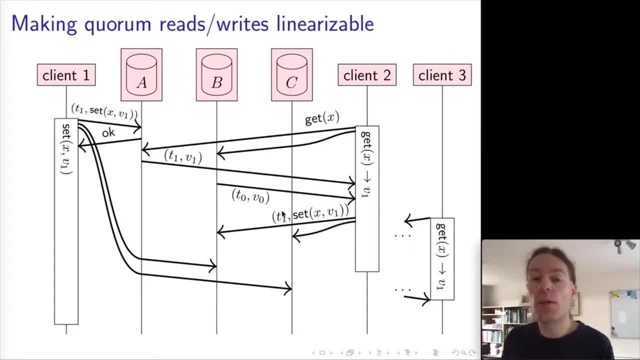 So in this case it's going to send the value V1, along with the original timestamp T1,, it's going to send that to replicas B and C And it's going to wait for at least one of them to respond. 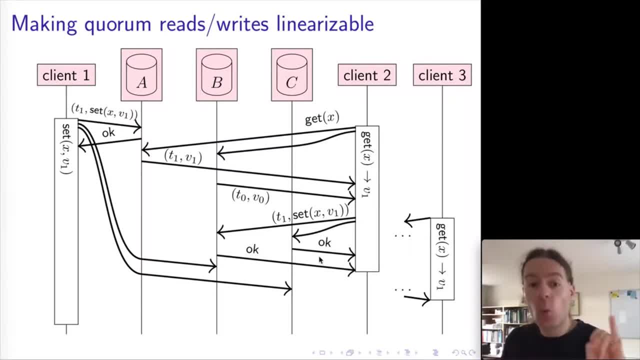 In this case it's waiting for both of them to respond, but one of them is enough. So if one of the two responds now, client two knows that the value V1 is present on a quorum of replicas at the time when this get request finishes. 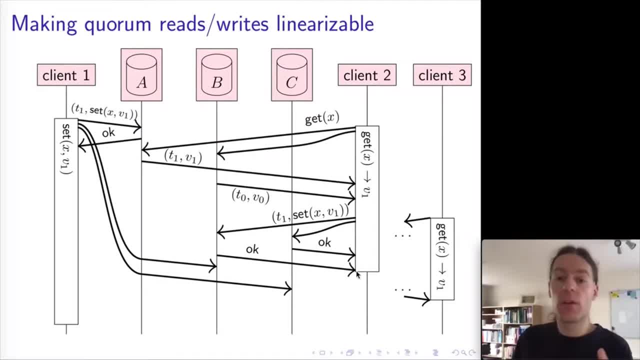 And because client two now knows that the value V1 is present on the quorum. therefore any subsequent get request that gets values from a quorum will also see that up-to-date value. So here what we have to do, this is what I called read repair in a previous lecture. 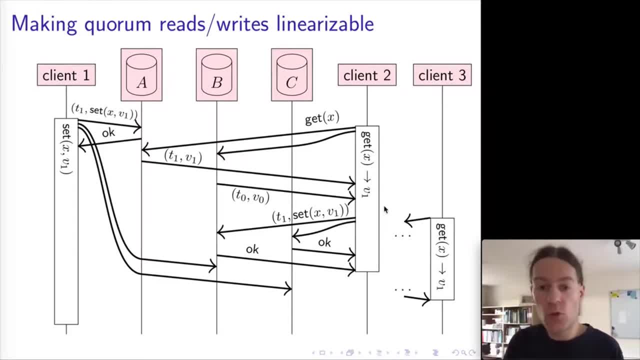 So that is the client taking a role in distributing the updated value to the other replicas, And here as long as the client two does not immediately return from the get request, but it has to wait until it is sure that the new value has reached a quorum of replicas. 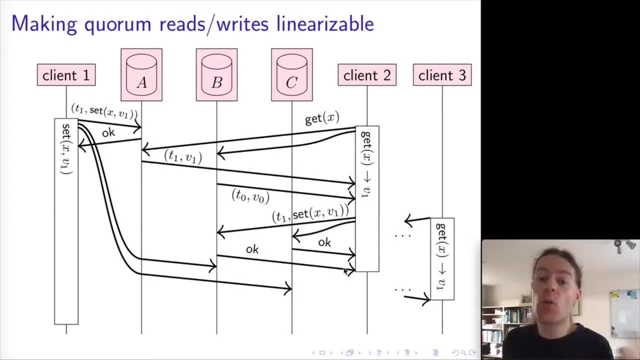 then it's allowed to return. And if we do that additional round of read repair as part of a get request, then the algorithm becomes linearizable. So in this case, now, finally, we have the response going to client one, And in this case everyone is happy. 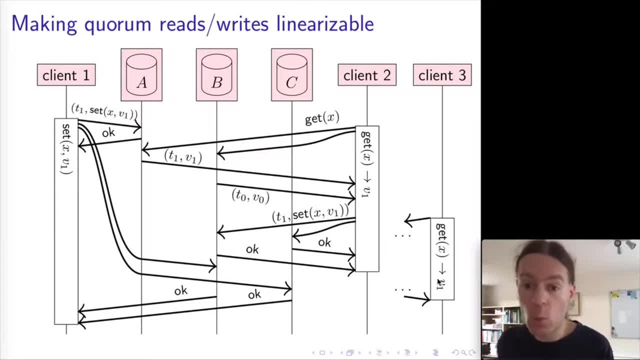 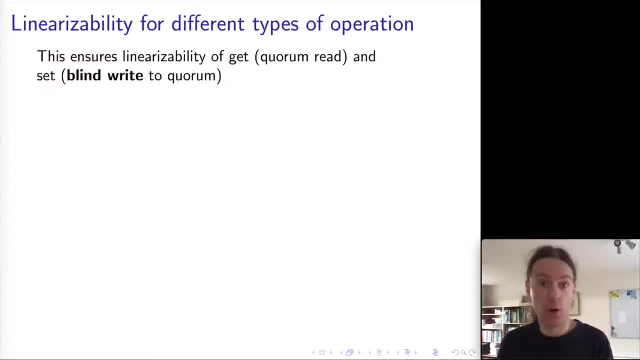 In this case, client three is going to see the value V1.. It's assured to see that. So this gives us linearizability for get and set requests. In this case we do the get by doing a quorum read with read repair. 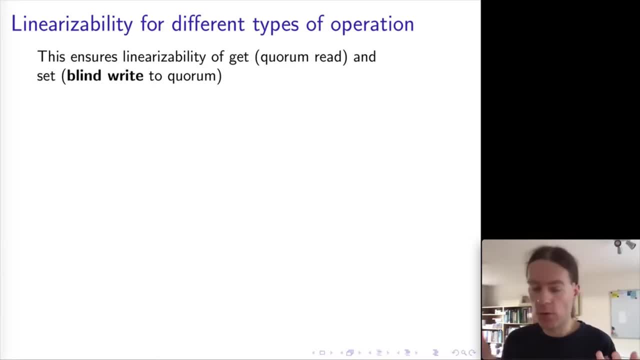 And a set request is what we might call a blind write. So the set request just overwrites whatever the value of this object is. It doesn't like conditionally overwrite it, It's just an unconditional overwrite its value with whatever the current value is. 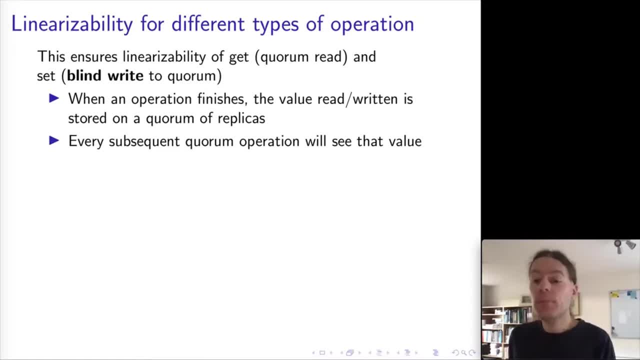 just overwrite it with a new value, And this algorithm- here it's called the ABD algorithm- is enough to ensure linearizability of these requests. However, what might happen is if multiple clients are concurrently writing to the same object, then those might overwrite each other. 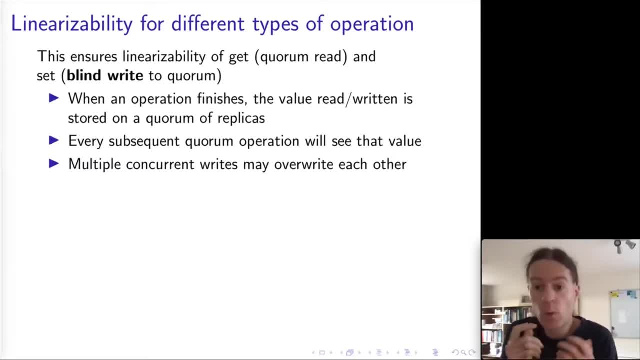 So there's no coordination between the writes. We will be ensured that they all end up with the same value across all of the replicas, but you might have a conflict due to two concurrent writes. So one other thing you might want is a compare and swap operation. 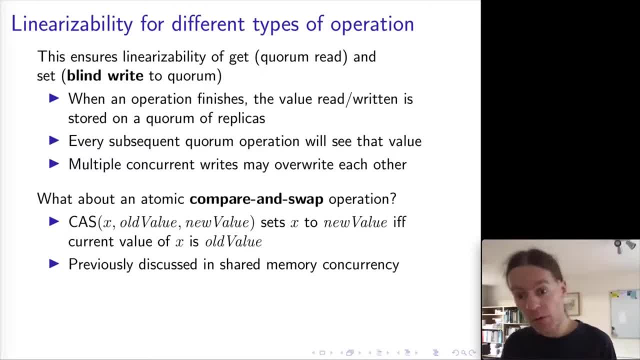 So remember this again from the first half of this course on concurrent systems, a compare and swap operation is often built into CPUs as an atomic instruction which allows you to set the value of some memory location to some new value only if its old value is some particular value. 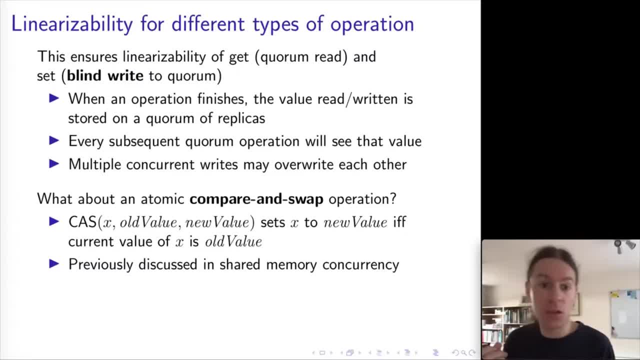 and it does this atomically. So even if multiple threads are concurrently executing these compare and swap operations, only one of them is going to succeed. So it's not going to allow concurrent context switches between, like the checking of the old value. 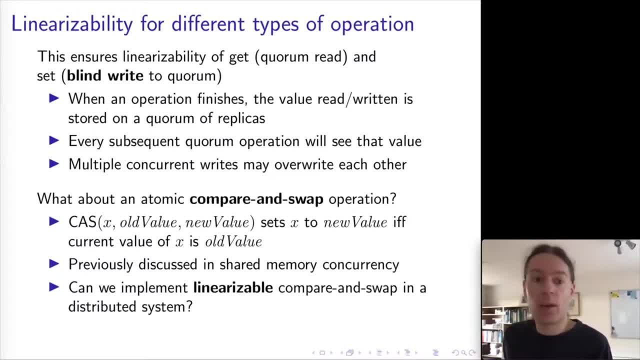 and the setting of the new value. And you might wonder: can we do the same thing? Can we do a linearizable compare and swap operation in a distributed system? On the other hand, if we do a linearizable compare and swap operation in a distributed system, 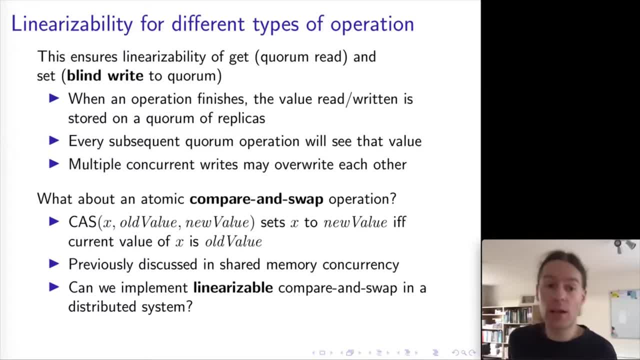 the answer is actually yes, we can, but we have to use a different algorithm from the quorum reads and writes. that we just did. We can instead use total-order broadcast again. So, once again, total-order broadcast comes to the rescue. 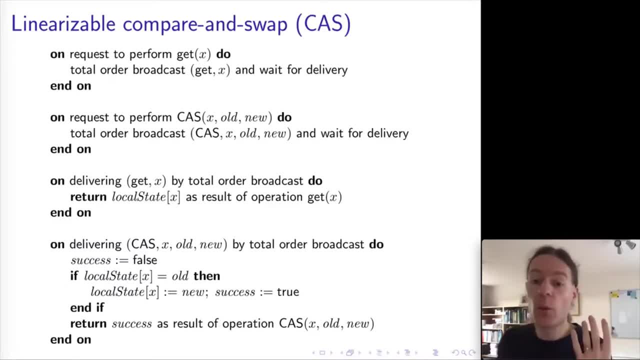 and this algorithm fits on just one slide. It's quite simple: The way we can implement a linearizable compare and swap operation and a linearizable get operation using total-order broadcast. If we want to do a get operation, we're going to make a message saying: 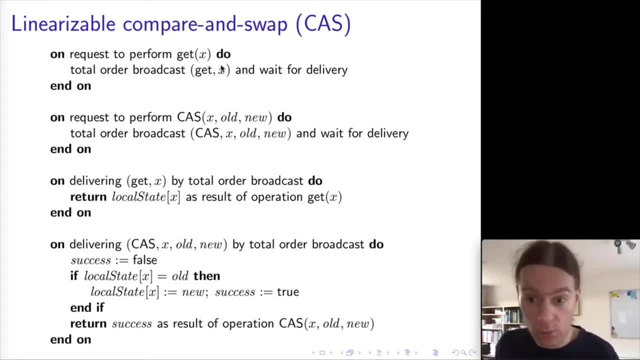 get x and we're going to total-order broadcast that to all of the nodes And we're not going to respond immediately. We're going to wait for that message to be delivered by total-order broadcast. Likewise, if we want to do an atomic compare and swap operation, 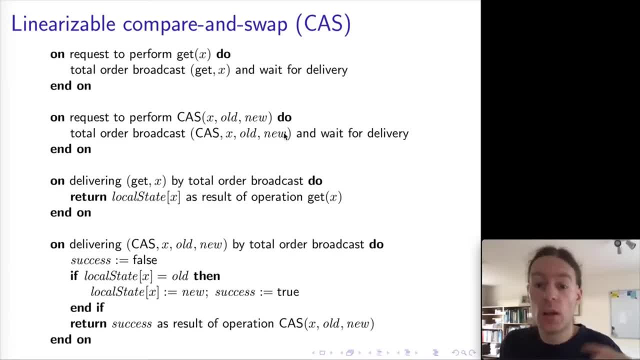 we're just going to package that operation up as a message distributed via total-order broadcast and wait for that message to be delivered. Now, when one of the get messages is delivered by total-order broadcast, well, remember what total-order broadcast is, What total-order broadcast does. 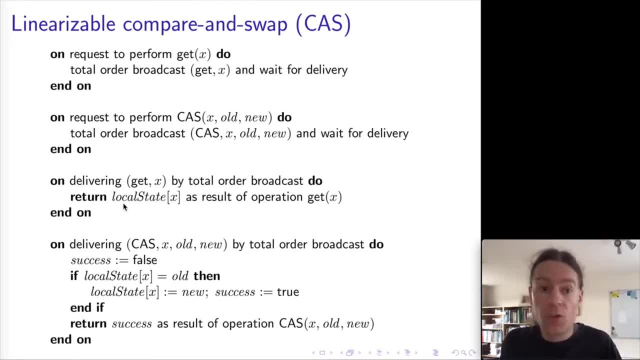 it just ensures delivery of the same messages in the same order. So therefore, all replicas are going to receive these messages in the same order. So therefore, here now, when that message is delivered, we can just read the local state, read the value of x. 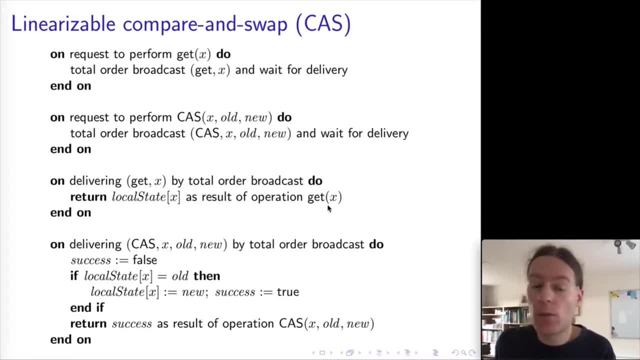 and return that current value as the result of this get operation. And likewise, if we receive a CAS message for compare and swap from total-order broadcast, then we just do the straightforward compare and swap algorithm. So if the existing state is the old value that we want, 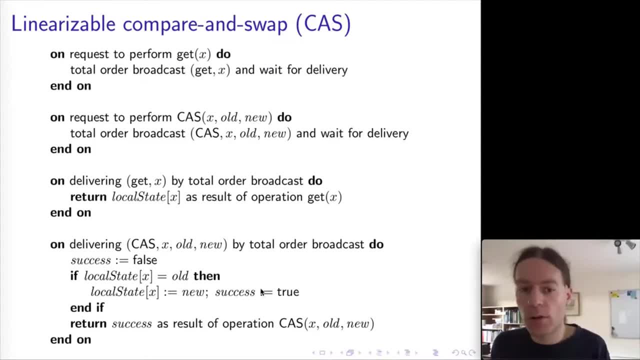 then we set it to the new value and we return success being true. Otherwise, we don't change anything and we return success being false. And we return this as the result of the compare and swap operation, And you know this is very simple. 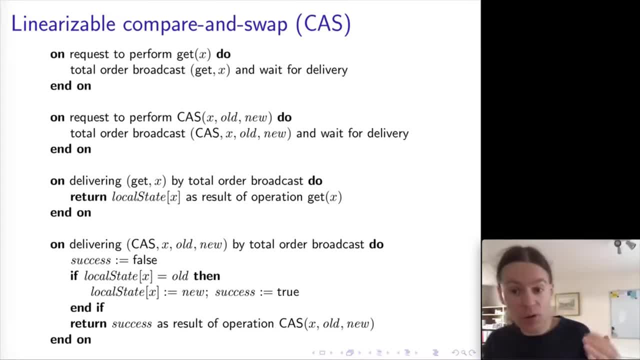 but because total-order broadcast essentially gives us this kind of single-threaded view that we can, you know that all of the operations are delivered in the same total order on all of the nodes. what we have here is essentially the same as state machine replication. 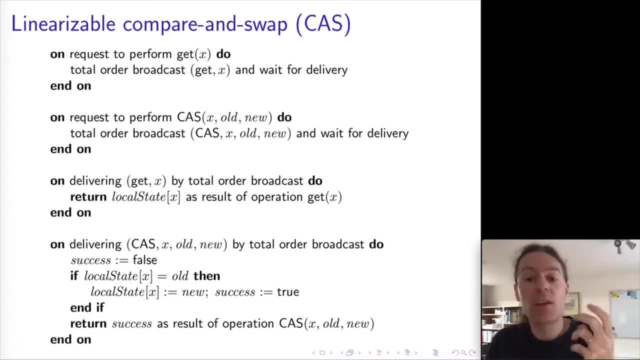 We are going to ensure that the get operations get the same result on each replica and the compare and swap operations have the same effect on every replica, And so here we get linearizability. We get these linearizable operations by building on total-order broadcast. 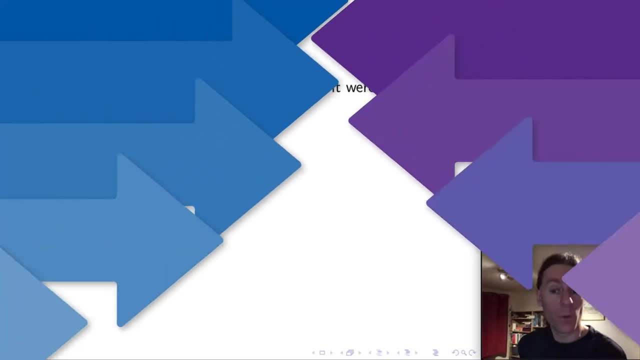 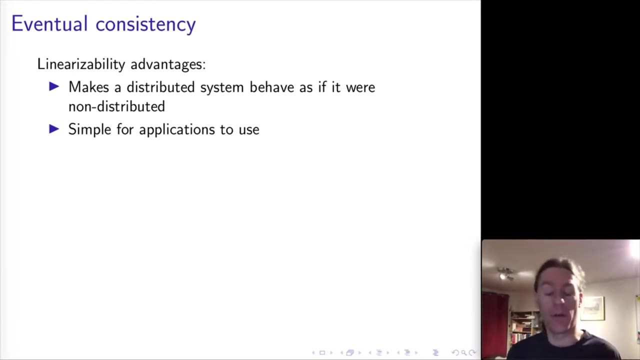 which I think is a very neat construction. So we've talked about linearizability as one possible consistency model for distributed systems, which is a very strong consistency model, And we said it has the very appealing property that it actually makes a replicated system look as if it were not replicated. 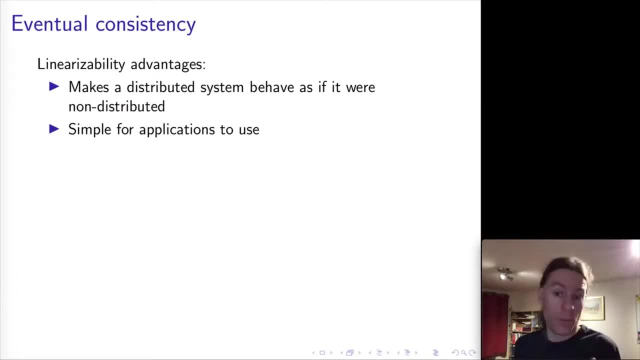 It looks as if there was only a single copy of the data, and all of the operations on it are atomic, which makes linearizability a very easy-to-use consistency model. You basically don't have to think about the fact that your system is distributed. 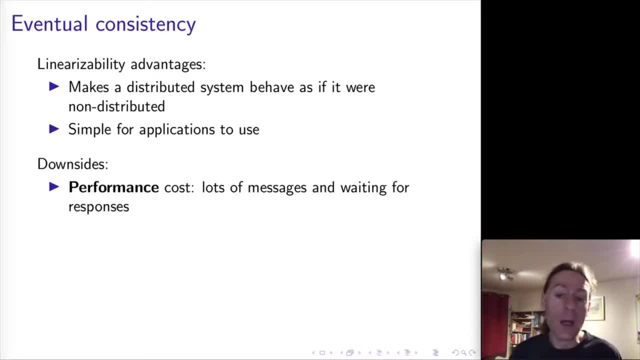 and it just kind of works in the way you might expect. Unfortunately, it comes at a price as well, So linearizability is not actually suitable in all possible circumstances, for several reasons. One possible reason is that it's actually quite expensive to implement. 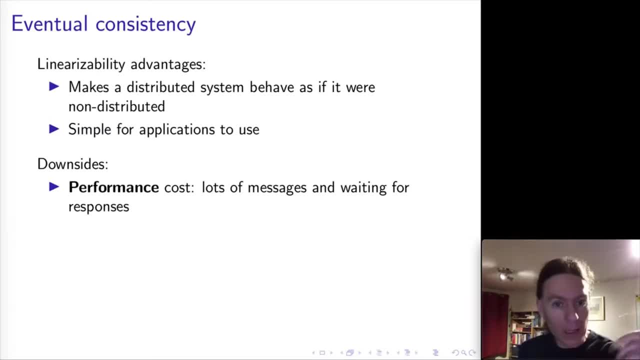 If you looked at the protocols that we discussed, there are lots of messages going back and forth, lots of waiting for responses, probably something like two round trips for most requests. So you know, it's just going to be a bit slow, basically. 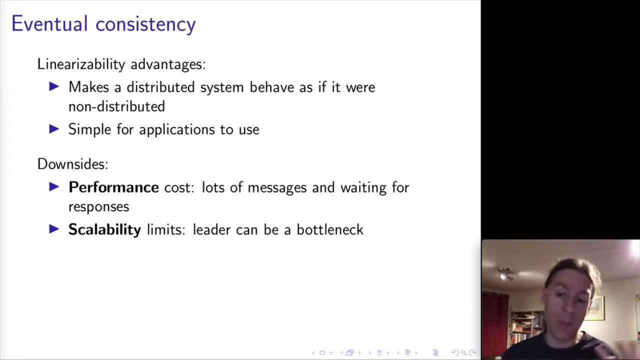 Another limitation is the scalability. potentially It depends a bit on the exact algorithm you're using, but if you're using a consensus algorithm like Raft, for example, all of the updates have to be sequenced through the leader, so there's a single node. 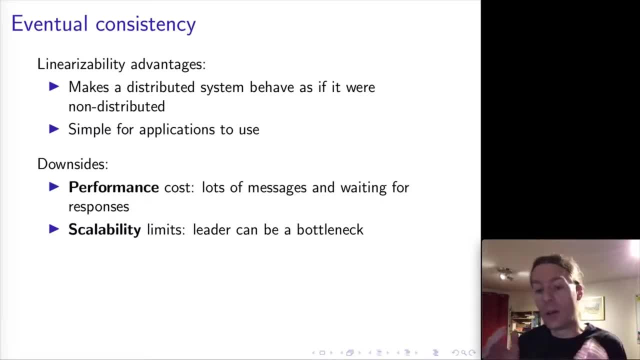 that all of the updates have to flow through, and so you are limited by the capacity of that one node. in this kind of system, That one leader node can become a bottleneck. And what is perhaps the deepest problem with linearizability and such strong consistency models? 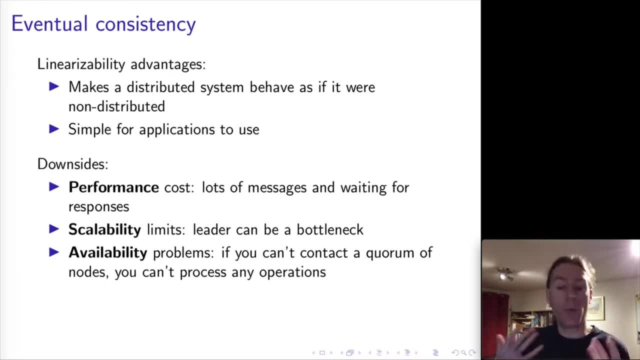 is problems with availability, and that is. every operation that you do needs to contact a quorum of nodes, and that means, if you can't contact a quorum of nodes for whatever reason, maybe you're disconnected on the network, or so you can't process any operations. 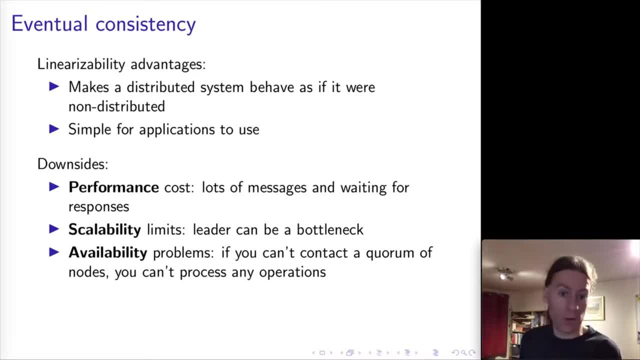 Neither reading nor writing is possible if you can't contact a quorum of nodes, And that's why, alternatively, if you can't contact a quorum of nodes, you can't process any operations. So alternative consistency models have been developed which have different trade-offs. 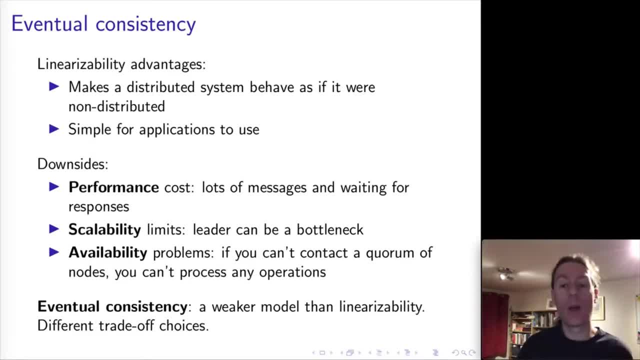 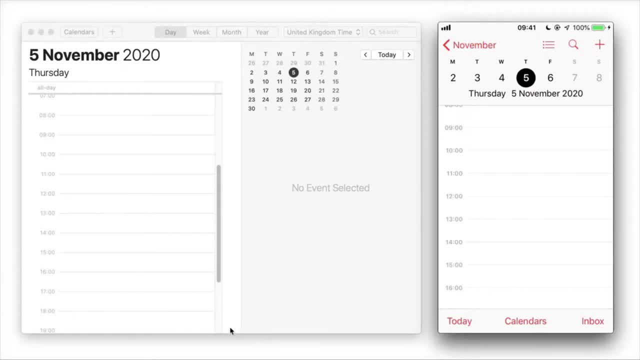 which are better in some regards and worse in other regards, And the one that we will look at in this section is called eventual consistency. As an example, let's consider a calendar app. So here I have, on the left-hand side, the calendar app running on my computer. 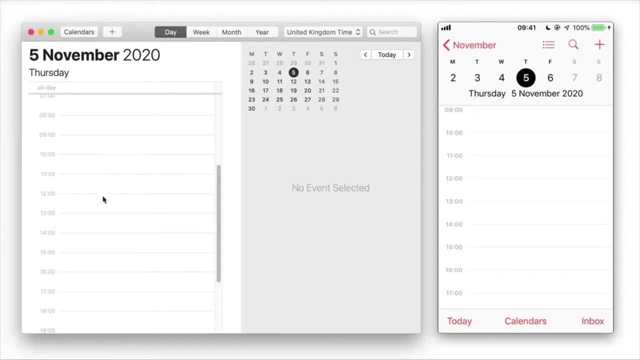 and on the right-hand side, the calendar app running on my phone, And you all know how this works. I can add an event on the left-hand side, say this: rootedSystems, and this will sync within a couple of seconds over to the phone on the right-hand side. 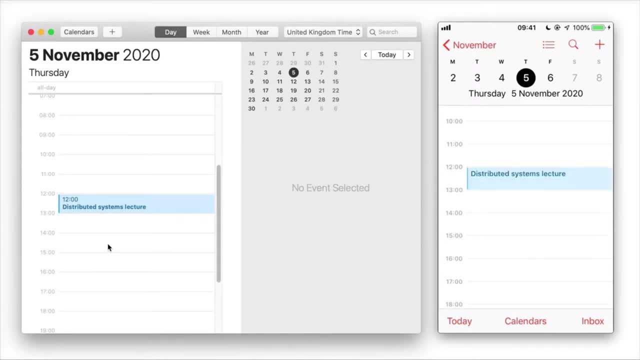 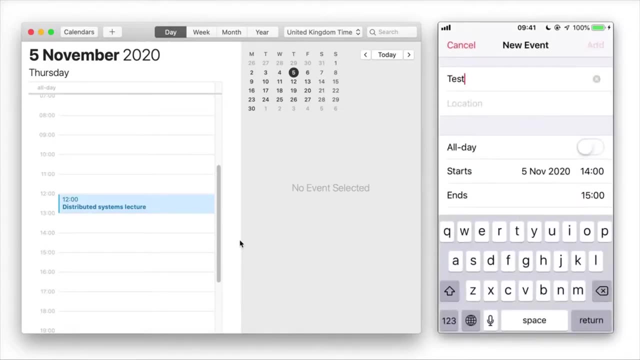 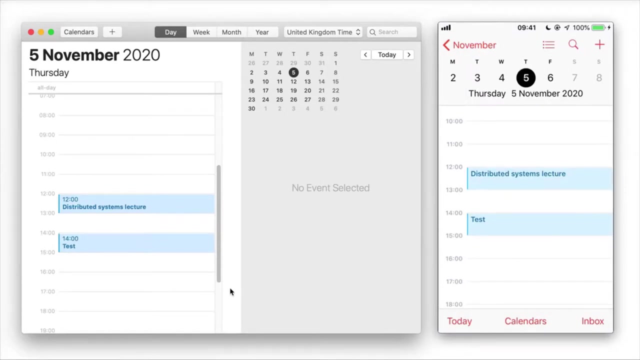 So then the same event should appear there. Here we go, And similarly I can add an event on the phone, and this should sync over to the computer. Now, what we've got here, if you think about it, is a replicated system. 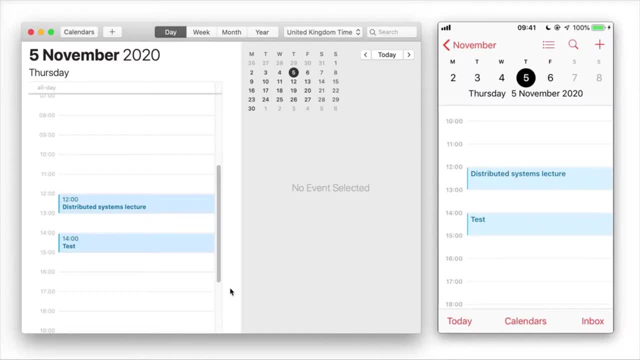 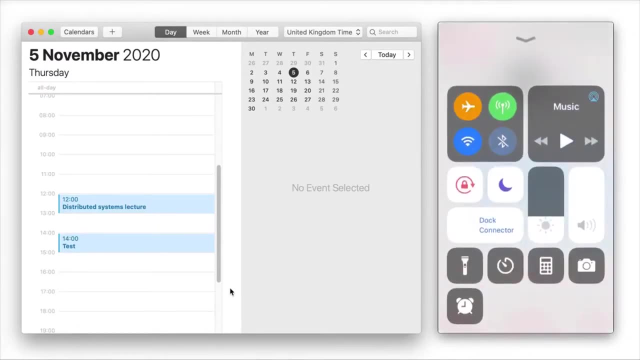 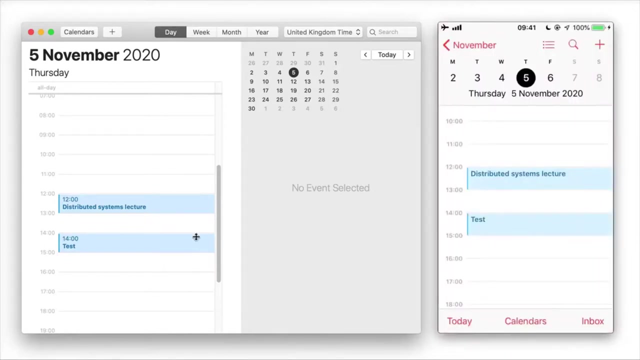 We've got a copy of the calendar on my computer and another copy of the calendar on my phone, And these two replicas are independent from each other in the sense that I can put my phone into airplane mode And now I have prevented any communication from between these two devices from happening. 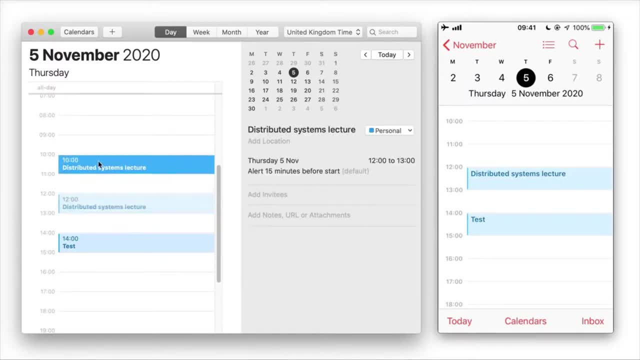 And so I could, for example, on my computer now change the time of the distributed systems lecture to 10 am, And this won't sync over to my phone because my phone is unable to communicate. And let's say, on my phone I changed the title. 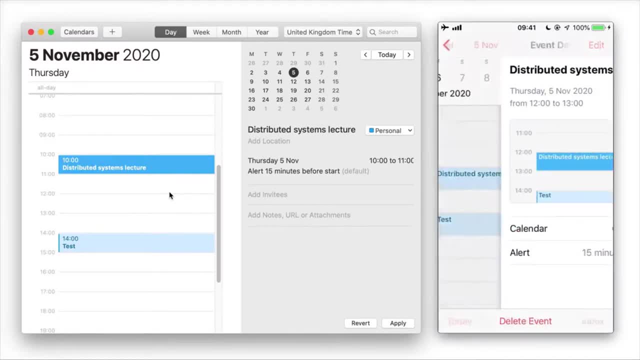 to say distributed systems, lecture one. And this also won't sync back to the computer until I eventually turn off airplane mode. And so now, after airplane mode is off, now the two devices should be able to sync up with each other again And the changes from one should propagate over to the other. 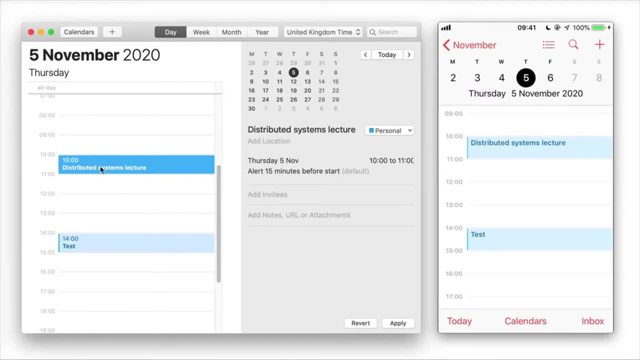 So you can see what has happened. now is the time of this event has moved to 10 am on both devices. but my change changing the title distributed systems lecture. I changed it to lecture one but that change of the title has somehow disappeared. 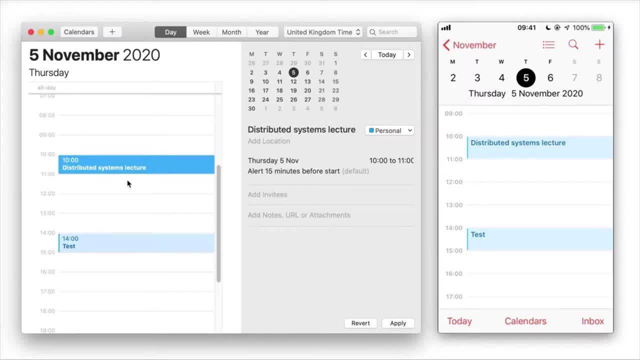 And so what we have here is a conflict, because I concurrently edited the same calendar event on two different devices while they were disconnected from each other, And we had a conflict resolution that had to happen here, and what my calendar app did apparently was a last writer wins resolution. 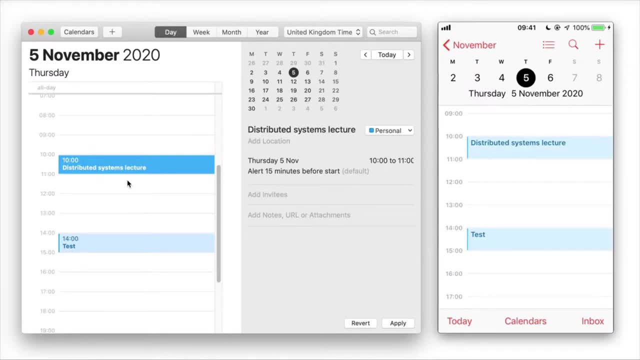 in which case? in this case, the update of the time to 10 am somehow took precedence over the update of the title, And so the update of the title was discarded, while the update of the time took effect on both devices, But we so, even though some data was lost here. 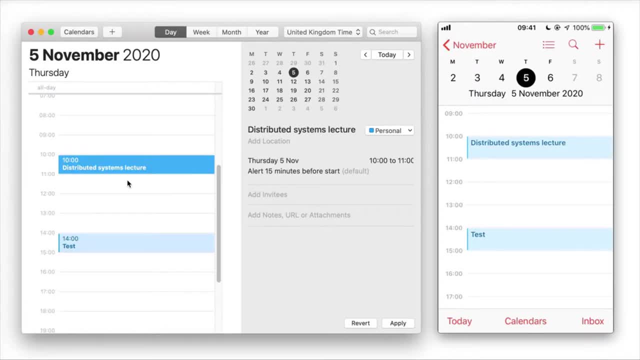 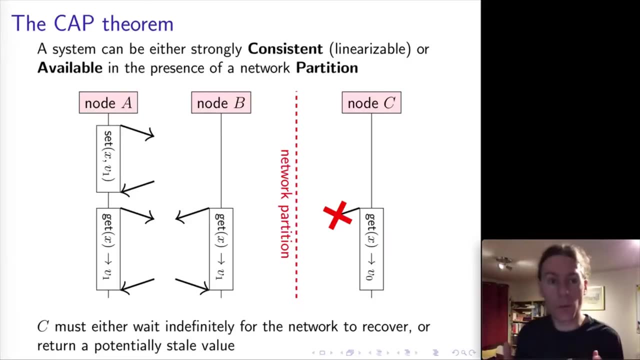 but at least we did end up with both devices being in a consistent state. Eventually, these systems, such like the calendar app, can be formalized using this result from distributed systems, called the CAP theorem, And this idea behind this is fairly simple. It is say: you have a system, 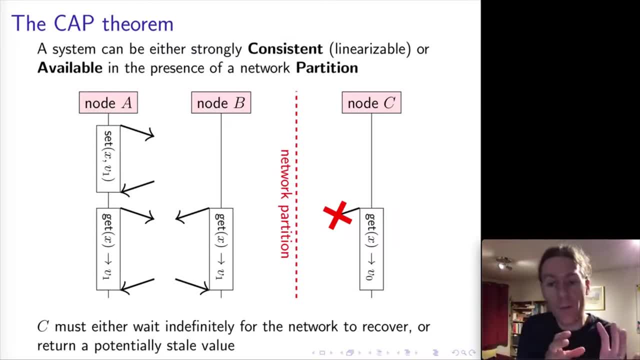 in which there's a network partition, that is, some of the nodes. one subset of the nodes is unable to communicate with some other subset of the nodes. In this case we have to make a choice. Either we can continue providing linearizability. 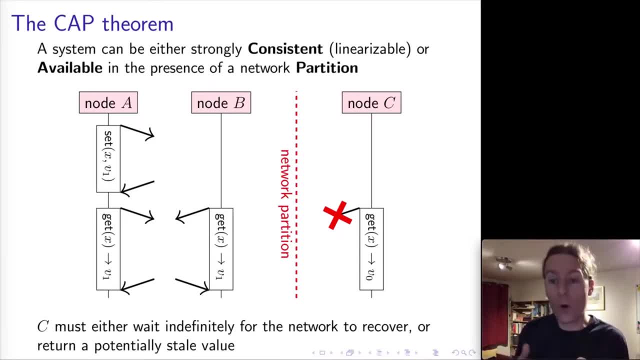 but some of the nodes won't be able to process requests, Or we allow requests to and operations to continue without contacting a quorum, But in that case we risk violating linearizability, And so we have to just make this choice in the presence of a network partition. 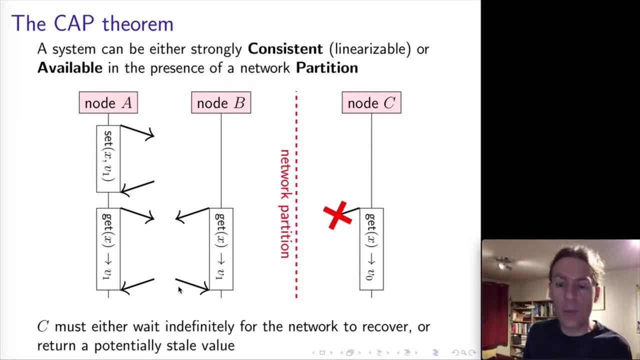 Illustrated here. so we've got, on the left-hand side of the partition, nodes A and B, which form a quorum, and they can continue providing a linearizable service for these operations. But node C, here on the right-hand side, is stuck in this dilemma. 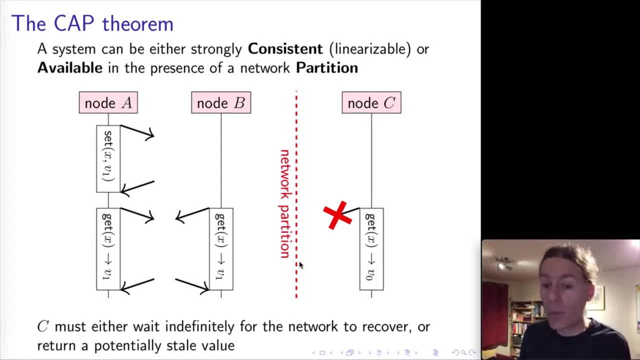 because either the node C has to wait for this network partition to be healed before it can reach a quorum, which might take indefinite amount of time, And so in that during that time, node C is effectively unavailable and not able to process any requests. 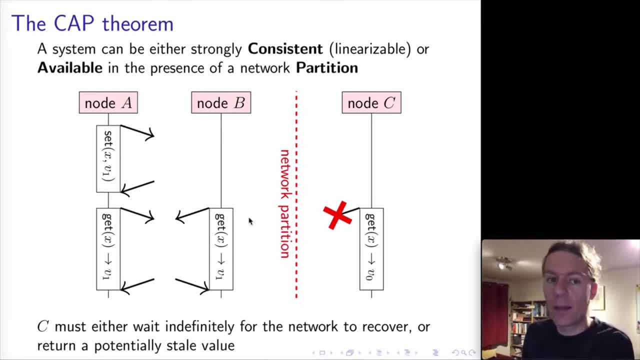 Or node C just goes ahead and uses its local state, but in that case it won't know about the value V1 that was written by A. So in this case we will have violated linearizability, And so this is just a fundamental choice that you have to make. 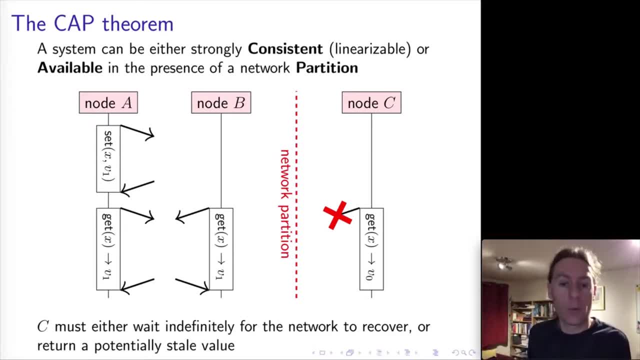 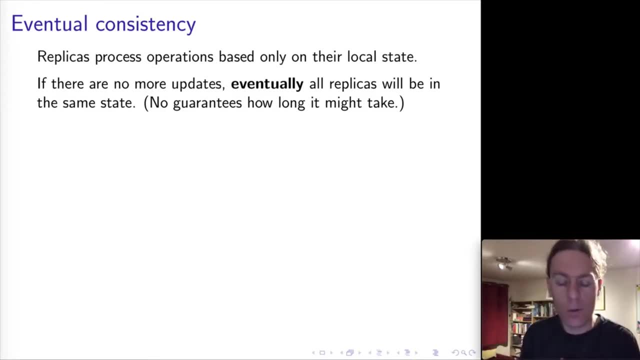 to make in a system in which network partitions might occur, And eventual consistency is sort of the broad category of consistency models that typically people move to if they don't want to make an assumption of being able to communicate with a quorum, something like that. 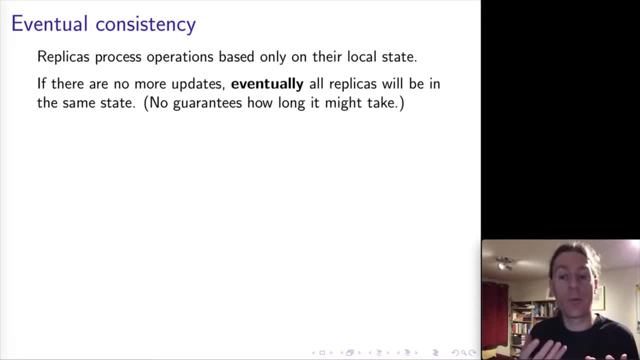 So if we want each replica to be able to process operations just based on its local state and without waiting for a communication with a quorum, we cannot achieve linearizability, but we can achieve weaker consistency models And the way eventual consistency is usually defined. 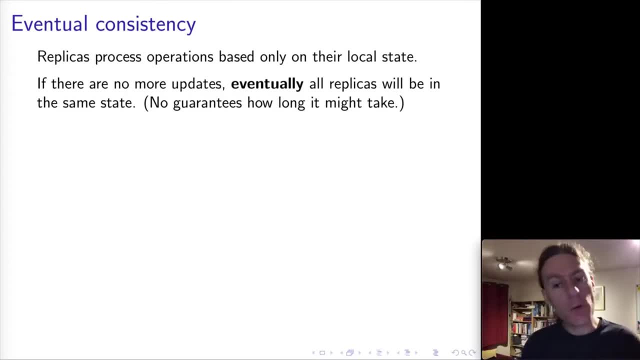 is like this: First of all, any read requests a replica can just process based on its local state, And then, whenever some updates get applied to one replica, they will eventually wander over the network at some point to other replicas, And what we want to guarantee is that. 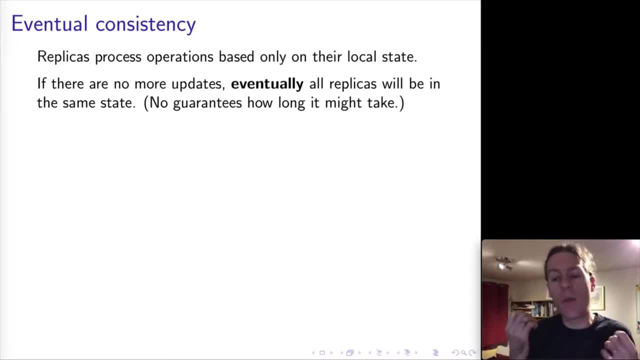 if we assume that we have a quorum, we assume that at some point the updates stop, then eventually, after the updates have stopped, then all of the replicas end up in the same state. Now, this is okay, but it's a fairly weak property. 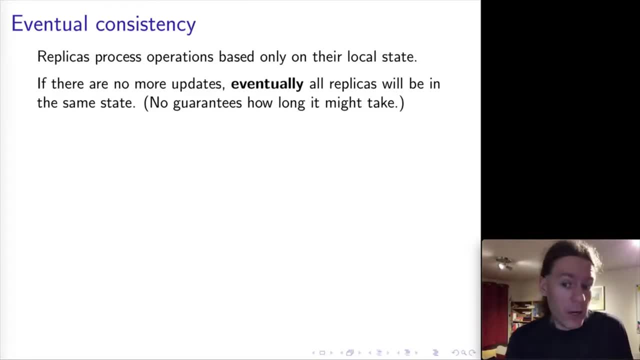 because, for example, what if the updates never stop? You could have a system in which continually updates are processed nonstop. And so, in this case, eventual consistency does not define what will happen in that case, because the premise of this statement, of this definition, 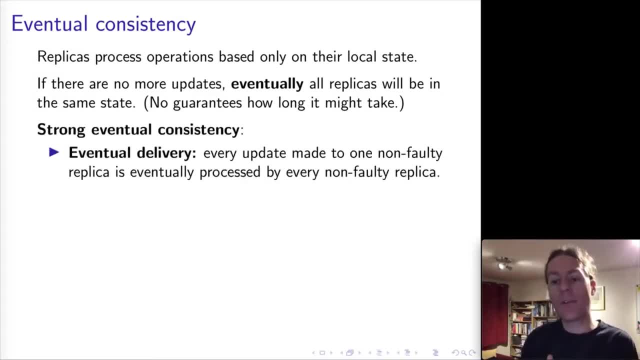 is not true. So what people have done is to define an alternative slight strengthening of eventual consistency, called strong eventual consistency, which is defined with two properties. So first of all, we say that any update that has been made on one replica will eventually also be made on another replica. 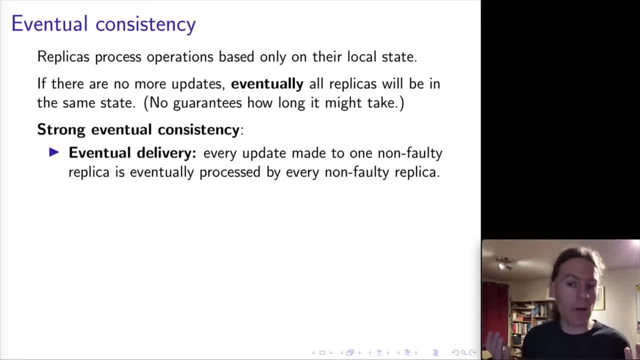 So updates get disseminated over the network. We don't make any guarantees about how long that's going to take, We just say eventually this will happen. And secondly, whenever you have two replicas that have processed the same set of updates. 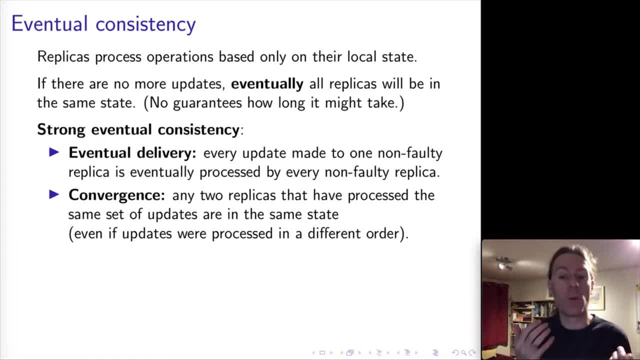 then those replicas must be in the same state and thus they will return the same results to any read requests, And this must hold even if those updates were actually applied in a different order on different replicas. And so this comes back down to the causal broadcast based replication protocols. 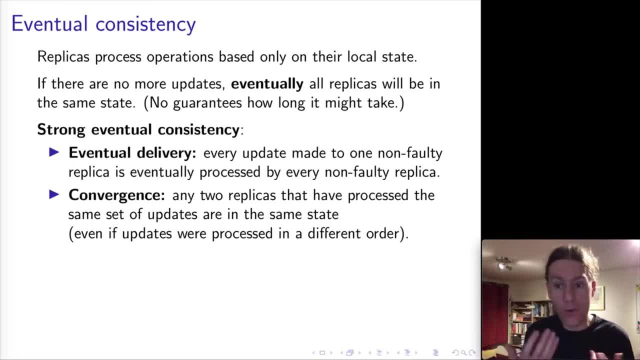 that we saw earlier, for example, where if you have commutative operations, you're updating the state, then you can have different replicas, updating the state in a different order and still converging to the same final state, And so this idea of convergence is really at the core. 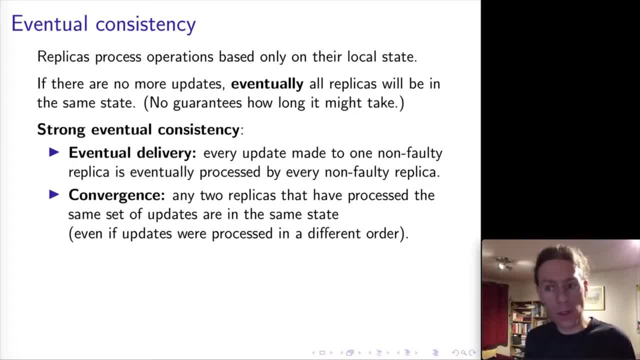 of eventual consistency and strong eventual consistency. Now, both eventual consistency and strong eventual consistency have some very nice properties. If you want to implement this model, there is no need ever for an operation to wait, for example, for communication with another replica. 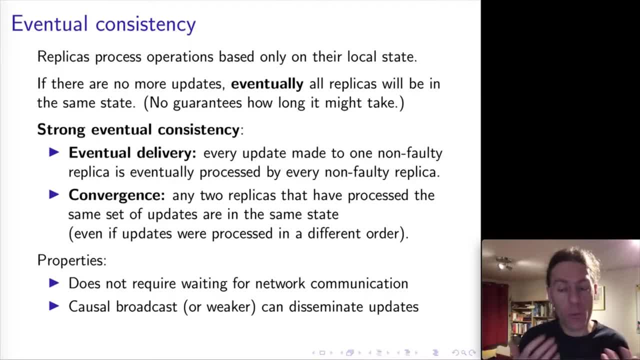 So a replica can always process operations. Both reads and writes can be processed just locally without waiting for any communication. Of course, eventually sometime communication will have to happen in the background, but the operations don't have to wait for it, which means that the operations can always be fast. 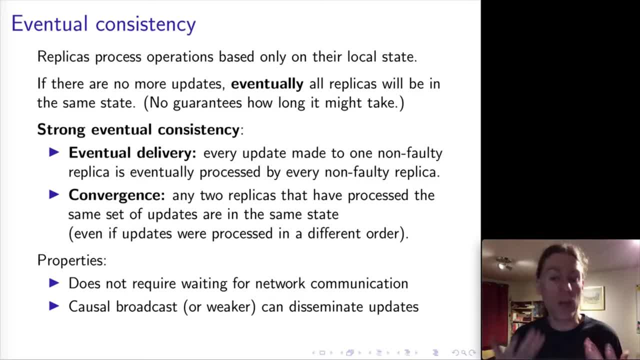 They're never waiting for network round trips and the operations can always be reliable because even if the network is interrupted, a replica can continue processing operations And we can use. we can use these broadcast protocols of causal broadcast or FIFO broadcast or these other weaker broadcast. 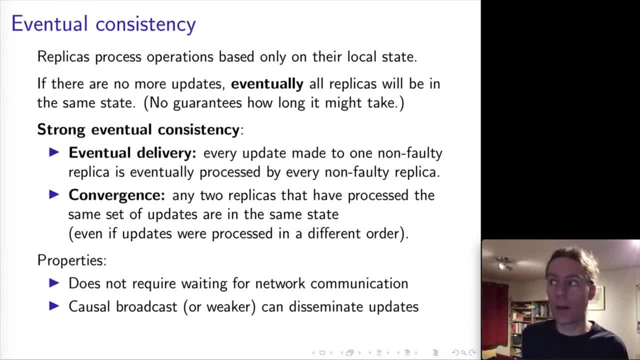 as a way of distributing the updates from one replica to another. Now, one problem that can arise with eventually consistent systems is that the same object or the same data item can be concurrently updated by multiple replicas, And there's nothing stopping this, of course. 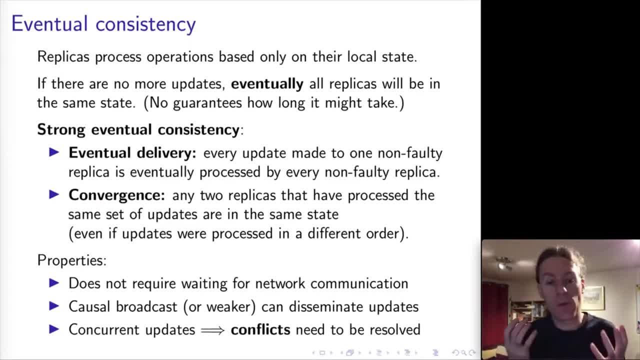 because they cannot communicate it necessarily, And so, because we have these concurrent updates of the same object, we might have conflicts, And so those conflicts will have to be resolved in some way or another. With the calendar app, what we saw is just the last writer wins policy. 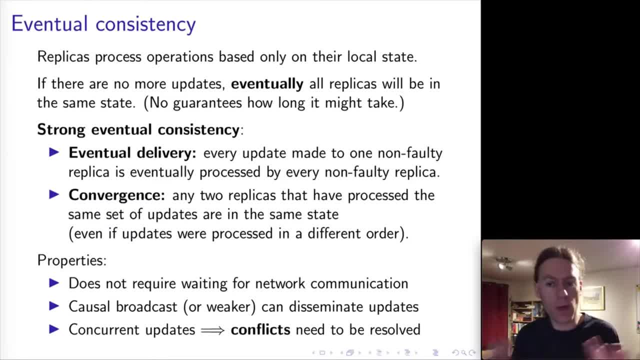 where one of the updates took precedence over the other. the other one was just discarded. but we can also devise more sophisticated conflict resolution policies- And I've actually done some research in this area- on merge algorithms which will take concurrently updated data structures and merge them together into a clean final state. 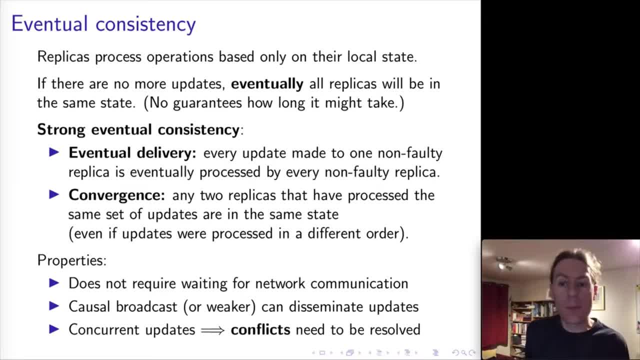 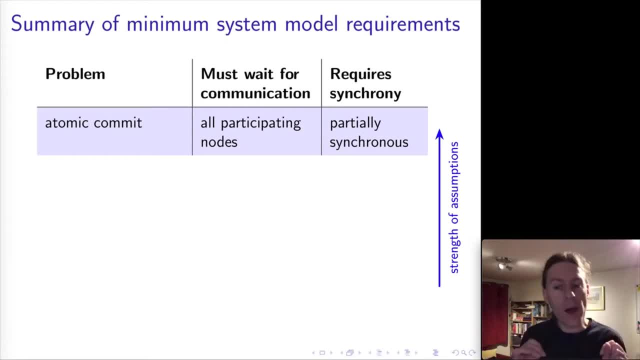 to resolve the conflict. So that's eventual consistency. I will now recap the consistency models and algorithms that we talked about in this lecture, and do that in the order of how strong the assumptions are that they make about the system model. This is an interesting way of comparing. 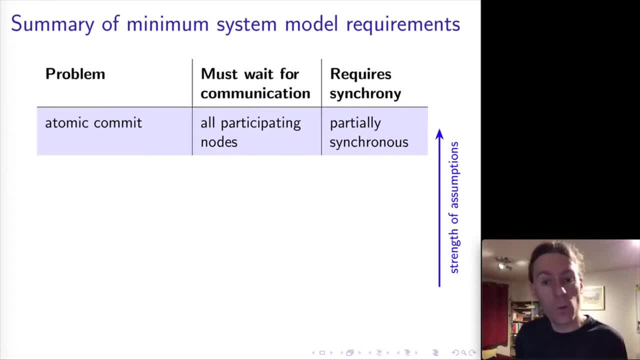 these different algorithms and approaches. So, first of all, we started with atomic commitment, as in two-phase commit, and remember that the model with atomic commit is that a transaction can commit only if all of the participating nodes vote to commit, And so this means that inevitably, 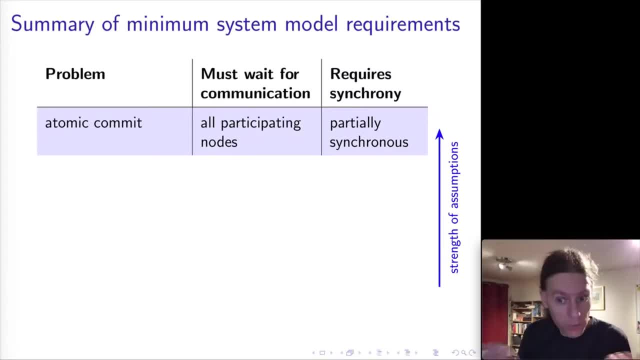 atomic commit requires communicating with all participating nodes, which might be all nodes in the system. So if any one node is crashed, atomic commit will not be able to commit any transactions. So this is a very strong assumption that we have to make about the communication that happens in a system. 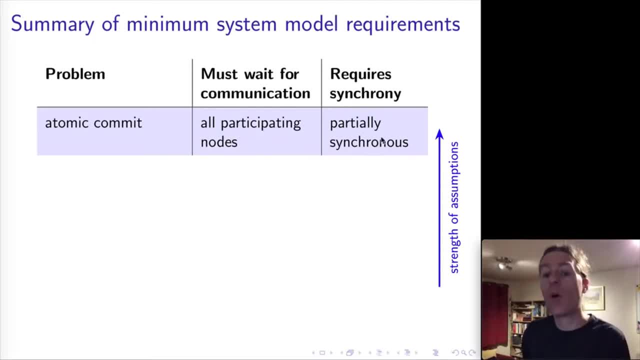 We have to communicate with all nodes and wait for their response. Moreover, we have to assume a partially synchronous system model because we have timeouts and failure detection. that has to happen Now. one step down from this is consensus and total order broadcast. And so consensus and total order broadcast. 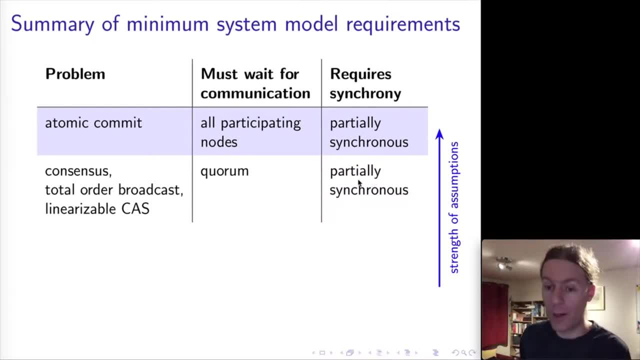 the FLP result told us that this also requires a partially synchronous model. So the FLP result says that there's no asynchronous algorithm for implementing consensus, And so therefore, partial synchrony is what we want. That's what we have to assume. 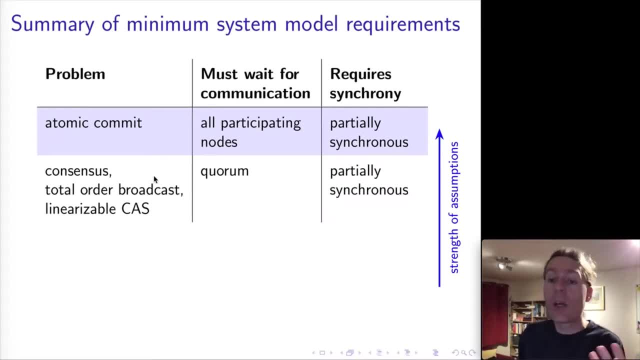 But in terms of the communication, these consensus actually assumes a bit less, because it only requires communication with a quorum, And so therefore we can tolerate a minority of nodes being unavailable, and the algorithm will still be able to make progress and complete as normal. 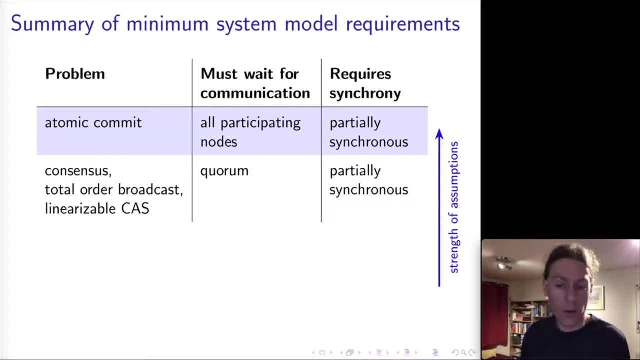 And so this holds for consensus and total order broadcast, which are equivalent to each other, as we said. Moreover, we saw that for linearizable compare and swap, we can implement that using total order broadcast And, in fact, it is possible to prove. 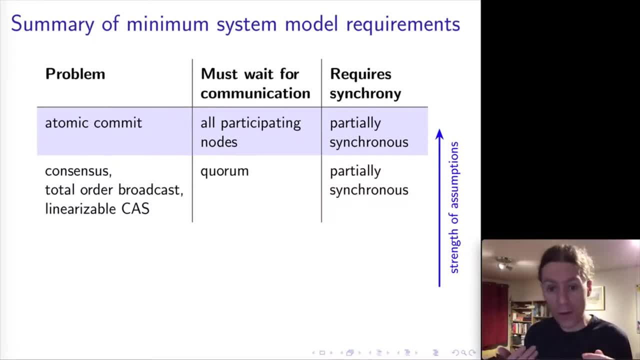 that linearizable compare and swap is also equivalent to consensus. So all these three problems are actually reducible to each other. They all have the property that they require a quorum and partial synchrony- Moving down in the list, interestingly- a linearizable get and set operation. 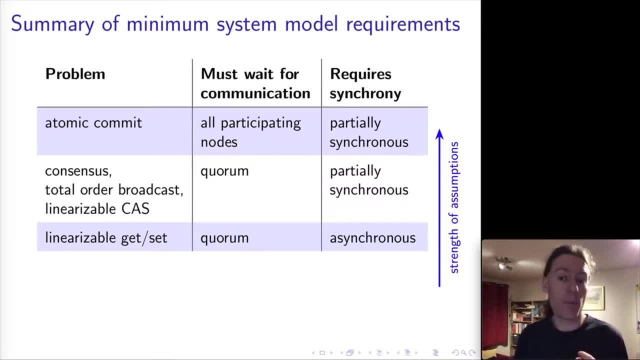 has weaker assumptions than a linearizable compare and swap operation, Because for get and set we can just use the approach we saw earlier, the ABD algorithm, which means quorum writes and quorum reads with read repair, And this still requires communicating with a quorum of nodes. 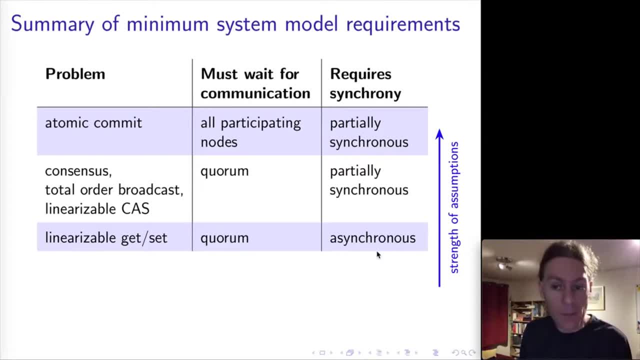 But notice that in this algorithm there are no timers, there are no timeouts, there's no failure detection. The algorithm is actually completely asynchronous. It doesn't require on clocks at all, And so this means that actually linearizable get and set has weaker assumptions. 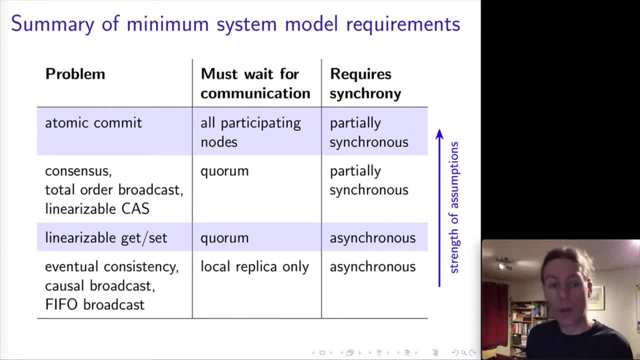 about the system model than compare and swap. And finally, as we move all the way down to the weakest assumptions that we can make, now we're with eventual consistency, where every replica can update and read its own local state without waiting for any communication. 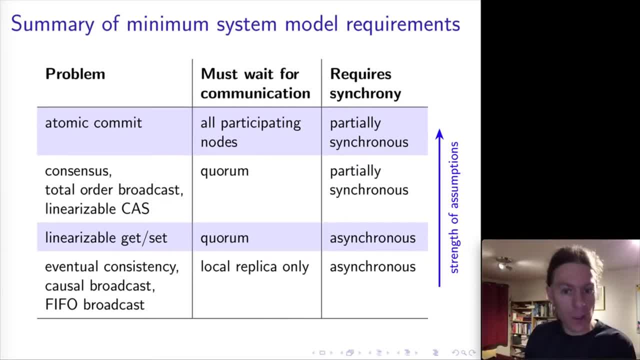 with any other replica. So the communication need is totally minimized here and we still make no timing assumptions. So this is about the weakest that we can assume for both eventual consistency and strong eventual consistency And also in terms of the broadcast protocols. call the broadcast FIFO broadcast. 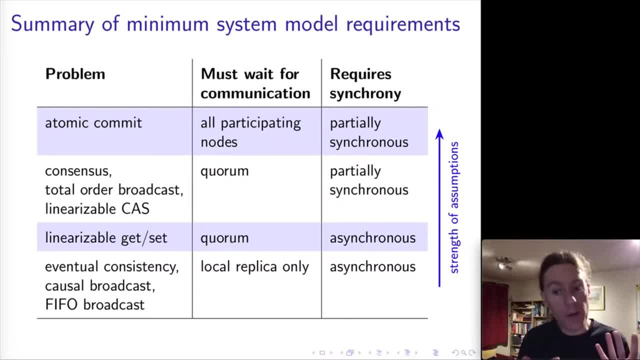 reliable broadcast, best effort broadcast- All of these have the property that they can deliver a message to themselves immediately. A node doesn't have to wait for communication with any other node in order to deliver a message to itself, And this thus also has the property. 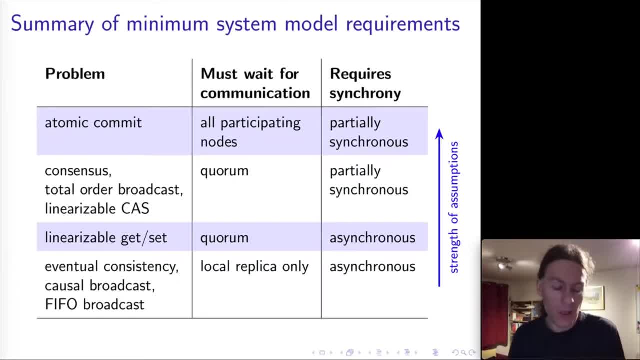 that if these messages are updates, that means updates can be applied locally without waiting for any communication. So this also has the property that no waiting for communication is required in order to process local updates. So that's all on consistency models for today. Welcome to the eighth and final. 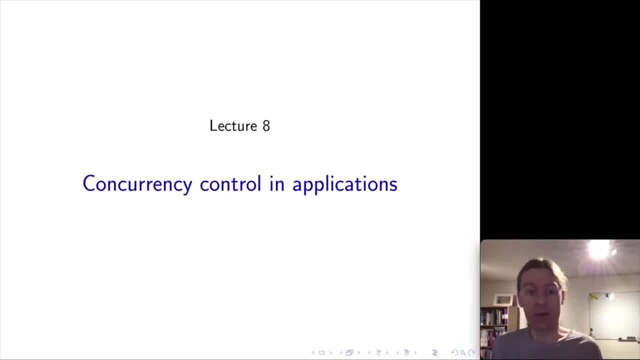 distributed systems lecture. This lecture we are going to look at some case studies of example applications, real-world software that uses the distributed systems concepts that we've seen in this course and, in particular, that has interesting problems to deal with around concurrency. So I'd like to start with 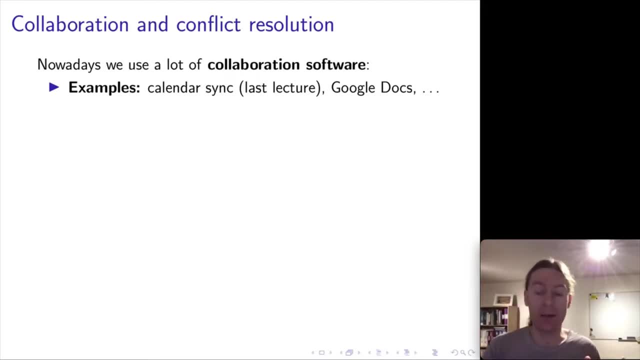 collaboration software. This is a fairly broad category of collaboration software, but you've probably used things like this before. What I have in mind are things like Google Docs, where you can have several people editing a document at the same time, or the calendar sync example. 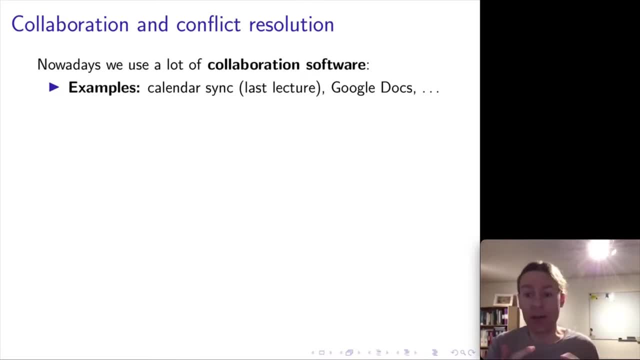 that we saw in the last lecture, where I can update some events on one device and have those synchronize over to another device, And many other applications that have this kind of similar collaboration built in nowadays, because it's just so useful to be able to work on something. 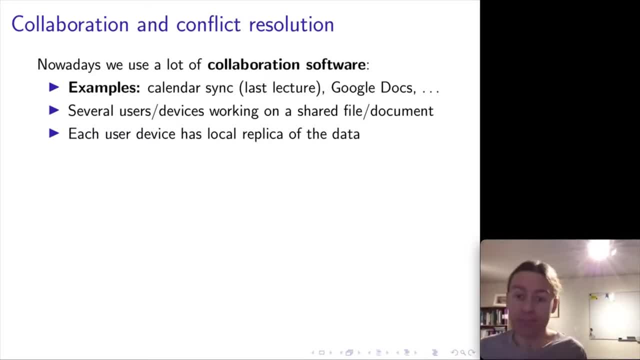 with your colleagues without having to email files back and forth, for example. So what these applications have in common is that there are several users, each user using some device to access some shared file or document or database. Each of these devices has its own. 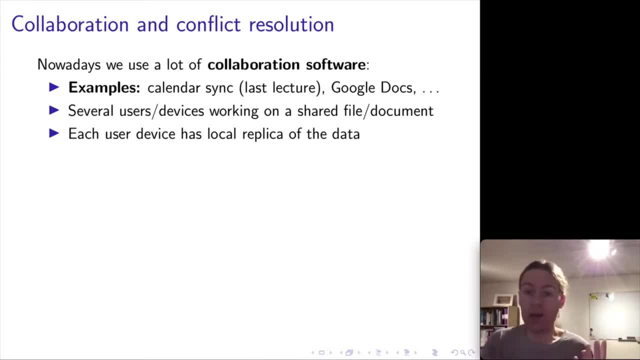 local copy of the data that it's working on. This might just be an in-memory, but we can still call it a replica of this shared data, And each user is able to update the replica of their own copy of this document, be it in their web browser. 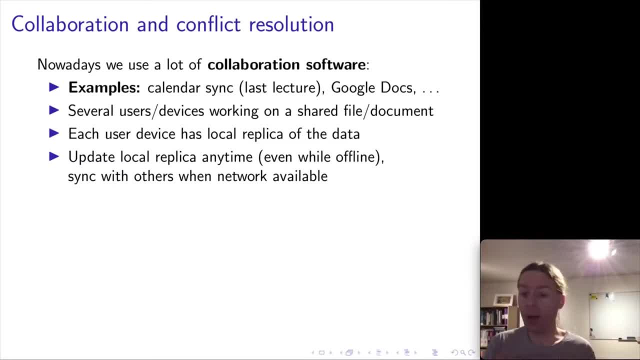 or in a mobile app or something like that. The user can update this data anytime, whenever they like, even if they're disconnected from the internet, ideally- And then sometime later, when they have an internet connection again, then they will sync back with the server. 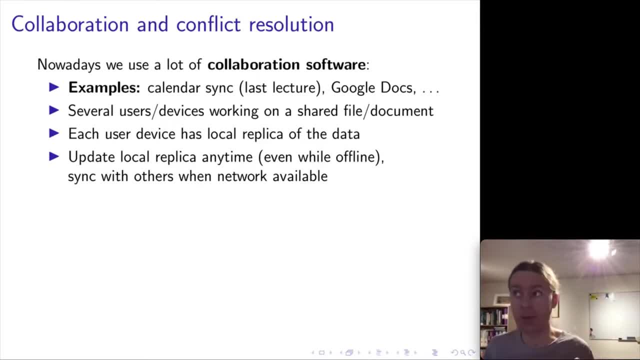 and with any other clients that have a copy of this document. Now the challenge in this is we can have several people concurrently updating the same document and we have to somehow reconcile those concurrent updates and make sure that everyone ends up in a consistent state so that the software. 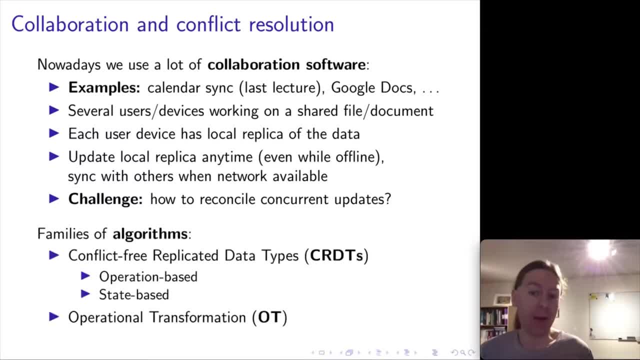 continues working as we might expect, And there are two main families of algorithms that are used in order to implement this type of software. One is conflict-free replicated data types, or CRDTs for short, and they come in two flavors: operation-based and state-based. 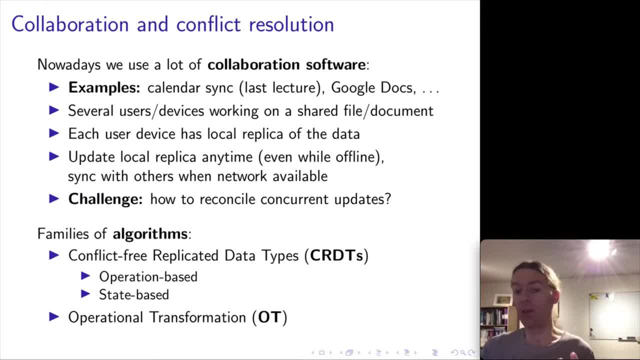 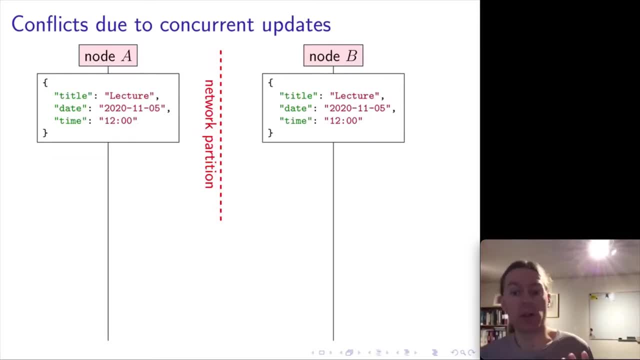 as I will explain shortly. And a second family of algorithms is called operational transformation, and you will see an example of that as well. So let's start with the example from the last lecture where I showed the calendar sync example. So I had my phone and my laptop. 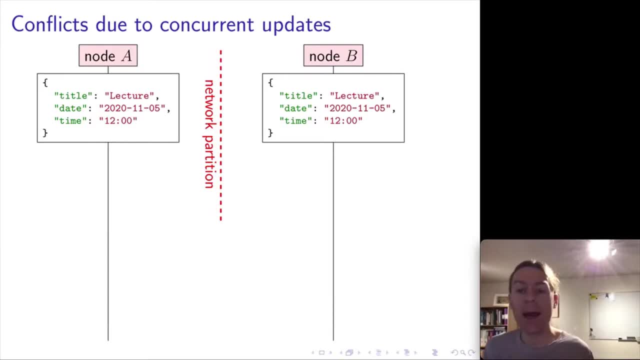 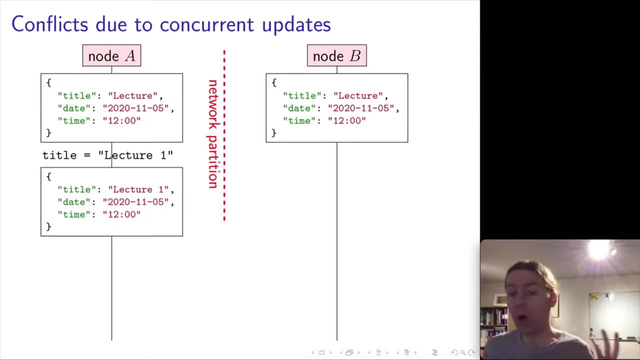 I had an event in my calendar saying a lecture on a certain date at a certain time and these two devices were disconnected from each other because I put my phone into aeroplane mode. So I update the title from lecture to lecture 1,. 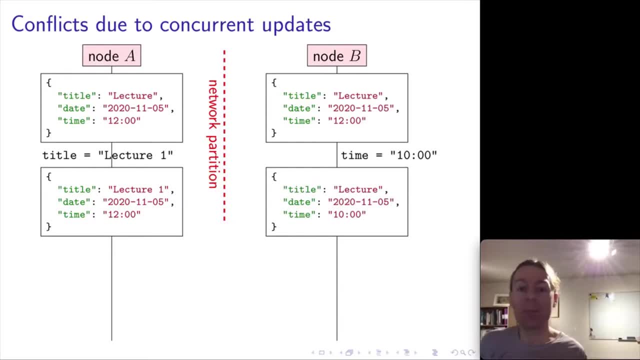 and while these two devices are disconnected concurrently, I update the time of the lecture on my phone to be 10 o'clock, And so now we have these two concurrent updates and sometime later the network is restored and these two devices want to sync. 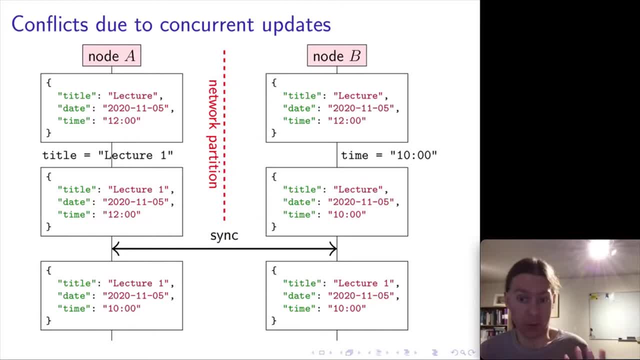 and we want to ensure that at the end we have the same information on both devices, that these devices converge, and ideally we would also like to not lose any data in the process. So in this example we have kept the update of the title. 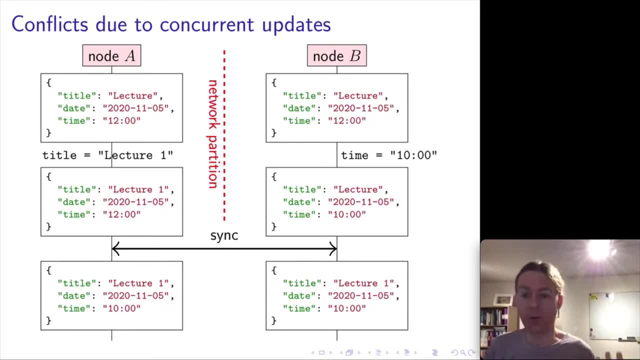 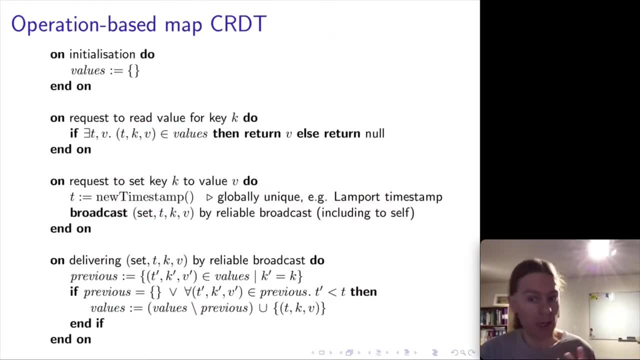 saying lecture 1, and we have kept the update of the time to say 10 am, and those two things have been merged together into a single update. So let's look at some algorithms that can achieve this. Conflict-replicated data types, or CRDTs. 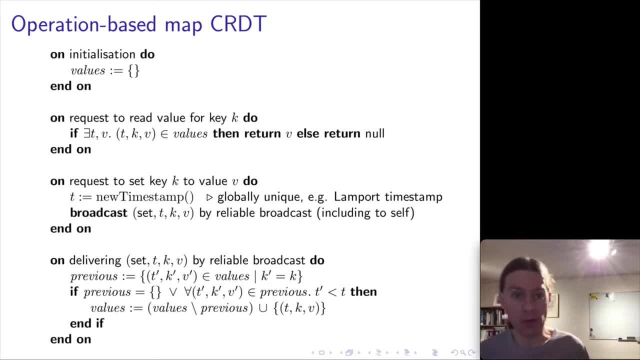 are, as I said, one of the types of algorithms you can use here, And this is an example of what is called an operation-based CRDT. You can use it in Java also, so you have this object-oriented interface that you are using. 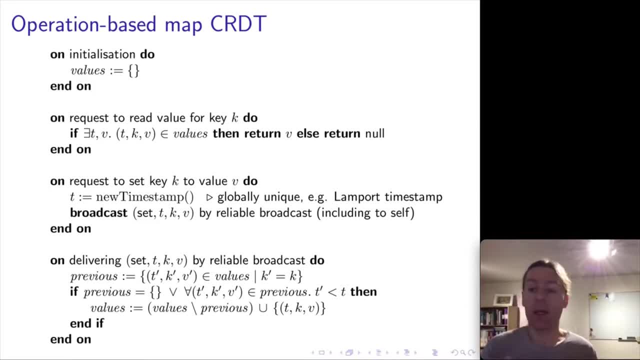 in order to represent your data and in this case, the data type that we have is a map from keys to values, So keys and values are not further interpreted. they could be strings or they could be numbers, or whatever we like, And the only property. 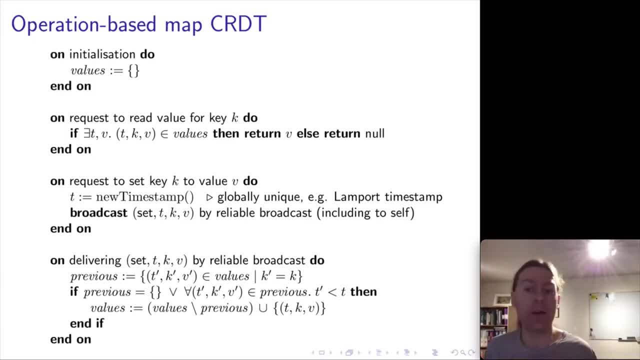 that we want to here ensure is that, for a given key, there is exactly one value, And so we can achieve this using the last-writer-wins approach that we saw in a previous lecture, And so the way you might do this is as follows. 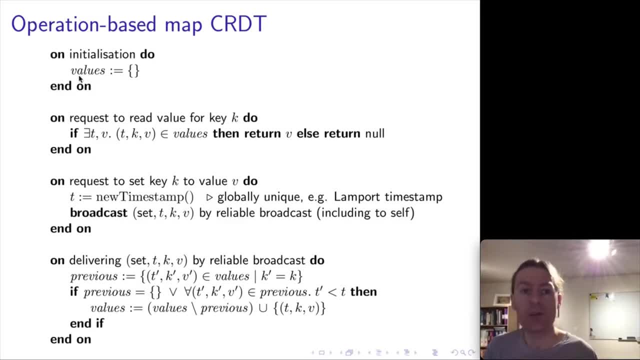 So let's say, when a replica initializes, it just sets up its own state to be this: variable values, which is just an empty set, And this set here is going to contain mappings from keys to values, and each mapping from a key to a value is also got an associated timestamp. 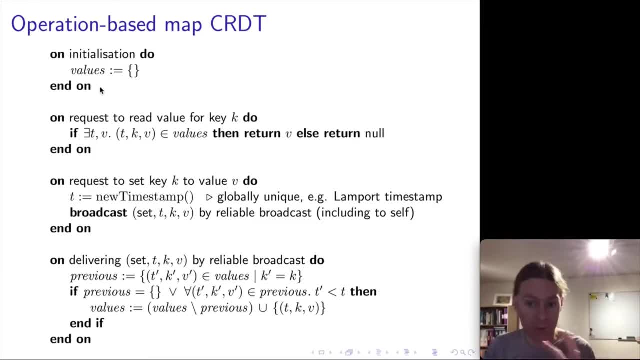 We can use a logical timestamp here, like a Lamport timestamp, and this will help us figure out which one is the more recent value. And so when we want to read the value for a given key, we just look for any entries in this set values. 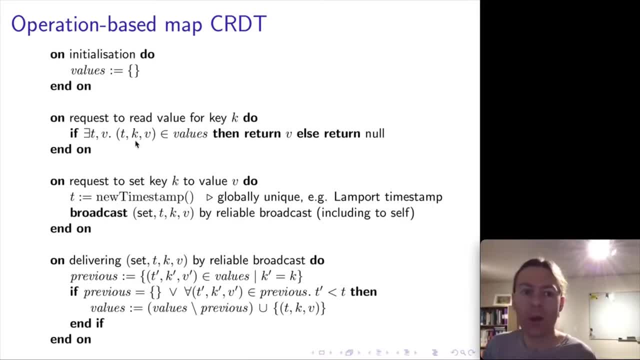 The entries are these triples of timestamp, key and value. So we look for any entry here for the given key with any timestamp, at any value, and if it exists we return that value, v, and if it does not exist we just return null, saying there is no entry for that key in the map. 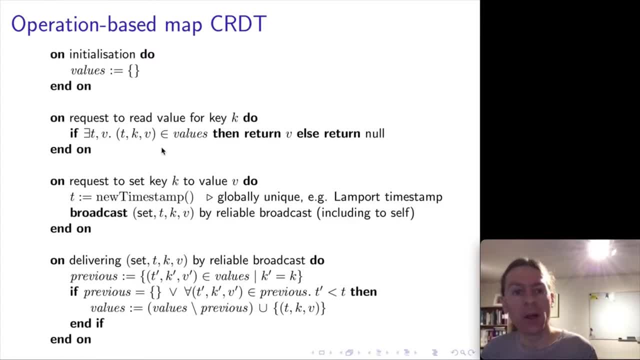 Okay, So this here works on the assumption that for a given key, there is at most one element in this map which the rest of the algorithm does ensure that particular invariant. So now, if we want to update the map, the way we can do that is as follows. 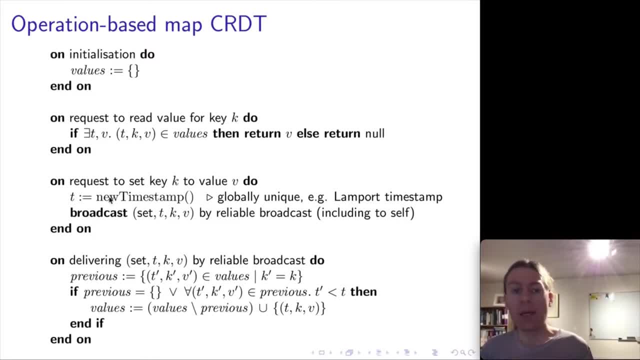 So let's say we want to set the key k to the value v. First of all, we make a new timestamp, and we can use a Lamport timestamp, for example, for that. What we do require is that this timestamp is globally unique, So we generate an identical timestamp. 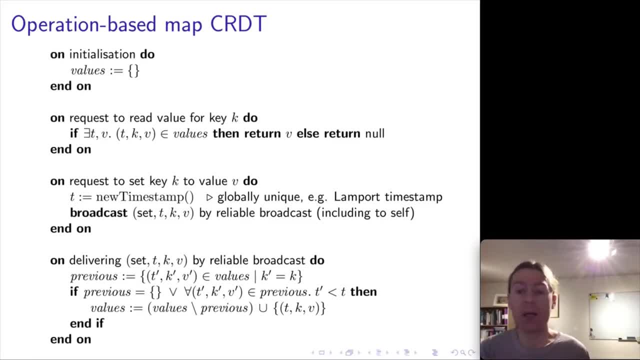 and, if you remember, the way we can do that with Lamport timestamps is by including the node id of the node that generated a particular timestamp and that will make it globally unique. So we're assuming this is just t the timestamp and now we're going to take 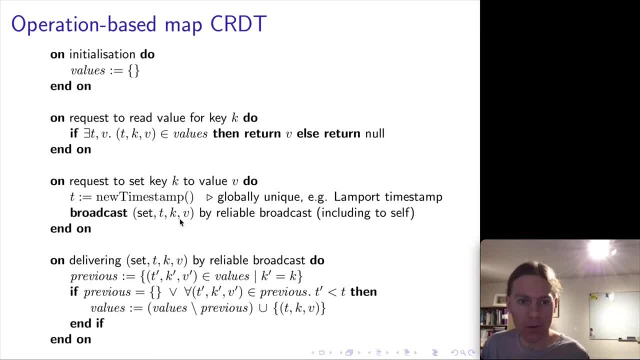 the key and the value that we were, that we wanted to set, and that timestamp that we just generated, packed this all together into a message and sent that via reliable broadcast. So remember that reliable broadcast means as long as any two nodes are not crashed, then they will deliver eventually. 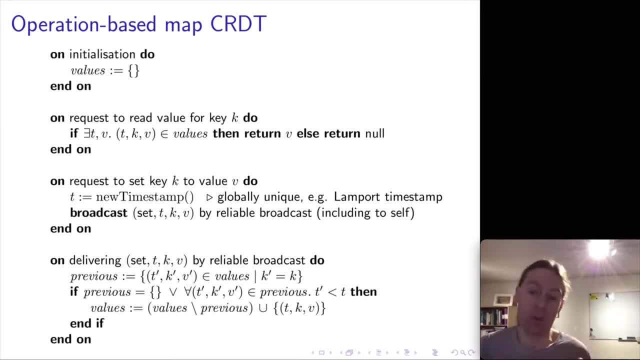 the same set of messages, but we're not making any guarantees about the order in which those messages get delivered And, in particular, this broadcast will also be delivered to the node that sent it itself, And that's what happens here. So when we deliver one of these messages, 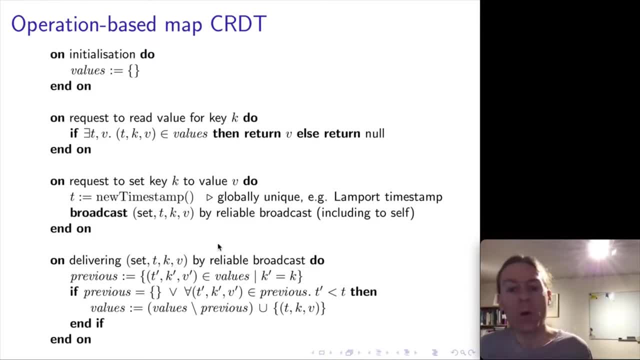 here via reliable broadcast. first of all, we figure out: are there any existing values in our set of values for the same key k? So we find any entries in this where the key of the entry equals the key of the update that we're making and we set that to previous. 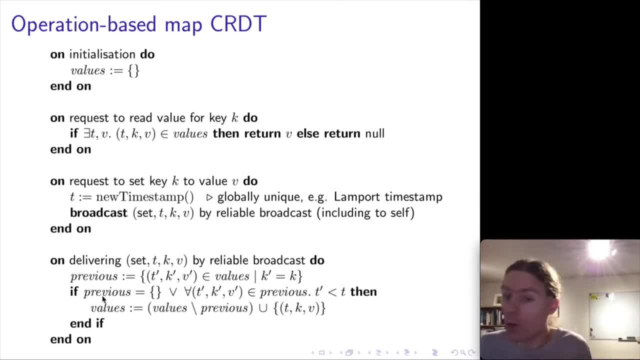 And so now this could be an empty set, if there is no existing value for the key k, in which case we go ahead. Also, we look at the timestamp of any previous value. So if there is a previous value for this particular k with a timestamp, 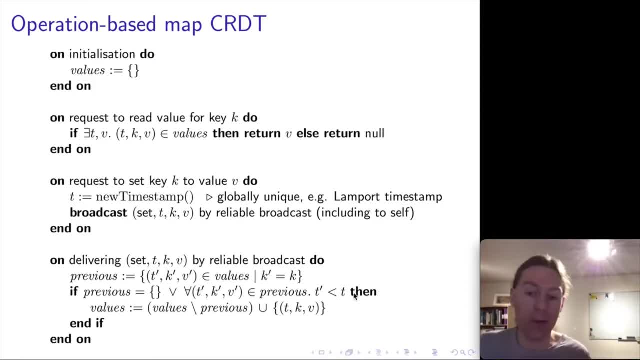 t' and if that timestamp t' is less than the timestamp t of the incoming update, then we overwrite it. So if this is the case- that either there is no previous value or the previous value has a lower timestamp- then we're going to remove the. 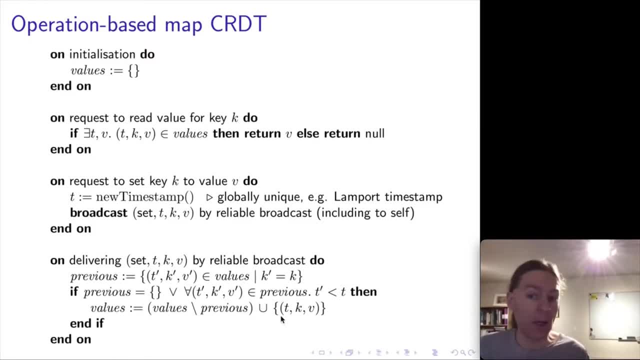 previous value from the set of values, and we're going to add the new mapping from k to v with timestamp t, to the set of values. Now, this ensures that there is up to one entry in the set of values for a given key, and so, therefore, this for all here. 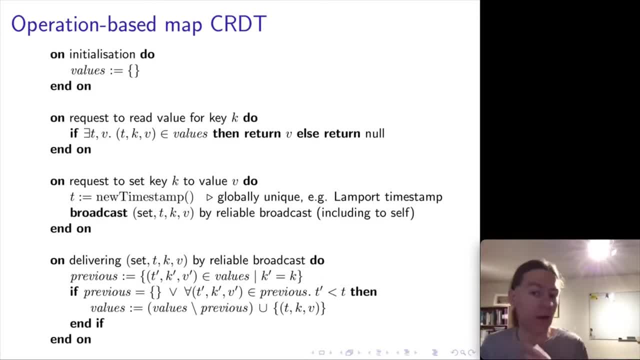 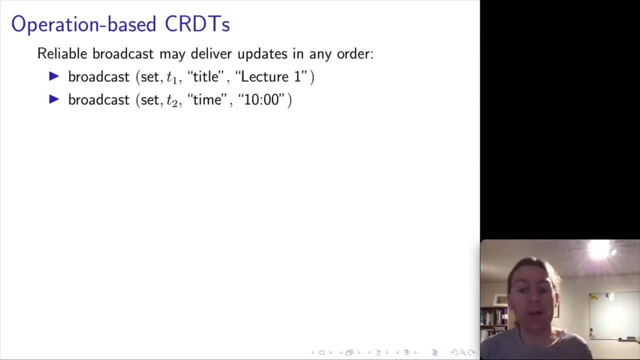 actually just means it's matching one particular item in the set, if it exists, And you know this is enough to ensure a strong eventual consistency. So the way that this algorithm works, as I said, is by broadcasting just these messages, and the messages describe what the key is, that's. 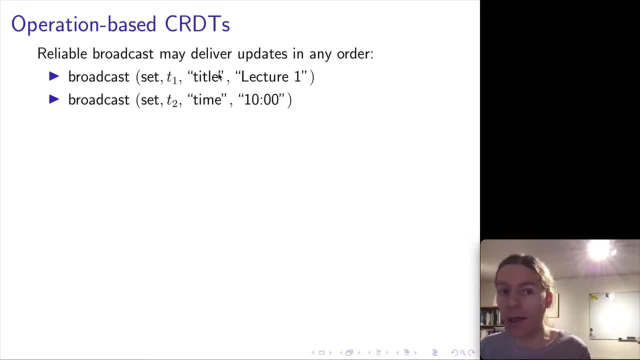 being updated and what is the new value being associated with that key? and so in our calendar example, the keys might be the field name, so title or name or date, and the value would, be well, the value that were associated with that particular field. Now remember what. 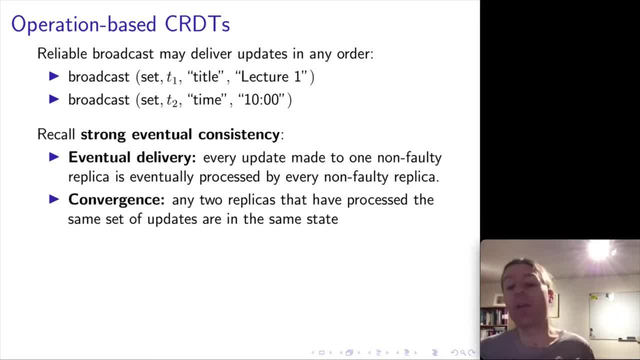 we talked about the concept of strong eventual consistency. This is exactly the consistency model that we want to ensure in an application like this, and strong eventual consistency consists of two properties. first of all, we want that every update is eventually delivered by every replica, as long as 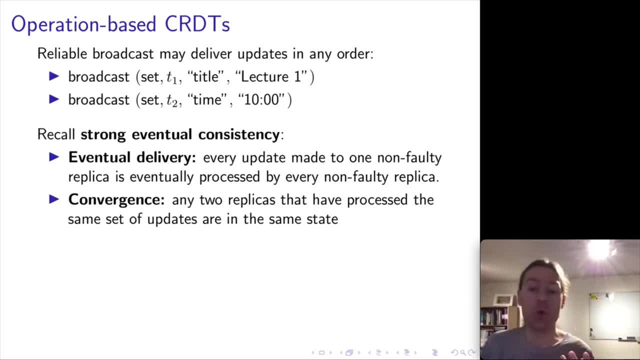 that replica is not crashed, and then, secondly, any two replicas that have processed the same updates must be in the same state. Now, the way we achieve the eventual delivery in this CRDT algorithm that I just showed you is by using reliable broadcast, and this is: 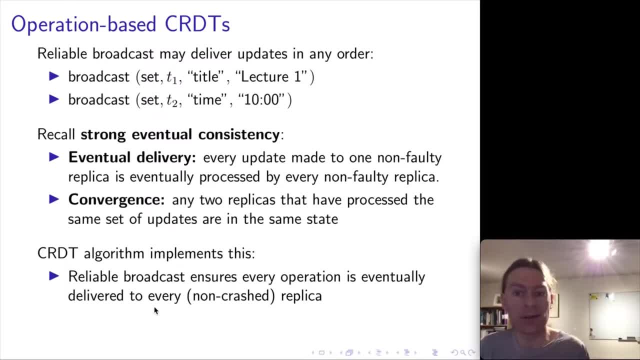 exactly what reliable broadcast ensures. it ensures that any two non-crashed nodes will eventually deliver the same set of messages. Furthermore, the process for updating a replica's state when it delivers one of these messages by reliable broadcast. this process is commutative and which means that we can apply. 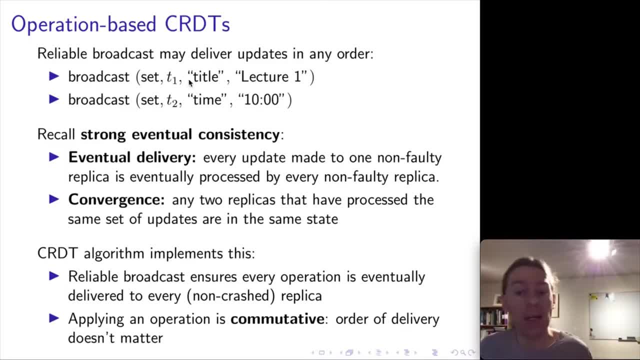 these various operations here in any order, and the final outcome will be the same. So this might require a little bit of thinking, and there's an exercise in the lecture notes asking you to actually prove for this particular algorithm that the process of applying an operation really is commutative. 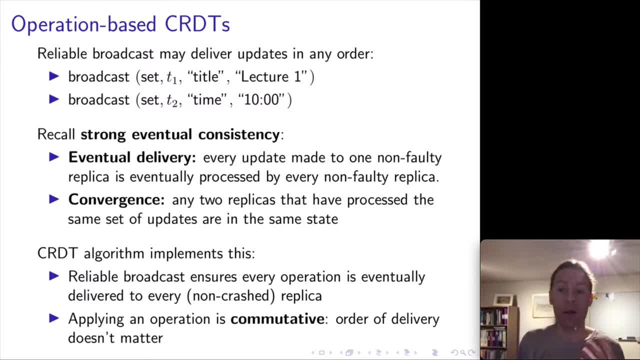 Now this is called an operation-based CRDT. It's an example of an operation-based CRDT because the things that we're broadcasting are operations, so it's one operation at a time in each broadcast. So this does require the broadcast to be reliable, because 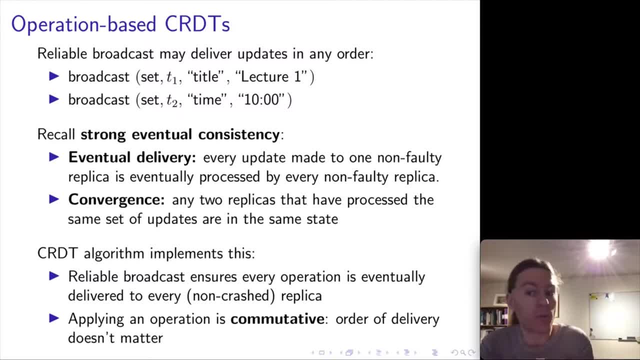 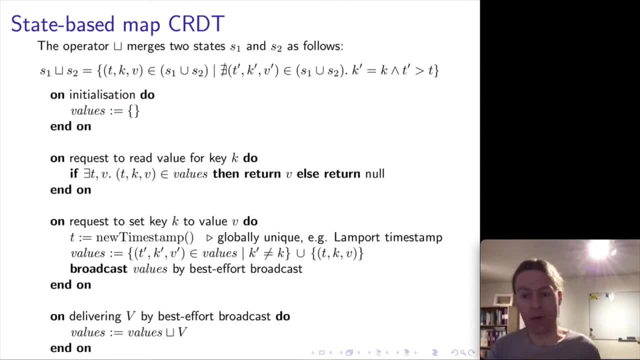 otherwise, if you're missing a message, then you will never end up in a consistent state with the other nodes, necessarily. There's an alternative construction for CRDTs that we can use, which is called a state-based construction, and here's an example of exactly the same. 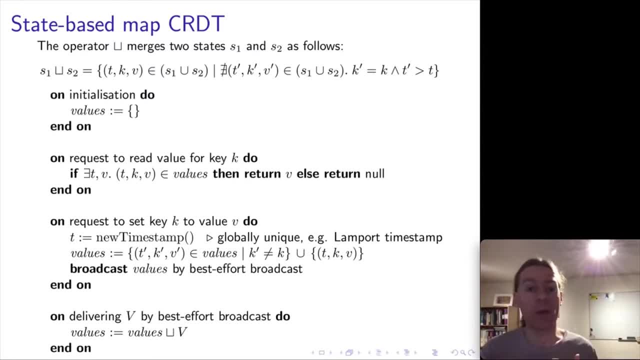 data type, but implemented in a state-based way rather than in an operation-based way, And so with a state-based CRDT, you always have a merge operator or this merge function, which is usually written as like a set union operator, but square rather than round, And 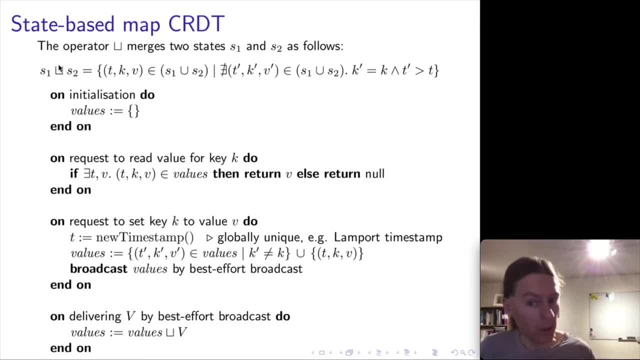 this merge operator here must satisfy several properties that I will explain on the next slide. And in this particular algorithm we will define the merge operator like this. So the merge operator is going to take two sets of values, in this case S1 and S2.. These are sets of values. 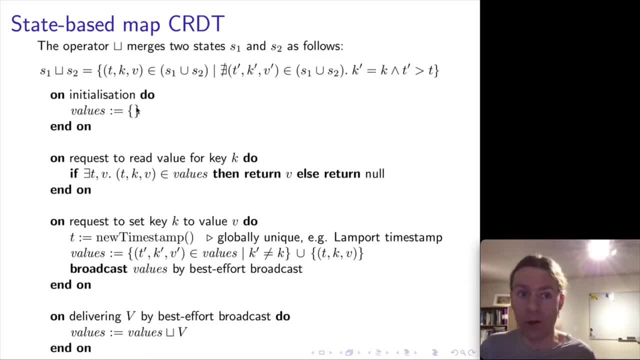 of exactly the same form as we had in the operation-based version, that is, their triples of timestamp, key and value. And in order to merge these two sets of values, we're going to take the set union of S1 and S2,, take all of the triples. 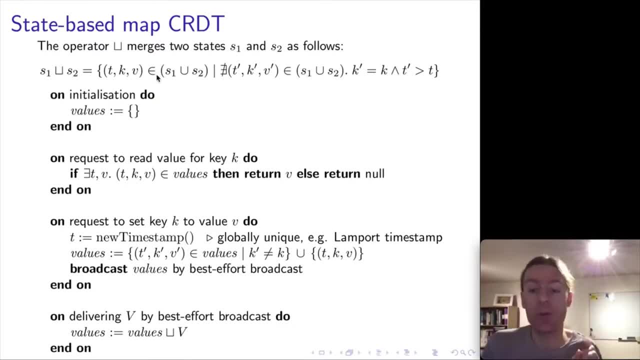 in there and then for every given key we're going to keep only the value with the highest timestamp and we're going to throw away any older timestamps for that particular key, And that's implemented by this logic here. So for every given triple, we keep only those where 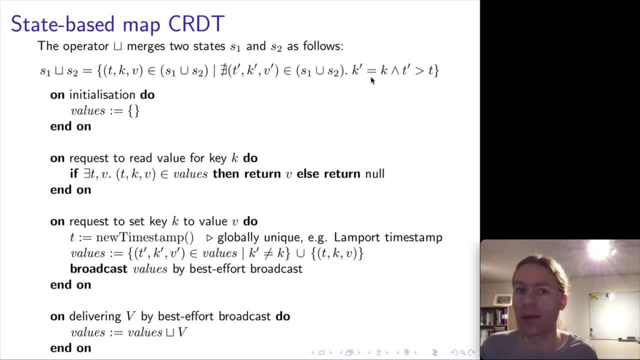 there does not exist another triple in the same set that has the same key but a higher timestamp, And the effect of this is that we keep only the highest timestamp for every given key. Okay, so, given this merge operator here, now the rest of the algorithm. 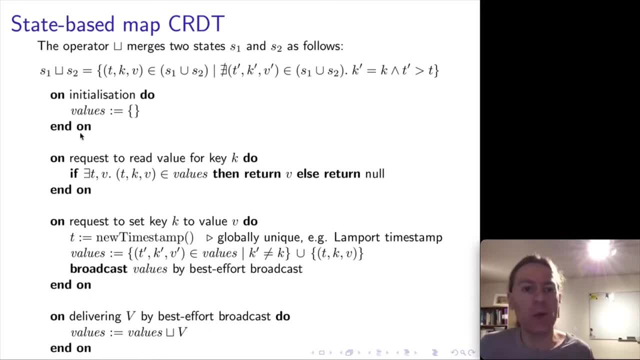 this looks kind of familiar. So the initialization is exactly the same. we initialize values to the empty set. The processor reading a key is exactly the same as previously, so that is given a key. We try and find any triple with that key in the. 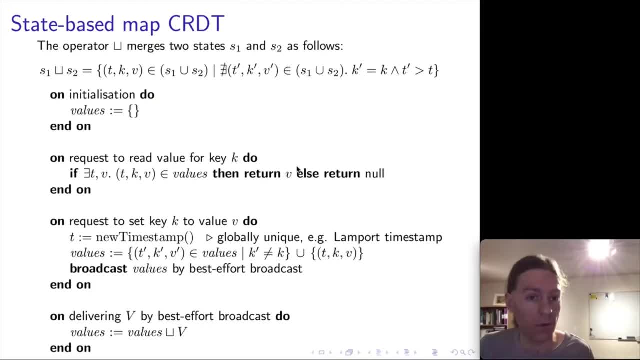 set values and we return the value from that triple, if it exists. Now the process for updating the value for a given key. This is different, And so here, as before, we have- we generate- a new timestamp. can be a lamp or timestamp, as before. 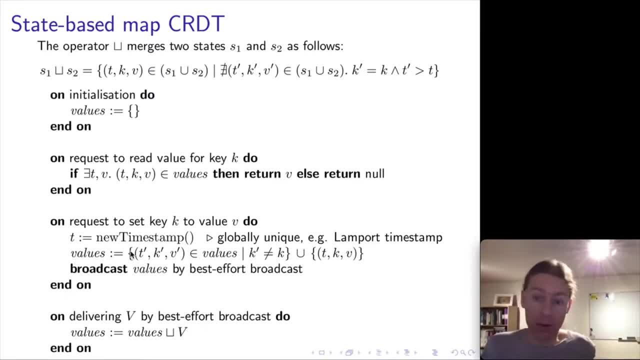 and now, rather than broadcasting this operation, we're just going to update the set of values directly. And so we're going to update it in such a way that, given the set of values, we remove any existing entries with the same key, k, which may be none if there is no. 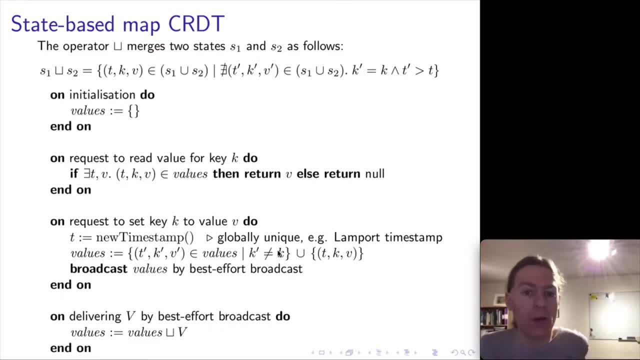 previous entry. but whatever current entry with key k exists, we're going to remove it and then we're going to add this new triple with the new timestamp, the new key and the new value. we're going to add that to a set of values And now we're going to broadcast. 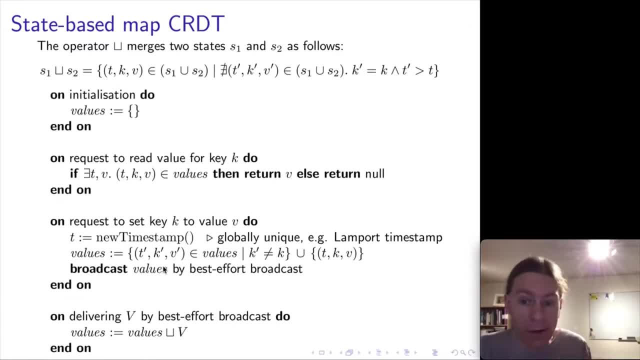 this entire set of values to any other replicas. so, rather than broadcast the operation, we're broadcasting the entire state of the replica, which is here. this value values, and this is why it's called a state based CRDT, because the thing we're broadcasting are these values. 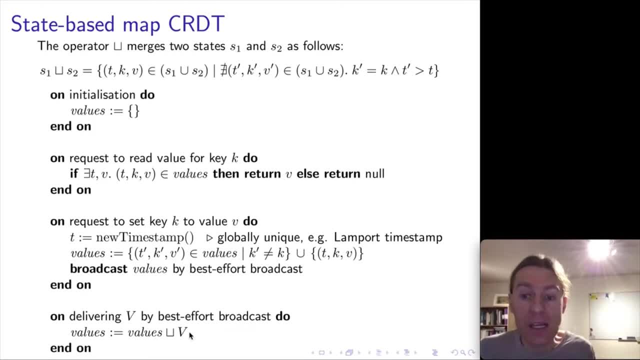 And now, when this set of values- capital V here- is delivered, we use the merge function in order to merge that with the recipient's set of values, And so this means you've got these sets of values flying around which may be delivered in arbitrary orders, and 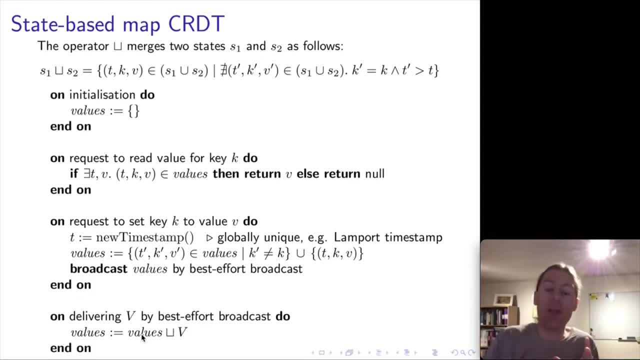 the end result is just: we keep each replica. when it receives one of these set of values, it just merges it into its own local state and, as a result, it keeps just maintaining the state that is, the latest version of whatever has been flying around. So the interesting thing to note here is that I 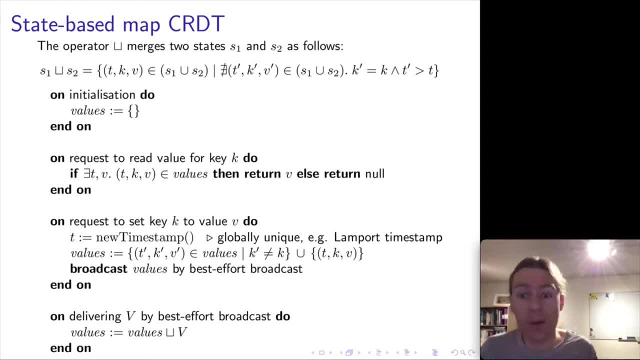 said that we can broadcast by best effort broadcast rather than by reliable broadcast, and this is indeed a distinction between the state based approach and the operation based approach, as we will see in a moment. So first of all, about this merge operator. So this merge operator. 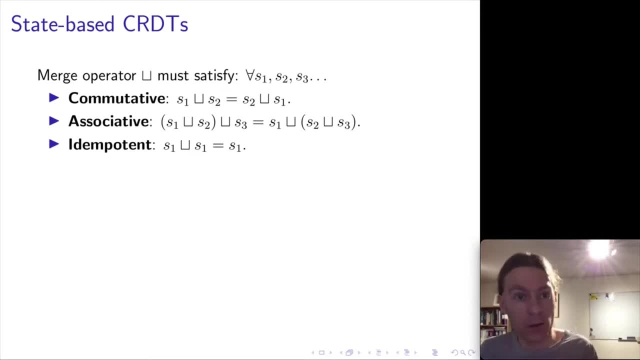 for it to work correctly, it must satisfy several conditions: It must be commutative, which means we can swap around the order. It must be associative, which means you can swap around the brackets. and it must be idempotent, which is the behavior that, as we saw, 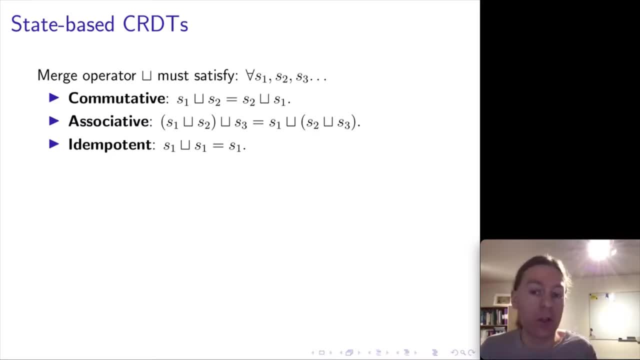 before. you can merge a state with itself and that does not change anything. And if we have a merge operator that satisfies these constructions, they then we can build a state based CRDT out of it, simply by broadcasting the states and merging them whenever we receive a state from another replica. 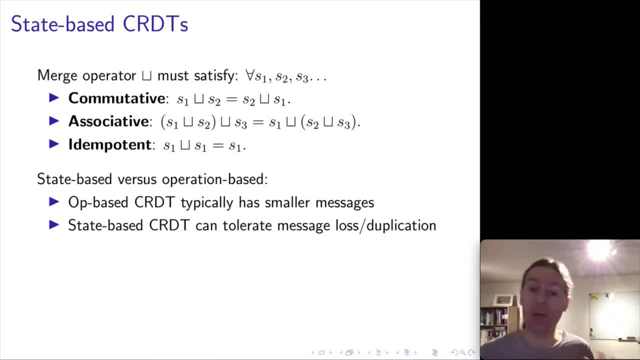 Now there is a trade off here between operation based and state based CRDTs. So as we saw with the operation based CRDTs, the broadcast messages contain just a single operation. so those messages containing just one operation are usually quite small, so they are quite efficient in terms of network traffic. 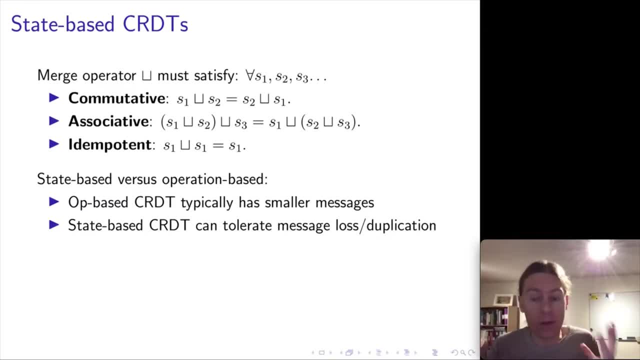 because, compared to the state based approach, where a replica needs to broadcast its entire state, that might be a much bigger amount of data. Imagine a key value mapping that has lots of keys in it. You're going to be sending all of the keys and all of the values associated with. 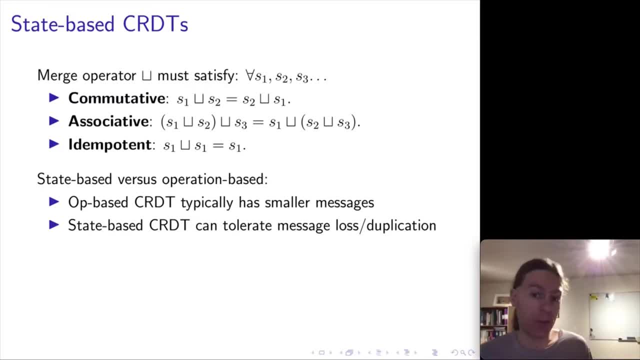 them in every single message. So here the advantage of the operation based approach is that it has smaller messages. typically State based approach has larger messages, but it can tolerate messages being lost and- this is quite interesting here. It can also tolerate duplication, Duplication. 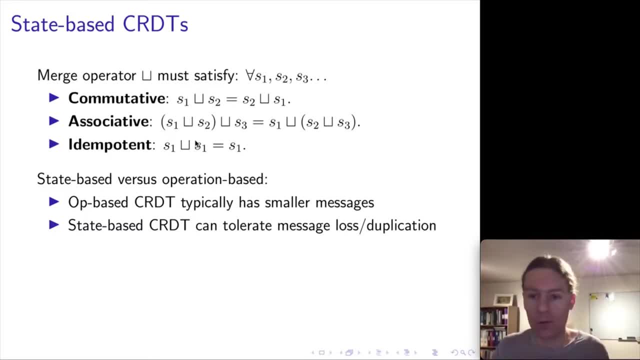 is easy because we have idempotence in the search function. therefore, if you receive duplicates, you'll just do nothing. But even with message loss, it can tolerate this because the entire state is encoded in every single message. So if you miss a message somewhere along the way, 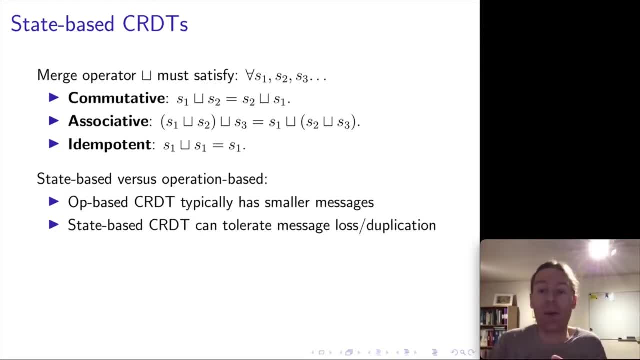 as long as you receive some later messages, that later message will supersede any previous messages anyway, and this actually ensures then that you will get convergence of the replicas, even if you've missed some of the messages in the middle. And so this is quite nice now, because 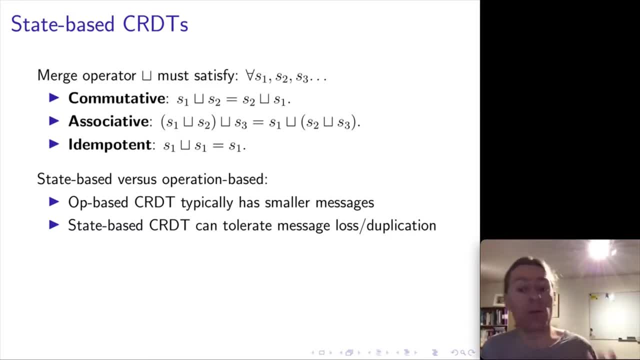 with state based CRDTs. you don't need to involve the costs of a reliable broadcast protocol because the CRDT itself can deal with unreliability. Of course, if no messages are ever delivered then it won't converge. but as long as eventually some of the 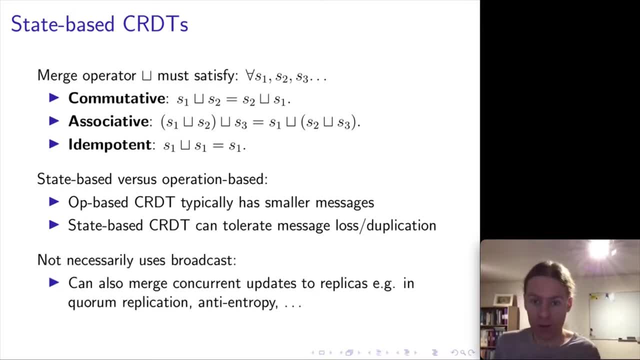 messages get through, then you can still get convergence properties. Another nice thing about state based CRDTs is here. I wrote it based on a replication protocol, based on a broadcast, but you can actually use it in other forms of replication as well, where it's not actually a broadcast protocol. 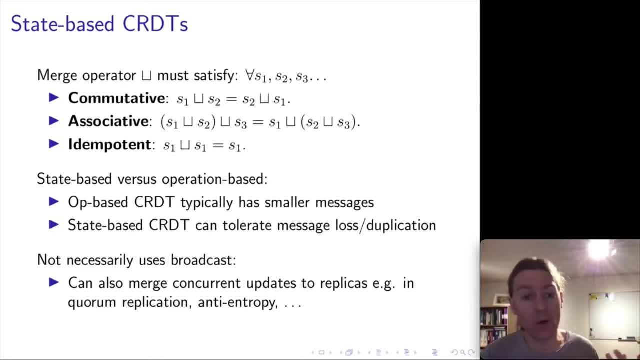 but if you remember back lecture 5- I think it was on replication- we had these ideas of quorum replication, where a client sends an update to a quorum of replicas and then maybe the replicas have an anti-entropy protocol amongst themselves in order to try and 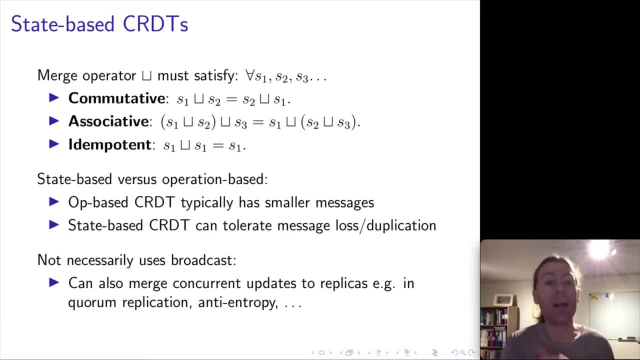 resolve any differences in the updates that they've seen, and state based CRDTs work very well in this particular setting as well, where you've got these replicas that want to exchange their updates through some kind of anti-entropy protocol. Okay, so this has been an example. 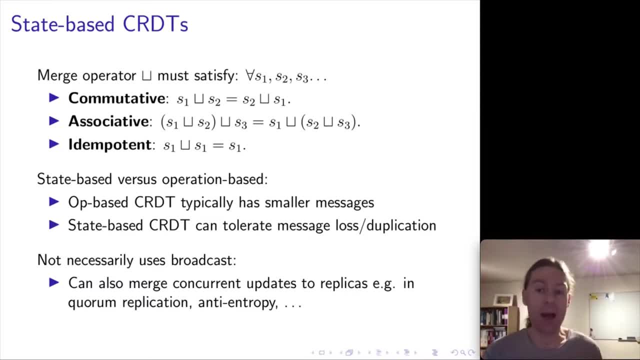 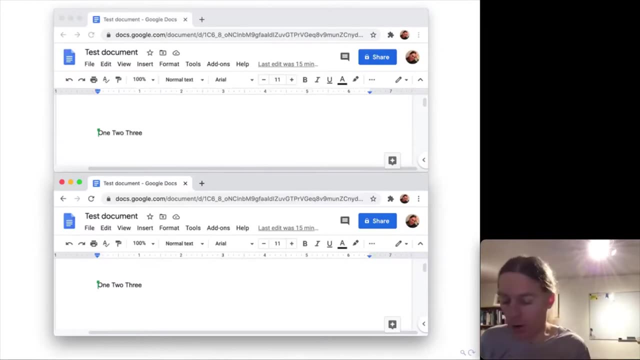 of a map, CRDT, so our data type was a map from keys to values. We can construct this kind of concurrency control for other types of applications and other data types as well, and so one interesting one to consider are collaborative text editors like Google Docs. 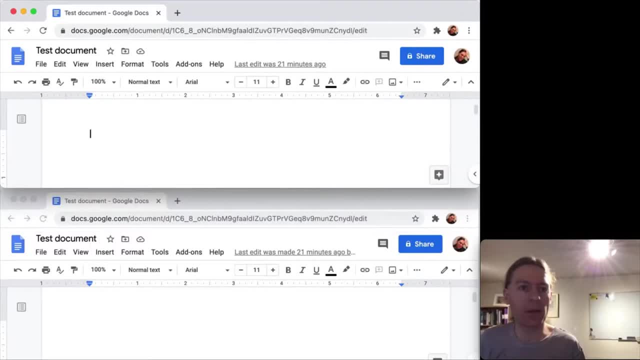 So let me give you an actual demo of this. I think this makes a bit more interesting. So I have here two windows of Google Docs and you can see if I type in one of them, this appears in the other window and I can go down here and I can add a smiley. 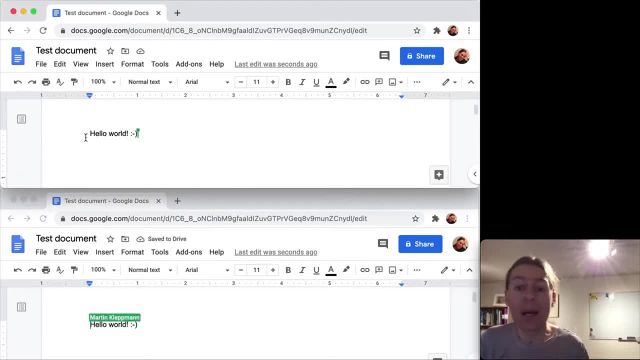 and this will appear in the top window as well. So far, this is probably familiar. you've probably used this kind of software before. Now the interesting thing is what happens if these devices get disconnected from each other for a little while. So let's. 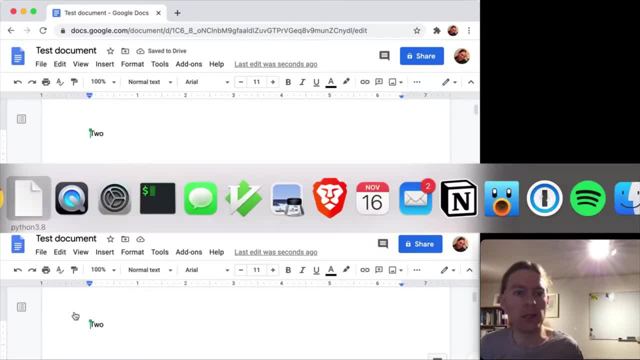 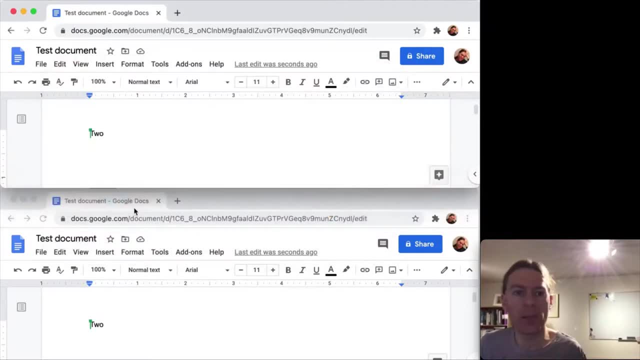 set things up like this. so I write the word 2 here and I'm going to go into my network settings and I'm going to fiddle with the network to drop all of the network packets. and so now these two apps will still work and at the top I can type: 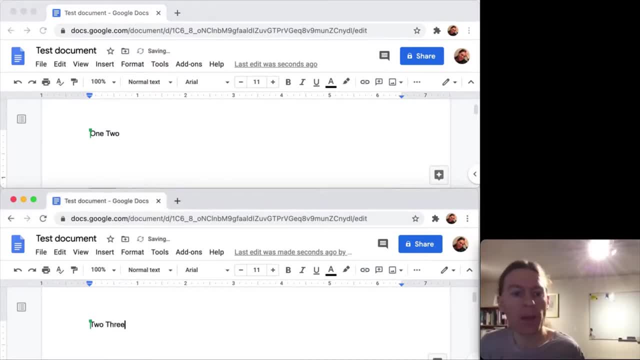 1, 2, and at the bottom I can type 2, 3. and Google Docs hasn't realized yet that my network is disconnected, so it's just happily letting me type here. but you can see that the two copies of the document have diverged, so they 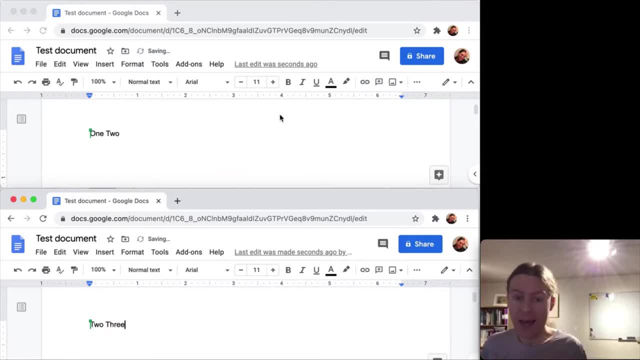 ended up being temporarily inconsistent with each other and as the network connection is repaired, we will want those to end up back in a consistent state. so let's say, I repair the network and you can see exactly what has happened. so Google Docs has been able to merge these. 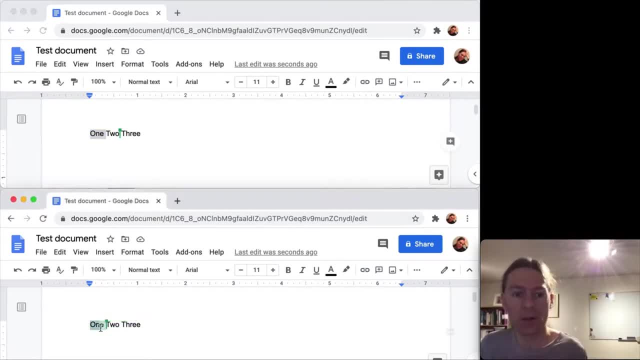 updates. so the addition of 1 has gone down and been added to the lower document and the addition of 3 has been added to the top document. so we ended up with 1, 2, 3 as a merged result automatically. you know we didn't have to do any conflict resolution here. 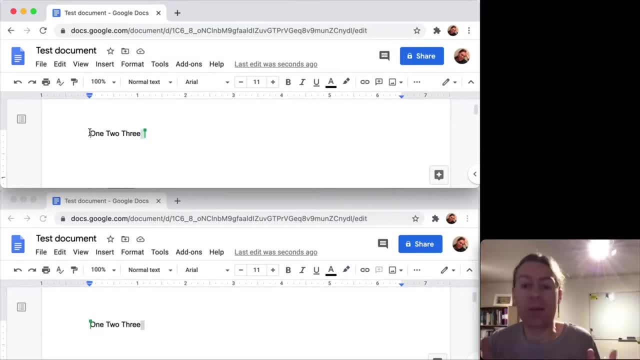 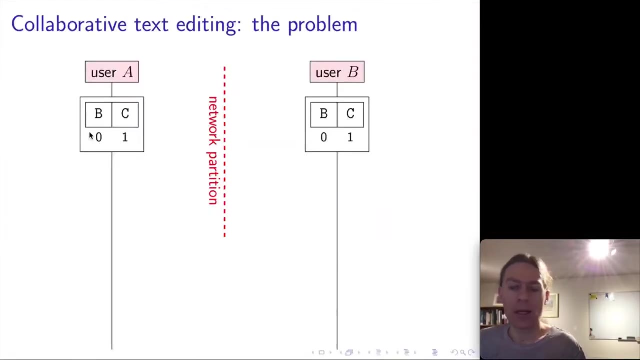 or do anything. particular Google Docs just figured out by itself what we wanted and just gave us the merged document automatically. so let's look at some algorithms that can achieve this kind of collaborative editing, and let me show you by an example the problem that arises when we try to build this kind of 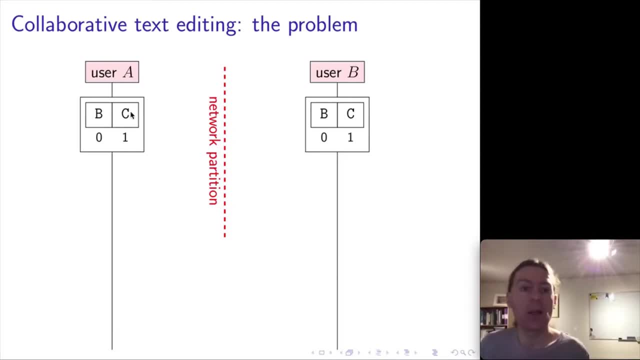 collaborative editing software. so let's say we here have got a document consisting of two characters, b and c, and we're going to allow users to edit this document by inserting and deleting characters, and we're just going to deal with the document one character at a time, just. 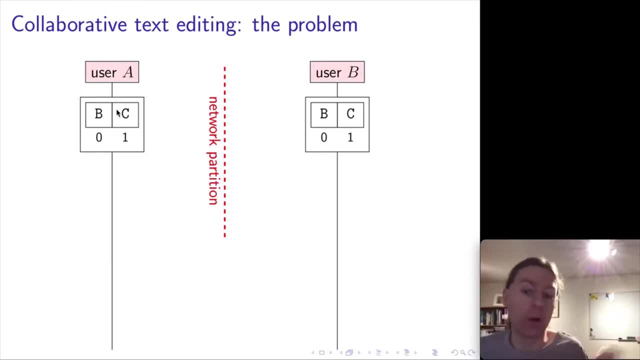 like Google Docs, you know, every single keystroke adds or deletes one character in the document typically, and so we've got user a and b. they start off with this in the same state, with a document containing b at index 0 and c at index 1. now 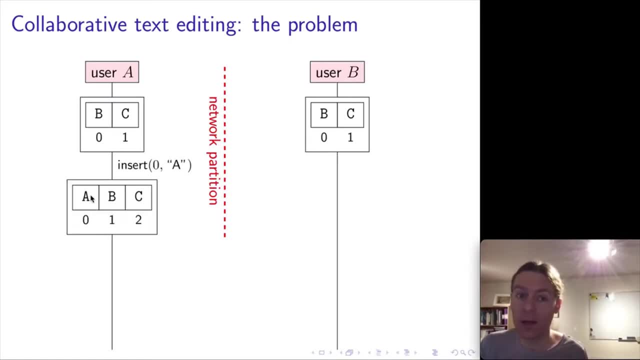 let's say on. user a wants to insert the letter a at index 0 in this document, and the result then of course is that b ends up at index 1 and c ends up at index 2, so the indexes get moved along by one, let's say concurrently, while 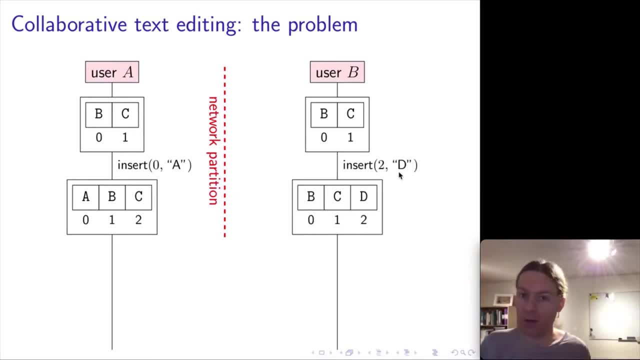 this is happening. the user b wants to insert the letter d at the end of the document. so this is just like the example I just showed you with Google Docs, with the 123, except with individual letters. and so here letter d gets inserted at index 2, as we expect. 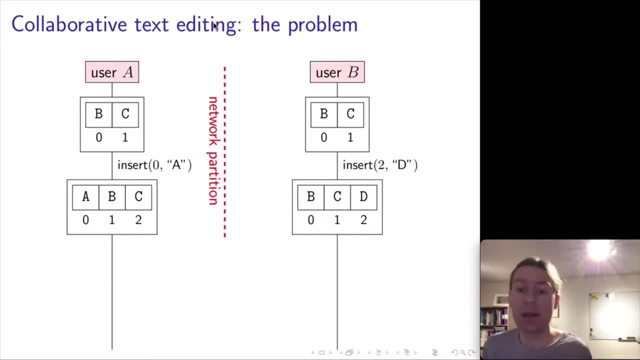 now let's try and synchronize these two. so let's say, now the network is repaired, the two nodes can connect to each other again, and so user a is going to send its operation, insert a at index 0, going to send that over to user b and user b 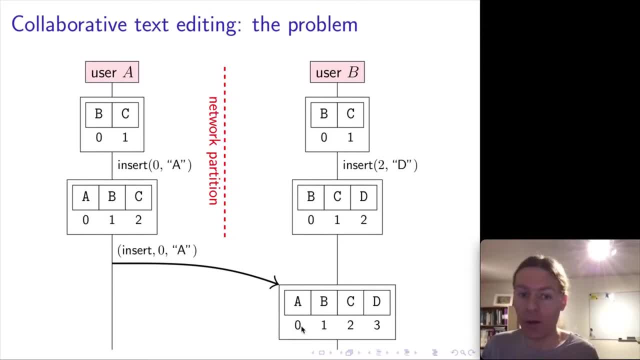 is going to apply that. so user b is going to insert the letter a at index 0, and we will end up with the document a, b, c, d, which is exactly what we wanted in this case. so that has worked fine. let's look at what happens if we go in the reverse. 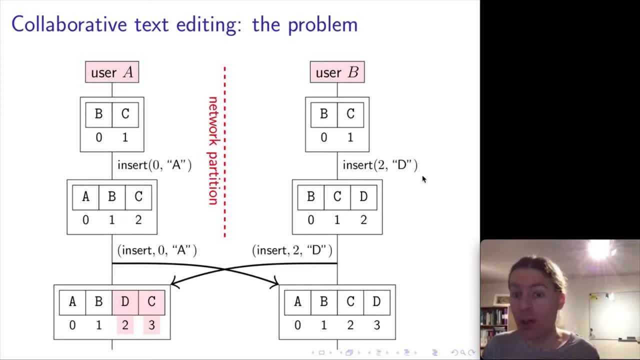 direction. so in the reverse direction, we take again the operation that happened. so in this case it's insert the letter d at index 2, we send that over to user a, and user a inserts d at index 2 and oh no, things have gone wrong here, because if you look what. 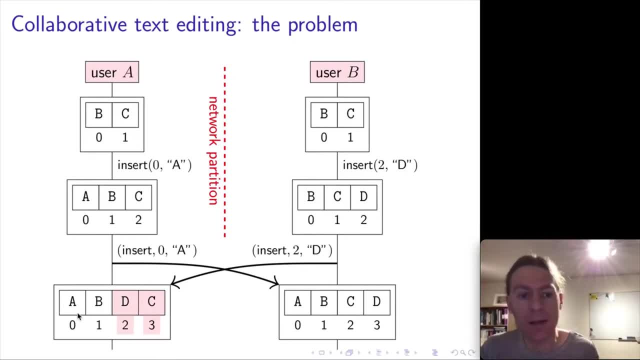 has happened here. we are on the left, user a, we have ended up with the document a, b, d, c, whereas on the right, we ended up with the document a, b, c, d, and the two users are now inconsistent with each other. this is not what we wanted. 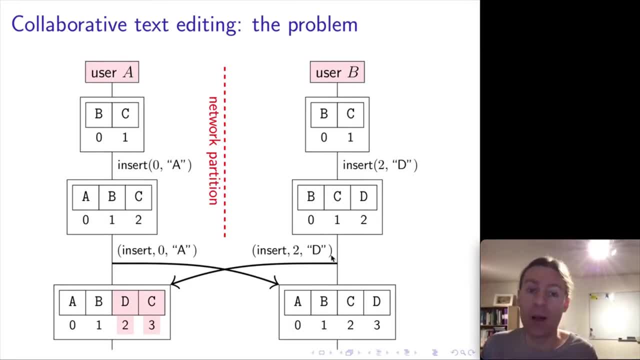 and the reason why they have become inconsistent with each other is, well, the problem with this insertion of d at index 2. here the problem with this operation is we can't just directly apply that operation here on the left hand side, because index 2 no longer has the same meaning. 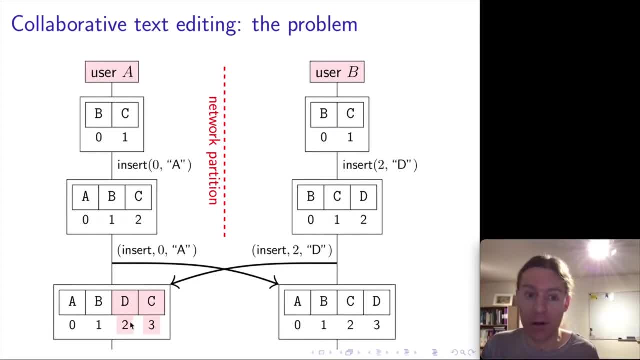 because we concurrently performed this insertion at index 0. really, the insertion here of d should have happened at index 3, not at index 2, so we have to now deal with the fact that this concurrent editing has happened and adjust the indexes accordingly. and this is exactly what. 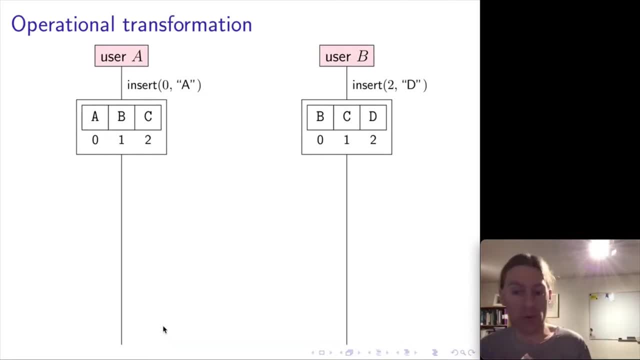 operational transformation does so. operational transformation is a family of algorithms that deal with exactly this problem of several people concurrently updating a text document, and they deal with it by transforming the operations, as the name says. so we have the operations, which are recorded as before, just like one character at a time. 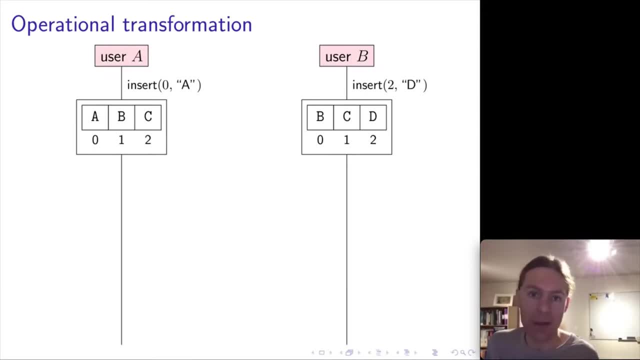 insert or delete. and so we have the insert of a at index 0 and the insert of d at index 2. and now when the operation, let's say this: index d at index 2, insert d at index 2, when this gets sent over the network to user a. 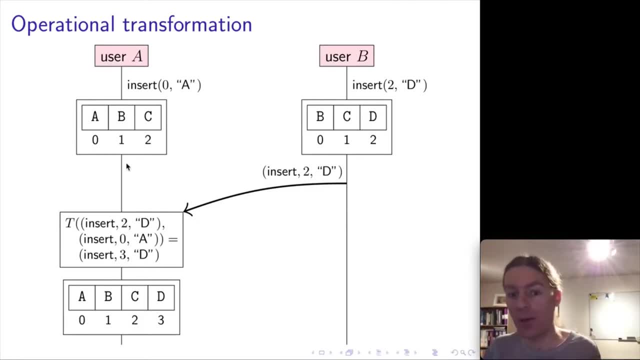 user a is first going to check any operations that were concurrent with this particular operation, and here it knows that its own insertion of a at index 0 was concurrent, and so it now calls this transformation function t, this capital t. here is the transformation function. it takes two operations. 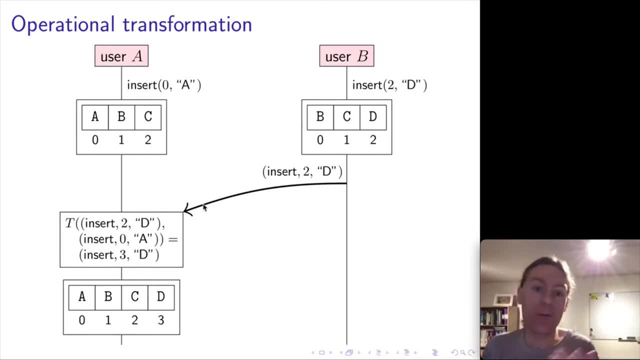 the first operation is the operations just received from the network, and the other operation is its own operation that is concurrent with the received operation, and based on these two, it returns a new version of the received operation that is transformed relative to this concurrent operation, and so, in this case, here the 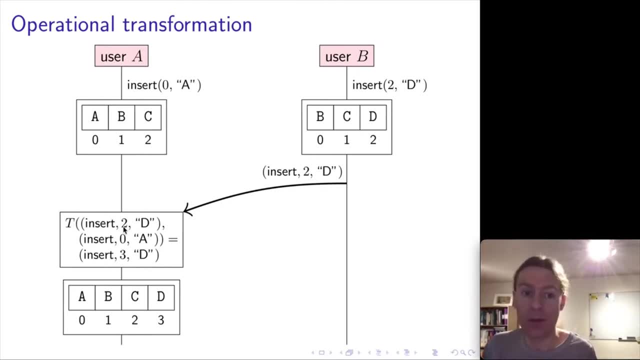 transformation function t is going to take as first argument the insertion of d at index 2 and it's going to return a transformed version of this same operation which is realizing that, okay, we've had this concurrent insertion at 0. this means we have to increase. 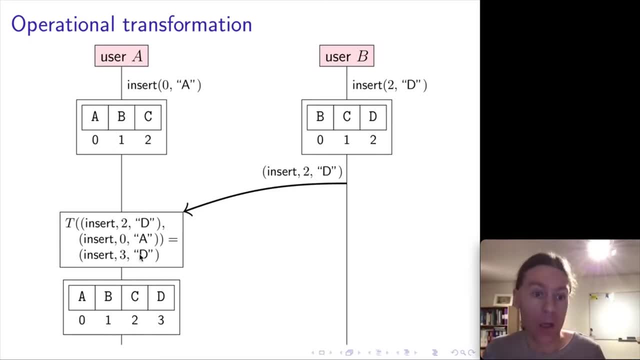 the index of the insertion of d by 1, and so therefore the result of this transformation function t here is that we now perform the insertion of d at index 3 rather than at index 2, and if we perform the insertion at index 3 now, we have the document abcd. 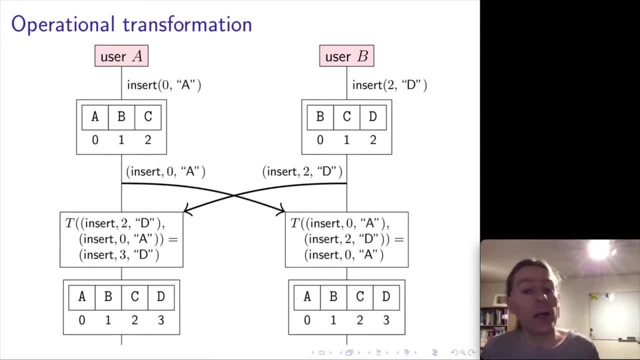 which is exactly what we wanted. going in the opposite direction, here, the insertion of index of a at index 0 also gets transformed with regard to the operation that is concurrent on user b's side. so the transformation goes just the other way around, because they detect the same concurrency. 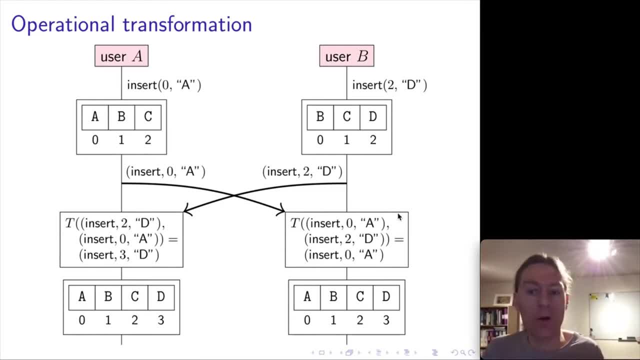 relationship between these two operations, probably using vector clocks or something like that, and in this case, here this operation of index 0 does not get transformed, because in this case the concurrent operation is further along in the document, it's further to the right and so therefore it doesn't affect the index. 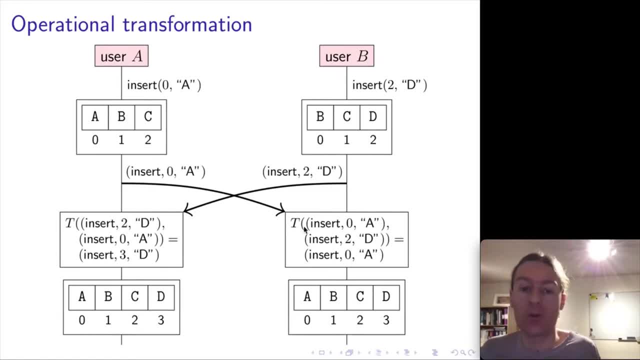 of this operation that happens earlier in the document and therefore this transformation function here returns the unmodified insertion of a at index 0, and here insertion a at index 0 is applied and we end up with the document abcd, as we expected. so I'm 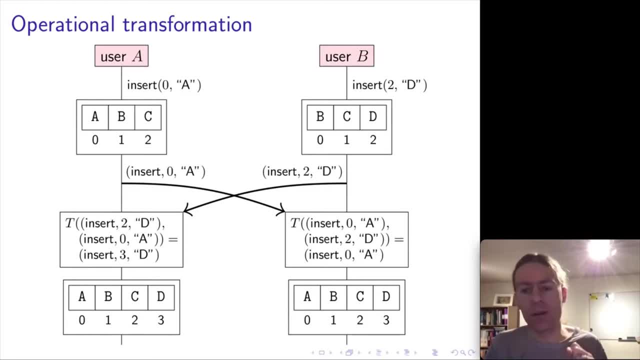 not going to run you through the full operational transformation algorithm because the details are actually quite fiddly and it gets quite messy and we don't really have time to talk about that. but this is the basic idea of how the algorithm works. now one downside of operational 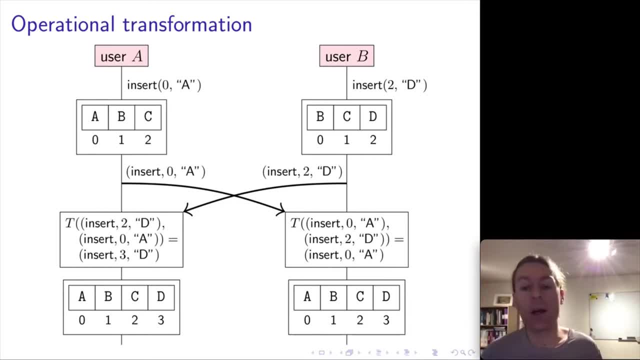 transformation algorithms is that generally they require total order broadcast as the mechanism for communication between the users. so even though a user can immediately apply updates to their own local copy, it relies on the network broadcast delivering the updates or the operations to all of the users in the same order. 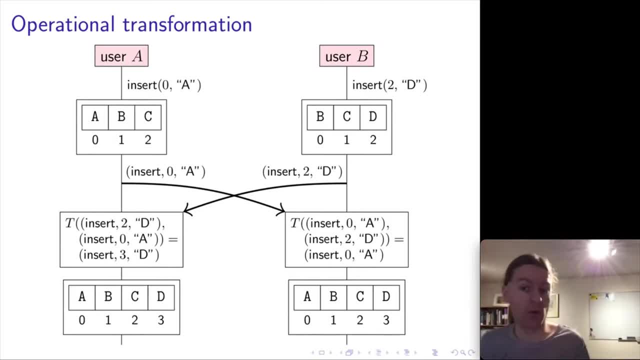 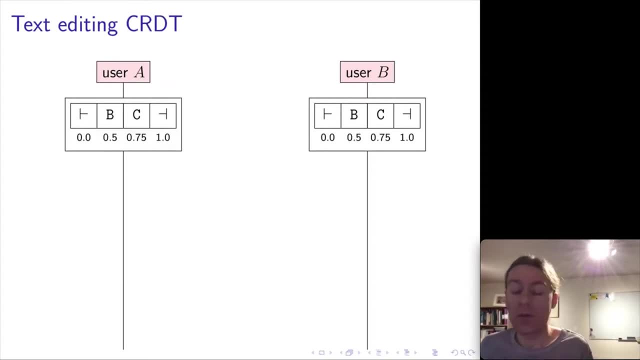 and so this means we do have all of the costs of total order broadcast associated with making operational transformation work. there's an alternative, which is to use a CRDT, and so CRDTs have the property that they don't require total order broadcast, in this case this particular CRDT. 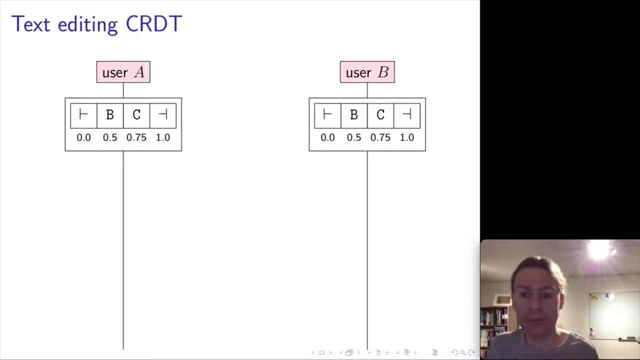 will require causal broadcast. I'll show you the algorithm in a moment. first the concept of how it works. so the real problem that operational transformation have to solve is the fact that the indexes don't have the same meaning if there are concurrent insertions or deletions. 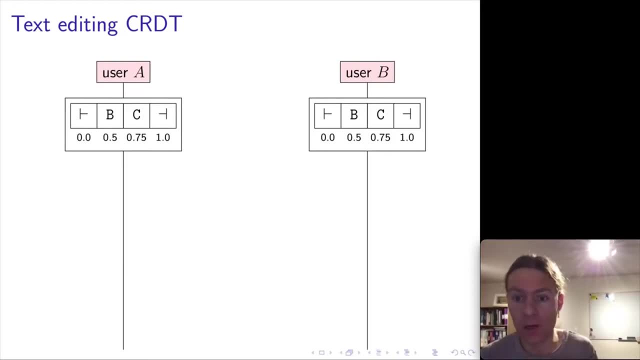 in our case, like the index 2 suddenly has to move along to index 3, and so we have to keep track of everything in order to perform that transformation. as an alternative, we could simply not use indexes in the first place, and instead of using indexes to refer to the places where we're inserting. 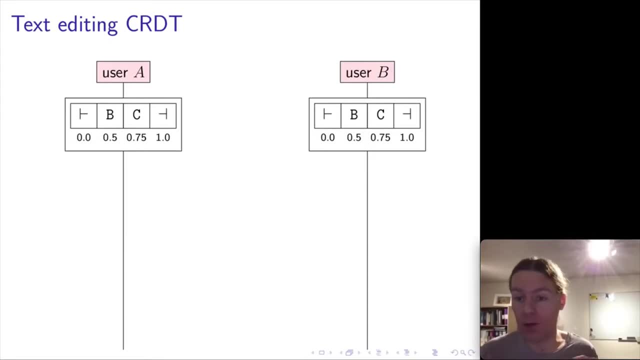 or deleting characters. we could use some other construction. so let's say we're just going to give each character in the document a unique identifier, and in my case this unique identifier is going to consist of a rational number, so some kind of fractional number, and it's also going to consider 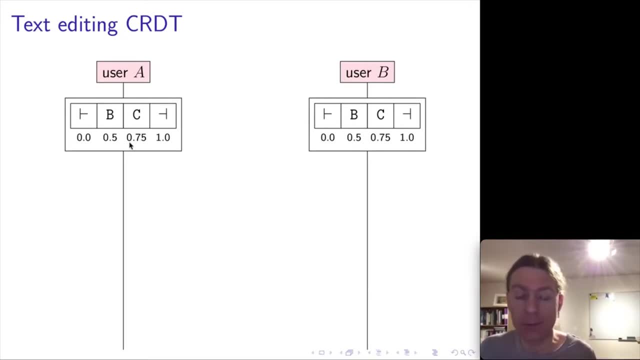 the node ID of the node that inserted a particular character, and we can think of the entire document as consisting of the number line between 0 and 1. so 0 is the start of the document, and here the start of the document is indicated with this little. 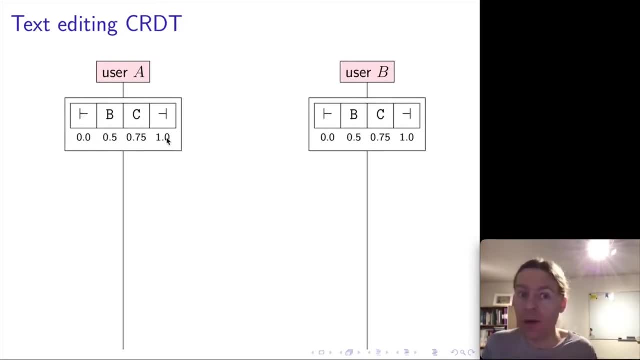 turn-style symbol here, and 1 is the end of the document, which is indicated by this little symbol here. so these two start and end symbols are not actually part of the document. they're just the placeholders to mark the beginning and the end, and in between we're just going to take all of the characters. 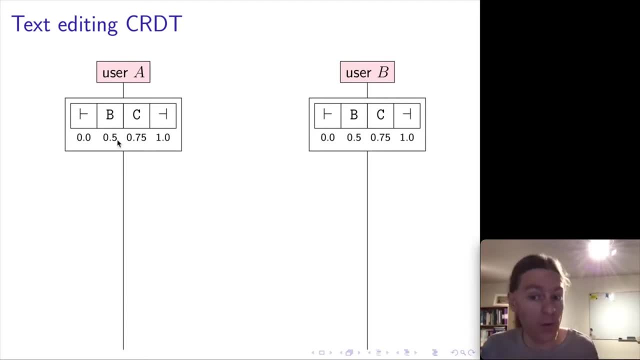 and sort them in increasing order by the number that's associated with them. we're going to call this a position number and then, when we put the numbers in that order, we will just get the document in the order that we expect. okay, and so here let's say that b has 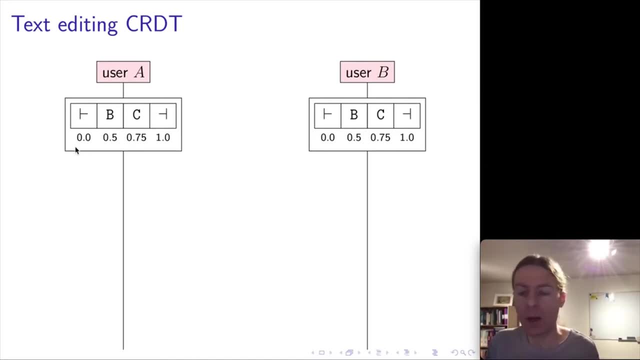 got a value of 0.5. the way we got that is well. we wanted to insert b as the first character in the document, so we just picked halfway between 0 and 1 and said, okay, b is going to have 0.5. then we wanted to insert c. 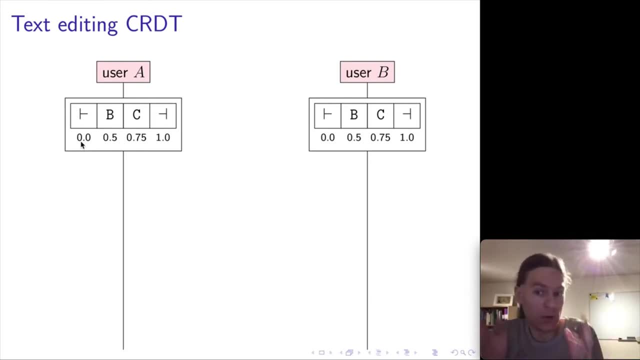 between 0.5 and 1.0. so we gave it a position number of halfway between 0.75. and so let's say now that user a wants to insert the character a before the b, so it's now going to pick a number halfway between 0. 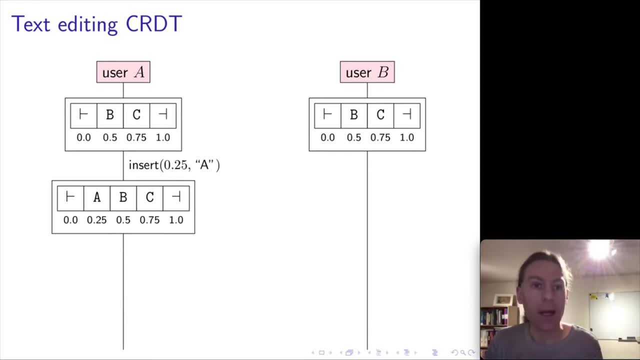 and 0.5, so it's going to be 0.25, and concurrently the user b on the right hand side- it wants to insert the letter d here- between 0.75 and 1.0, so it's going to pick halfway between. 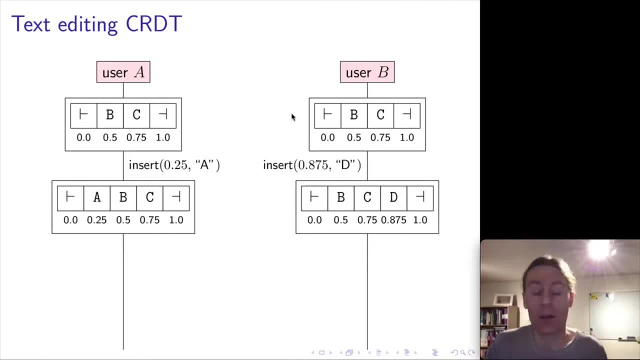 which is 0.875. now you can see, you can keep subdividing these intervals to be smaller and smaller. if you use regular floating point numbers, then you will eventually run out of precision and you will just end up with all of the numbers being equal. so that won't work. so you do have to. 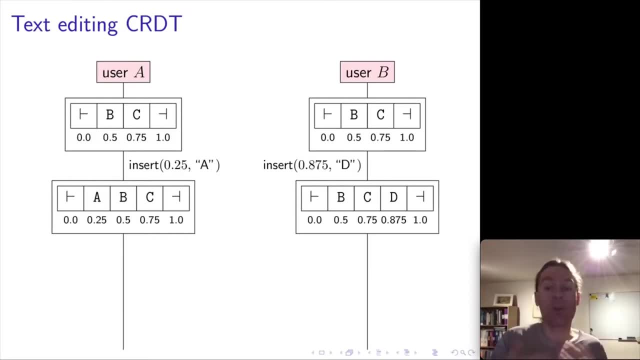 use arbitrary precision arithmetic in order to make this work. but assuming that you have a suitable number library that performs arbitrary precision arithmetic, then you can take these operations and you can just send them over the network in a straightforward manner. so this insertion here of d at position. 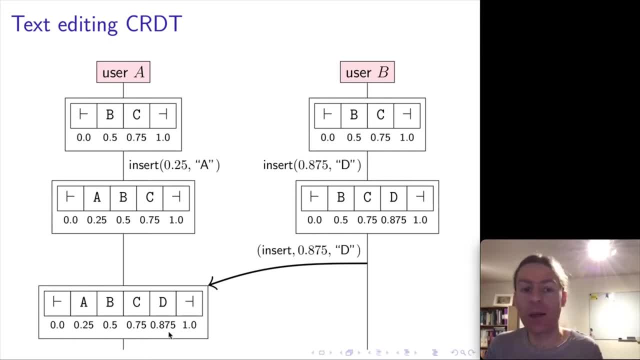 0.875, you can apply here on the right hand side, and 0.875 will slot in just in the right place, just where you expect it to happen. and likewise in the opposite direction, the insertion of a at 0.25: it will just slot in into the right place. 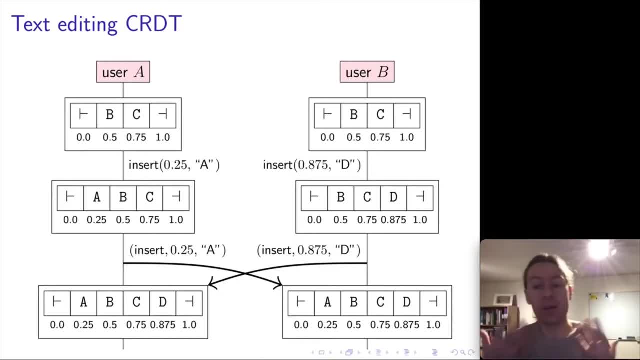 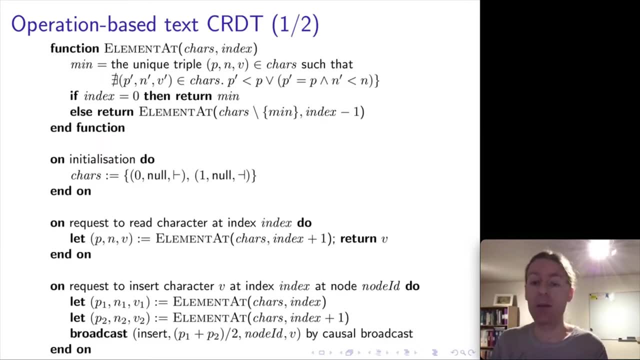 so this is actually a very simple way of achieving the same property, but without all of this complexity of operational transformation. and here is the algorithm that does this. so this comes on two pages. this is the first page of this algorithm. first of all, I want to define a function. 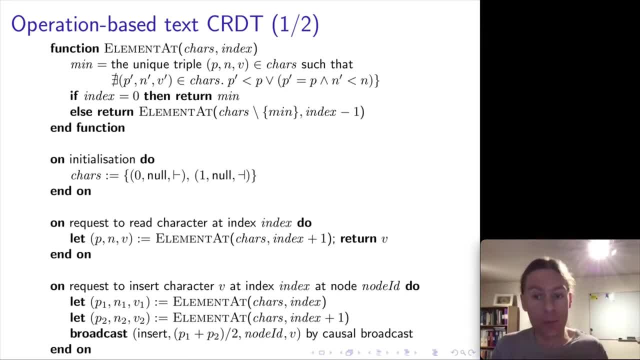 that, given an index into the list, it will find the appropriate element based on the ordering of these position ids, and that's done with this function here. so the way this works is that first of all, we want to find the minimum element in the set of characters, and so we're going to find 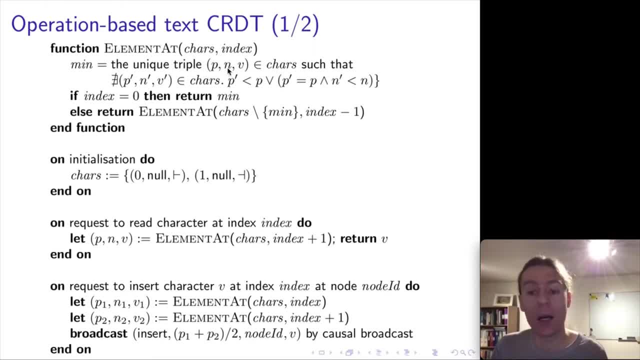 the minimum element that has some position identifier p, node id n and value v, and we're going to find the smallest one, which is the element such that there does not exist another element in this set of characters with a position identifier p prime that is less than p. alternatively, 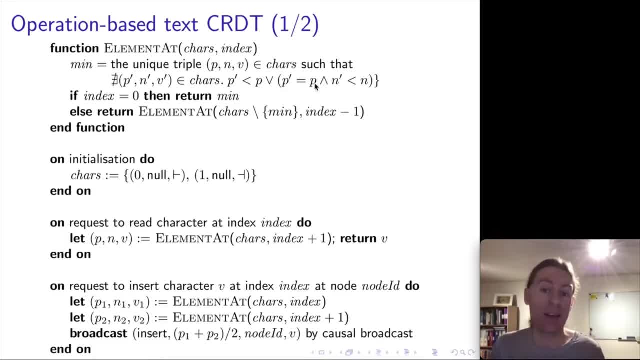 we also don't want that to be a position identifier with the same position number and a lower node id. so the purpose for this is that you could actually end up with two characters having the same position identifier if two different users concurrently insert a character at the same position, and so they will. 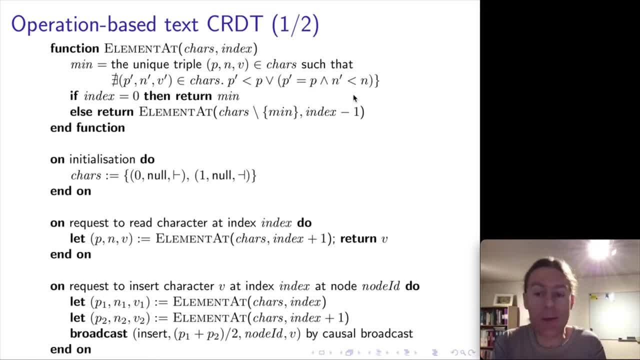 calculate the same position number, because you're just doing halfway between between the two endpoints, and so in this case now we have to do a tiebreaker, and the tiebreaker is going to be based on the node that inserts a particular character. so here this gives us a total ordering over all. 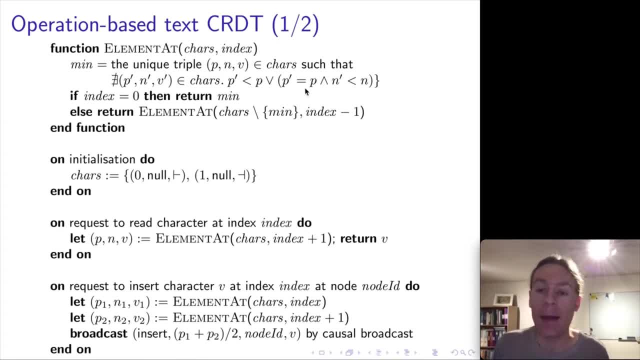 of the characters, where we first sort by the position number and for any characters that have the same position number, we secondarily sort by the node id, and this expression here finds the minimum of all of these characters, and if the index that we're looking for is 0, then we're just going to. 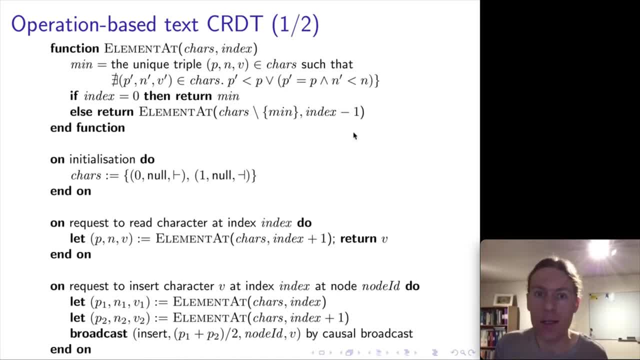 return that minimum. otherwise, if we're looking for an index of 1 or greater, we're going to call this function recursively. we're going to remove the minimum element from the set. so now the next minimum is going to be the next one up and we're going to 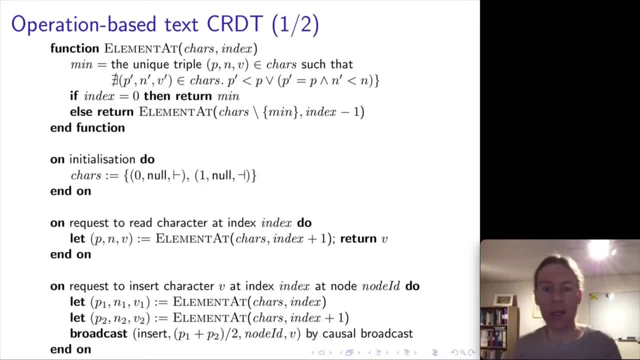 decrement the index and so then recursively, as you keep calling this, eventually index will return 0, index will be 0 and eventually it will reach this first case here of returning minimum. now this is a very slow algorithm, but I just want to illustrate the functionality. in reality, you could implement this in a more 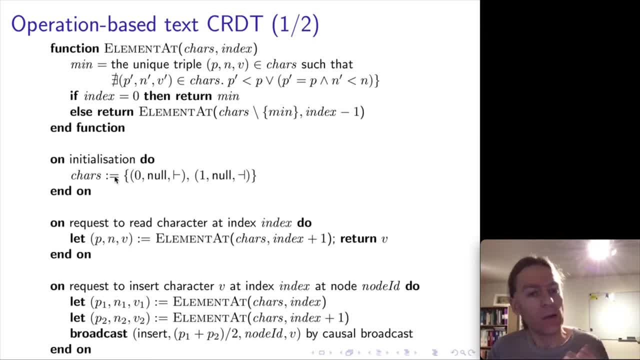 efficient way. but that's not the point here. so let's look at the initialization. so this time we set up our list of characters to start off with the two endpoints. so the endpoints are kind of special marker characters for the beginning and the end with a position of 0. 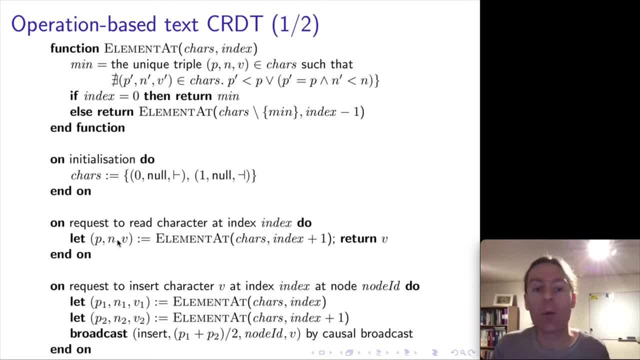 and a position of 1 respectively. when we want to read the character at a particular index in the document, we're going to use this element at function that we just defined and we're going to use index plus 1. the plus 1 just skips the. 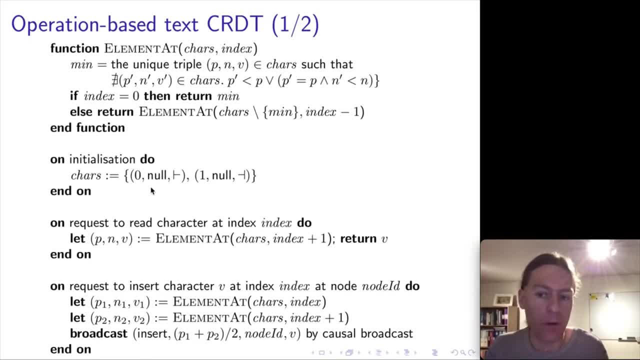 initial character with the placeholder character. so that just makes sure that we actually return a particular index as 0 as seen by the document, not counting that initial placeholder character, and then we return that value. now, if we want to insert a character at some index index and this is executed by: 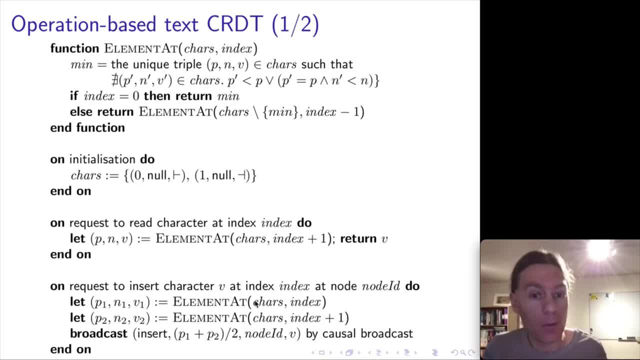 some particular node id. we do exactly what I explained earlier. so we find the element at that particular index and the adjacent element at index plus 1. so this now gives us the position id, position number, just before and just after the position where we want to insert. 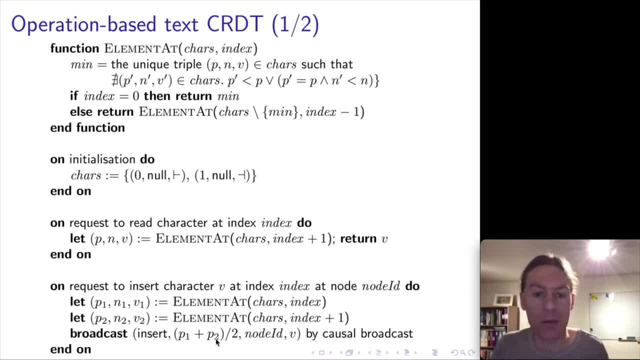 so then we can calculate the halfway point as p1 plus p2 over 2, and that's going to be the position number of the new character. we're going to include the node id, as I said, in order to tie break any insertions that happen to. 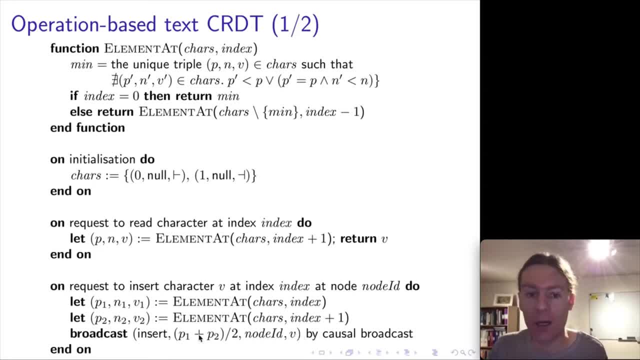 have the same position number and v is the character that's being inserted. so now we're going to broadcast this message here by causal broadcast. I'll explain in a moment why it's causal broadcast this time and not just reliable broadcast. so now, when one of these insertion 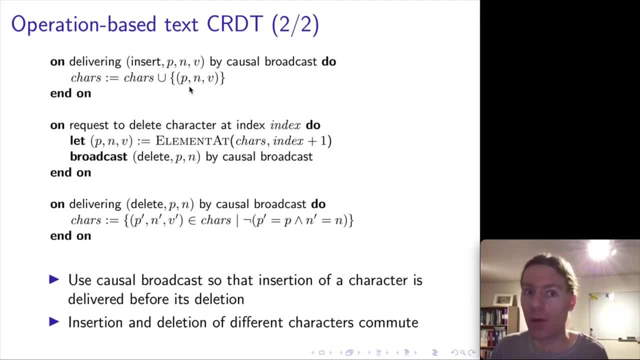 messages is delivered by causal broadcast. well, it's easy. we just add that particular element with the particular position number, particular node id and particular character. we add that to the set of characters and that's all we need to do for insertion if we want to delete a character. 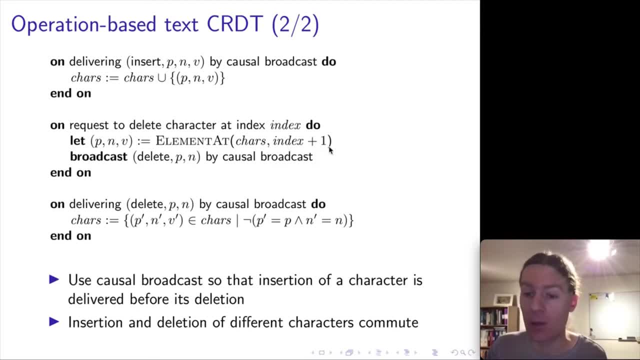 that's also quite easy. we find the element at that particular index again, we do plus 1 in order to account for the placeholder character at the beginning. we get back the position id, the node id and the character at that particular index. and now we're going to. 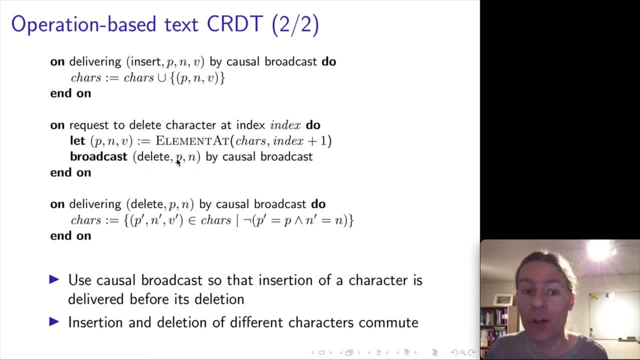 broadcast by causal broadcast a message containing the position identifier and the node id, because, taken together, the position number and the node id are going to uniquely identify a particular character in the document, and so that's uniquely going to tell everybody what is the character that we want to delete. 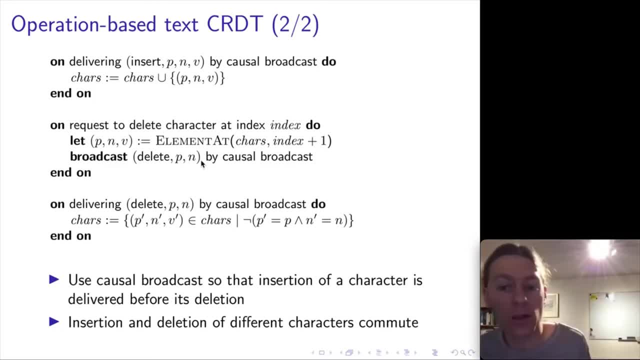 without referring to it by index. so we don't need the operational transformation. and now, when we deliver one of these deletion operations here by causal broadcast, well, we are just going to remove from the set of characters any character that has exactly the position number p and the node id. 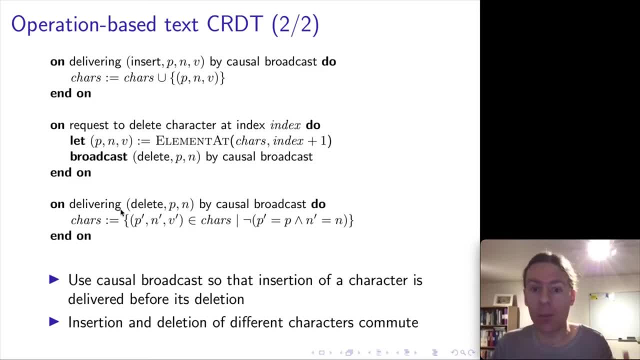 n in the deletion message, and so this is just going to update the set and remove whatever that deleted character was from the set, if it's still there. of course, it could happen that several users concurrently deleted the same character, in which case deleting it several times is the same as. 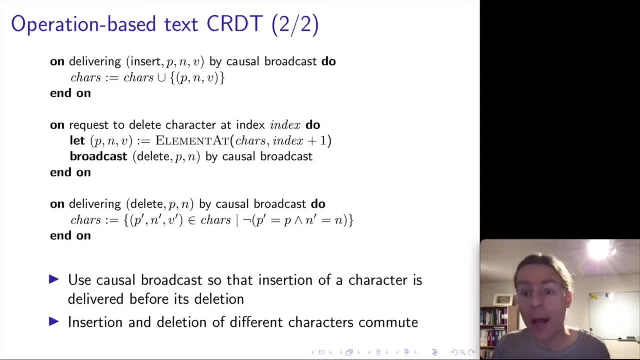 deleting it once it's just gone in that case, and this is enough. this is a CRDT that ensures strong eventual consistency for a text document. the reason I use causal broadcast here rather than reliable broadcast is because of the deletions, and so here we have to be. 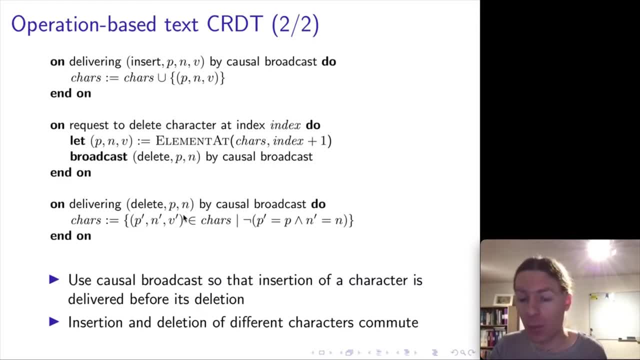 sure that, when we're deleting a character, that deletion operation happens after the operation that inserted the character, because it only makes sense to delete a character that has been previously inserted, and so, in this particular algorithm, it's not safe to reorder the insert and delete of the. 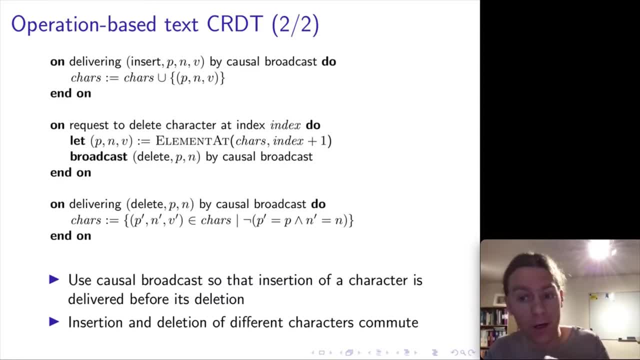 same character, because if we did the delete first and then the insert, there's no record of that delete having happened, and so we would end up then with the delete not taking effect, and so this would not be safe. but we can use causal broadcast in this case. 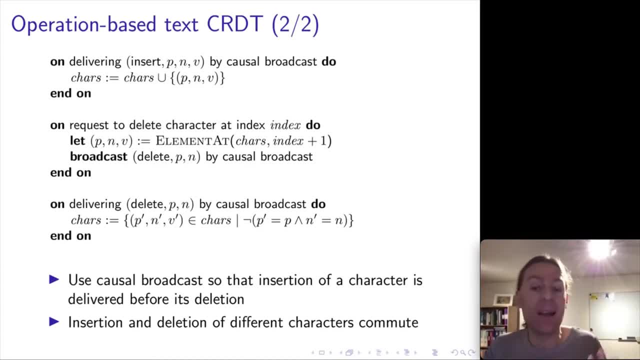 and because the deletion of a character always happens causally later than the insertion of that character, the insertion always must happen before the deletion, and so therefore, all of the nodes, all of the replicas, will deliver the insertion before they deliver the deletion, and therefore the deletion then will have the desired effect of actually 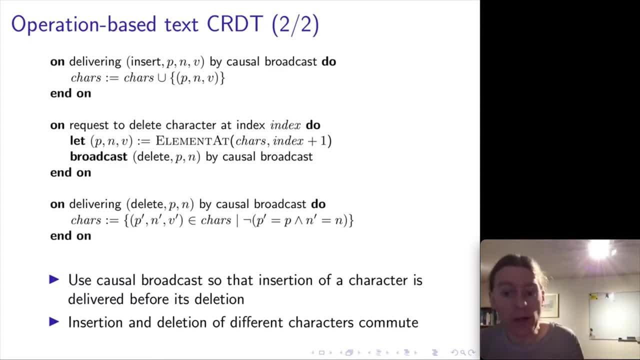 deleting the character and otherwise for any insertions of deletions of different characters. insertion and deletion just commute, that's easy. insertion is just the set union operator which commutes, and so on. you can even convince yourself that these procedures here commute and as a result it's a CRDT. 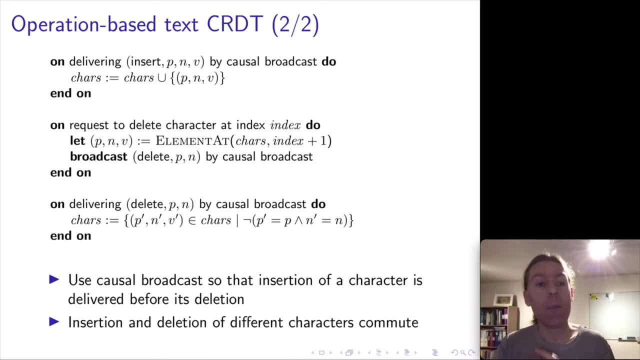 and we get strong eventual consistency again. so here making this efficient can be the challenge, because in this case now we're carrying along these potentially quite large arbitrary precision numbers with every single character. so how you take this algorithm and actually make it really efficient so that you can build. 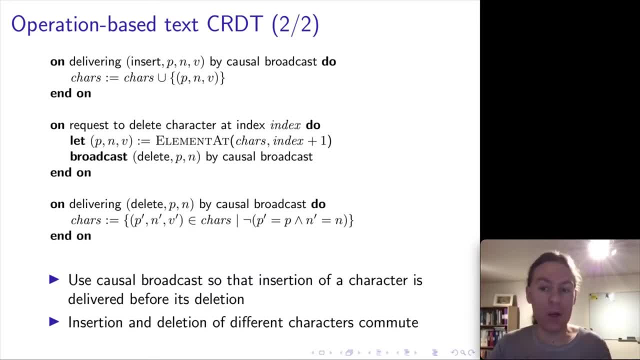 something like Google Docs in practice. that's an interesting area of research. in fact, it happens to be one of my areas of research, but this really goes beyond the scope of this particular course. I just wanted to give you the flavour of how these CRDT algorithms work, so 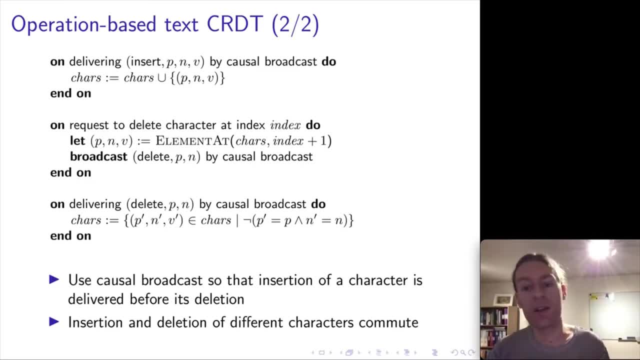 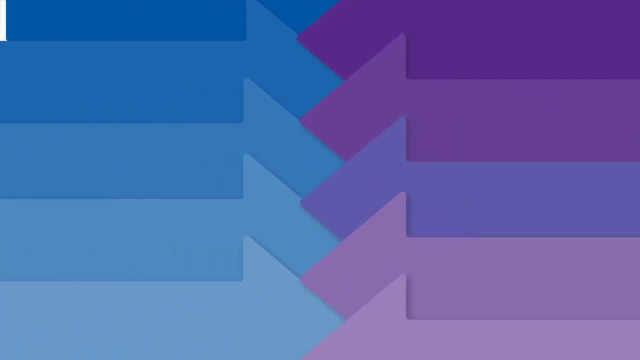 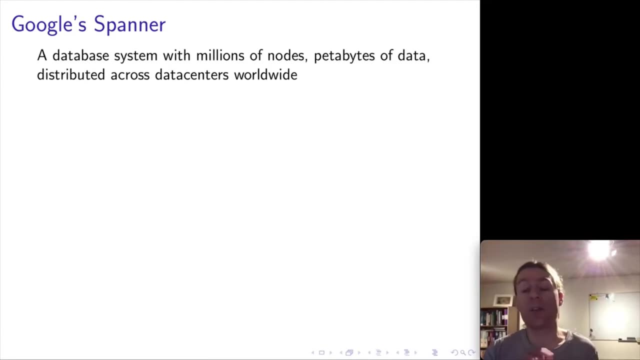 that's all I wanted to say about collaboration, software, CRDTs and operational transformation, so we've talked about these. eventually, consistent systems. for the last section, let's switch back to very strongly consistent systems, and what I'd like to tell you about is a very interesting database system. 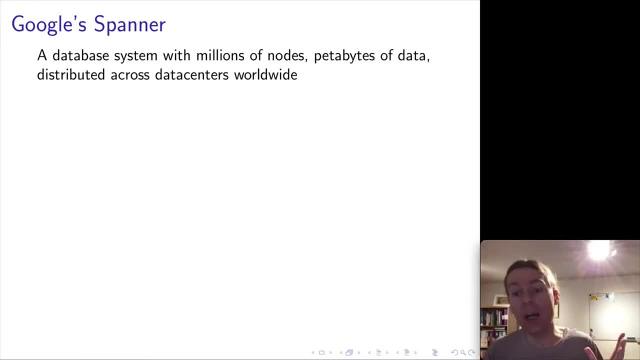 developed by Google called Spanner. this is a very large scale database system. it's intended to be used with huge amounts of data, with millions of nodes spread all around the globe, and nevertheless, despite this huge scale, we want to achieve very strong consistency properties in this database in particular. 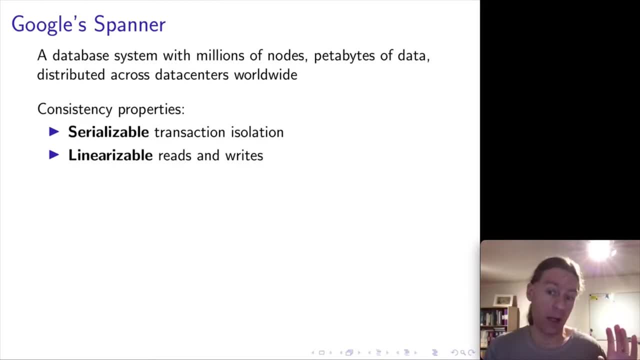 the classic that we've seen. we want serializable transaction isolation, the strongest isolation we can get. we want linearizability for reads and writes. that means we're always going to see an up to date value from any value written. moreover, we need to support sharding, which means that 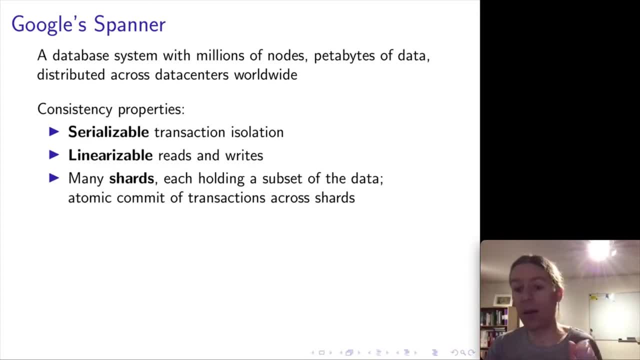 this huge amount of data, which is far too much to store on a single node. we have to split into subsets of data. each node has a replica of a subset of the data, so that now you can distribute the data across all of these different nodes. but this now means that you might have a transaction. 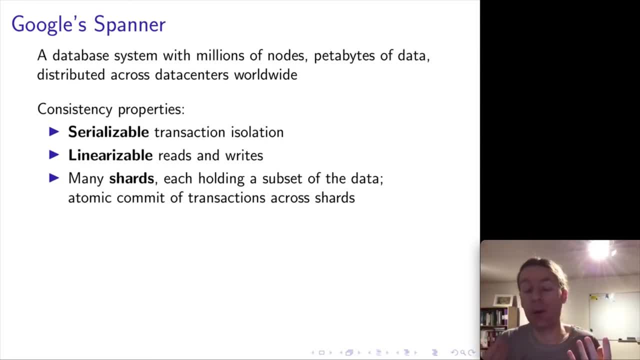 that needs to read and write data on multiple nodes and, if this happens, distribute a transaction like this. we need atomic commit so that any changes made by a transaction will either be committed on all of the nodes or aborted on all of the nodes. so all of these classic properties we want. 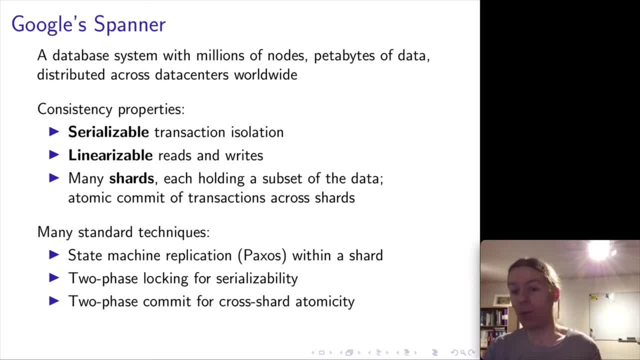 and a lot of the techniques that Spanner uses to implement these properties are equally classic, standard algorithms. so in order to replicate the nodes within a shard, it uses state machine replication. it uses the Paxos consensus algorithm rather than Raft, but they are reasonably similar and the principles are very much the same. 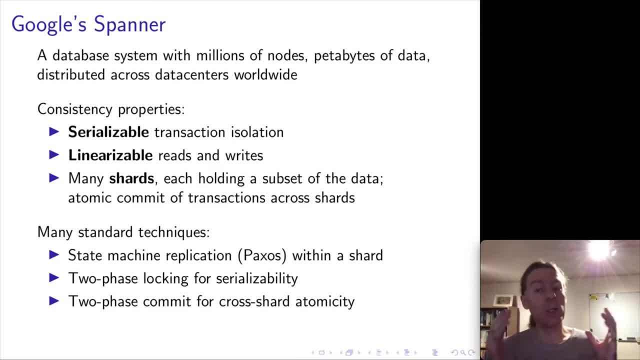 in order to achieve serializable transaction isolation, we use the classic two-phase locking. that means, for any reads, we take a shared lock on any data that we want to read and for any writes, we need to take an exclusive lock on any data that we write and we need to hold those locks until. 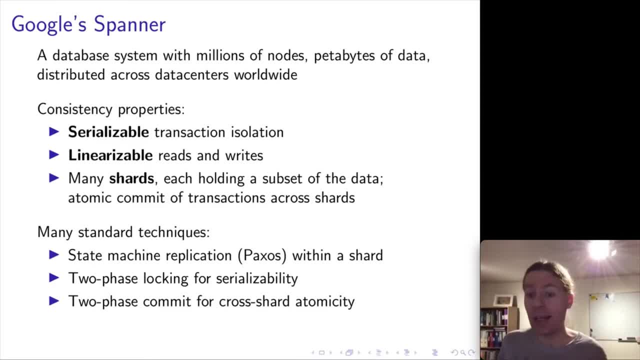 the transaction commits. finally, in order to achieve atomicity across multiple shards, we do the classic, we do two-phase commit, exactly like we saw in the last lecture. so so far, you know, actually implementing all of these things well is still a significant engineering challenge, but there's nothing conceptually. 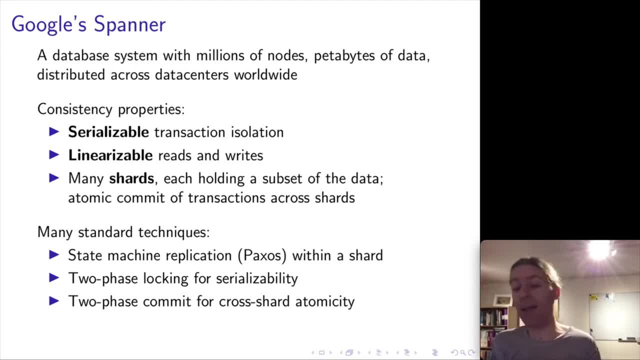 very new here. where Spanner gets interesting is that it has support for read-only transactions that take no locks. now, this is special because if you remember what two-phase locking means means, if you want to read any data, you first have to take a shared lock on that data. 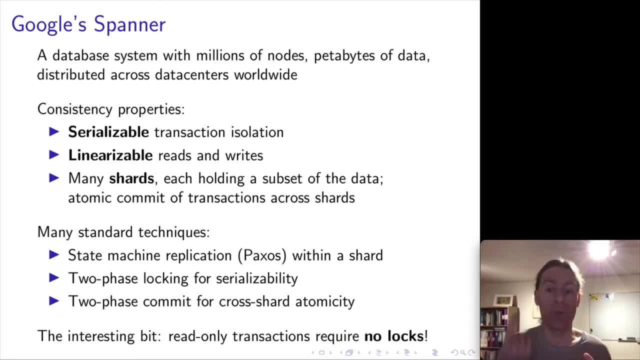 and the shared lock is going to prevent any other transactions from updating that data. but now in real systems you often get very large read-only transactions. so, for example, taking a database backup is a very large read-only transaction that needs to read essentially the entire database. that's what a backup is. it's a copy of. 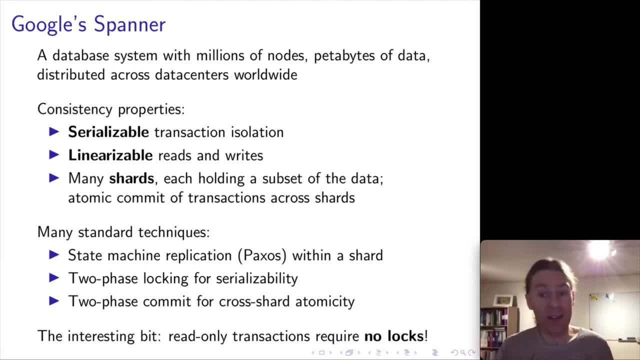 the entire database, and so this backup might take a long time. and if you have to take a shared lock on the entire database for a long time while you're doing a database backup, then users are not going to like that very much, because it means that no rights. 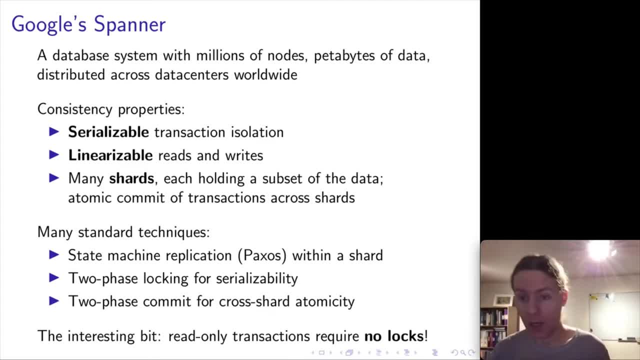 can be made to the database for the entire duration of this backup, so that would simply not fly in practice. we have to have some way of doing read-only transaction that does not require any locks, and the interesting thing about Spanner is how it enables those kind of read-only transactions. 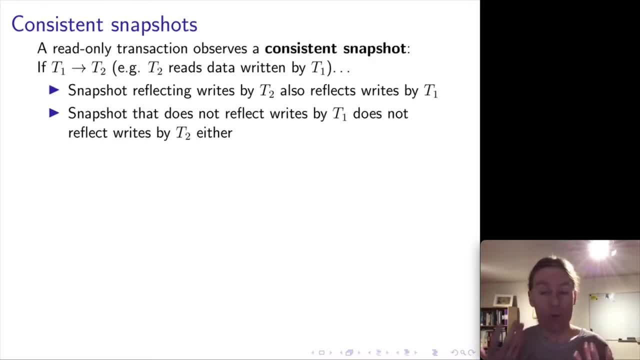 so the way this works is that a read-only transaction can read from what is called a consistent snapshot. so a consistent snapshot is a way of essentially looking at the entire database at one point in time, and the way it does this is using timestamps. now the important thing. 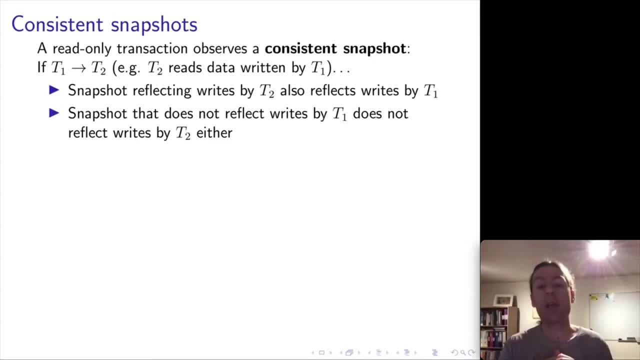 for this consistent snapshot. the consistent aspect is that it means we're consistent with causality, and so what I mean with this is if we have two transactions- T1 and T2- and if T1 happened before T2, then if we have a snapshot that contains 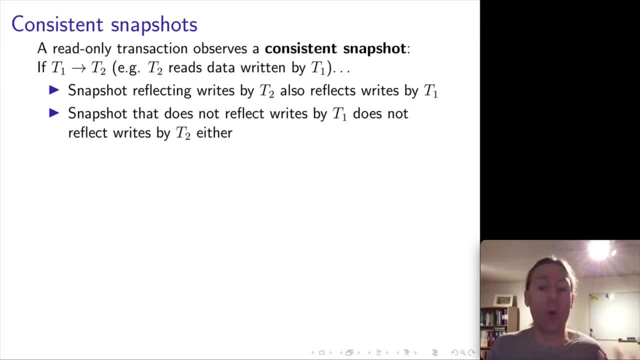 the rights that were made by T2, then that snapshot must also reflect the rights by T1. that means that we don't end up with some of the causal dependencies missing from the snapshot. likewise, if the transaction contains the rights by does not contain the rights by T1. 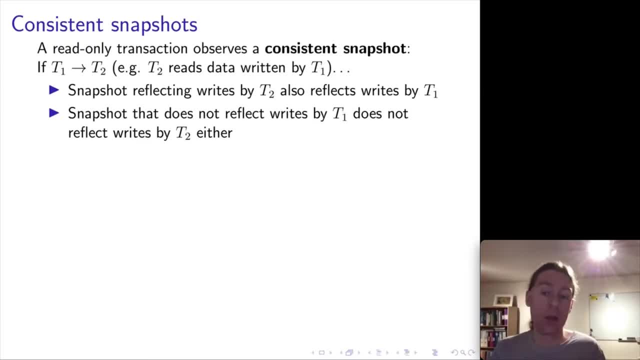 then it will not contain the rights by T2 either. so this goes both ways. now this is what we mean with a snapshot being consistent with causality. it just means that we don't have bits of the bits of the database snapshot that don't make sense causally. so if the snapshot 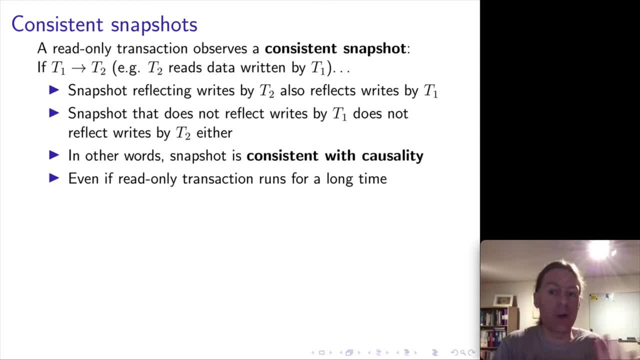 contains the cause, then contains the effect, then it will also contain the cause of that effect, and so we want to ensure this consistent snapshot, even if the read-only transaction runs for a long time and without taking any locks, and the way this is done is through approach called. 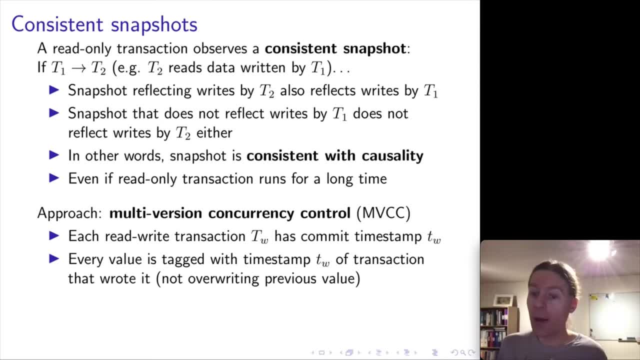 multiversion concurrency control, or MVCC. now, MVCC is actually a very common technique. it's used in lots of databases, including Postgres and MySQL, for example, and the way it works is it attaches a timestamp to every transaction, and this let's say that a read-write transaction has 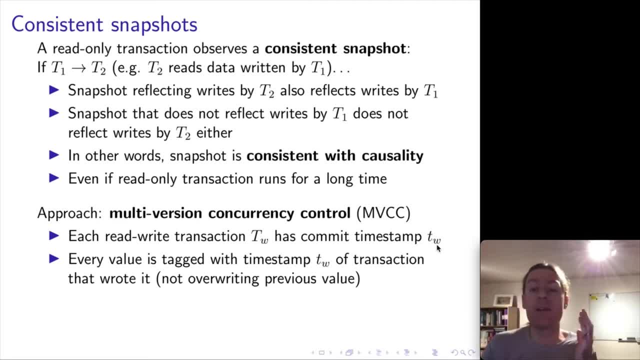 a timestamp, TW, and that timestamp is assigned at the time when that transaction commits and when we have a read-only and sorry, and then any data that is written by this transaction TW is that any data is associated, it's tagged with the transaction timestamp, with the commit timestamp of the transaction that wrote it. 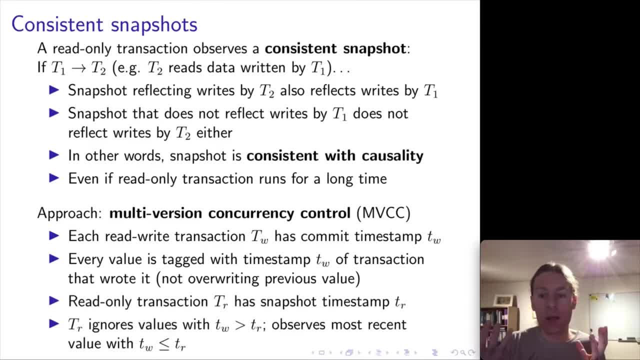 and now if we have? if we have an object that is being updated by a transaction, now we won't simply overwrite that transaction in place, but we will. we won't simply overwrite that object in place, but we will make a new copy of that object and that new version of the object. 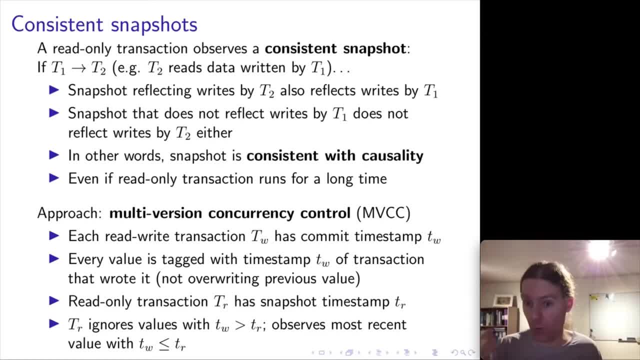 will be tagged with the timestamp TW of the transaction that wrote that version. but we will keep the old version of the object in place in case there's a read-only transaction that actually needs to read the old version. and now we associate each read-only transaction also with a timestamp and that 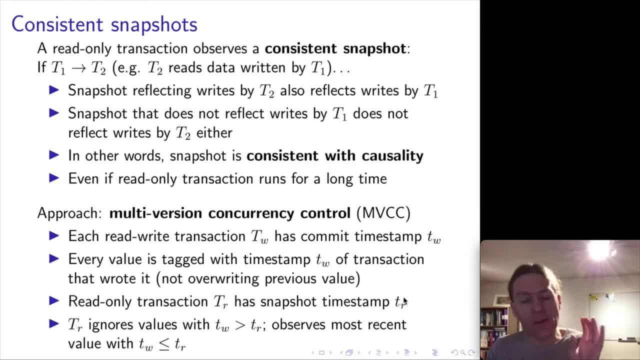 timestamp identifies the snapshot at which, which is the point in time at which that snapshot is observing the database. and now, if the read-only transaction wants to read a particular object, it looks at the different versions of that object, each version tagged with a timestamp. it ignores any. 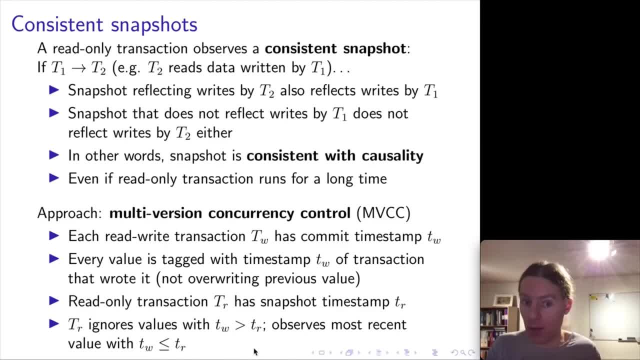 versions that have a timestamp greater than the snapshot timestamp, and then of those versions that have a timestamp less than or equal to the snapshot timestamp, it picks the highest, and that is the version of the object that this transaction is going to see, and so this now allows. 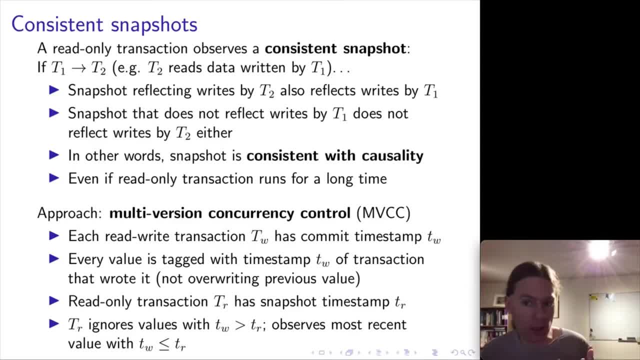 the read-only transaction to simply ignore any writes made concurrently. so the read-only transaction is going to see the entire database as of this particular time TR, regardless of whatever writes happen otherwise and without taking any logs. now this works. this is very standard MVCC. what is interesting about the way? 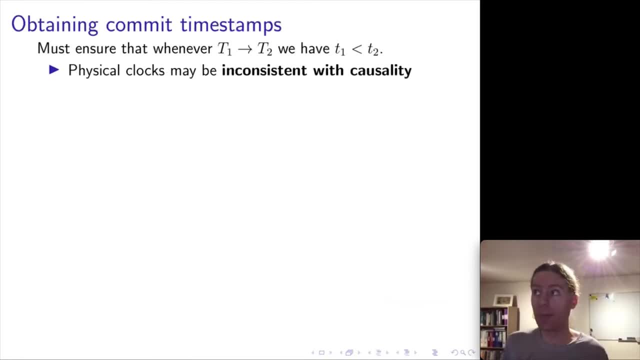 Spanner implements. this is the way these timestamps are generated. so, in order to ensure that our timestamp, our snapshot, is causally consistent, what we require is that if transaction T1 happened before T2, then the timestamp of T1 has to be less than the timestamp of T2, because 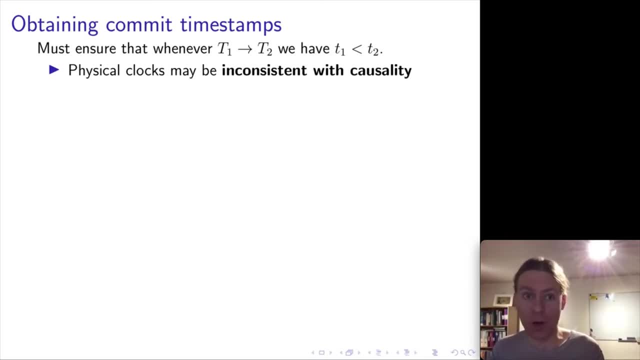 that's what this ordering property in MVCC is relying on, and recall from the lecture, when we talked about physical clocks, that physical clocks do not actually guarantee this. so with physical clocks, you could end up in a situation where transaction T1 happened before transaction T2. 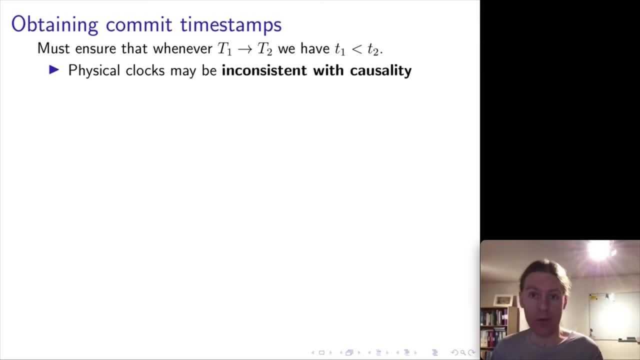 but T2 had a lower timestamp than T1 and we don't want this. so we have to take some other measure to ensure that our timestamps are consistent with causality. the obvious answer is: well, why don't we use logical clocks? because that's exactly what logical clocks were designed to do. unfortunately, logical clocks like Lamport clocks are not actually sufficient in this case either, and the reason for this is by this particular example. so let's say that here we have two replicas, A and B, and the user executes some transaction- T1 on replica A. 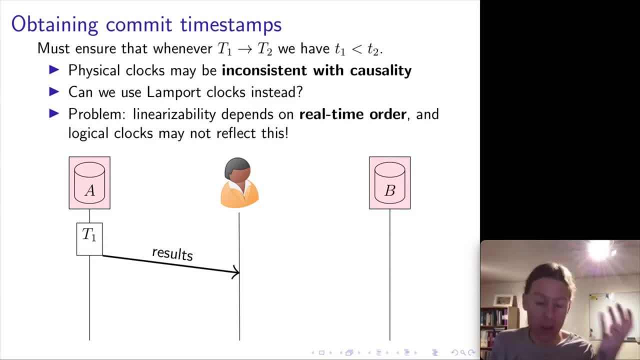 and then views the results of that transaction. so the user has the results on the screen. then the user chooses to perform some action and that action results in some transaction T2 being executed on replica B. so here very clearly it's the case that T1 happened before T2. 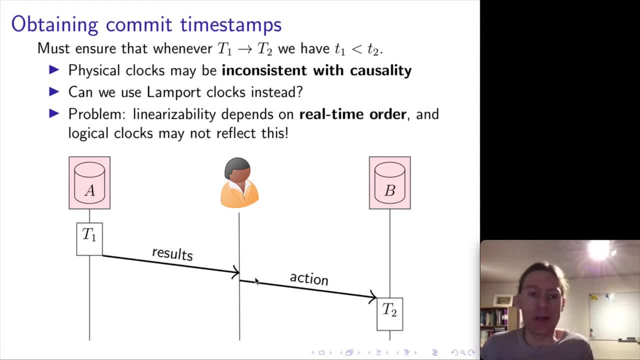 because there's this user communication in the way. the communication ensures that the action depends on the results from T1. so definitely in this case we want T1 to have a lower timestamp than T2. but if we're using Lamport clocks, well, remember the way Lamport clocks 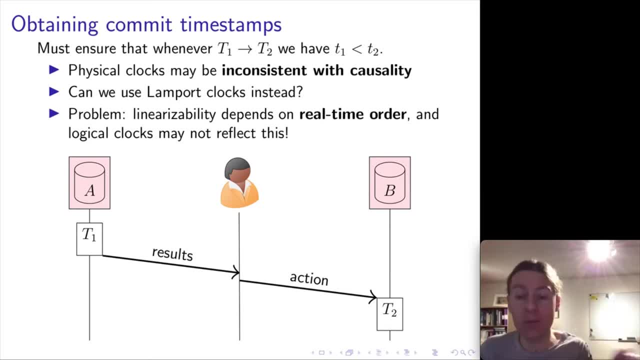 work is they work by attaching a timestamp to every message that is sent over the network and then, when you receive one of those messages, you bump up your own local clock to the maximum of the local timestamp and the one you received. but in this case, here, in this example, 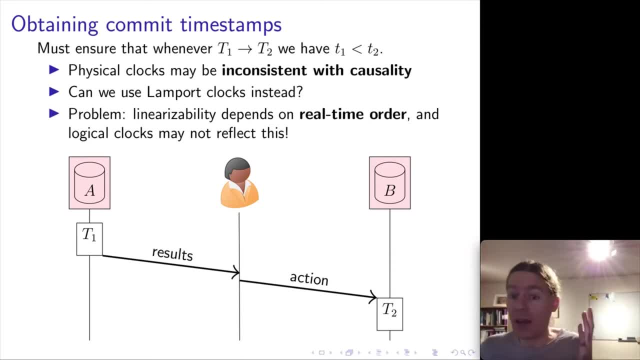 there might not be any communication between replicas A and B, so replica A may never send any message to replica B while this is happening, because the communication is going via a user and so there's nothing that can propagate our timestamps from A to B, because there's no message. 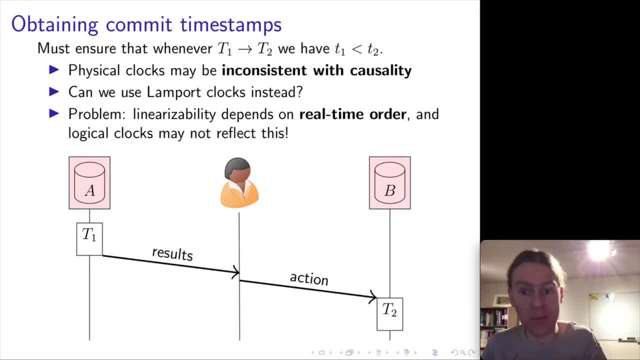 that can propagate the timestamps and we can't rely on the user to type in timestamps or something like that here. so replica B may not actually realize that it needs to have a timestamp for T2 that is higher than the timestamp of T1, because there's nothing passing. 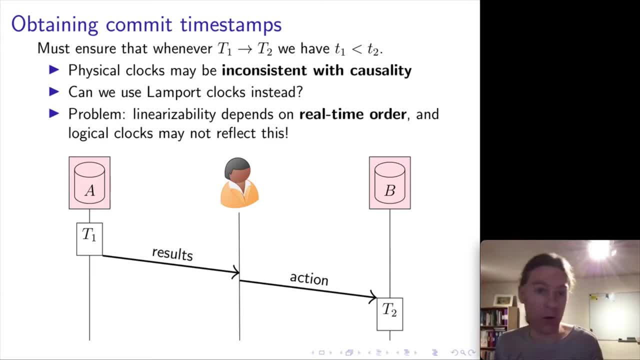 along these timestamps that we would need for Lamport clocks. so Lamport clocks don't work either. so what can we do in this case? well, we can go back to physical clocks, but we have to adjust the physical clocks and do some extra measures in order to make sure that this 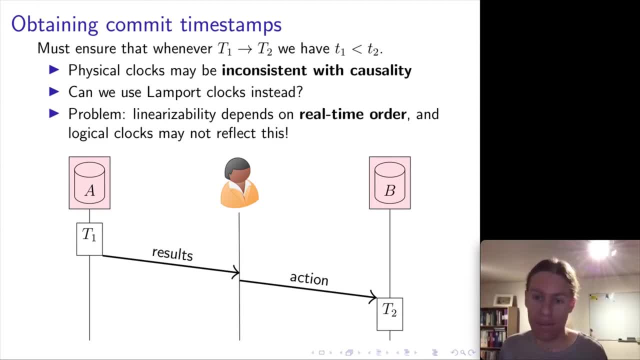 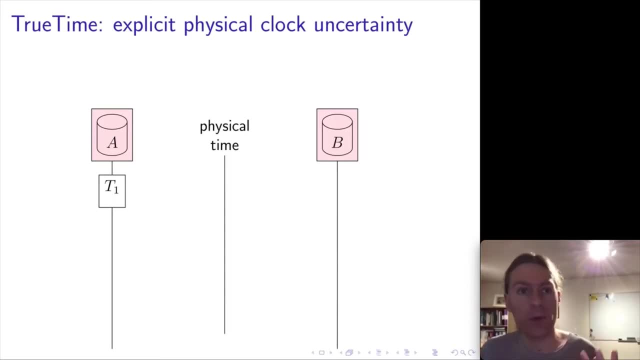 causal ordering property here is satisfied, and the way Spanner does this is using a system called TrueTime. so TrueTime is a system of physical clocks that explicitly captures uncertainty in the timestamps. so this is the really interesting bit about Spanner and the way this works is. 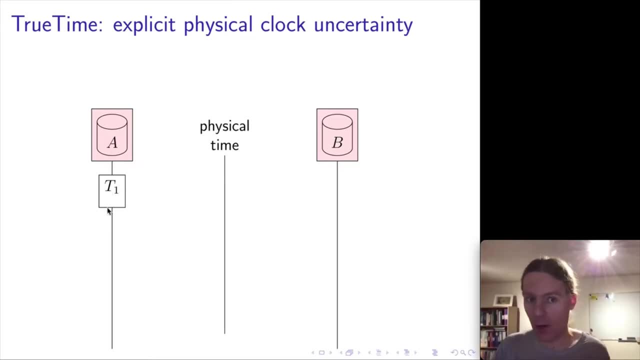 say, replica A wants to commit transaction T1. at the time when it wants to commit that transaction, the replica requests a timestamp from TrueTime and TrueTime does not reply with simply a single timestamp, but it returns a range. it returns two timestamps: the earliest possible and the latest possible. 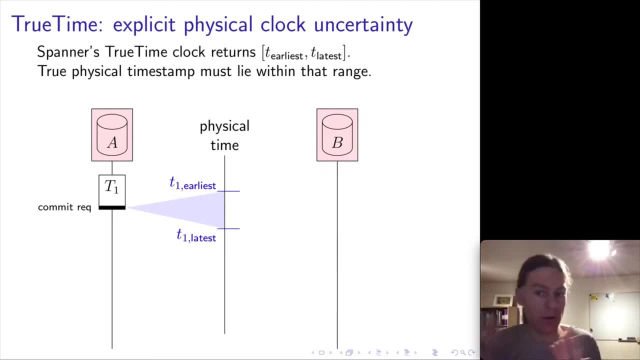 and so, because of the uncertainties we have, there's no perfect synchronization of clocks in the systems that we have. we can never be totally certain about what the current real physical timestamp is, but we can track all of the errors in the system and all of the uncertainty in the system. 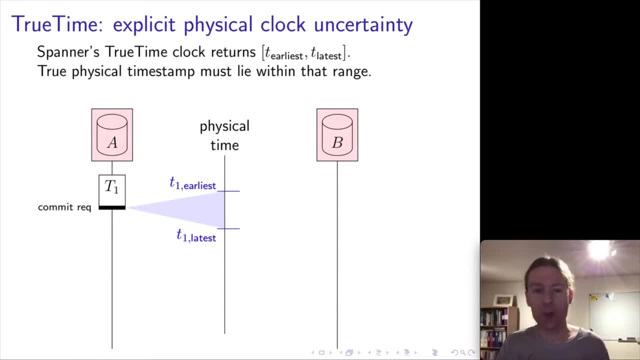 and if we correctly account for the uncertainty, then we can be sure that the real physical timestamp will be somewhere between this earliest possible and latest possible, with very high probability. so this means we have to track, like the round trip time to the clocks server we need to account for. 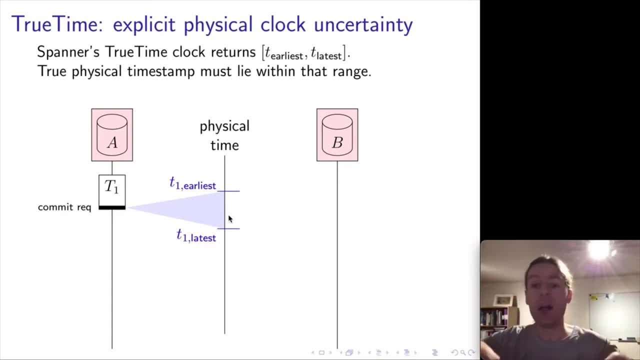 clock drift, we have to account for any sort of things that might cause error. add up all of those potential causes of error and factor this all into a single uncertainty interval so that we know that the real timestamp lies somewhere in between this earliest possible and the latest. 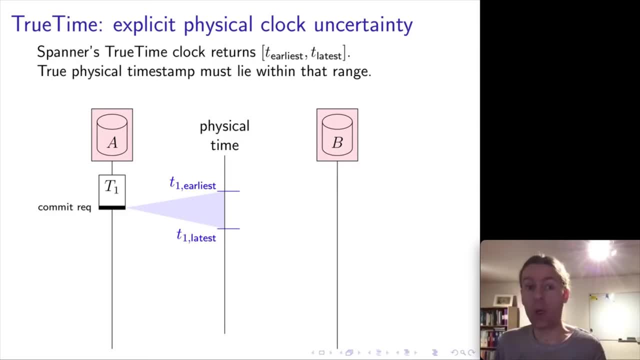 possible. and now what Spanner is going to do is it gets this pair of earliest and latest from TrueTime, and now it's going to wait, and the time it's going to wait is exactly the difference between the two timestamps, and so this length of the 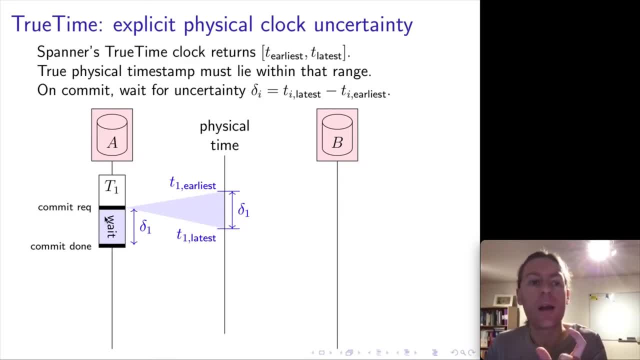 uncertainty time interval called delta1. the transaction is simply going to wait for that time. it's not going to do anything during that time. it's going to continue holding all of the locks. so the transaction is ready to commit. it just hasn't actually committed yet and it's going to wait. 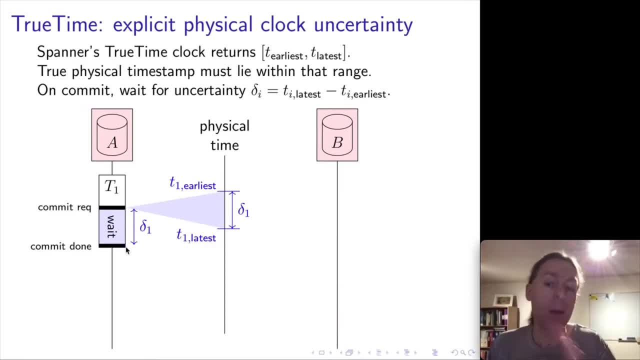 for this period, delta1, and once that time is elapsed, now it commits, it releases all of the locks and it moves on. so this extra wait is the key thing here. now let's say that replica B wants to execute transaction T2. it does the same thing when it's 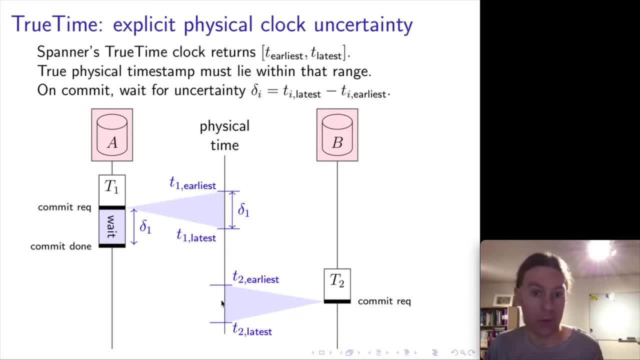 ready to commit. it requests timestamps from TrueTime so it gets back an earliest possible and latest possible, and again it waits out the uncertainty. in this case delta2, the times, the difference between the two timestamps. now, in this case, here we have this real time dependency, so that 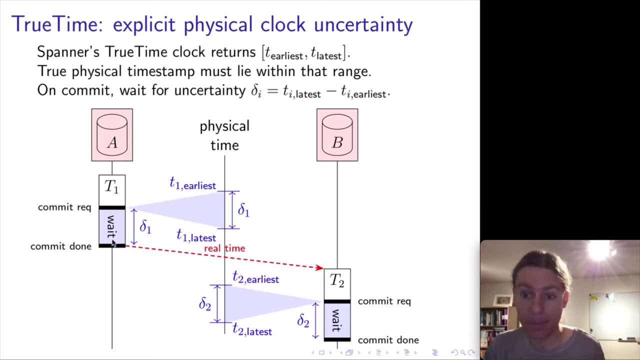 T2 started after T1 ended and the effect that this meeting has had is to ensure that if we have these two timestamps where there's a real time dependency, then their uncertainty intervals from TrueTime will not overlap. and because the uncertainty TrueTime intervals do not overlap, 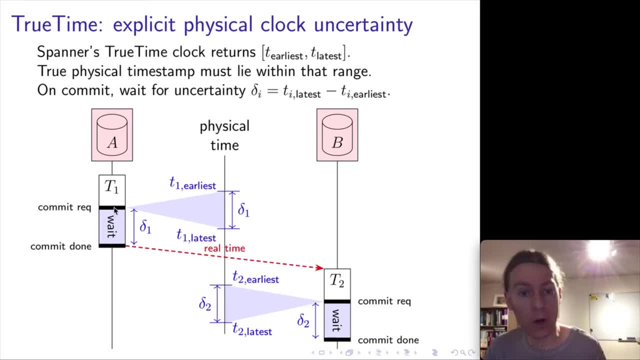 this means now that the commit timestamp for T1 will definitely be a lower timestamp than the commit timestamp of T2. by having these uncertainty periods- non-overlapping- we have got rid of the possibility of the timestamps getting reordered and thus being inconsistent with causality. so the 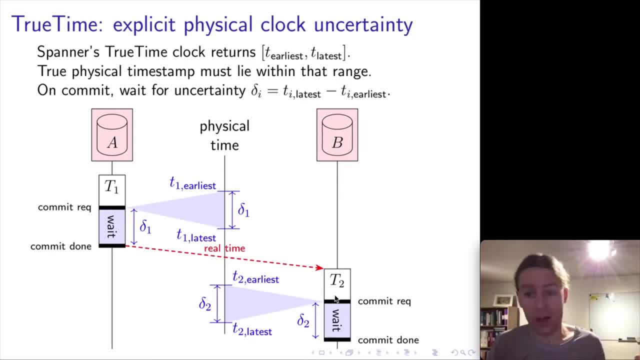 key here is this: waiting, and of course, in a real system, we want to wait for as short time as possible. so we now need to do two things: firstly, we need to precisely quantify the uncertainty so that we know how long we have to wait, and then, secondly, we have to keep the uncertainty as small. 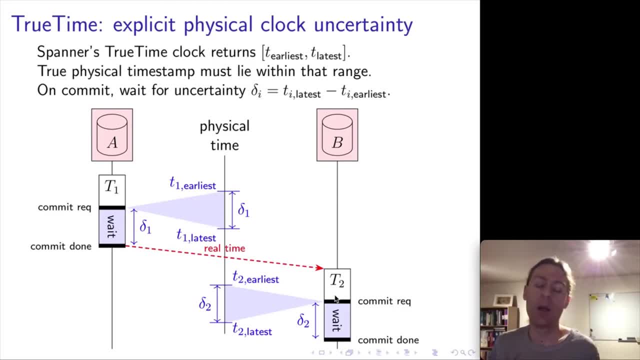 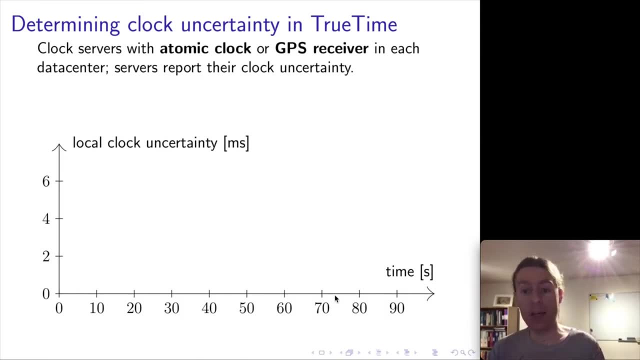 as possible so that our waiting time is as short as possible, and the way that TrueTime does this is by actually putting atomic clocks and GPS receivers in every data center, and these cost some money, of course, but Google has figured out that they are actually affordable enough. 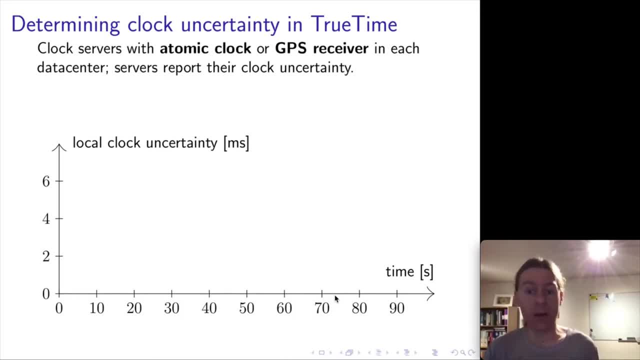 it is alright. you can actually put GPS receivers and atomic clocks in every data center and this gives each data center a reliable clock source. and now every other node in the data center that is not directly connected to these reliable clocks- normal node- just has the usual quads clock. 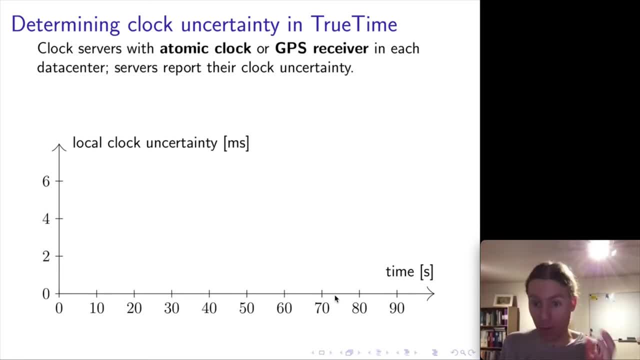 and it is going to periodically synchronize its local quads clock with the time server. that has the atomic clock or the GPS receiver attached, and TrueTime actually performs this clock synchronization every 30 seconds and so every 30 seconds there is going to be like a ping. 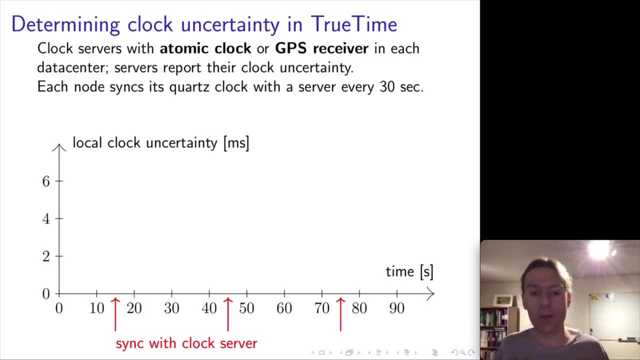 from each node in the data center to its local time server, and the result is that every time that clock synchronization is performed, the uncertainty drops down, because the uncertainty now is just essentially the round trip time to the server, plus any uncertainty that the server had about its own time. and so because 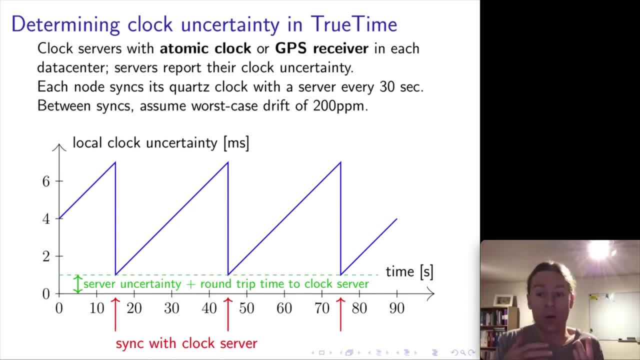 we are assuming that here the time server is in the local data center. locally, the round trip time to the clock server will usually be less than one millisecond, because there are no big geographic distances to be covered here, and so therefore, whenever we sync with the clock server, 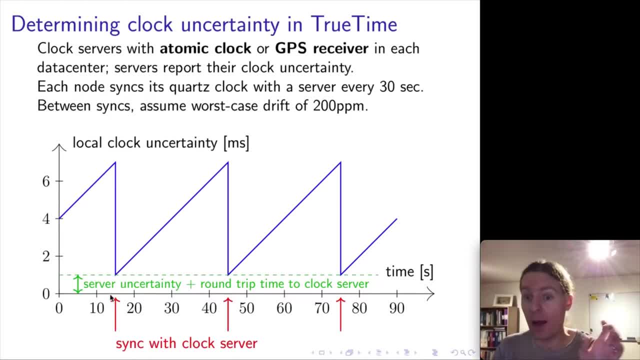 the uncertainty about our clock, about the local clock drops down to about one millisecond and then in between, in these 30 second intervals between the synchronizations. well, it depends on the rate at which the local clock drifts with respect to the actual real time, and so, for this, Google did some measurements. 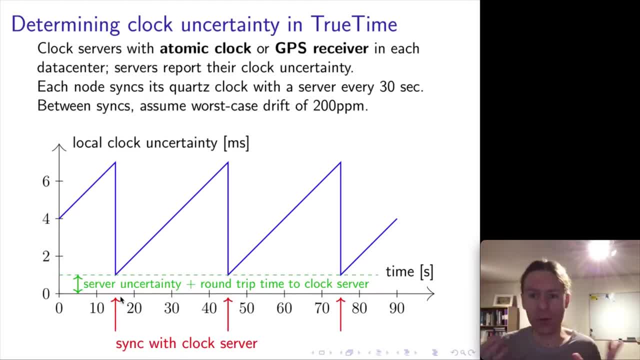 and they figured out what is the worst case clock uncertainty that we have to assume to make sure that all of the clocks have a drift that is lower than this bound. and they figured out that a worst case drift of 200 ppm was a safe assumption to make. 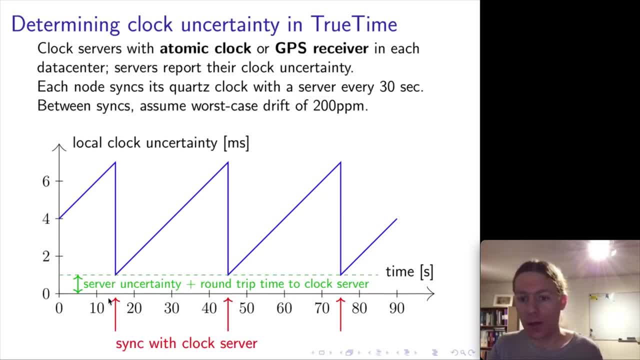 and so this means here that in between these 30 second clock syncs, the uncertainty of each local clock keeps drifting up at a rate of 200 ppm. so this means, over the course of 30 seconds we rack up about 6 milliseconds of clock uncertainty. 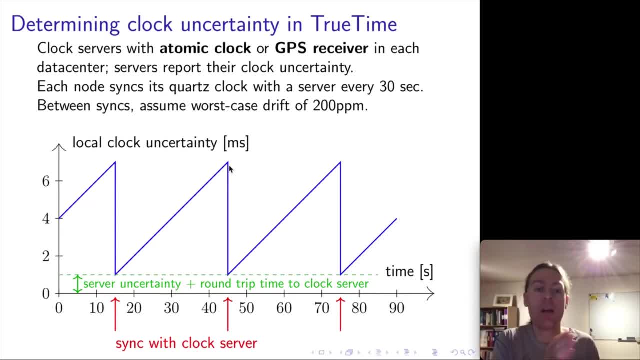 and TrueTime keeps track of exactly how long it's been since the last clock synchronization and therefore it has these uncertainty intervals that keep widening and widening, and widening until the next clock sync, and then the uncertainty drops back down to 1 millisecond, and then they start. 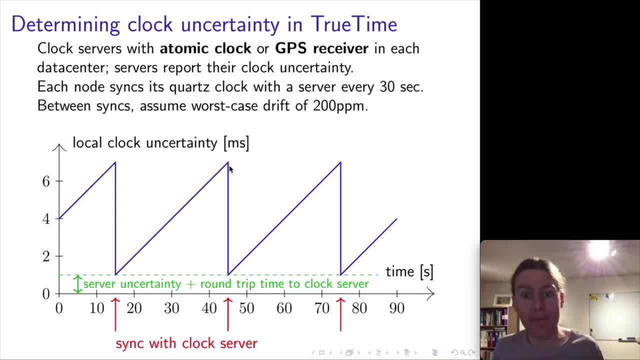 widening again and so on. we get this kind of sawtooth pattern here, and the result is now that we have a very accurate notion of what our clock uncertainty is, which allows us to determine the wait time for each transaction and, moreover, because we're using these local 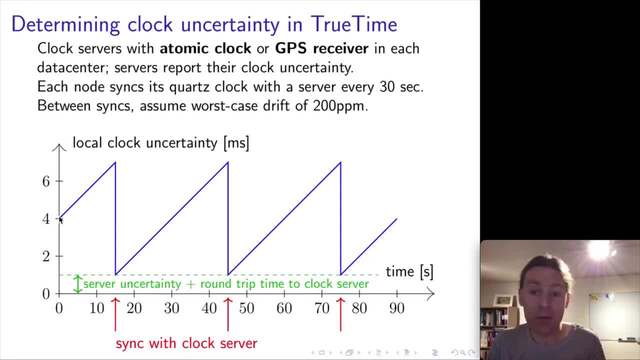 accurate clocks, atomic clocks and GPS receivers. the average time uncertainty is actually quite small uncertainty average, uncertainty interval average length is about 4 milliseconds and so, on average, about 4 milliseconds is the time that the transaction needs to wait before it's allowed to commit. 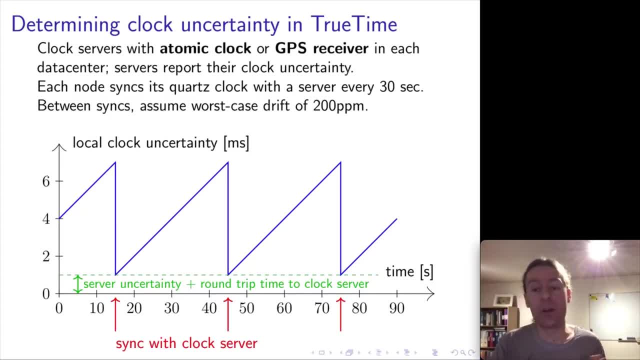 and 4 milliseconds is a pretty short time. actually. it's certainly a lot shorter than the time it would take to do like a round trip time to a data center on a different continent, which would take like 100 milliseconds or more. so this is really the.